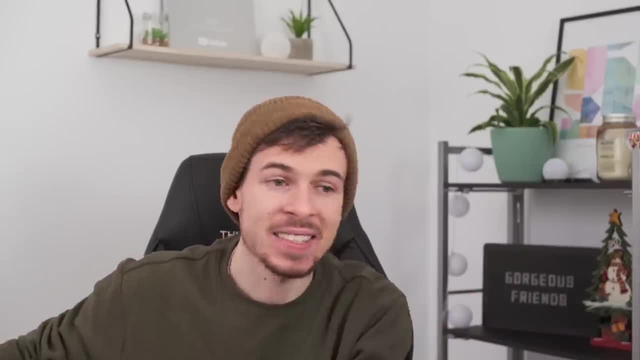 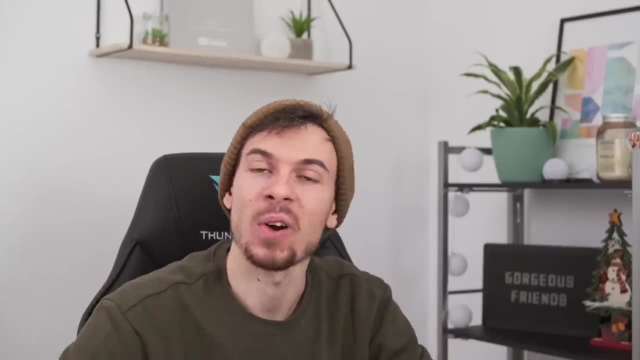 know about HTML and everything you need to know about CSS. So hope you enjoy it. Make sure to let me know what you think And from next week on we are going to go back to our normal routine, just doing fun, creative stuff on this channel. So thank you again. very much for everybody who. 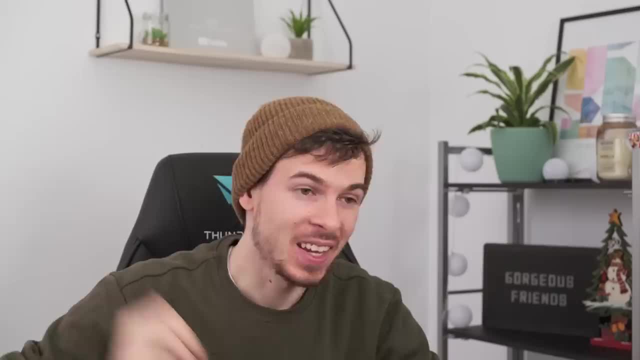 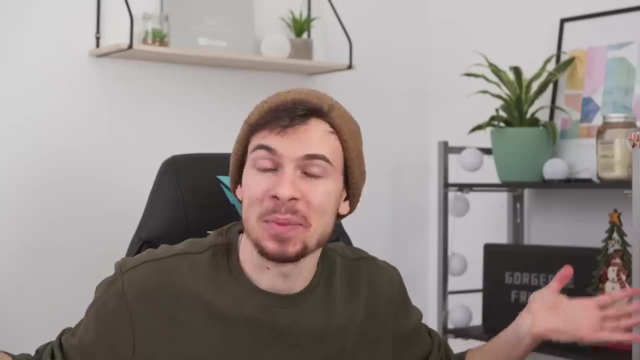 purchased the course. I want to give you a big shout out. And the first day, 350 people joined- awesome, gorgeous friends, So it's unbelievable. I did not expect as much support, So thank you from the bottom of my heart. 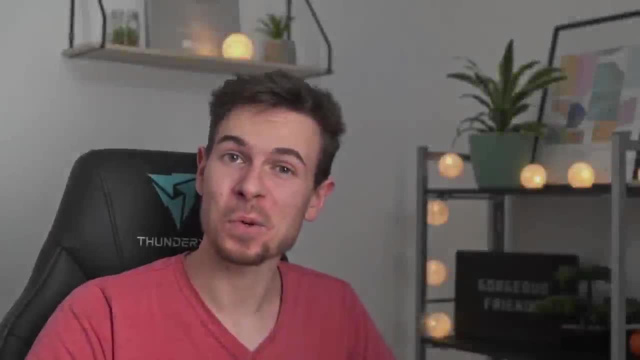 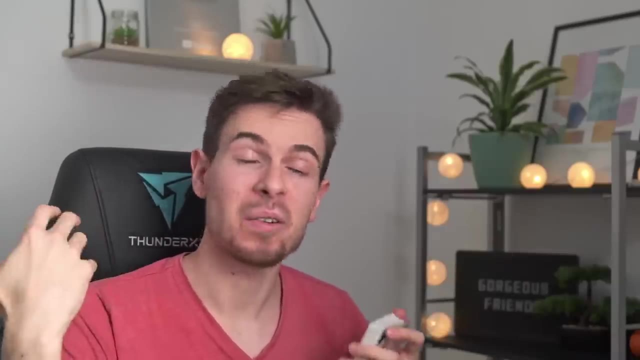 All right, let's get going. Enjoy. Hello there, and thank you for joining the course. All right, so we're going to take this kind of easy At first. we're going to just kind of take a look at the basics of things, If you feel like. 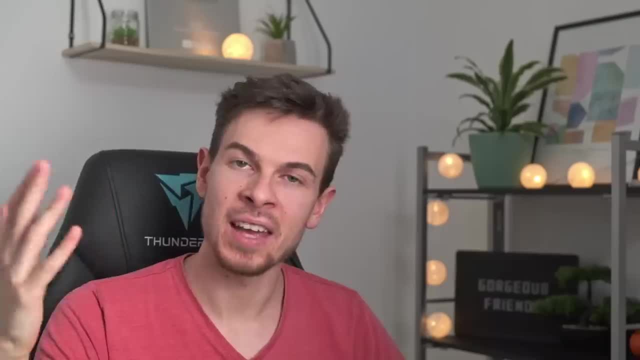 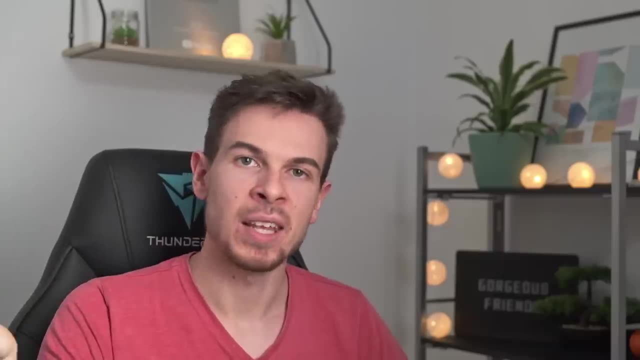 you're very comfortable with HTML and CSS, you can skip ahead towards the mobile responsiveness section. That's where you're probably going to get most of the information, And building out the actual projects is going to give you a lot of information. So if you're interested in learning, 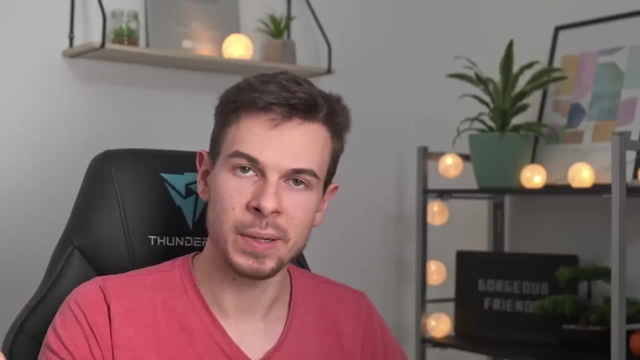 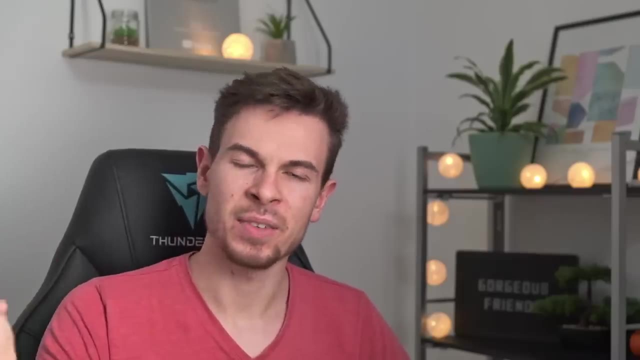 about HTML and CSS. I'm going to give you a bit of practice and everything. So if you're already experienced then you can go all the way to that section. But I still recommend kind of skimming through all of these sections because maybe you might find specific things in HTML and CSS. 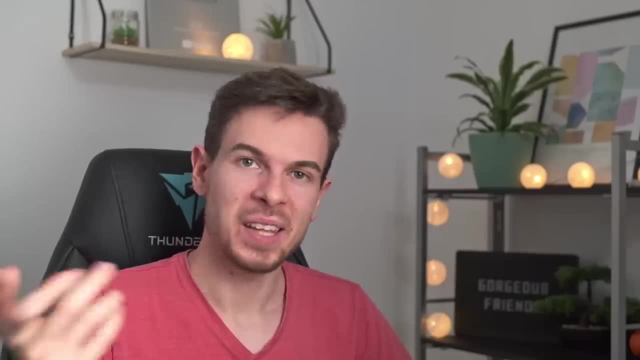 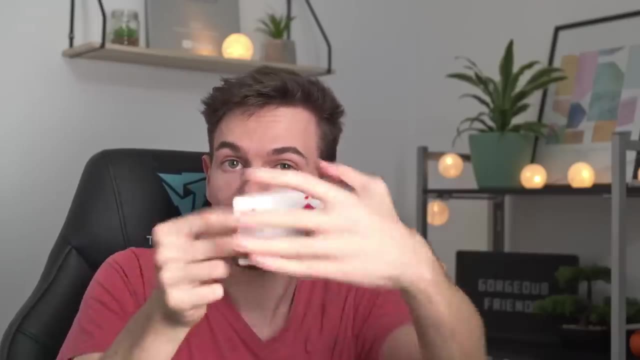 that you might have not known, And if you're a beginner, obviously we're going to start right here And it's going to be very exciting. And let's start with a magic trick. Is this going to be good? Hopefully you didn't catch it how I did it. If you did, then. 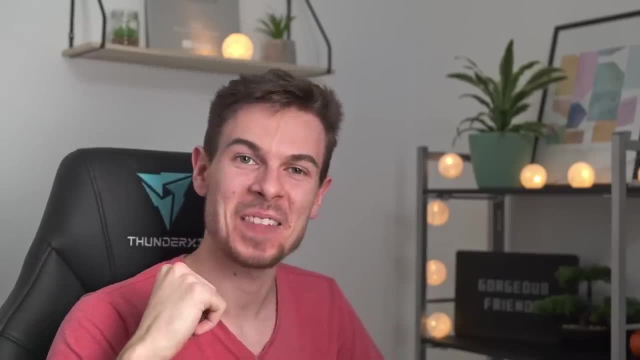 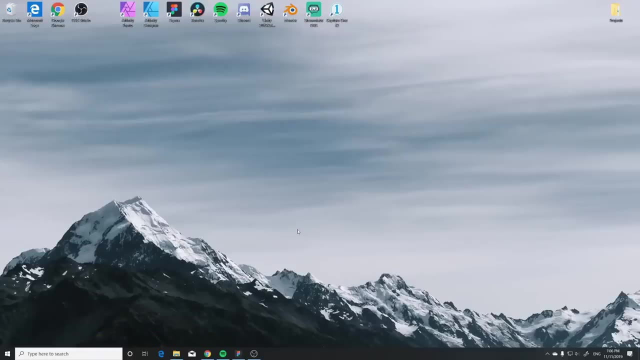 Congratulations: you have passed the first test. Okay, let's get going. This is going to be. Okay, let's get started. The first thing we're going to do is install Visual Studio Code, which, basically, is just a text editor that allows us to write code, And it has all of 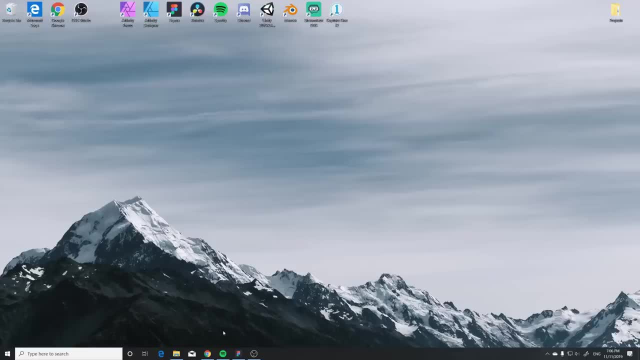 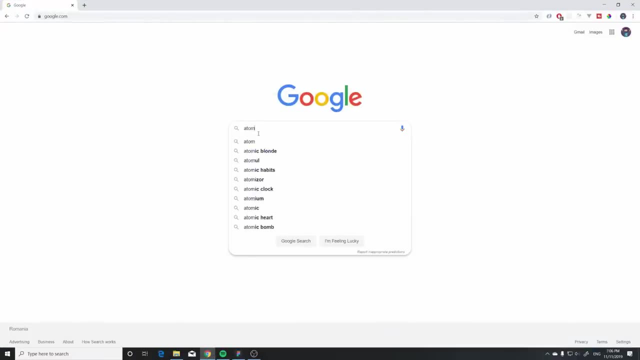 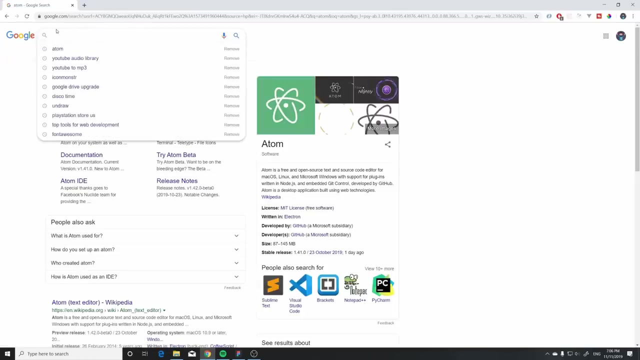 these cool extensions, And it just makes it very easy for us to write code. Now there are different alternatives out there, like Atom and Sublime Text, But Visual Studio Code is just so lovely to use, So that's what we're going to be using for this one, But after a while. 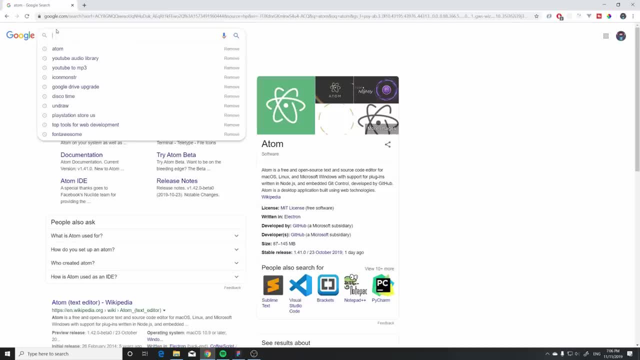 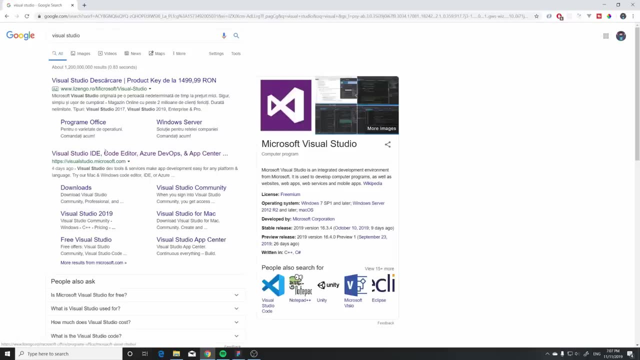 if you want, you can feel free to switch to anything else, But for now we're going to use Visual Studio Code. So just go to your Google and write Visual Studio. It should be. Let's take a look. Make sure you write Visual Studio Code, because there is another one specifically for. 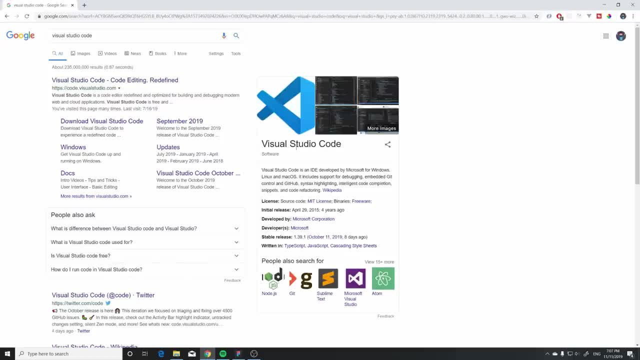 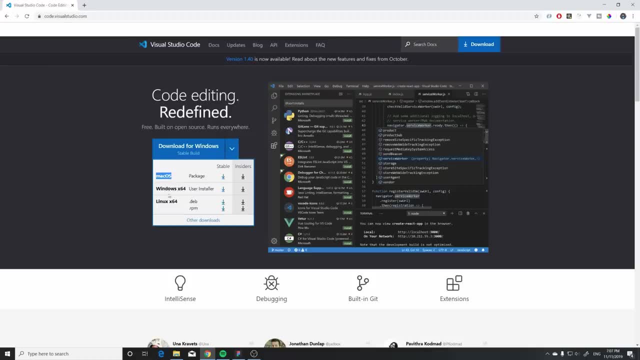 NET to write C-sharp code, And we don't want that. We want Visual Studio Code, So make sure that one. All right, I'm on Windows so you can get Windows, But if you are on Mac, on Linux. 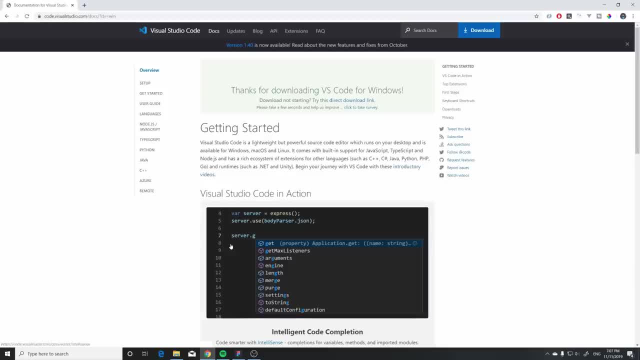 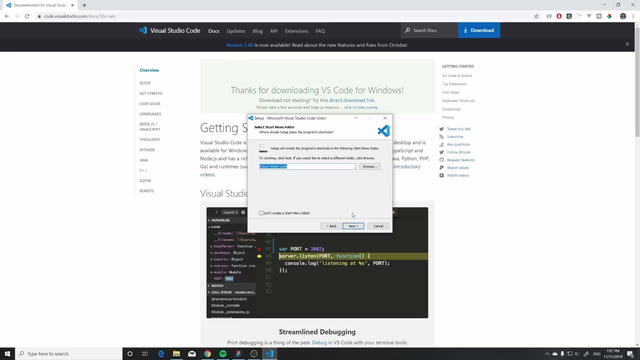 this is pretty much available everywhere for you. So let's get the stable build Hit download. We're going to get the file here. We're going to keep it. Let's open this up. We're going to hit accept on this page. Hit next. We can leave the default. Hit next. All right, Just next again. We can also. 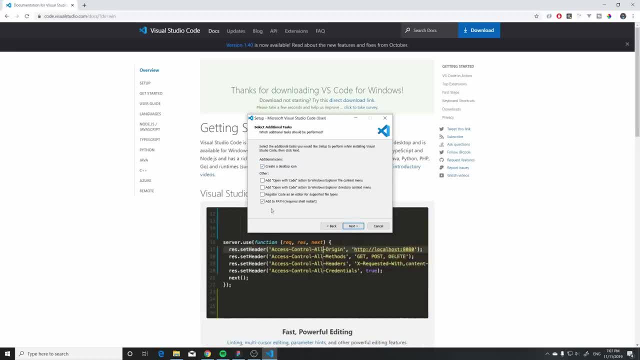 create a desktop icon here And make sure you also have add to path Here Checked. Okay, Then we're going to do next and install, And that should be it Pretty simple. Next up, what we're going to do is take a look at the interface a bit and also take a look at some 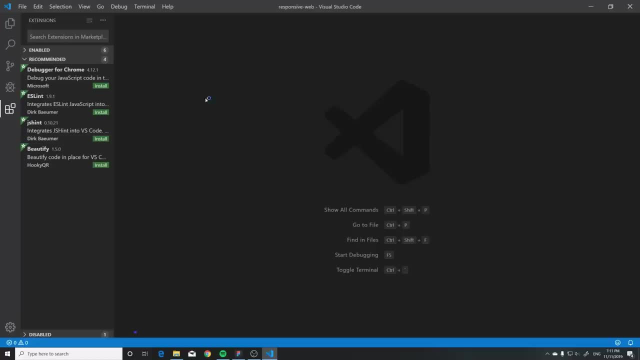 extensions to make writing code a bit easier. Okay, So here we are. This is what you're probably going to get when you open up VS Code the first time, And it's pretty simple. There's not much that we're going to spend our time in. It's going to be this explorer. So here is where all of our 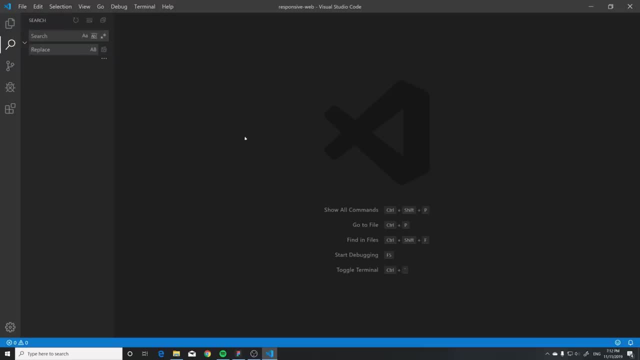 files and folders are going to be. Then we have the search. So later on in our code if we want to search for something specific, we can do that here And we can also replace it too. These two we're not going to cover yet because they're not going to be helpful for us for now. But then we 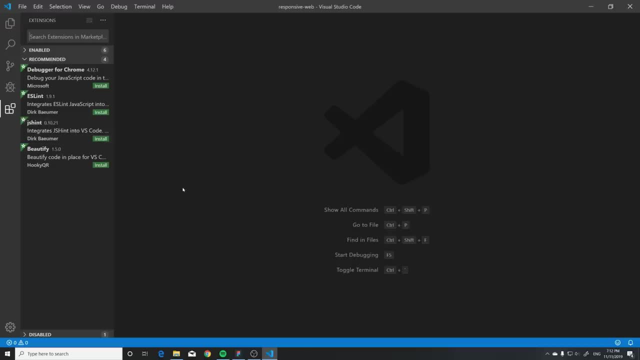 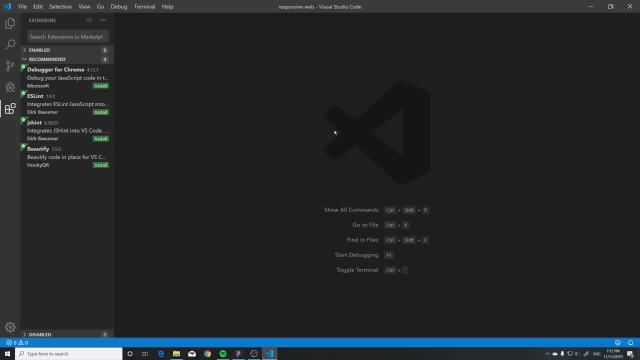 kind of going to explain what they do. The first one is: I kind of want to change the color of this. I'm not a huge fan of it. If you want, you can leave it like this, But I'm going to change mine. 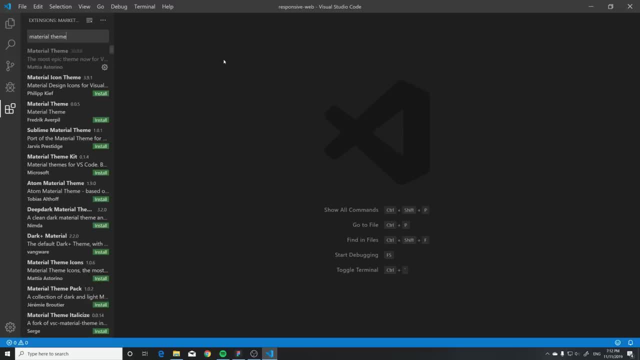 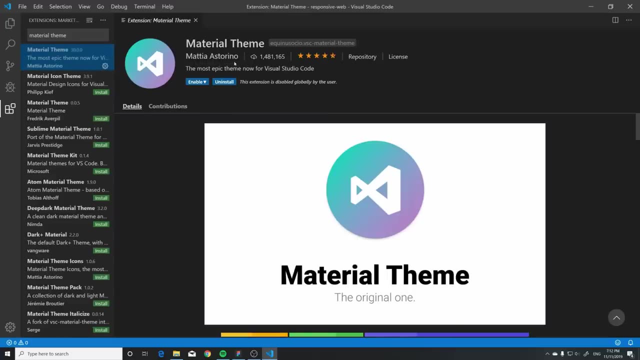 So what I'm going to search for is material team, And this one is a pretty nice looking one, So it's the first one here. It's by Mattia Astorino. I'm sorry if I misspelled your name, But you're going to hit install here. I'm just going to enable it. 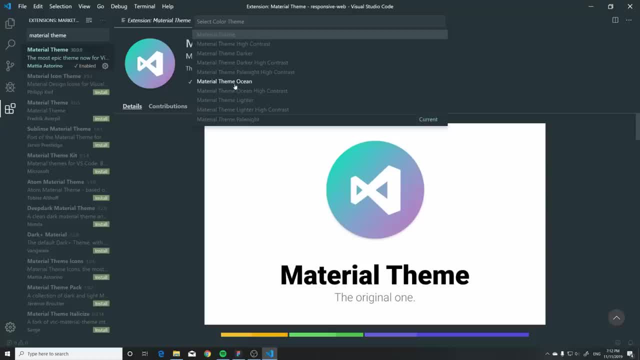 And then what you can do is set color team here. All right, You can click that, And then you have all of these different teams. What I'm going to set it to is this Pelonite high contrast. I believe this looks very good. I like the way it looks, So I'm going to keep this one. Another one is going: 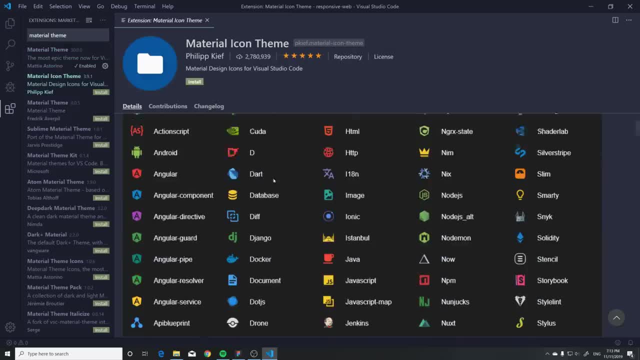 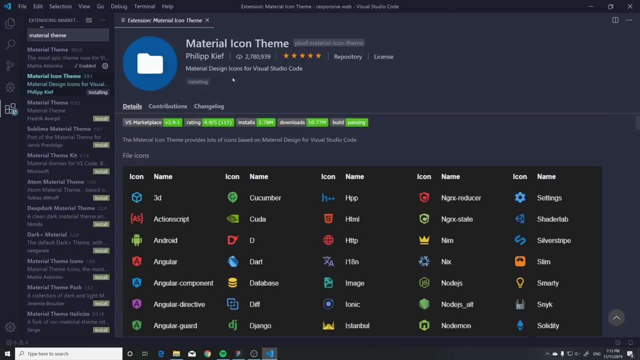 to be right, the one below it, the material icon team. This just changes up the icons Again. this is just super optional. You don't really have to install it, but I'm going to install it, Okay, And then we're going to choose material icon team here, Another way you can access if 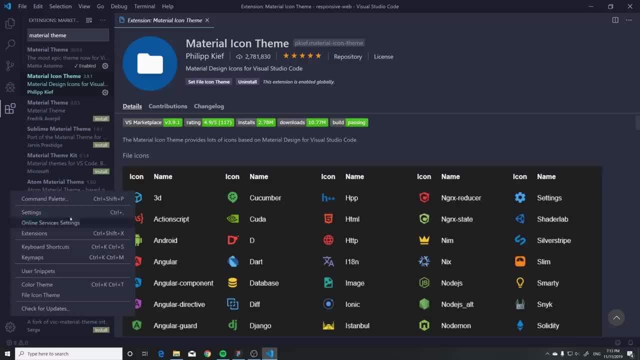 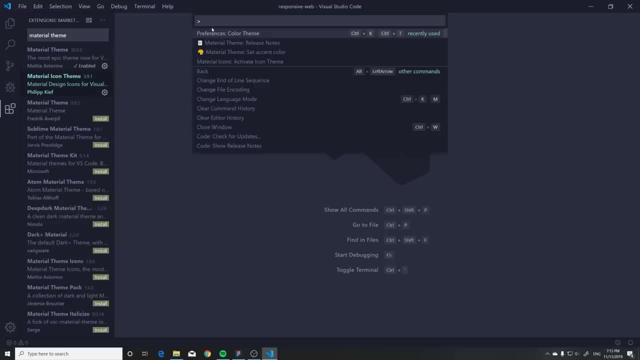 maybe you want to change it again- is you can go to the wrench down here and go to the command palette And for some reason, when you're in the extensions here, it closes. It's bugging out. I'm not sure why, But if we close this up it should open up now And here you can search for color. 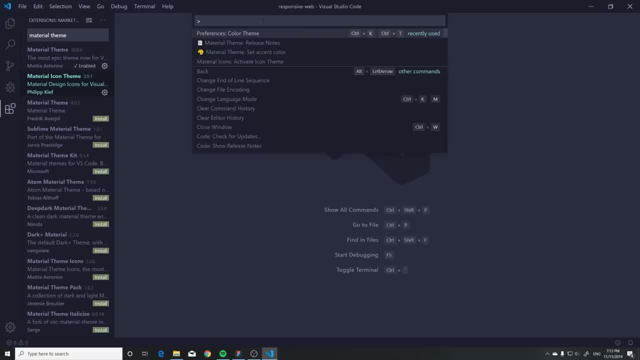 team. Okay, You can just type in here or maybe it might pop up here, But if it doesn't, you can search color team And then you can go to the extension here And then you can go to the extension team And here later on you can pick one that you like. Okay, So those are the first two. Now 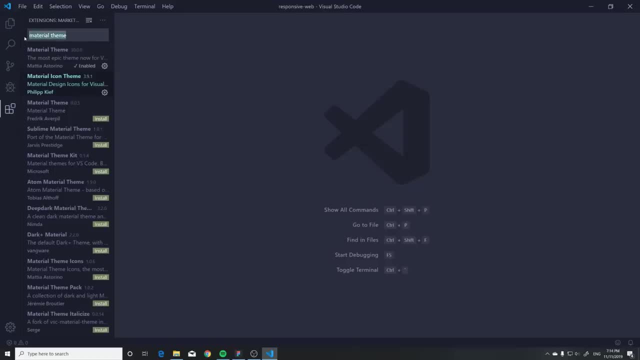 I'm going to install just one more And then, throughout the course, we might add another one or two to it. Okay, But these two I want to change, And there's another one that's very important, which is going to be live server, So make sure you search for live server. It's going. 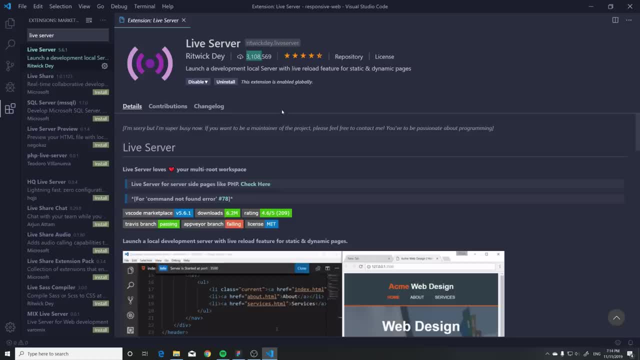 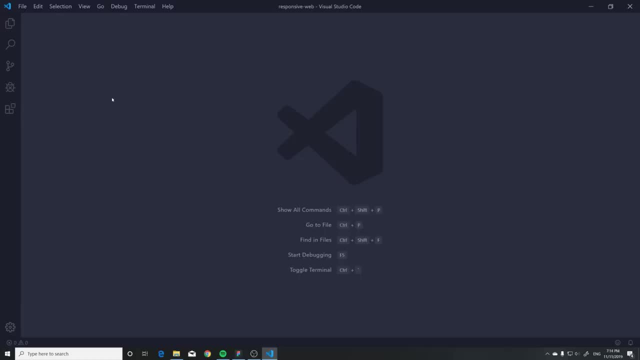 to be this one by Ritwik Day with 3 billion downloads, And make sure to install that as well. And that's going to be it. We're going to close this up And let's start writing our first HTML code. Hey, exciting. So right now I'm on my desktop, here in my file structure, What we're going to do. 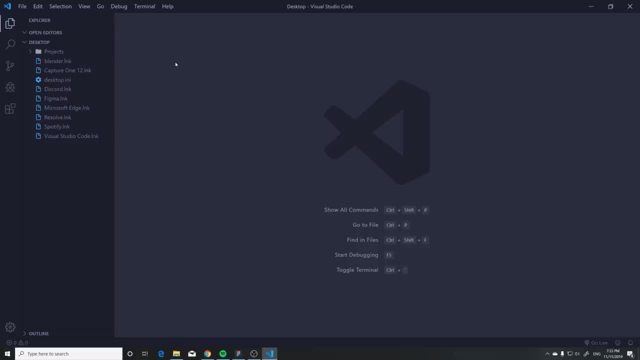 is just create a new folder and create our first HTML file and our first HTML tag. So what we're going to do is go up here to file And what we're going to do is create, go to open folder, And then I'm going to just navigate to desktop, Okay, And then I'm going to go to my file structure And 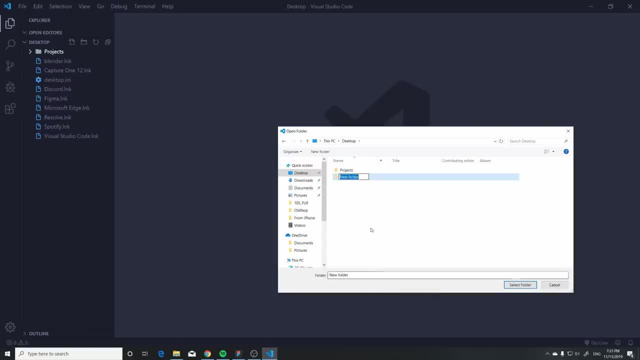 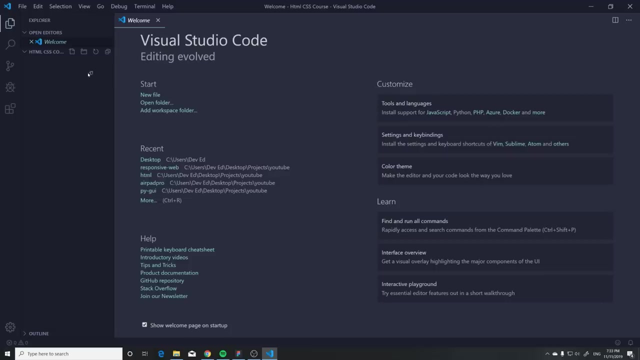 in here. I'm going to create another folder And I'm going to name it HTML and CSS course. Okay, And we're going to open this up. I'm going to select the folder and click. As you can see, this brings us in here And there's nothing in the folder. So that's good. 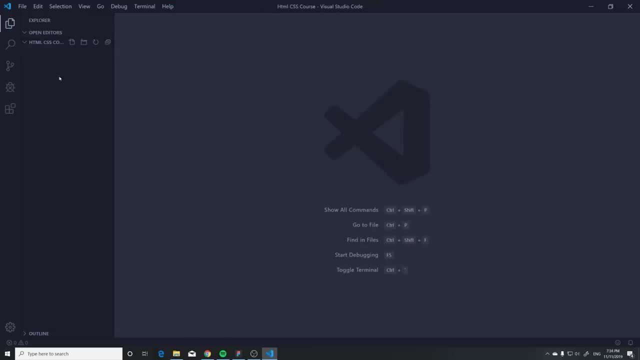 I'm going to close this welcome message- Get out, We don't want you- And to create a new file we can go up here. So, as you can see, this is a new file Here. the second one is a new folder. 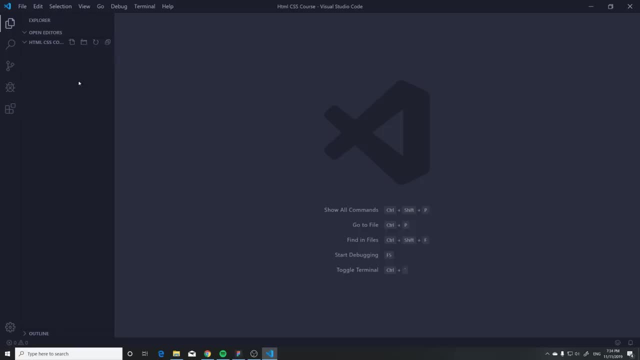 Here. what we can also do is refresh the Explorer in case something doesn't update properly. But to be honest, I never really used this. It always kind of worked fine for me. And we also have this to collapse this whole structure. So what we're going to do is click the new file And we're 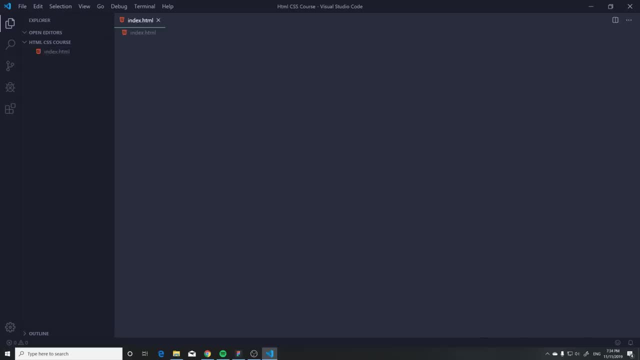 going to name this index dot HTML. So this is how we can create our first HTML file. Now why do we name it? index the extension. Okay, it's kind of obvious. We're learning HTML, So it's probably about HTML, but why index? Well, when we upload our website to a web server, the 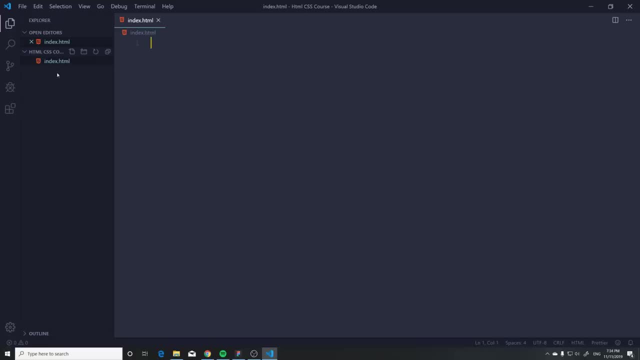 first thing that that web server is going to do is it's going to look for this specific name. it's going to look for index dot index, not HTML for the index. as soon as it recognizes that, that's the first thing it's going to display, because eventually we can have multiple HTML files in here. 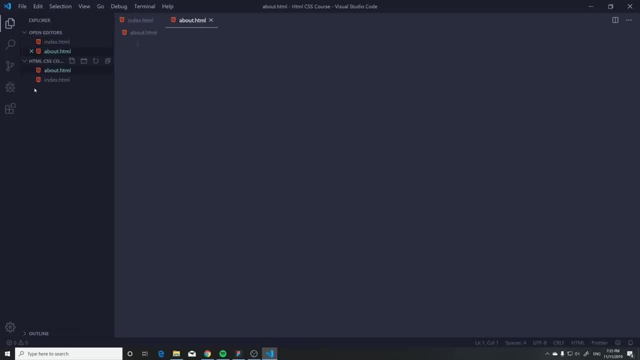 we can have maybe an abouthtml dot HTML. maybe we have an about section on our page, So we can have that, maybe a contact dot HTML. But as soon as we upload it online, the first thing that the users are going to be served 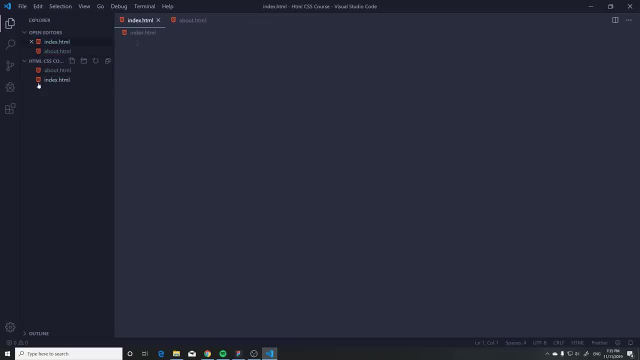 is this index dot HTML. So this is going to be always the default. All right, so you're going to mostly create index dot HTML when you create your website, So let's delete this for now. We're just going to keep the index And just to keep this simple, we're just going to write one HTML. 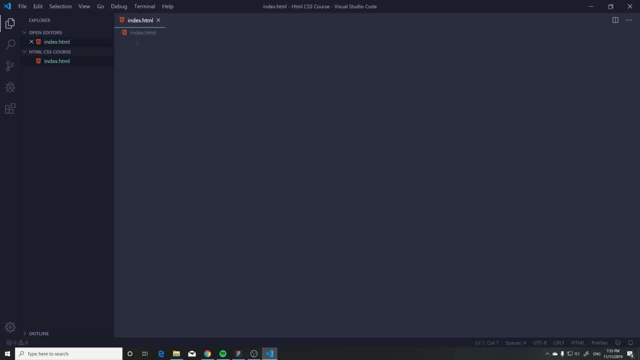 tag in here, And then we're going to set up a proper layout or kind of a structure that you're going to be using for all of your websites, And then I'm also going to show you a shortcut. that's very awesome in VS code, That's. that's just going to make it super fast And you're going to be up. 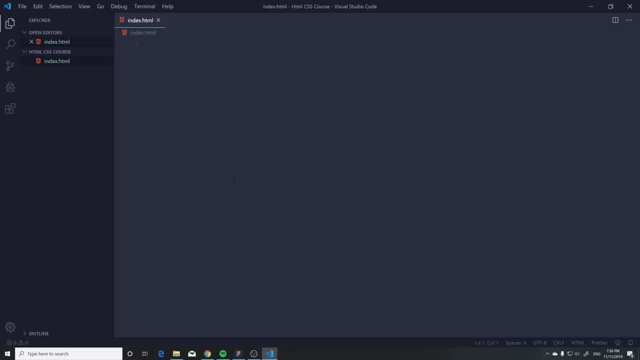 and running in two seconds. Okay, Ed, stop talking. Show me how to do this. So all I'm going to do is I'm going to write a smaller than sign and h1.. And, as you can see, this is basically a heading on your website. So this is how it looks now. 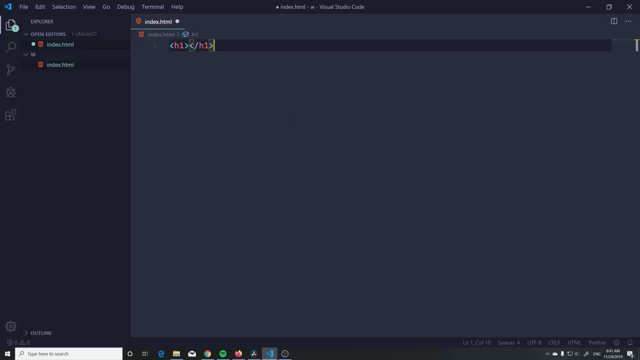 VS code automatically, automatically completes it for us, So tries to help us, But let me kind of get rid of it. So this is what a HTML tag is All right And we can close this up. The second one kind of looks the same, but we have an. 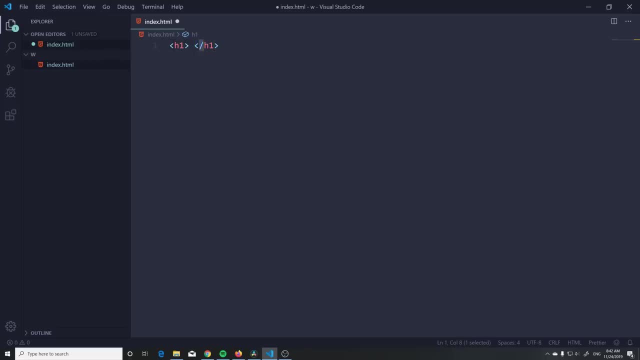 additional slash here like this: Alright, so it kind of looks like a sandwich, not a Subway sandwich, but just a normal sandwich. So, basically, whatever you put in between here is going to be displayed on the screen. So whatever you put in between these HTML tags. So in this case, let's. 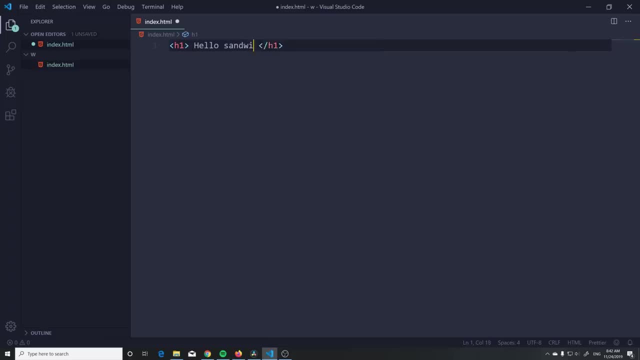 just put Hello sandwich boy, like that, and hit save, So I can do Ctrl save. Okay, and now to visualize this on the screen, what we can do is hit the right click and then hit open with live server And that's going to put it up on the screen here for. 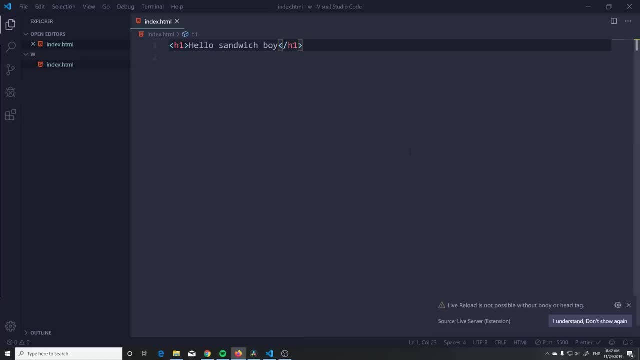 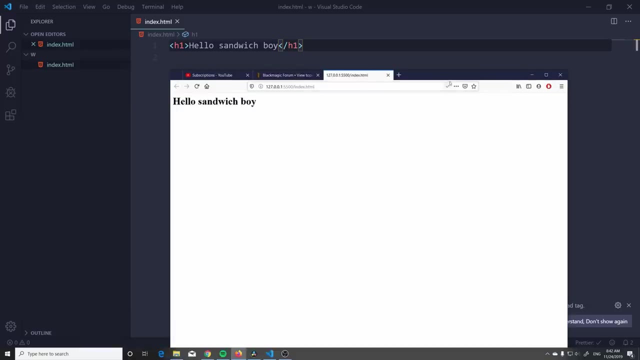 us. Let me drag the screen on the side of the page. that doesn't work. Okay, let me just do this. And, as you can see, we have a heading that says Hello sandwich boy. So everything worked. Okay, this is super basic. So in the next section we're going to set up a proper structure. Okay, if you've seen, 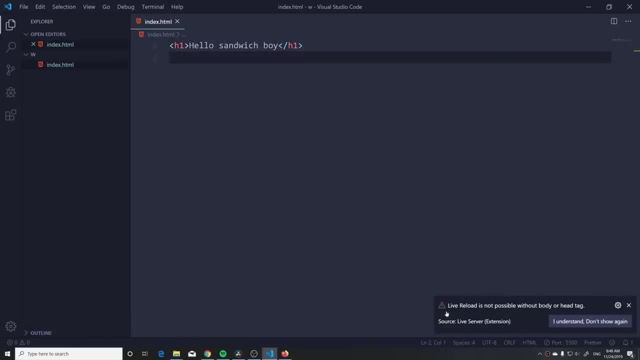 this. you probably get an error message here with this yelling at you saying: live reload is not possible without body or head tag. Oh my goodness, leave me alone while you do this. So basically it's telling you that hey, this needs a proper 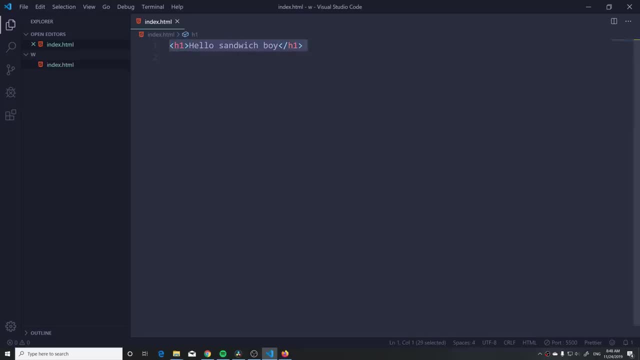 structure. So you kind of need to define a HTML tag And there's something else called the head and a body. So I'm going to kind of explain everything as we go on. So the first thing we need to do is basically specify to the browsers that, hey, we are working here with a 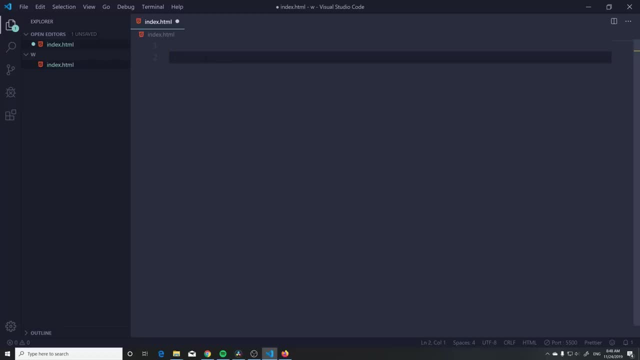 HTML document. So the way we can do that is there's a special tag here called you do an exclamation point And you can see doc type like this and you can write HTML. Okay, so you don't need to kind of memorize this. this is just a thing that we do once And that's kind of it All. 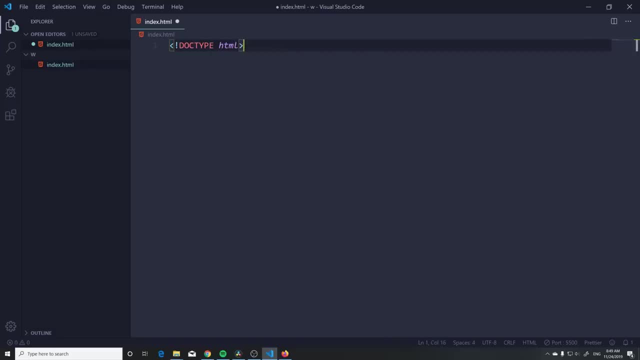 right. So this is. you can imagine that this is just the one type thing. we never really go back to this And we're going to do it in all of our pages, So don't really worry too much about this, Okay, but essentially what it's saying is: yo, I'm a HTML document, So very cool, Okay. 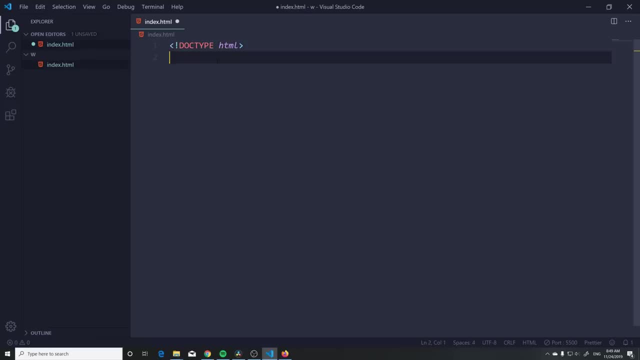 so here's where we're going to see the sandwich effect with these HTML tags. So what we're going to do is to find our HTML document. Now here's a cool trick: you can hit tab and that's automatically going to complete everything. So you just write HTML and tab and the same thing. 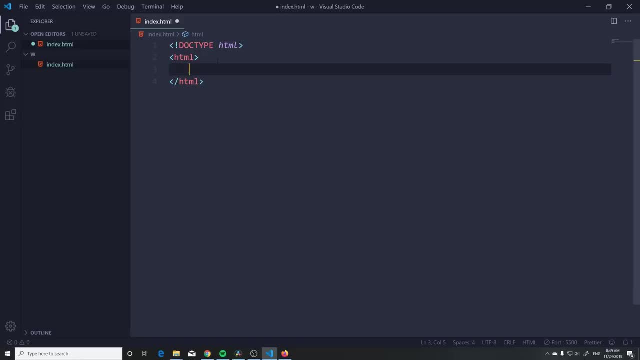 works with the H1 as well, that we saw. Okay, so this basically takes two things. So this is our documents are HTML document And this has a head- I'm going to hit tab again- And also a body, which I'm going to do down here. Alright, so, as you can see, these are kind of 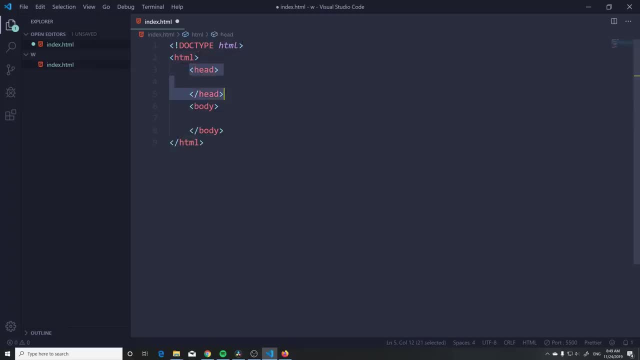 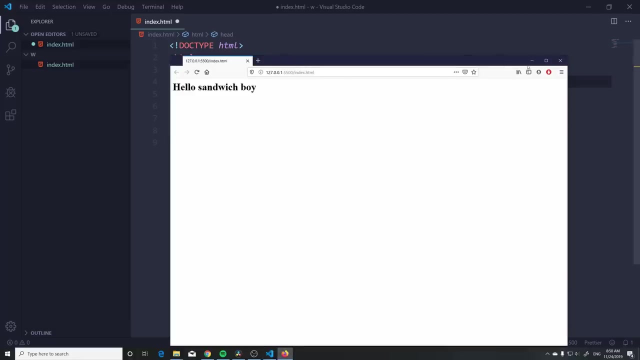 separate. this is kind of like the parent element to these two children in here. Okay, and what this head is is basically where your meta information goes in your title that you see displayed on the website So up here in the corner, and things of that sort. 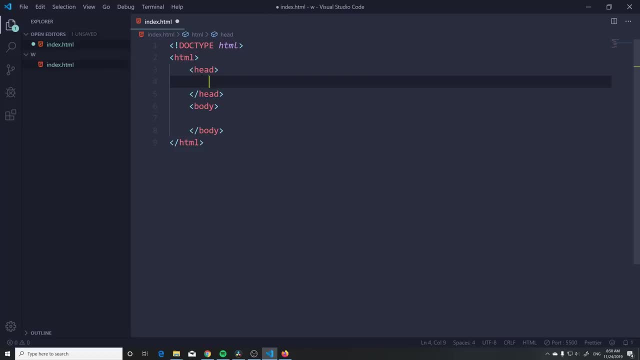 for search engine optimization, for Google to find your page, to index your page, And also you're going to see that here is where we're going to link our CSS and our fonts and things of that sort, Okay, so things that are kind of in the background, that we don't necessarily see on the 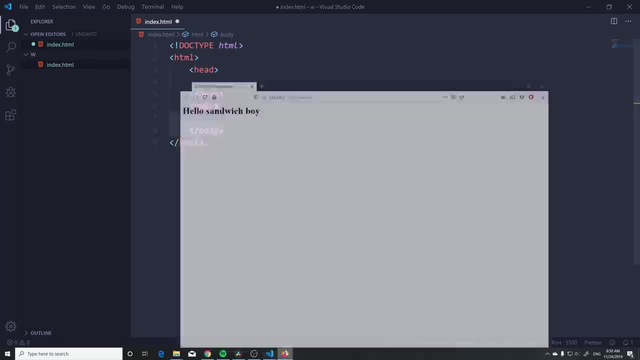 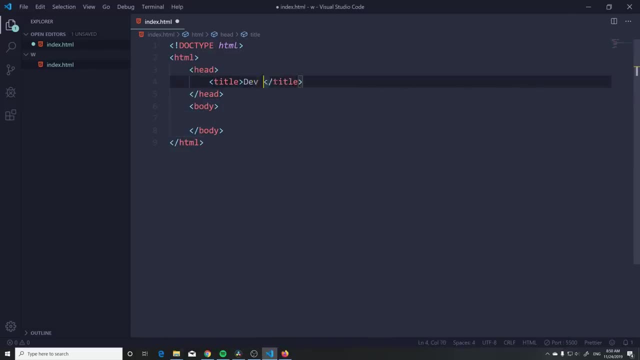 screen And the body basically holds all the information that we do see on the screen. So for now, let's just do one here. I'm going to say title and I'm going to say David or sandwich boy. Let's go back to the sandwich boy. Okay, so that's one here, All right? So if we hit save, 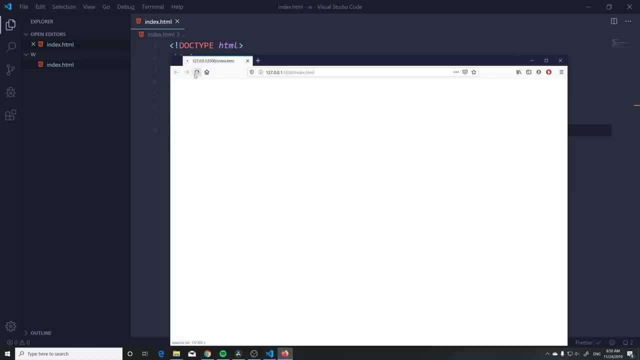 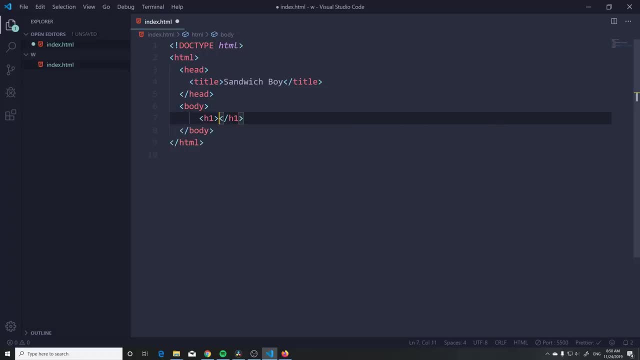 all right, let's see if this refreshes automatically. Okay, there we go. Sandwich boy we have there. Okay, and whatever we put in our body here. so I'm going to just write the H1 sandwich and hit save, control, save, and you're going to see this popping up here. 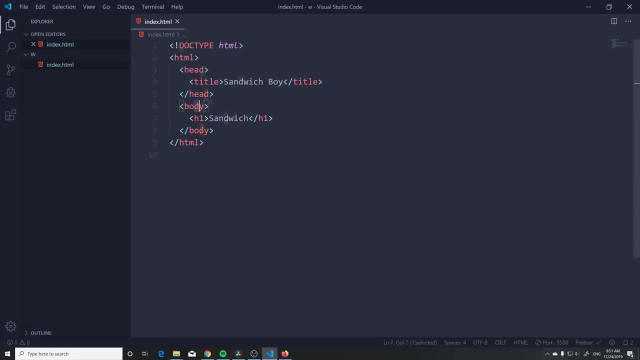 So the main part of your website is going to be in this body And all the rest is going to be in the head- the information about the website, linking style sheets and things of that sort. fonts, Okay, but you probably saw that when I tap this over like 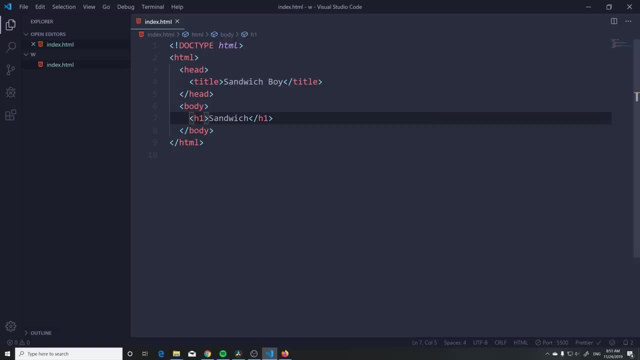 this and I hit save, it automatically reloaded and made it nice for me. So even if I have these extra spaces, it kind of organizes everything for me. So let's introduce another extension. This one is called prettier, So go here to the extension tab and search for prettier. 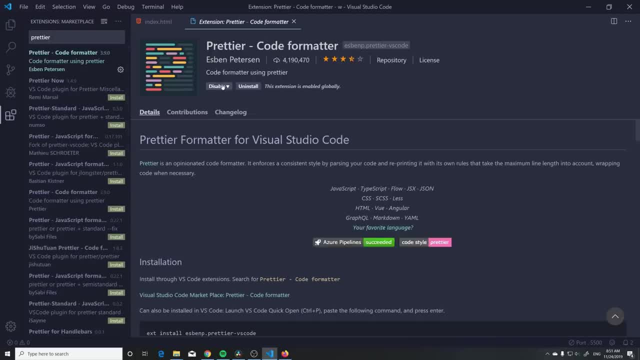 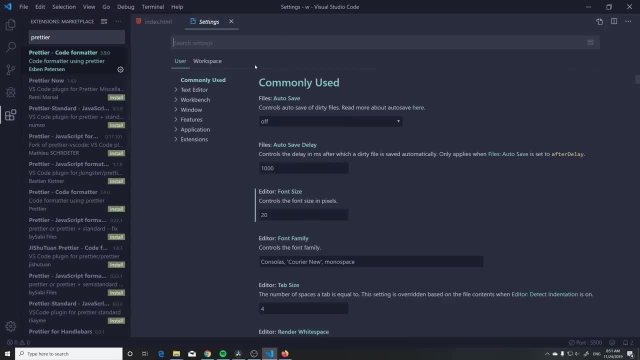 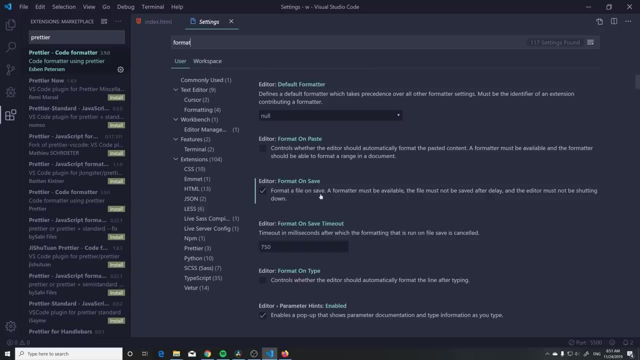 Prettier Like this. click on this one. it looks like this: hit install And once you do that, what you can do is go to the wrench tool here, go to settings, and you can search format And you can enable this format on save And basically it formats the code for you. 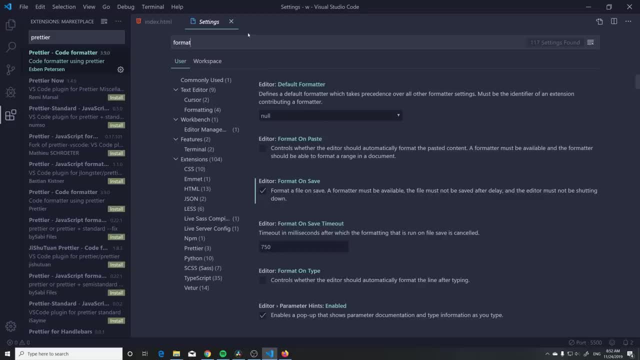 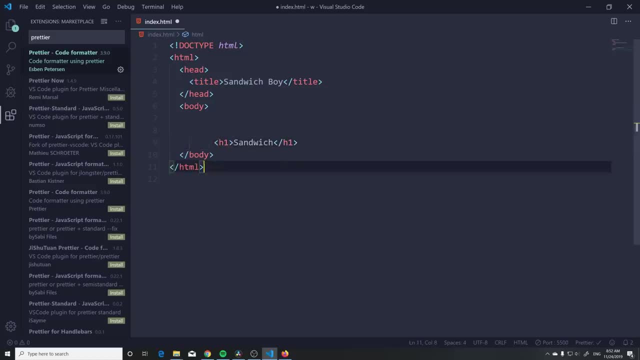 if a formatter is available. So prettier is a formatter And it's just going to keep your structure very organized, even if you write sloppy code or you kind of if random spaces here So this kind of looks hard to read But when you save it does it. 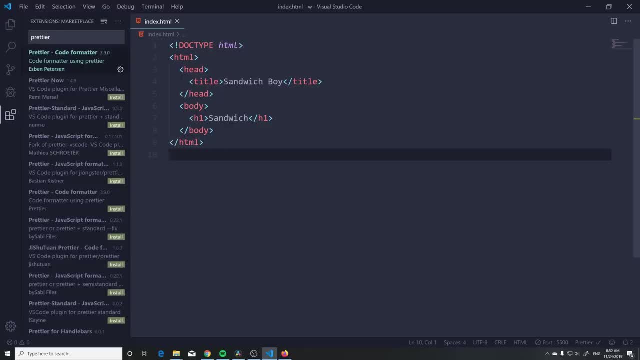 automatically for you And it's kind of nice because you can see what parent is whose parent and who are the children. So I know that the head is the parent of the title and the body has a parent of age one. Okay, so this kind of keeps everything nice. Okay, next up what I want to. 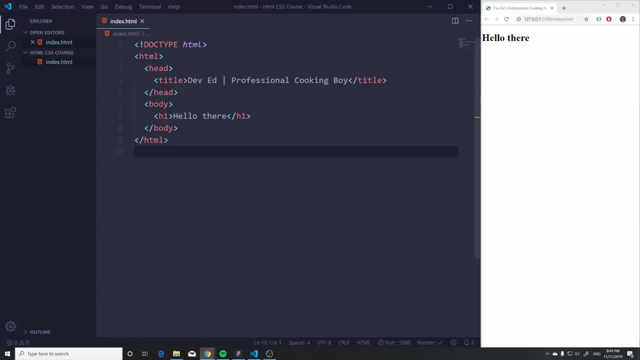 show you is a bunch of awesome meta tags that we can add to our head here. So again, just a few more things that are not visible, And then we're going to go ahead and hit save, And then we're going to get straight into the fun I promise. So here, what we can do is add some SEO. that's going to 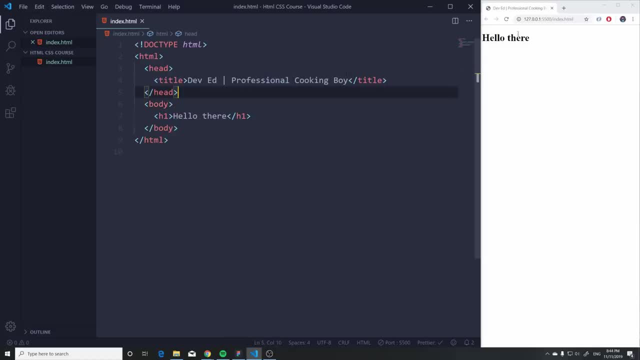 improve our search engine optimization. Alright, so our website is going to be more easy to find, So we added one which is the title here, And actually you can make this longer, like this: dev ed. professional cooking boy. I just added this for fun And, as you can see, it updated right there. 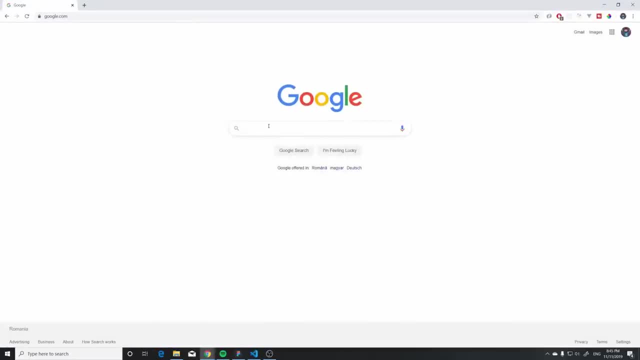 You can also view this on a bunch of websites. If you search like YouTube here, you're going to notice that the title: well, they just have YouTube. but okay, let's search another one, Amazon, as you can see Amazon online shopping for electronics apparel. So it has a pretty long. 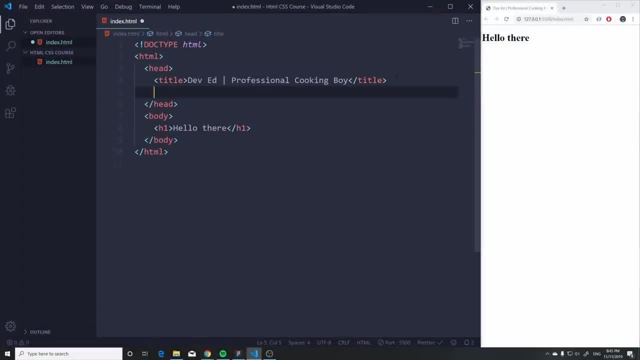 title. Okay, so let's add another one. The other one we're going to add is called Meta and hit tab, But, as you can see, this one is actually doesn't have this closing tag, like like H1 or like title, just it's like Meta And that's it. So you're gonna find some some tags. 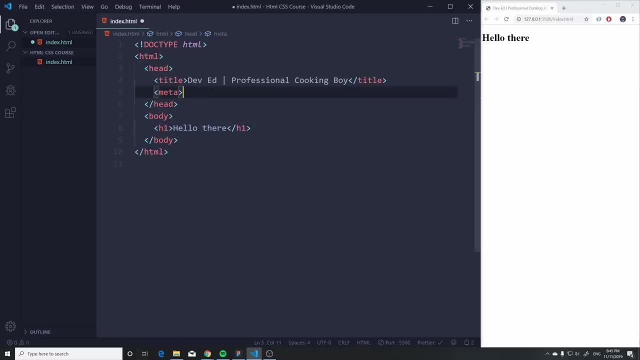 that do come with the title. So let's add another one. And, as you can see, this one is actually doesn't have this closing tag. So let's add another one. And, as you can see, this one is actually doesn't close some that don't close And I don't really want you to beat your head over and like: 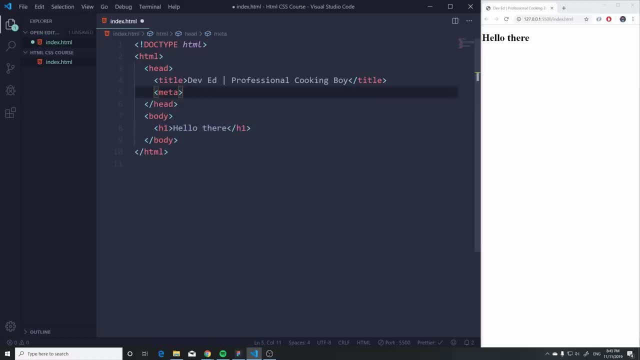 sweat and and invest a lot of time in remembering which tags close and which tag, which tags don't. So what I recommend you to do is just hit tab, just write H1 tab And VS code is automatically going to know what to do. So this way you're going to write them and 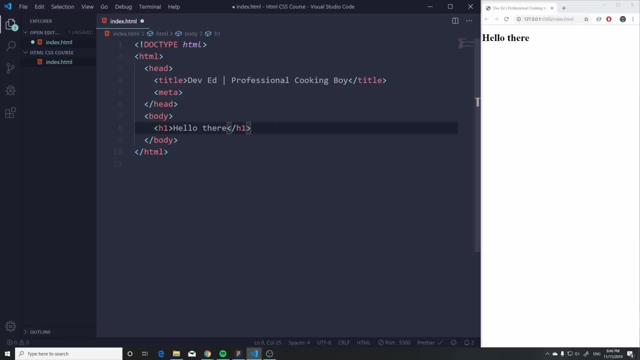 you don't have to worry about it And if you keep writing more HTML, you are going to remember it because you keep using them a lot, So it's going to go into your memory. So don't really sweat about which tags close which tags. don't just hit tab and let the auto complete? do it for you. 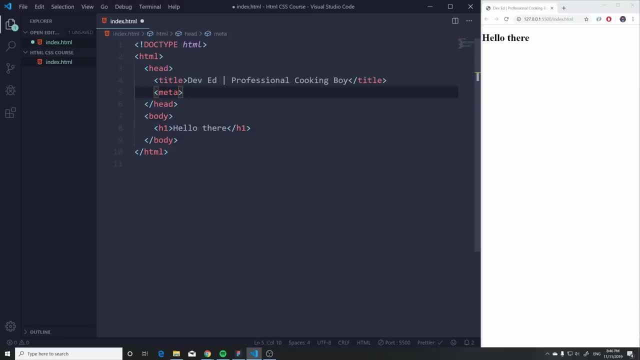 And then, yeah, it's just, you're just going to remember it easier this way. So, Meta, another thing I want to introduce you is if we come here after right inside this, this, this tag here, and just add a space, we can add something called an attribute And all, all in. 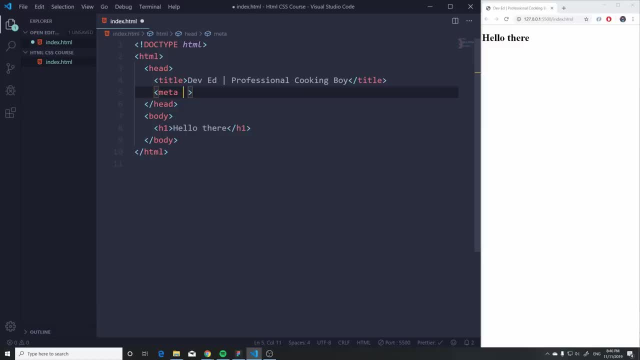 attribute is. it just basically changes the behavior of your, of the meta tag that you are on, And you're going to see this being used a ton, especially here when we're in the body, and we're going to add inputs And we're going to add a bunch of other things. we're going to 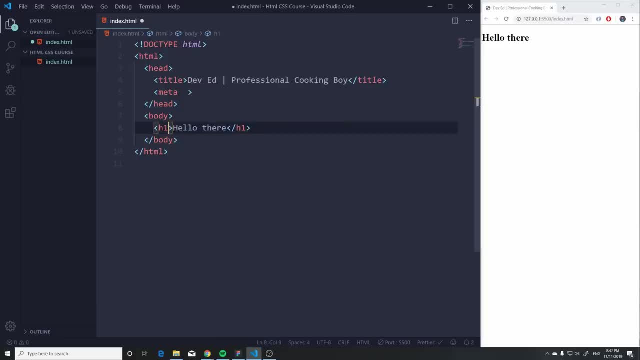 add a bunch of attributes in here that's going to change the behavior or maybe just give a name to our tags. So let me show you what I mean. In the meta. we're going to add an attribute called and we're going to set this equal to description. So this is a meta that's going to handle the 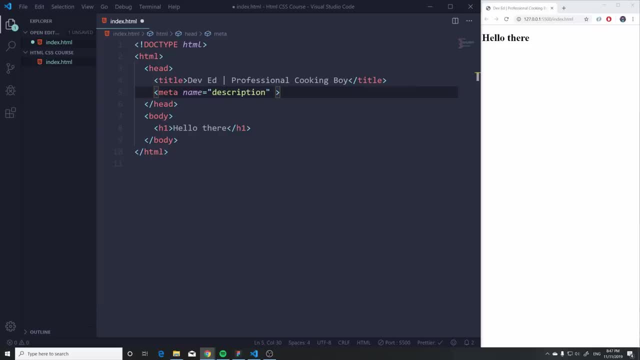 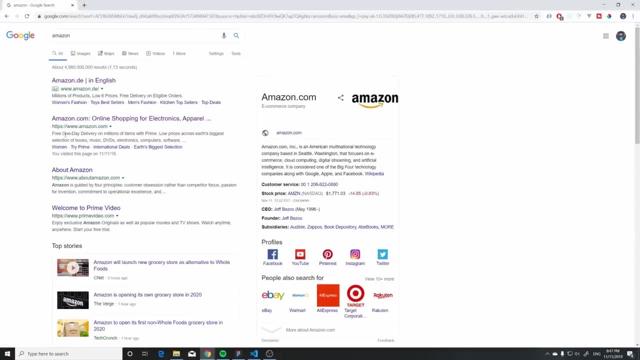 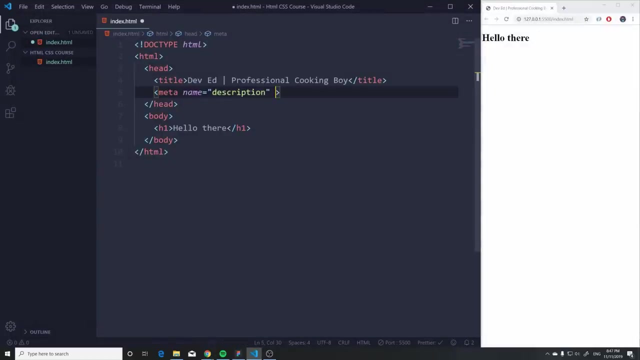 description on our page. So if I'll go back to the Amazon, if I still have it open, let me go amazoncom and pull it up here on the screen. So, as you can see, it has a description down here. So that's going to be our, our meta tag, And here we can add: 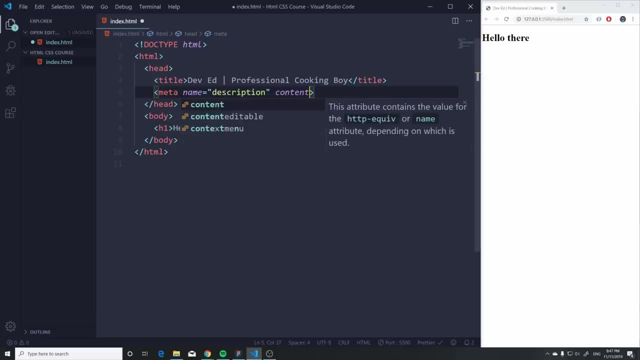 another attribute called content All right, and here if we add hit enter, it's, as you can see, auto completes it for us, just like it did before. here we just set it equal and we just add two quotes Okay. And here we can say: dev ad is a professional cook with Italian dish expert. 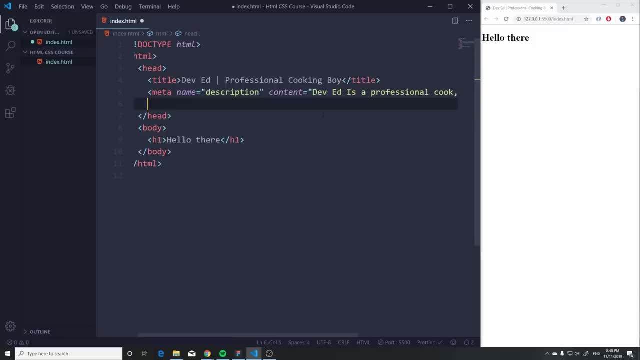 I don't know, I'm really bad at adding these, But when, if you do a portfolio or something, you're probably going to mention a lot of keywords here, like front end web developer, HTML and C CSS and things of that sort, Okay, But a title is still going to be way more important. 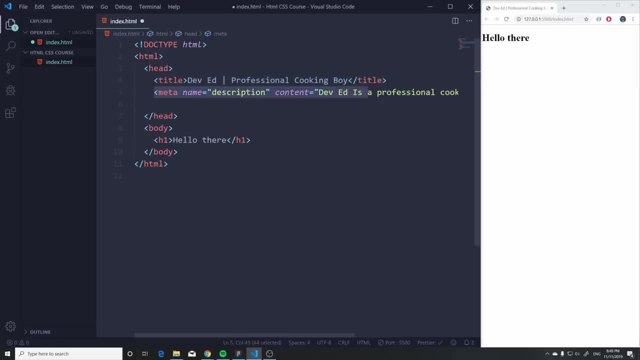 than this description meta tag, But it's very good to add this as well. Okay, that's the first one. The second one is going to be a bit weird, But I'm going to write it down here, for you are going to say meta and the attribute is going to be called character set and we're going to set this equal. 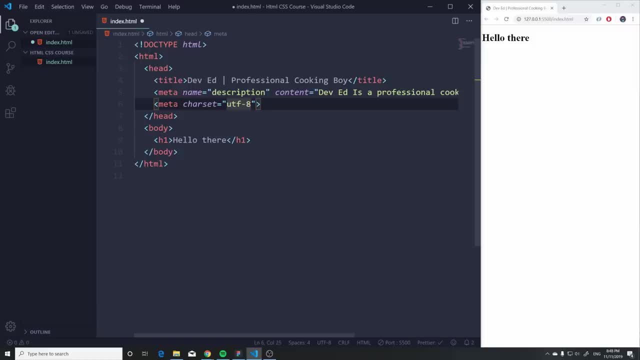 to utf eight. This is something again I don't really really want you to worry about that much, but it's pretty much in encoding. it's an encoding that our browser can understand. so, basically, all the the words like ABC, the FG, and one, two, three, four, and these symbols, like like dollar sign, and these 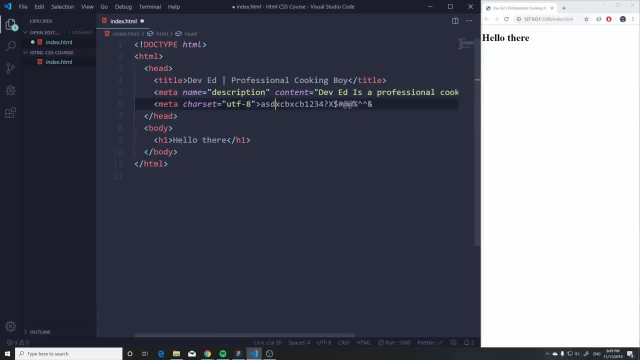 symbols is basically you. you're telling the browser what kind of character set to use and encoding to use. you can kind of hover over this car set and you can car set and you can see kind of more of the meaning. it's kind of, it's not that. 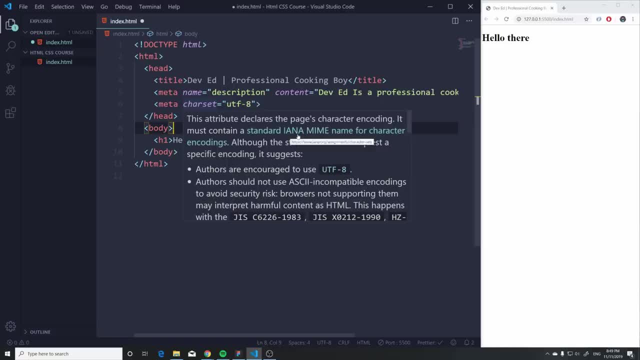 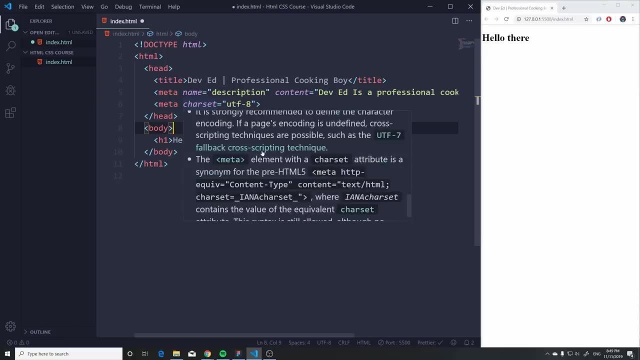 clear. the attribute declares the page characters encoding and must contain standard Yana my name, for yeah, it's a bit weird, but all it basically is it's just an encoding that recognizes the characters that we generally use here, especially in in Europe or US, right, it's not. 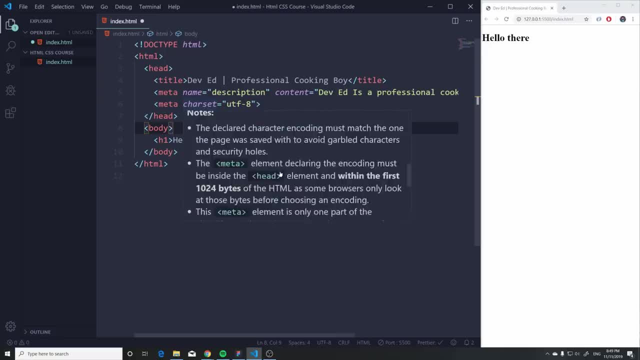 Chinese characters or or any other things like of that sort. okay, so again, this is just something we add. I wouldn't worry too much about it, but it's good to have it here. okay, so that's another one. let's do another one. we're gonna say: 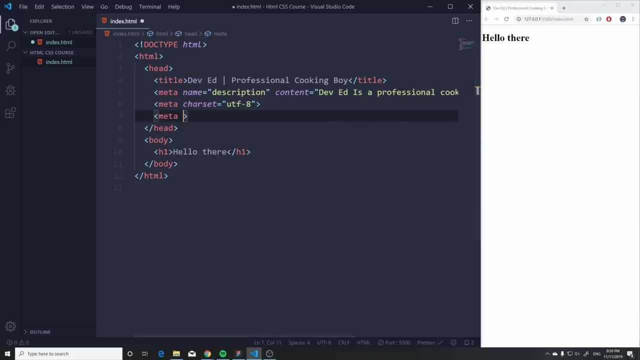 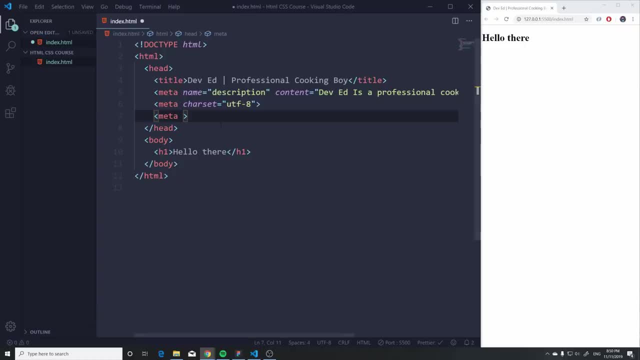 unfortunately. but what the robots? unfortunately, but what the robots meta tag does it basically provides meta tag. does it basically provides meta tag? does it basically provides instructions to the web crawlers, whether instructions to the web crawlers, whether instructions to the web crawlers whether to index your web page or not. so so it. 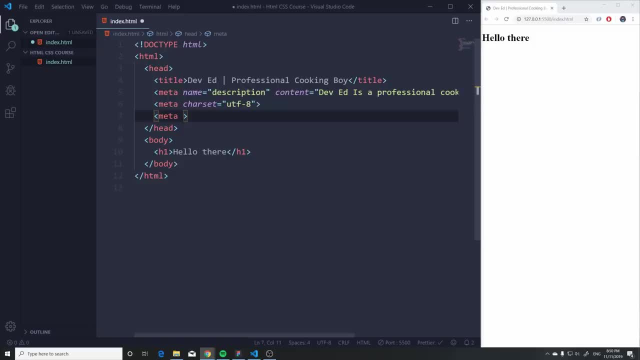 to index your web page or not, so so it to index your web page or not, so so it has an easier time finding your web. has an easier time finding your web. has an easier time finding your web page. or you can declare it for for it to not. 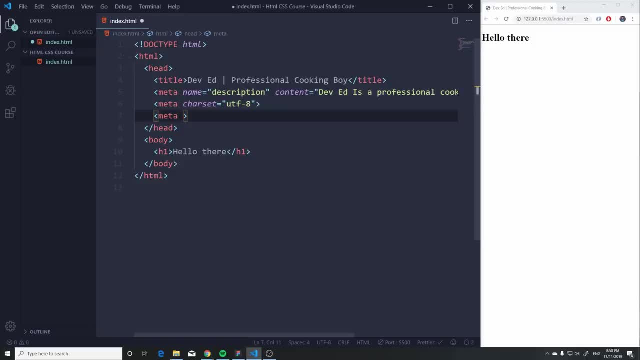 page, or you can declare it for for it to not page, or you can declare it for for it to not be visible if you don't want it to so be visible, if you don't want it to so be visible, if you don't want it to. so the way we can add this is: we can go. 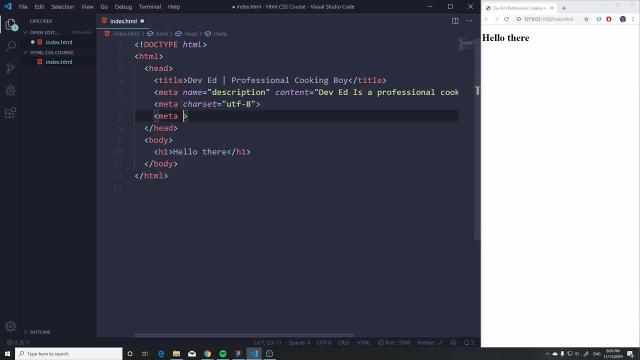 the way we can add this is we can go. the way we can add this is we can go meta here and we can say let's say name meta here. and we can say let's say name meta here and we can say let's say name, just like we did with the description. 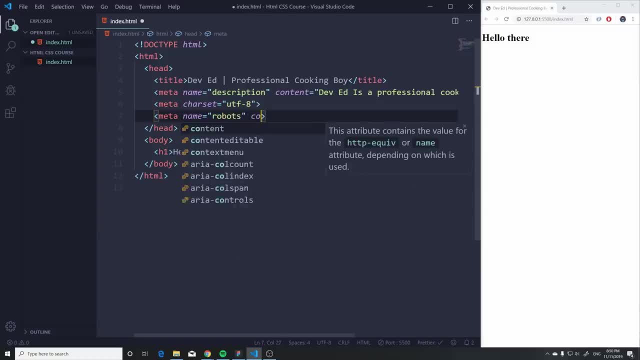 just like we did with the description. just like we did with the description, and set this equal to robots, and then and set this equal to robots, and then and set this equal to robots, and then the content here is basically gonna be I. the content here is basically gonna be I. 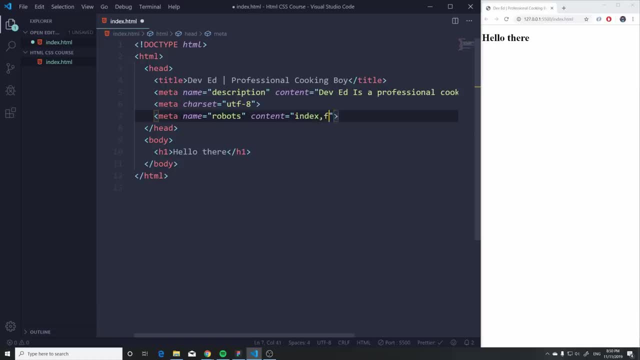 the content here is basically gonna be: I mean you can do two things here. you can mean you can do two things here. you can mean you can do two things here: you can say index and follow, or optionally you say index and follow, or optionally you say index and follow, or optionally you can say no index and no follow. but I 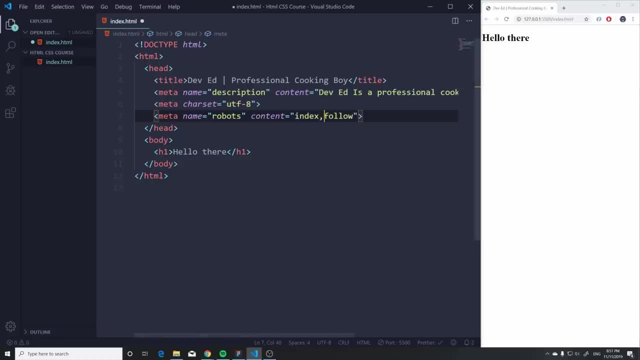 can say no index and no follow, but I can say no index and no follow, but I wouldn't recommend that anyways, so wouldn't recommend that anyways, so wouldn't recommend that anyways. so basically, what follow does, basically the. basically what follow does, basically the basically what follow does, basically the search engine crawler will follow all. 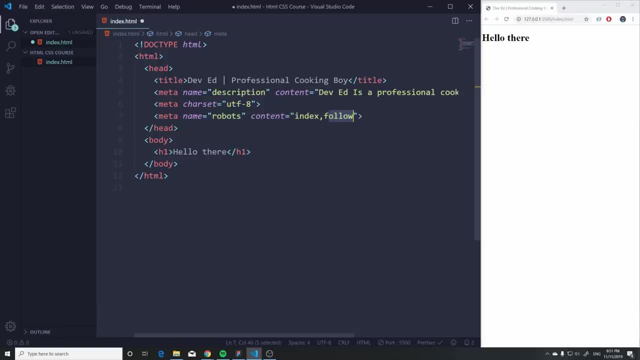 search engine crawler will follow all. search engine crawler will follow all the links in that web page- okay, and the the links in that web page: okay, and the the links in that web page: okay. and the index is the crawler will index your. index is the crawler will index your. 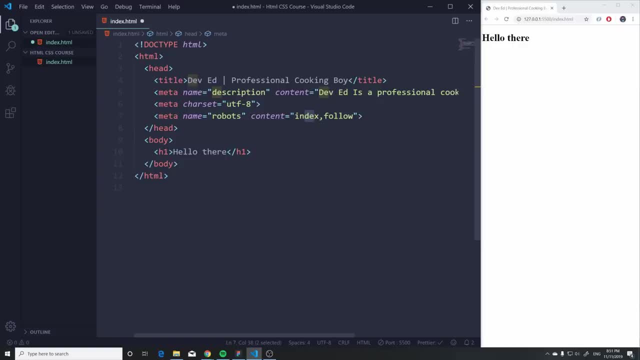 index is the crawler will index your whole web page. okay, so you add this and whole web page. okay, so you add this and whole web page. okay, so you add this and it just helps out the crawlers, it's. it just helps out the crawlers, it's. 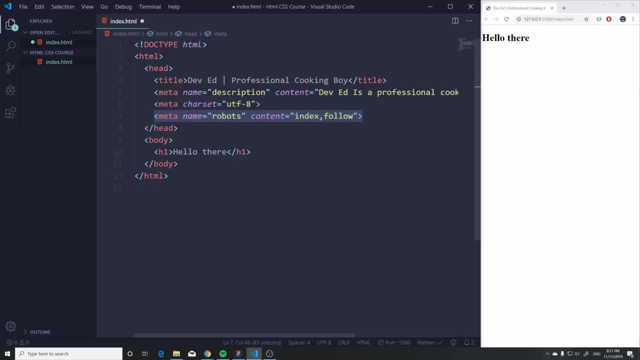 it just helps out the crawlers. it's gonna find your web page easier and gonna find your web page easier and gonna find your web page easier and you're probably gonna appear on Google. you're probably gonna appear on Google. you're probably gonna appear on Google faster. okay, so that's another one. I kind 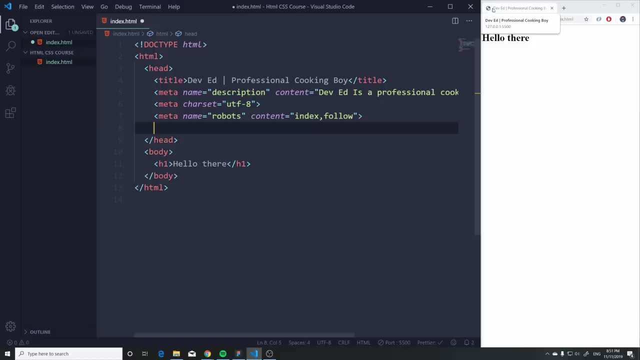 faster, okay, so that's another one. I kind faster, okay, so that's another one. I kind of want to change this little logo here, of want to change this little logo here, of want to change this little logo here because I don't really like it. this is: 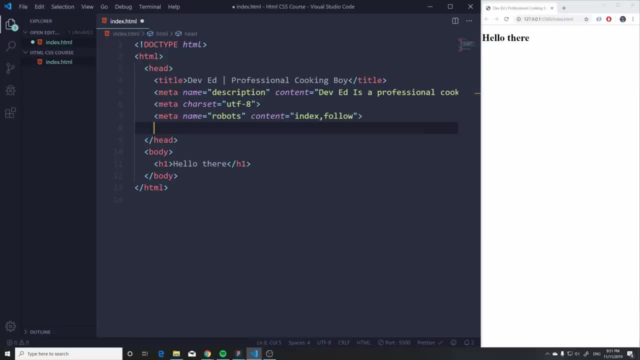 because I don't really like it. this is because I don't really like it. this is just a default that it gave to us, but I just a default that it gave to us, but I- just a default that it gave to us, but I don't like the globe. I don't want to be. 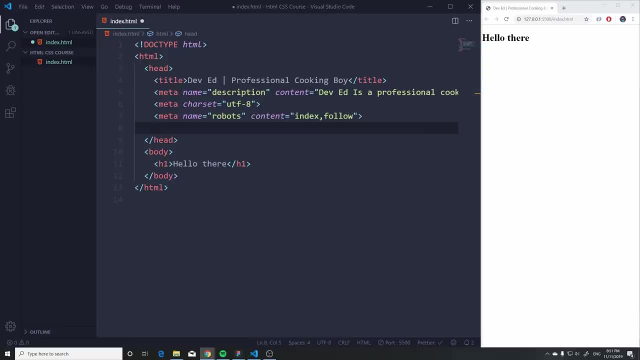 don't like the globe. I don't want to be, don't like the globe, I don't want to be mr worldwide, I want to have my own. how, mr worldwide, I want to have my own. how, mr worldwide, I want to have my own. how can I change that? well, what we can do is 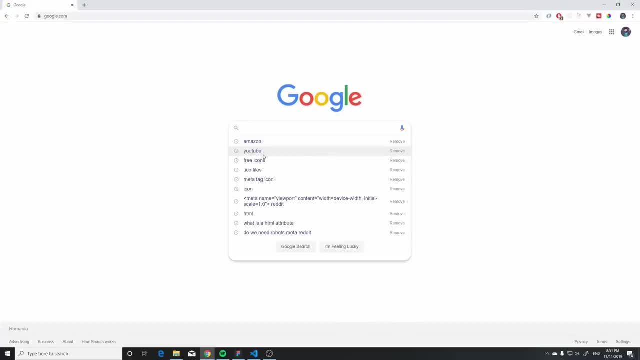 can I change that? well, what we can do is: can I change that? well, what we can do is we can go to Google again, our dear, we can go to Google again, our dear. we can go to Google again, our dear friend, and we can search for some icons. 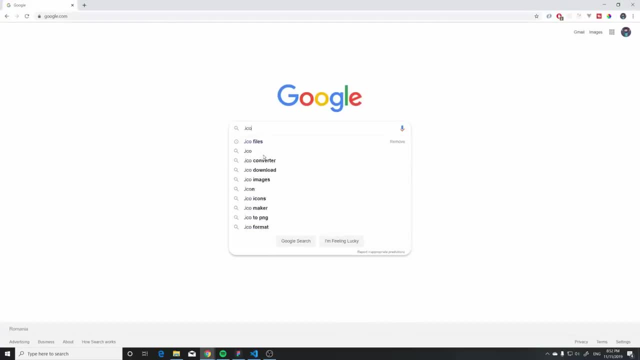 friend and we can search for some icons, friend, and we can search for some icons. so what we can do is we can say dot Ico. so what we can do is we can say dot Ico. so what we can do is we can say dot Ico files here, and I don't remember the name. 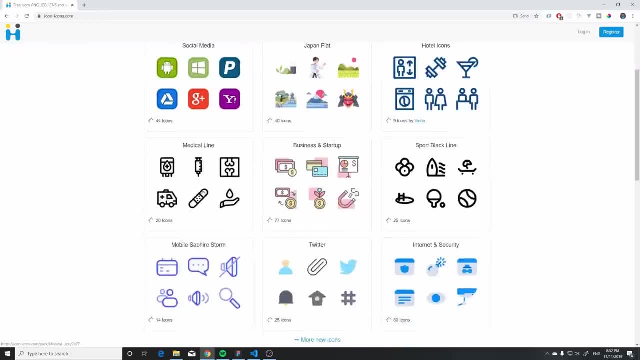 files here and I don't remember the name files here and I don't remember the name: icons dash icons. this was the website. icons dash icons. this was the website. icons dash icons. this was the website. they kind of provide you some some. they kind of provide you some some. 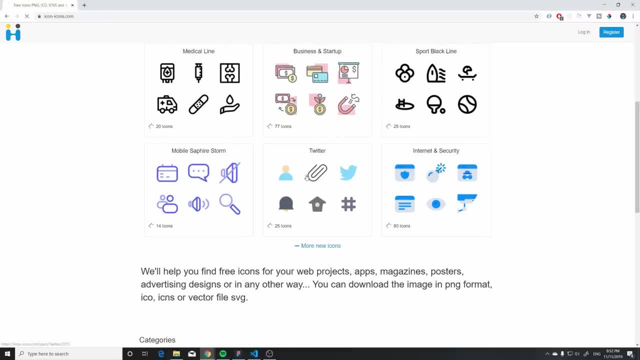 they kind of provide you some, some simple icons here, let's just use one. simple icons here, let's just use one. simple icons here, let's just use one. and just for fun, let's go to this one. and just for fun, let's go to this one. 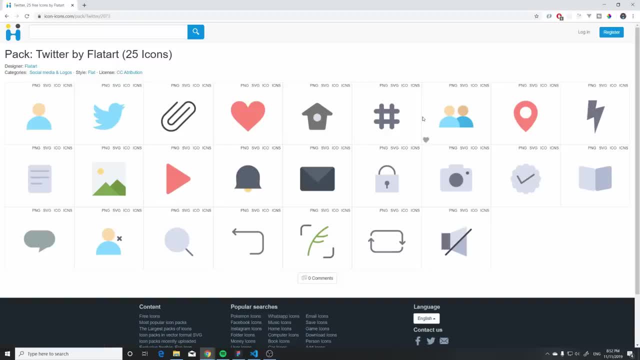 and just for fun, let's go to this one. and I don't know which one do you like I and I don't know which one do you like I and I don't know which one do you like. I like the little house. I want to get the. 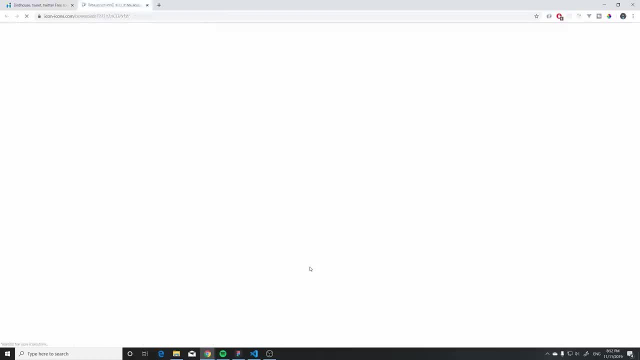 like the little house, I want to get the like the little house, I want to get the house. so let's go on the house and house. so let's go on the house and house, so let's go on the house, and we're gonna download this Ico file. okay, 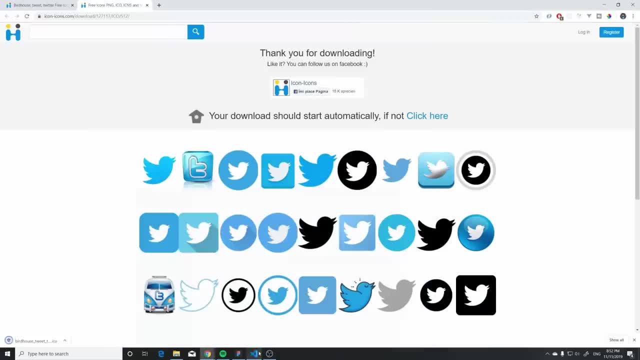 we're gonna download this Ico file. okay, we're gonna download this Ico file. okay, so hit on that. it should download for. so hit on that, it should download for. so hit on that, it should download for you. and after it does, we're just gonna. 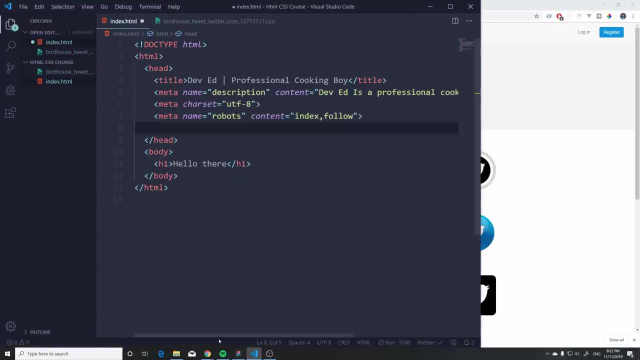 you, and after it does, we're just gonna you, and after it does, we're just gonna drag it in here. drop it in here and now drag it in here. drop it in here and now drag it in here. drop it in here and now. what we're gonna do is: right here, we're. 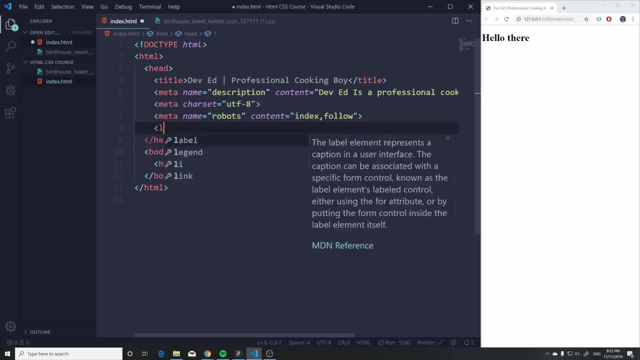 what we're gonna do is right here. we're what we're gonna do is right here. we're gonna say link this time, not meta. gonna say link this time, not meta. gonna say link this time, not meta anymore. and as you can see the link anymore, and as you can see the link. 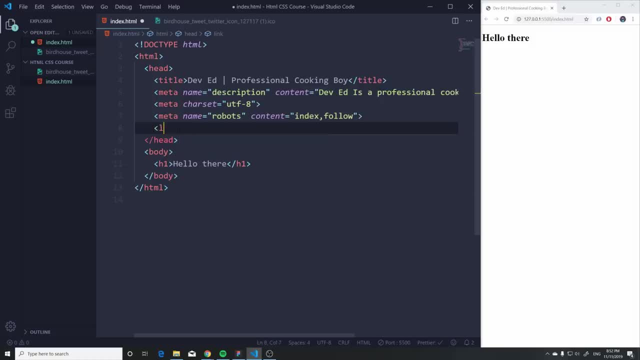 anymore. and, as you can see, the link element allows you, we're not gonna hit. element allows you, we're not gonna hit. element allows you, we're not gonna hit tab here. and I'll tell you why if we hit tab here. and I'll tell you why if we hit. 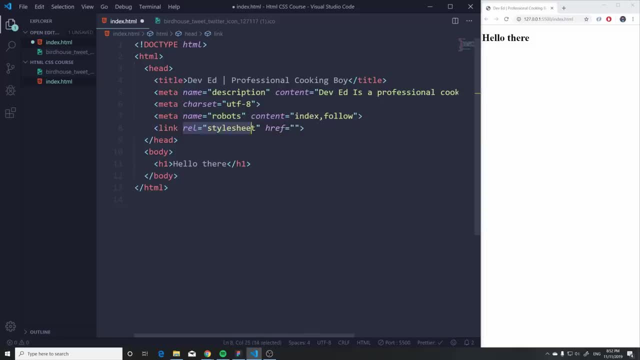 tab here, and I'll tell you why. if we hit tab, it's automatically gonna generate tab. it's automatically gonna generate tab. it's automatically gonna generate us this rel stylesheet href 10: now it us. this rel stylesheet: href 10: now it us. this rel stylesheet href 10: now it does this because it's very commonly. 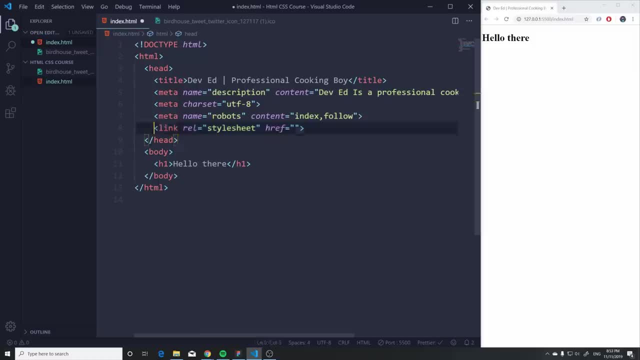 does this because it's very commonly does this because it's very commonly used to link our stylesheet. so this used to link our stylesheet, so this used to link our stylesheet. so this link thing you basically use to connect link thing you basically use to connect link thing you basically use to connect your CSS to your HTML or to connect. 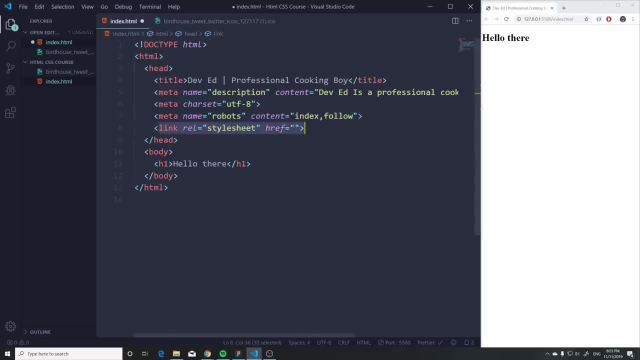 your CSS to your HTML, or to connect your CSS to your HTML, or to connect different things to your HTML. however, I different things to your HTML. however, I different things to your HTML. however, I don't want to do the CSS right now, but don't want to do the CSS right now, but 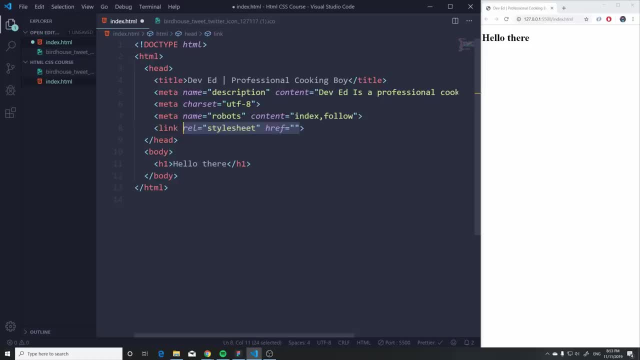 don't want to do the CSS right now, but you attach a logo, so all we do is we have you attach a logo. so all we do is we have you attach a logo. so all we do is we have this attribute. well, here, I'm actually this attribute. well, here, I'm actually. 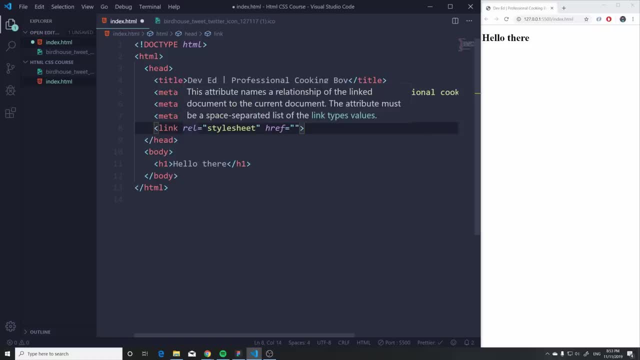 this attribute. well, here I'm actually not gonna delete it and, as you can see, not gonna delete it and, as you can see, not gonna delete it and, as you can see, it's just the attributes name: a. it's just the attributes name: a. it's just the attributes name. a relationship of the link document to the. 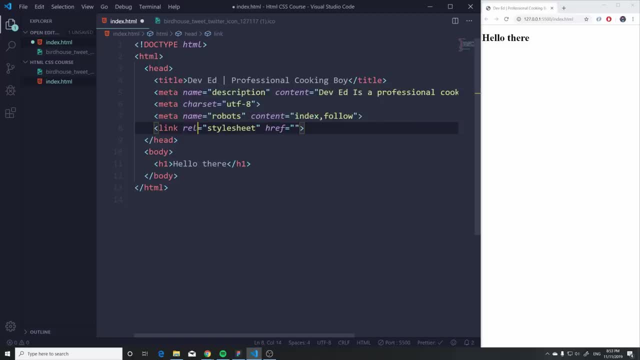 relationship of the link document to the relationship of the link document to the current document. the attribute must be current document. the attribute must be current document. the attribute must be space separate lens- okay, so I think space separate lens. okay. so I think space separate lens. okay. so I think they even have a link type here. so 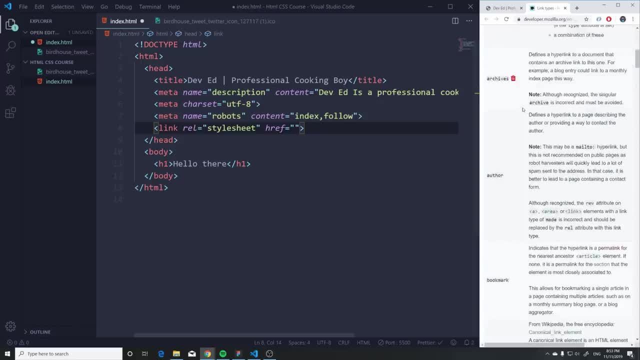 they even have a link type here. so they even have a link type here. so let's open up. let's actually see what let's open up. let's actually see what let's open up. let's actually see what they show us. okay, we have author. they show us, okay, we have author. 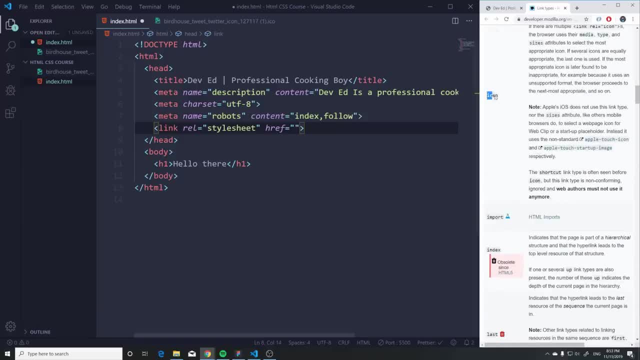 they show us. okay, we have author bookmark, there's a bunch of here. but look, bookmark, there's a bunch of here. but look, bookmark, there's a bunch of here. but look, there's one called icon, so we can. there's one called icon, so we can. there's one called icon, so we can replace that with icon, because that's. 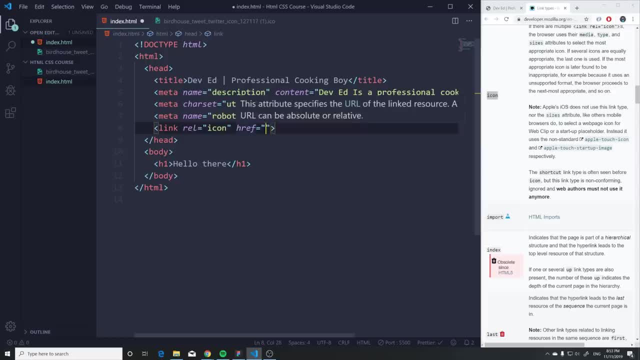 replace that with icon because that's. replace that with icon because that's what we have and href is basically gonna what we have and href is basically gonna what we have and href is basically gonna gonna be the URL or the location of our gonna be the URL or the location of our. 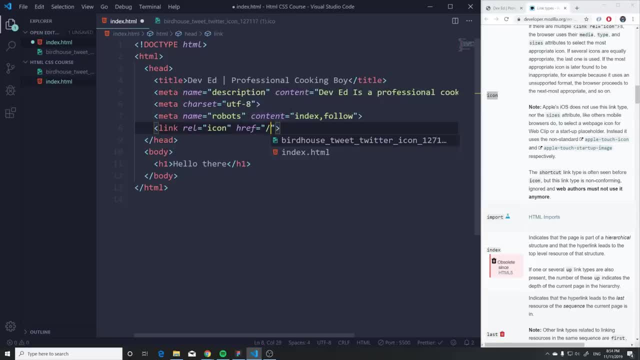 gonna be the URL or the location of our icon, and the way we can find that is we icon and the way we can find that is we icon and the way we can find that is: we can just add a slash and that's. can just add a slash and that's. 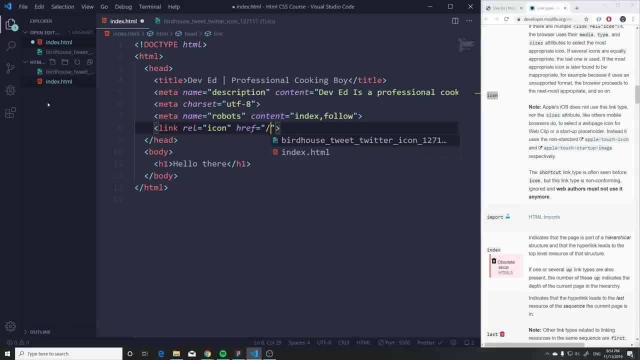 can just add a slash and that's automatically gonna pull up the whole. automatically. gonna pull up the whole automatically, gonna pull up the whole file structure that we have in the left file structure, that we have in the left file structure, that we have in the left, and we can just click on it and hit. 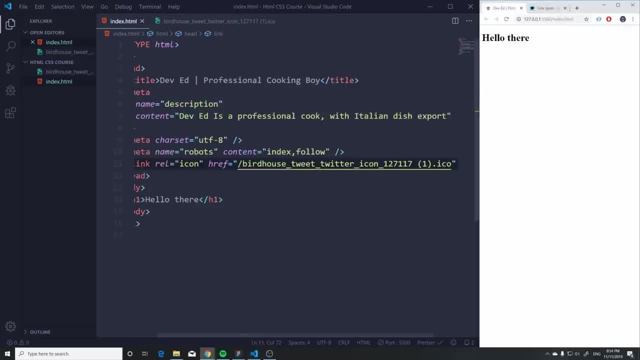 and we can just click on it and hit. and we can just click on it and hit control save and take a look. we have our control save and take a look. we have our control save and take a look. we have our little house, little house, little house. yay, thank you so much. that's so cool. 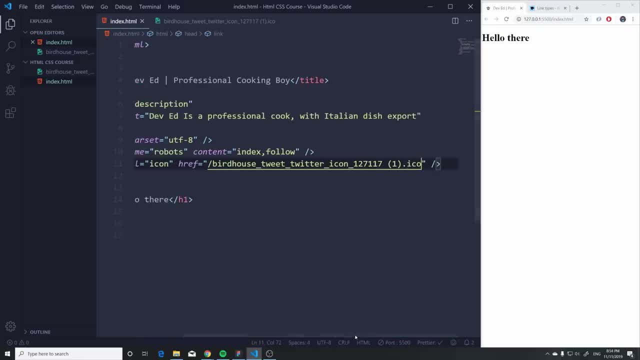 yay, thank you so much. that's so cool. it's so cozy already and our html is empty, but hey, it's a good step. there's one last one i want to introduce you, which can be a bit kind of weird, but it's very, very helpful. so we're going to say: 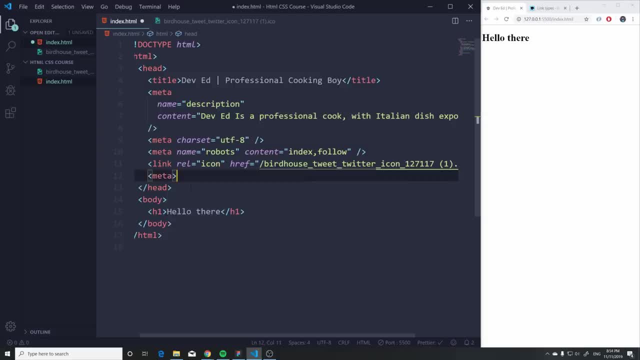 meta: all right, we're going to click on it and then we're going to say name and this is going to be viewport, okay, and the content is going to be equal. just follow along with me here a bit, it's going to be weird. we're going to say width equal to device width. 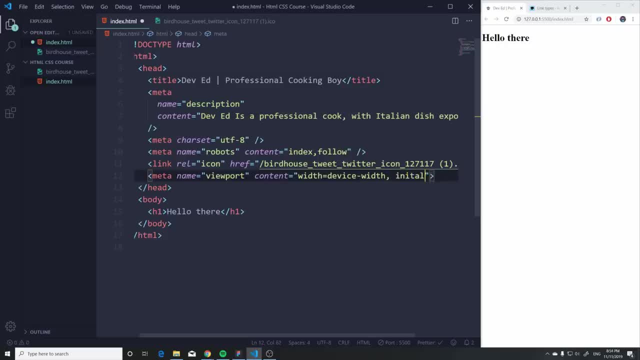 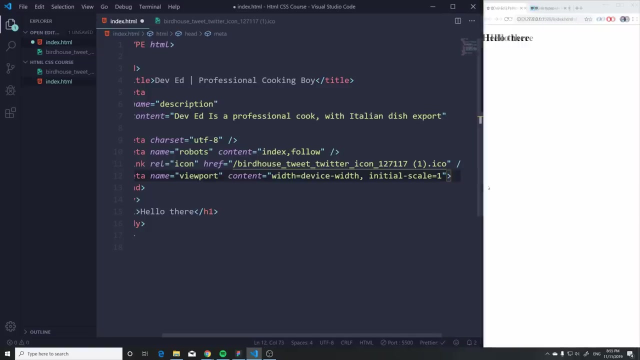 and then we're going to add the comma and we're going to say initial, and then let me make sure i initial dash scale is going to be equal to one. all right, let me make more space here so you guys can see. okay, here we go. so initial scale one, okay, so this kind of looks weird, but all it does. 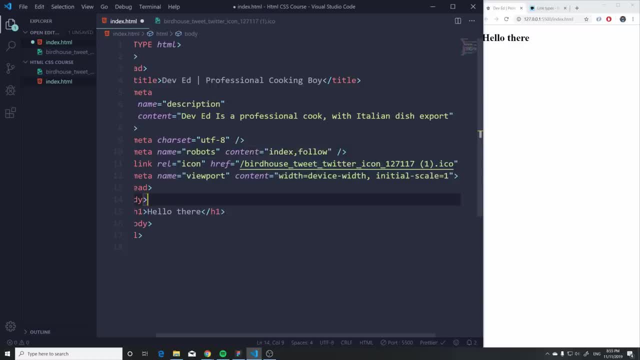 does is well, like 10 years ago, websites weren't really made for for mobile, it was all desktop. so what this helped with is basically scaled the website all the way up till it filled the whole screen for maybe a smartphone or something. so, as you can see, you can kind of read it: width equals device width, so the width 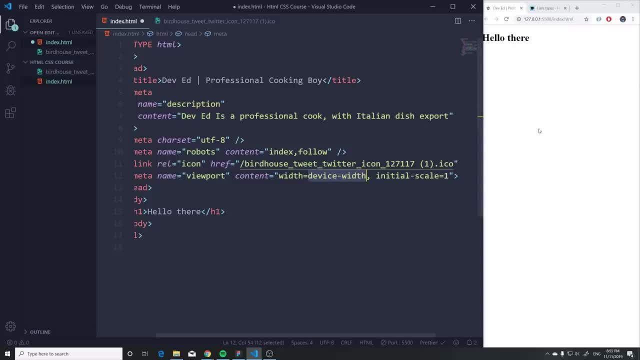 of the website should be the width of the device and the scale should be basically so you can see the whole content. so it should be scaled like one and not zoomed in like this or zoomed out like this. it should be fit perfectly and I actually want to show you a quick example here, and I quickly want to show. 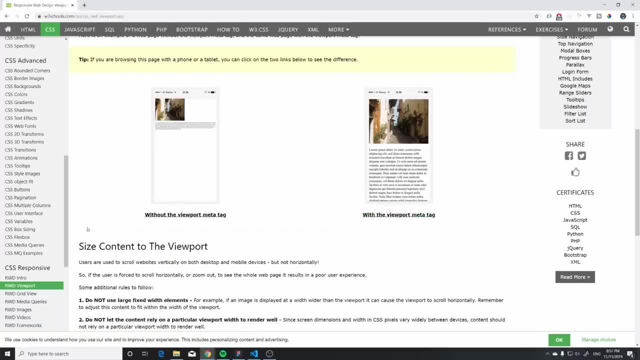 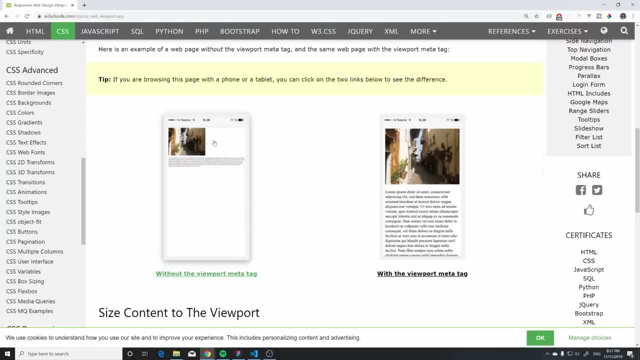 you this example right here on v3 schools, which is a really good resource. as you can see, without the viewport meta tag, this is how our content looks on a mobile screen. however, if we add the viewport meta tag, it makes it more responsive. it takes advantage of the. 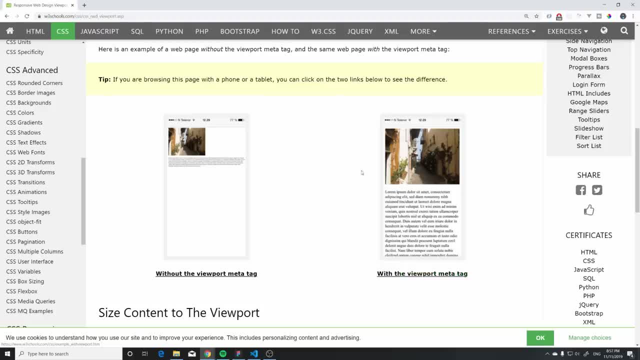 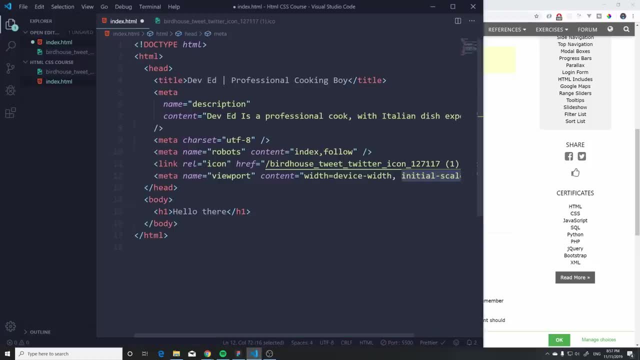 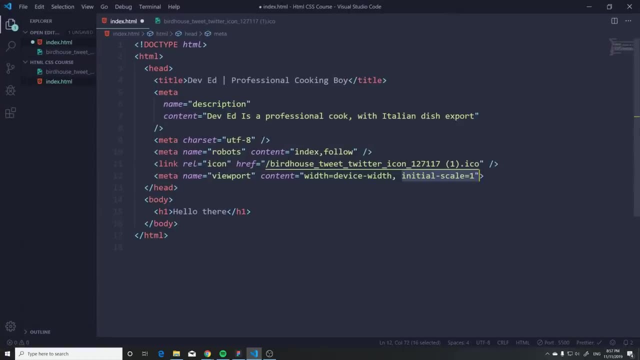 full space of the device, of the width of the device. so that's it. we just usually add this as well without actually worrying about it, and there we go. we have a proper structure of our website. now you're gonna be mad at me because I'm gonna show you a cool new trick to set this up from scratch super fast and 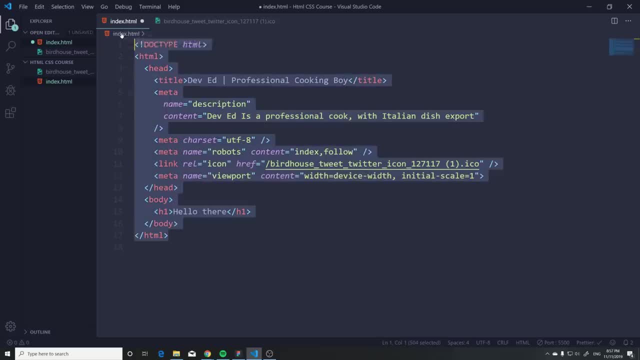 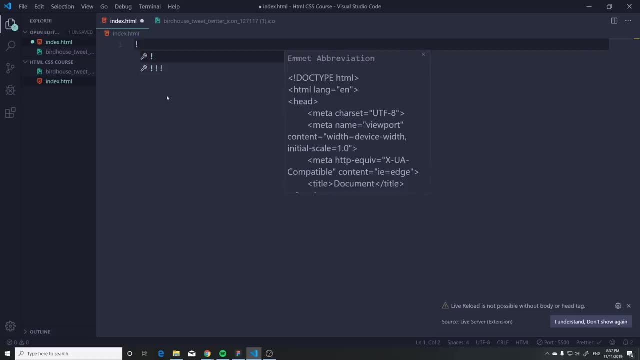 so I'm gonna delete everything here. I'm just gonna cut it out and take a look right here. if I hold shift and press 1, we're gonna add an exclamation point. I'm gonna hit tab and take a look. that's automatically gonna generate us. 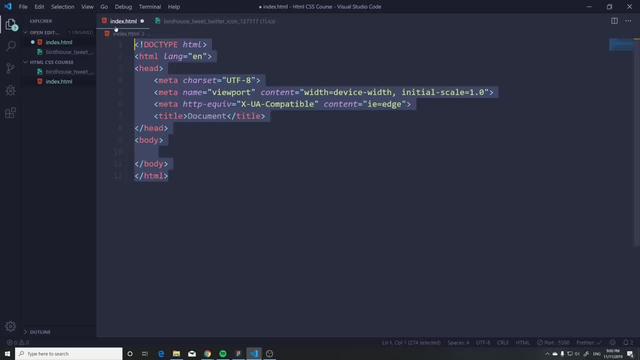 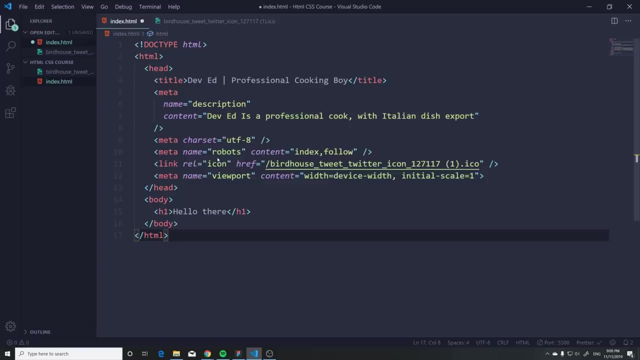 this whole structure. there we go, look how quickly we can do this, just shift tab and boom, we have our boilerplate generated now. it doesn't actually add those other meta tags like the, the ones that we had here, like the robots and the, the icon and the, the. 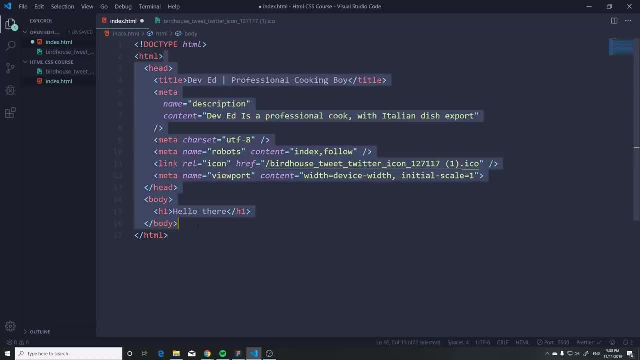 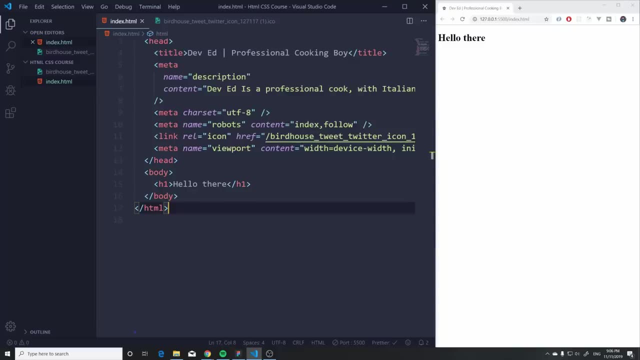 description here, but I kind of wanted to show you the two ways we can do it. you can add it after if you want, but I'm gonna stay with our original one that we have. let's take a look at some fairly common HTML elements that we use. so we 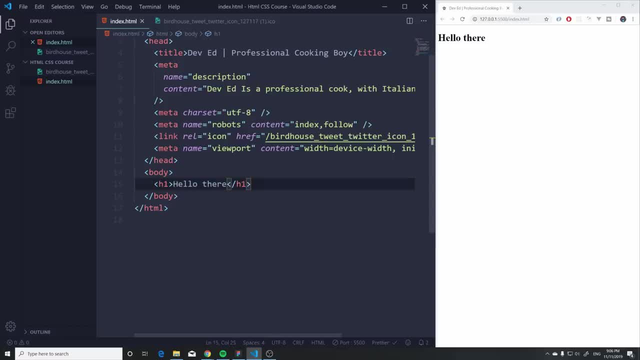 did the h1, which is heading 1. now there are a few others, there's h2 as well, and let's say hello there. and, as you can see, this is gonna be smaller and it goes all the way to 6, so we can. there's actually a cool trick you can do. 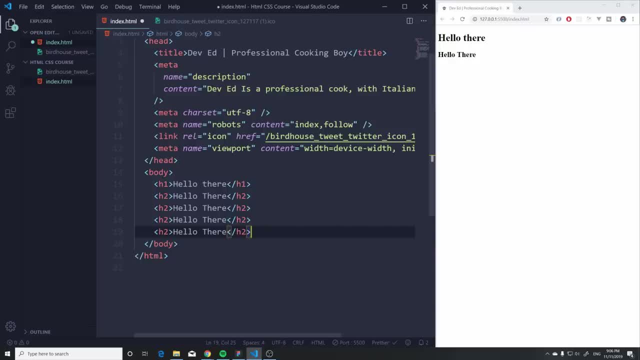 you can hold shift alt and press down on your arrow key and we can rename this to h3, h4, h5 and h6. so let's do that really quickly. oh, my goodness, there we go. h3 and, as you can see, my visual studio code editor. 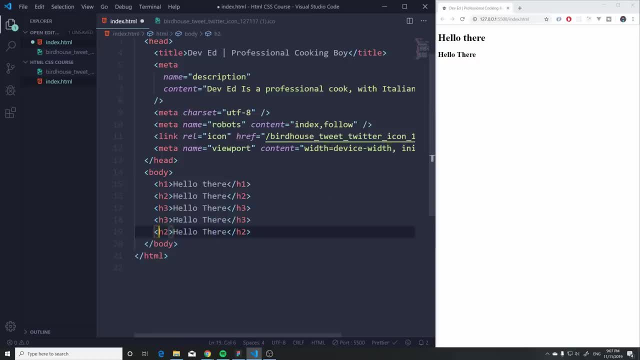 auto completes the last thing if I want to change it to. so if I change this to h4, it changes automatically there too. h5 changes there automatically as well, and this is again just a small little extension that you can add if you go to the marketplace here and you can search auto rename tag and install that auto. 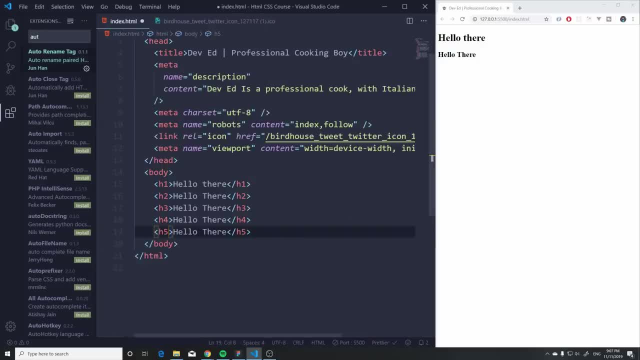 rename tag here installed and you are ready to go. so h5, and let's do h6 as well. let's also copy this. h5 and let's do h6 as well, and let's also copy this and just say hello there. so these are all the different headings that you can. 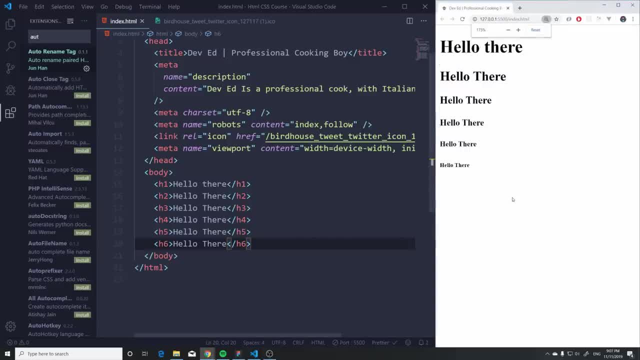 use. I'm gonna zoom in a bit here so you can see: okay, and basically you would use these as titles, you would use these as logos, and also what I want to clarify is that the importance matters here. so heading 1 is way more important than a. 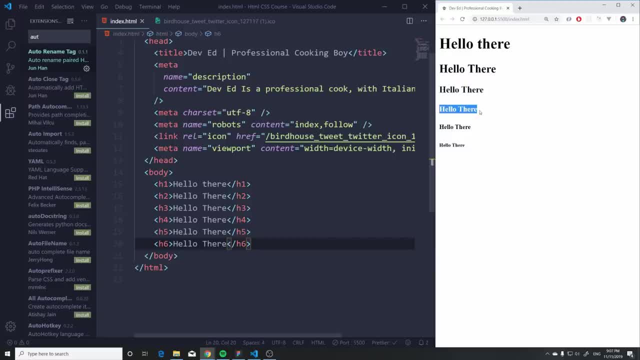 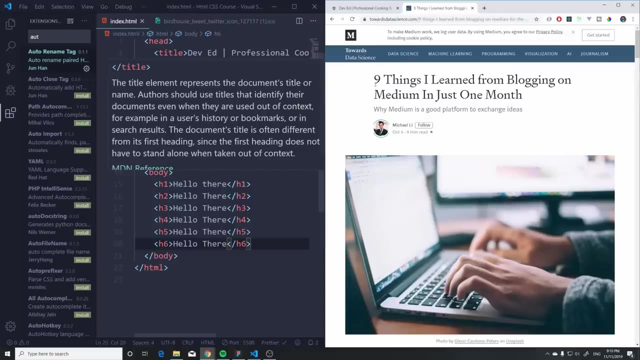 heading 3 or a heading 4. okay, so to give a proper example, let's go and navigate to a website and see what's up. here is a quick example that I want to show you. on this website, you can use the headings to give importance to the things that you have on the page, so maybe the logo here. 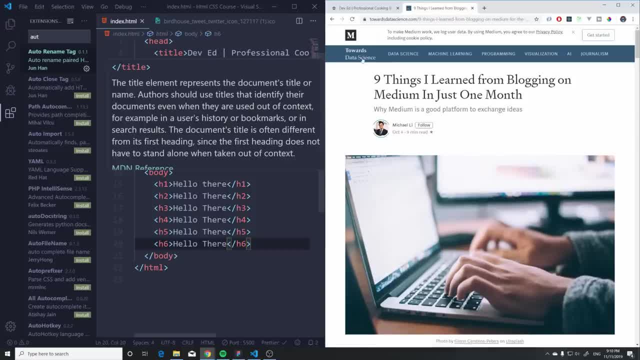 towards data science can be a heading one, because that is very important. this site of your name is very important, so you would add it as a heading. the title of this article can be a heading 2, because it has it's still very important. you might want this to. 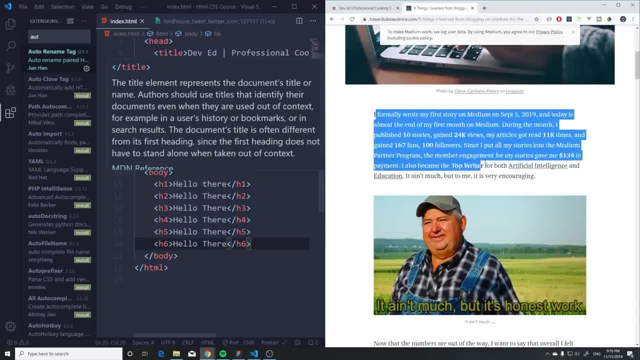 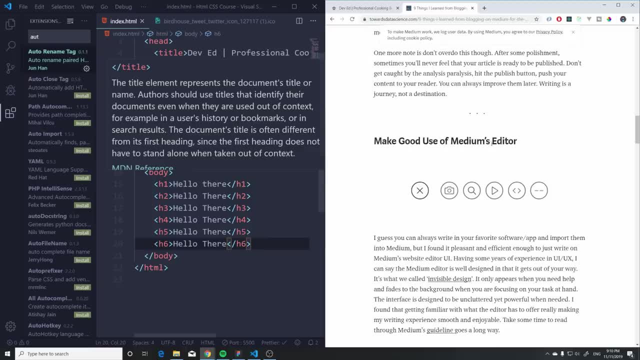 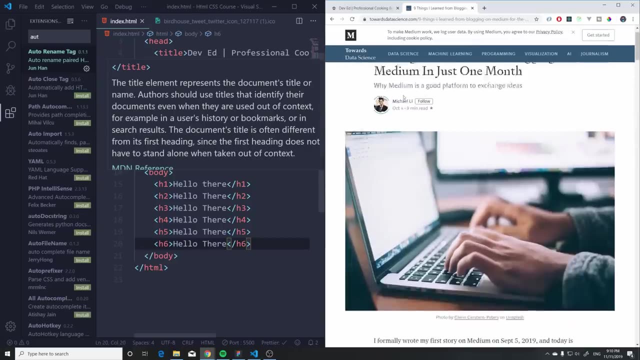 show up in search results and then you have some paragraphs going on here and if you go down, this might be heading 3, so it's kind of like a subtitle and another heading 3, another heading 3. okay, so you basically have one important title up here and then you would go down in the headings and so on and so forth. 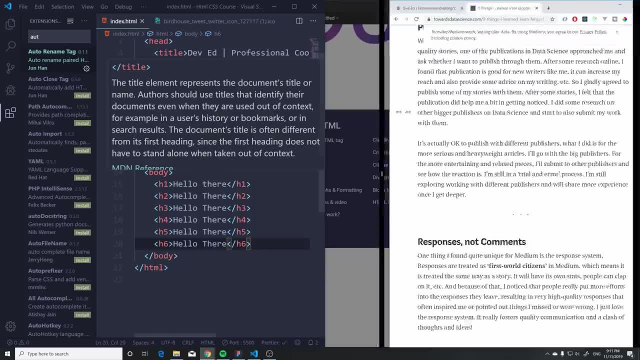 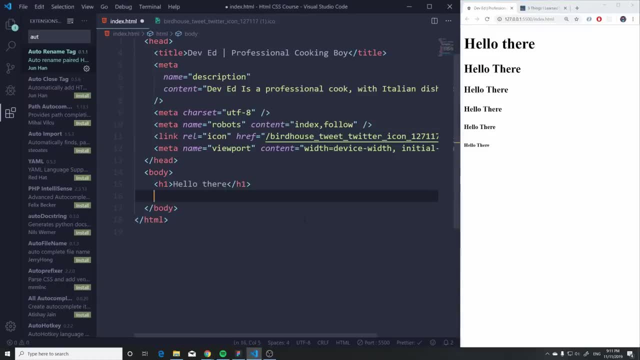 okay, so that's a very quick example on headings. we're gonna obviously implement this, our website and, as you can see, besides these headings, we also have paragraphs. I'm gonna get rid of all of those. we're just gonna have the h1 to create a paragraph. what you're gonna say is just say p and hit tab, and. 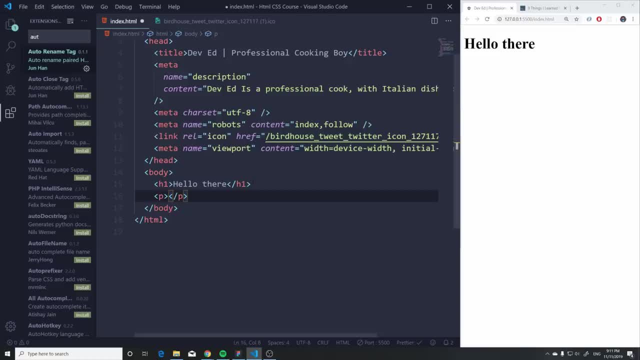 boom, we have a paragraph element. so here again, hello there. this could be just some normal text, and there we go. you could use this now. I'm zoomed in so it's probably not as big for you. so let me zoom out something like this and, as you can see, the browser. 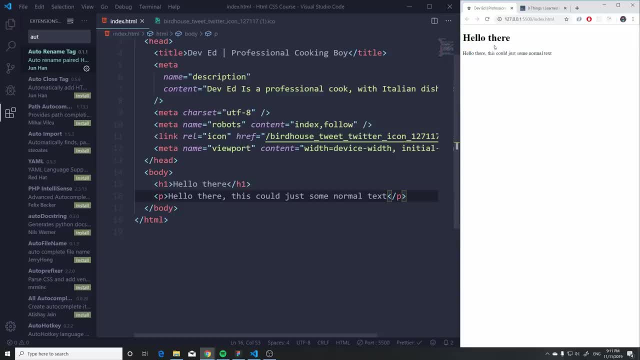 also puts like a basic font size on it. it styles it a bit for you. this is bold. it just creates some basic styles and it kind of varies from browser to browser. as you can see, there's also some space in here. if I duplicate this paragraph and hit save the space in between, these are not necessarily exactly the same as. 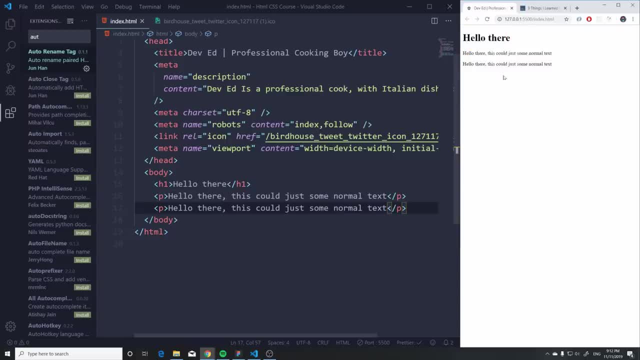 with the header. so, as you can see, the space is bigger here. so the browser does do some basic styling automatically for you, and I also want to point out when we are gonna get to styling: you don't really want to use headings just to give your text some bold font to it or make it larger. all right, that's, that's not. 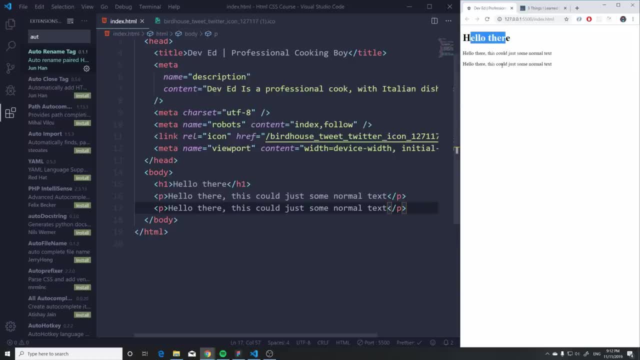 why we use headings. headings should be you to give importance of the structure of our HTML and the importance of of the text on our website. that's why you use the headings. all right, you wouldn't use a paragraph as as the title of, maybe an article post. okay, because we can style. 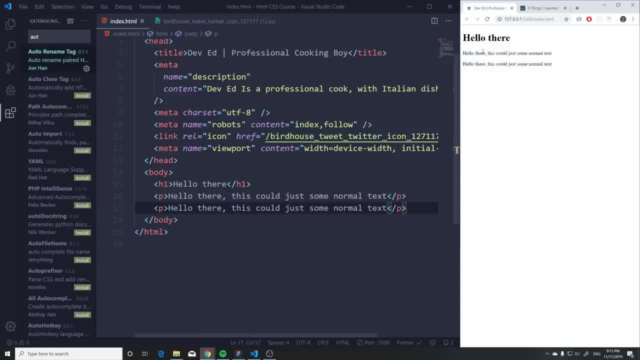 this. if we want to look like this, that wouldn't be a problem, and also you might just want some bigger text. I don't want you to straight-up jump to a heading just because it gives this automatic styling for you. really, I want to show you some elements that help us format our text here and our heading, and 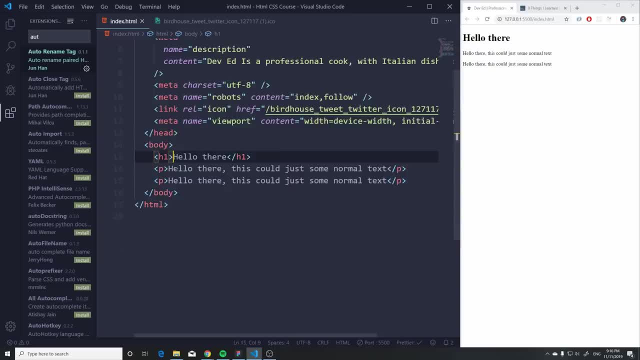 everything else. so what we can do is we can actually wrap, so we can go in the paragraph here and we can wrap something inside another tag. so again, we can do this nesting that we kind of already did in here. we have the body right, that's the parent element, and then we have all these small ones nested inside. 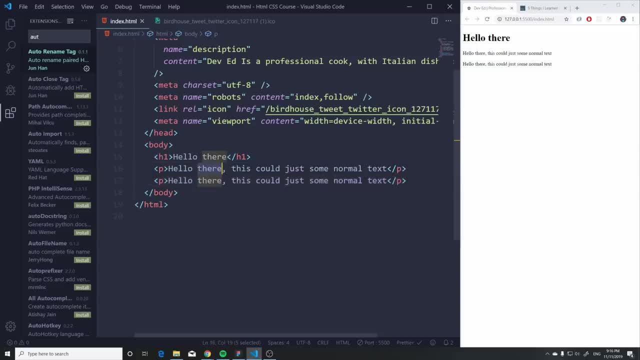 okay, same thing I can do here with the paragraph. I can nest another element inside here, so maybe I want to make this last one italic. okay, so this could just be some normal text. I want to make this italic, so what I can do is go here and 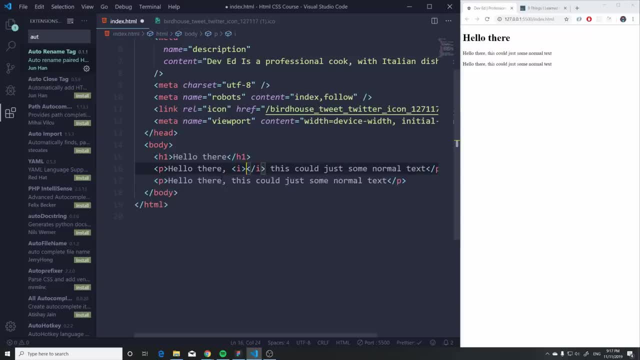 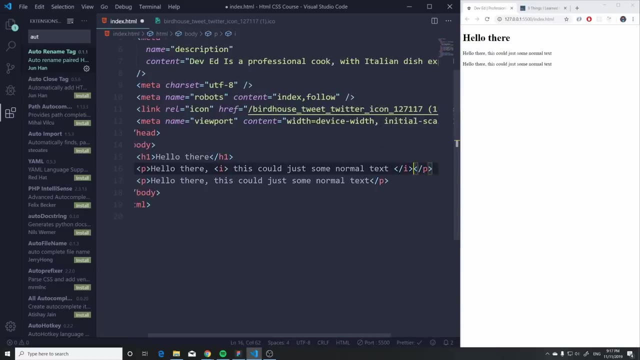 just add a space. I'm gonna say hi and hit tab. as you can see, that's gonna generate it for me and I can take the ending, ending, closing tag and just wrap it around this like this. so this looks a bit weird, but it's. it's actually very simple. you just have the paragraph and then you 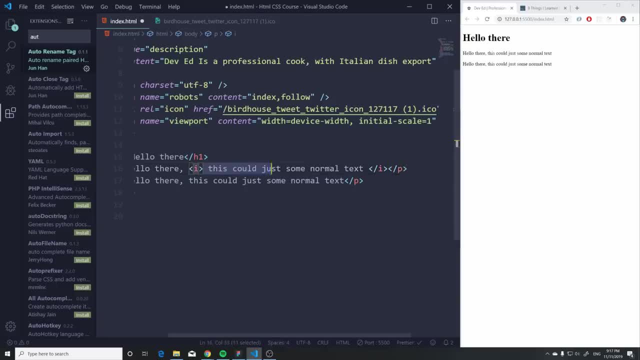 just wrap the following text that you have inside this: I- and if we hit save, as you can see- I'm gonna zoom in a bit here- that's gonna make it italic and there's a bunch of them. let's replace this with strong hit save, as you can see. that's. 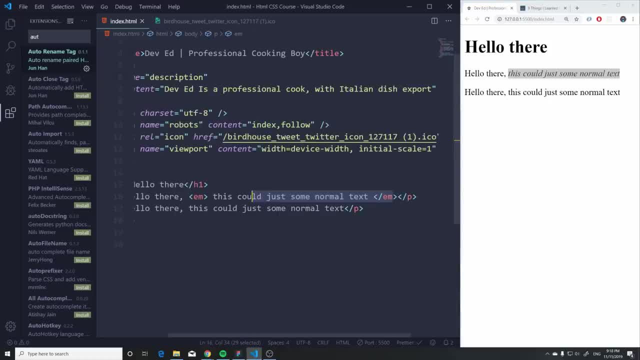 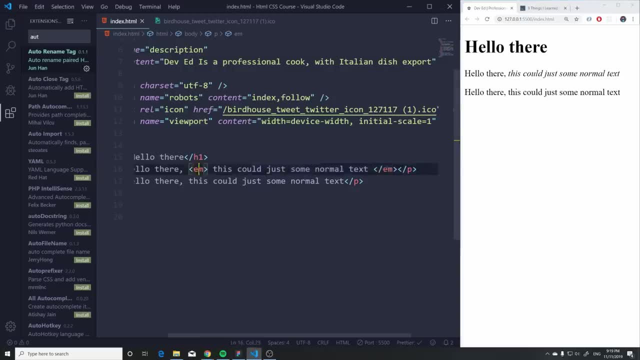 gonna make it bold for us. so there's a bunch of them here. I'm not gonna go through all of them because we're not gonna be using these as much as you might be thinking, but let me just show you how to do that. so let's go ahead and 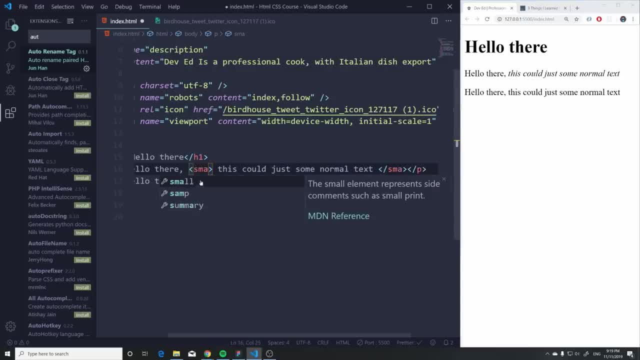 show you a few for fun. there's one called small and, as you can see, it kind of pulls it up here for you. you can kind of see what it does. it represents a side comment, such as a small print. so if we hit save, we have this, we have small, we. 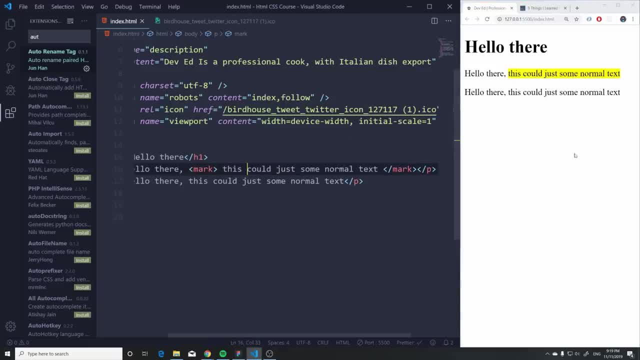 also have the mark. let's hit save and, as you can see, this kind of marks. it like with the pen, with the blue, not blue, it's yellow. with the yellow marker, it's kind of like you drawn over it to mark it. and there is also one delete, which is kind. 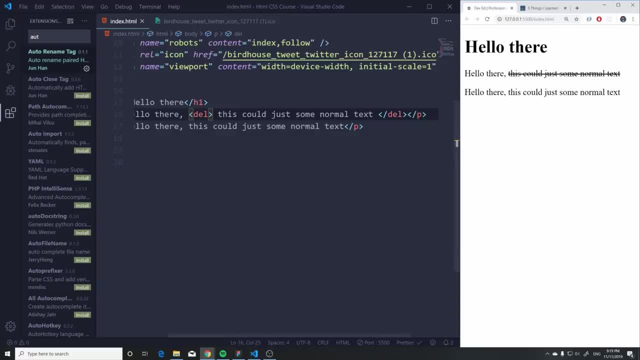 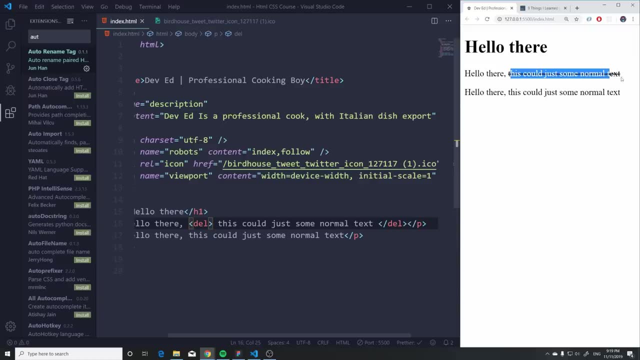 of gonna cross it out like that and there's just a bunch of them that you can use. but again, we're rarely gonna use this it's, we're not gonna be using it as much. but if you ever need it, you you know at least what to look for. you can. 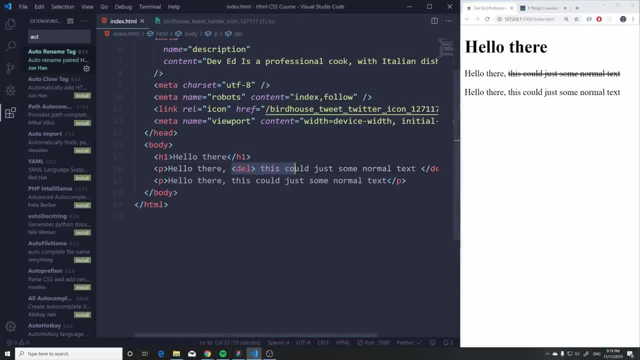 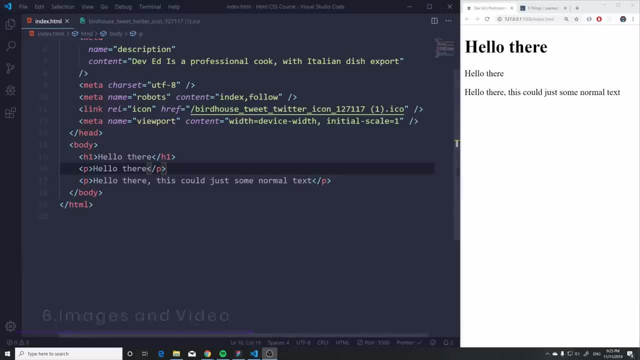 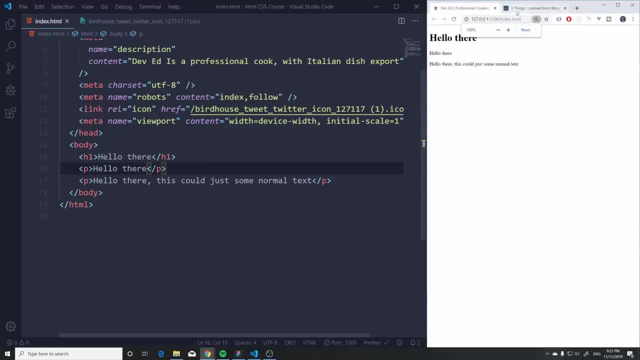 just search up a. you can just search up a formatting 4d text. next up, let's take a look at some images that we can add to this little website that we made here. there's not that it's it's not amazing, but hey, we are getting there. so what I want to do is I'm gonna show you a cool website. 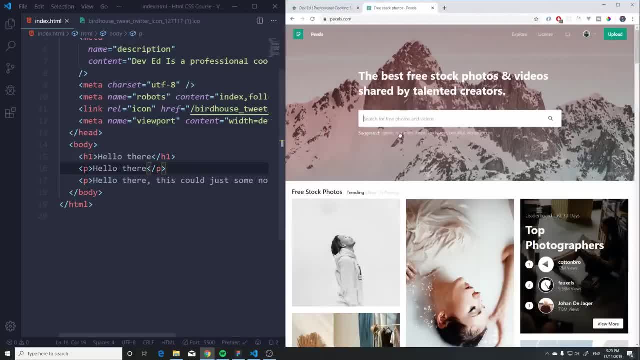 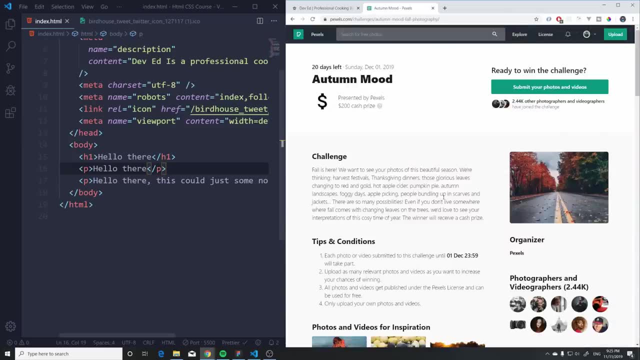 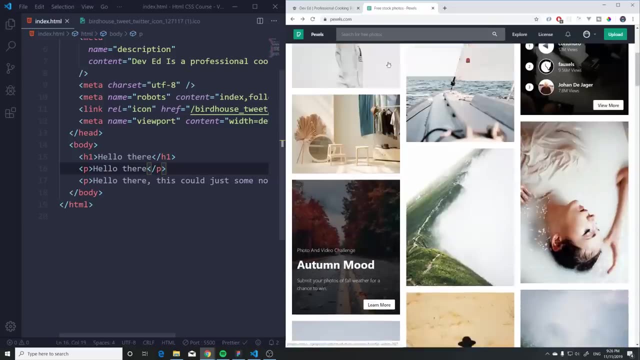 for images. it's called pexels and they have some very high quality images, so let's search for one to add autumn mood. it's almost winter here, but hey, oh, never mind. this is like a photo submission thing. okay, let's move on. let's hey, who doesn't like mountains? everybody likes mountains. I've never. 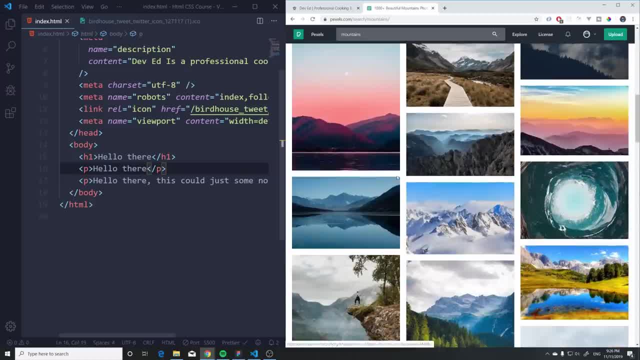 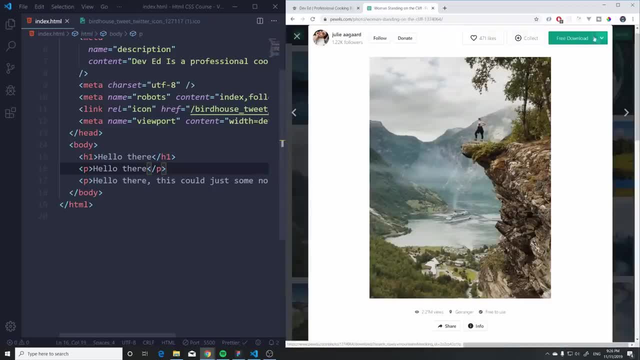 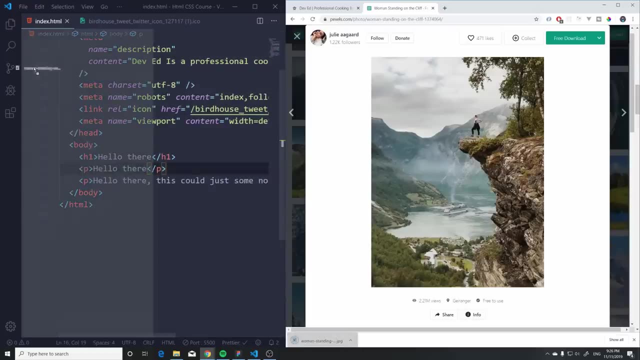 been to. actually, I've been to like one or two, not not too big of a mountain, but okay, this lady on the mountain, take a look at that. very nice, the boat is underneath- perfect, so it actually gives you multiple sizes here. I'm gonna get a medium one and hit download and all I want to do is just drag this inside the. 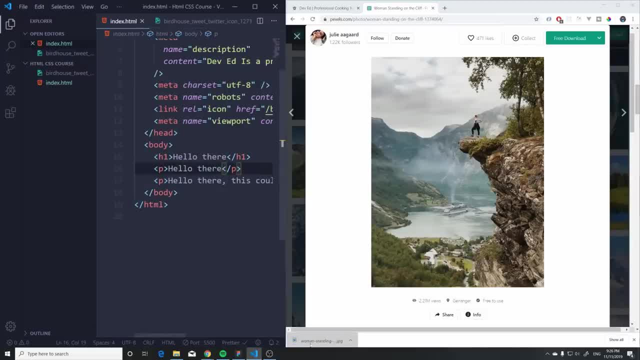 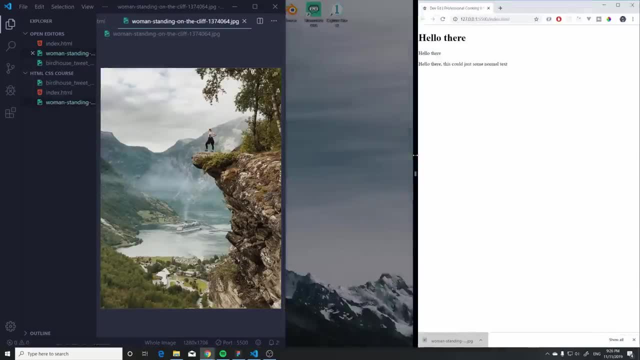 folder here now. I don't have that open, so let me open this up. I just closed it, so I had the extra space and drop it in there. perfect, so we can close this up. let's make the screen bigger here now. as you can see, it's a little bit bigger than. 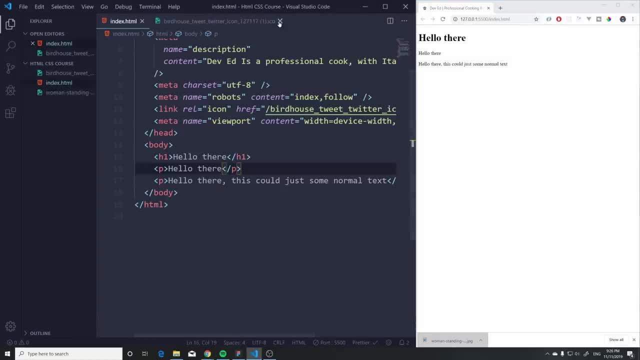 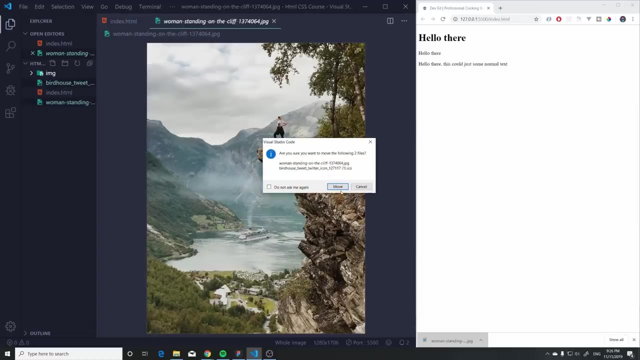 it should be, but, as you can see, the file structure already starts getting a bit weird. so what you can do is actually create a folder here, a new folder, and we are gonna name this image like this shorthanded image: perfect. so now we can take the woman with the boats and the birdhouse and just drag it in there and 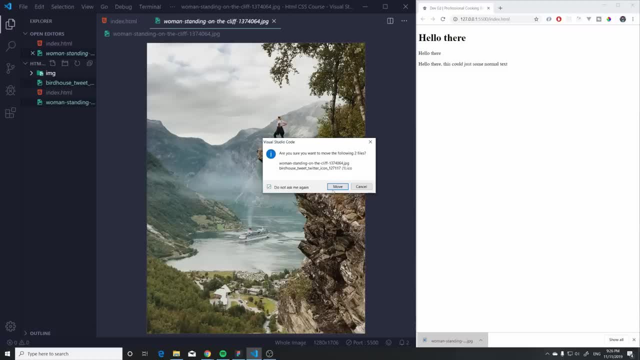 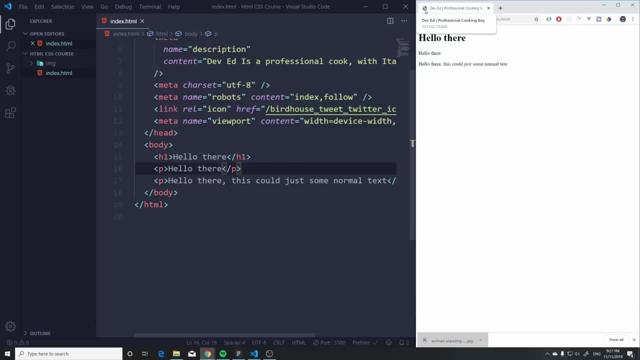 then it's gonna say, hey, are you sure you want to move it in there? and you're gonna be like, do not ask me again please, and then move it there. perfect, okay, let's refresh. but take a look, our icon is gone. why we gave it a path here. that's not there anymore. so if we add a slash now, as you, 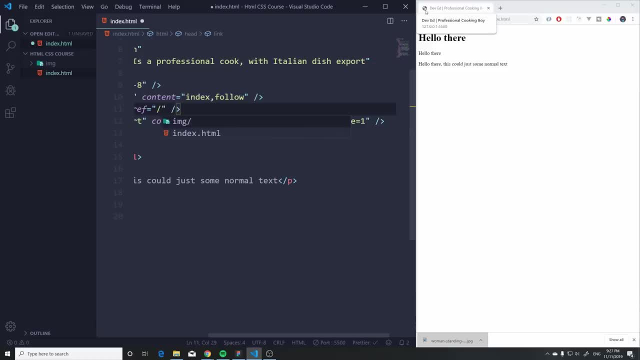 can see. there's no image there, so it's automatically. it's gonna be like: oh, I don't know what to do, goodbye, it's not even gonna bother looking for it. oh my goodness, Mr HTML, why you do this to us, why you do this. so what we need to do is: 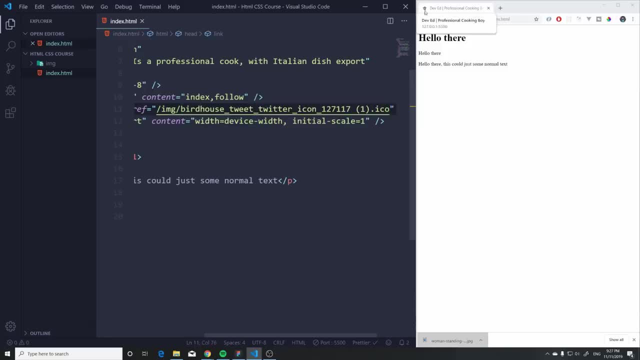 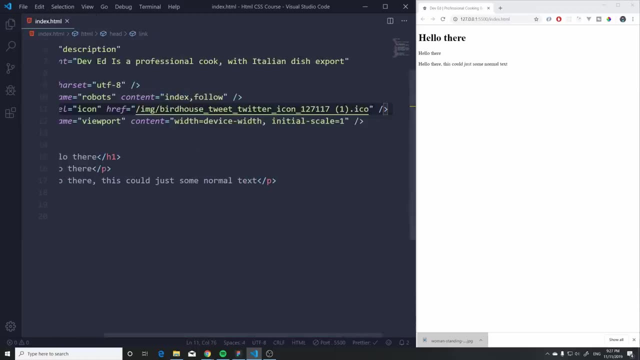 navigate to the image and now hit the birdhouse and then we're gonna get the logo back, the icon back. okay, great, so let's put the image here. how do we do that? I'm gonna close this up here, just so we have more space and all we have to do it's gonna be very simple: just hit enter and we're gonna. 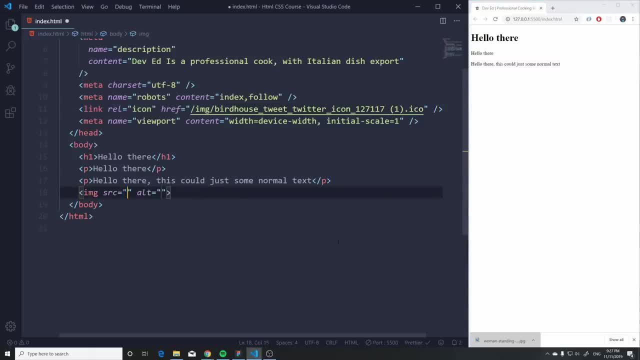 say image, and we're gonna hit tab again. okay, and take a look, this is again one of those elements that are that doesn't have a closing to it. it's just simple like this and it's gonna give us an alt and a source. I'm gonna delete this alt. 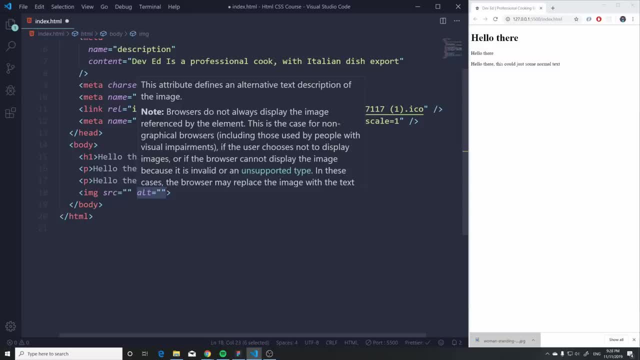 because we're gonna cover this in another section, but all it means to quickly explain it to you. it's just an alternative text for the people who cannot view this image. maybe the image doesn't load. maybe people cannot see the image for various reasons, so you can add a description here to: to whatever you. 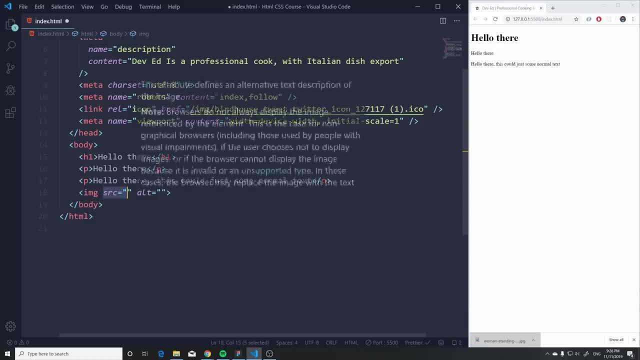 have on the image. okay, you basically describe the image in words, but for now we're gonna remove it. we're gonna get back to it, so don't worry. but we have this attribute called source, which kind of works the same way as this link thing. so you just add the path to the image that you want to use- source- and as you 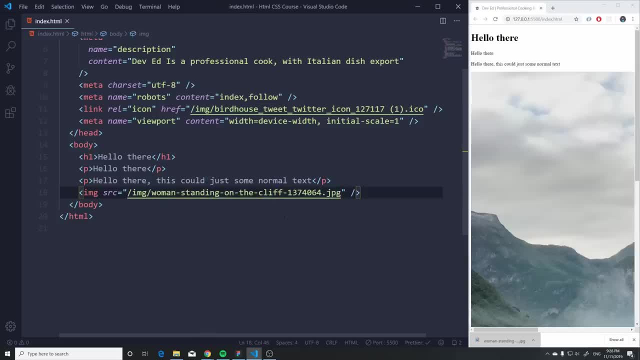 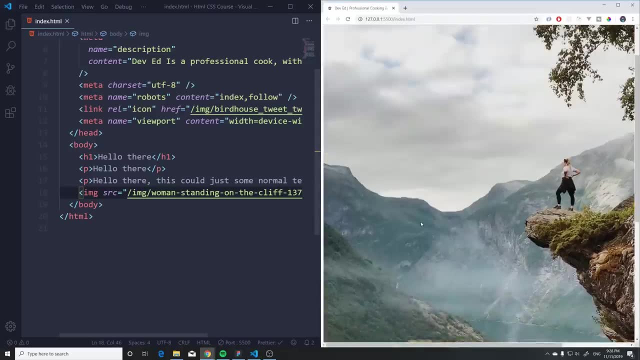 can see, we have the woman in the background and we have the woman in the standing on the cliff, so we're gonna hit ctrl save and take a look, we have this now. it's gonna put it in the original file size, so it's gonna be extra large here, as you can see. we can scroll and go. 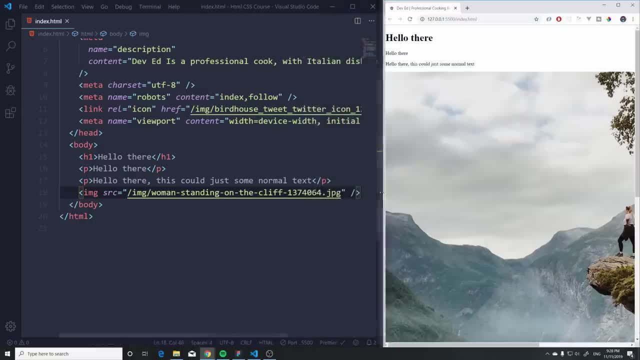 crazy. now there are a few attributes that you can also add here to make the smaller, so you can actually set a height and a width to it. this later on we're gonna do it in css, but for now take a look, just to make this a bit more more pleasurable to look at, we can just add a width. 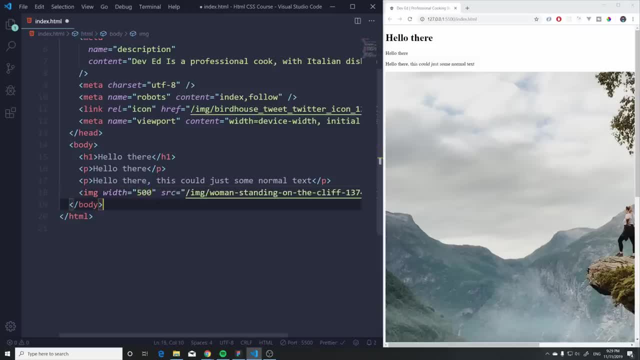 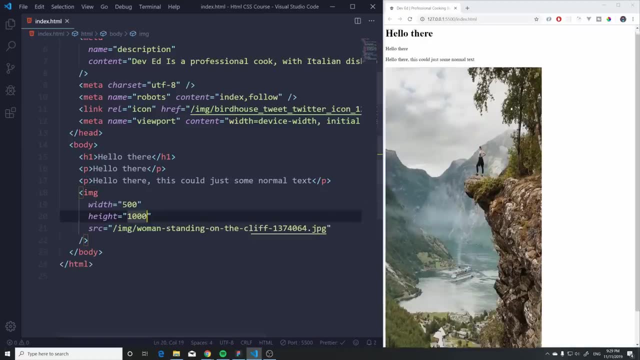 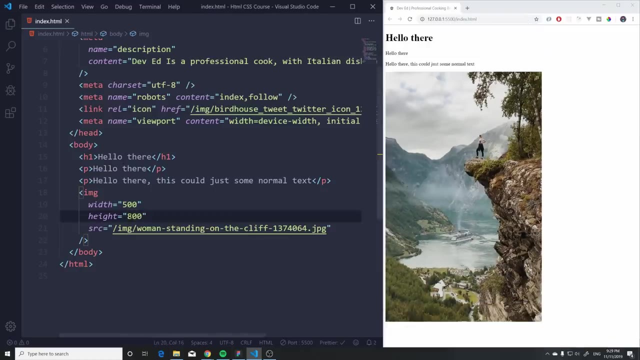 of 300, for example, or 500, and a height of, let's say, a thousand. okay, let's see if that's too large. okay, this kind of looks a bit squished, as you can see. it doesn't look that nice. so let's change the height to 800, maybe. okay, we're getting there. let's do 700 and that's. 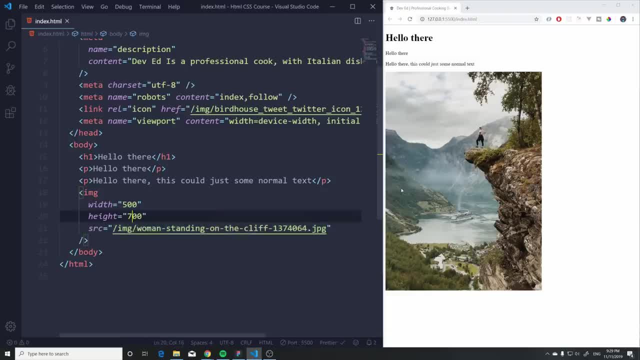 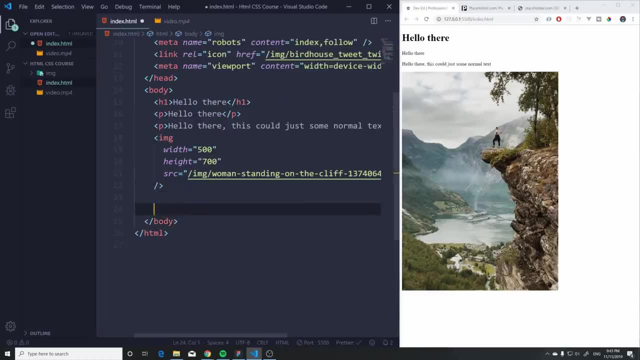 gonna be fine. so there we go. that's kind of the original aspect ratio of the image. perfect, so looking good. okay, let's quickly jump into the video. so to add a video, you can say video and we can hit tab and, as you can see, it automatically gives us. 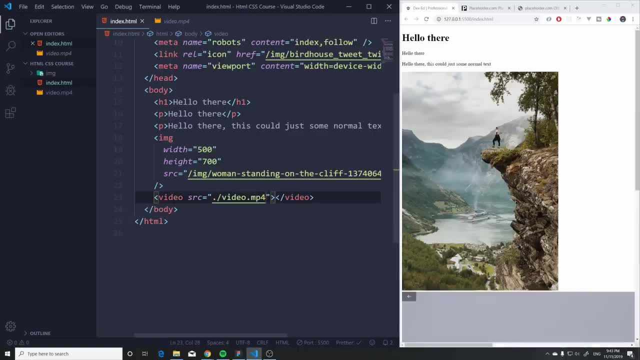 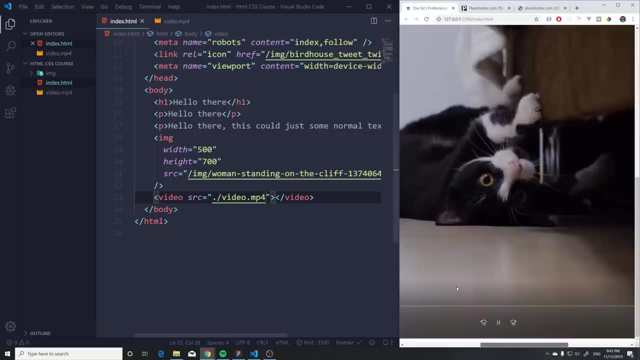 a source. I can just say: dot slash, and I have a video here with my cat. so there she is, she's doing mischief. she's very bad, but she's cute, okay. so this is super large again. so what we can do is just add some attributes here, like height. I'm gonna give it this five for now and I'm gonna 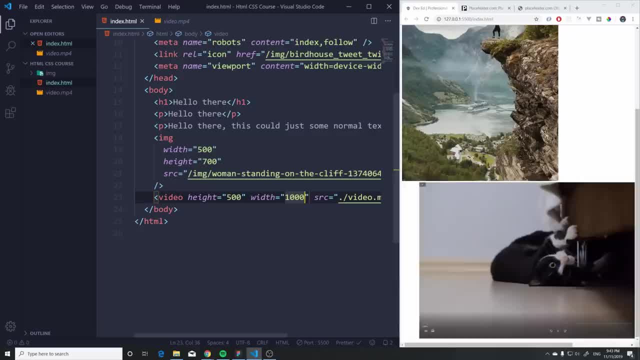 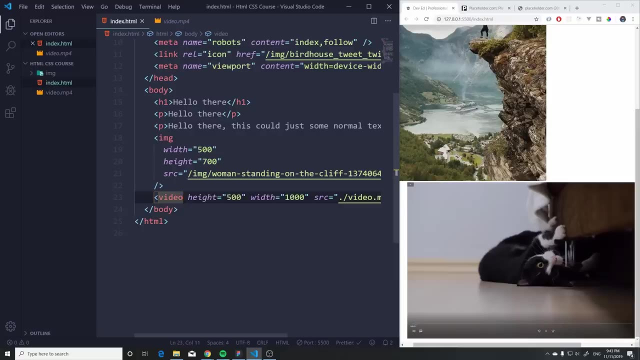 hit 500 and add a width of something like 1000.. it's safe. okay, made it small again. well, I cannot play this and it's just a picture. so what we can do is: I want controls, I want to be able to play this, scroll through this and make this full screen and things of that sort, so to do that we can. 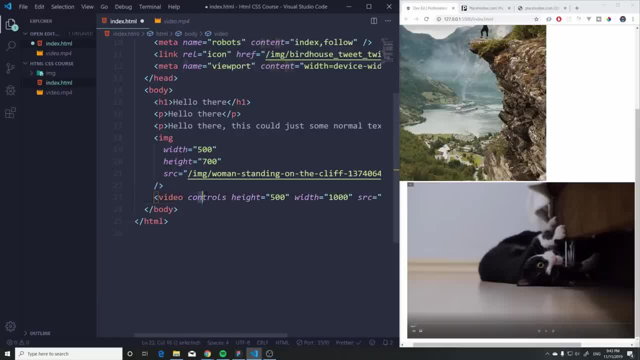 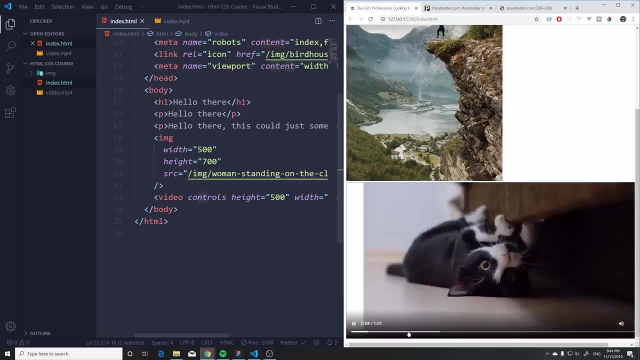 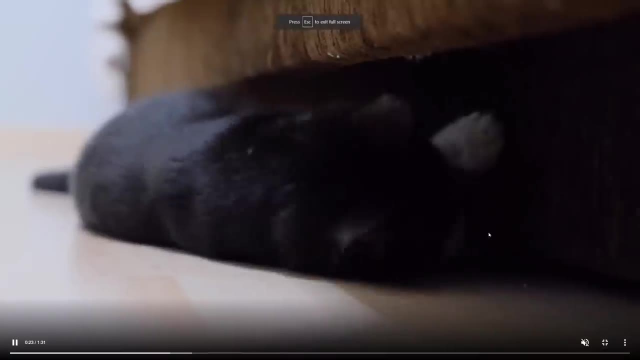 actually add an attribute called controls- controls. there we go, hit save and take a look. now we can play the video. let me make this a bit larger. we can skip forward. we can also mute the sound if we want. this video doesn't really have any sound and we. 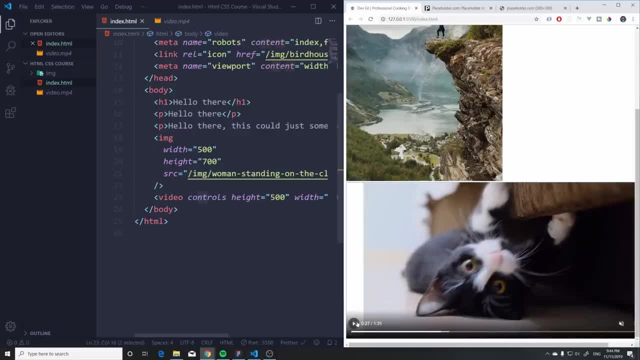 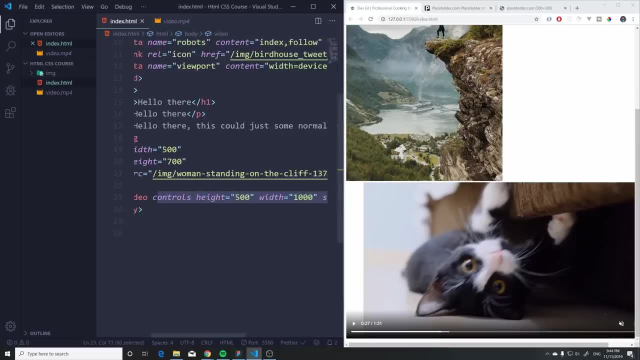 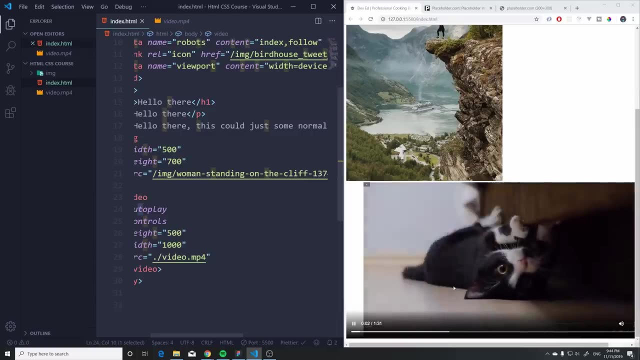 can also full screen this. so, hey, everything works perfect. okay, so that's that's pretty much the video there for you. you can also autoplay this if you want. so when the page loads up, you can just say autoplay, we can add this attribute, hit save and boom, there we go. it's all the place for. 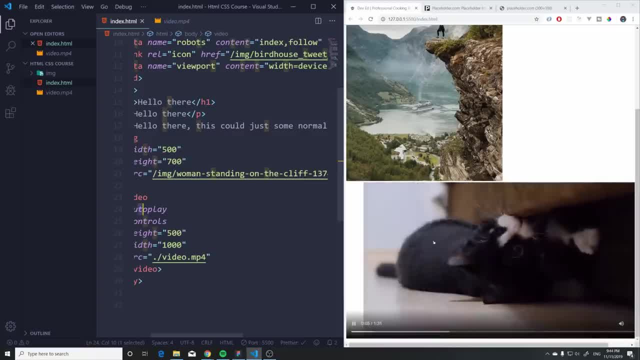 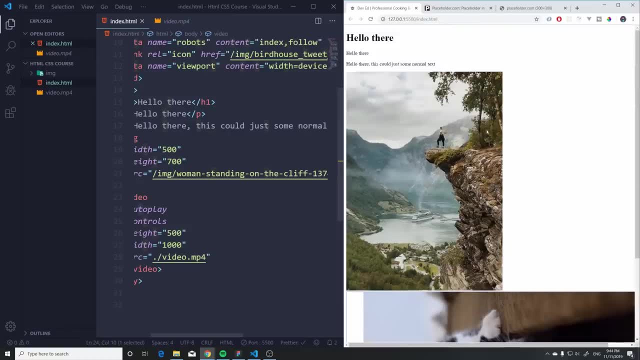 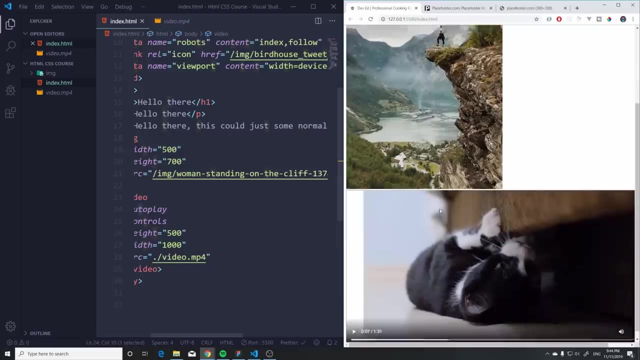 us. I wouldn't really recommend doing this if you just have videos laying around here, but it might work well if you want to do it as a presentational style maybe. maybe you have a website where you have those big, large videos playing in kind of like in the background just as a visual aesthetic. 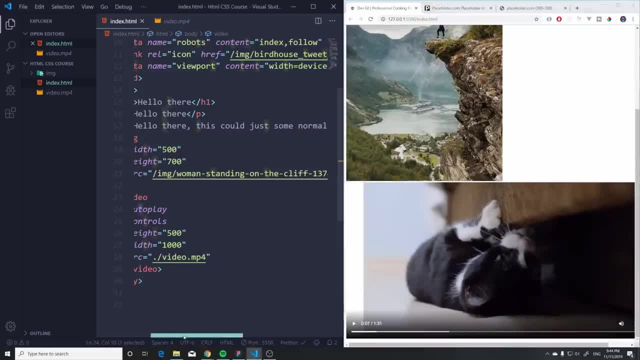 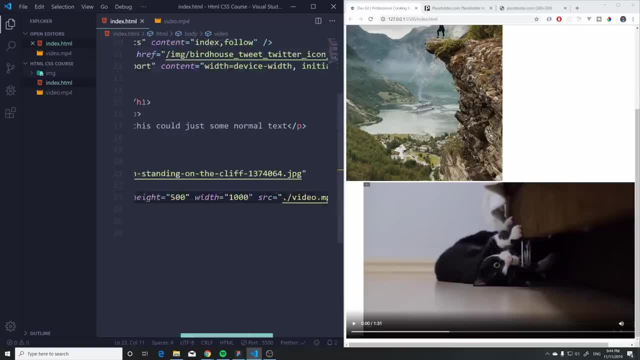 so that kind of works okay, but hey, we have this as well. there's so much we can do with video. now, actually, what we can do is we cannot, if we want, we can not give the source here on video we can actually provide. so let me remove this. we can actually provide. 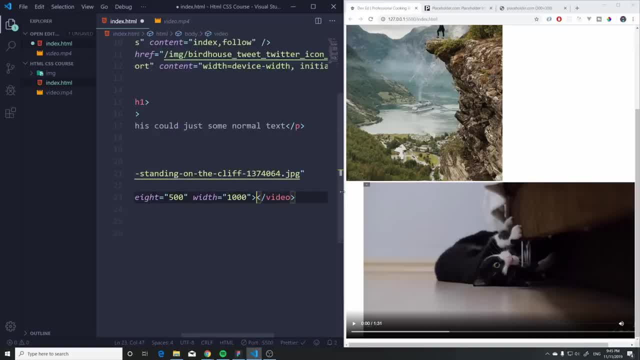 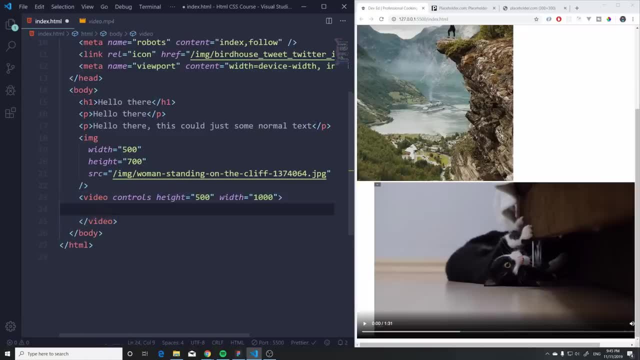 a source in here, so I'm gonna open up the video. let me just close this, make more space. I'm gonna open up here. so we are inside the video tag and here I can provide multiple sources if I want, I can say source and set the source here to video and before, and I can also add the type of 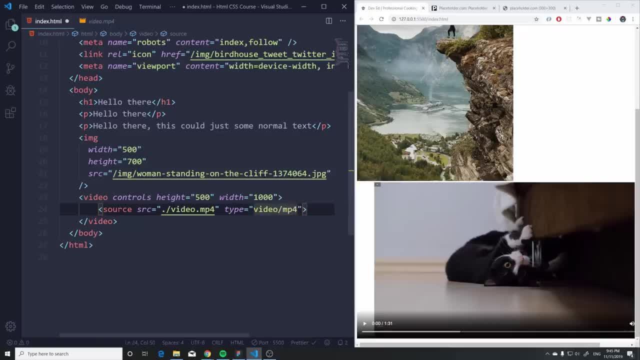 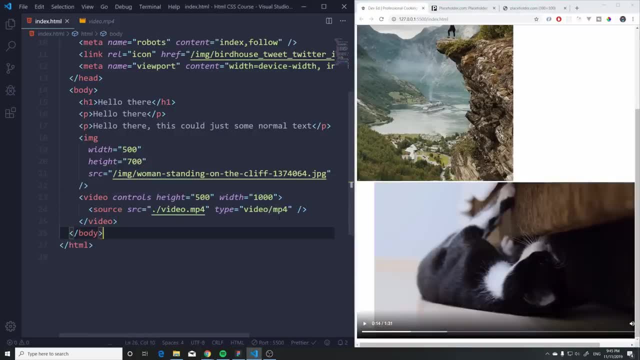 video, and before dash and before to make it clear. so what's what's the deal with this? well, it's generally kind of the same thing, but if you have, maybe the mv4 might not be supported. so what you can do is you can add multiple sources here and the ones that's going to be supported is going. 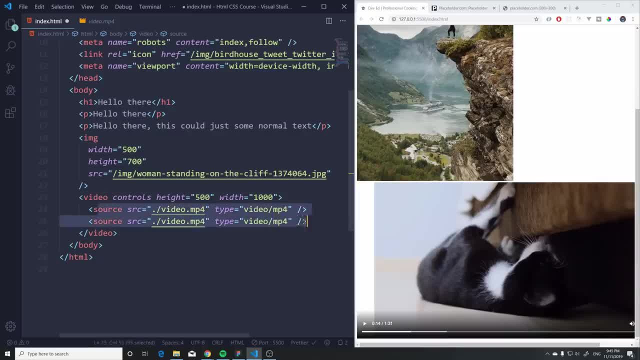 to play. okay, so you can add multiple formats of your video just in case it's not gonna work. but generally you can be fine just using the video here without this source. and, uh, the most common types of support video formats are mp4, webm and ogg, so as long as you use those, you're probably going to be fine. 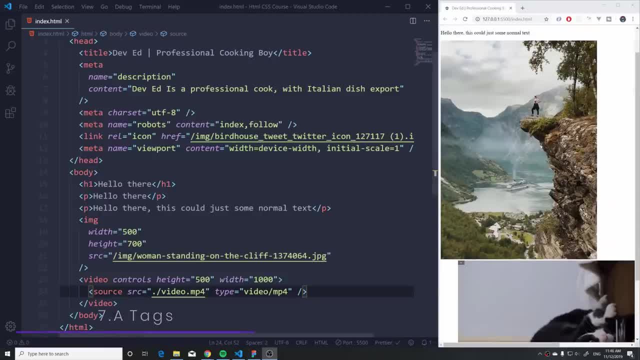 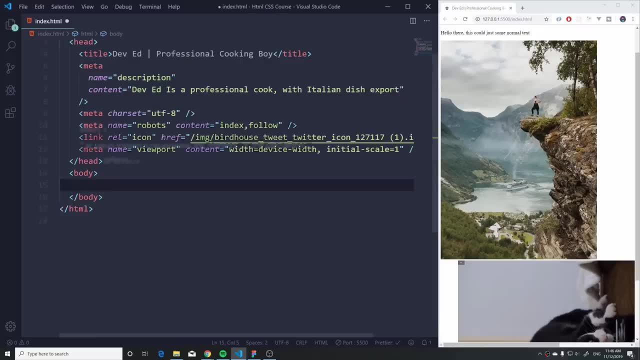 okay, next up. what i want to do is actually clear everything up here because it's starting to get kind of messy. so let's remove the video, the images. actually we clear the whole body. okay, everything is removed. so control, save, and that's going to get rid of everything. so i want to show. 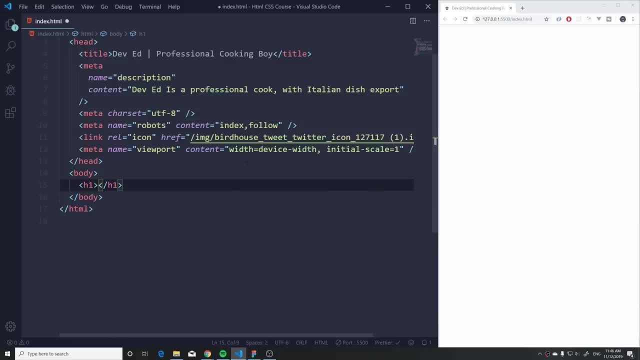 you how links work. so let me just add a h1 here so we do have something on the screen. hello there, link and hit save so we get that. and now under this i want to add a link, maybe to my youtube, or let's just do something simple. so what i can do is i can press a and hit tab and that's going to. 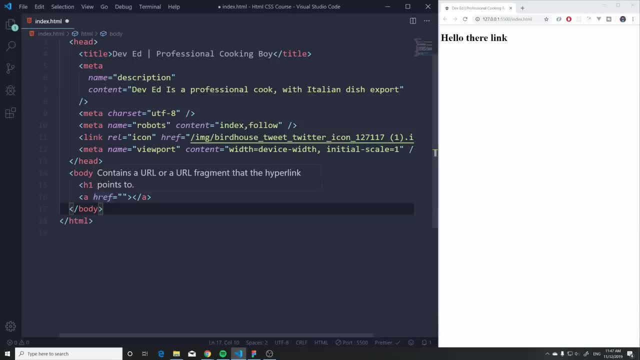 generate us an anchor tag and, as you can see, it has this href, which all it means is that you need to add a link to the link that you want to add to the link that you want to add to the link, that link kind of like this link up here. So this can be a bit confusing. here, Anchor is going to be the. 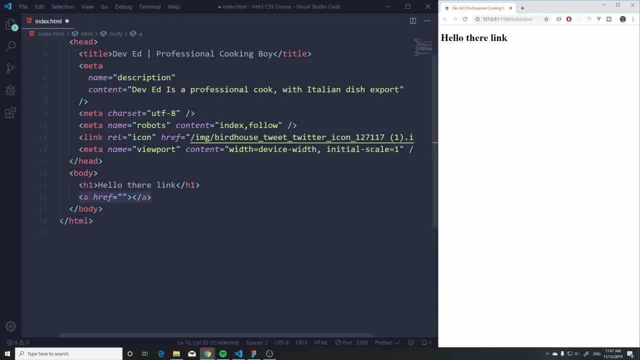 link that you click on to visit a page, but this link is actually different. This is basically for linking your icon or linking your style sheets in the header. So anchor is used to actually have links on your website. Okay, so let's provide one. Which one shall we do? Let me pull up, let's search. 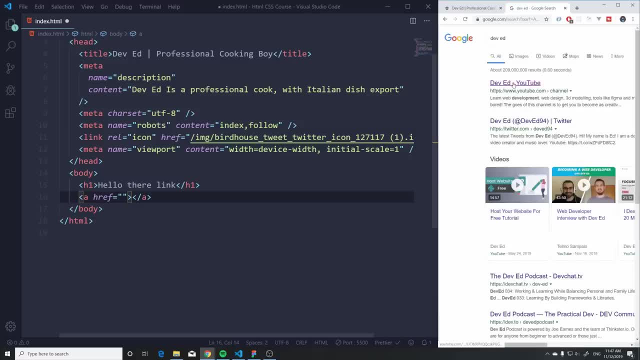 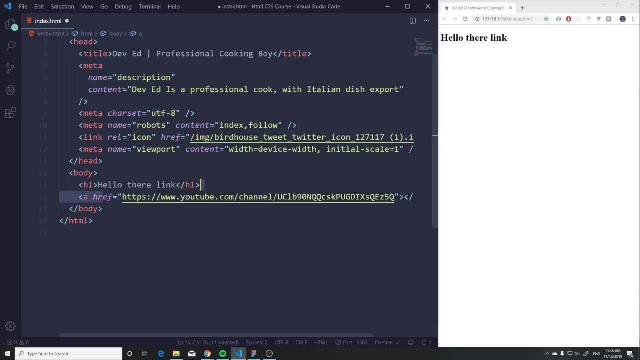 for DevEd here. I'll do my YouTube channel for now, but all you have to do is just copy the link and we're going to drop it into the A tag here and to the href. my apologies and hit save And you. 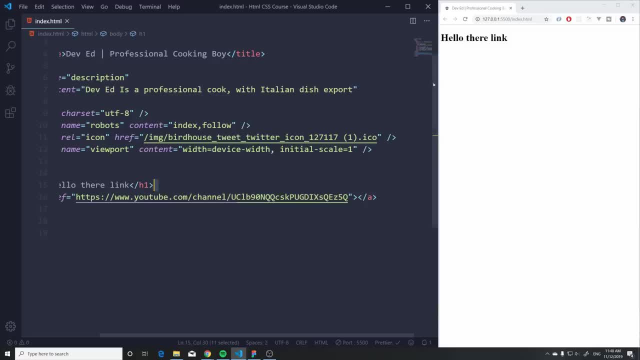 might be wondering: okay, well, there's nothing here. What is this trickery? Well, we also need to add some text here, so it shows up as a link. So what we can do is say DevEd's YouTube, like that, and hit save. There we go. 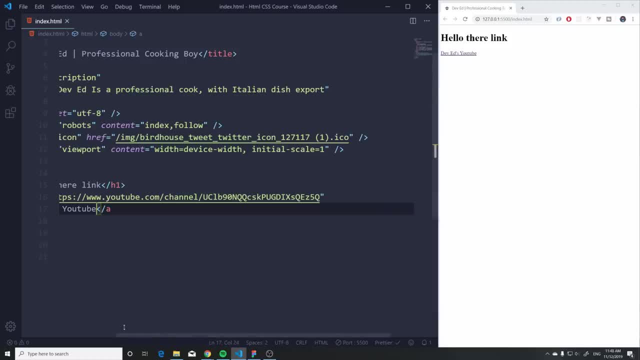 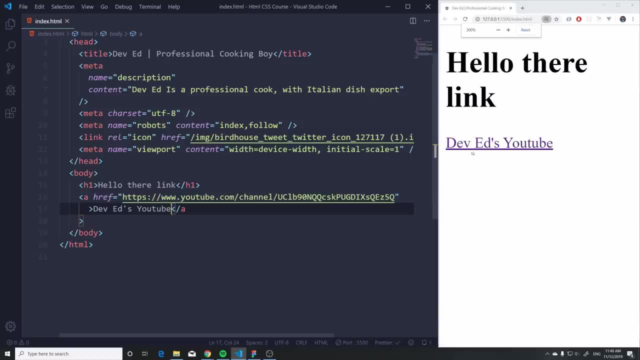 And, as you can see, now we have that And, as you can see, this again has some basic styling on top of it. So you have this kind of bluish color. Is it bluish? It's purplish, purplish color And it's underlined. 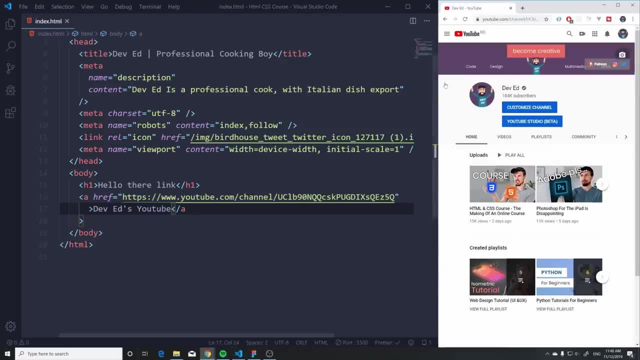 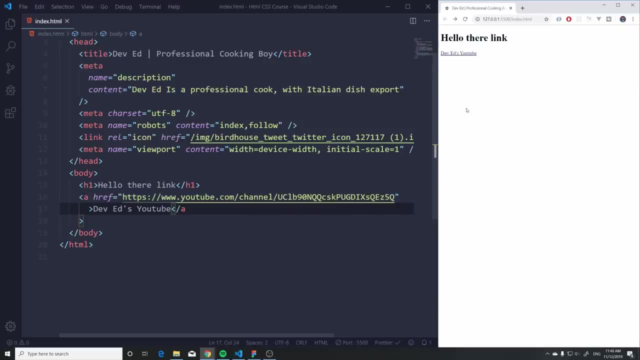 there. So when we click this, it navigates to the link that we provided here. Okay, that's cool, But, as you can see, it actually opens up the page here and we left our original destination, And sometimes you don't want to do that, especially if you have a website, or maybe you have your portfolio right and people are 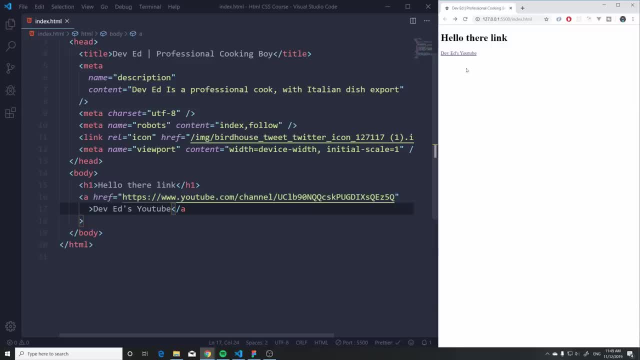 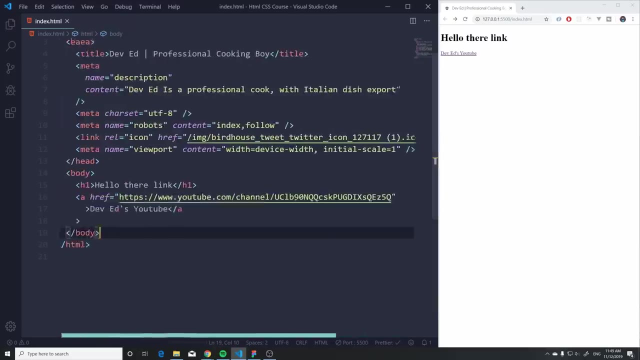 looking at it And then you click on maybe a project that you made, and then they leave your website, basically Right. So what you want to do is you can also click on this and it's going to open up in a new tab. So what this means is there's an actually an attribute here called target, And by default, that. 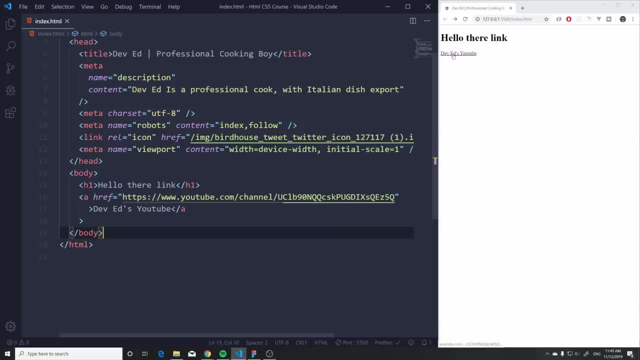 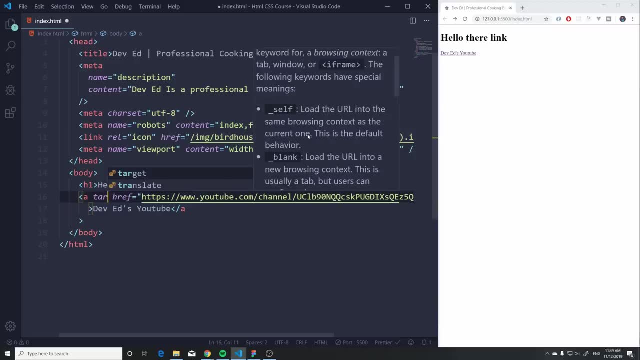 target attribute is going to leave the page and it's going to just go straight to the link that you sent it. Well, we can go here to the tag and we can say target like this And, as you can see there are a few, It's. 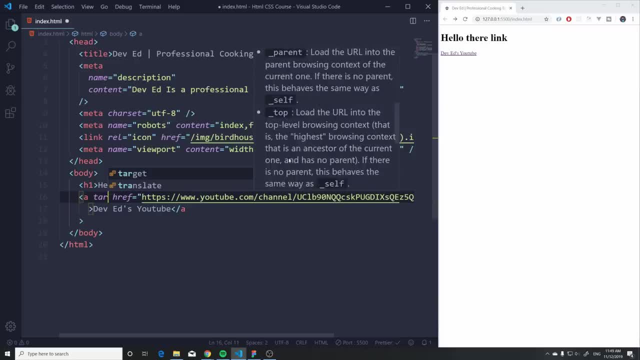 very nice VS Code. This is just fantastic. It gives you all the options that you have. So, as you can see, it has self. All right, This is the default behavior, So it's going to redirect, But then you have this blank And all. 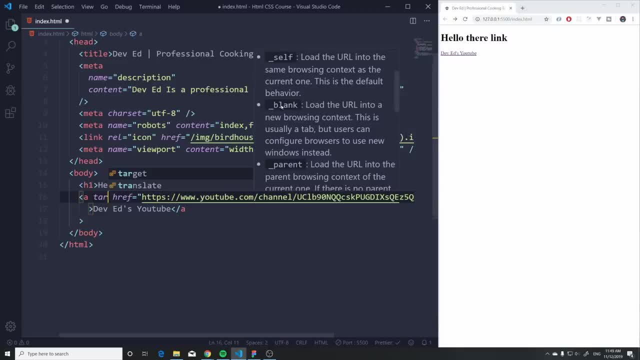 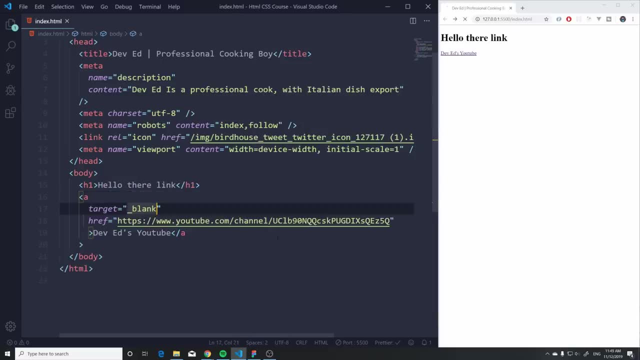 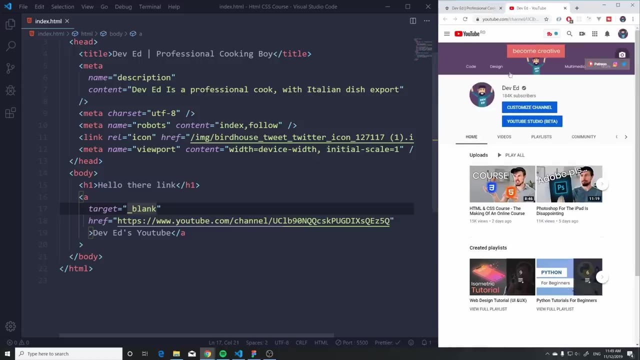 it's going to do is it's going to open up in a new tab. So this is exactly what you have to write: target and underscore blank. So let's do that: Target, underscore blank. See if that works. Click and take a look. We have arrived to our new page- Awesome. Now I actually want to show. 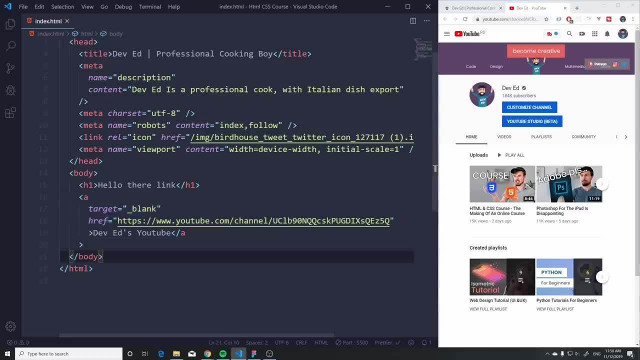 you something. We can also combine the anchor tag with a link. You might not necessarily want to have text in here, You might want an image or a logo, So take a look. Let me show you something very cool. We can go to icon. 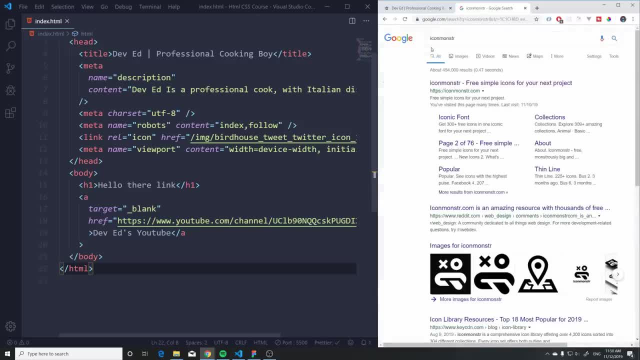 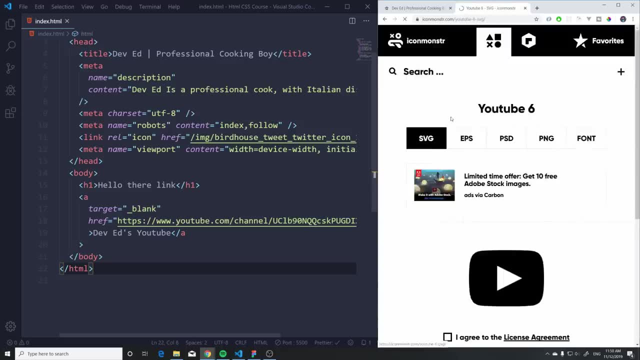 monster And this is a website where you can get a ton of super awesome icons, And I'm going to search for YouTube here. So let's search YouTube And let's just get this one. This is fine. I'm going to hit OK and download And I'm just going to open up the file. 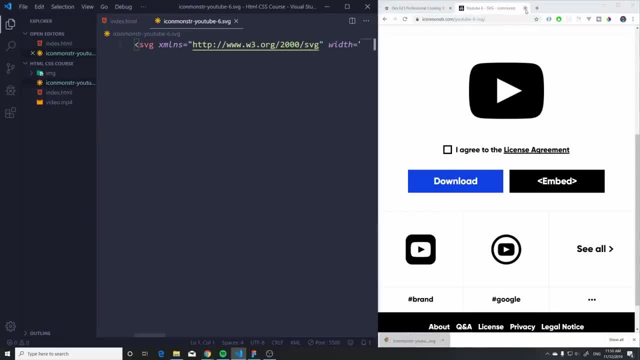 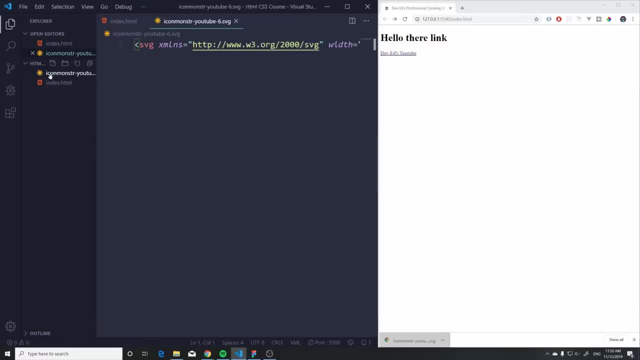 directory here and drag it inside here for now. Okay, perfect, Let's close this up. I'm also going to get rid of the same before. we don't need this anymore. And you know what? let's get also rid of the images folder here. So now take a. 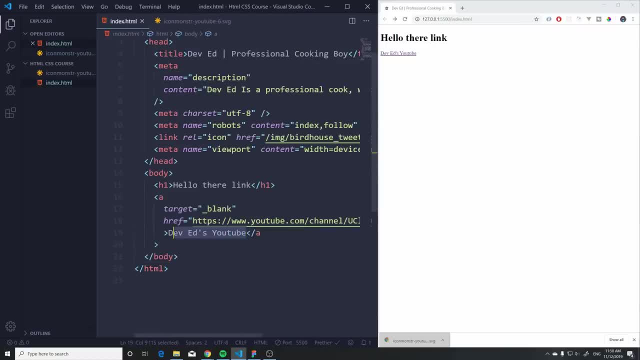 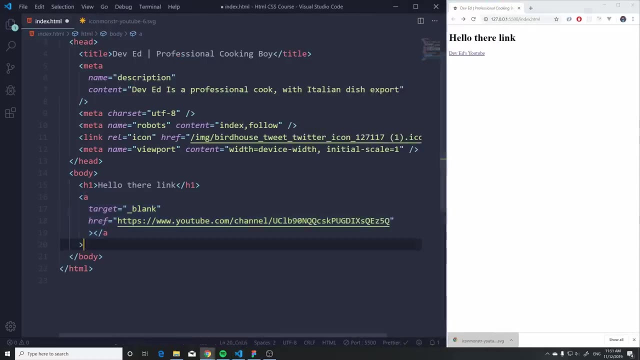 look, I can just go here and I'm not going to add the text anymore. I'm going to take everything out here And I'm just going to drop in an image, So you can actually nest an image inside this anchor tag. Let me make more space here so it's a bit more visible. Okay, so let's. 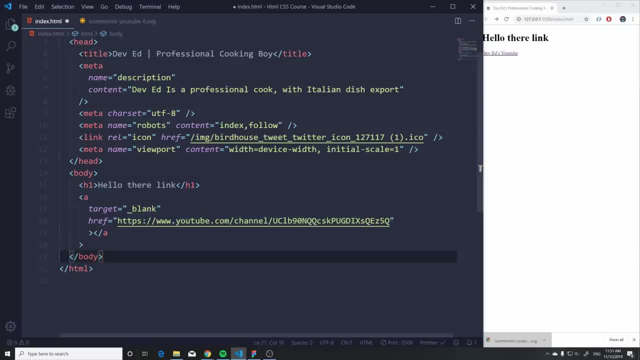 make even more space. This link tag is a bit too long, So it's a bit might be a bit difficult to to see what's going on, But I'm just basically adding the image between the anchor text, So the in between the, the opening and the closing one, where we add the. 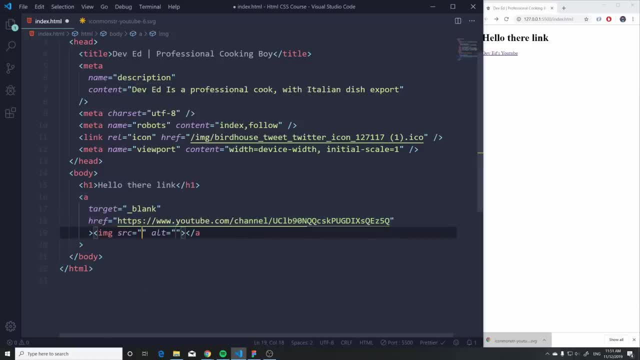 text. So in here I'm just going to write image and hit tab And that's going to give me a source. here Again, I'm going to talk a bit about the old later, So let's get rid of that, But in here I can. 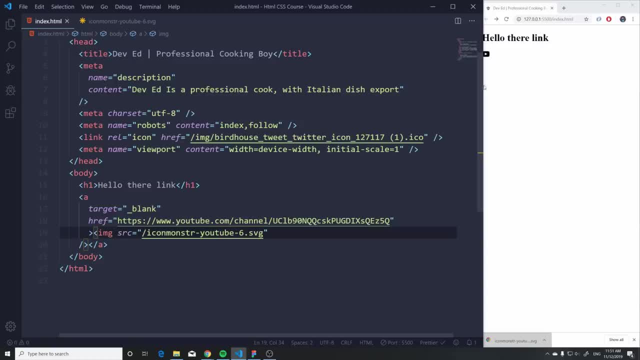 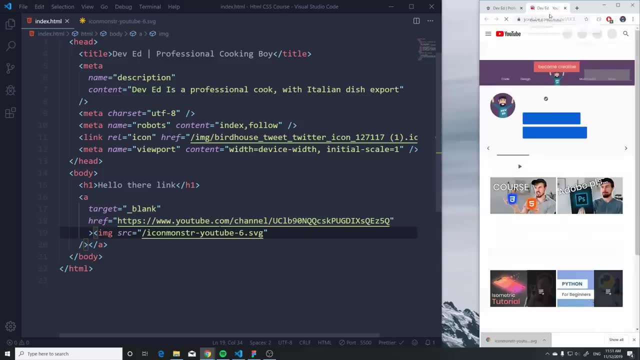 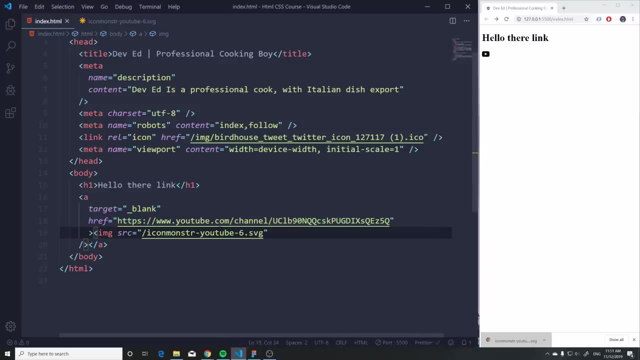 just add a slash and link to that icon monster And, as you can see, we have the button now as a logo. So when we click on this it still works the same way. But you can also have images, PNGs, JPEGs, whatever you want here to show up as a link. So there we go. Next up, let's 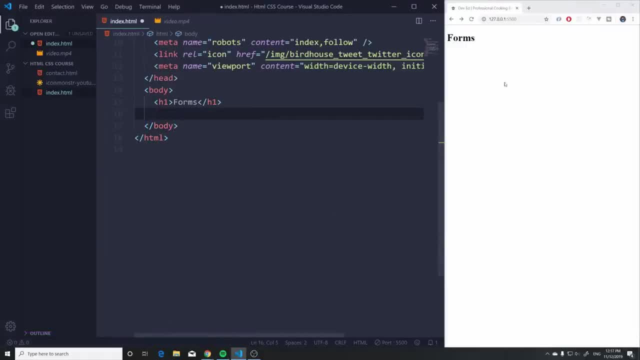 cover the forums, And we will actually be using one form on our first project where we're going to submit some user data and we're going to receive an email, So forms that are typically used again to collect some user data. So you probably know this, but whenever you sign up on a 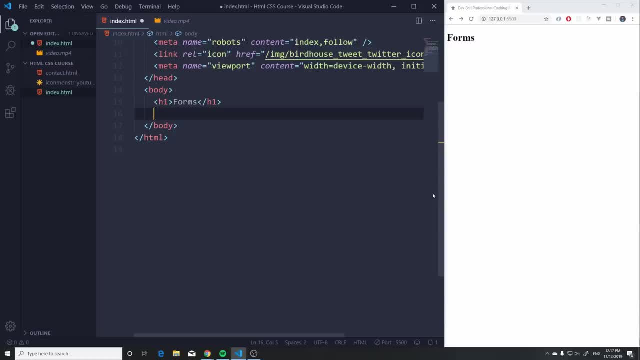 website. there's a form there. you enter your email, you enter your, your password, your username, and then they receive that information and they're going to create an account for you. Same thing goes with contact. When you hit submit, they're. 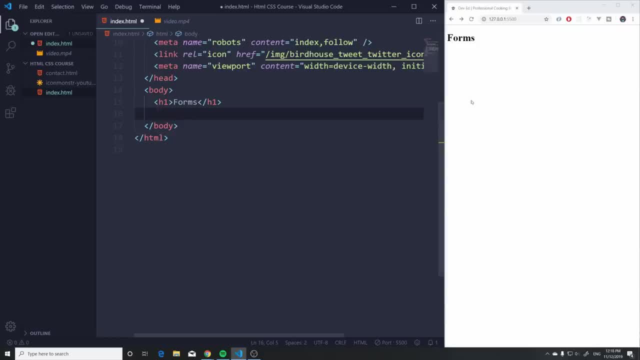 going to receive an email. So basically, all it does, it collects some user data and it gets sent somewhere, Depends where, Who knows. There's a lot of options you can do with forms. So how can we create a form? Well, we just use the form tag. So I'm going to say form and hit tab. 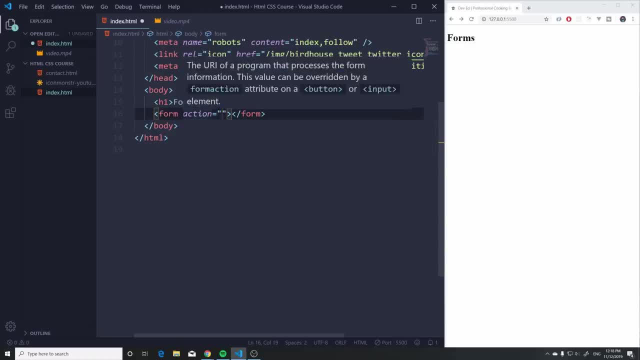 And, as you can see, it automatically gives me one attribute, which is called action. We're not going to be using this for now, because all this action does is it submits the form somewhere. So after we submit the form, this action gets executed, But for right now let's remove it. we're going to add it a bit later And in this form we can. 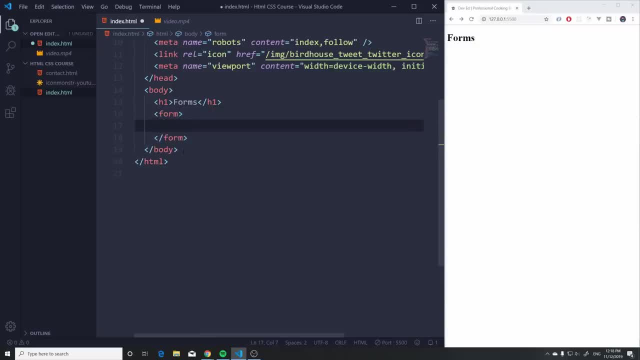 add a bunch of different kinds of inputs. So the first one- that's going to be probably the most common one- is going to be called input type text. So if I just type input and hit tab, obviously it's going to give me the most default one And this one's called text. So if I hit save, I 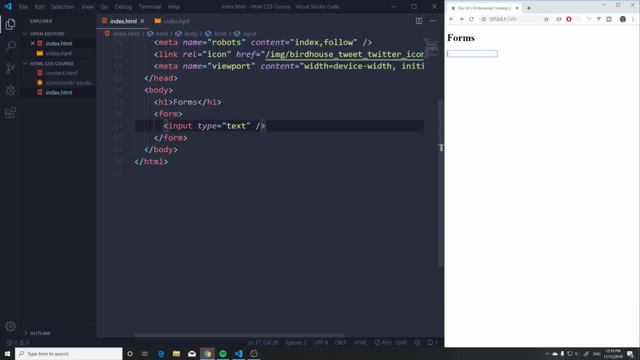 can type just normal text in here, All right. So now it's very hard to see what this does because it's unclear. it doesn't have, like a, a title or maybe something, a label to it, So we can actually add a label to it. So if I go up here, I can type label And I'm going to hit tab And, as you can see, it gives me four All. 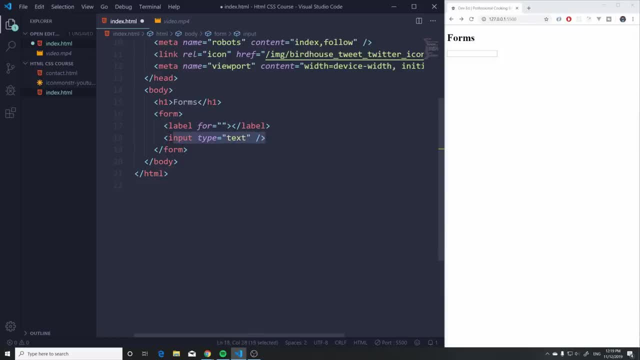 right. So for what? Well, I need it for this input. I need to describe where this label belongs to, And it's to this input. So, to give an identifier to this, you just add an ID and I can set an ID. as you can see, it's a unique identifier And it's also. 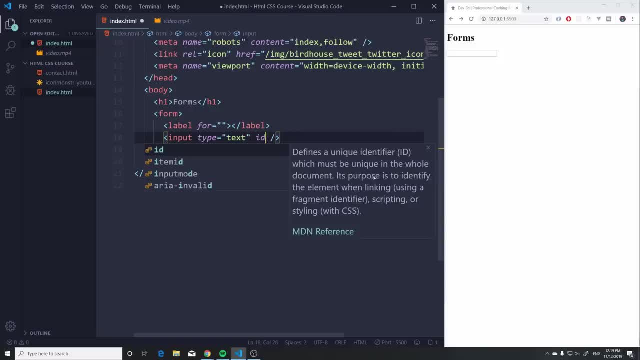 heavily used to to basically to modify in CSS or to identify it in JavaScript. if you want, you can use there as well. So if I give an ID here, we can access this input basically through our CSS and JavaScript, And then here I'm just going to give it an. 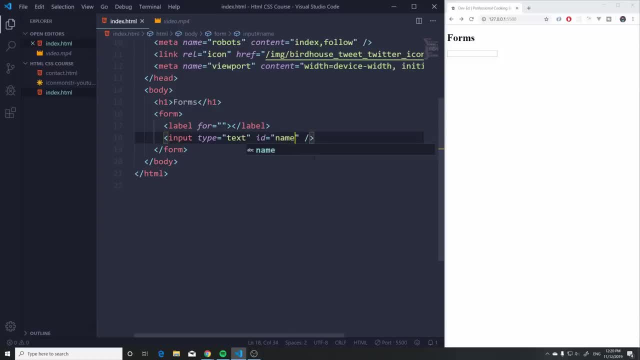 id of name, all right. or user, let's call it user. i want to have the user so i can say the label is for user and i can add a descriptive text that you see on on, like every website is in this label. here i can say username and this doesn't have to match the text that we add here, can be anything. 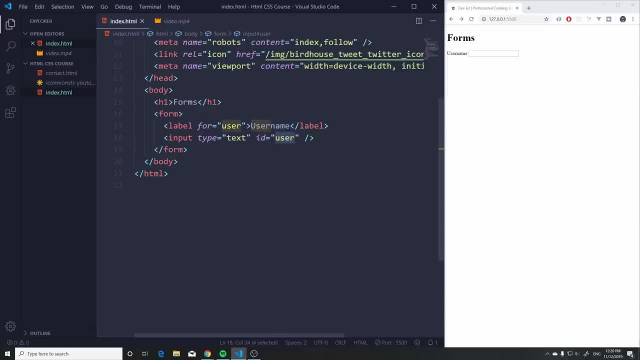 that we want. but as you can see, here i kind of keep it simplified and easy. but here i can use the full name. i can do username here as well, but i like to keep it very simple. everything lowercase just user. okay. so as you can see, now we have username and we have our label and our input. 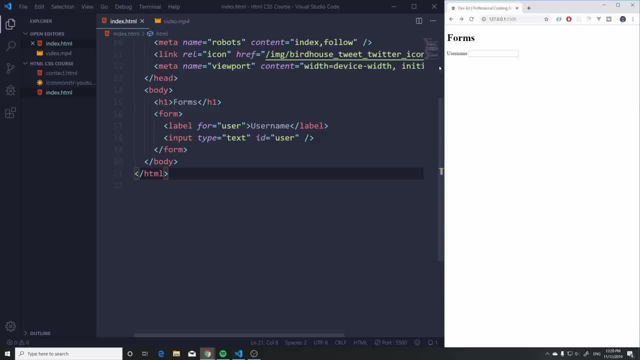 so super cool. now, besides this, uh, the label. it's very useful because let me show you something: if i add another input here, i'm actually going to change this to type email. right now, check this out if i add another label here- and i'm not going to name this in any way, i'm just going to say email. all right, well, 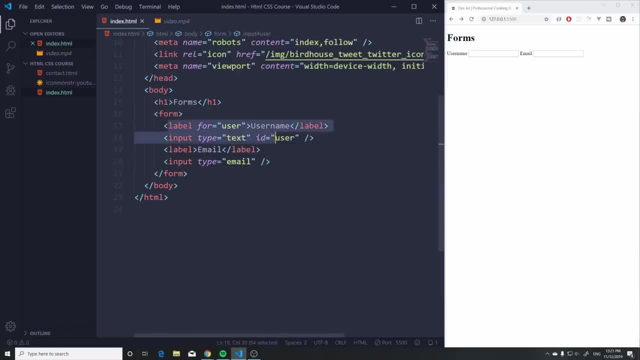 what's the difference between this and this? like these two and these two like what? what does it actually help me with by adding for user here and binding it to this input? what's the difference? well, check this out. if i'm gonna click on email here, on this label, it doesn't really do anything. 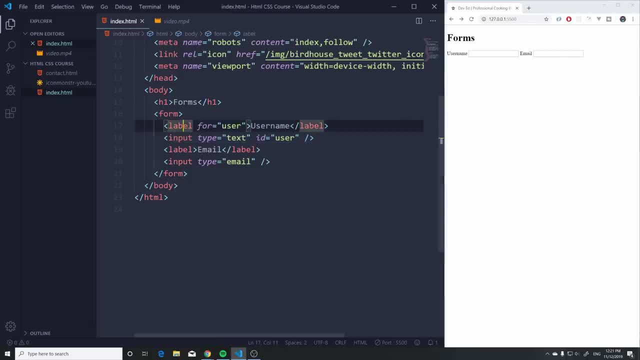 i have to click in the input here. however, if you specify on the label that, hey, this is specifically for this id of user, this, well, if i click on the label now, it automatically jumps me in to the input tab here. so boom, as you can see it just, it activates the input so i can start writing. so this makes it a bit more. 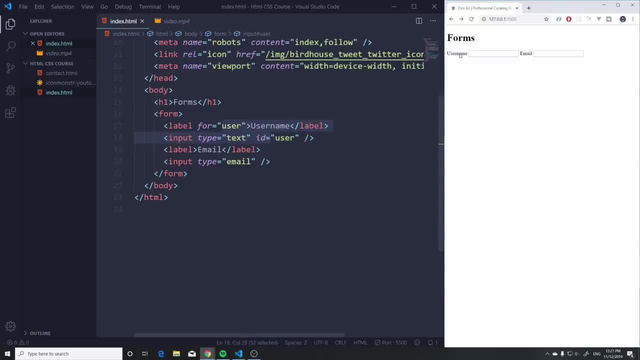 accessible and a bit more easy for the users to to write the inputs. so, lastly, what i want to show you, and i also want to show you the difference between text and email here is at the end, if i just add a simple button here and i'm going to say submit. 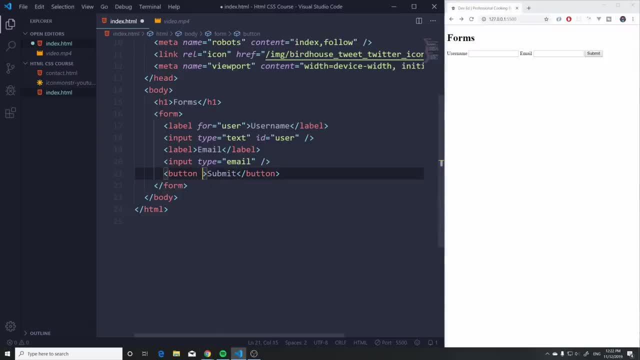 like this and take a look, i can add a attribute of type submit, and all this is going to do is it's going to submit all the information that we have in the form. so if i hit save and i'm going to just type something and i'm going to add an email, all right, just the random old email that i have, i'm. 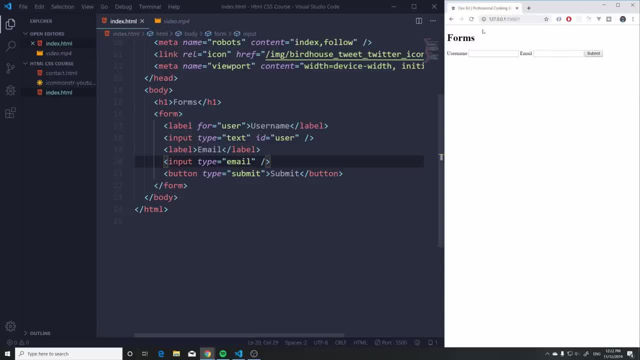 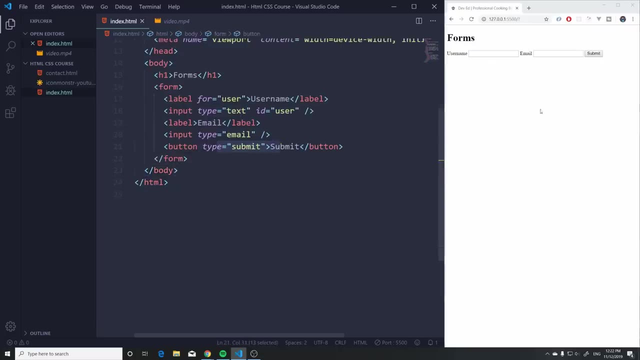 going to hit submit, boom, the form gets submitted. now it doesn't get submitted anywhere. unfortunately, we don't have an action here, but it works then. that's all that matters. so here's the difference between the type text and type email. i can add any text i want here. however, here, if i don't add, 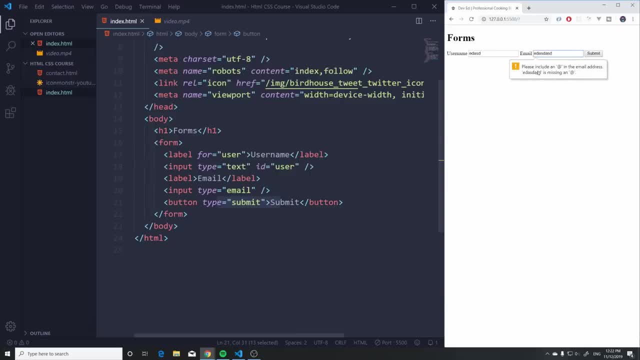 an email. as you can see, we get an error here saying please include an ad for in the email address, so it doesn't actually submit the form. so html actually does some validation for us if we specifically specify that, hey, this is an email. okay, we only want to have an email. so the form doesn't get submitted. 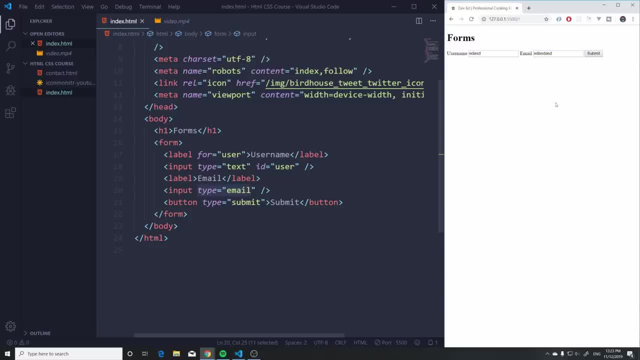 anymore until this is actually an email, so that's super awesome. now let's go up here to the form and i'm actually going to add an action. okay, and i want to show you that we can also use action to navigate to another page. i made a contacthtml here. it's super simple. there's nothing really in it. 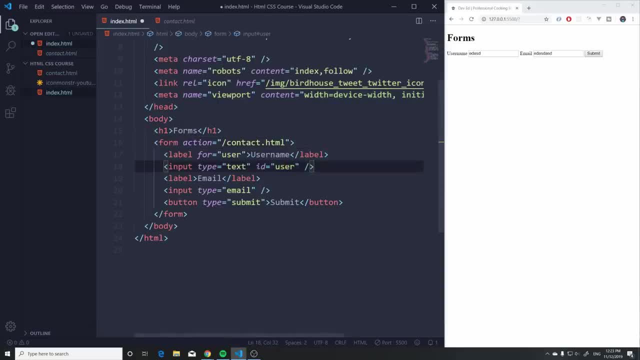 and i can add a slash contacthtml. hit save and now take a look. whenever i submit something, it's going to jump me over to that page. so you can also do that if you want. and this, by the way, also works with an anchor tag. so if i add an anchor tag here and i'm going to say, link me. 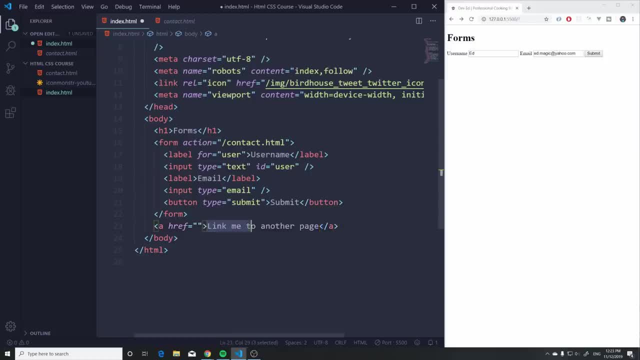 to another page. we saw that we could have used this with links, but we can also navigate to another html page, so i'm going to say contacthtml and i'm also going to add a target of blank. so hit save and take a look. even this link tag can also navigate to another html, so i thought i'd show you that as well. however, the way 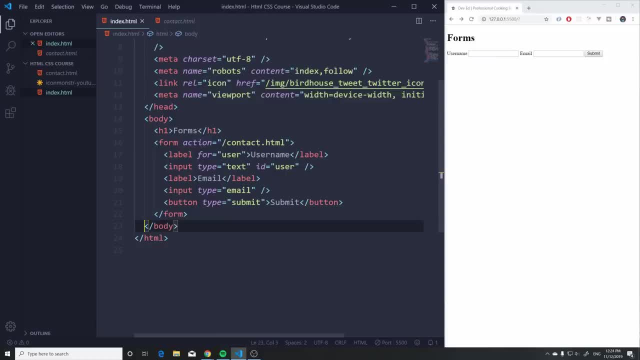 we will be using. action here is: we are actually going to use a third party website and we're going to submit the information there for them, or, later on, when you're going to work with javascript and nodejs, another programming language, you're going to submit this one to a specific URL. So you get. 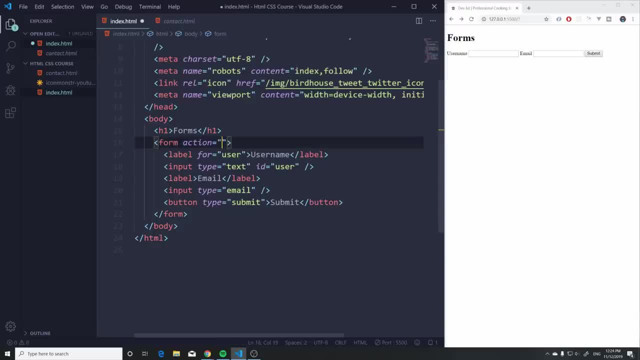 that in your backend server or somewhere else. So for now, this is kind of useless for us. So we covered this, we covered the labels, we covered the inputs and we covered the ID, which is again just used specifically So we can access this specific input in our CSS or. 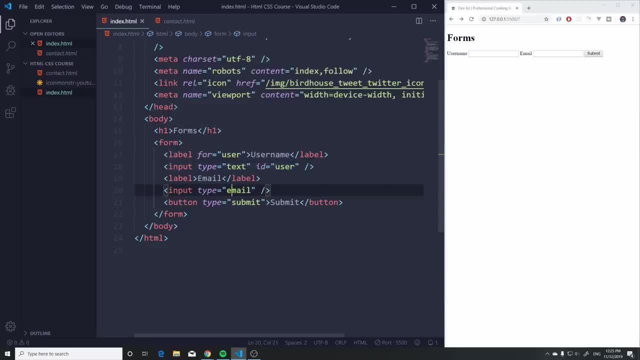 JavaScript. Okay, And lastly, what I want to show you is something called name. So on the input here we can also add a name called user. So I'm going to use the same as the ID here And for the input. 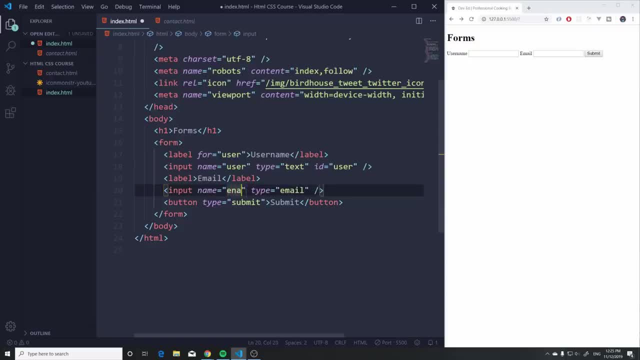 type email. I'm also going to give a name of email And the reason I am doing this. although I'm not going to use the ID here, I'm going to use the ID here And for the ID here. I'm going to use the ID here And for the ID here. I'm going to use the ID here And for the ID here. 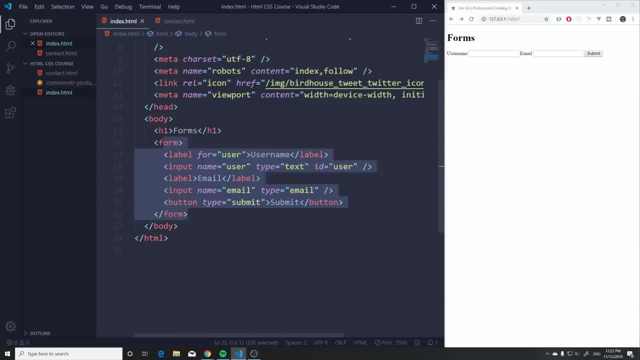 the only fields that get submitted in this form are the ones that have a name on it. So make sure you put a name of all the inputs that you want to submit in the form And just to kind of quickly show you what gets submitted. If I type here, add and just provide a random email, And if I 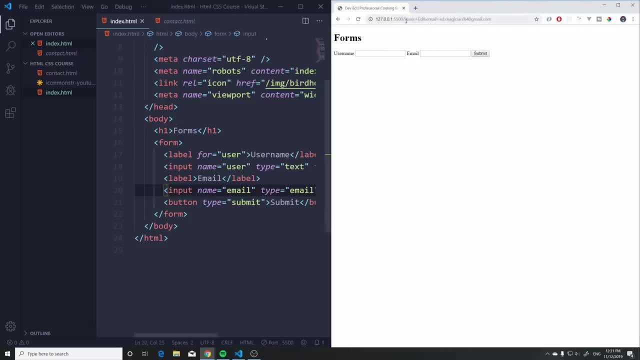 hit submit. you're going to see up here in the URL. we're going to get user equals add And this is going to give it. And then we have email. So the name email equals add magician at gmailcom. Okay, next up, I want to take a look at a drop down where you can select multiple different values. 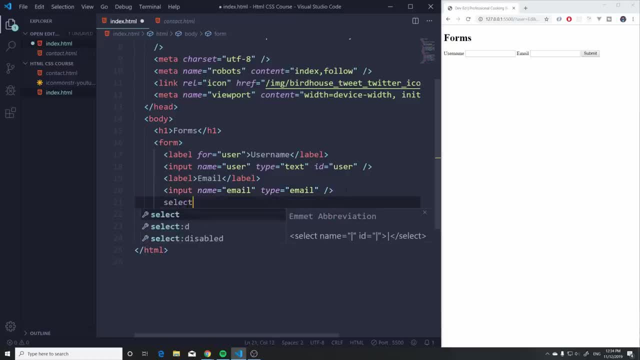 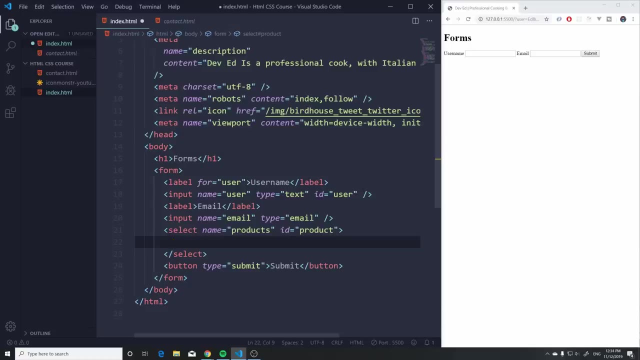 To create a drop down. all you have to do is say select and hit tab, And now this also gives you a name and an ID. I'm just going to call this products, All right, and I'm going to give it an ID of product. So if we ever want to select this in our CSS or JavaScript, we also have 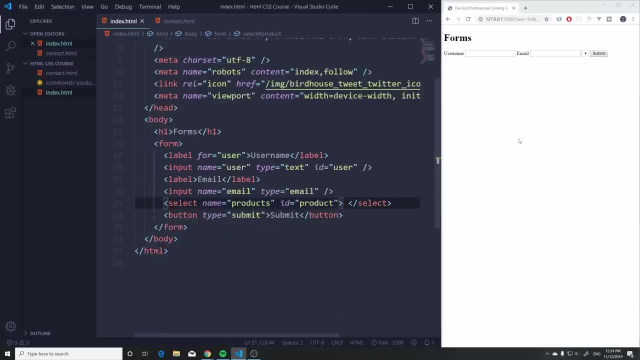 a name and an ID. So we're going to hit select And now this also gives you a name and an ID, A unique identifier, And in here, if we save this, we just have the simple drop down here, but it doesn't really do anything. So, to add options, well, we just write option. That's a. 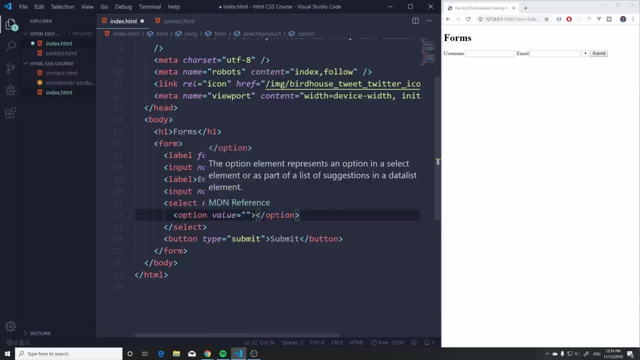 HTML element that we can use, And in here I can give a name to my product. Maybe I have a MacBook, All right, So there we go. We have a MacBook, I can duplicate this, bring this down and call this an iPhone or something. Hit save. And now we have two. So there we go. And what this value? 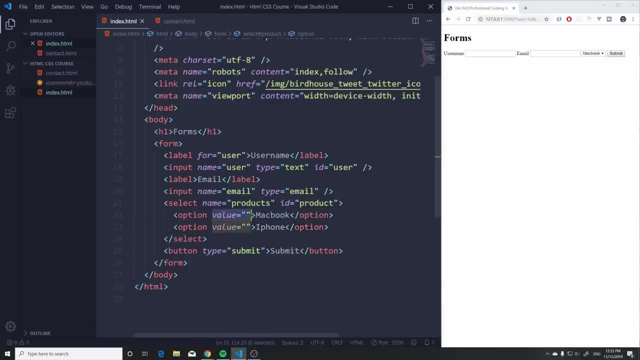 does is this is actually the thing that gets submitted in the form, right? This is kind of the text that we want to give it. This can just be whatever we want, But when we hit submit, the thing that's in the value is going to be submitted in the form. So I can see MacBook. 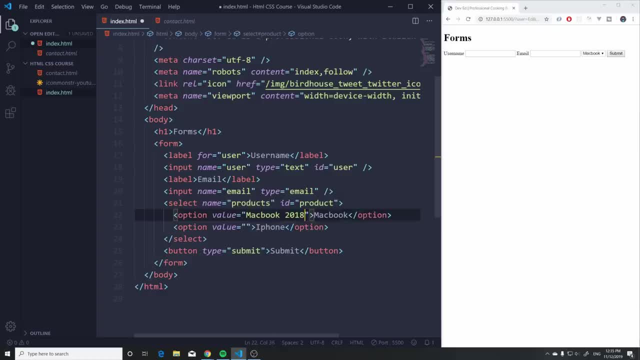 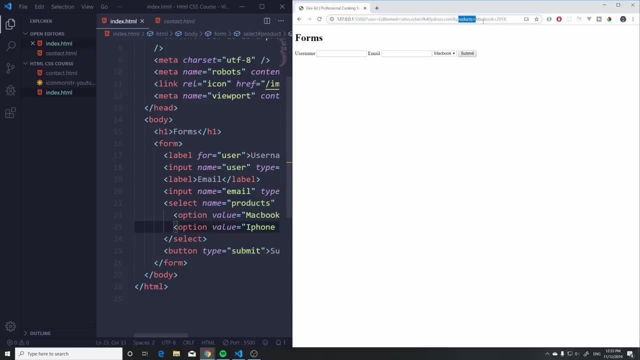 2018 like this for the value. And I can say iPhone 11 like this. So when we actually add our information here, I select MacBook, Hit submit. If we expand this, you're going to see that product is going to be equal to MacBook. 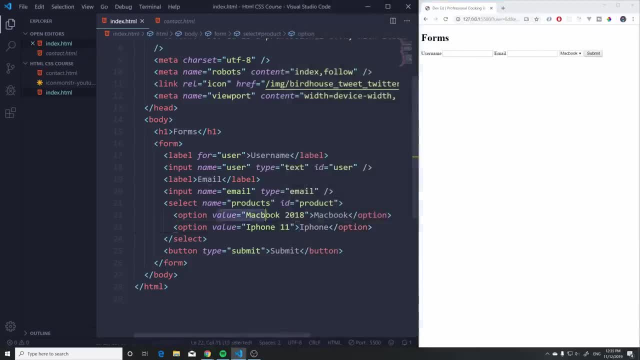 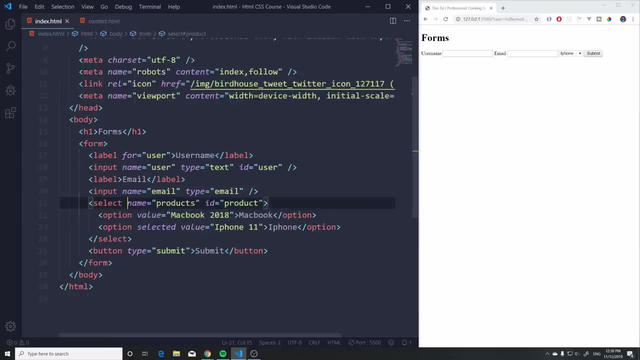 2018.. So the actual value that's in here is the thing that's going to be sent to, wherever we are sending it to. Okay, But what if we want to submit a message? Having the small input is not that great, because if we write a lot, we cannot really see anything else that we previously wrote. 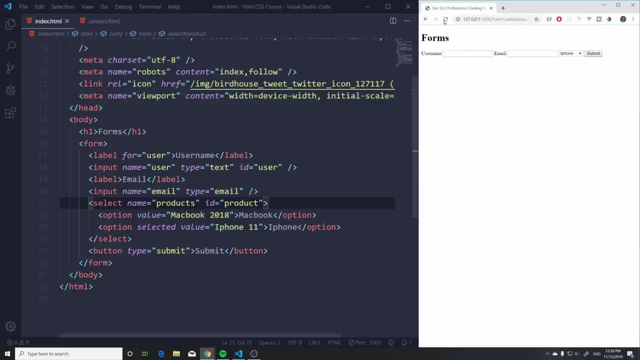 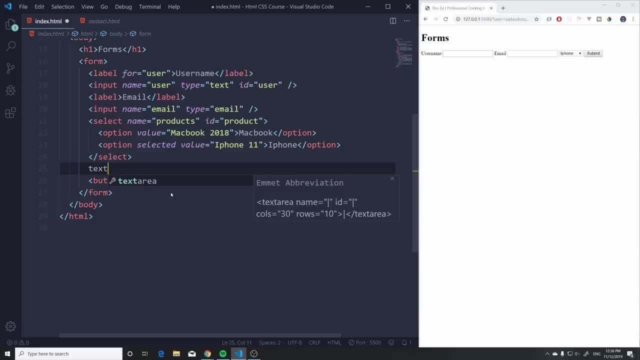 Right And I cannot add a new line. If I hit enter then the form is getting submitted. So how can we get around that? Well, we have another element called a text area, So I'm going to just say text And, as you can see, 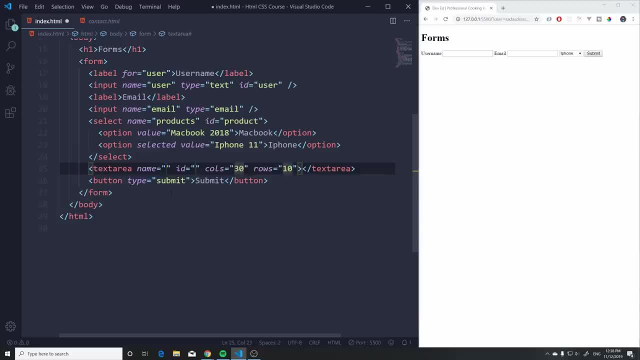 it appears there, I'm going to hit enter And, oh my goodness, what's going on here? Well, we know name, So I'm going to give it a message. I'm going to give it a message ID as well, But we 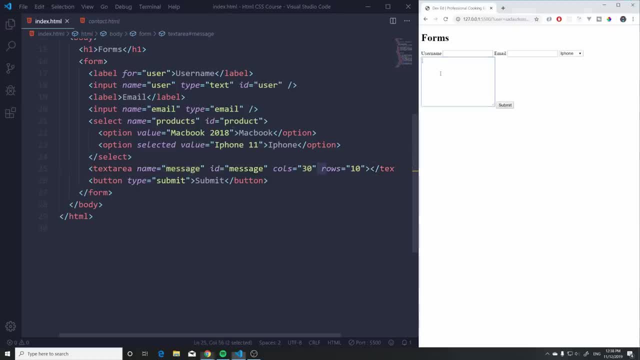 have this calls and rows. So if we hit save, as you can see now we have a multi-line element here. So we're going to hit save And, as you can see now, we have a multi-line element here That we can write a lot of text to, And we can also expand this if we want, like that, Take a. 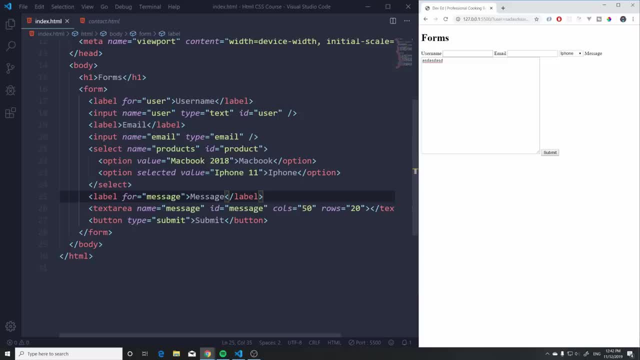 look, That's pretty cool. There are a few attributes that we can add to these inputs, And I want to show you a quick few ones that might be useful. If we go up here to the input tag, we can also limit the number of texts that we can add in here. So let's go here And all I'm going to do is type. 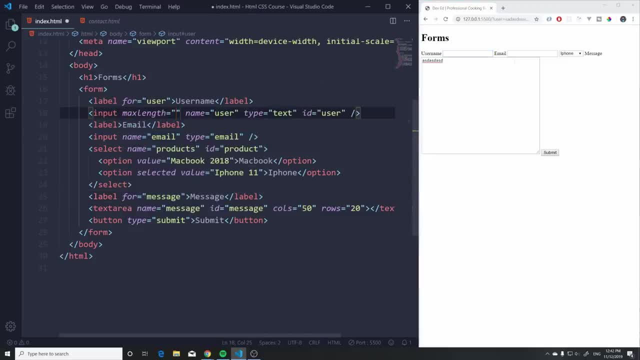 max length like this And I can set a max length equal to- I can say, 12 or 16, maybe I don't want more than 16.. I'm going to do something low like 8 for now, just so I can show you. And now, if I 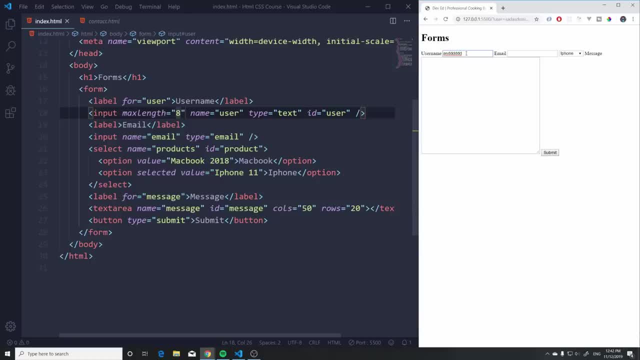 have something superbly long. I cannot type anymore. As you can see, it limits me from typing. So you can do a limit of something like 60 here, just so it's not like super spam, or 30. And we can also do a min length here, So we can say minimum length should be at least six. 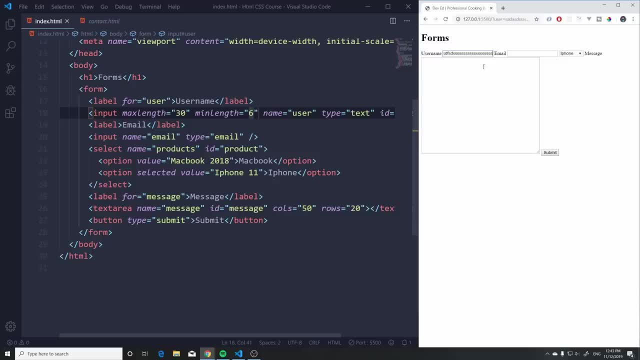 characters. So this is probably a bit more useful for you. So if I add something like one, two, three and hit submit, as you can see, it's going to give me: hey, you need six characters. You're using only four right now. So this is another great check that you can add to your text inputs. if 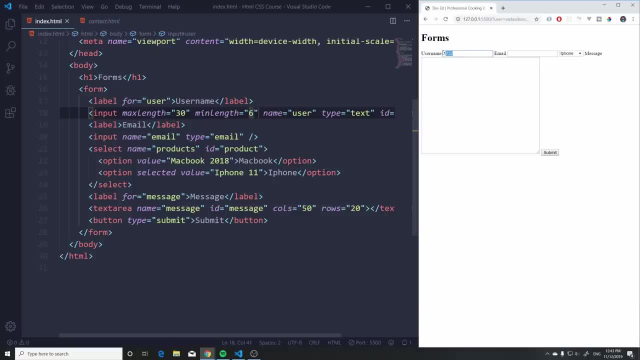 you want to limit it. So we have limited our input here for the username And we also did it for the email. Now if you don't want to have this autocomplete thing, you can also turn this off. I wouldn't recommend turning it off. It's a nice option to have. 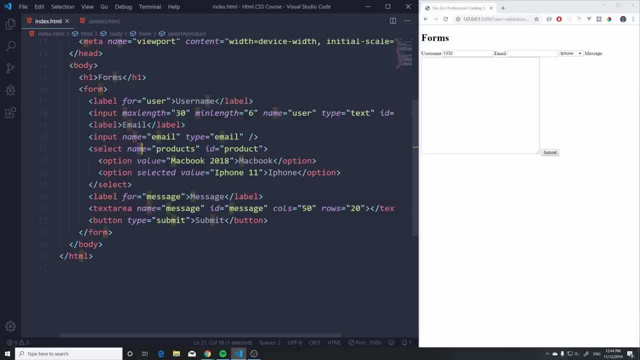 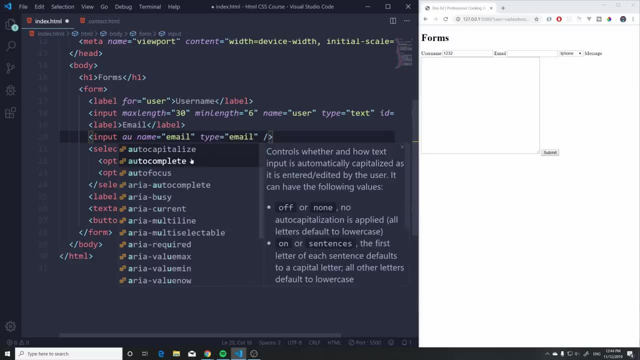 but you can do that as well. So if we go to the let's see, where are you email here And you can say auto autocomplete, As you can see, you can turn that off like this. So when we go here now, 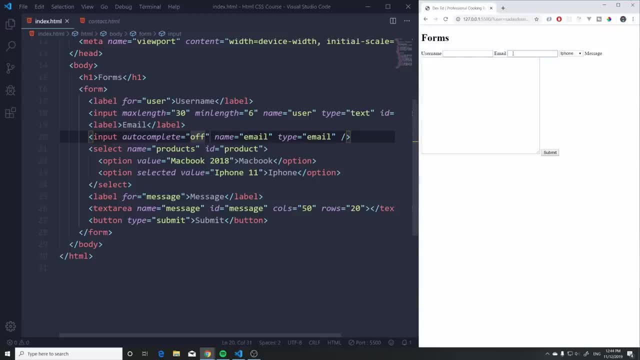 it's going to display that for us. It still displays here, but it doesn't display here anymore. You can also add the autocomplete on top of the form if you want to disable everything. So if you don't want it to appear here or either on the email, you can just go here and say autocomplete. 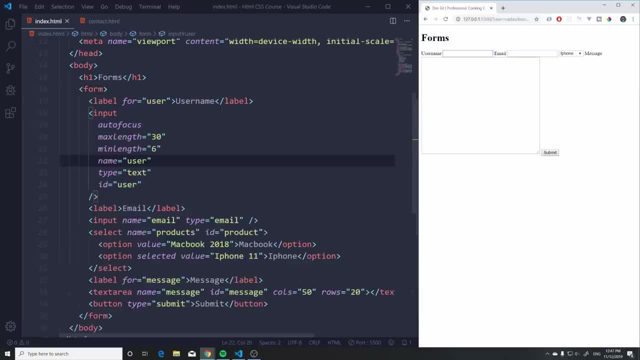 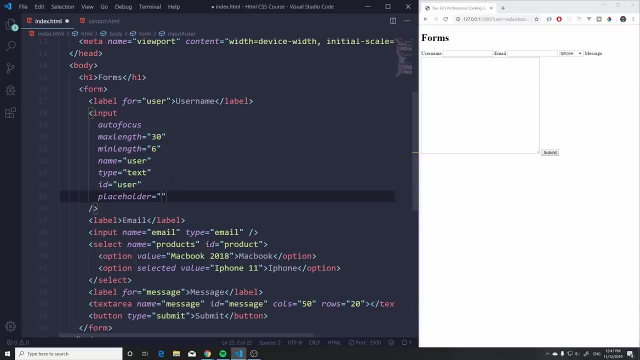 off and it's going to get rid of everything for you. Another one that might be useful is you can also add some placeholder texts in here, in the username, in the email and in the text area. So maybe let's go here, add another attribute of placeholder, and maybe we can add something like: 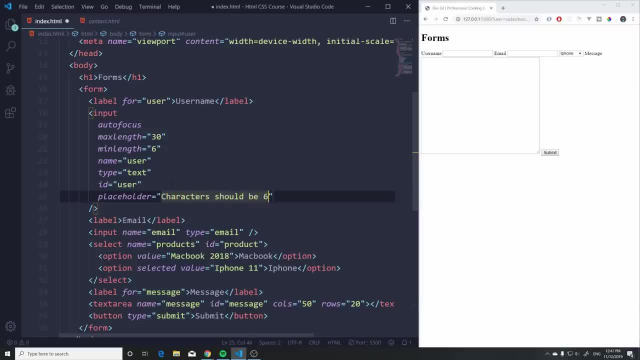 characters should be six minimum or something like that. As you can see, that appears in there as well. Or I've seen some people not use the label and they just use a placeholder. To be honest, I'm not a super big fan of that, but you could say username in here, So when you click. 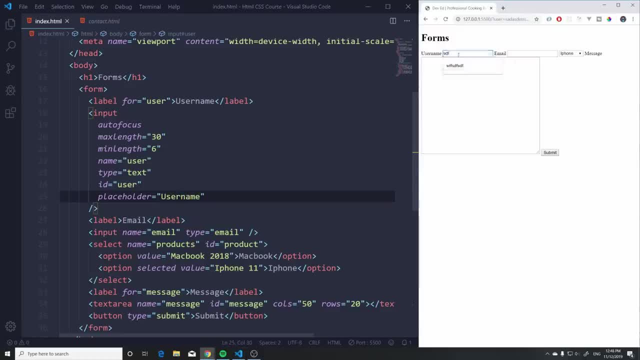 on it and you start typing. as you can see it disappears. So you can see that it's not disappears, So it just stays there until you start typing. Might also have some elements that might not be required. It might be just optional. Maybe we want to have the username and email and 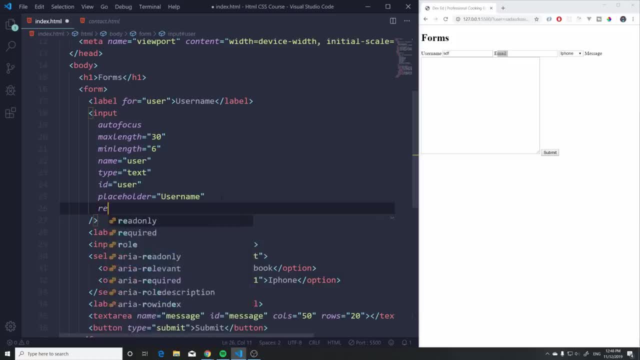 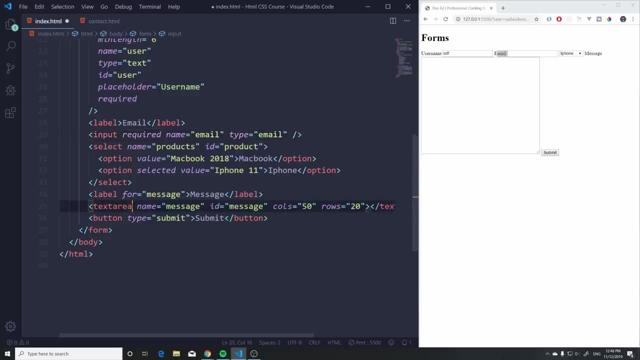 the message. So we can go here and on the username we can add a required. We can also do the same for the email here, and we can also do for the text area. So for this one we might necessarily not even need a value selector. So we can just go here and add a value selector, And we can also. 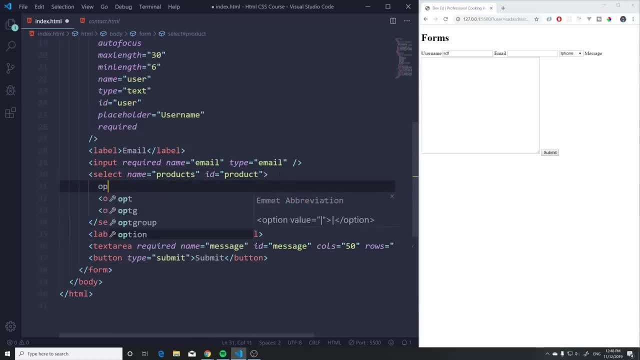 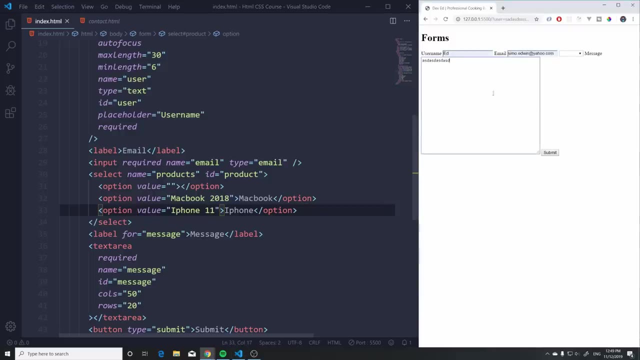 select it. So what I can do is just add another option here and just leave this empty, All right. So no value and just empty, Okay, And then I'm going to move the selected, I'm going to get rid of it. So nothing is selected. So now, if we add some text and an email, let's make this longer. 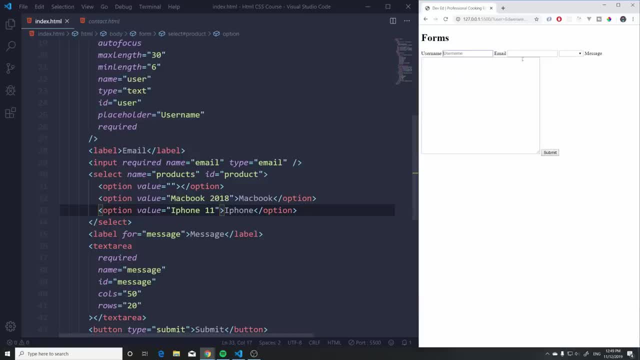 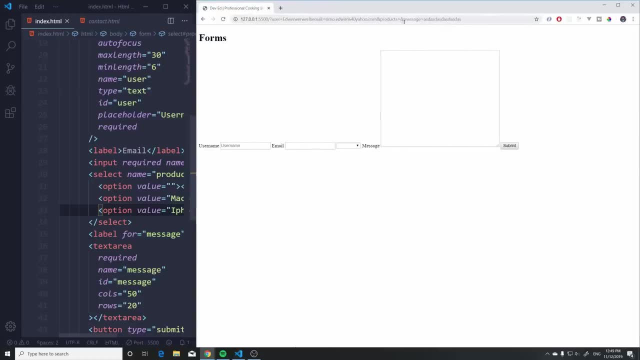 because I think I have that limit on And if I submit, this is going to work just fine. So, as you can see, the value there is going to be submitted with nothing. So let's go ahead and let's take a look. Where is it: Select products. As you can see, it doesn't have anything in the 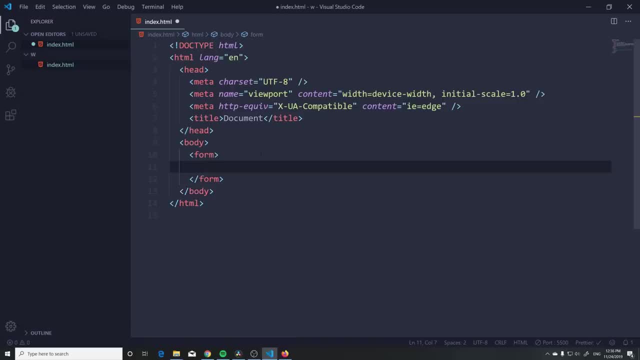 products, It's equal to nothing. Let me show you another quick one that might be useful. This one is called input type radio. So let's type in input type radio And here again we basically can give it a name, whatever name we want, Let's say MacBook, All right, And we can basically copy. 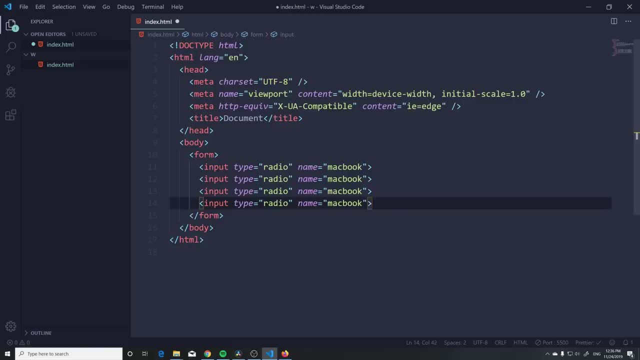 this multiple times, So like four times, Okay, And what we can do is change the value of it. So I'm going to say value And this is going to be the MacBook. All right, Now here's the interesting part. Let me also add a button type. 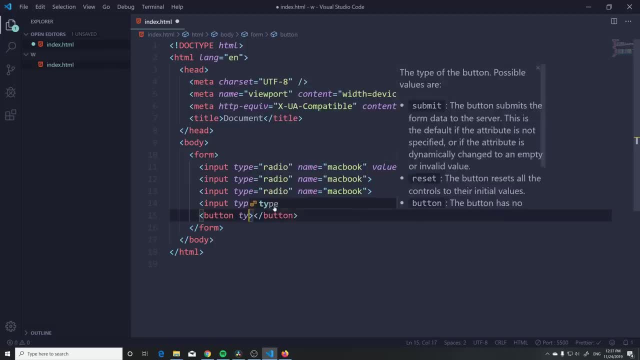 submit, Type, submit. And there we go. We're going to say submit. So here's basically the difference between this and this. This one we want to make general kind of what is this about It's product, All right. So we don't want the actual product name in here, because this is the 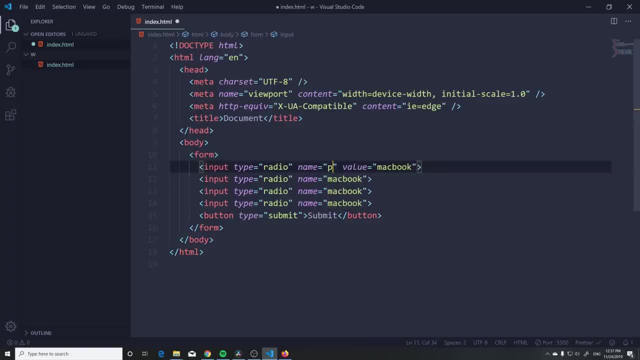 value that's going to be submitted. So here we're going to actually rename this to products like this, Products Okay, And I'm going to copy and paste it here. This is going to be the same value across the whole name, All right, And only the value is going to be different. So I'm going to 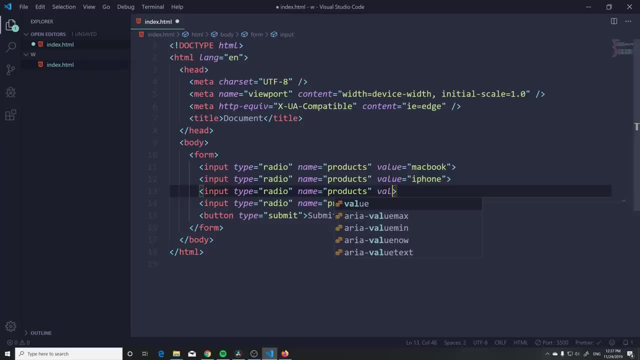 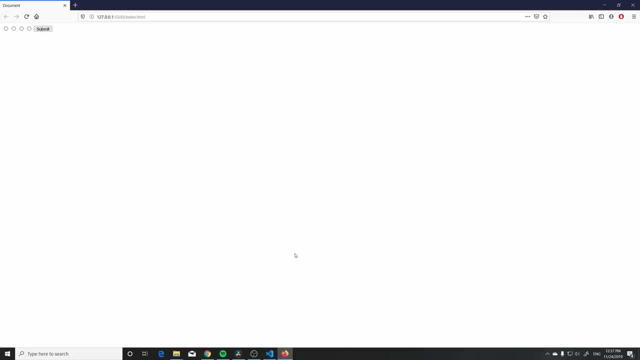 say, value This one's iPhone And let's do another one Value- I don't know- Amazon. We are buying Amazon. everybody Value And this is going to be Cookboy, which is me, So let's hit save, All right. So when we're submitting this, so if I click on one and hit submit as you can. 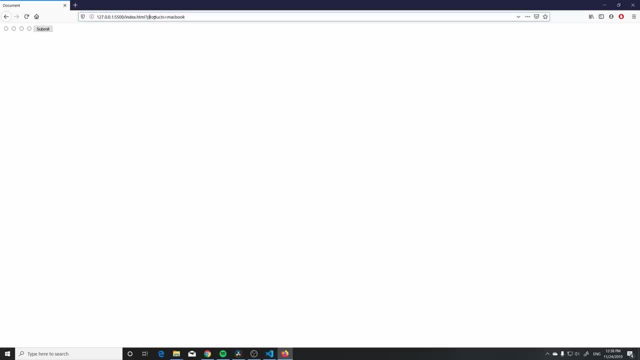 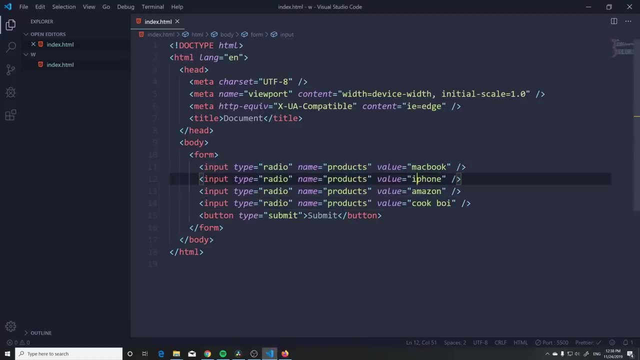 see, the products is going to be equal to MacBook. So this is kind of a general one that we're going to give to the name, We're going to give it to all of them And then this is going to be the actual product or value that's going to be submitted. Okay, Okay, Next up, I want to cover lists. 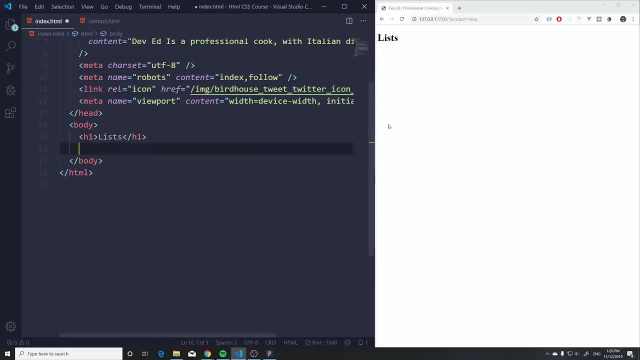 which is going to be a little bit more complicated, So I'm going to go ahead. and fairly simple. So if you want to have a list of some sort, all you have to do is we're going to type in UL and hit tab. All right, And what UL is? there's basically two types of lists. There's: 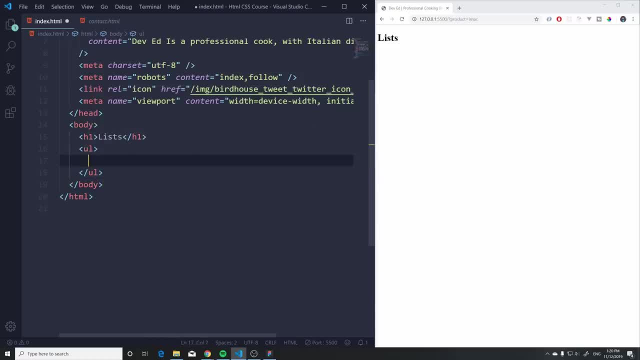 ordered list and unordered list, And you're going to see the difference in a bit. This is the unordered list. So UL and ordered list would be OL. Okay, So UL for unordered and OL for ordered, And inside this UL you basically take. 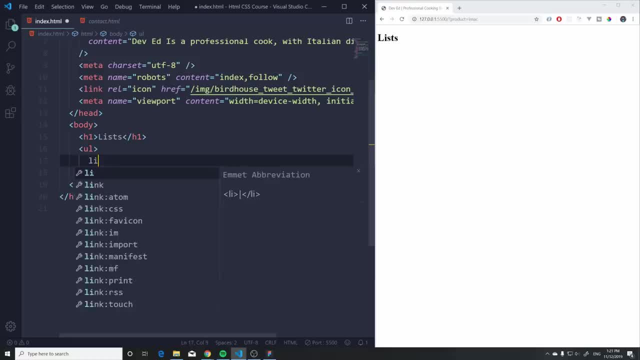 the individual lists that you have. So list is LI And in here we can say let's say whole, And there we go. We have one. I'm going to zoom in for this one so you can see a bit easier And as. 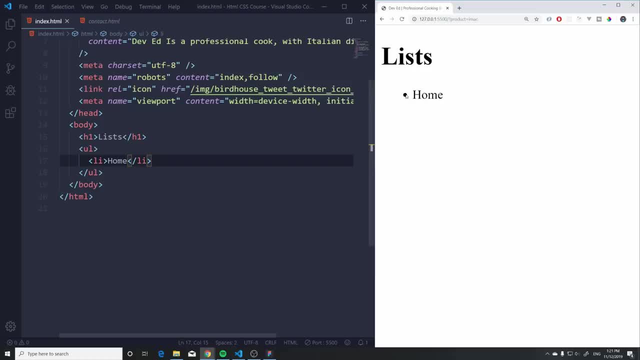 you can see the unordered list. all it has is basically just this simple dot here. So if I add another one, let's say contact, and hit save, And, as you can see, we have that. If I change this to an order type, everything is going to be numbered One, two, three, four, five. Now 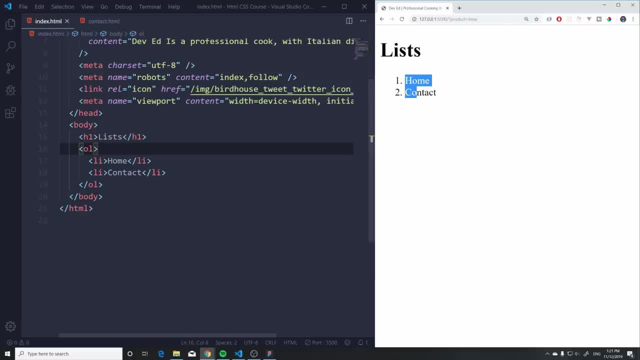 you're going to use lists often like this, But where the most common is where you're going to find lists. the most common is in a navigation bar. I cannot speak anymore, Oh my goodness. And a navigation bar, So home contact. you might have projects, LI projects. This is where you're. 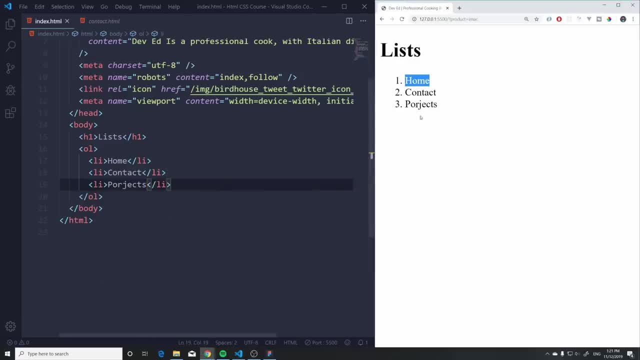 going to see it, most common. Now we're going to do some CSS magic, of course, And we're going to get rid of these numbers, or usually what we do is we just use an li here and then we're going to get rid of of these. now i have an empty one here because i accidentally added a list to another. 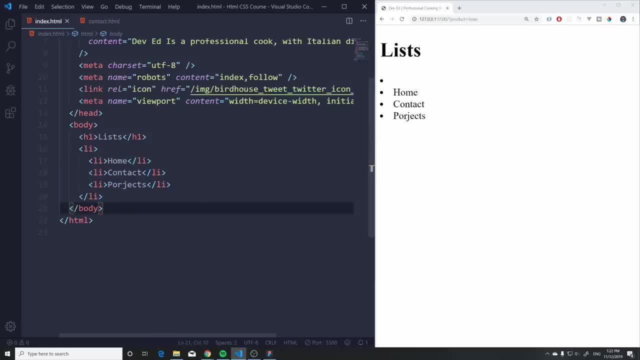 list, and that's something you can have as well. you can have multiple types of lists, so let's change this to ol again like this, so we have one, two and three and you might have a order list inside another order list. this is something that can happen as well. let me copy these and paste. 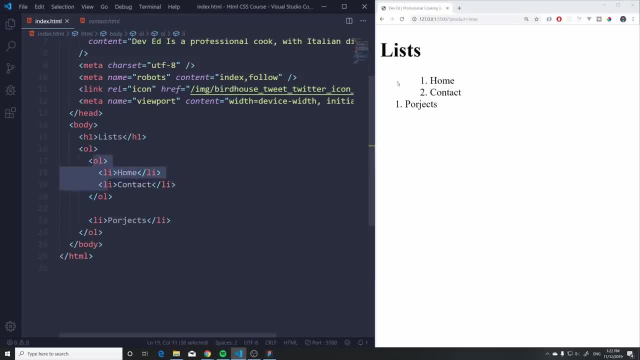 them in here so, as you can see, if you have another list, it's just going to kind of push it to the side. so maybe if you have like a book or something and you want to have like chapters or something, you might have something like this: so chapter one like this chapter one. so that's the first one. 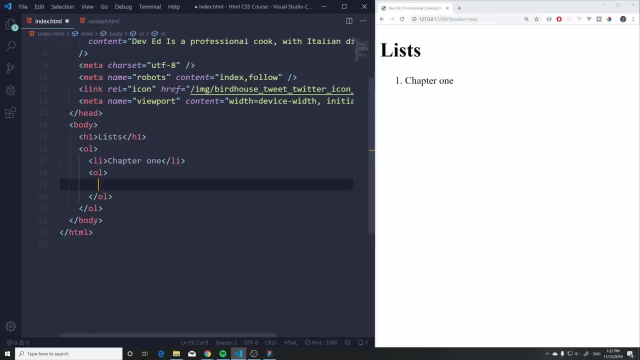 and then underneath we might have an ordered list again, where we have li the homecoming or something, i'm not. i'm not sure. so there we go. take a look, now we have have it like this, and we can have multiple ones under, and then after that we can just go outside. 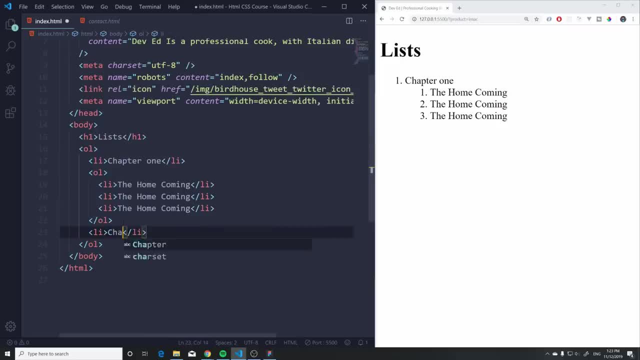 of this ordered list and start again. li chapter two and boom, we can start from here. okay, so we can stack those together as well, if we want. that's it. lists are very simple, as you can see. they're not too hard. what we're going to do eventually is remove these dots in css, and what we're going to 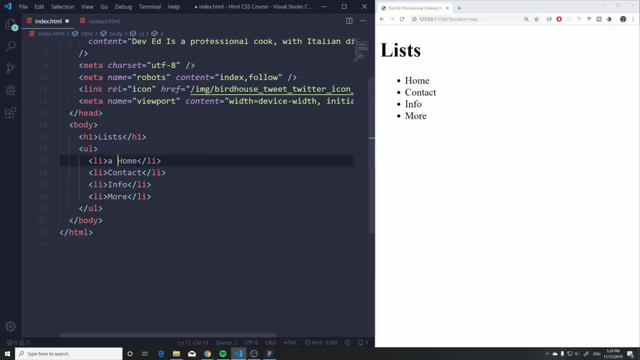 do is we can also add an anchor tag inside here to actually link it to somewhere. so we can say li and inside the li we can add this, and maybe this navigates us to another page, like about dot html. but since this is the index one, we can go to indexhtml like this. and you know what, when you 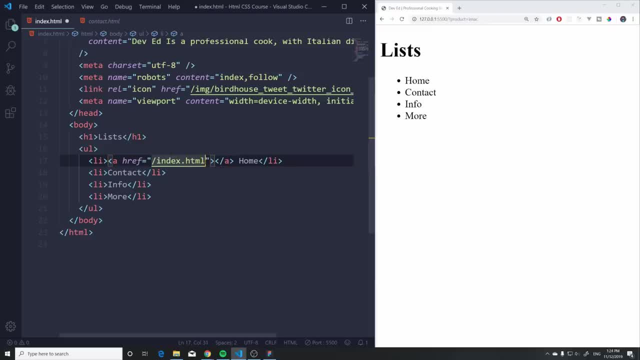 are on the base html. you don't actually need to even link it anywhere. you can just add a simple slash and that's going to recognize it. that, hey, index is the home, and we can also copy the home from here and add it inside the a tag like this: so when we click this, as you can see, it brings it home. now here, if we want to. 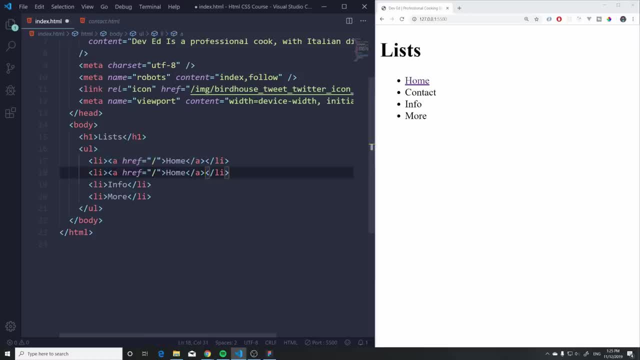 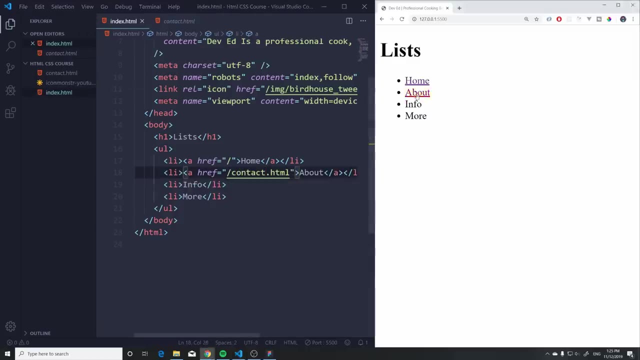 do this. um, let's just paste it in here. this can. this can go to about dot html, and here we can say about: and this is going to work just fine. now it's not going to work because we don't have one. well, we have a contact one. we can change it to that. but let me just show you really quickly, so there, 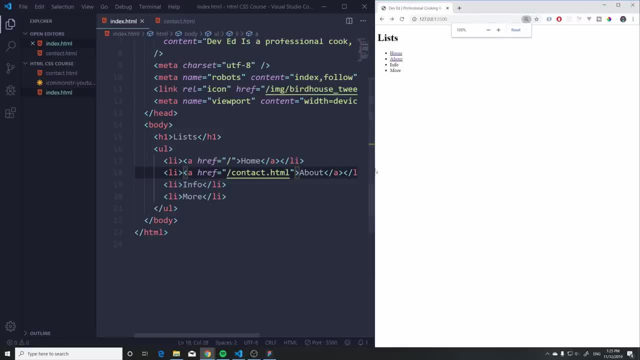 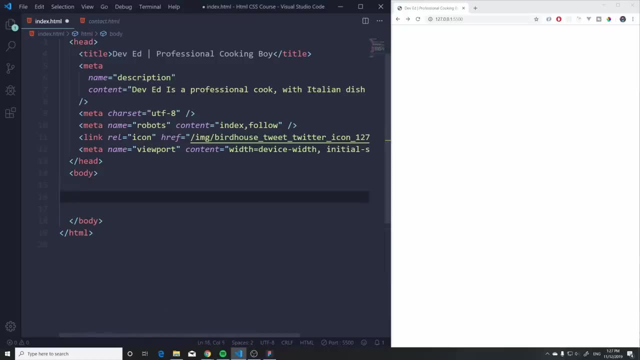 we can go. we can go to another page very easily, okay. okay, let me quickly talk about comments, because this is something fairly important that a lot of people don't use, but it's very important to make your code look nice, and it doesn't actually change your code in any way, but it 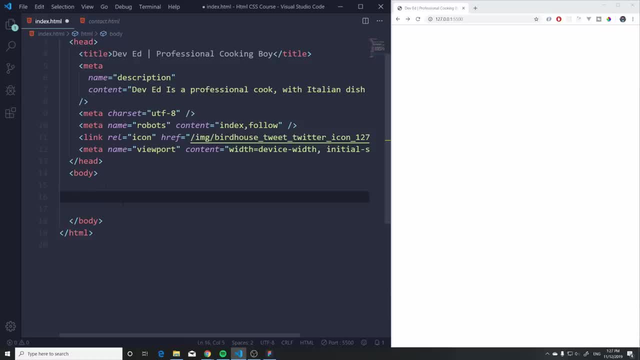 helps you organize everything a bit more. so comments are basically text that you add to your html that does not have any impact to it, so it's just something for you to know and to remember and to let other people know what's going on in your code. so maybe i might have a section like that. 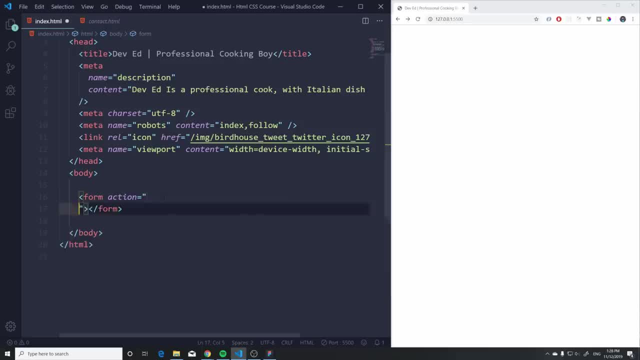 form that we created here and it does something right. so let me just add a just a empty form here, and you might have some things in here, okay, so what you can do is go up here and you can leave a comment on what the functionality of this form down here is. okay, just to make everything clear. 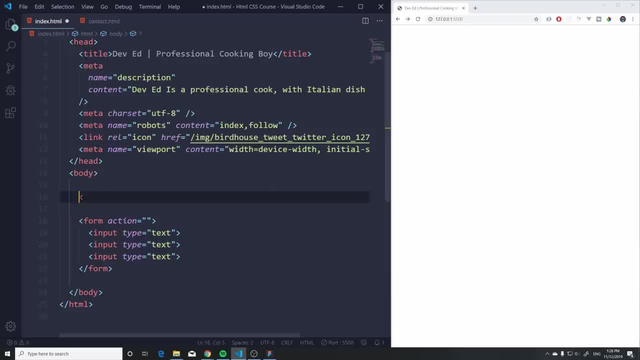 so to create a comment, what you can do is say: you can add this arrow to the left, the arrow to the left- oh my god, that's the smaller than sign- and then the exclamation, and then you do two lines like this. okay, and it auto completes everything for me, but it adds two more lines and a bigger than sign. 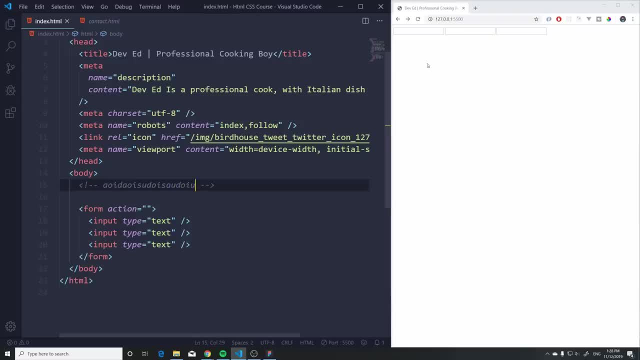 so basically everything that you write here, it doesn't matter, it's not going to show up anywhere. as you can see, we only have these inputs. it doesn't show up, but it helps you kind of know what what you did. so maybe here i can say this is a form for 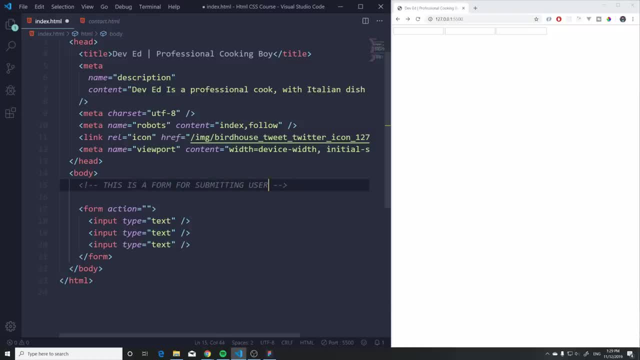 submitting user or submitting a login or something or a register. okay, so now you can have a section like this and then you can go down here, maybe you can add another comment like this, and then maybe you have a section here with some content, maybe some images. this is going to be an image. 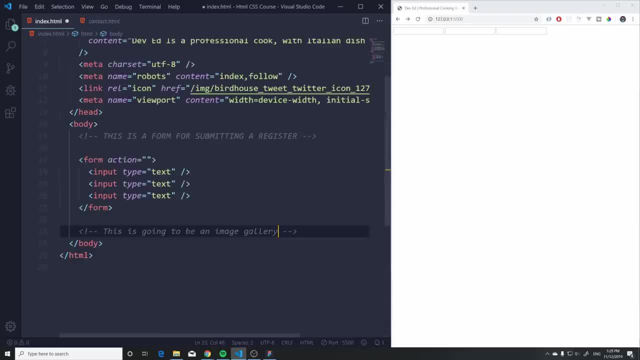 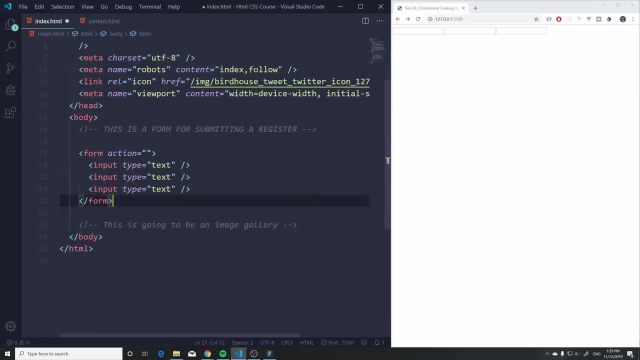 gallery. so when you're navigating through the code, it's going to be very easy to identify these small comments and to know what the code below is doing. so it's very important. i highly recommend you to add as many codes as you want, but also keep these simple, because if you have like a super big stack of code and then you 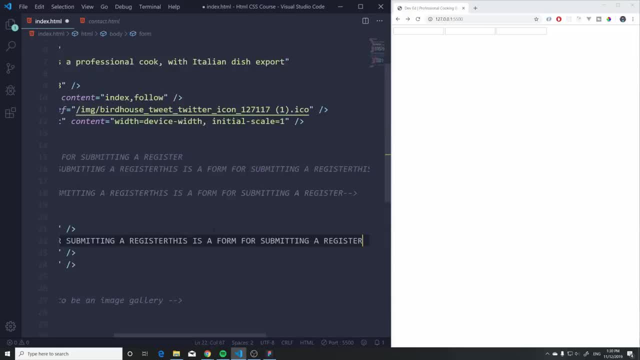 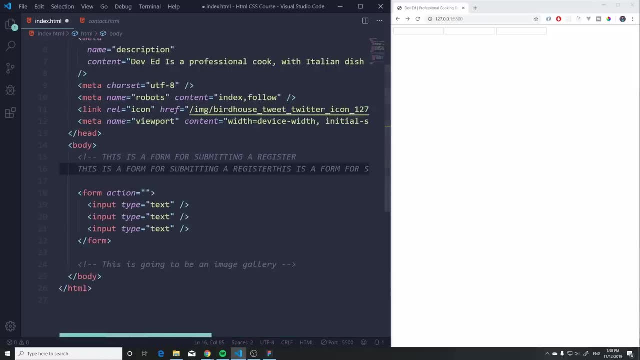 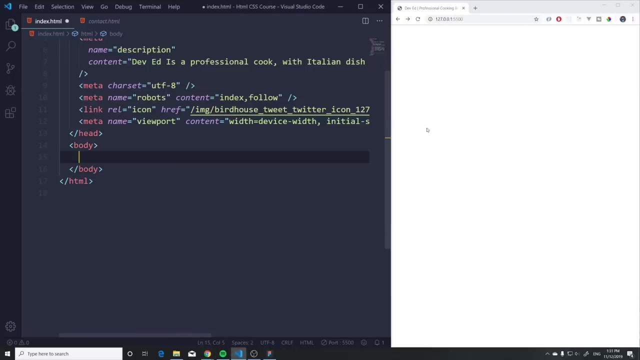 add a lot of code in between the elements as well, like this, then it can get quite messy. so try to keep them as simple as possible and as short and useful as possible. i quickly added a list of things, quickly want to jump and cover tables. I want to say quickly because it's not used as much as you. 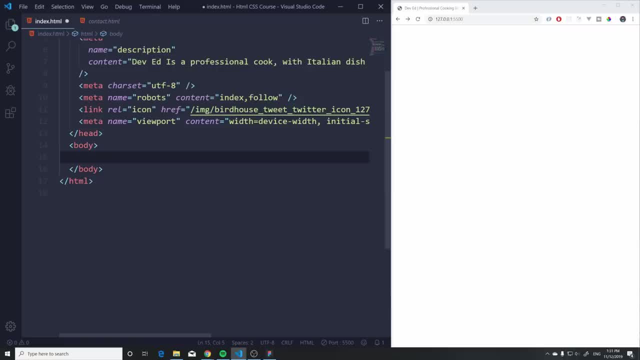 might think anymore. In the early days people would use tables to kind of organize and structure all the elements on the page. So it was used a lot for structuring and to move things in certain positions. But these days you're going to use tables, probably if you really need a table. 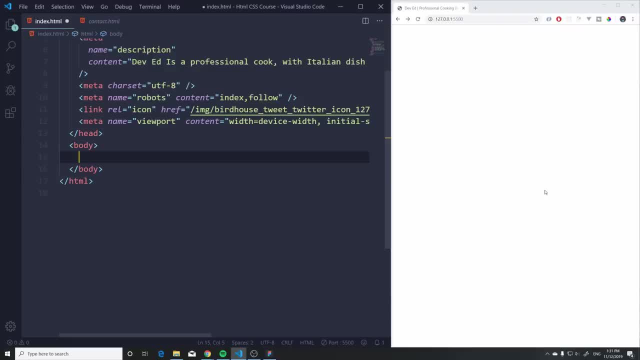 So if you want to show some kind of statistic or something or you want to display some information in a table form, then you can use that. But generally you're not going to find yourself doing this a lot, But let me show you nonetheless- So to create a table, what you can. 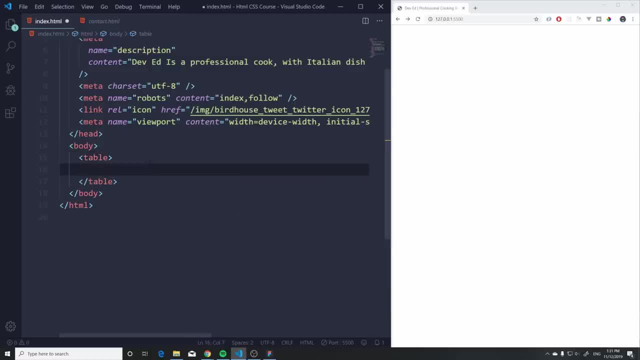 do is say table and hit tab, And inside this table it basically takes two different elements. It takes a tr, which means table row, So the horizontal ones that are going to go this way. So inside this table row, we can add a th like this And let's write something in here: So let's. 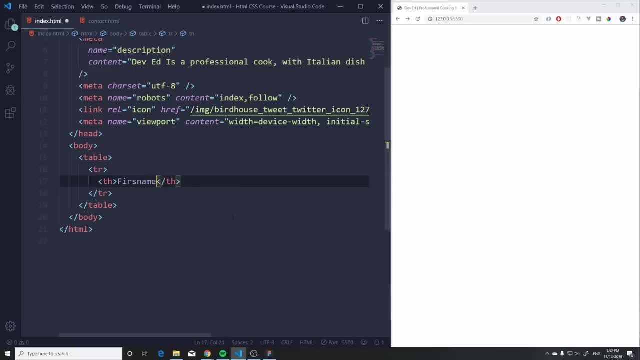 say first name or something. Okay, that's one. Let's duplicate these two more times. Let's write last name And let's write h in here. Okay, there we go. And outside of this table row, what I want to do is add a table. 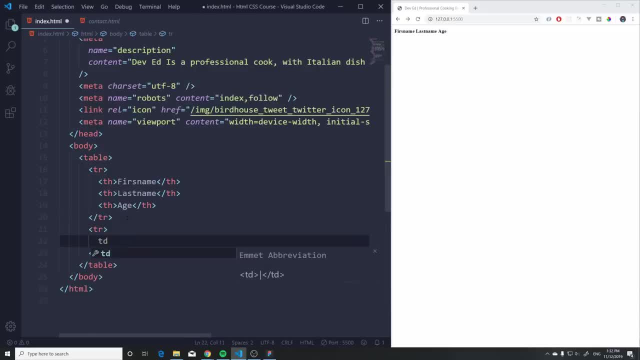 Another table row. And then here I'm going to say td like this: And this is going to be ed, This is going to be u, And finally shout out to my mom: She made the course Yay And hit save, So as. 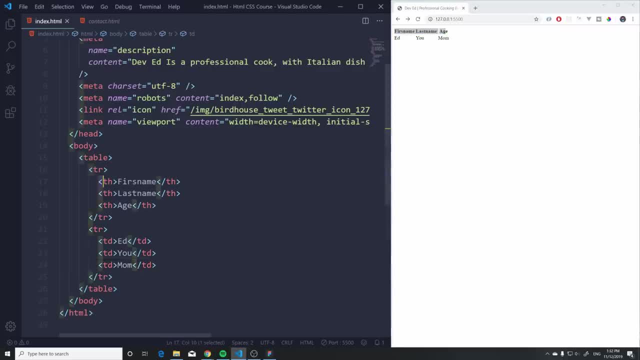 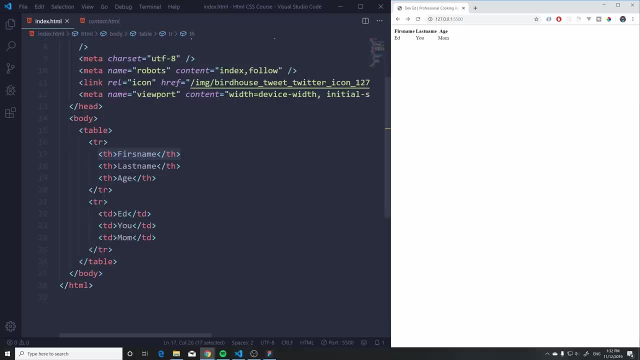 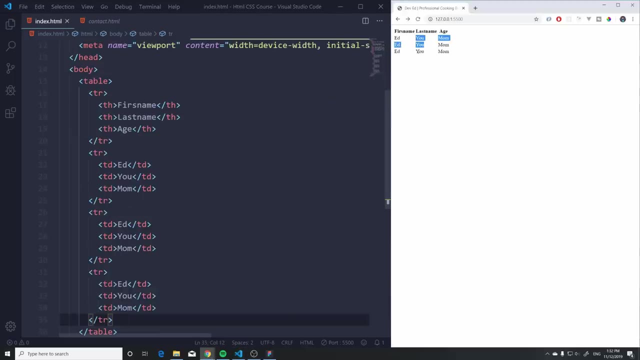 you can see, this is basically the title, the header, the table header in here, And these are the individual values that you can provide down here. So if you want to have more of these, I'm just going to copy this table row multiple times like this: And boom, there we go, We have. 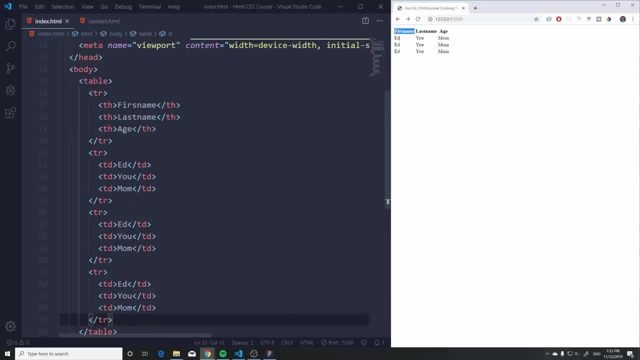 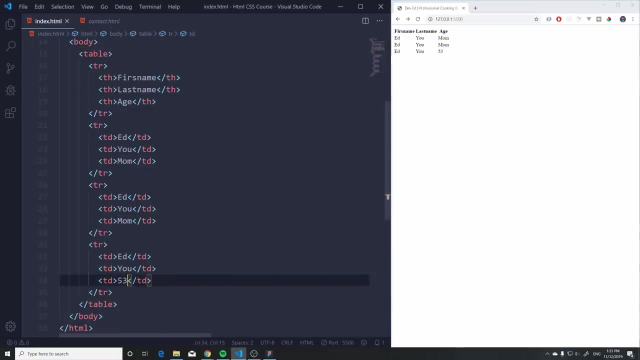 more. So again, this is going to act kind of like the title And this is the list that you have down here with the names and with the last names and with the age. Well, age is mom. That's kind of weird, So we can change that to: how old is she? Oh, mom, I don't know. 23,, 53,, 23.. Goodness, I am. 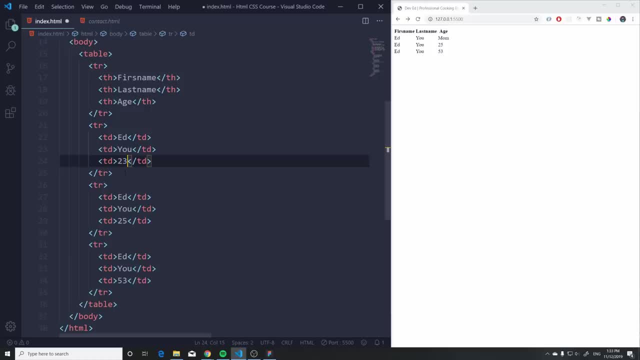 25,, I believe, And you are 23?, 21?, Am I guessing correctly? No, Okay, so this is tables. Very, very simple. If you want to have another column, you just add another one in here, like this, and you have another column And 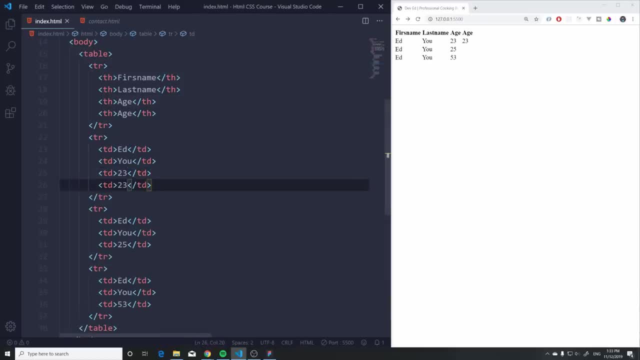 if you want to have another value, you can add it like that, And then we can modify this to date of birth or something, And there we go. It's very simple. I wouldn't worry too much about it. It's nothing too complicated, If you ever need it. 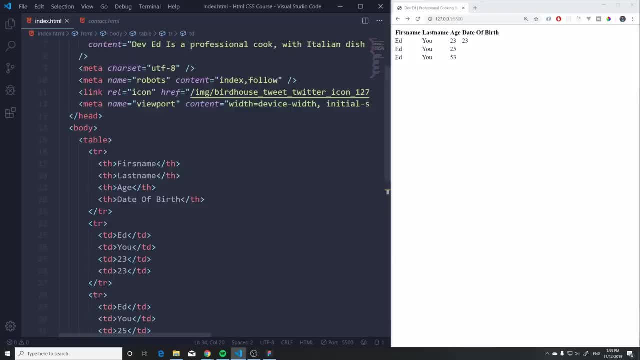 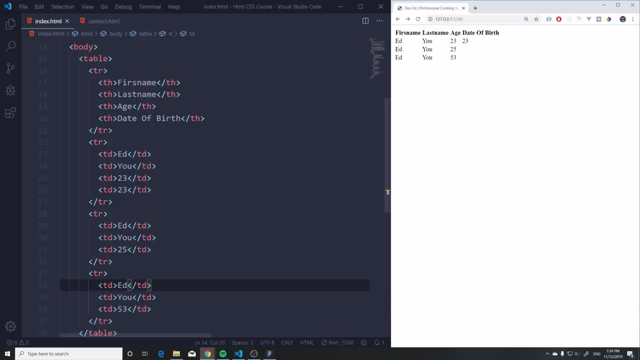 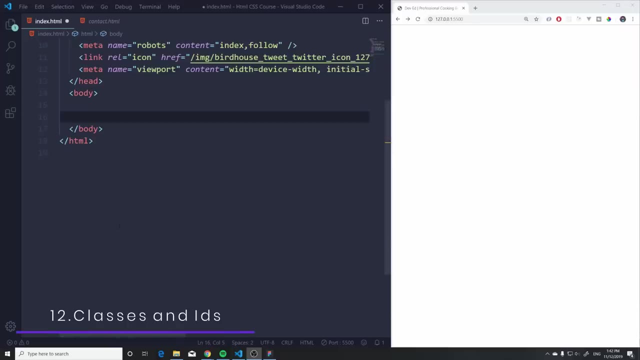 though it's not that difficult to create, And later on we can also style this in CSS if we really want to, But that, again, is just going to be a very, very simple process. So those are tables in a nutshell. Let's cover classes and IDs, because these are so important. You're going to 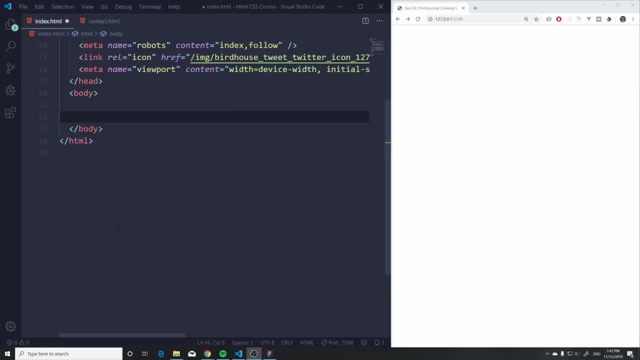 see that you're going to use these, Speaking of that language, we're going to use these across every website, Whenever you start building your own projects. you're going to use these constantly. So they're very, very important. So what I want to show you is: 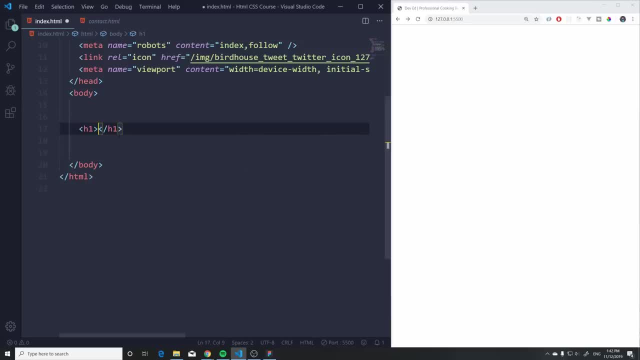 hey, maybe we have some elements on the screen, Maybe we have a H1 here that might be our logo of our website, And then we might have an article here. Let's do a H2 article title like this, And then we might have some paragraphs And we can actually generate random text here by writing. 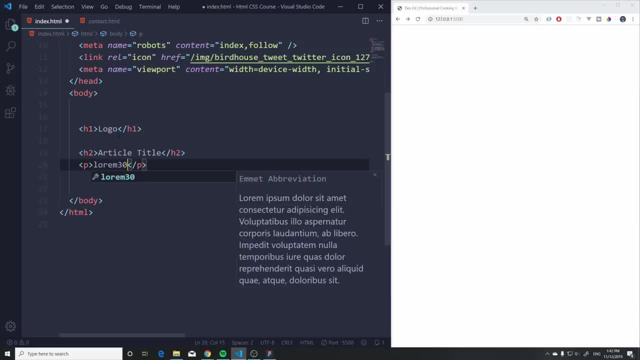 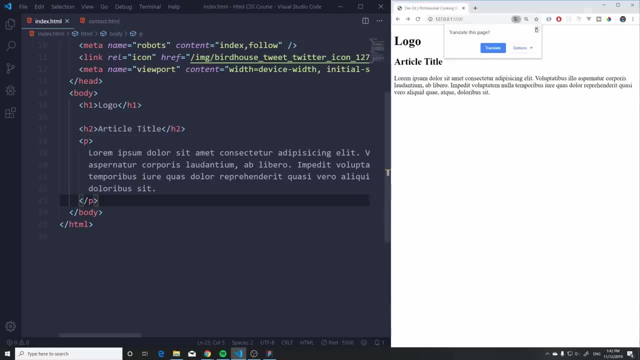 lorem and typing a number. If I want 30 characters, I can type 30 and hit tab And, as you can see, that generates us some random text here And Google Chrome is like: do you want to translate? No, I don't want to translate this. So what we can do is we can copy these multiple times. We can. 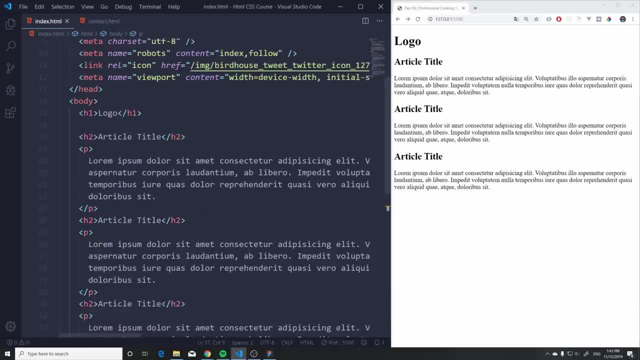 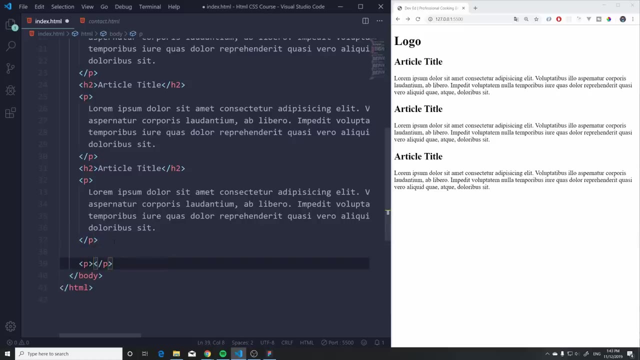 imagine we have a blog or something on our website, A small little blog. Now, when we're going to write to CSS, you might want to style these in certain ways. But right now, what happens if we might have some paragraph here that's totally unrelated? Maybe this is: 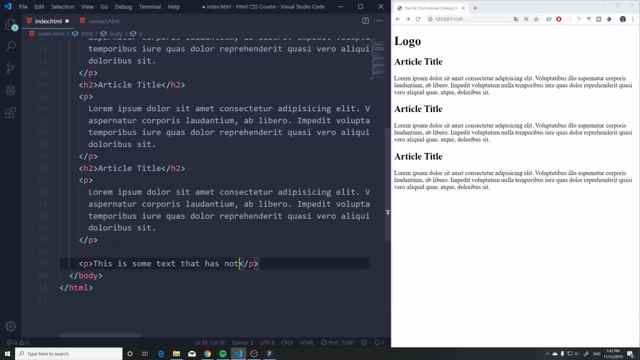 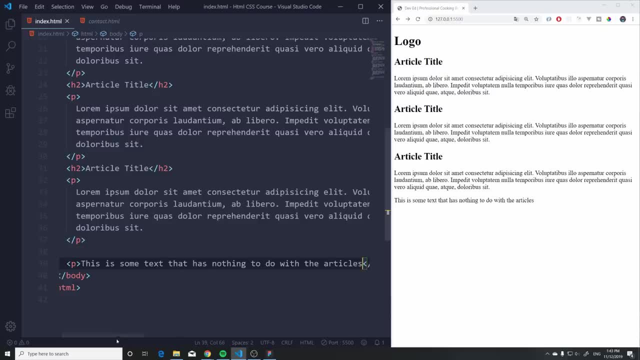 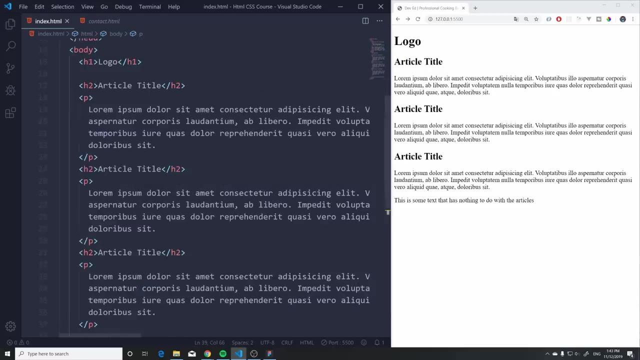 this is some text that has nothing to do with the articles. Well, here is where classes and IDs are going to help us. A class and an ID is basically a selector And it allows us to select certain parts of our HTML. So later on in our CSS and in our JavaScript, we can manipulate and style. 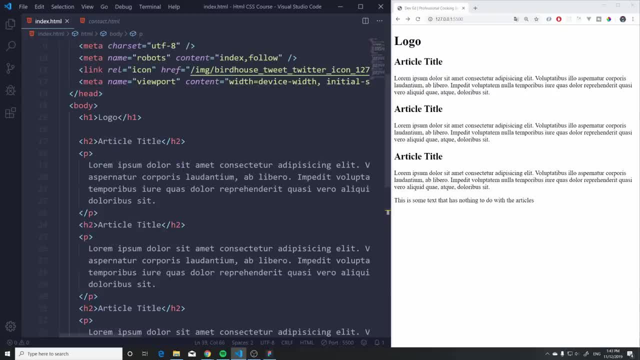 in different ways. So we saw the ID before in our image And we can manipulate and style in different ways, And what an ID is is basically a unique identifier. As you can see, it's a unique identifier of a particular HTML element. So here a great example is the logo. here This can be an ID. 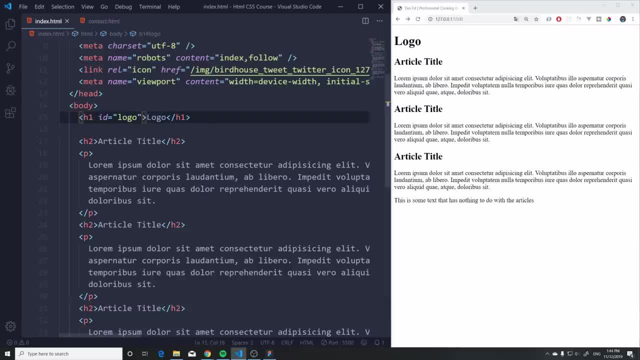 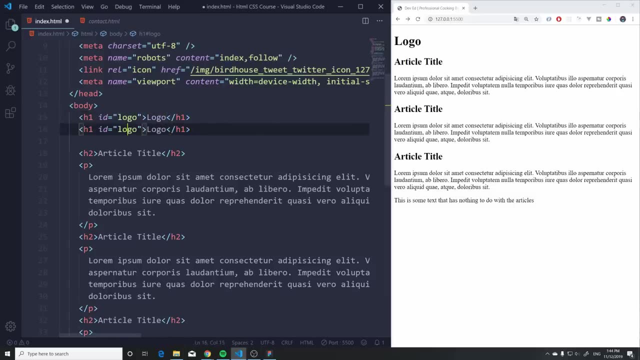 And the reason why it's special is because an ID cannot have the same name. You can only one. you can have multiple IDs, but the name needs to be unique. You cannot, you cannot, have another H1 here with logo. Okay, that's not good. You only can have one. 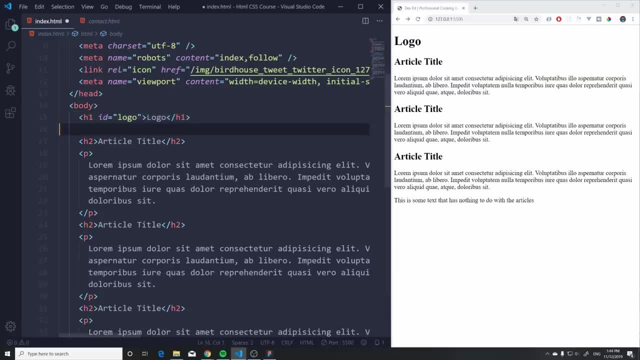 But in classes you can have the same name very easily. And let's take a look on how we can add a class. We just write class, So it kind of works the same way And we can just say something like article text, And I'm going to do it with like a small dash between, like this: All right, 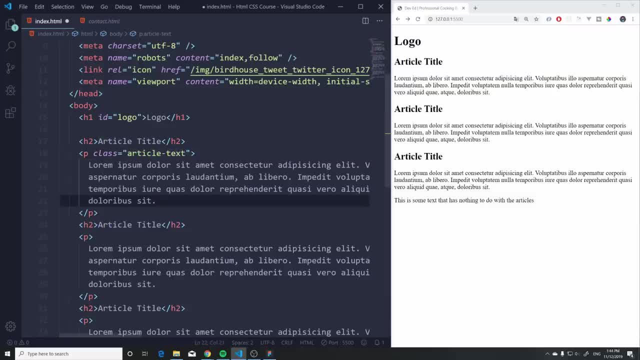 this is very simple and clear to read, And you usually want to give names to your classes and IDs that resemble of basically what the HTML element does. So what is this? Well, it's the article text, So that's what I'm going to name it, And also separated by 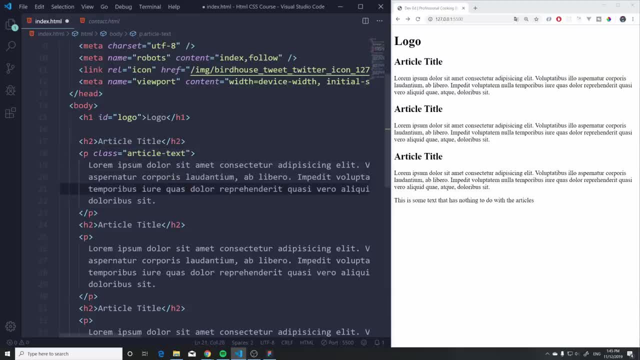 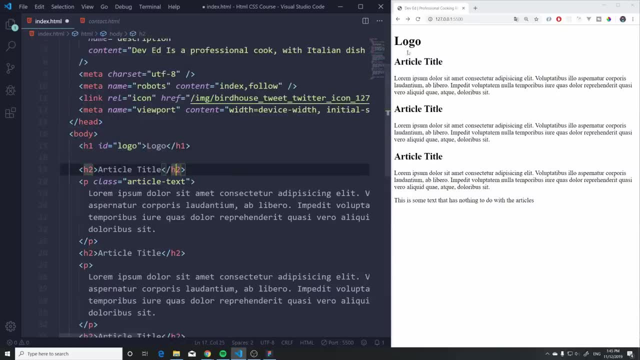 a small dash here just makes everything clear and very readable. Okay, so that's the difference between the two. This is unique. you can only have one of these And, again, a great example is maybe a logo on your website. That is probably only one. So it's very unique. So you would. 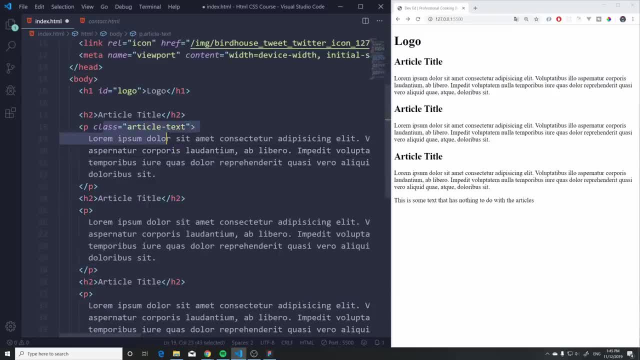 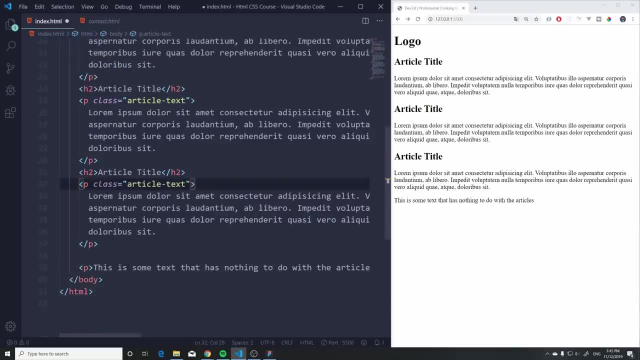 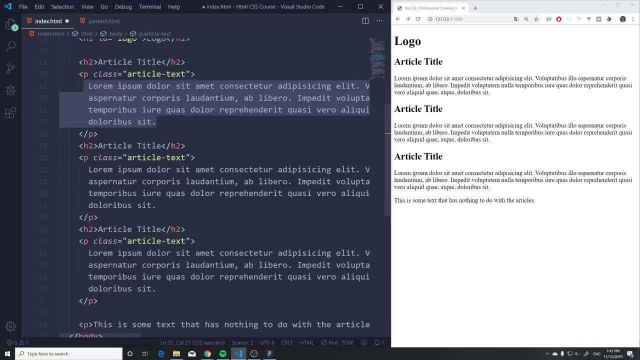 name it logo And here classes. we can have the same name added multiple times So I can have it across all of these different paragraphs. So later on you can imagine that we can select this class by the name article text and we can style only these specifically. And the difference is that 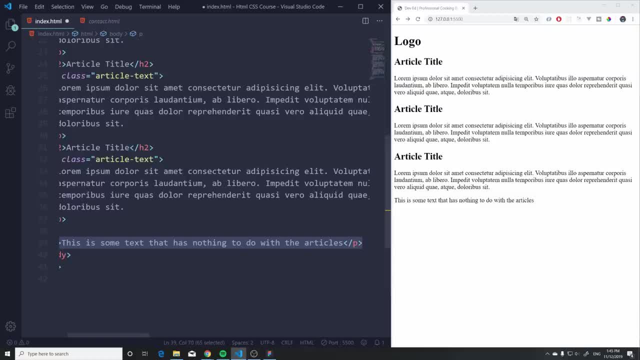 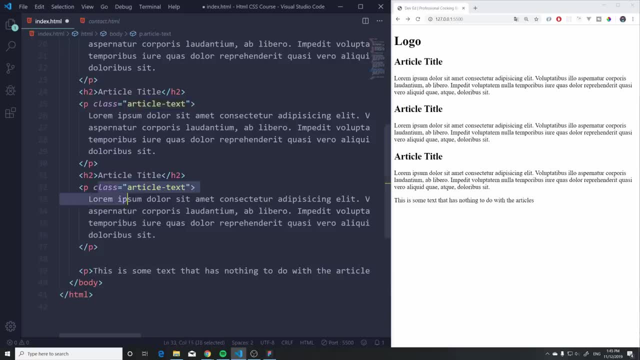 it's not going to affect this right- the ones that don't have this specific class. So what we're going to do is select this class and it's only going to style the classes or the paragraphs that have this specific class. That's kind of a tongue twister. 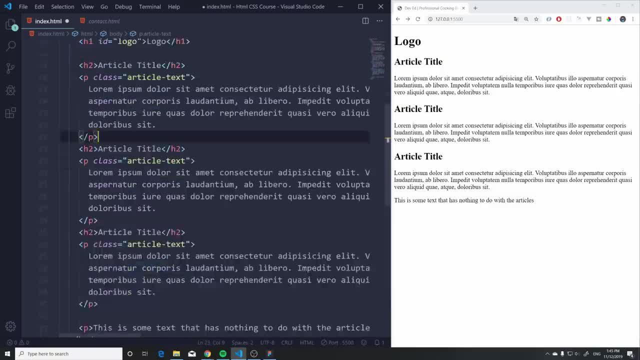 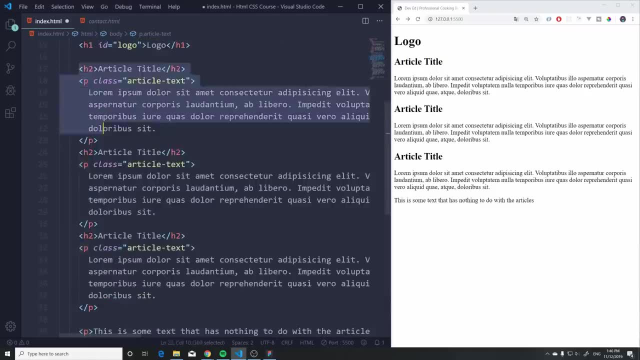 Did that even make it? I'm not sure if that made any sense, But again, because we're going to see later on in CSS, if you just select our P tags and you want to style them, it's going to affect everything that you have all the P tags in your HTML. However, with classes and IDs, you can select. 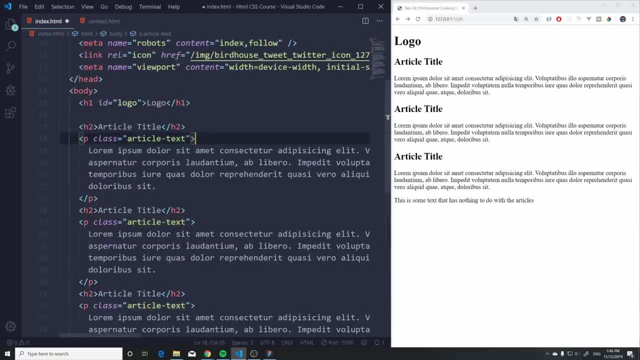 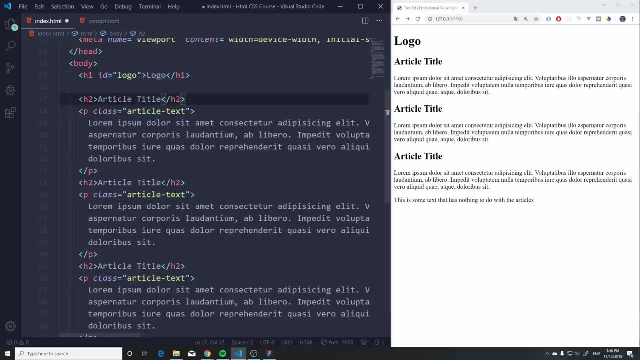 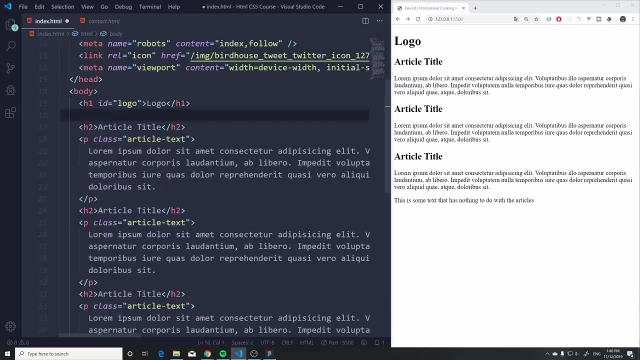 them by the name that you provide in here. Okay, and we're going to also see some differences with classes and IDs When we arrive to CSS, because there's like a specificity going on which is more important than which. But that's all you have to remember for now. Logos: if you have something unique on your 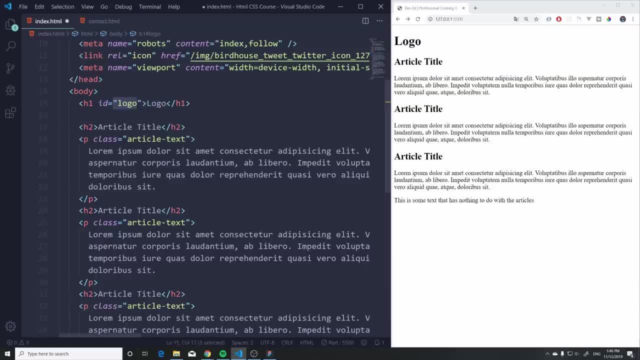 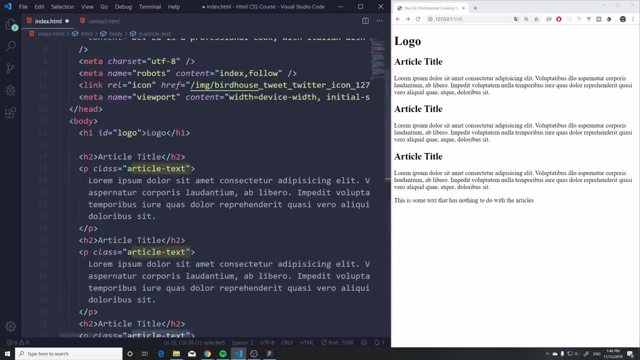 website and you want to give it a name, so later on you can style it in your CSS and JavaScript. then you can use an ID as long as the name is completely unique. When you have multiple things or less important things or things that you want to name the same, then you can use classes for. 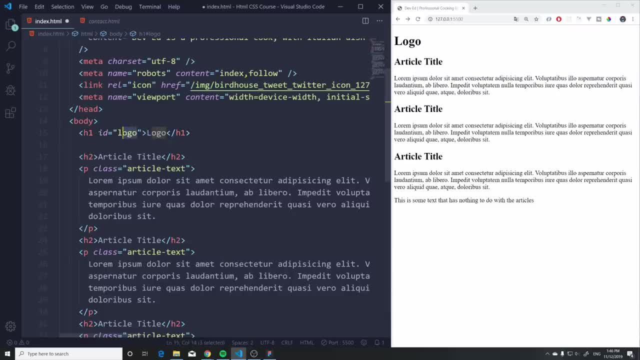 that Also very quickly. the character needs to be at least one character long, Okay, and you also cannot have spaces or anything like that. make sure you negate any spaces. don't do something like this, Because what you can also have is two classes on one element. 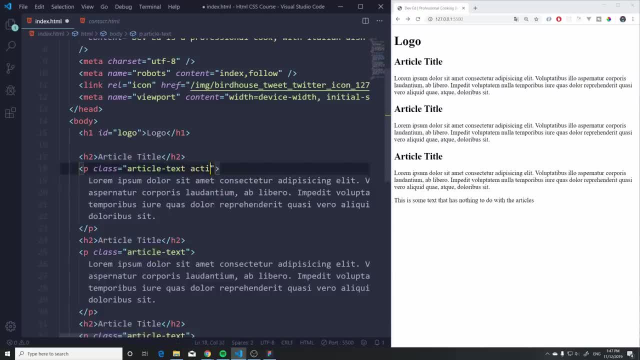 you can have article text and maybe article text active, Alright, so these are two separate classes here, Alright, that's the difference. So we can maybe style this in one way and we can style the active in another way if we want. 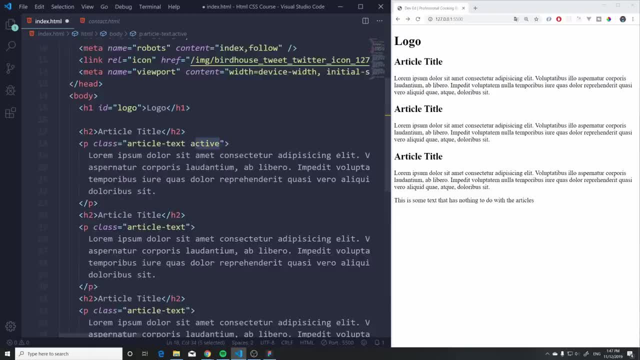 Okay, so, without confusing you too much, I'm gonna leave you to it like this, and I promise it's gonna make way more sense when we get to CSS, Because right now we're just naming these for no reason and nothing's happening. 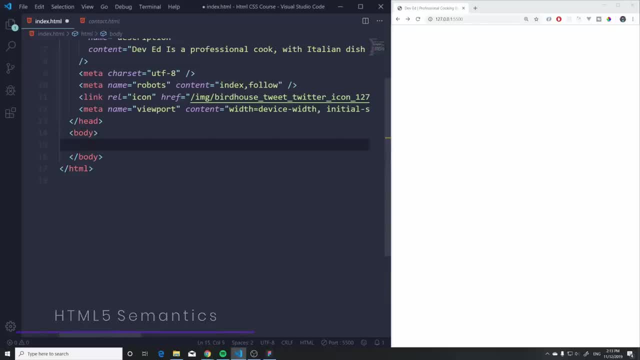 Okay. so one problem that we might be facing is, let's say, we want to create a website, So we add our H1, here we. this is this can be our logo. And then we have our UL with our Maybe. this is our contact, So this is our navigation. So let's say: home here. Let's say: 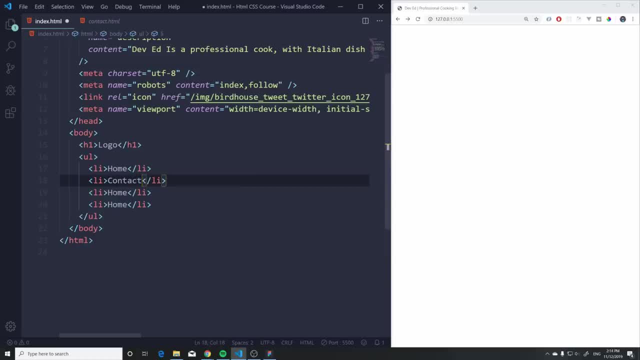 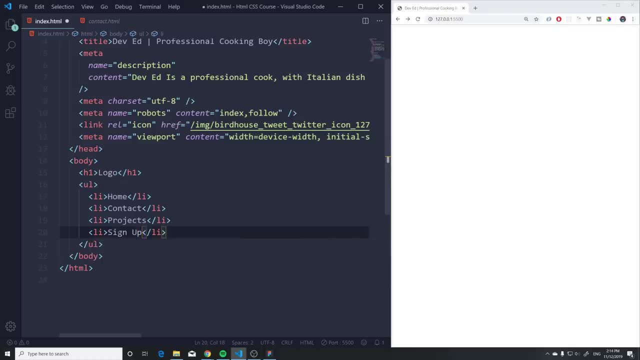 contact projects And I don't know, maybe we have a sign up or something. Sign up, Okay. And then let's say we have another section here that we want to write about ourselves, So we can add a page to: this is us, And then we might have a paragraph here as well: form 20.. And then we 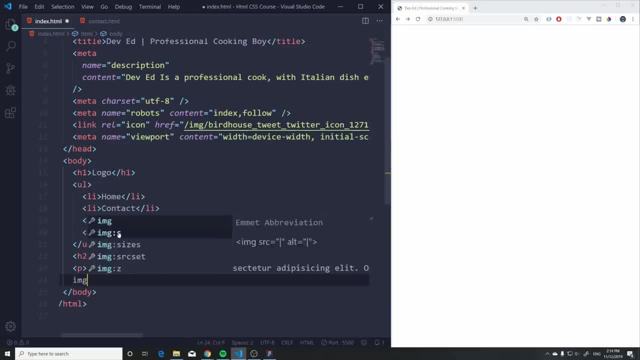 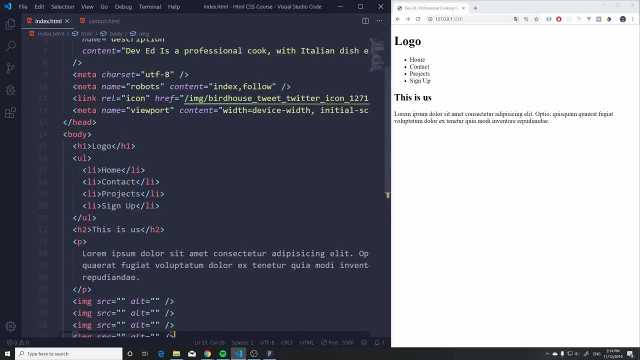 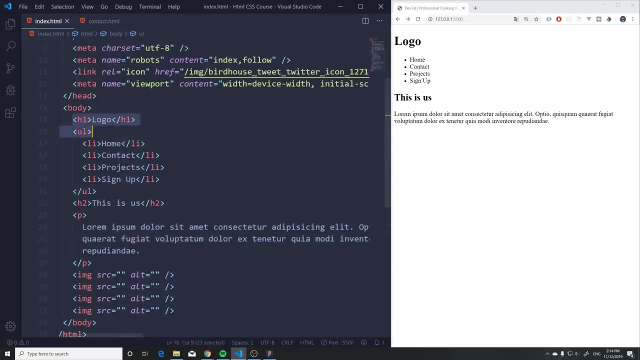 might want to add some images down below here, So image, and we might have multiple images like this. So what's the problem with this? The problem with this is that everything is kind of chaotic and everything just kind of flows here together. There are no clear, distinct sections between our 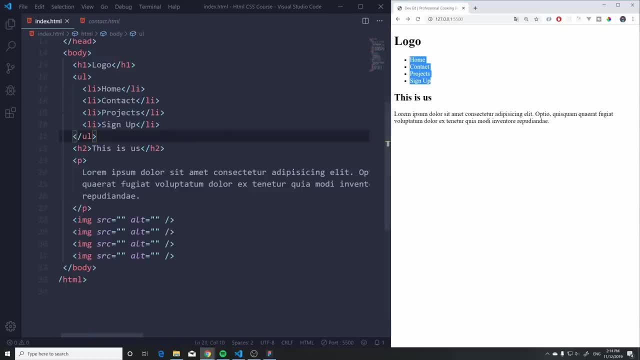 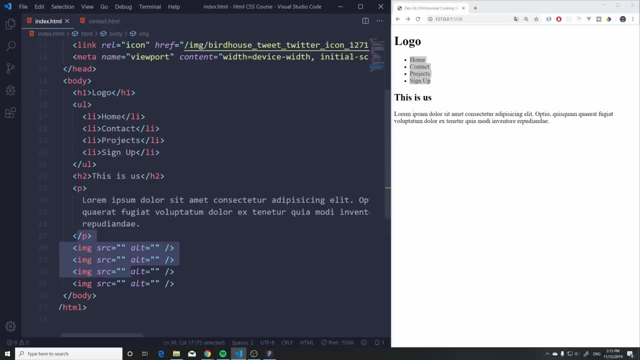 header here, or our navigation, or our paragraph here, or the image gallery that we have down here below. So we have a HTML element called div, which is mainly used as a wrapper to kind of organize everything together for you, And this is also going to help us tremendously in our CSS. So what you can do is you can wrap all the necessary. 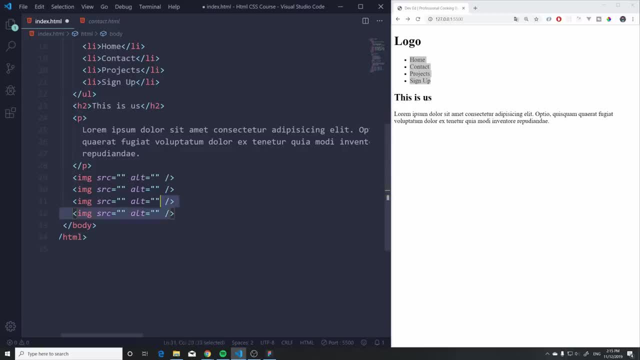 things that you want inside a div. So maybe this is going to be an image gallery, So rather than having them floating in space, you can wrap them inside a div like this: And now everything is wrapped inside this div, So maybe we can add a class to this and we can call it gallery. So now in our CSS we can just grab this: 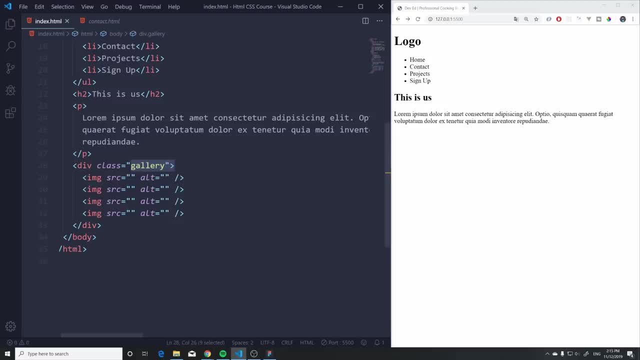 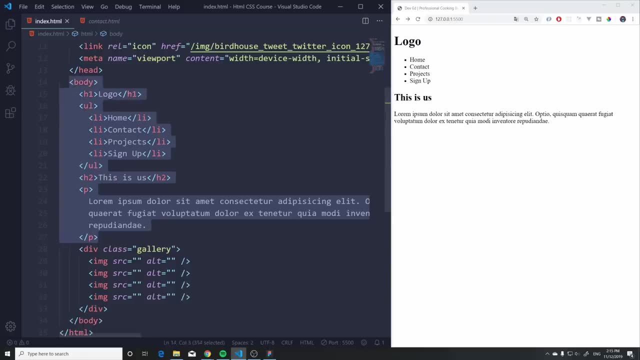 gallery and position it and modify it the way we want. But it's way easier to do it like this and everything is organized, then just have everything floating out here on the screen. Now, one thing that we're going to get into in just a bit is called the new div, So we're going to 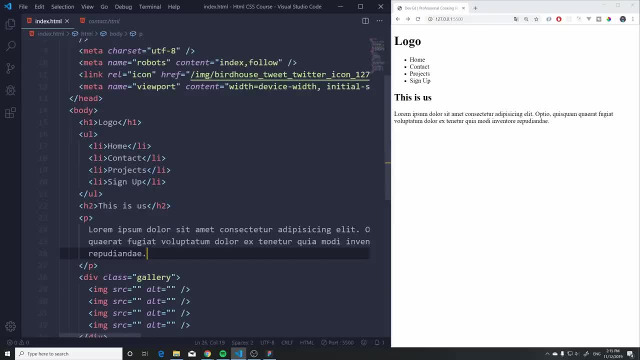 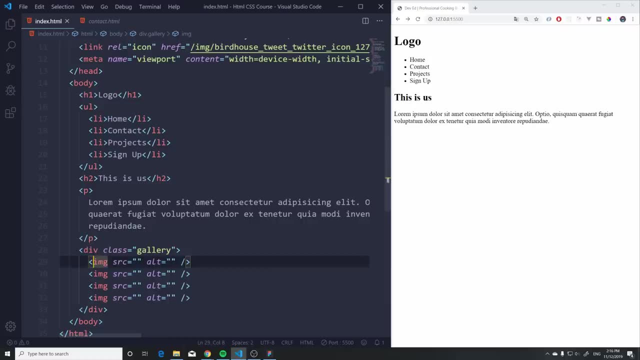 get into the new HTML5 semantic elements, which are very important, because the difference, the thing with these divs is that they're non-semantic. okay, They don't actually have a special meaning at all. As you can see, it even says it to us. Element has no special meaning, It just represents its 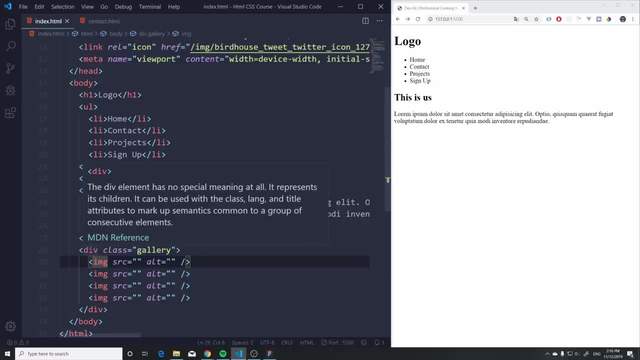 children. It can be used with a class, lang and title to group consecutive elements together, So it has no meaning, Just as we had span before. this is also called a non-semantic element, So this is a non-semantic element. It doesn't actually tell us anything about this. Fujiyat here. okay, However. 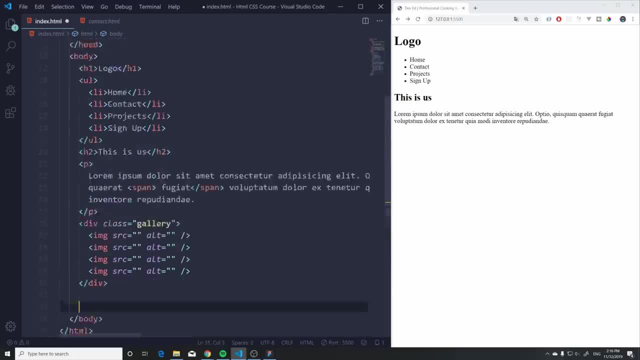 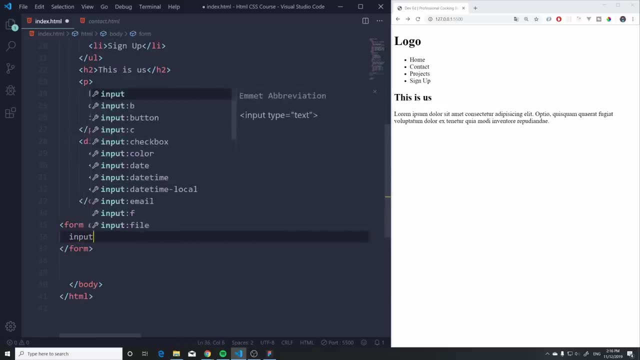 a semantic element, just to kind of give you a good example for you is something like a form. This also acts as a wrapper to our input elements like this, But this has semantic meaning to it, rather than a div. A div doesn't say anything to us, But a form is. 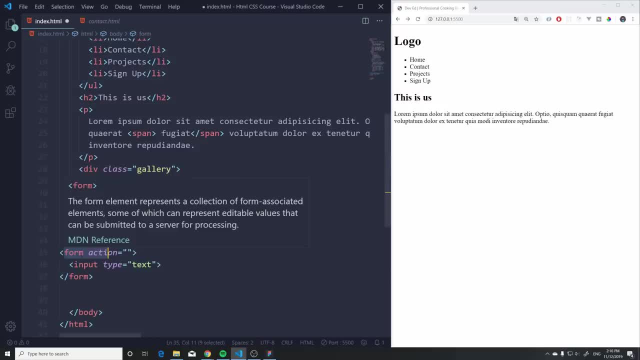 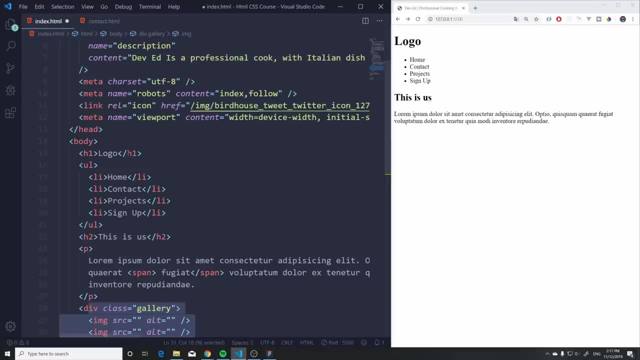 a clear semantic element that has a clear purpose, And what we want to do is we want to replace these empty things with specific semantic elements that have a purpose. So even this thing, this h1 here, should be our header, So we could drop this in a div. 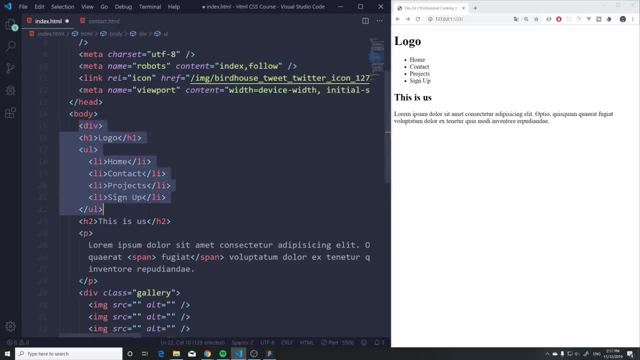 like this and we can wrap actually everything here, The whole thing until here. so this can be maybe our class of header and this ul thing can be our navigation, right? so let's do another. and here's a quick shortcut also to create a class very quickly with a div: you just add a dot and you give it a name, nav, and then hit. 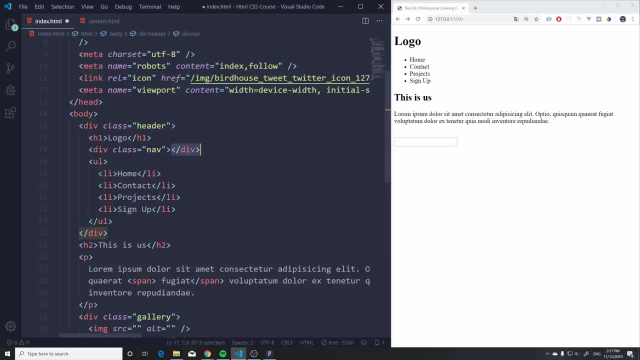 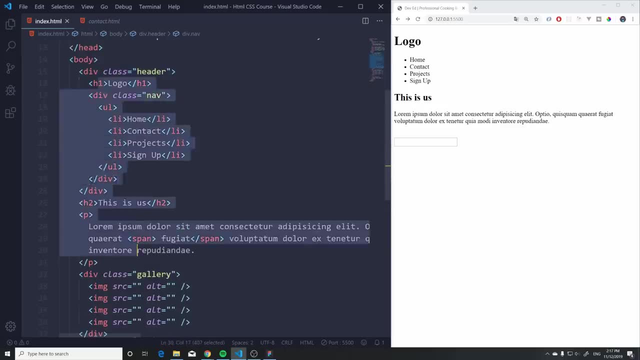 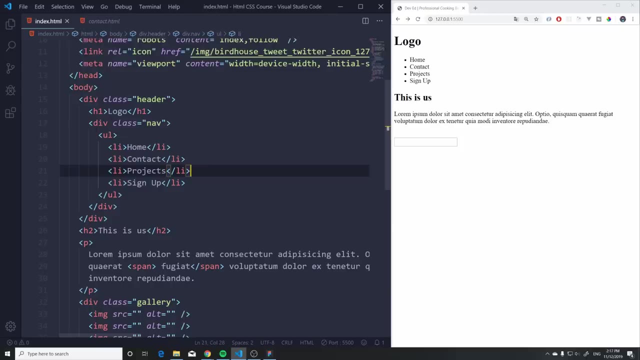 tab and that's automatically going to generate you a div with the class of nav. so i'm going to wrap this everything in here together and there we go. that's kind of the gist of it, but again, this is kind of problematic because it doesn't actually have any semantic meaning to it. so, with html5 and 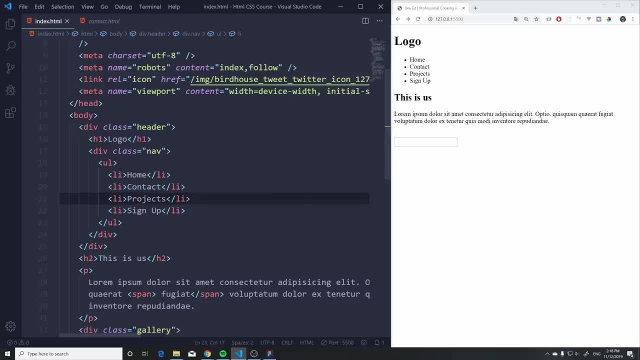 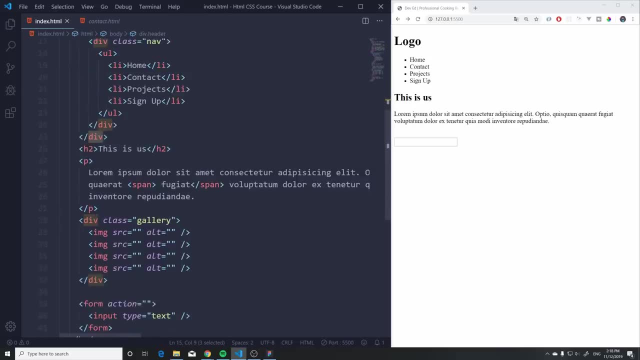 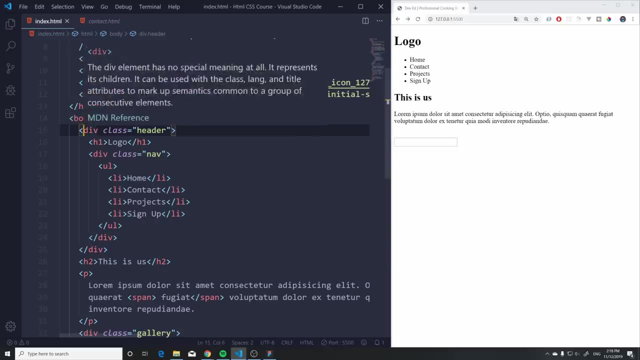 the recent years, we got some new elements that perfectly describe what, what we have on the screen. so, rather than wrapping everything in these empty divs that don't mean nothing, we have these semantic elements, so let me show you. rather than naming this div, i'm gonna get rid of the header. i can. 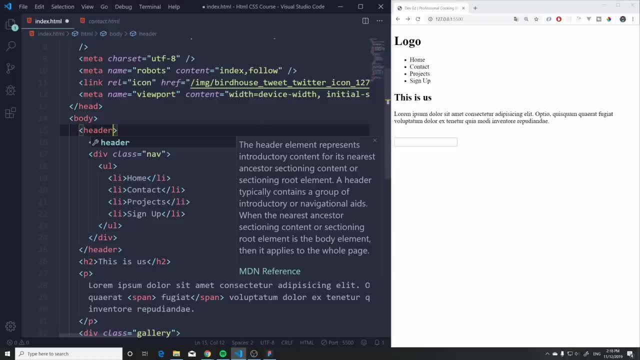 just name it, header you. there we go and, as you can see, you also get a small description. it says: the header represents introductory content for its nearest ancestors. okay, so a element, a header typically contains a group of introductory or navigation aids, so it doesn't actually describe any of your content. 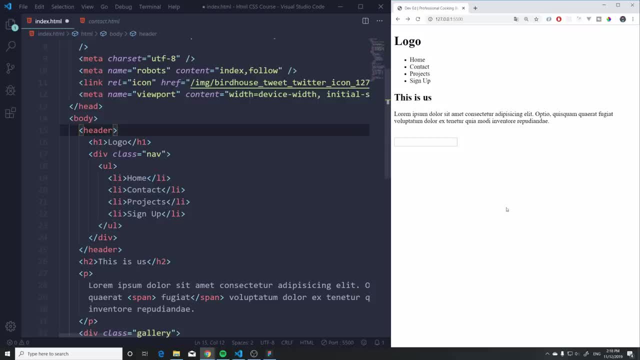 that you're going to have on the page later on. maybe you have a section with some images, maybe you have a blog post and things of that sort. you don't want that in the header. it's just kind of a introductory content for its nearest ancestors. okay, so a header typically contains a group of: 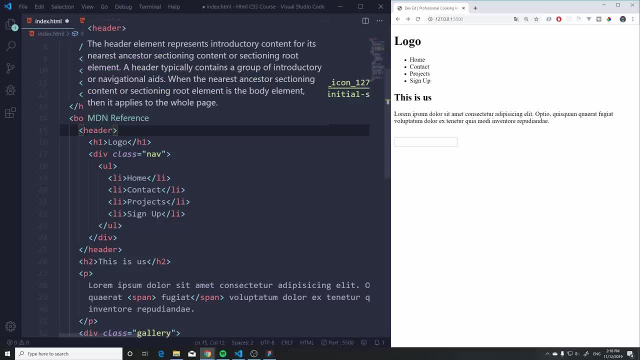 introductory thing that's going to help you with navigating and things of that sort. so we have our header here, and a good thing to have is our logo. so there we go. we have our logo, which is a h1, so it's very important. it's a big heading and, rather than naming this a class of nav, what we can do is 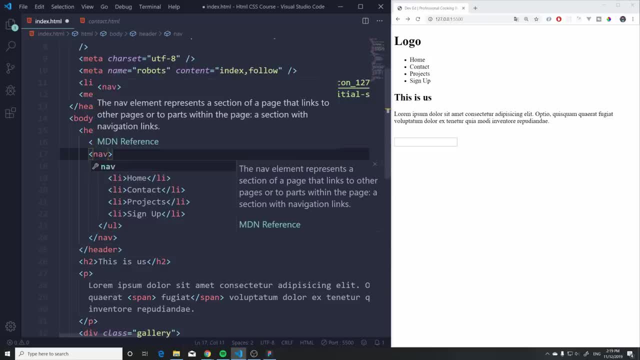 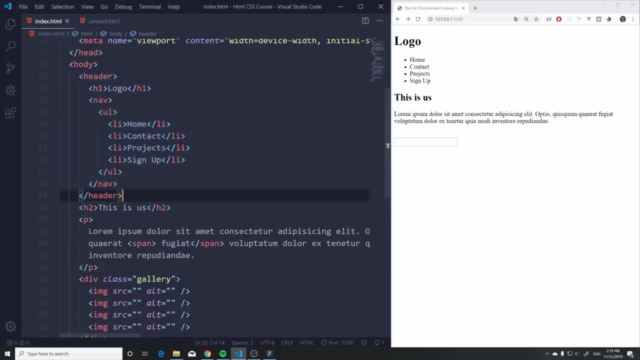 replace this with nav as well. so this perfectly describes, as you can see, represents a section of the page that links to other pages or parts within the page, so it's very important to use this, specifically made for navigating. okay, perfect, so now we are using the correct semantic html elements, so let me quickly show you a part of the page, like this one that 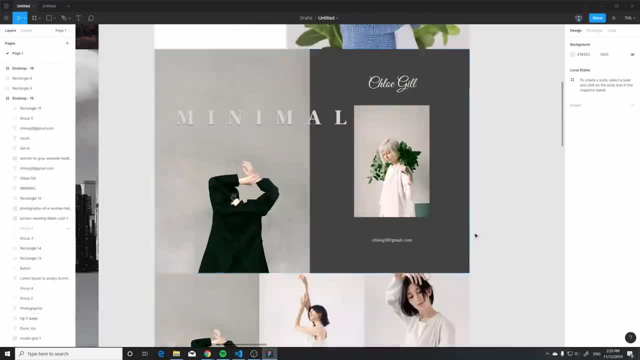 we're eventually going to build out. so we have this part here and maybe i want to group it together. so, rather than making one big diff here, we can create a html element called section, and a section is usually used just to group together some content, typically with a heading. all right, so it's just. a section is a thematic grouping of. 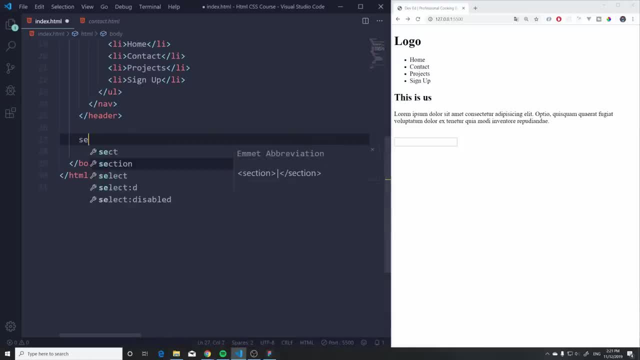 some content, okay. so what we can do is we can write section like this: and here maybe we can have a h2, that's gonna say, here is my image gallery, like this: okay, so that would be a section and in here we can have all of our images. but typically we used images like this: boom, boom, boom. 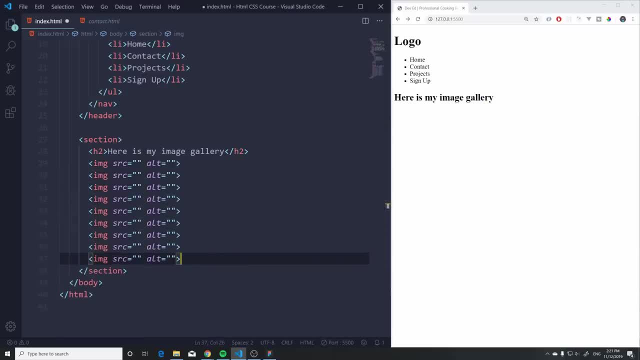 and there is nothing wrong with this. there is absolutely nothing wrong with using images like this, but recently there has been a new element added that's called figure, and all a figure does. it helps add some visual explanation to an image. all right, because there was no proper way of adding. 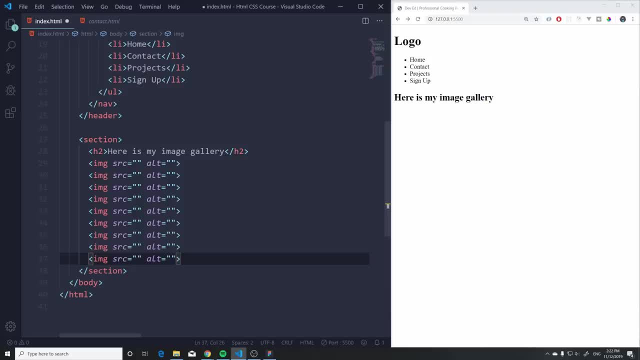 semantically adding- you know, you know a caption to an image. but now you can do that. you can do a figure like this, and inside this figure you can add your image, and in here we can also add something called a fig. let me not make a mistake. 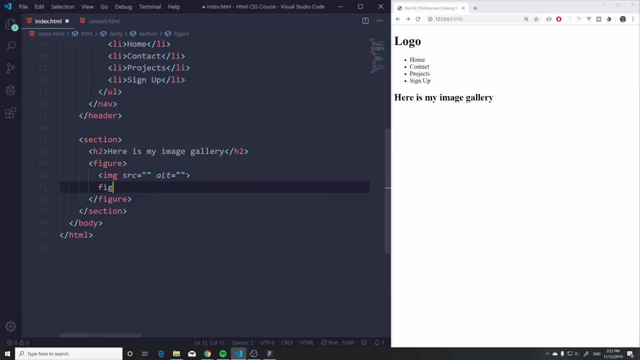 here fig caption like this. all right, it's not working for some reason. let's say: fig. oh, there we go, fig caption now it appears. so fig action elements represents a caption or a legend, for the fig caption elements parents figure elements. oh my goodness, that's very long, so we can add a fig. 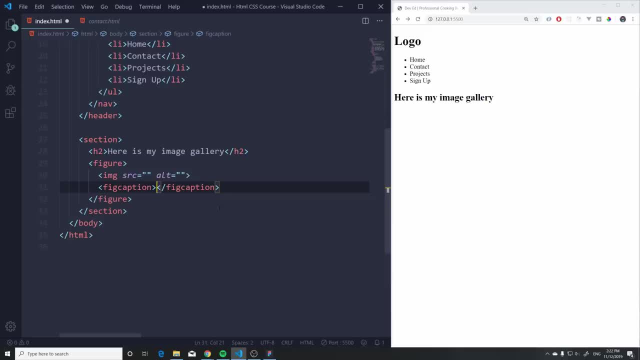 caption like this and we can describe the image. so just add a simple cash caption. uh, let's say, major picture by dev head, all right, and this is going to be different from the alt tag, because this actually describes what the image is. so maybe i have a picture with a mountain mountain. 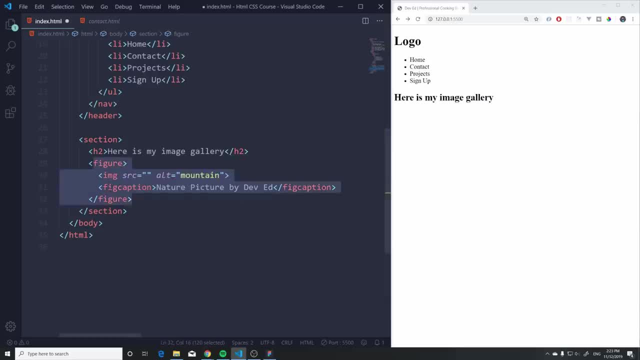 like that. okay, so we can also use this figure to add captions and it's going to be semantically good, okay, so section: we use it to group in together a part or a section of our website and also figure that helps us add some semantic to our images with captions. at the end of our website we also have the footer that typically. 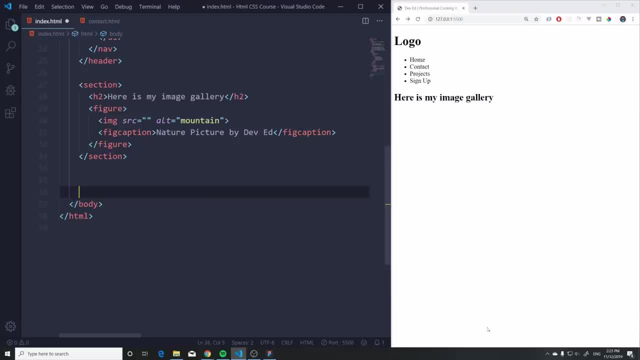 gives some more information about the website or maybe some social links, so we can use that as well at the bottom of our website and then we can add some more information about the website at the bottom of the page and rather than again making a simple div with a class of footer, we can. 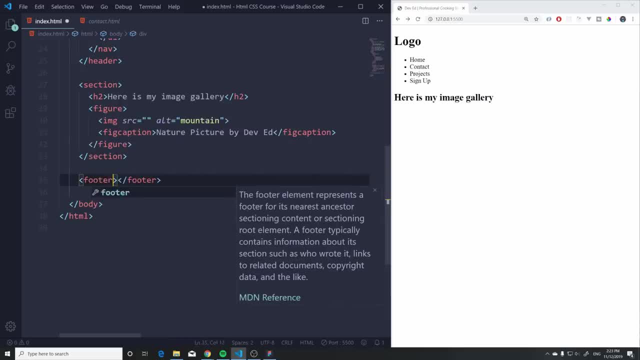 just use a footer, so let's rename this to footer like this and in here in a footer, typically you have the author of the document, copyright information, contact information, social links and things of that sort. so maybe created the website was created 2018, copyright, whatever things of that sort- and maybe we can add some more information about the website and then we can. 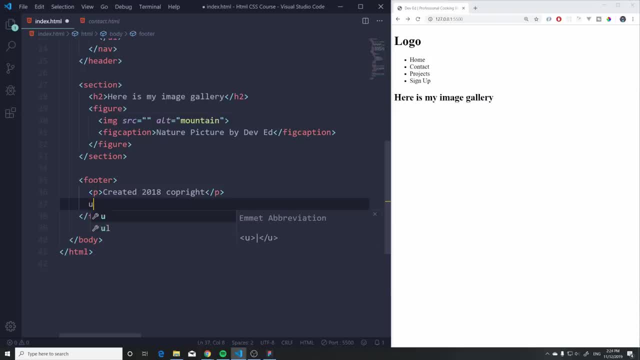 add some more information about the website and maybe you have some social links in here, so maybe you can have a ul with an lia, all right, so we add an anchor tag and we have some a link to my twitter dot com- slash, whatever we have- and this says here: twitter. all right, so this is a footer we're gonna. 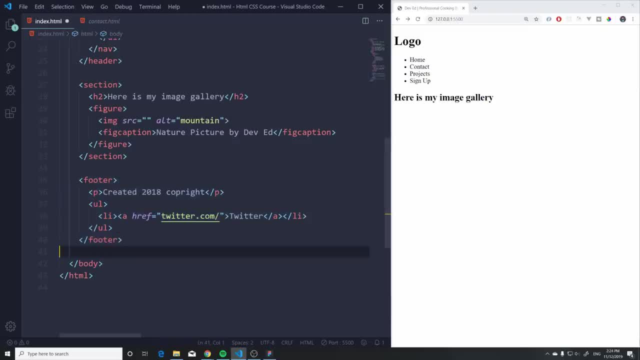 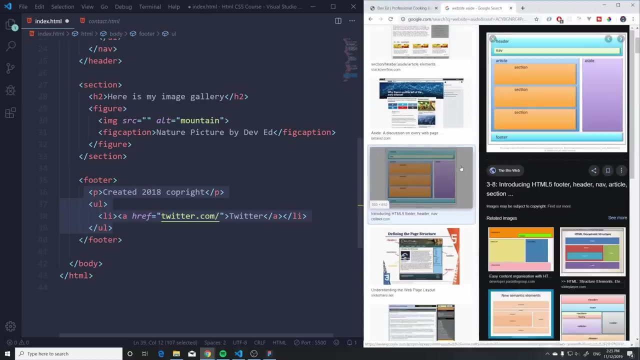 add this later on to all of our websites as well. but just more information about social links again contains just information about the author or about the website. okay, there's two more i want to cover, and i was quickly google searching here and i i didn't find anything that looks. 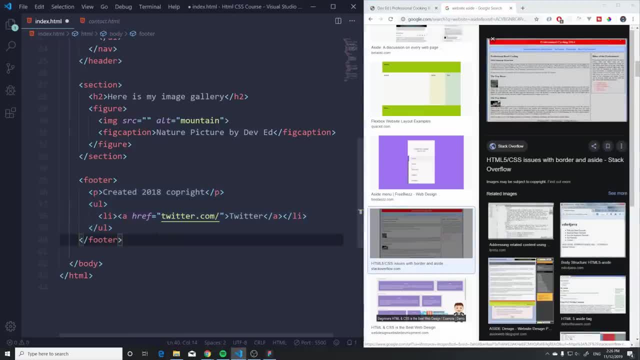 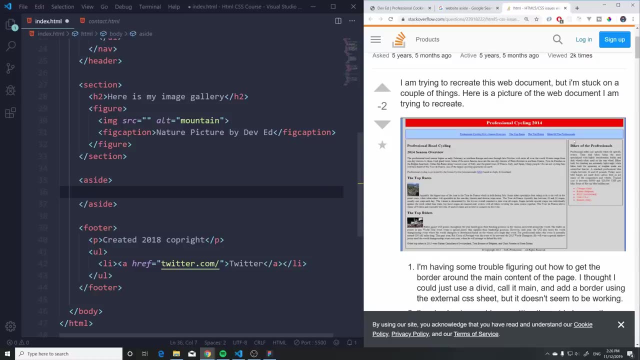 remotely decent, but there's one called a side, so let's go up here and you write it exactly like this: a side and this typically. can i open this image? all right, this a side is this part of the website, okay, as you can see down here, and all it does is it acts kind of like a sidebar. okay, it has. 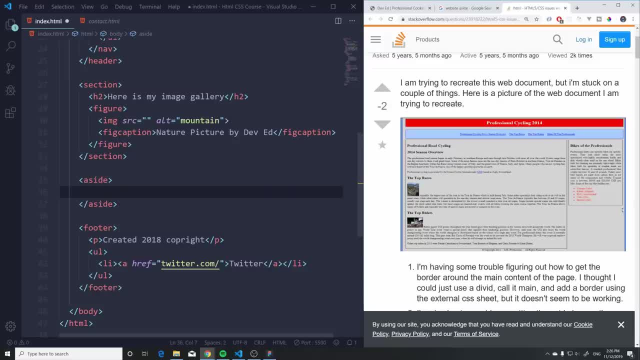 content that is typically used in a sidebar, and all you have to know is that this sidebar should have content that is related to the surrounding content. so this, so this can act like maybe you have a book here or something and then you have an a side with all the chapters that you can select. 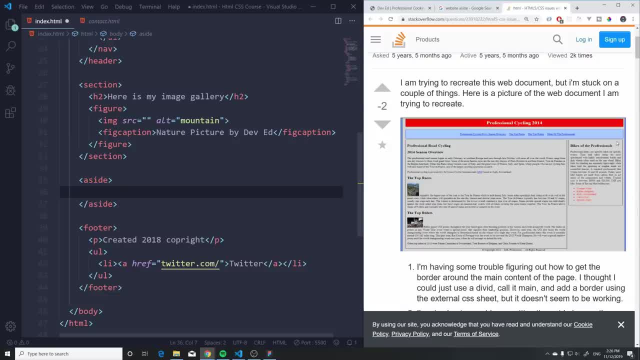 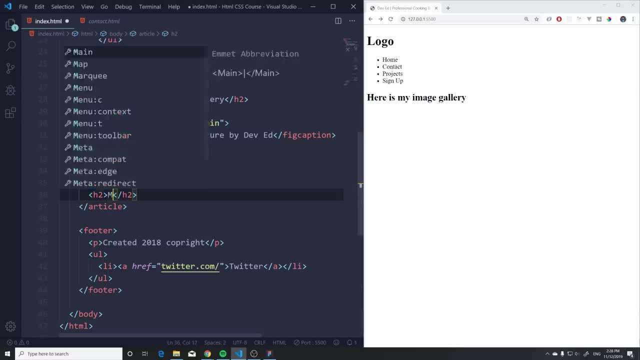 so you can click through the chapters. that can be a perfect a a. we have an article and that can look similar to a section. we might have a heading here as well- my little book, and we might have some paragraphs as well, and maybe some images too. so what's the? 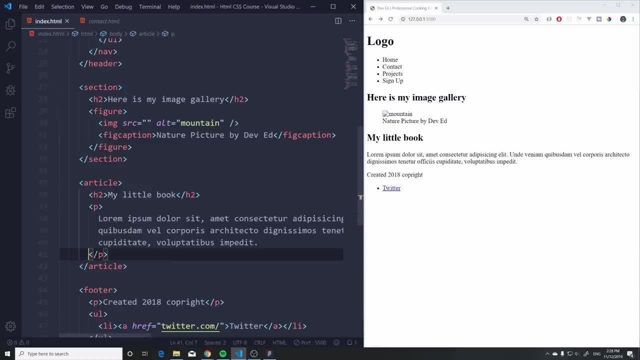 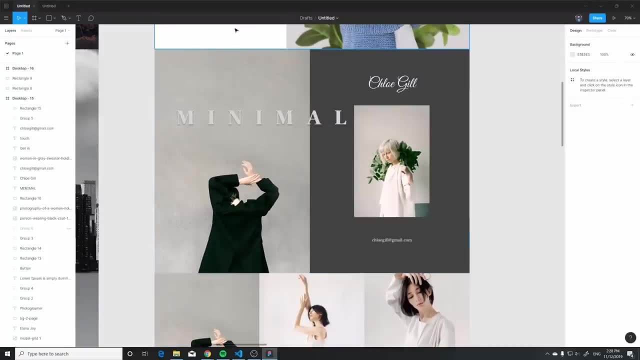 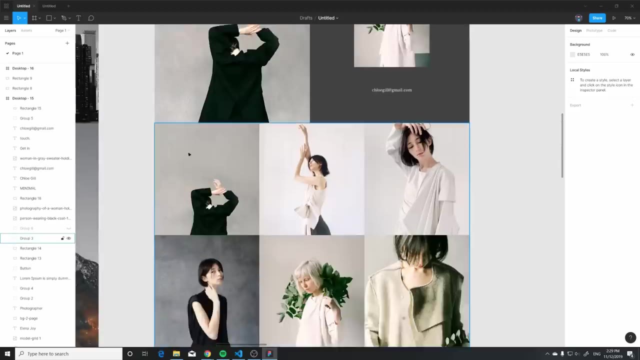 difference between this and this. well, a section is well. imagine like we only have this section on our page. okay, so this section only. well, this doesn't tell us too much, it doesn't really make any sense, right? but if you have multiple sections and you can see all of it, then it makes more sense. 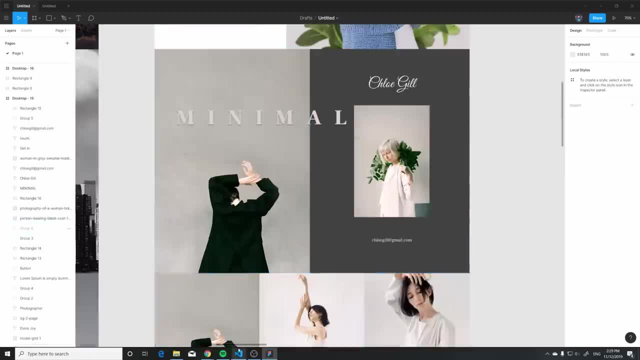 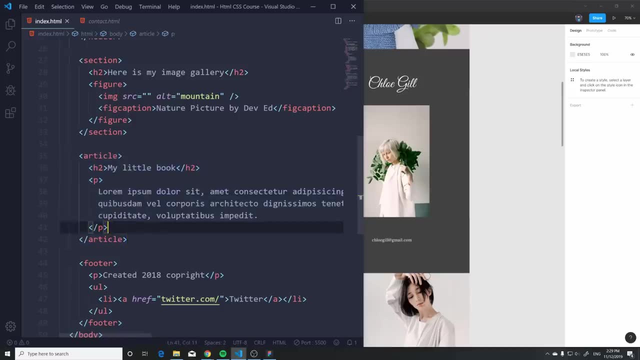 right, you need to have the general scope of the website. however, an article needs to make sense on its own, so you can imagine it, as you can read this whole thing in here and and you get the context, it makes perfect sense. you can imagine it as being like a blog post or an article, right you? 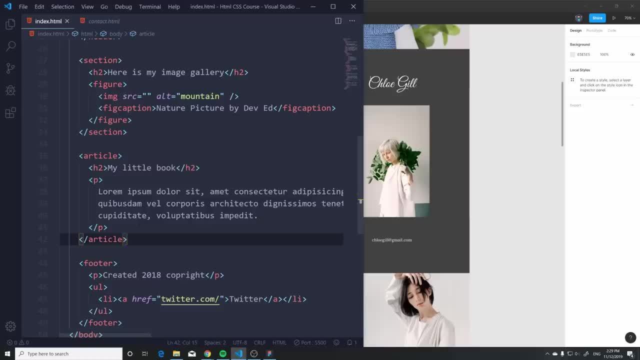 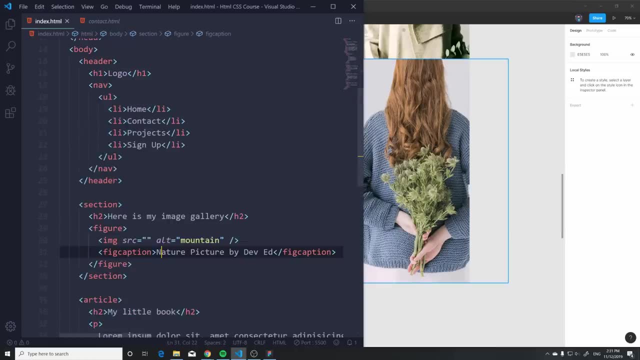 can read an article. you don't need to know anything else about the website and you can imagine it as something that's gonna make perfect sense. lastly, what i want to cover is the html element called main, and main is used only once in our document and it covers basically your main. 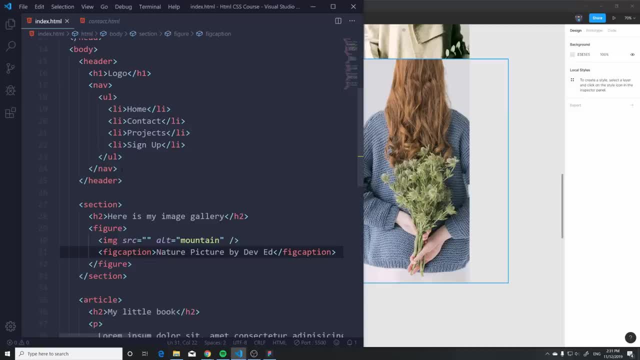 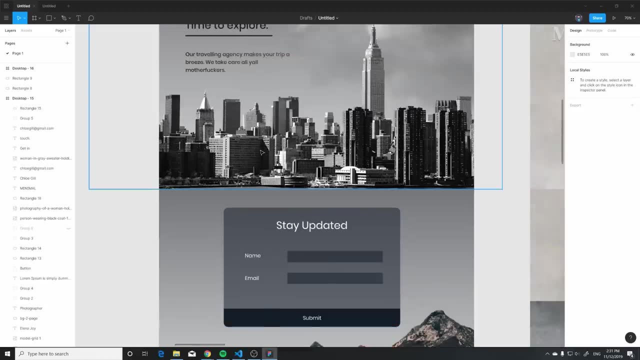 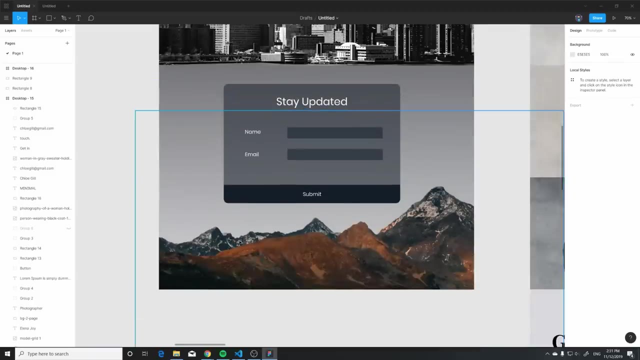 content, so not navigation links, not anything else. so basically, for example, on this web page, the main content would be from here all the way down here. all right, the, the header and the heading and the navigations and footer that we're going to add the in the main content and then we're going to add the footer and we're going to add the main content. 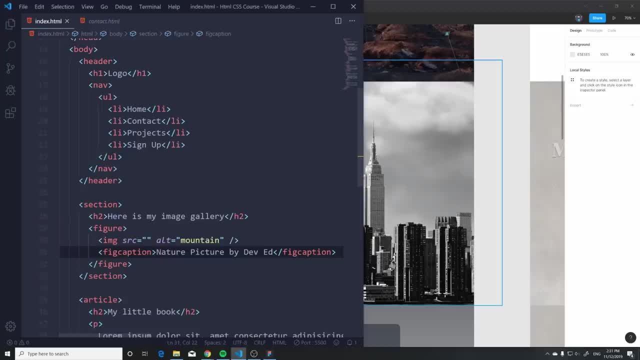 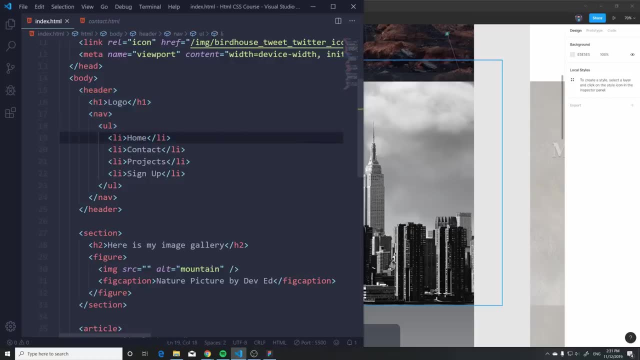 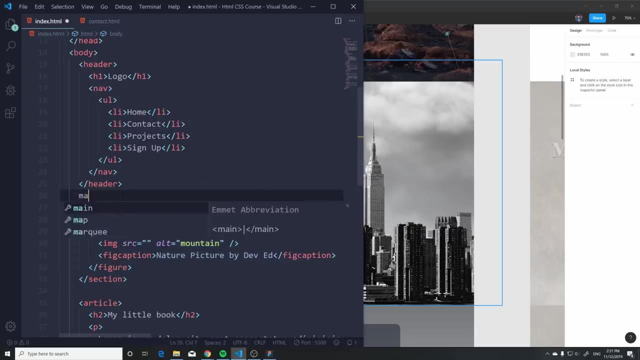 eventually down here, has nothing to do with the main content of our website. So here, what I would do is I would have my header- Okay, that's fine. And then we have our nav, which is fine, And these sections and articles and everything else. we can wrap it once in main, because this is the main. 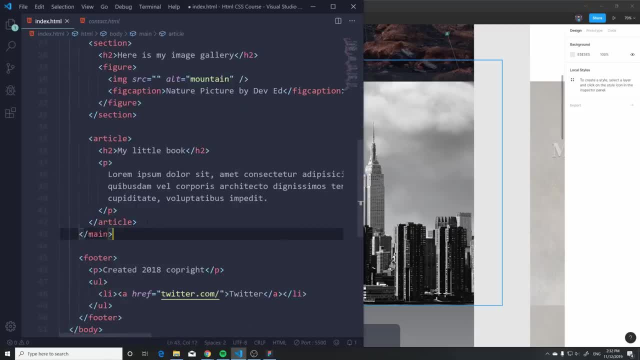 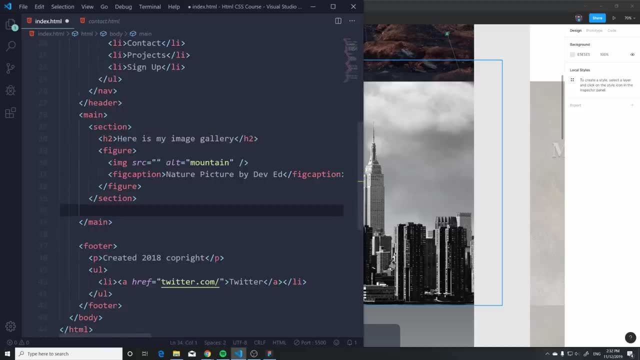 content of the website. So let's go all the way here and wrap everything up, Okay, And actually I'm going to take this article and cut it out here and add it to these sections, So maybe I have multiple articles like this. All right, perfect. So let's take a look at this again. 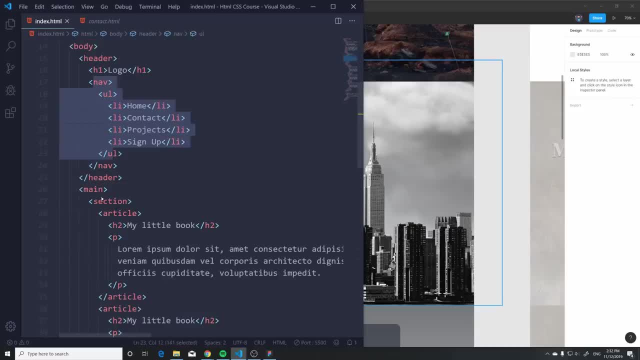 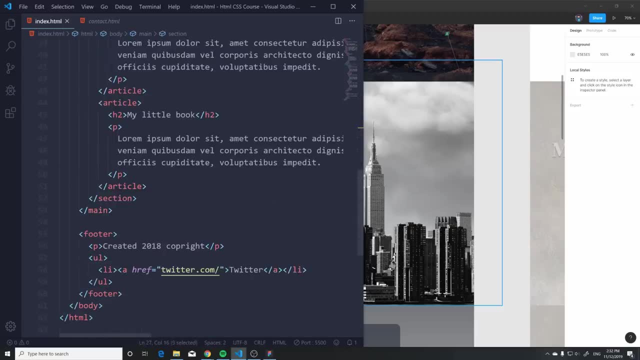 We have our header with our logo. in navigation, We have our main, which holds the main content of our website, And then we can have a section that holds all the articles. We might have another section that has an image gallery of some sort, and we can add a class of. 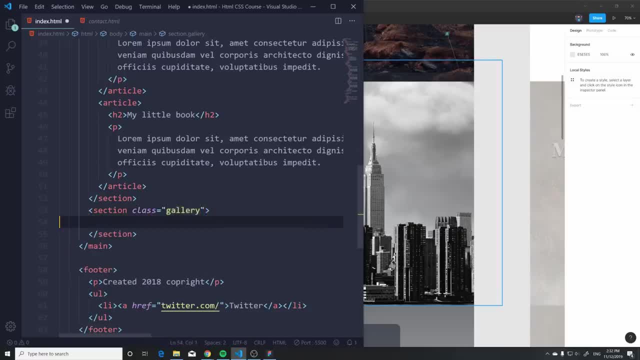 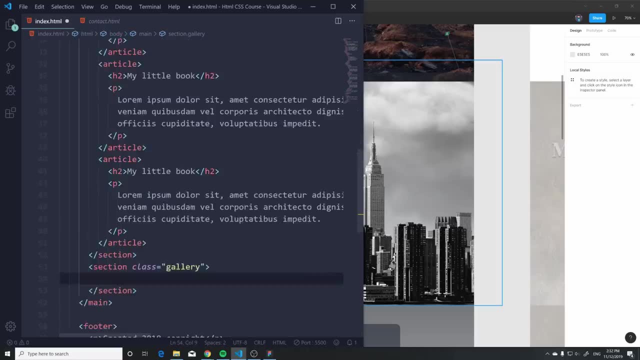 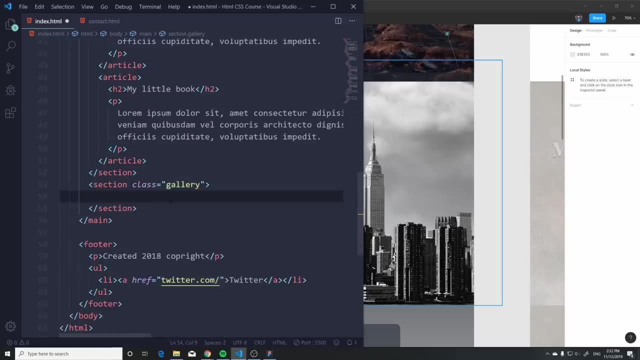 gallery. Now just to make it clear that we might still need divs. just because we have these HTML5 semantic elements doesn't mean that we are not going to use divs, because in certain cases you might want to group specific things together in some way, So in this gallery we might have a. 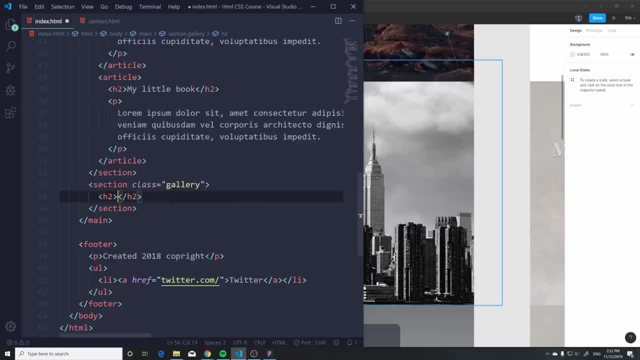 title or a heading, So we can say: these are my images and I might want to group some things in specific ways. So maybe I want to group some things in specific ways. So maybe I want to group some specific things in specific ways. So maybe I want to group some things in specific ways, So maybe I 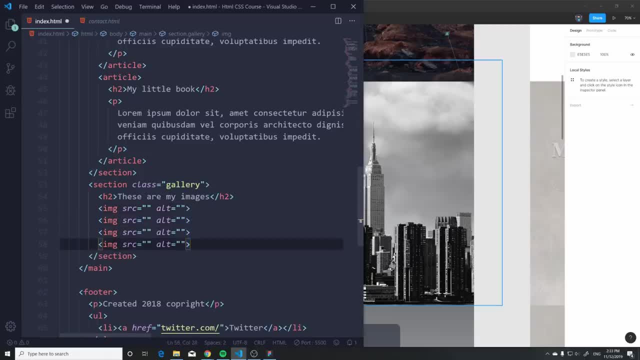 group some things in specific ways. So maybe I want to group some things in specific ways. So maybe I want to group these two images like this and maybe have two more. So I want to group these in different ways than this. I want to maybe manipulate these styling and everything different from these. So what? 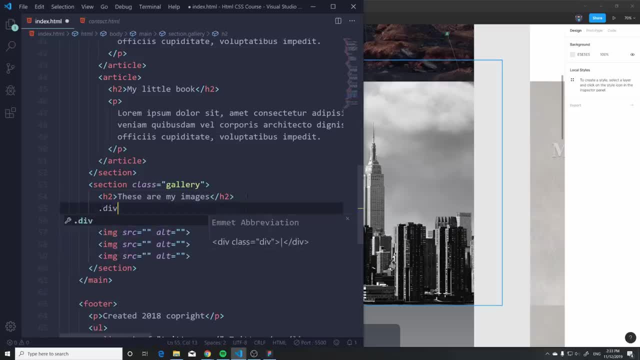 you can do is you can add two divs around these. So let me just add one, Let's say row one, and group this in row two. Or maybe I want these to be styled differently, Maybe I want these to have a black background, or maybe I want to have the avatar, And so I want all these to 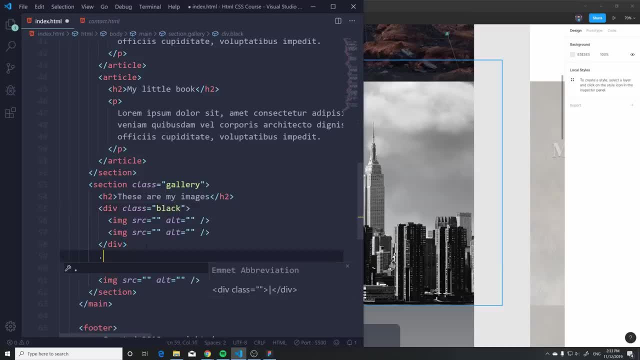 have like a black background. As far as I know, I want all the cover art to come from all the different. I'm going to name these black. and maybe I want to have this on a red background, so I'm going to name these red. So I'm grouping these together just for styling purposes, not really for semantic. 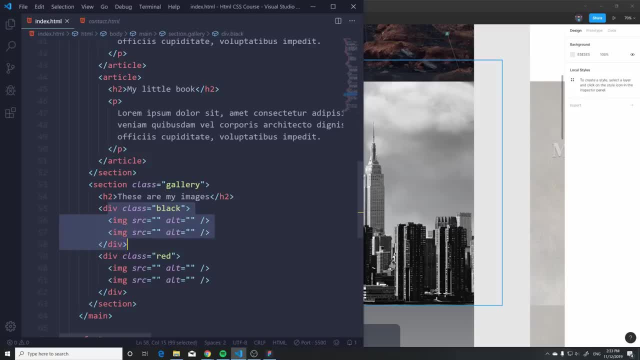 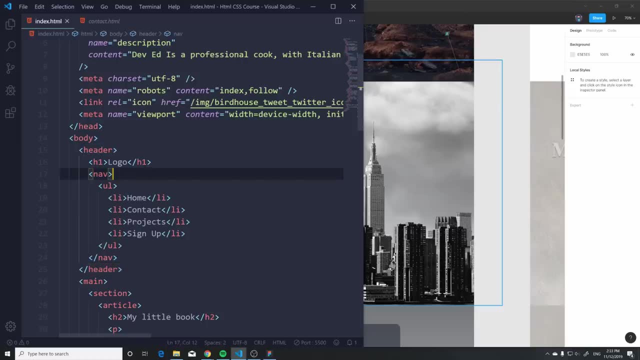 purposes. So these are still important and we're going to use them a lot, but for these big main sections, you should use these HTML5 semantic elements that they provide us. So there we go. These are the HTML5 semantics, and don't worry if you don't get them straight from the start. 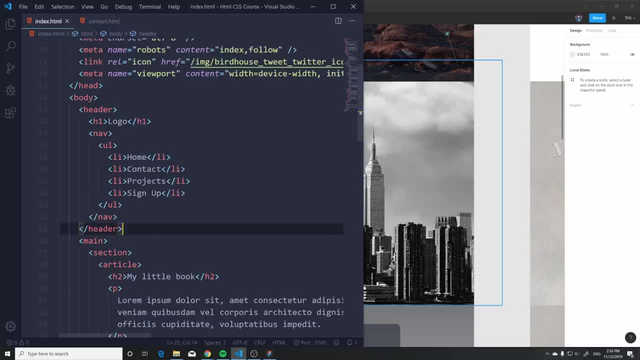 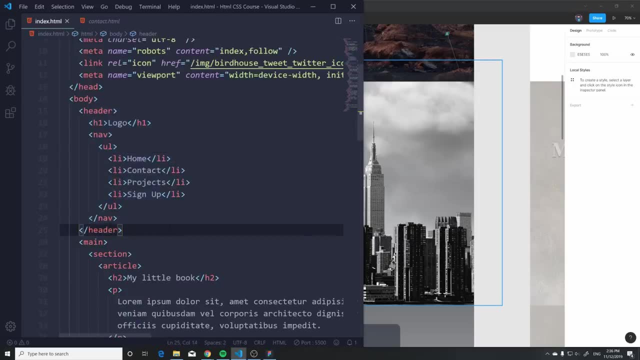 and you don't remember all of these. we're going to practice when we're going to build projects and we're going to reuse them, and it's going to make more and more sense. But don't worry if you don't get them at the first try and you don't know where to place things, because even 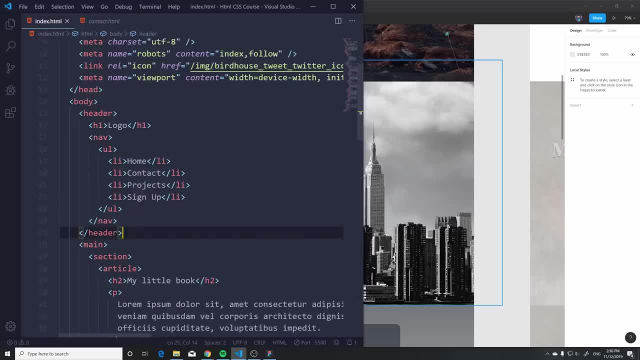 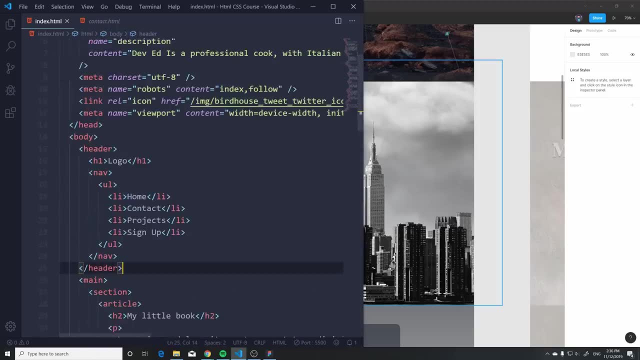 these days, people are still debating what is semantically correct and where they should put what, So don't worry too much about it. But what I want to clarify is that we can also reuse these. So headers are actually. you can use it more times, So maybe in an article you can wrap your introductory. 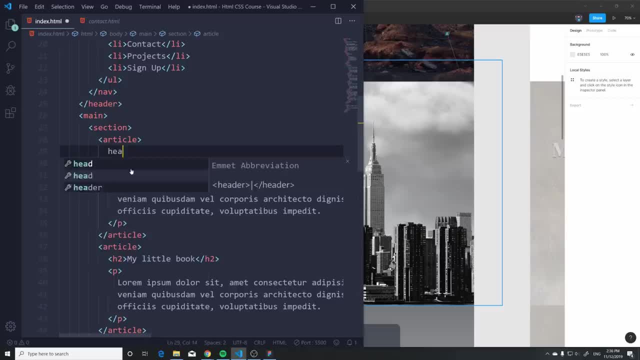 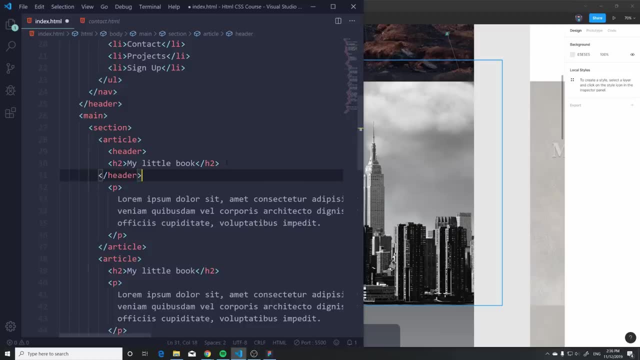 elements inside of a header. So maybe the title here can be wrapped inside of a header and that's perfectly fine And you can do that header. and maybe we can also add a subtitle in here, maybe with a header tree, So we can say: this is a book about love or something like that, And then you 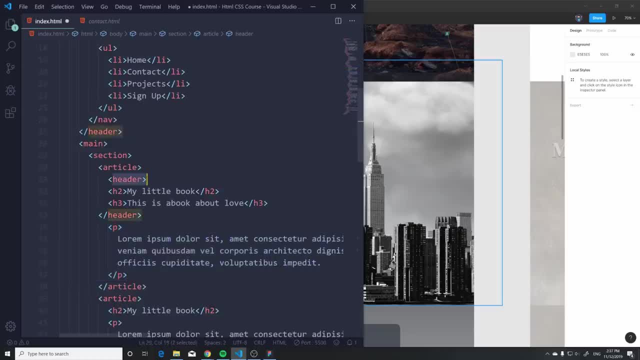 can actually use it more times. So maybe in an article you can wrap your introductory elements inside of a header, maybe with a header tree, So maybe the title of your book is as further dangers to you, or maybe you can ever do the same thing. So we can have your textbooks, we can have. 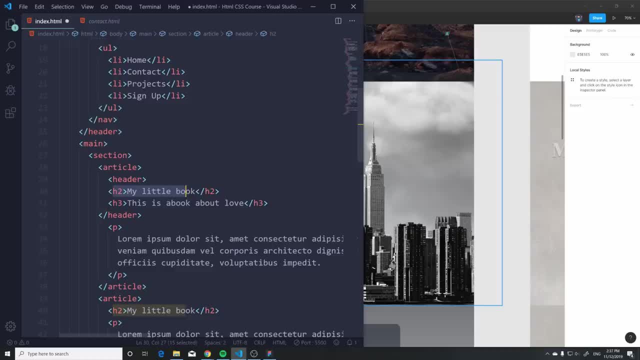 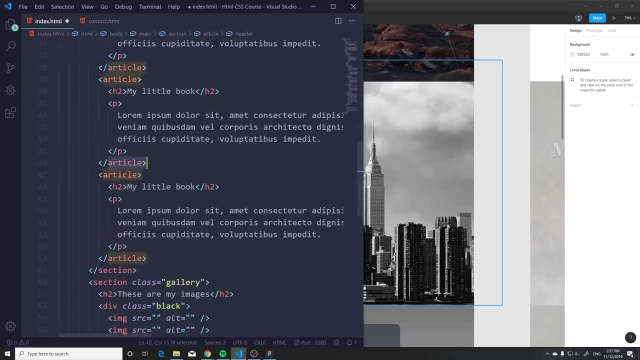 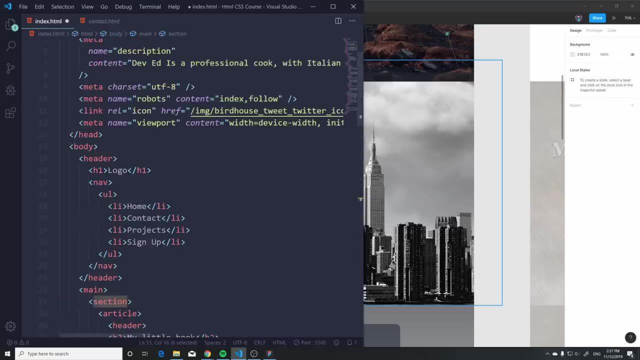 your text and the rest of your content. So you can still use headers just to give information about the title of your article. and here And also, we saw that we can reuse articles as well, we can reuse sections as well, those figures that we saw: Footer: You only have one footer. 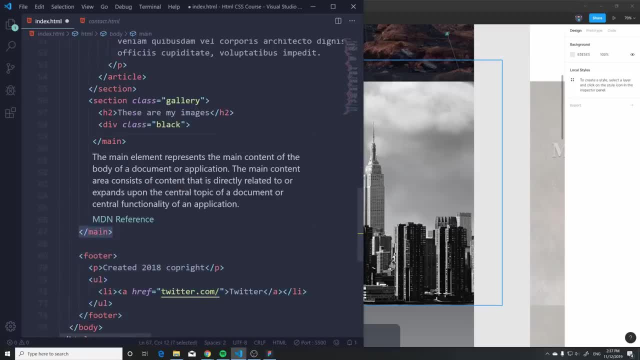 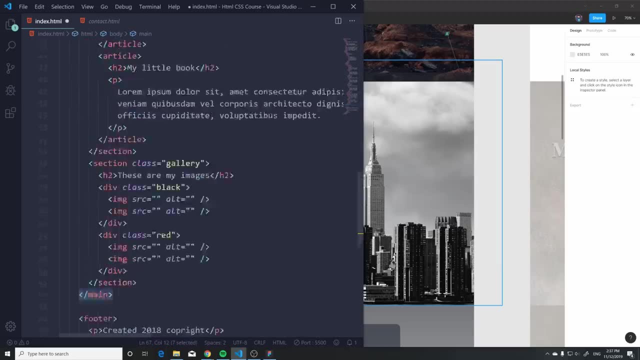 usually, and main can be only used once, and then we also have theafters, So it's not like there's as well to represent the main content of your website. okay, but we're gonna get more practice with this. okay, I'm not gonna go too too, too deep into this and 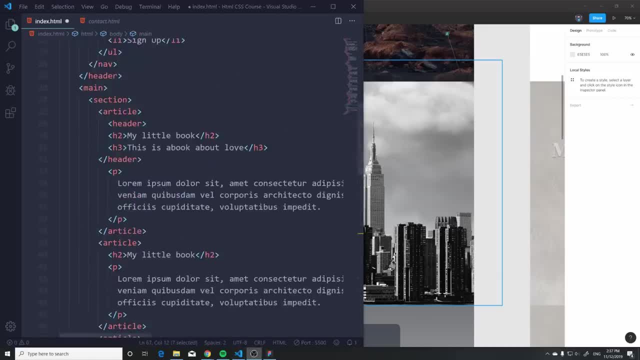 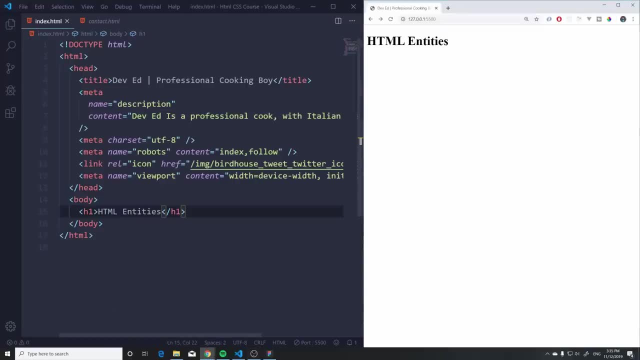 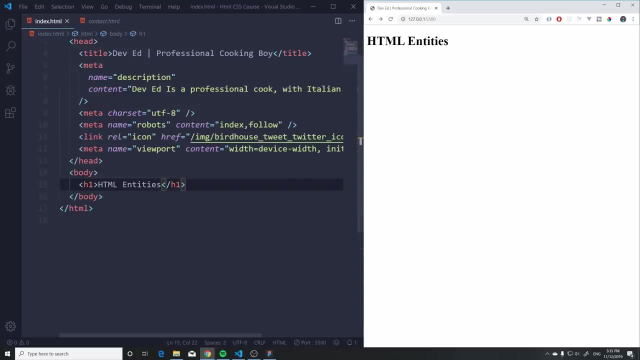 yeah, let's continue, let's keep going and soon the fun will begin. hey, congratulations. you have reached the end of the first section. we have finished HTML and we can start with CSS, and this is where things are gonna get fun in just a bit. so the last thing I really want to cover is HTML entities and this. 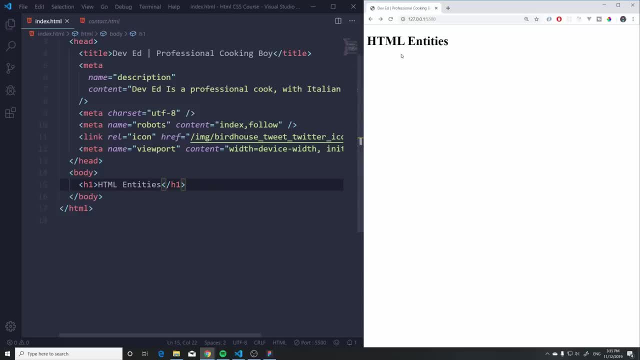 one's very simple it's. all it is is basically characters that you might not have on the keyboard that you want to add in your HTML code, and also certain characters that might break your HTML code if you add it. so, for example, on this HTML entities title, I want to add a lesser-than sign at the end. 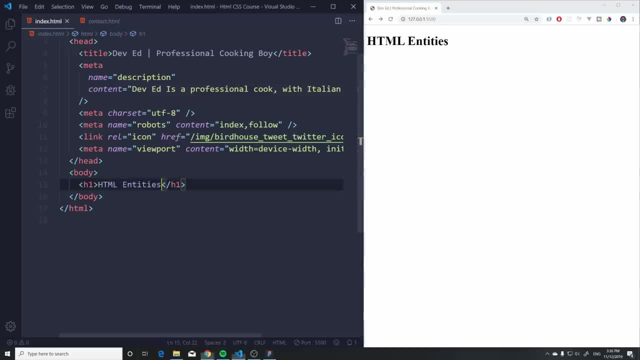 okay, just maybe I just want to add it for some reason. well, if I do that here, it's gonna break the code because this is reserved as a tag. right, this is how we create tags, and the HTML is gonna think that, oh, we're trying to add another tag. 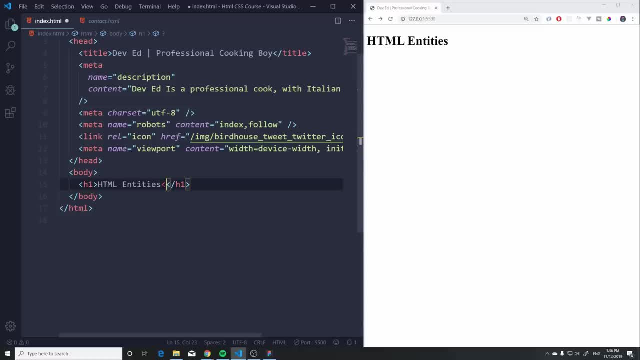 here and it's not complete. that's well. that's why we're getting that red underline. so we cannot do that. we cannot add this tag without messing up our HTML code. so what do we do? we use HTML entities, characters, and you can find this, you can look it up online, because 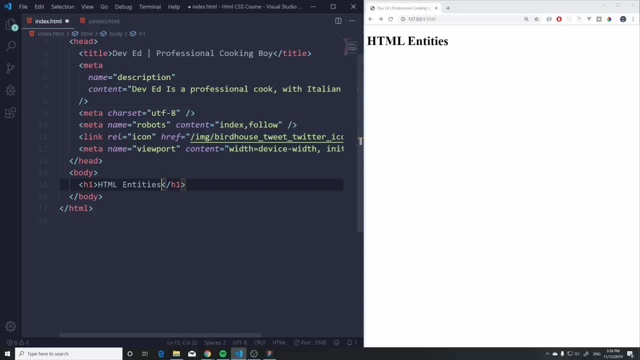 there are certain codes that you need to add here to add those characters. so I'm gonna show you one. here is the character for the lesser-than sign. it looks like this: and symbol, and then you have LT and if I save this, as you can see, hit appears on the screen. so if you want to look for these specifically, 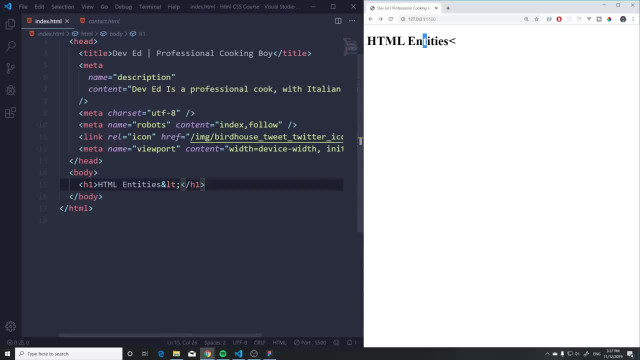 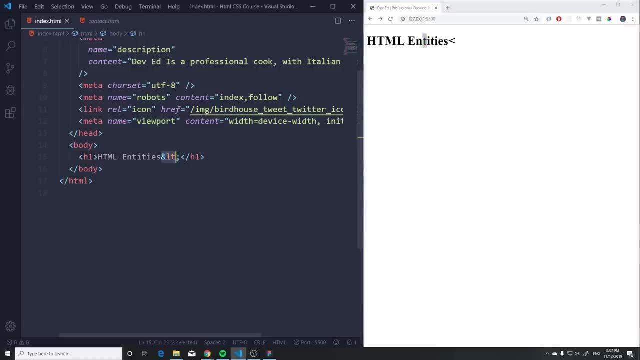 you can just search up a huge, huge list of HTML entities and you can just copy and paste them. You don't need to please don't remember these, because there are a lot of them and there's really no point to it. So a lot of them can start with an and symbol. 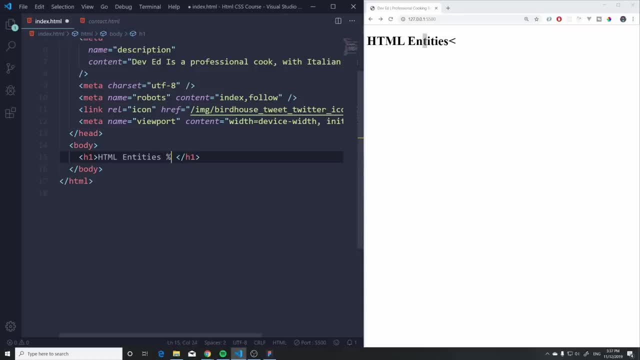 So let me show you. So if I go here, we can do the and symbol. I'm not sure if it gives you some kind of auto correction. Actually, look it does. All you have to do is add the and symbol and then hold control space. 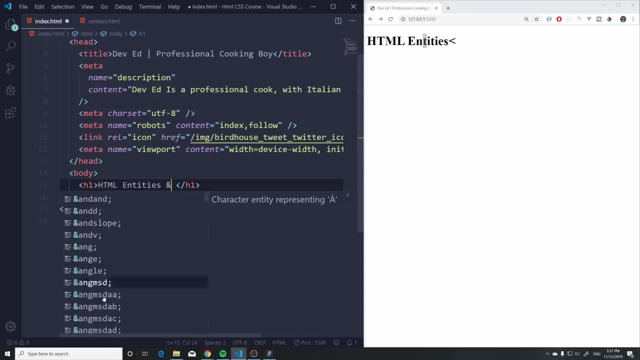 And when you do that, as you can see, it kind of gives you a short description. Actually, some of them they're not even clear, I believe, only if I click on it. So, yeah, okay, so if you go down with your arrow, 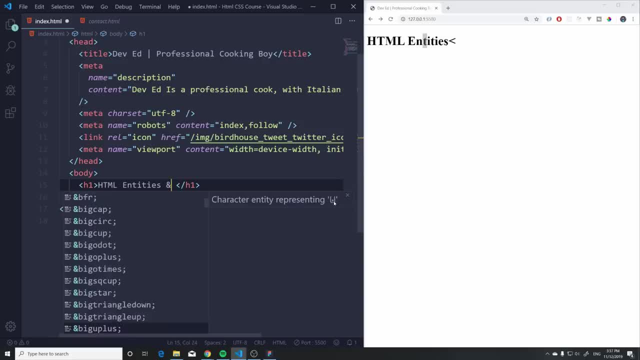 then it displays all the characters, each of them what they mean. So there we go. So maybe you can go through them like this, but I still don't recommend. Maybe I wanna add a copyright symbol. That one is actually very simple. 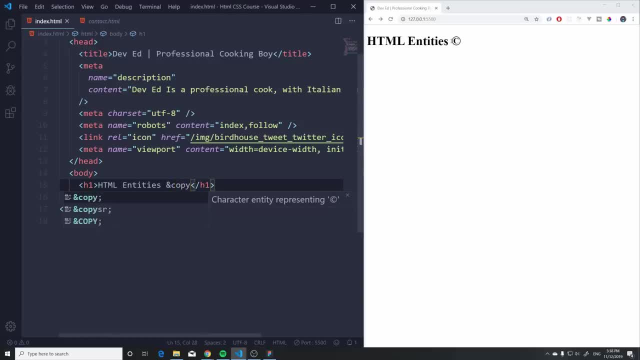 You can just say copy like this and hit save, And there we go, We have our copyright symbol. So very simple. These are HTML entities. If you ever find yourself in need of using a character and it might break your HTML code, then search up HTML entities or special characters. 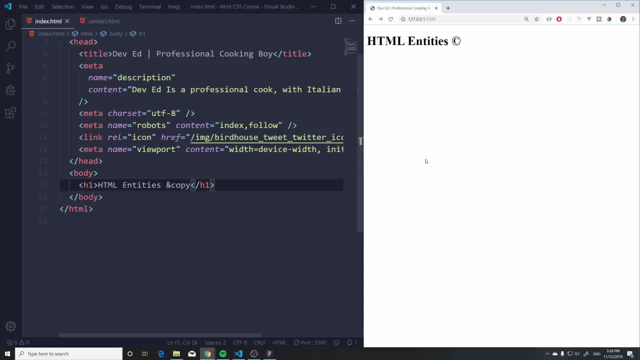 like the copyright sign that you might use on the website, or maybe euro or pound and things of that sort. If you don't have that on your keyboard, search up the code for the HTML code, the HTML entity on that specific one, and you should be good. 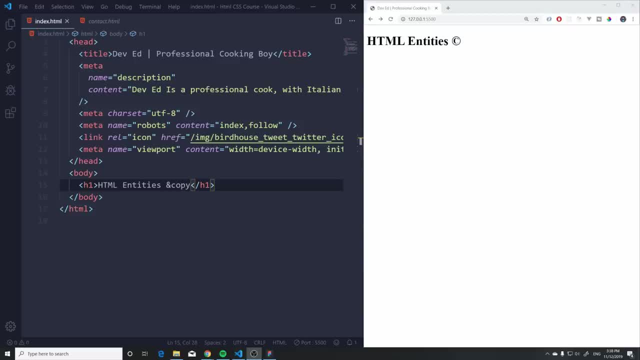 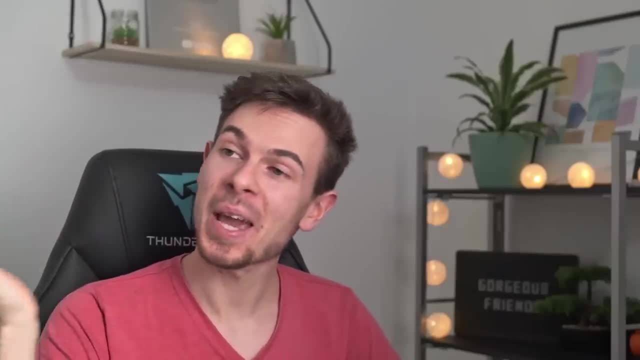 Okay, that's it. Let's have some fun. now Let's start with CSS. It's gonna be awesome. Okay, so we have successfully passed through the boring stuff, as some people might say, because hey, we just have text on the screen. 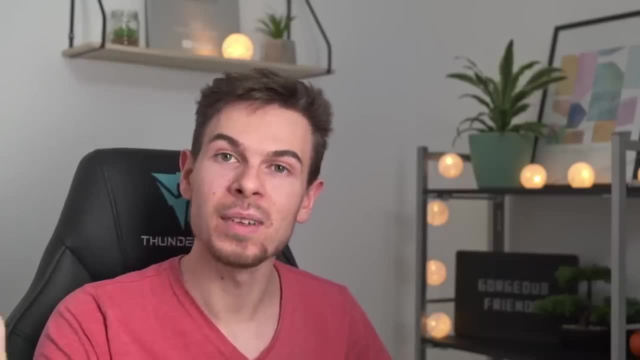 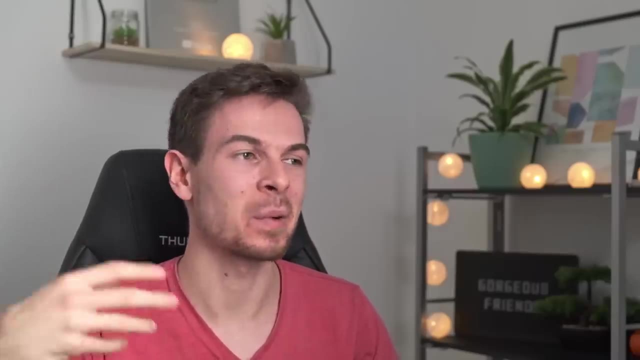 That's not exciting to anyone- Maybe some old people, but let's not say that. So in the next section we're actually gonna take a look on how we can style things, how we can create layouts, how we can make things look pretty. 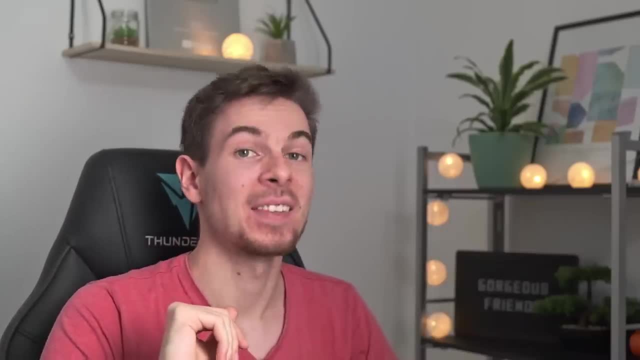 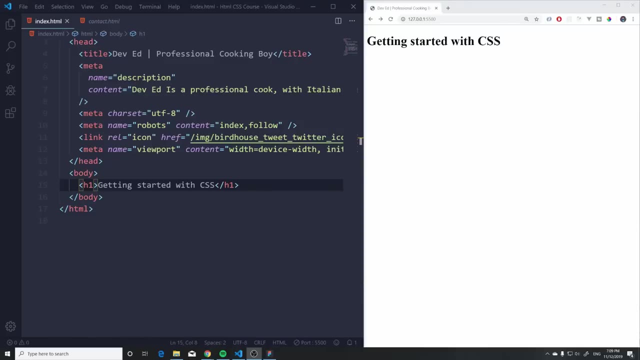 and this is where web development starts getting fun. So let's get going. We have finally arrived to CSS, the exciting part of this course. CSS is just a large monstrosity of a technology. You can do so many crazy things with CSS. 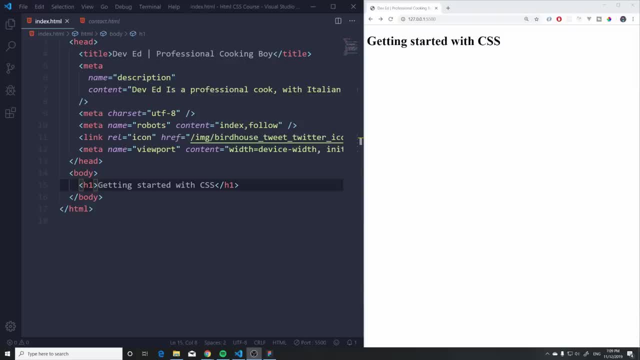 You can start styling. Some people even created animations like full-on cartoons with CSS or like 3D-looking objects, Faking 3D models and just a bunch of crazy stuff. But let's get started. very simple for now, Super simple: just styling this red H1 that we have here. 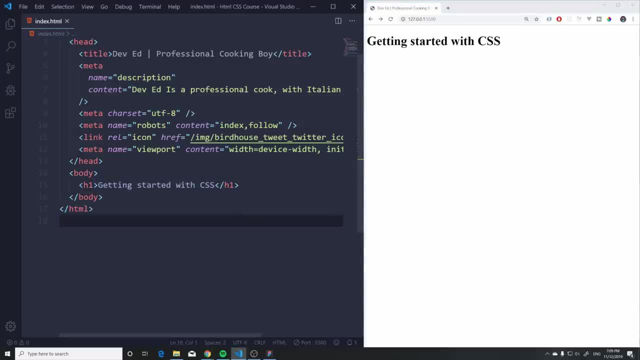 So, before we start, I actually wanna show you a few ways we can connect our CSS to our HTML. So there's three ways you can start styling your HTML. So, first of all, what I wanna do is actually get rid of this contacts and just everything else. 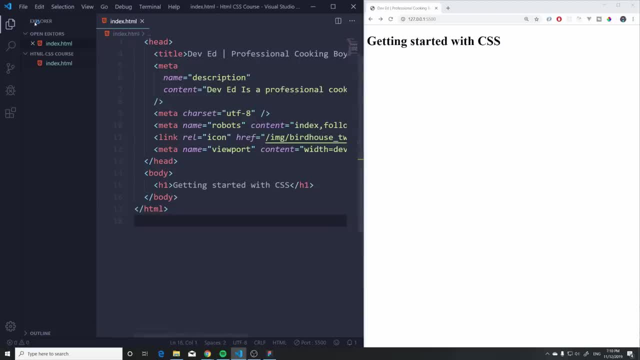 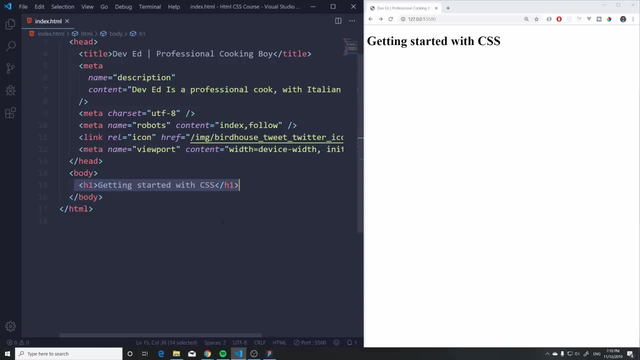 I don't want your message. Windows Goodbye. Okay, So the first method is to directly style the element using an attribute, So I can go directly to the element and style it here. So the way you do that is you add an attribute of style. 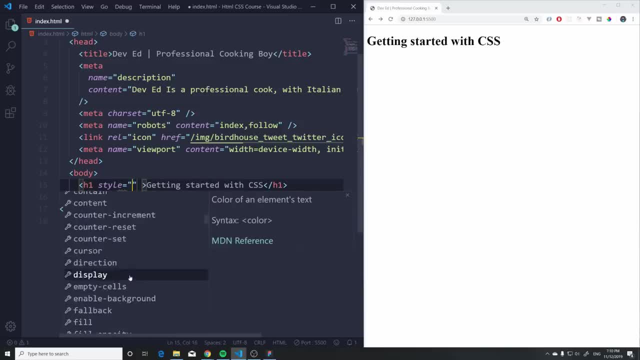 like this, And if you hit enter, you can choose from all of these different styles. The one we're gonna look at is color. So let's do this color and let's choose one here- Crimson, why not? So, as you can see, 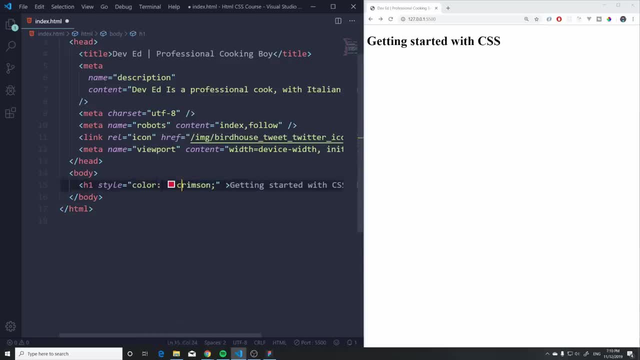 the syntax kind of looks like this: You say color, then you have a colon, then you give it the name, and then you do a semicolon And that's it. If we hit save, boom, there we go, We have our red color. 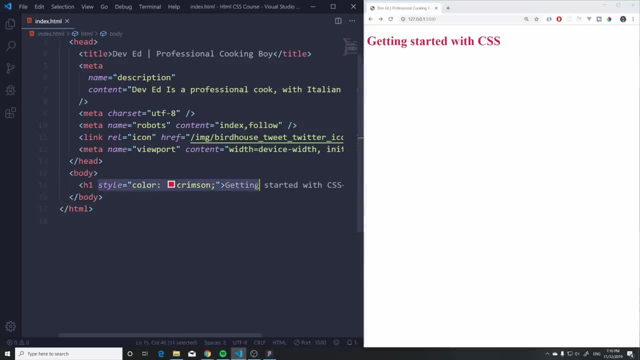 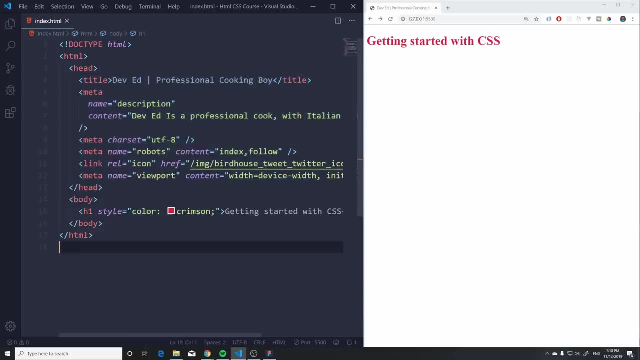 Yay, Awesome, Okay. So is this a good method to do it? Not really. There's two problems with it, I would say. It kind of bloats your HTML, It adds unnecessary things in here and it just makes it harder for you to read. 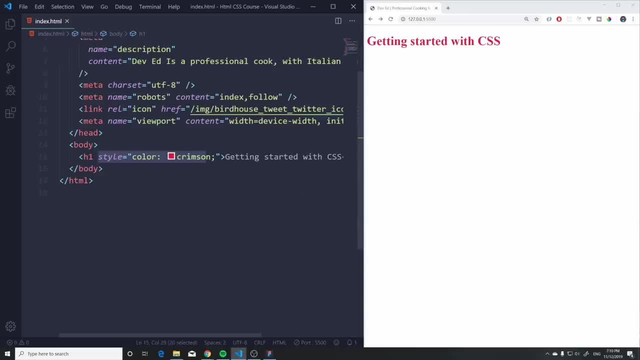 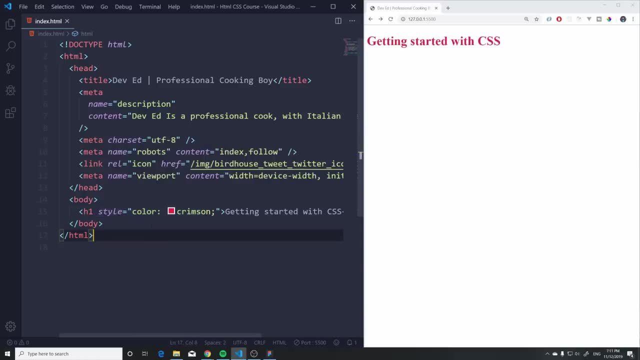 So I wouldn't really recommend this method. And also, if you wanna style multiple elements, you would have to add the style tag to all of them, and it just makes it a bit more cumbersome. So we are not gonna do that. Let's get rid of it like this: 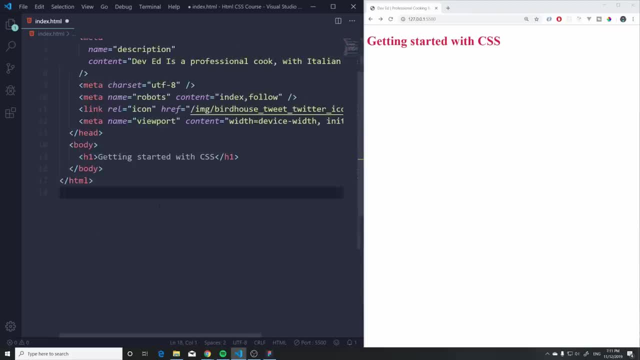 Perfect. The second way you can do is you can go all the way down here and you can add a style tag like this and you can hit tab okay And in this style tag you can start styling your CSS. So I'm gonna show you. 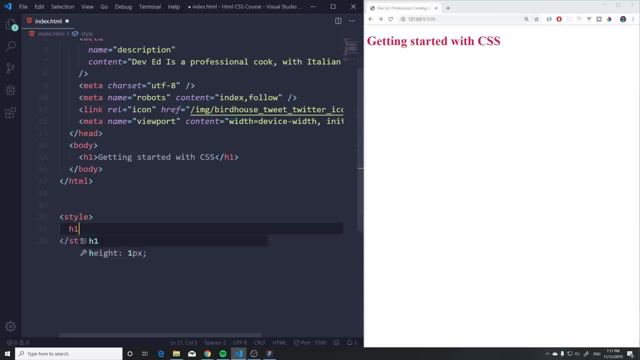 a quick way we can select it, but I'm gonna cover this in a later video. Here you can do something like this: color red, All right, hit save And, as you can see, we have the color red. This is a bit of a better way. 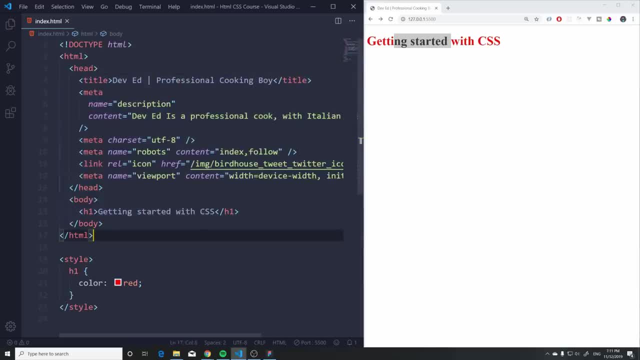 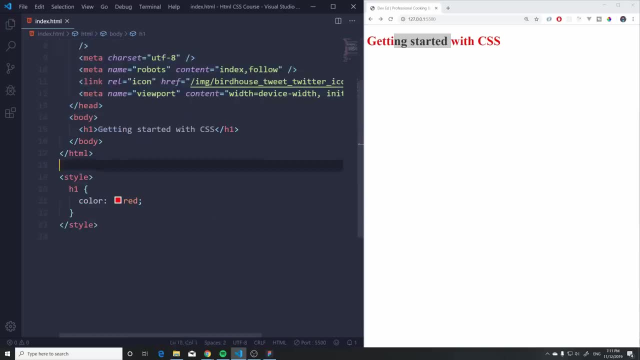 just because you're not really adding anything on top of the HTML elements. but it's still not a super nice way because we're still adding both HTML and CSS in the same file, So it can get quite large after a while and it's just not as nice. 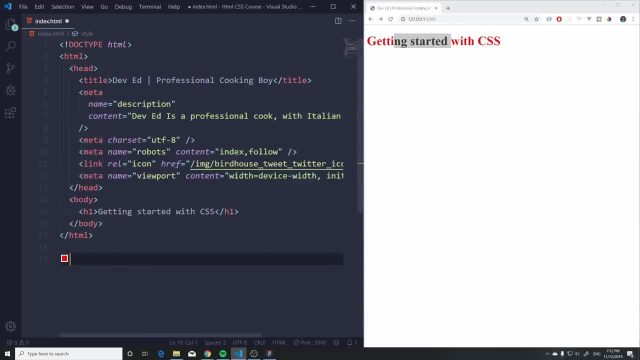 So the best way is to remove everything and just keep your HTML in here, Nothing else. You just have your HTML in here and we specifically create another file for that. Typically, let's go here. You're gonna see a file named stylecss. 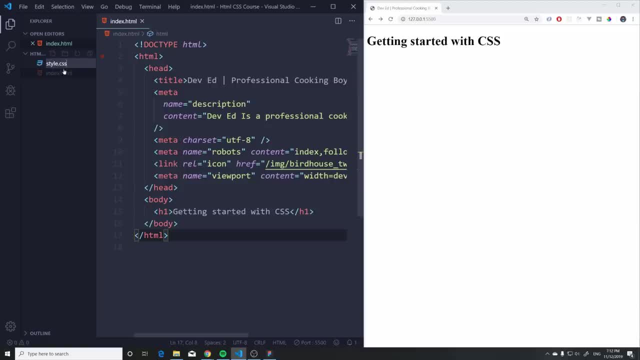 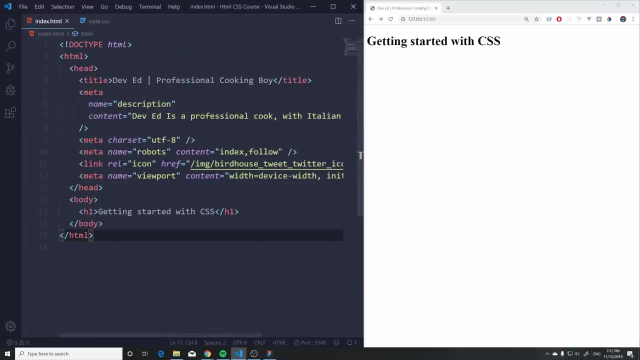 That's what people most commonly use, So let's name it like that, okay? So stylecss- And I've actually kind of covered this and it's a bit of a spoiler, but we kind of did it the same way with the link. 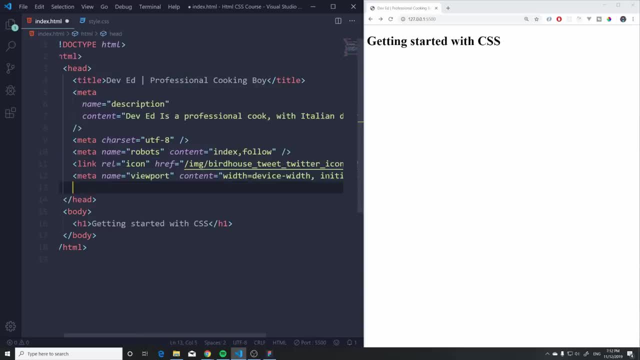 So the link here, so the icon. all we have to do is literally just come here in the head and say link, hit, tab, and the relationship here is gonna be style sheet. So we clarify what kind of file we wanna attach here in the header, in the head. 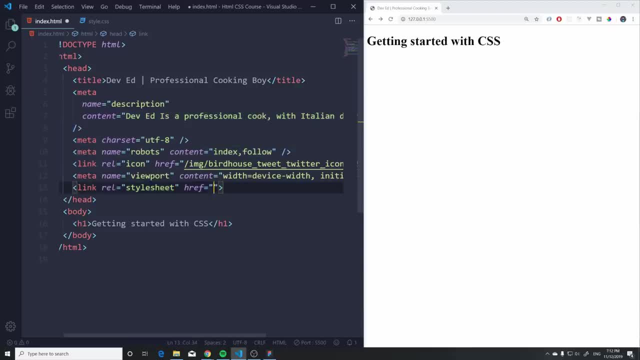 My apologies, not header, And the href is just gonna link to the file. So I can say slash, stylecss And literally that's it, So simple. So let's move on to the next video. So let's move on to the next video. 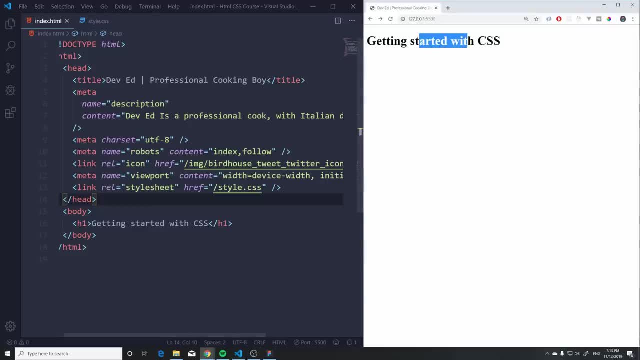 So let's move on to the next video And we're gonna see how we can mess around and make this fun. Next up, I wanna kind of show you how we can select multiple things on this page. I wanna show you the syntax and the way these selectors work. 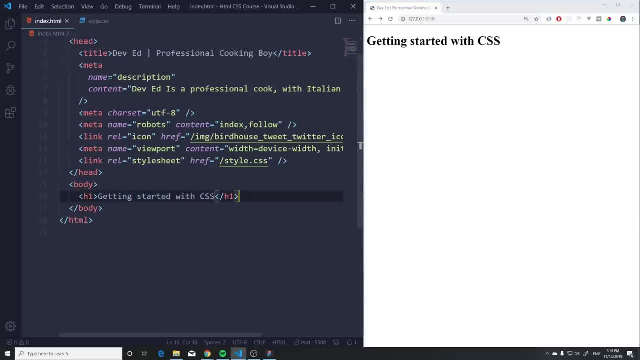 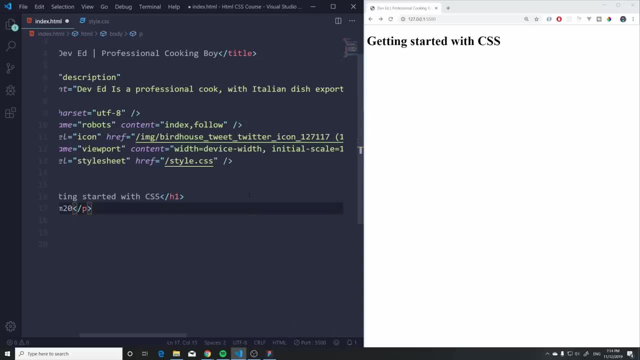 So let's get started. We are gonna keep this h1 for now, but we're gonna also add a few different elements. I wanna add a p tag here. It's gonna be some random text like this. Actually, let's just keep it short here. 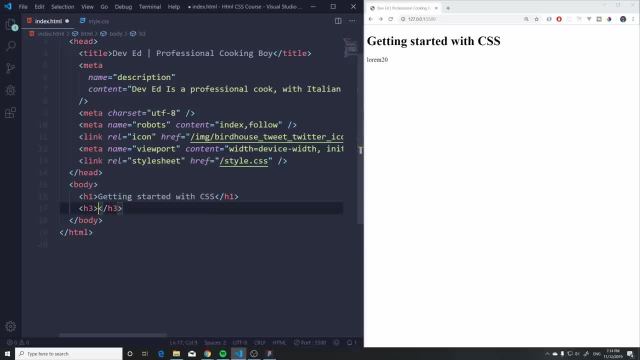 I don't need anything too crazy. Actually, let's just add a h3 because that's a bit easier to see. This is gonna say: mom is cooking the good stuff, like that, And I also wanna duplicate this a few times because I wanna show you a few things. 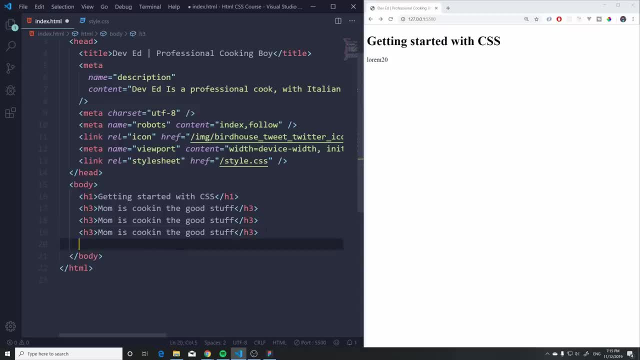 So we have this three more times and let's also add maybe an anchor tag here. If I add this, hold on, let me change my language again. If I add this hashtag here, it just basically means that this link is not taking me anywhere. 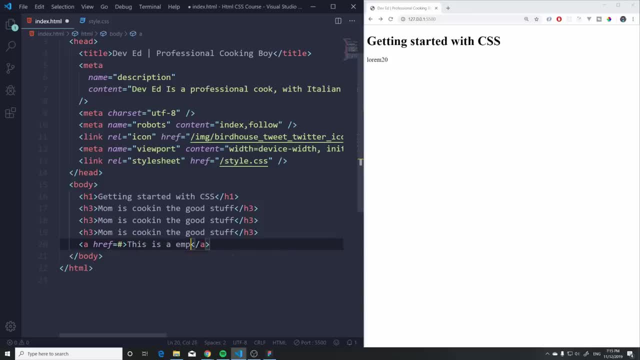 So here I'm just gonna say this is a empty link. Okay, I just wanna have a few things here so we can start styling. okay, I'm gonna add a class to this. I'm gonna say: let's name it firsttitle, like this: okay, 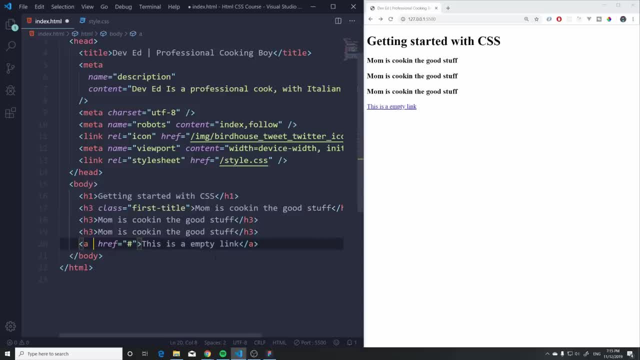 And on the anchor tag I wanna say id. we're gonna throw an id, I'm gonna say id on this And the id on this is gonna be YouTube link like this: Okay, and we're gonna hit save. So when we go to CSS here, 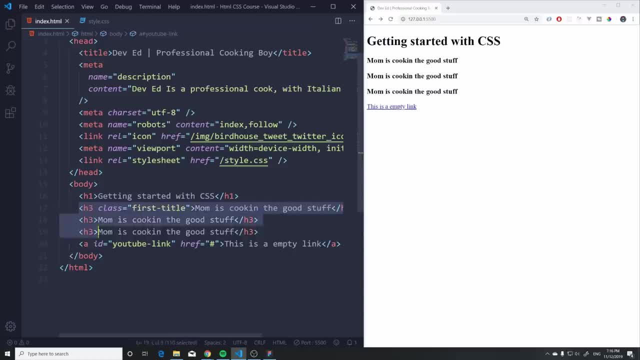 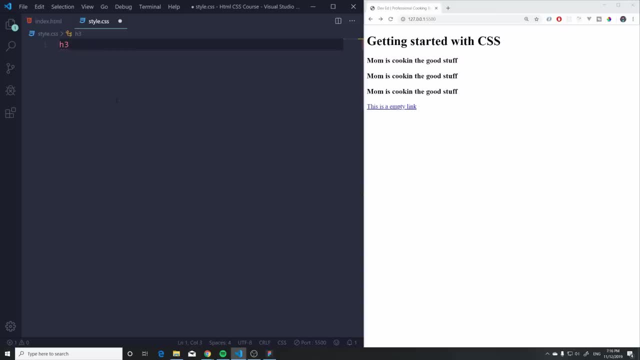 all we have to do to select something is write the name of the element. So that's one way we can do it: h3, all right. So we write h3, the name of the element we wanna pick, and then we do these curly braces. 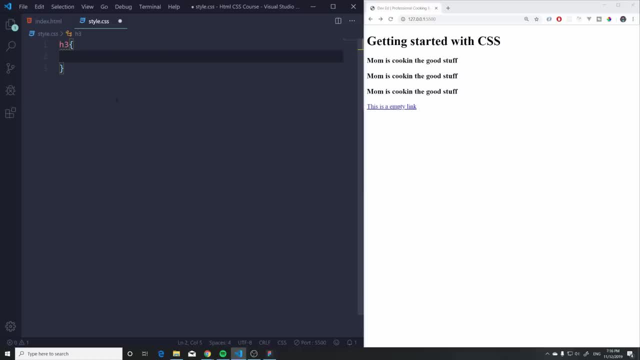 Okay, the squiggly wormy curly brace. I sometimes forget. In case I say squiggly worms, that just means curly braces. okay, So we just open it up like this, and all these tiles that we add will be in here. 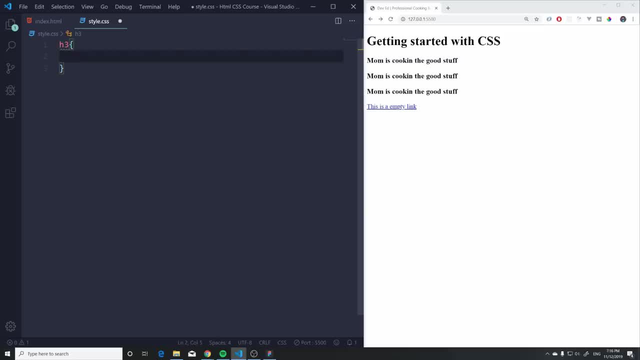 So everything that I wanna add to this h3, this header tree, will be inside here. So let's do the color, because we did the color And we can choose a color like this if we want, and hit save And, as you can see here, 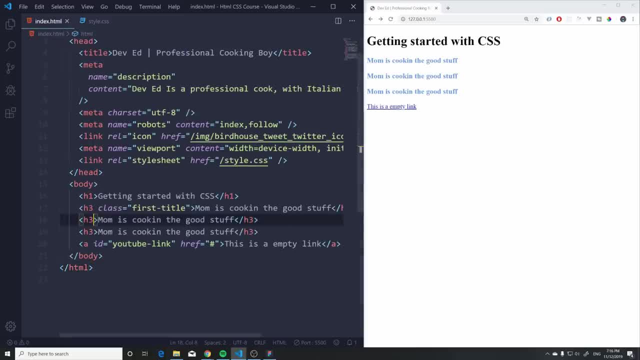 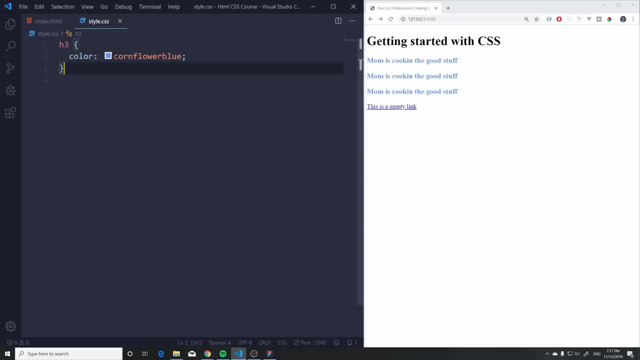 the syntax is kinda like the same that we did inside here when we styled it with the attribute is just: you say color or the name of the property you wanna attach, and then you do colon, you say the name and then you end with a semicolon. okay, 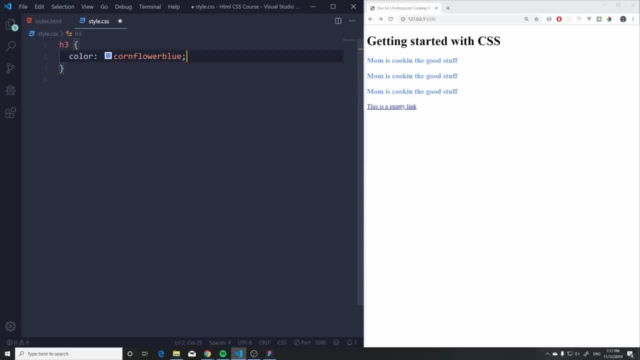 So now we can add more things in here if we want. Now you don't necessarily need these names. You can also color pick. choose one with RGB, like this. So VS Code has this awesome thing, So that's very cool. 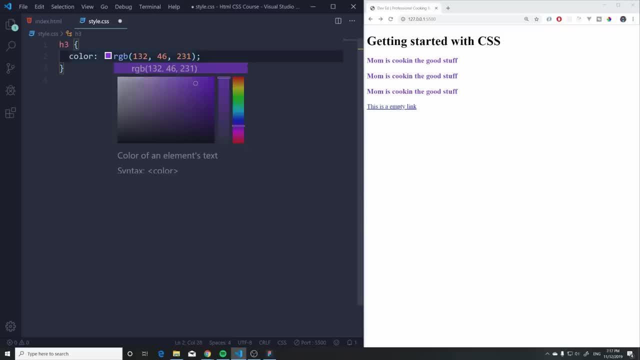 Let's go down here something that we can see a bit easier, maybe a bit darker. We can use RGB, and we can also use hex like this. I don't know what this hex means, but it's probably not a color. 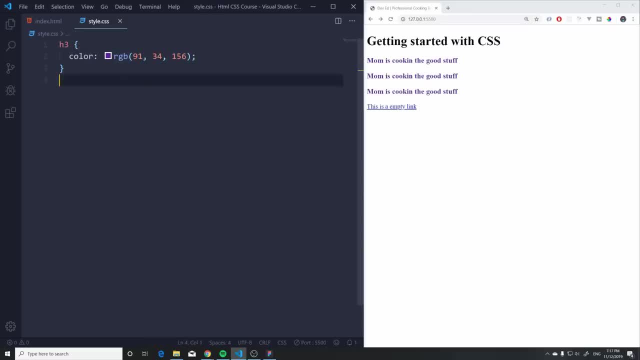 But anyway, let's get rid of that. So, as you can see, we can add it like this. So when we use it like this, we just say h3.. Well, all the h3s on our page are gonna get this style. 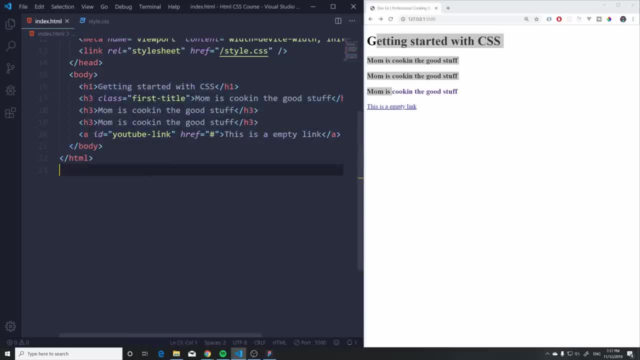 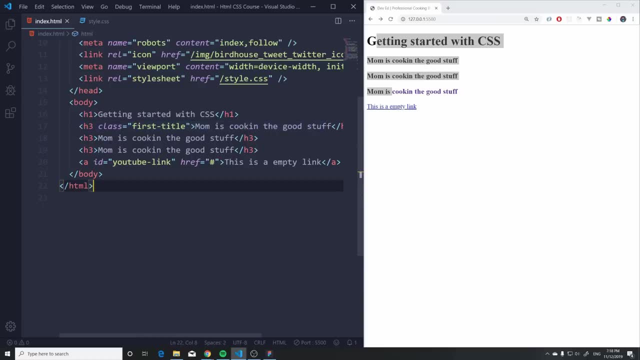 So, as you can see, everything in here gets the style All right. but what if I wanna do something specific? So maybe I want this h3 here, the first one. Well, we can do that by just using the class, So I can say: first title, all right. 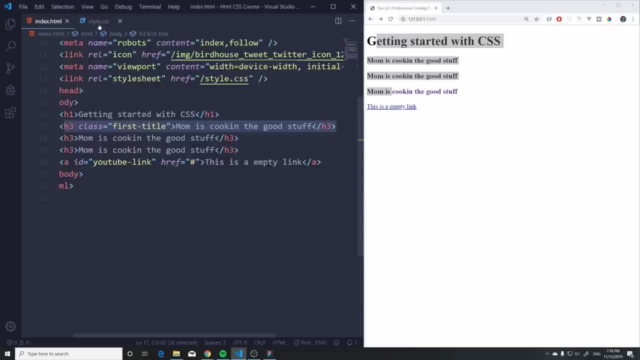 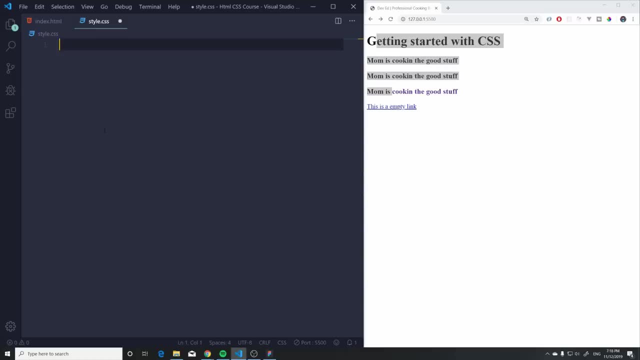 I'm targeting directly this element. This is the only thing I wanna style. So rather than doing it like this, I can just get that class. And the way you can get classes in your CSS is you just add a dot. okay, Just a dot. and then you say first title. I believe it was. 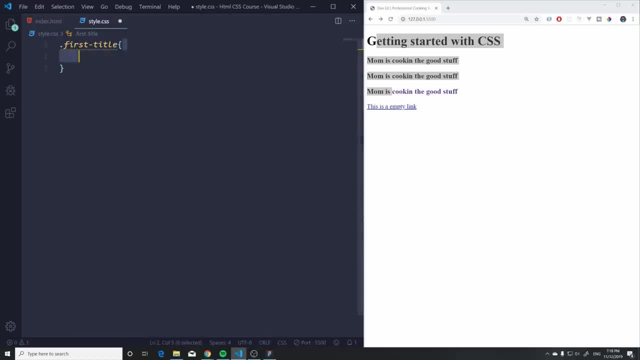 And the same syntax applied with the curly worms, And you just write your color- color red- Hit save and I'll take a look- Only the first one gets changed. So when you're applying it like that, when you're getting one specific element, 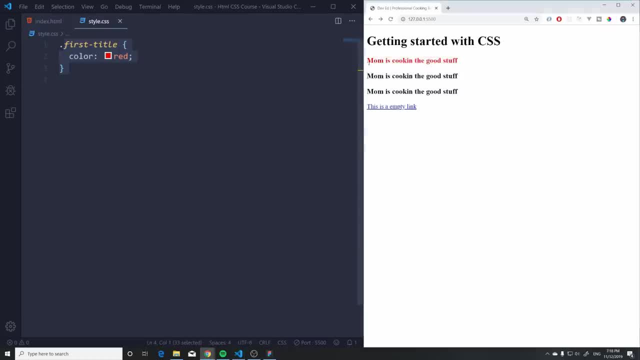 because this is the only one that has a class on top of it. well, this is the only one that's gonna get it. okay. So this is how the syntax works. Let's also check out the one with the id and the way you can select an id. 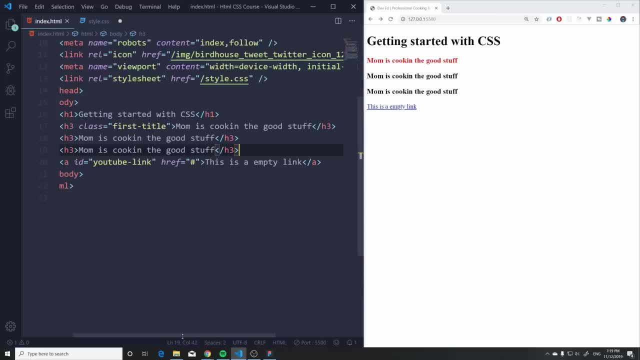 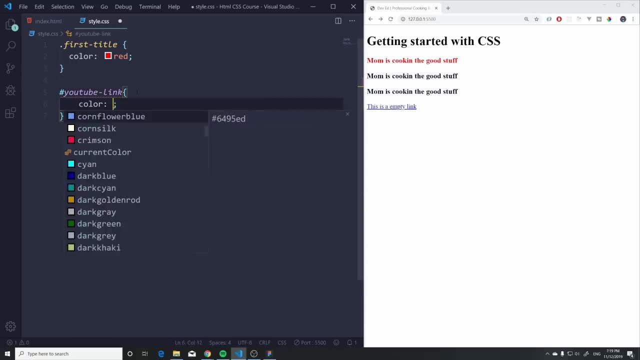 is by adding this hashtag. okay, And by doing this hashtag you can just do YouTube link again and that's gonna work just fine. So we can change the color of this to black, because the default is gonna be that blueish color. 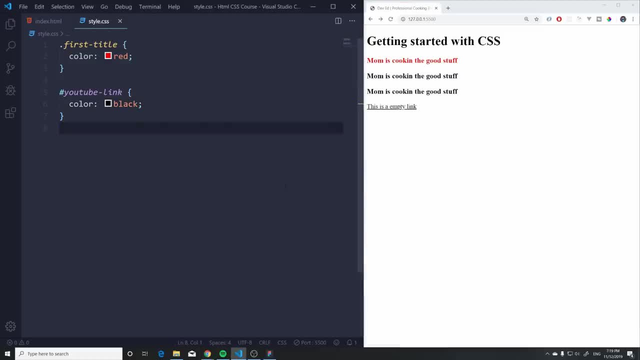 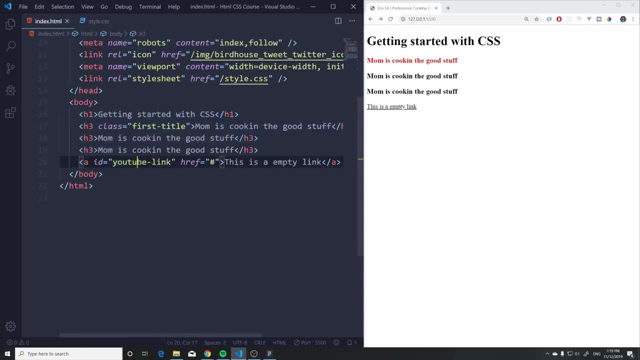 So there we go, everything works fine. And the next video we're gonna get more into, more specifically into the specificity, how we can select specific elements, what we can do with specific elements, and then we'll get to the next video. 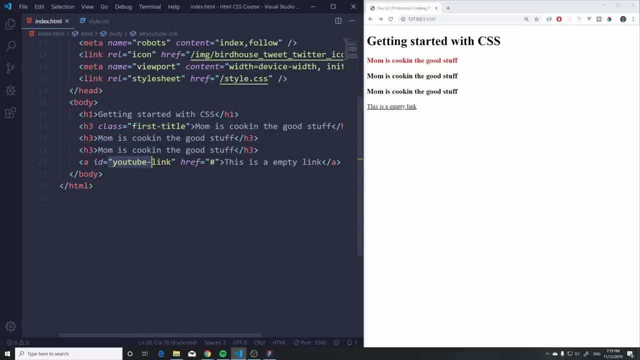 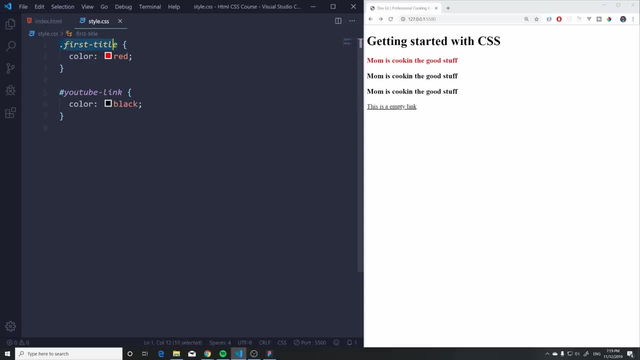 So there we go. everything works fine. elements: the importance of class and id. how does it prioritize, what style it's gonna get, and things of that sort. so this is just kind of the syntax on how you can select elements. you have three, so you have selecting the element directly. you can do it with a class or this is. 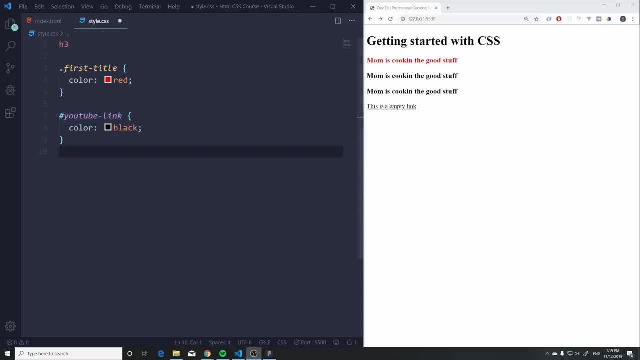 how it looks like with the id. okay, so let's get into specificity and some more tips and tricks. okay, so, before i get into the specificity of, like what's more important- class or the normal selector or which id like, how does css know what to apply where? before we get into it, i kind of 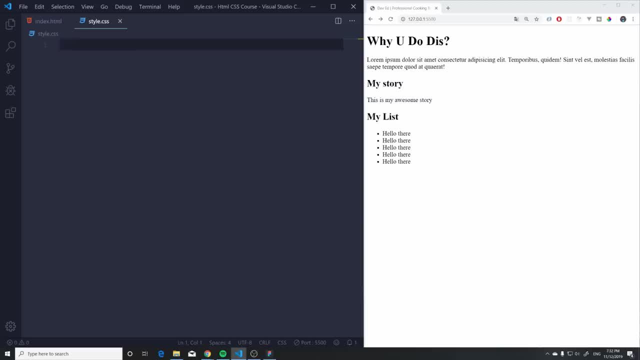 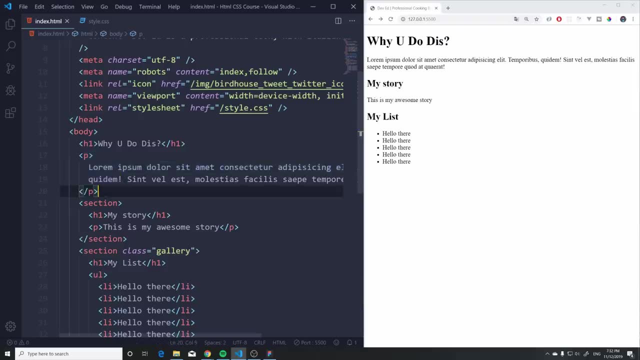 want to show you a few selectors that are very commonly used, so i added a bit of text here. i just added one, each one, a paragraph here. these are not contained in anything, okay, they're just general here. this is just a little bit of text here, so i'm just going to show you a little bit. 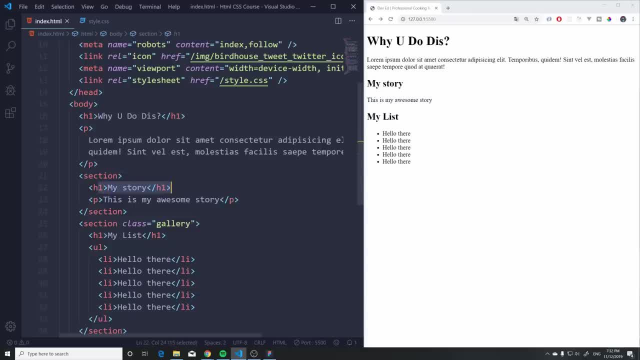 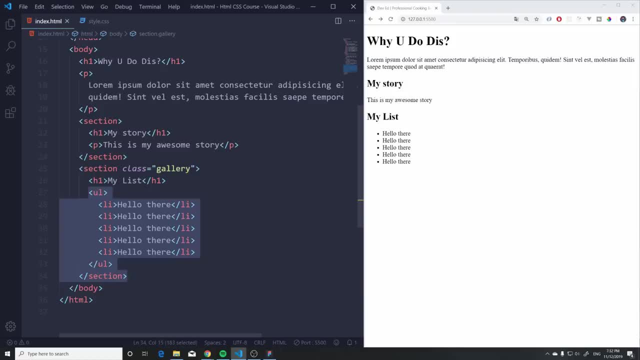 for example purposes. we have a section here. here i did add a h1 and a p tag. then we have a section here that has a class on it, and then a h1 with a ul and an li. okay, so the first one we saw is just: 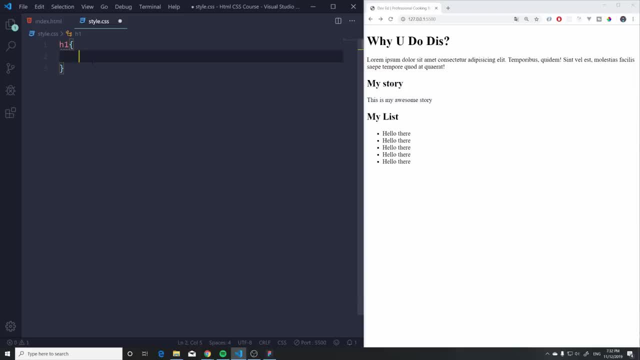 selecting h1 like this. now, the problem with this is that sometimes we just want to style one h1, all right, maybe just this one. but if we just select it generally, like this, we just say h1, then basically what css is going to be like is: 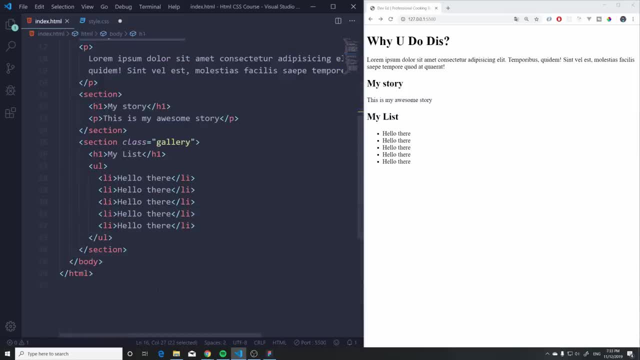 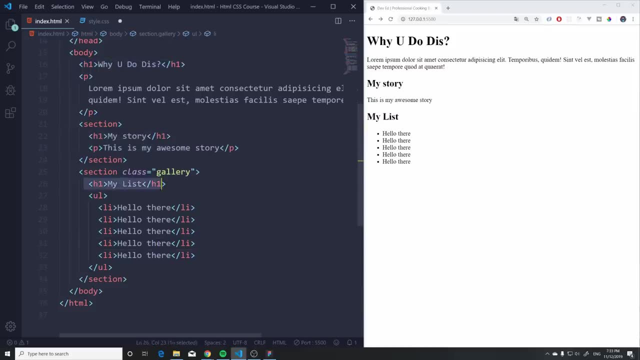 oh, okay, i'm going to look at all the h1s on your page. so it's gonna look at everything. it's gonna analyze it up. there's a h1, okay, so i'm going to style that: hey, this h1 and this h1, okay. so if we add a color of red here, i don't like red, i want cornflakes blue. 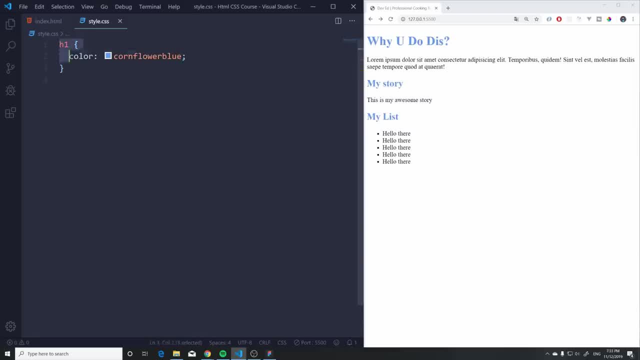 oh, it's cornflower, okay, never mind. so it just styles all the h1s, okay. this is a very, very general select selector. sometimes you might want to do this, but a lot of times you might want something specific. These are generally good. again, when you want to style all DH1s in one. 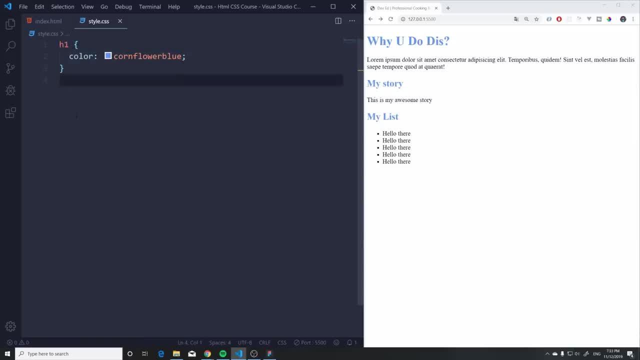 specific way That can work. or maybe you want your paragraphs to look in one specific way, so all of them. Then this is fine. The general selector can be very good. Other times you want to do something more specific. So how can I select this if I just 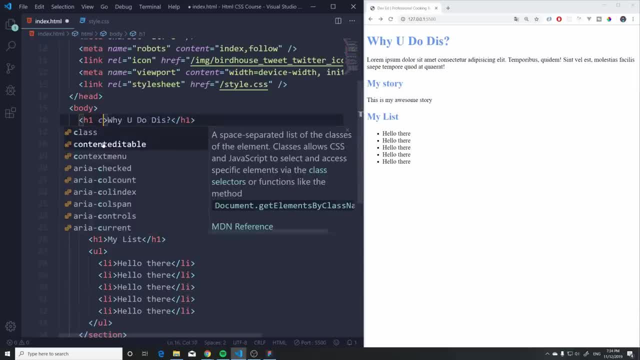 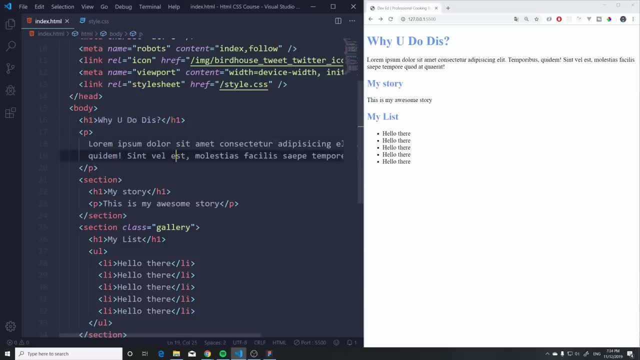 want this to be selected on its own. Well, I can either add a class on it or I can add an ID on it, depending how important and unique this is. If it's something very unique, like a logo, then I'm going to add an ID. If it's something more basic, then I can add a class. if I just 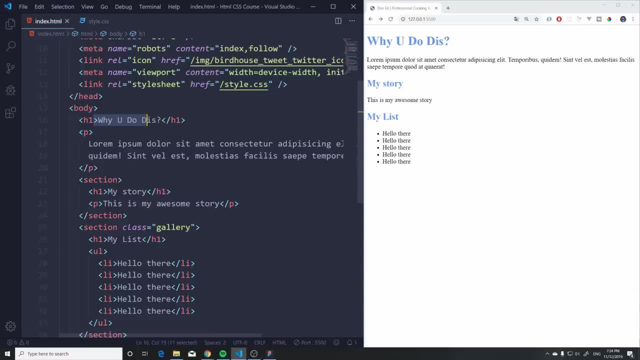 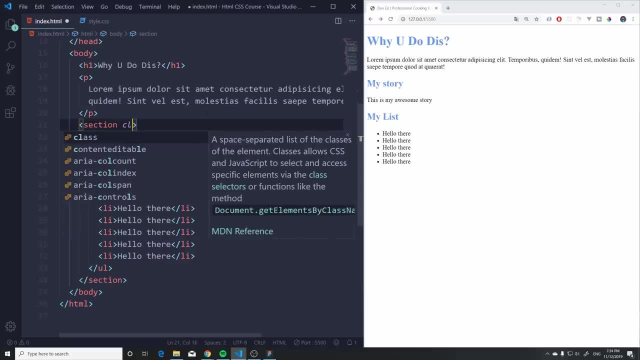 want to select it for the sake of selecting it and styling it. But sometimes you might have one here, like in this section, and this section might also have a class on it. I apologize, but not necessarily, But for this one let's just add a class of. 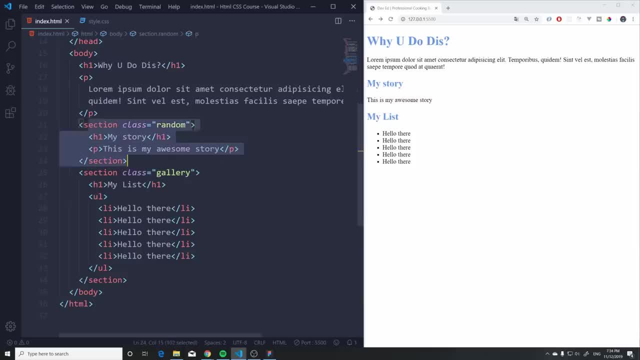 Let's just: This is the random section. okay, Let's name it a random section that we might have on the page. Sometimes, when you might just have one here and you want to select it, you can actually access that with the section. So take a look, I can actually chain together multiple words here. 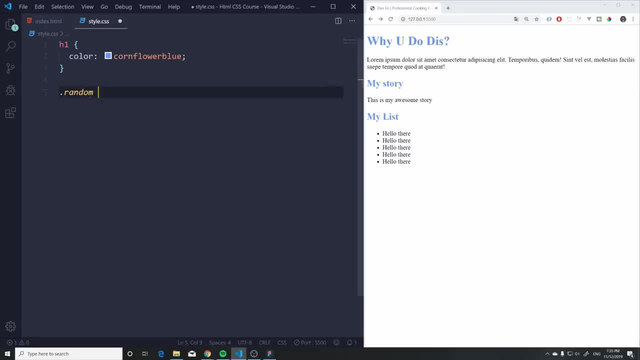 I can say: I want to get that random section and in that random section I want to style the H1s. Okay, so I just write the class and H1.. Okay. so the way CSS looks at this is: okay, let me get all the H1s. It looks at all the H1s and then it's going to be like: okay. 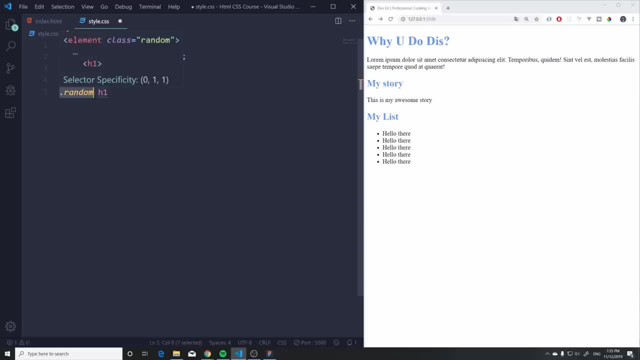 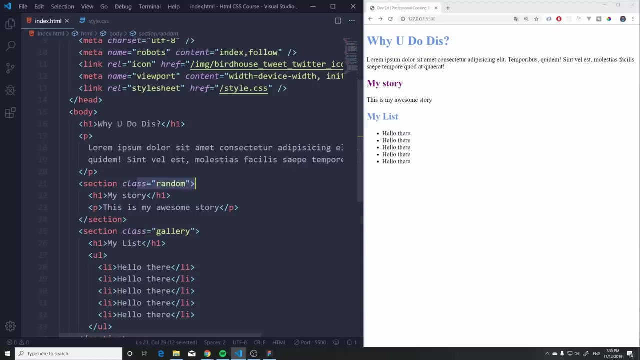 but only the H1s in the random class. So now, if we add a color to this- let's do dark magenta- then it's only going to style that one. As you can see, only this one gets styled, because it takes a look at the random class and only the H1s in the random class. Now, obviously, 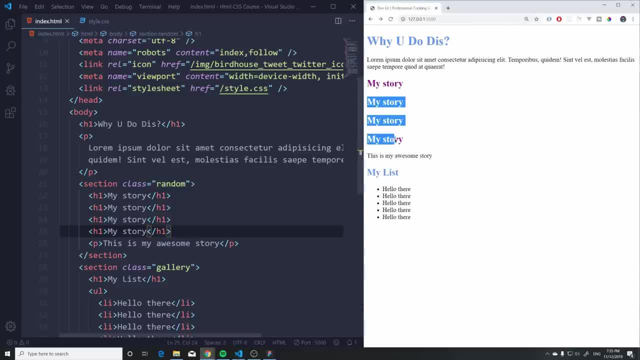 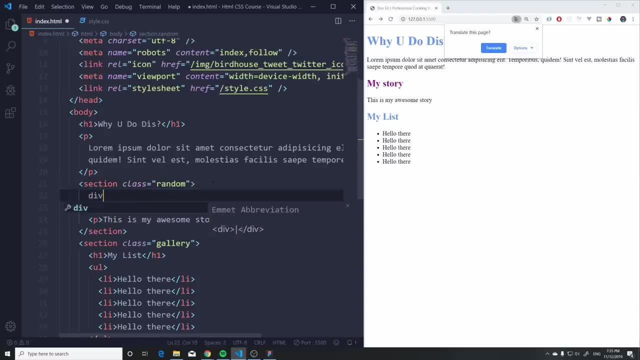 if you have more H1s in this random class, it is going to apply to it. Sometimes you might want that, Sometimes you might not. It kind of depends. Sometimes you might have divs wrapped around these like this, to avoid running into that issue. 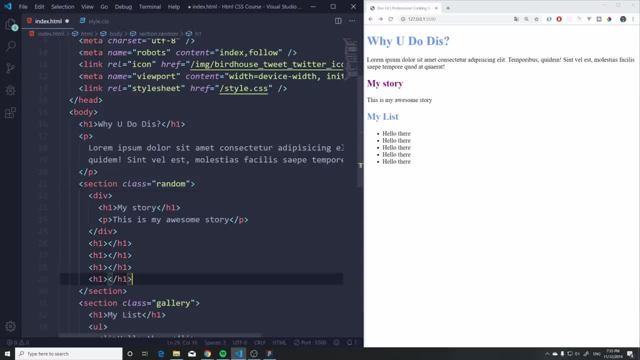 and then you might have multiple H1s here. Then you would select the div and the H1, or you might have a class specifically added to this, So main title maybe or something, and then you could select main title, H1.. So it kind of depends on how your 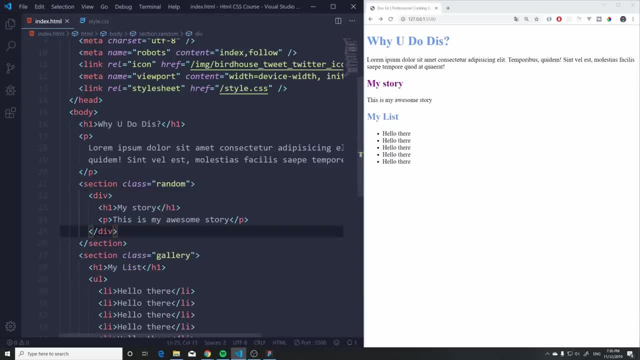 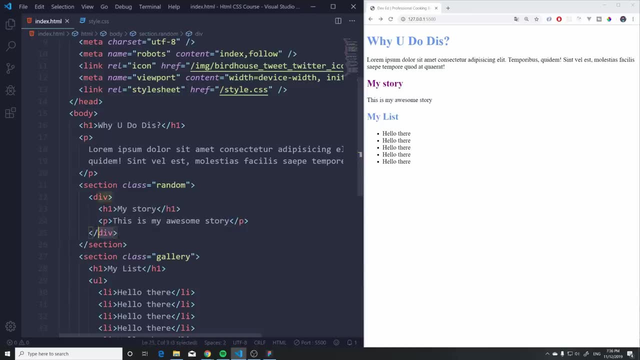 HTML is going to work. So if you have a class specifically added to this, you would select main title H1.. So you're going to get most of the experience out of this when we're actually building out some projects. Okay, But those are a few ones. 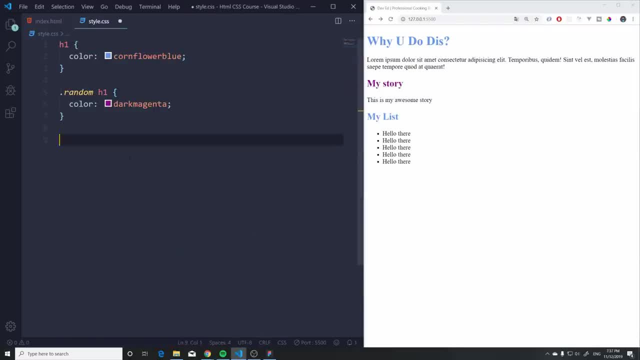 Another selector that I want to show you, and that is the star selector, And all this does is it basically selects everything on your page. I'm going to show you a new property here, which is called font-size. This just changes the font size of everything that you have on the page. 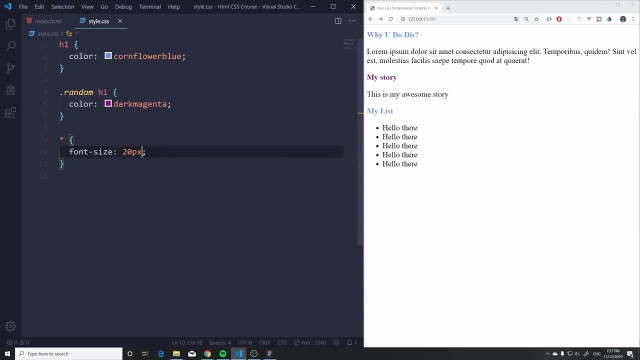 So if I go to something like 20 here- 20 pixels- it's going to change every element to 20 pixels. So it looks at everything. H1, P section. I don't care, I'm changing everything. So this is the star selector. This is greatly used, if you maybe want. 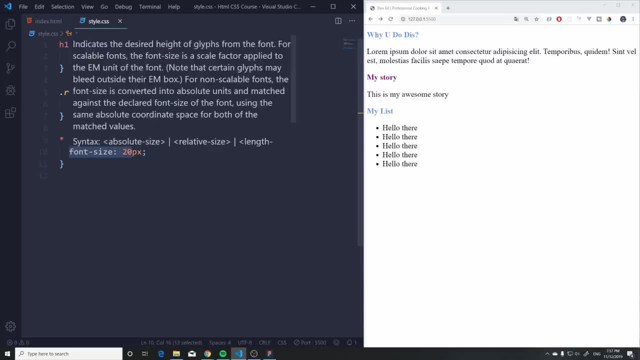 to get rid of some basic styling that is usually provided on elements, So as you can see, these spaces that the H1 has and the paragraphs and things of that sort. sometimes you might want to just get rid of everything, because every browser kind of behaves differently. 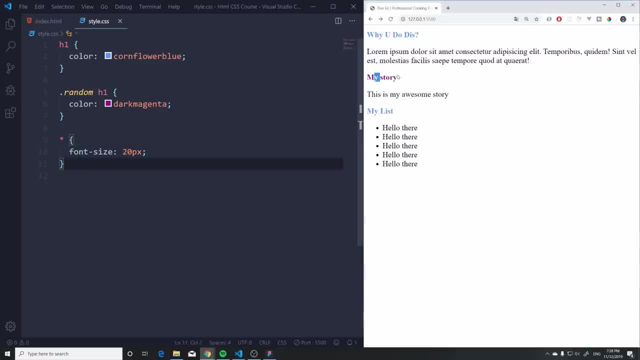 So what you would do is you would remove all these spaces and everything and then you would add it on your own where you want just to have a bit more control. So this can be used greatly, and it is used actually in almost all projects. Let me show you two more selectors that you might. 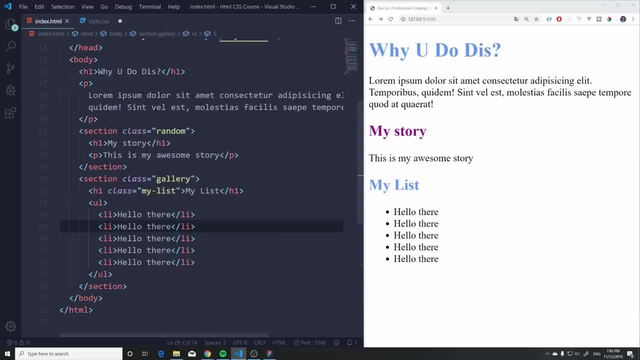 encounter. One is: maybe sometimes you want to target On this H1, I added the class of my list. Sometimes you want to target something that's below it. So in this case, if maybe I have the H1 selected, I'm going to add the class of my list. So I'm going to add the class of my list. So in this case, if maybe I have the H1 selected, I'm going to add the class of my list. So in this case, if maybe I have the class of my list, So I'm going to add the class of my list So I can target. 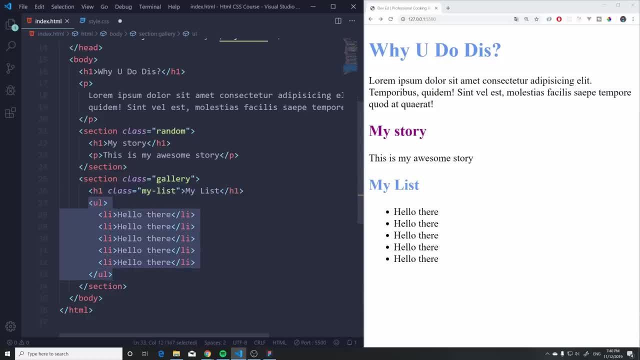 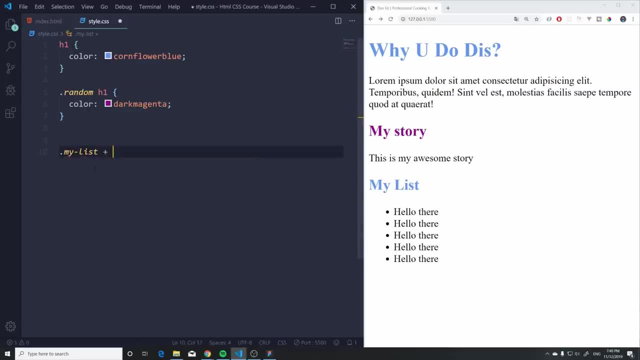 something below it like this UL. The way I can target something below is by adding a plus symbol, So I can get the my list, I can get the H1, and if I add it plus, I can select that UL below it. 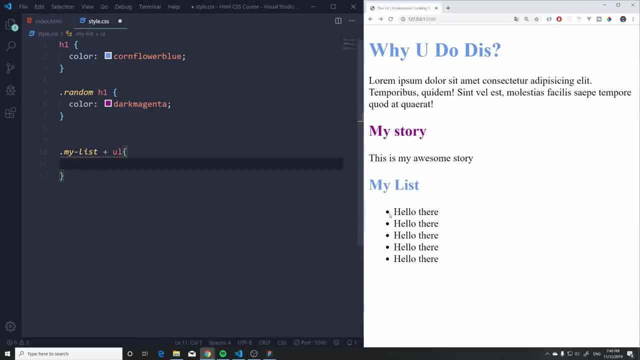 Okay, and then here let's introduce a new one. Maybe I want to get rid of the style on that, those dots on the unordered list. we can add a List style whoops, and we can say None and hit save and, as you can see, that gets rid of that. so anytime you want to. 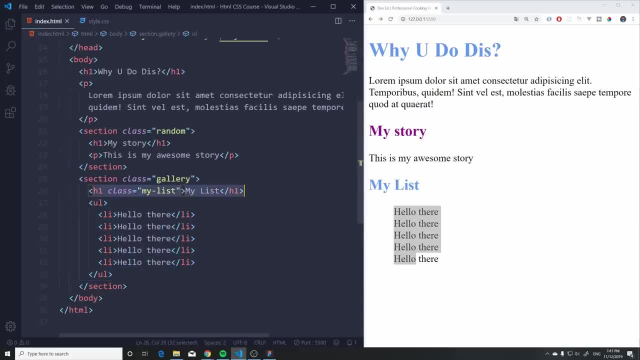 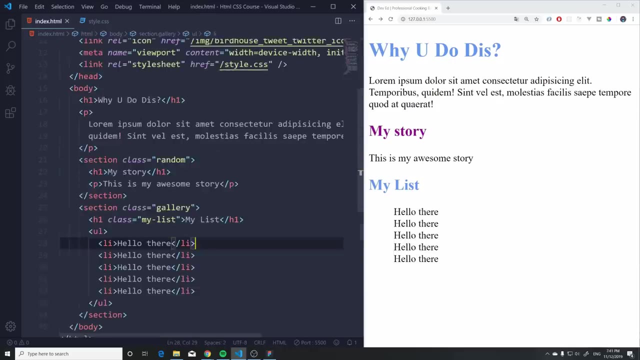 target something below. you can have the element above selected and you can target that with the plus, in this case h1. you could you need to add h1 plus P and it would select this P tag. okay, other way we can select elements is: maybe I have this list here and maybe I don't have a class on it or anything, and 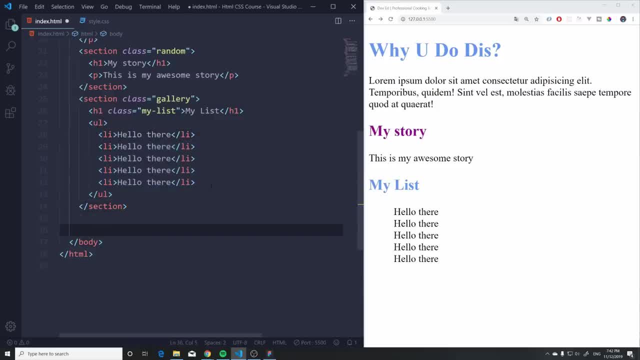 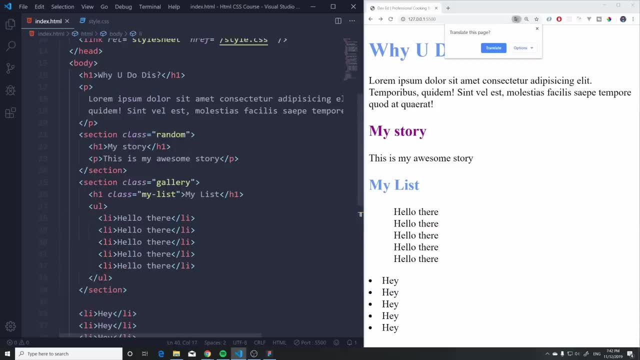 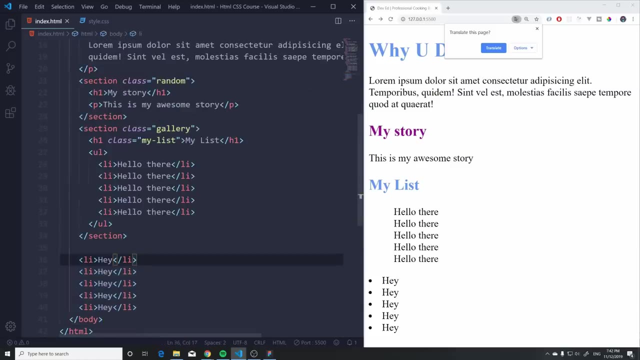 maybe I have another, another list out here. maybe I just have some list laying here. I mean, normally you wouldn't have this anyway, probably just list laying here, but you might have it on a different side of your page. so what we can do is I can select the lists that are specific to a ul. okay, so I know that. 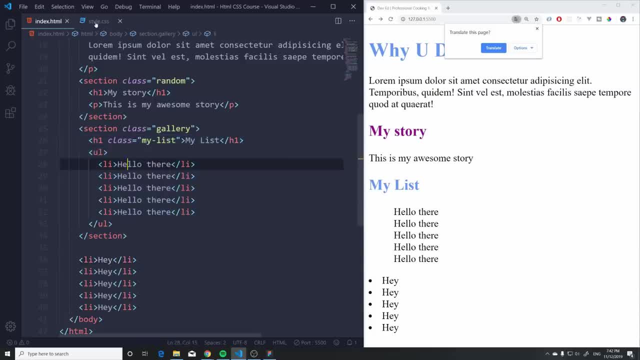 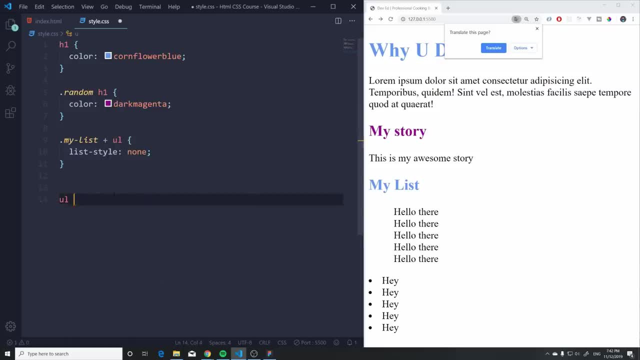 I just want to select the list that belongs specifically to a ul. so what we can do is we can say: li, excuse me, we can see ul that has lists in it like this, and if I change the color of this to let's do, what shall we do? 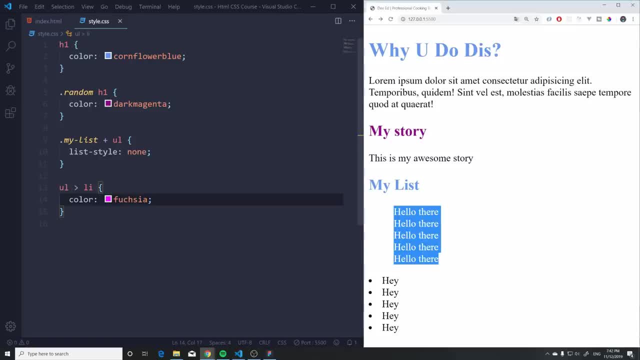 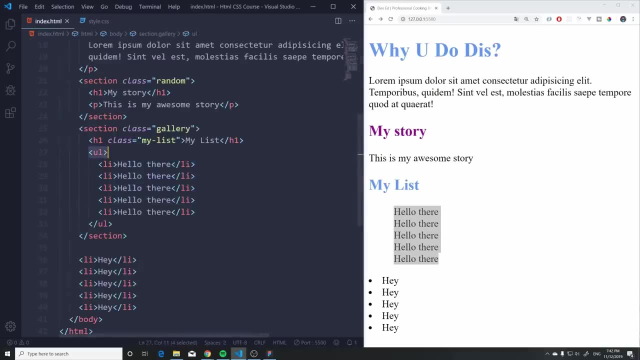 fuchsia, it's safe. as you can see, it only changes the Li's that belong to a parent. that's the UL. so whatever is the parent. so the big element that holds all of these small allies are the only elements that are going to be applied to, so like. 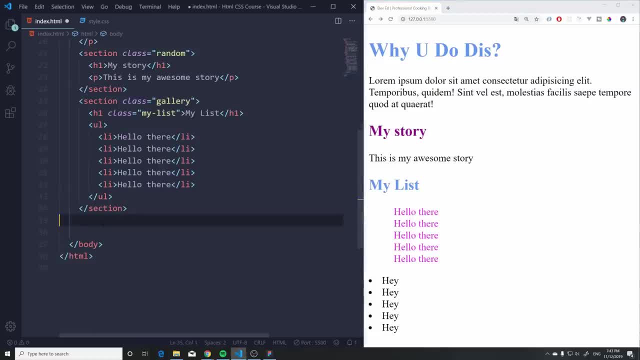 this now again, this you might probably also have released and you know that you can use it here. for example, you have a list, have it in a ul to be semantically correct, so this wouldn't work, but what you might have is a class on top here. so let's say this is my navigation or something: nav links like this: 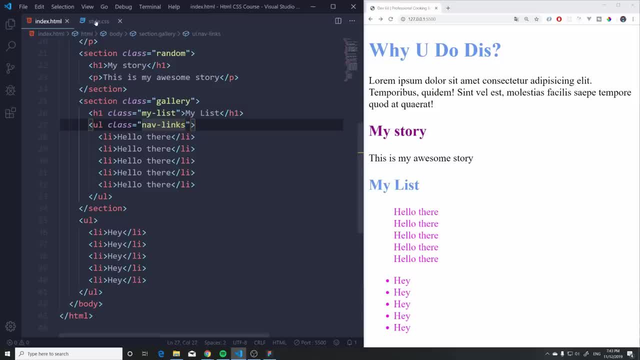 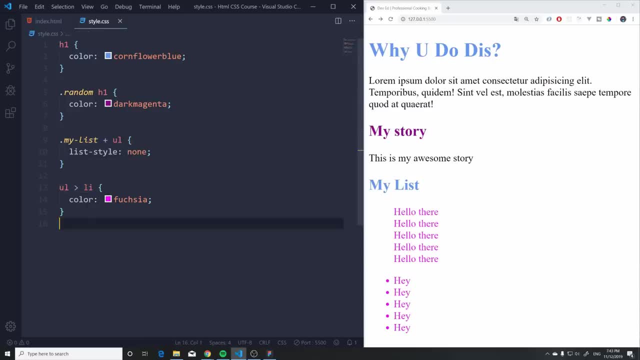 you can also add a class here, so you can combine these with classes, ids. so everything i'm showing you here you can add classes and ids as well, all of these symbols. so here i cannot, i can get rid of this ul and i just say that, hey, every li that belongs to this specific class, to this nav links. 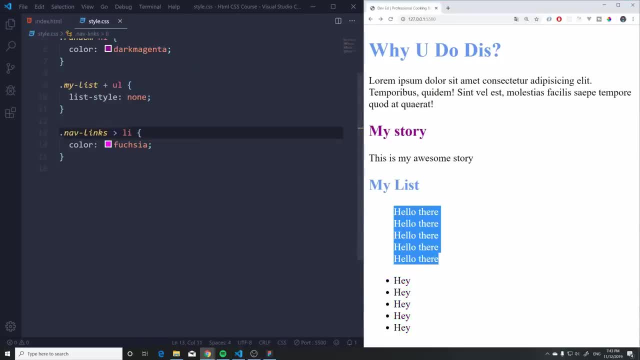 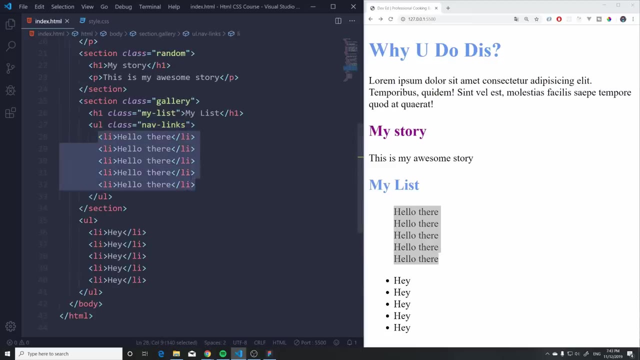 like this and, as you can see now, this only changes. but make sure when you're using this symbol, it only applies to when your parent is nav links, so only the li's that have a parent of nav links. so make sure you just look outside. so here are the nav links. oh, what's my parent? well the thing. 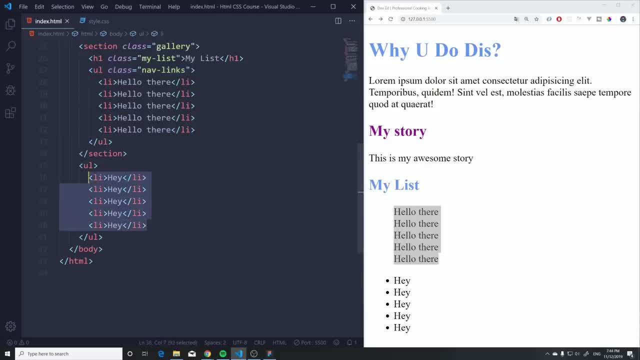 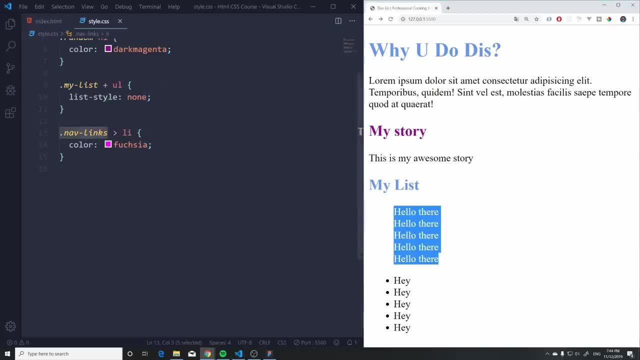 that wraps me, which is navlinks- navlinks In this case. oh okay, what is my parent? Well, just this ul. It doesn't have that class of navlinks, So obviously it's not going to be applied In the other case, when we didn't. 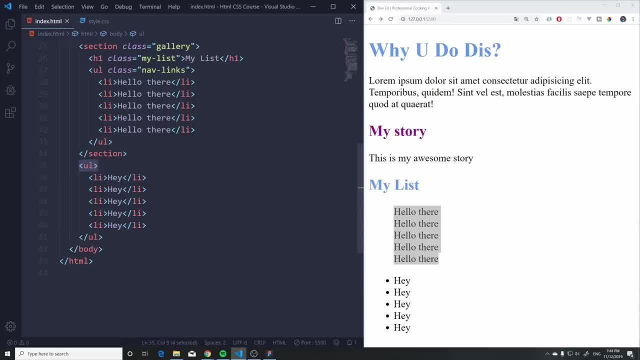 have the class. well, it was the same. Oh, the parent is the ul. Perfect, I'm going to apply the styles. Oh, the parent is ul. I'm going to apply the styles, But here it's a bit more. 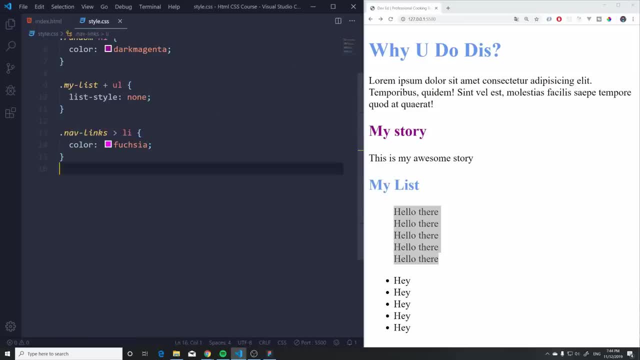 specific, But sometimes this is kind of redundant and you might not want to do this, Since you have a class already on top of it. you can just get this by saying navlinks, li, and you're going to be just as fine. So there's different ways of selecting elements and there's no one specific. 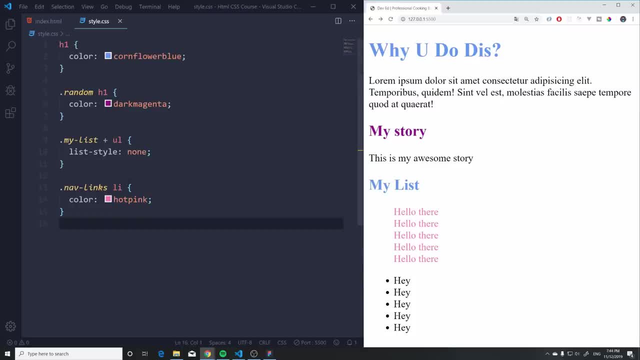 right way of doing it. You have a lot of choices here that you can mess around. So, yeah, it's just about messing around with it and trying to figure out what would be the best choice without even overblowing and adding a class. 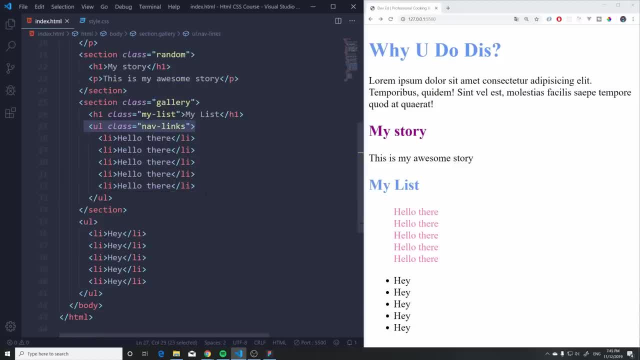 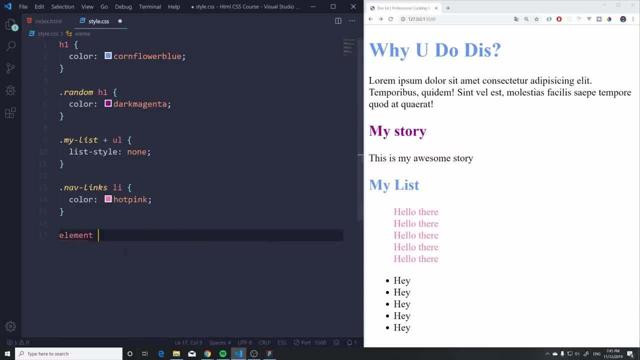 to everything, right. Sometimes it's enough to just add it to a parent element and you can drill down using the selectors by saying elements, using the elements and then, or maybe having a random class and then saying li. Sometimes that might be fine and it might be just enough to do it. 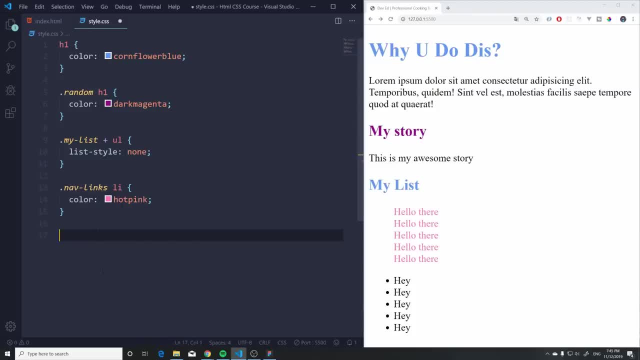 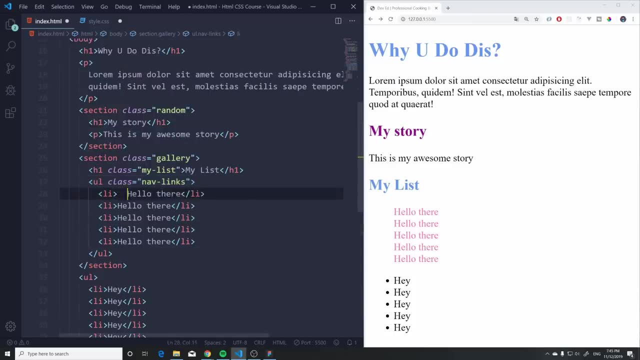 okay, But technically you can chain together as many as you want. Imagine that we can have an li and then we might have an a in here, So an anchor tag that's going to link us somewhere. Let me just drop this here and, real quick, we're going. 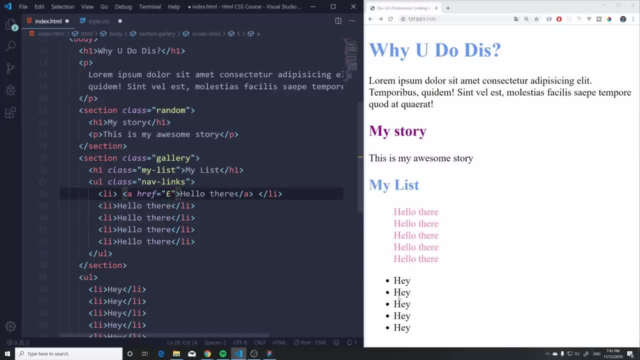 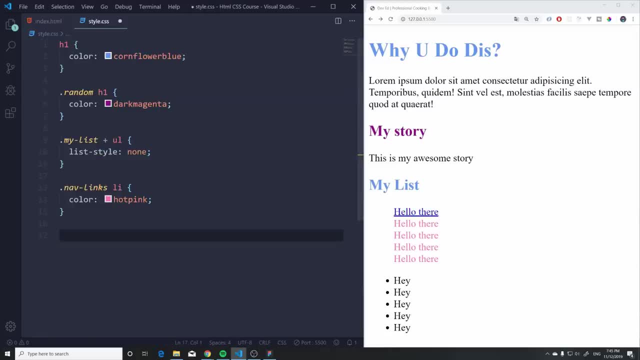 to add a hashtag. to quickly get rid, Let me switch the keyboard, Let me. there we go, So you might have a anchor tag here. So to access that, you would need to drill down, You would need to go from ul to li to a, So we can do that like this: Let's select the class. I forgot. My memory is: 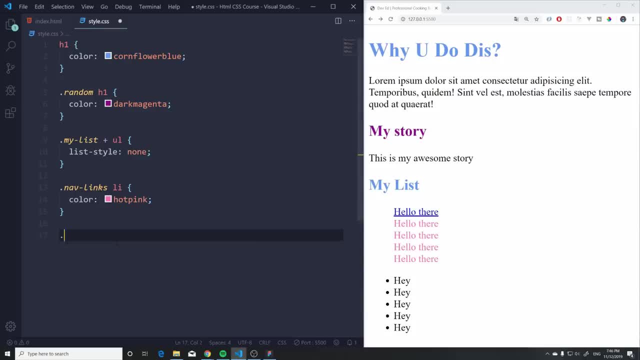 very short today. Nav links, So we can get that. nav links like this: Li a, So this works just as fine to color black. okay, Hit save Boom, It got rid of it right, But sometimes again, this is if you want. 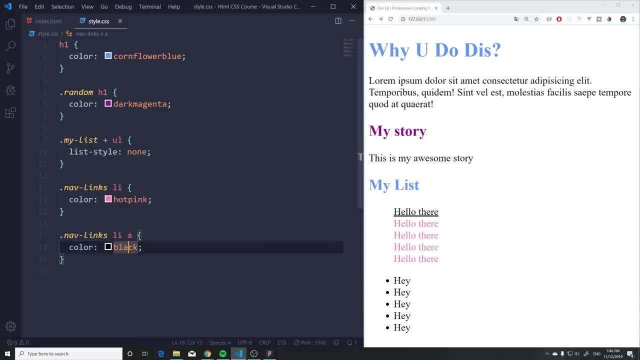 to go all the way down and be very specific. If you have only this anchor tag here, you can even get rid of this li, because there's no real reason we should add this li in here, because what this specificity means is what this selector means is. I should go to the nav links, which is here. 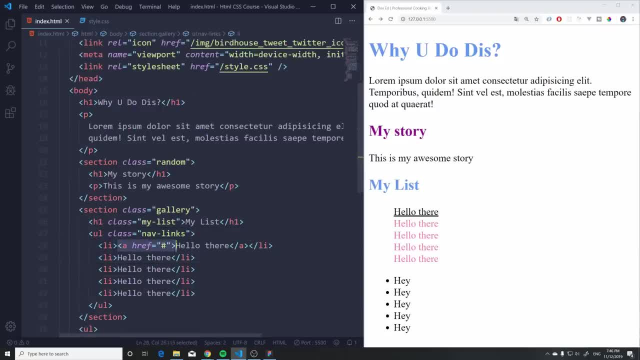 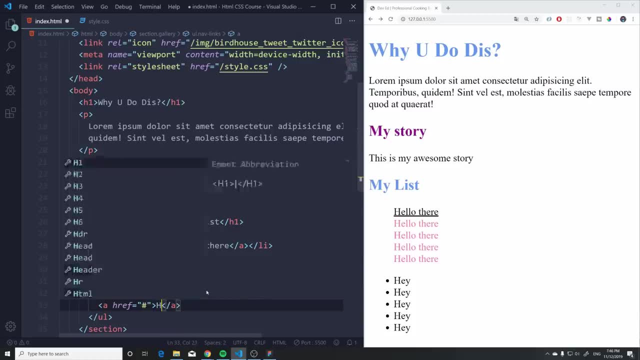 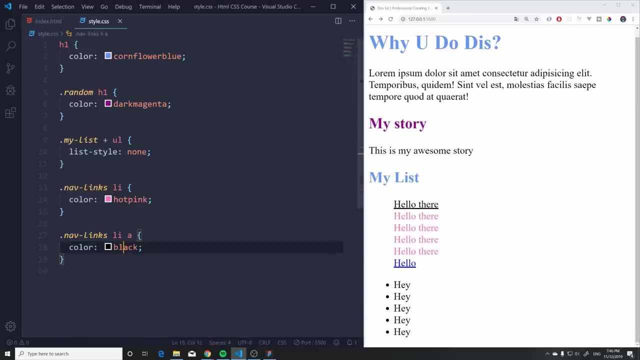 and then take a look inside the li's: modify only the anchor tags, Because if I have another anchor tag in here, let's say hello. If we have another anchor tag in here, as you can see, it doesn't modify it. Why? Because I selected it specifically. I said nav links, only the a tags inside the li. 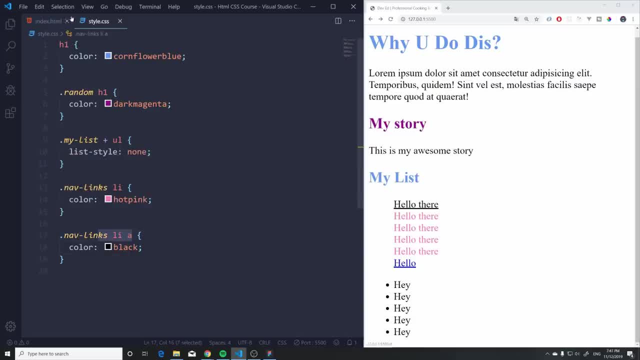 right. So by doing that, only this one is going to be black and this one stays blue. If I want both of these blue, then I would have to get rid of this li. So boom, there we go. Now both are. 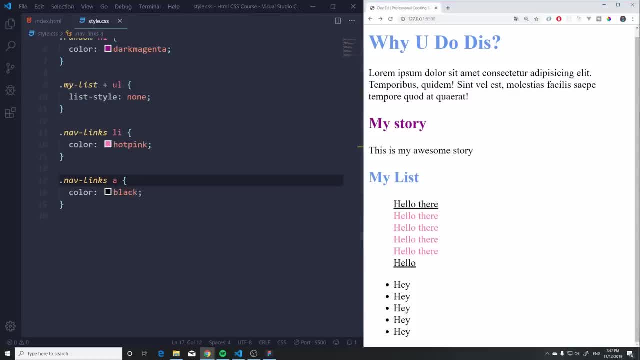 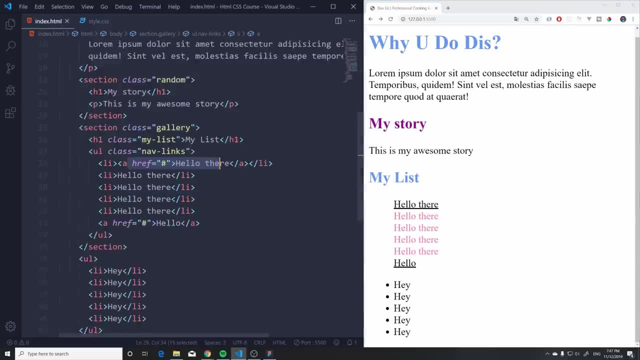 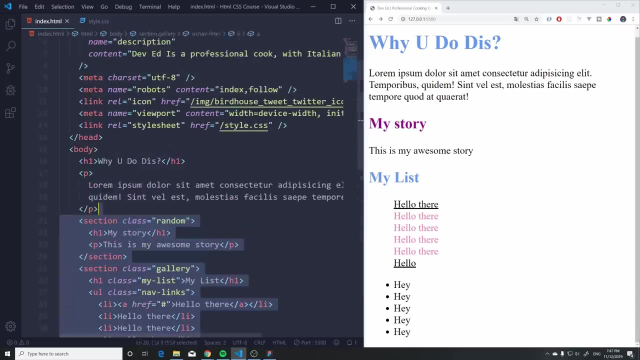 dark, Perfect. So those are a few ones. We can also select elements by their number, by where they are positioned inside a group here. So I'm going to clean this up a bit to make sure that this is a bit more simple to read. So let's get rid of everything. I'm just going to get a ul here. 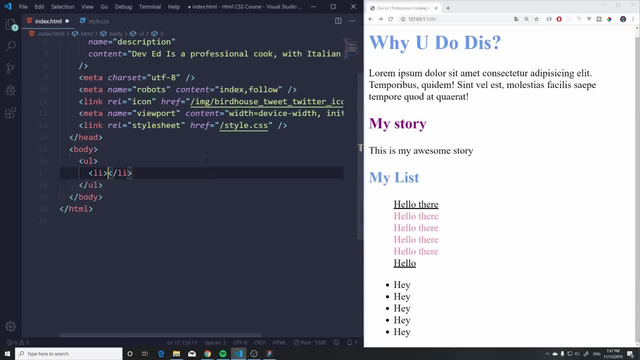 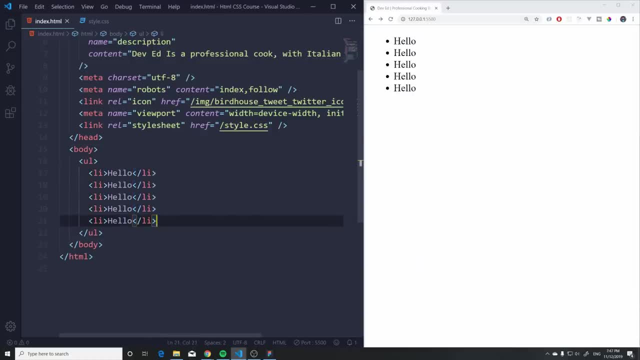 and I'm going to add a few li's, Li, hello, and then we're going to duplicate these a few more times. okay, So the way we can do this, I'm going to add a class of links in here We can get rid. 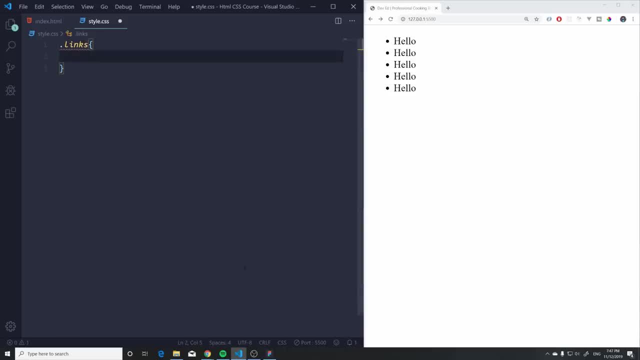 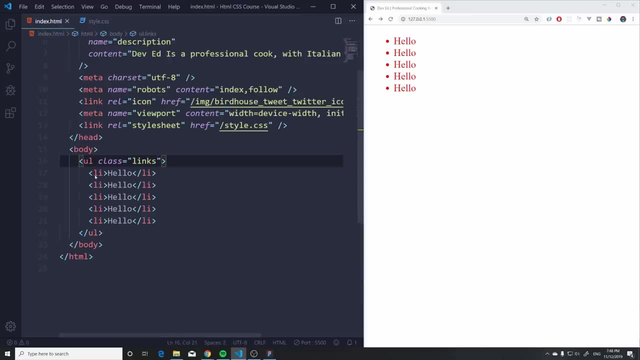 of everything. We can select those links like this: Again: if we add a style here- color red- it's basically going to apply everything. So if you add just a color red to this or something, it's going to apply the color red to everything that you have inside here. Okay, but maybe I want to do something. 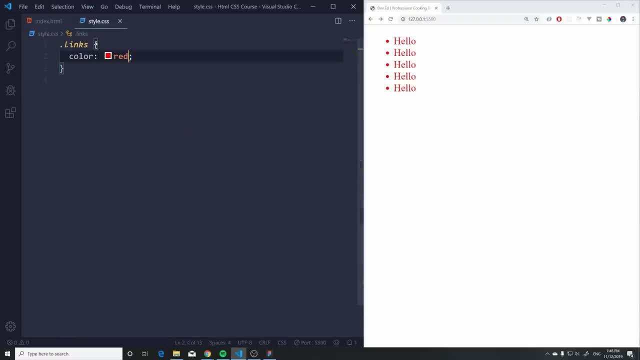 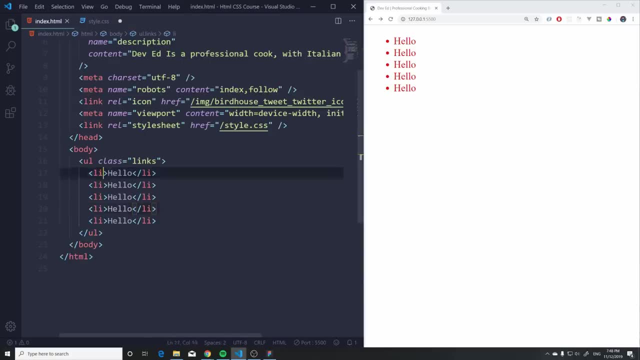 specifically to only one. So what we can do is, with this links so the class, the big ul that we have, we can select a specific number in here, right. So on the position, that's what I'm trying to say. So this would be. 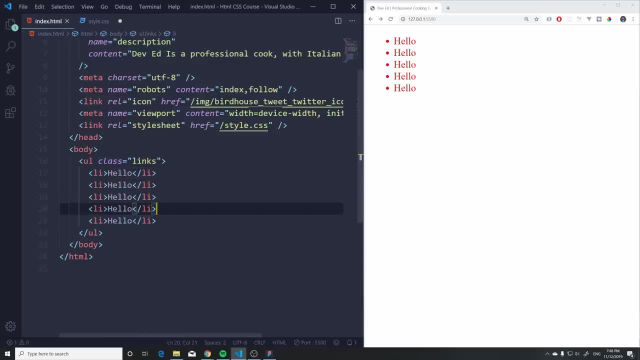 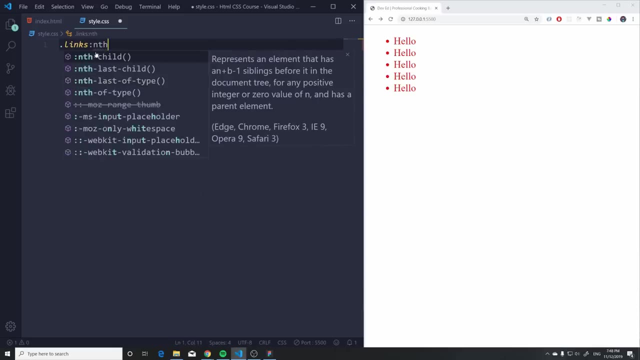 one, two, three, four, five, right The numbers of the elements and their positions inside this ul. So the way we can do that, if I want to select one specific one, we can say links like this, and then we can add a colon like this and say: and child, all right, And here we can provide. 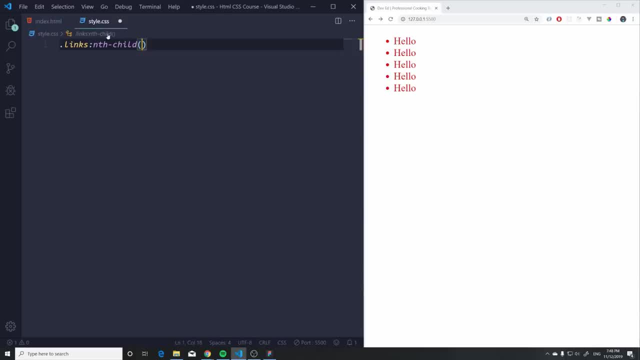 the number. If I want the first element inside this links, I can say one and then I can say: color red. I don't like this red, I need to change it. So I'm going to add a color red to this. 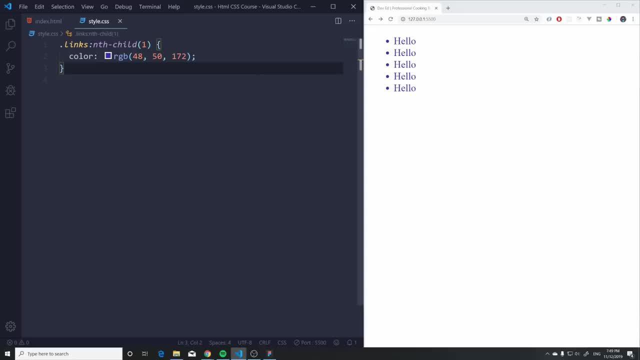 I need to change it. That's so awful Blue, God bless. Okay, There we go. So if I say and child one, so if I say and child one, as you can see, everything gets turned into blue. Well, 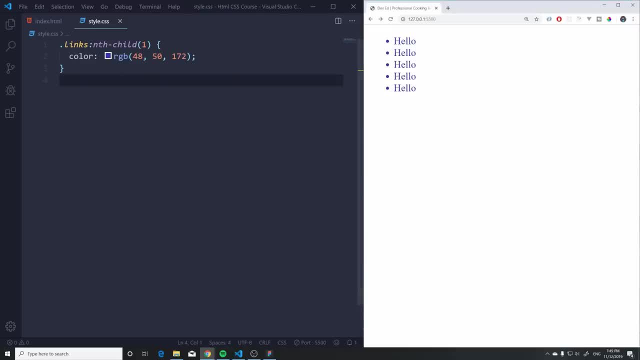 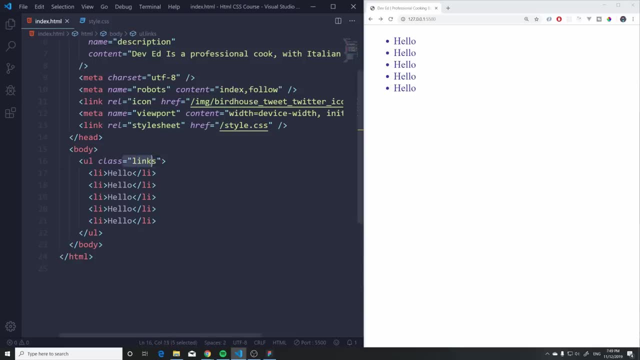 why is that happening? Well, we need to add specifically what element we want to target, because right now we just say, hey, the links and child one, which is only one. we only have one class of links. So what I need to say here is in the links. 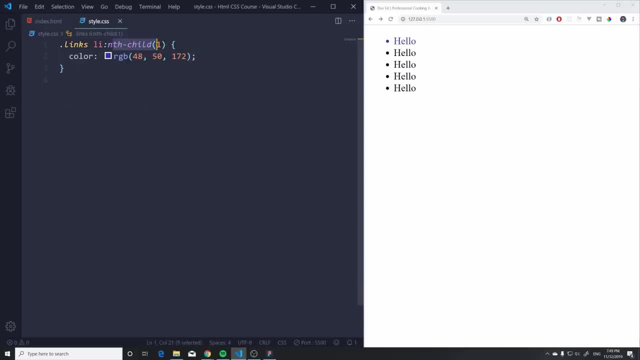 I the first ally with the ends child. Okay, So let me change the color of this because it's again hard to see. So, as you can see, I need to write the class that we want to take a look at, and then the ally, and which ally, and this list of groups. Well, the first one, So ends child one. 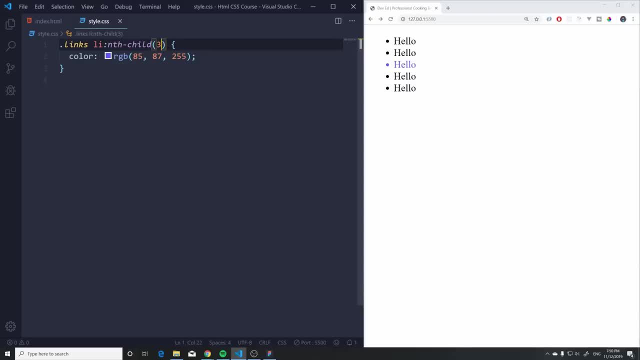 if I want the third one, I just write three, And let me make this clear why that happened. So if I go back here, this happened. as you can see, nothing applies now, But if I say one, it applies, And the reason why this is happening is because we only have one. 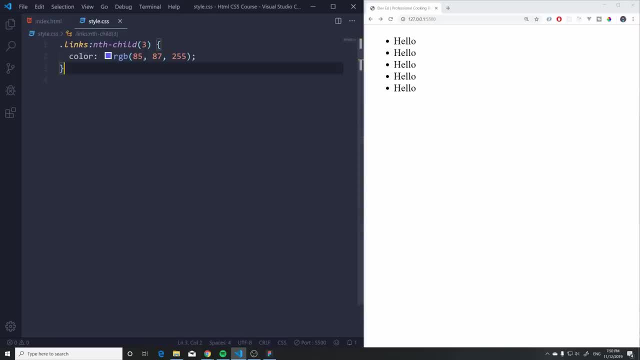 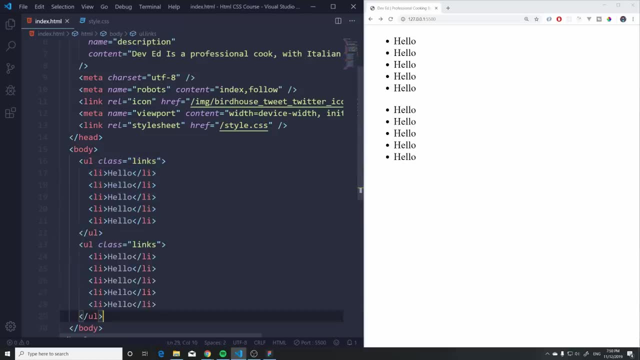 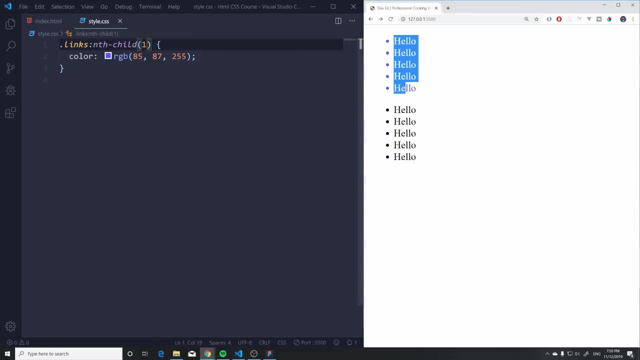 class of links. So it takes a look here and adds that color to everything, basically that we have in this links. Uh, but if if we have two of these, then take a look. If I do two, it only applies to this one. If I do one, it only applies to this class. So we strictly looked at the classes and 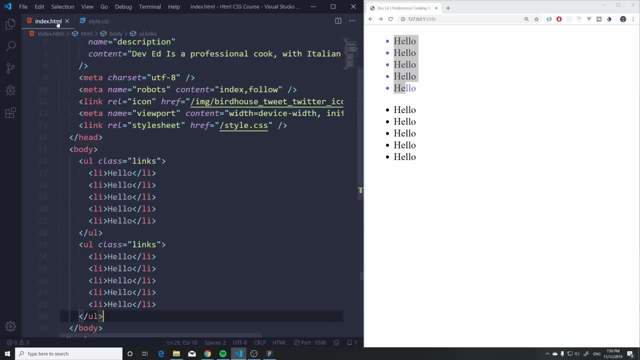 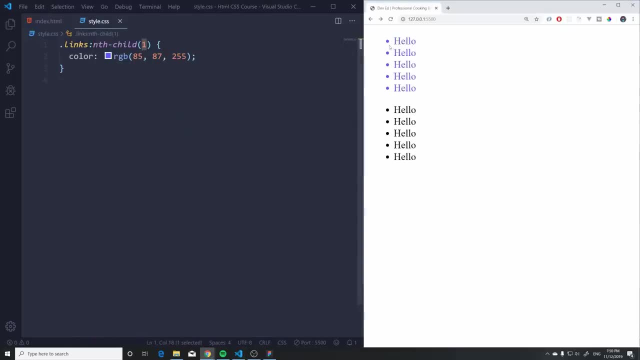 the links class To the ends child, uh, and not the ally or something else more specific. Okay, So that's why, when we added one, it just applied the color to the whole thing, because it was like, okay, well, I just apply, you can read it like this: links color blue. That's basically what happened. 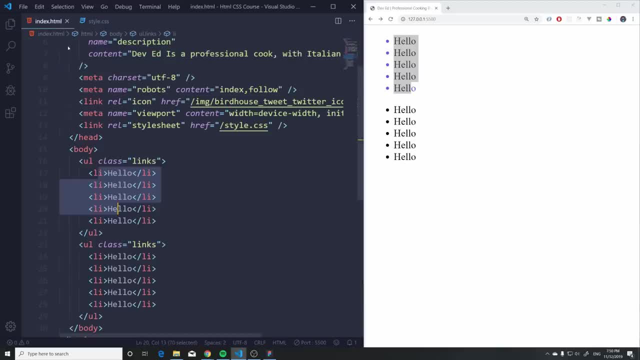 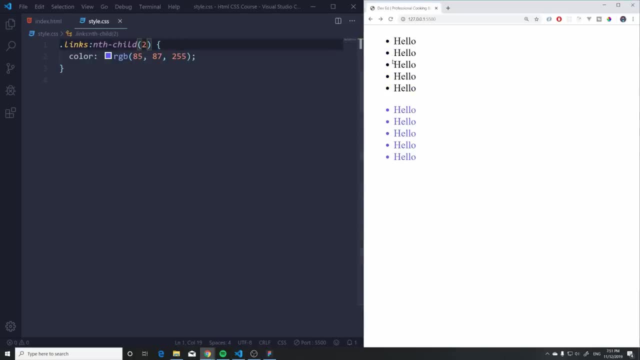 because we had one, So this had no effect on it. But if we have multiple ones like this, like one and two links, then you can specifically select one or two of these, All right. So let's get rid of this. We're only going to keep this one and let's change this back to ally. 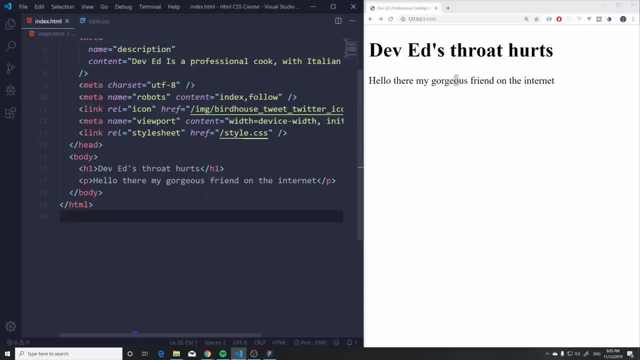 And we are specifically selecting the second one. Okay, Here is where we are going to understand CSS way more, how it works. Uh, my throat hurts a bit, So I apologize if, if I, if you're not going to hear me in a bit, I need to take a break a bit after this one. Uh, but you're not going to know. 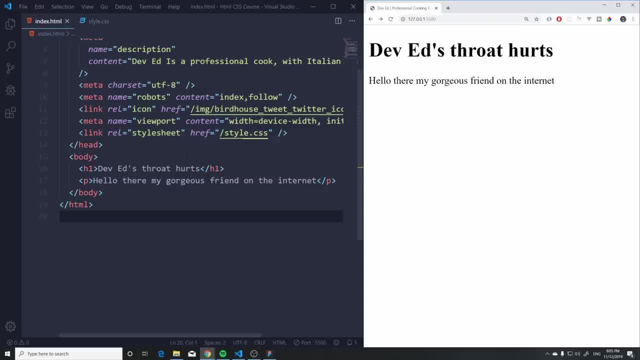 that because, yeah, you can just watch the next video and it's like, Oh, three days passed, Okay, Anyways, let's move on. So I kept this as simple as possible. I just have a H one here and a P tag, Okay, So take a look If I 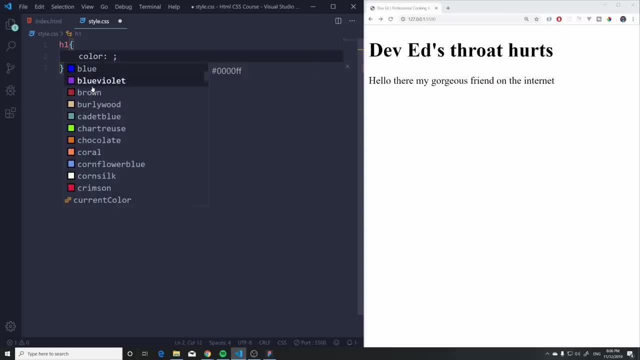 select that H one and I changed that color to coral. Okay, We have that nice coral color. What happens when we write H one again here and we say color cornflower blue? Well, the color changes to cornflower blue. Why is this happening? 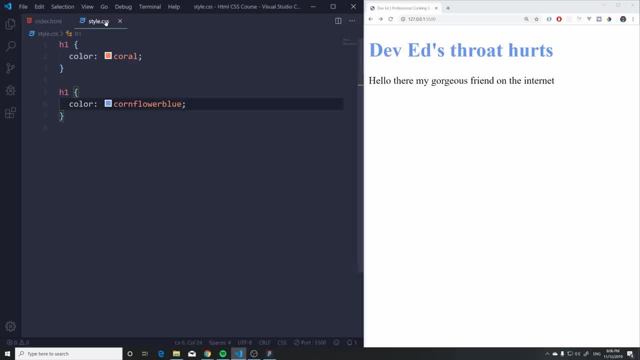 Well, CSS works from up to down. Okay. It reads the first one, It says: okay, H one should be coral. and then goes, goes, goes and gets to H one again and says: okay, color should be cornflower blue. So the last tile always gets applied. Okay, If we select the same thing, the one further down. 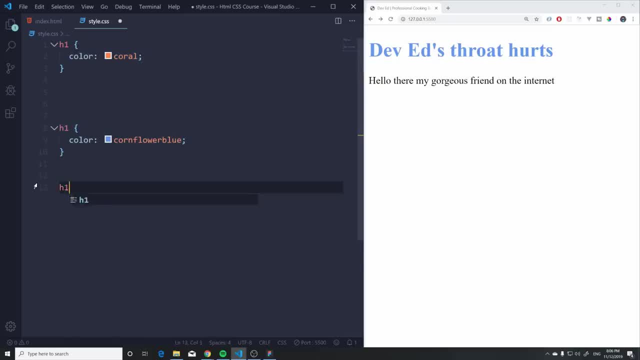 is the one going to be applied. So if I write H one again and change this again, it's going to change cyan. Okay, So it's cyan now. but if I move this up here, well, cornflake is going to cornflake. I keep. 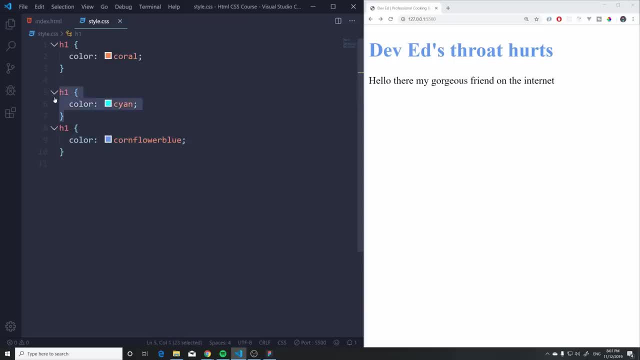 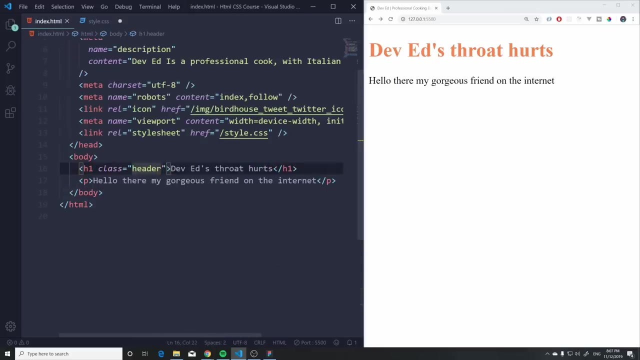 saying: cornflake, Cornflower blue is going to be the one that's going to be applied to. Okay, However, Okay, So we know that it goes from up to down and the last one gets selected. Okay, What happens if I add a class to this? I'm going to say class of Heather, Okay, And then we 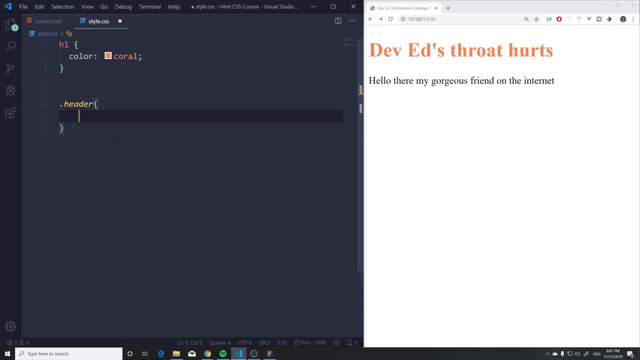 go in here and I just write Heather, and we change the color to cornflower again, like this: save. okay, that's blue, that's what we expected. right, because we read it from up to down. but what happens if i move this up here? well, is it going to change the coral? no, 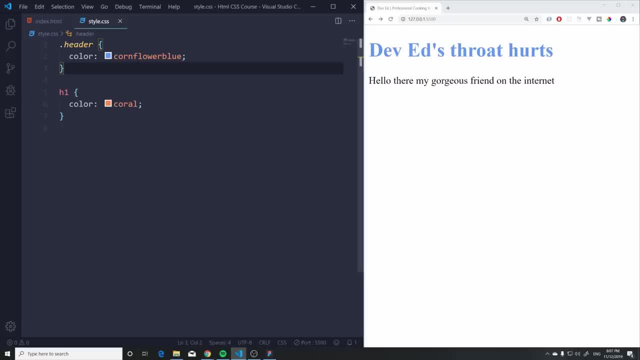 it's still cornflower blue. why is this happening? well, the reason why this is happening is because the class has a bigger priority over the element selector, and a good way you can see this is just by hovering over the element and you're going to see that the selector specificity is 0, 0, 1, whereas 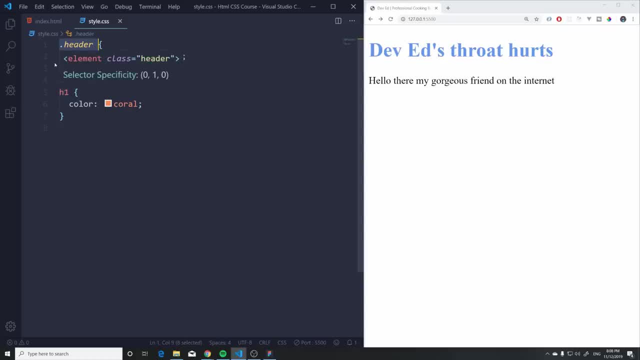 this one is 0 1 0, so the one further on the left is going to be more and more important. okay, so this is 0 0 1, this is 0 1 0. so what is 1 0 0? well, 1 0 0 is an id that's the most valuable one, because 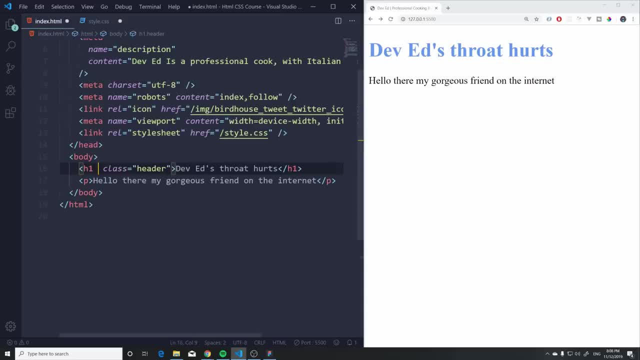 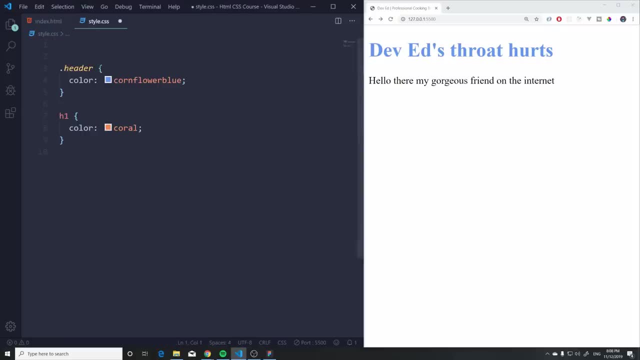 it's the most valuable one. because it's the most valuable one, because it's the most valuable one, most unique one. so if i add an id to this of head, i'm just going to say head, like this. if i say head and i apply a color of dark red, 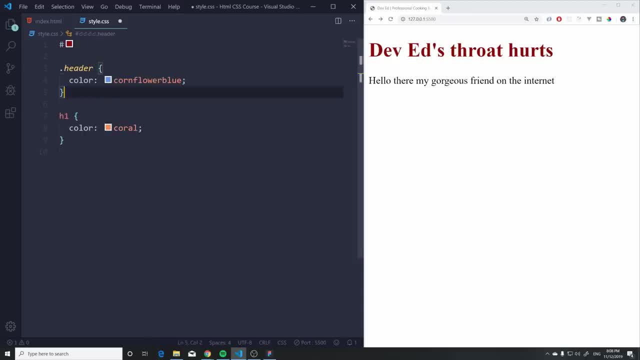 now, this is going to be the most important one. it doesn't matter where this is. it can stay here. it can stay here. it can stay here. it doesn't matter, this is the least important one. 0 0 1 0 0 0 0 0 0 1. 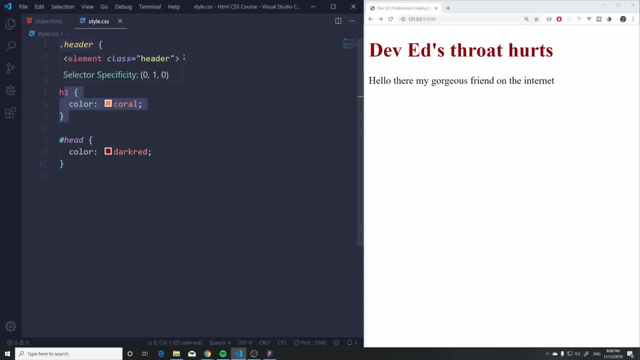 this is secondary: 0 1 0 and this is the most important one: 1 0 0. however, this is mostly what you are gonna encounter- these three in here- but there are certain cases where you might have a style on the element, if you have a style. 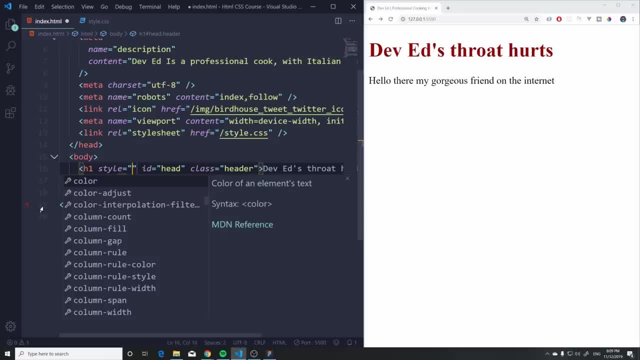 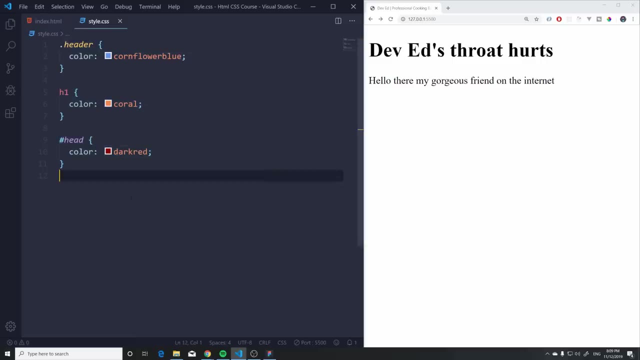 on this element. so I'm gonna say style color, I'm just gonna say black and hit enter this. you can imagine it as this: having a greater priority over everything that you have here in CSS. okay, it's more important than everything you have, whether it's h1, whether it's a class, whether it's an ID, as soon as you. 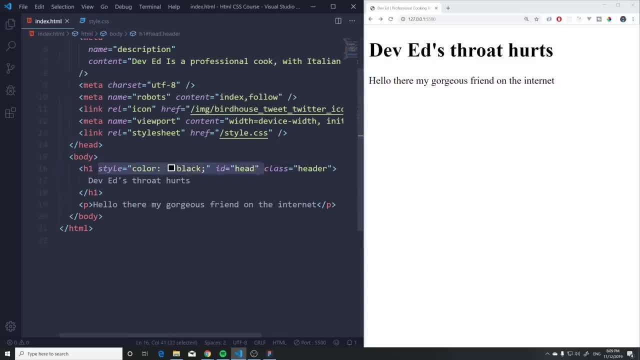 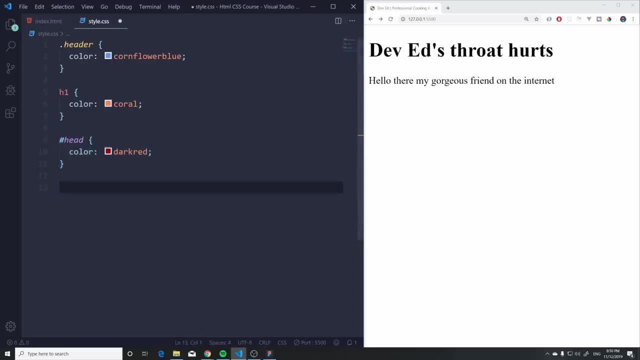 have the style directly applied to the h1. that's gonna win. however, there is one more. oh my goodness, what did they do there? they smoked something, you probably. but there's one more. if, if you have no idea how to change the style and you cannot find in your code what's happening, what you can do on whichever. 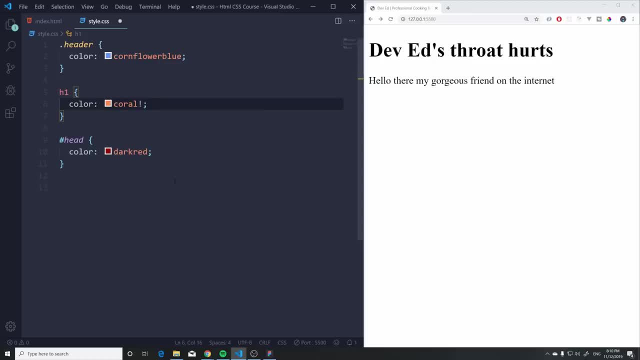 element you want. you can add a exclamation point, important like this, and this is basically gonna override everything. this is like the last solution. this is. this is not good to do. you don't want to add this important- usually almost never, but this overrides everything, so it doesn't matter. this is. 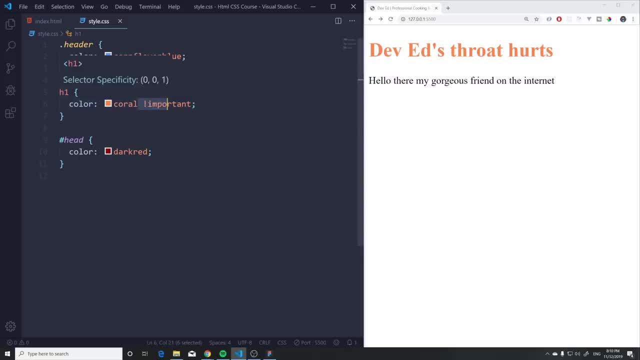 kind of like a fifth level of specificity that you can add important, but generally what you're going to be sticking to is h1 class and and this one. okay, you're, you're never gonna use this important, okay, so let's remove at this. you're better off trying to figure out. 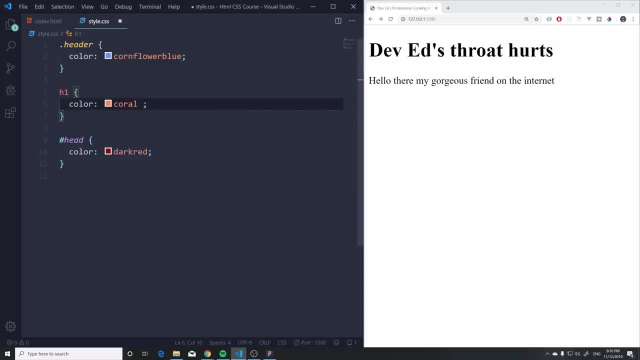 why? why this important is not working right. because the problem here is: if later on- let's say later on- we're gonna work on something and i want to change something about that h1, i want to change the color to maybe a dark slate blue and it's not working. okay, i'm gonna select. 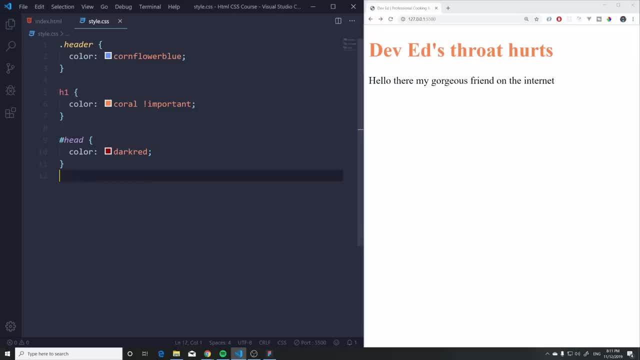 it like this, with a header not working. so you're gonna mess around and try all of these different selectors and you cannot get this to change. so again, to override this, again you're gonna have to say important here, so it's gonna override the one on top because again we are reading it from: 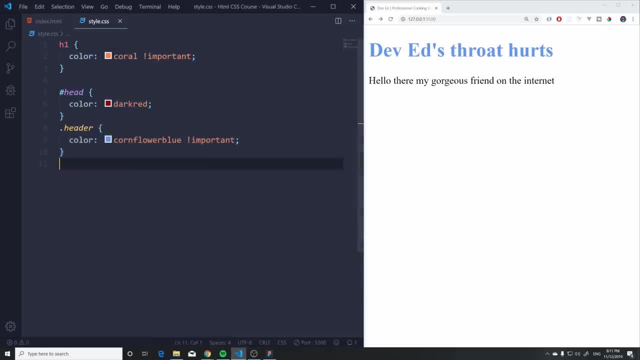 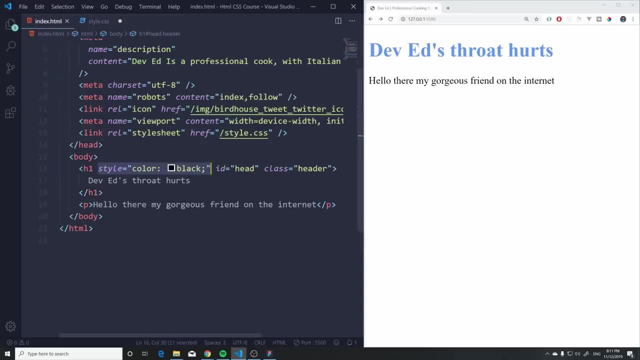 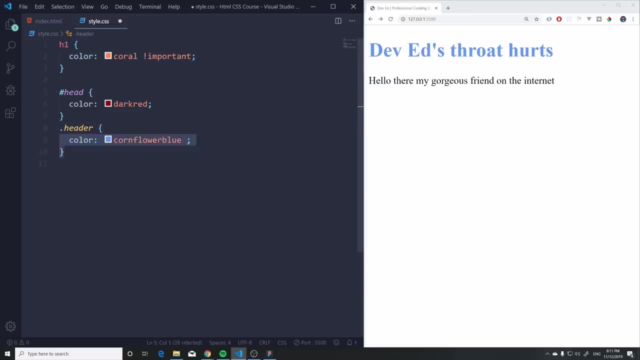 top to bottom so it gets really messy. so try to ignore this, try to ignore styling it with important and also ignore styling it in the h1. here, the only ones you should be sticking to are normal selector, like this class and id, and that's gonna make everything work right. so if you're gonna 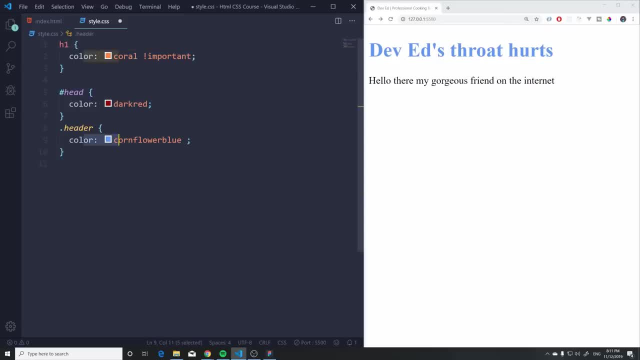 super clear on which is how important. Okay, even if you have multiple classes, the one that's below is still the one that's going to apply. However, we can also select elements. I'm going to show you a new one that we haven't covered so far. What if I do h1 active like this? So basically, 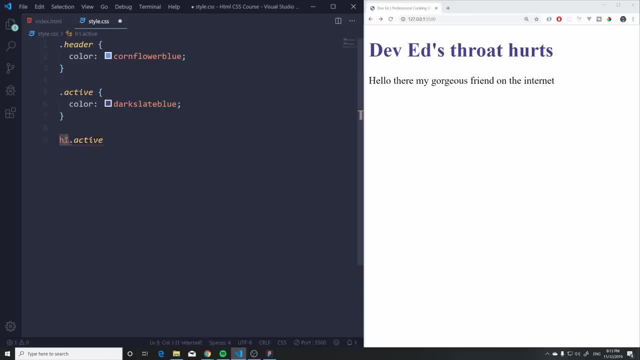 I want to select only the classes that are h1.. So now, if I say color deep pink, well, that's a new one, deep pink, it changes, and I can even move it up here. Why is that? Well, if we take a look, 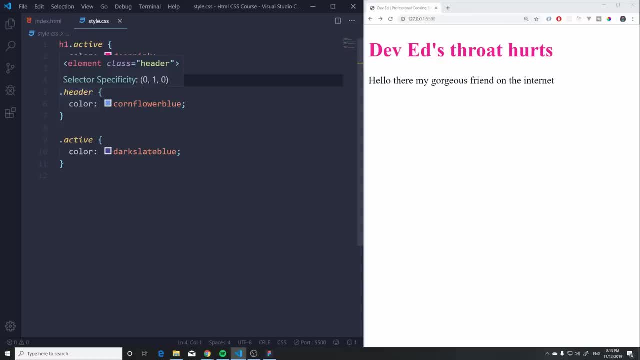 again 010,. the one in the middle is the class, So that's good, That gets one point. However, here we also have the element, So 011, right, the first zero being ID, this the second zero. 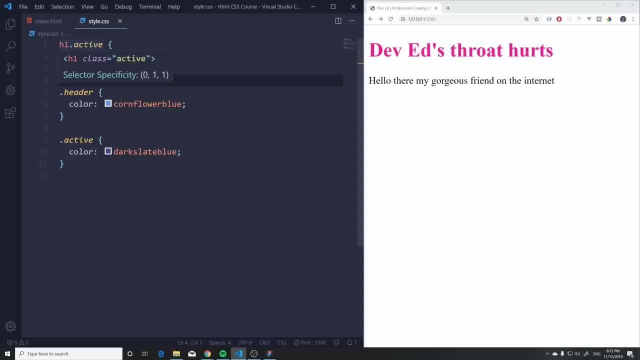 being the class and the third one being the element. So here we define specifically that I want to select. I want to select the h1 specifically that have a class of active. So it's a bit more specific than just throwing out a random class because, hey, we can have this active class technically on anything. 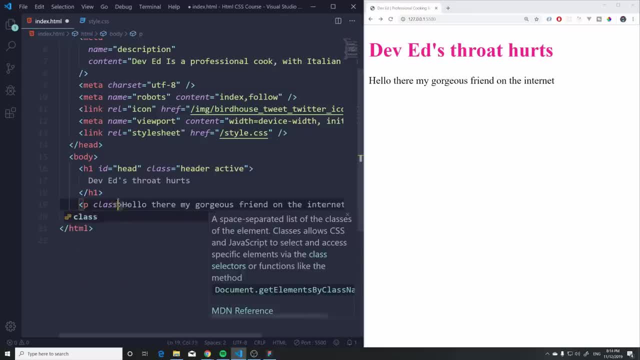 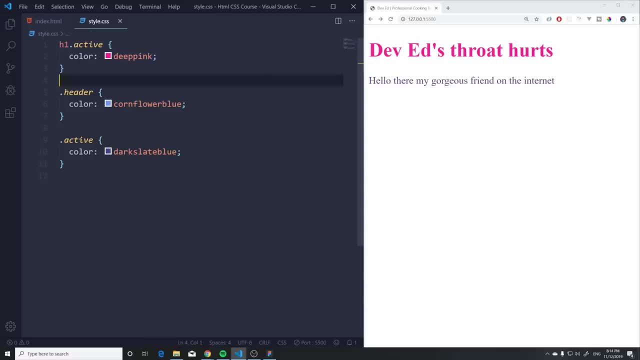 we want. I can add the active on here- Class active- okay, so I can have the same thing, But that doesn't mean that I want to apply that deep into it. So this is more specific. Okay, margins and paddings. 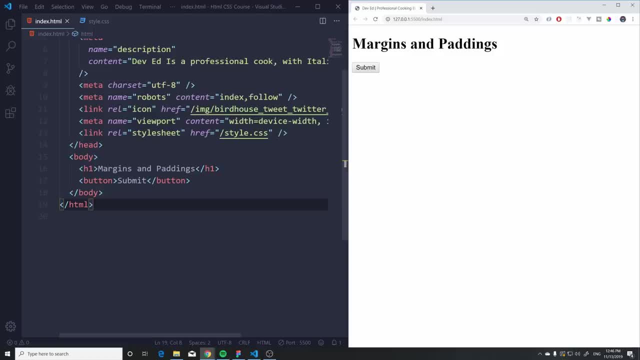 So what are these things And why are they so important? Well, we're going to use these a ton, So I really want to cover this so you understand everything. Okay, so we talked about how the browser basically put some default styles already on our elements And we saw that there's this big 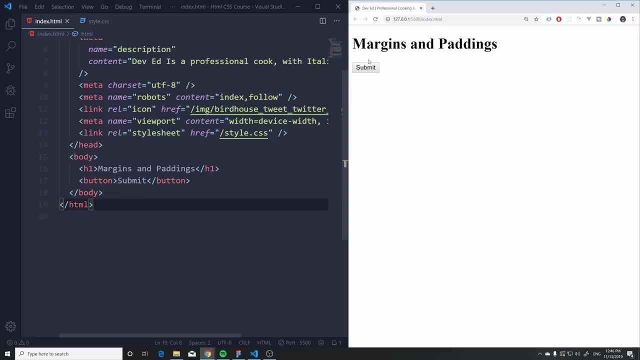 space with the header and heading one here. So look at this space between this and the button. And the way we can look at that is if we tap f 12 in the browser and then if we go over to this tool, click it and if we hover over or optionally, you can just go down here to 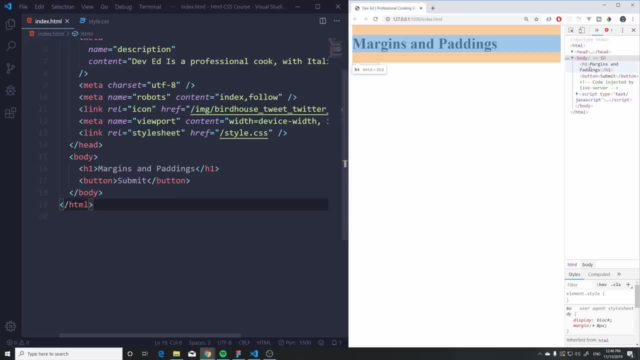 the elements, and if I hover over, you're gonna see that there's the element which has a blue color to it and then there's an orange color that has that space. so that orange color is actually the margin, okay, and, as you can see, it just gives. 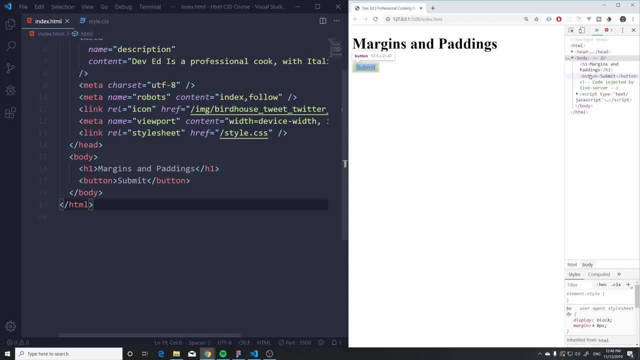 space between the elements, and if we go down to the button now, this is kind of hard to see, so let me zoom in- you're gonna see that there is a a green one as well, besides the the orange one. so what is that? that's weird. all right well. 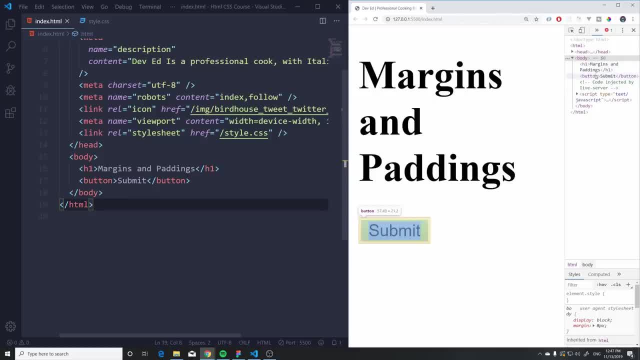 let's see: the green one is the padding. but why? how is that any different than the margin? okay, let's take a look at the difference. so I'm gonna zoom a bit back out, but I'm still gonna be zoomed in so you guys can see. okay, so here it is. 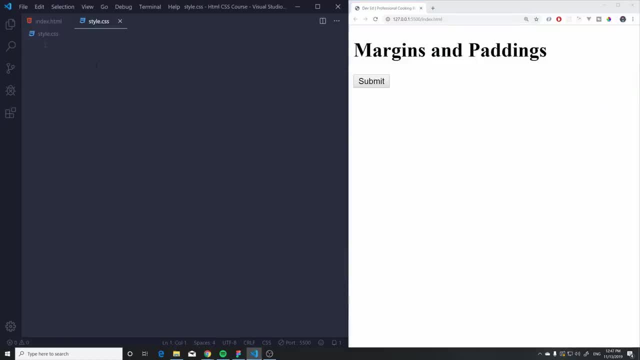 let's actually see how we can add a margin and padding. so let's just get the button here, okay? and if I add a margin, I just write margin and I'm gonna say 100 pixels, so that's gonna add 100 pixels of margin. hit save. as you can see it actually. 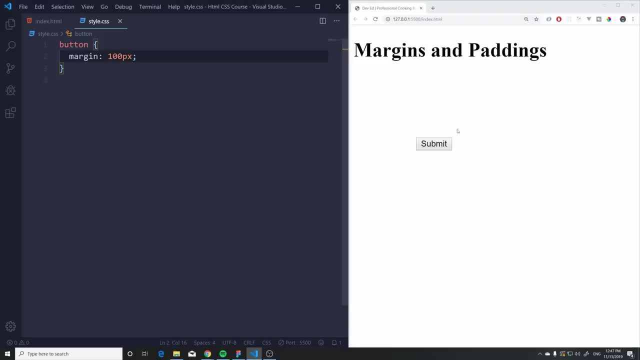 applies the margin everywhere: top, left, bottom and right. okay, so if you just say it like this margin 100, that's gonna add space up left, bottom and right everywhere. all right, if we change this 50, you can see that as well. if we check here, you're gonna see that that orange grew a ton. 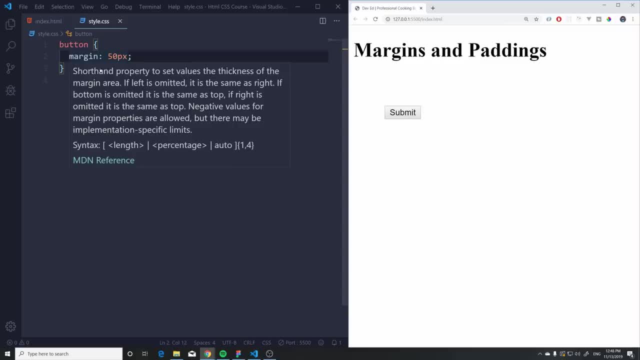 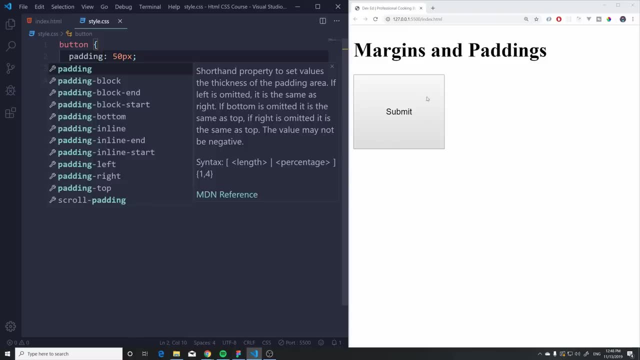 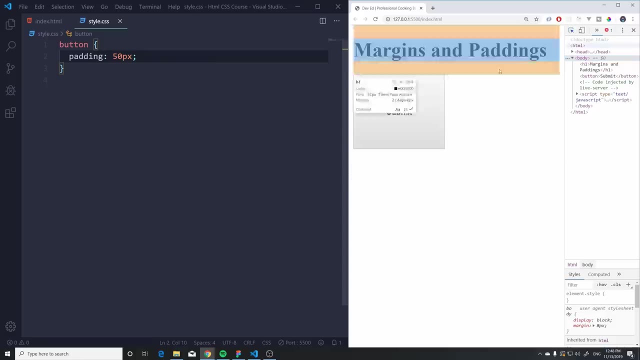 that's cool, but what happens if we add a padding? so if I add a padding of 50 pixels, that's gonna grow the element, but it's gonna be the inner space, as you can see. so if we take a look again, as you can see, the element itself grew okay. 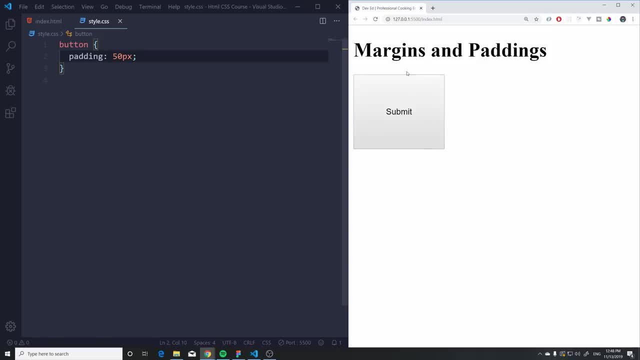 so that's the difference between padding and margin. the margin is gonna be on the outside of the element and margin is gonna be on the outside of the element element and the padding is going to be on the inside of the element. Now, if we do this on the 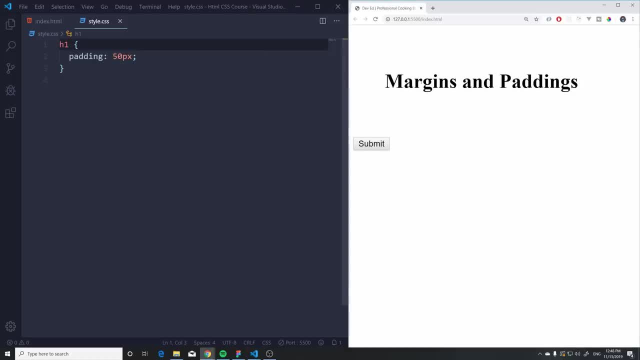 H1, it might be hard to see. As you can see, it kind of looks the same as margin. So if I change this to margin 2, it looks identical. However, this gets changed a bit as soon as we start adding. 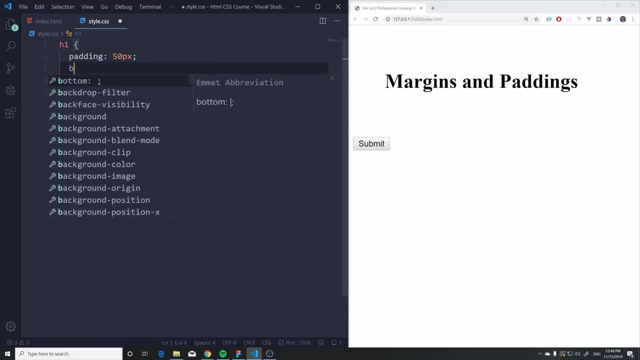 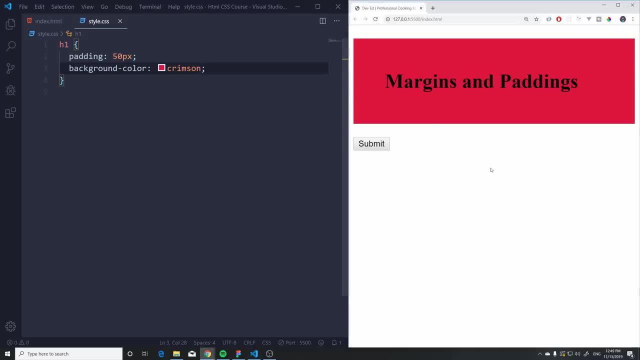 a background color. So take a look On the padding. if I add a background color of crimson, as you can see, this is the size of the element And if we click on this button, you're going to see that if I hover over the H1, look how large this H1 got. okay, This is going. 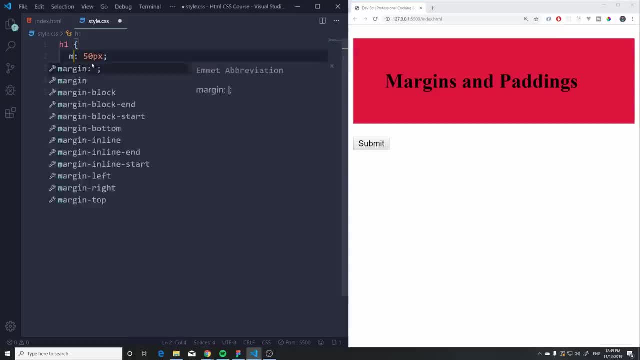 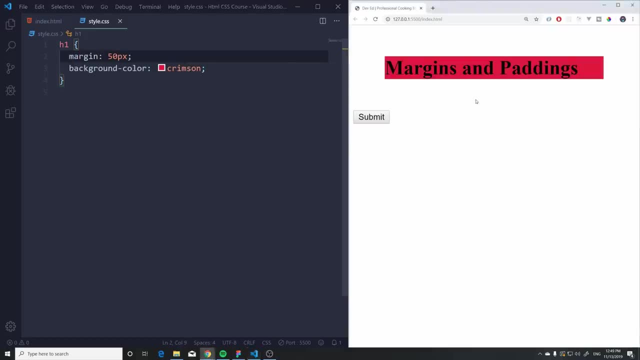 to be the inside space. However, if I change this to the margin, then the element itself is going to stay the same size and it's just going to add the spacing outside. okay, So let's take a look and there we go. Look at that. That just gives the empty space. 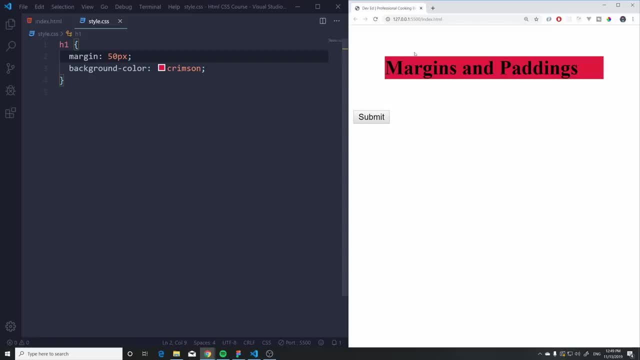 So that's all you have to do. You have to remember: margin is going to add the space outside and the padding is going to be on the inside. okay, That's the only difference. Now let's see different ways that we can add. 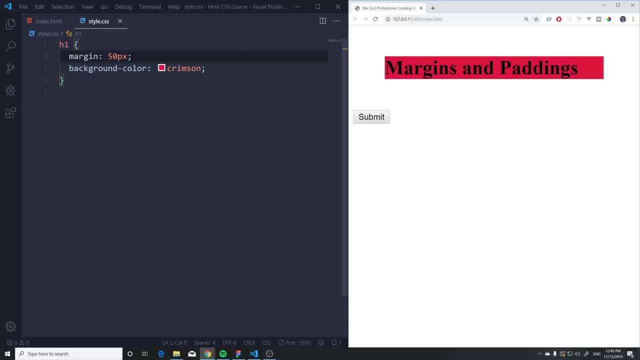 paddings and margins. I apologize, So this is the first way we saw. if we just add 50 pixels like this and that's going to apply it everywhere on each side. However, if I add another value here, let's actually do this on the button. 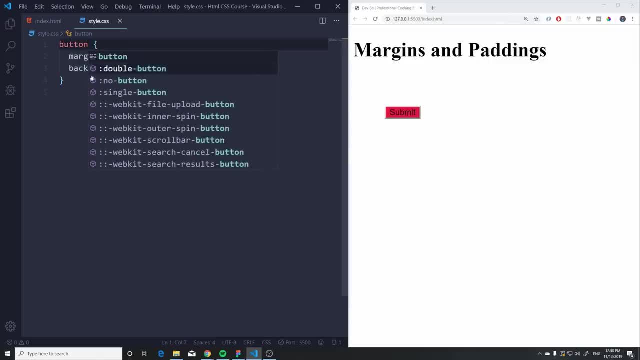 Because it's going to be a bit easier to see button, Hit save, And I'm going to. what I'm going to do is change this to padding, because it's going to be a bit easier to visualize. okay, So we have 50, 50,, 50, 50.. If I add another value here, let's say 20 pixels. 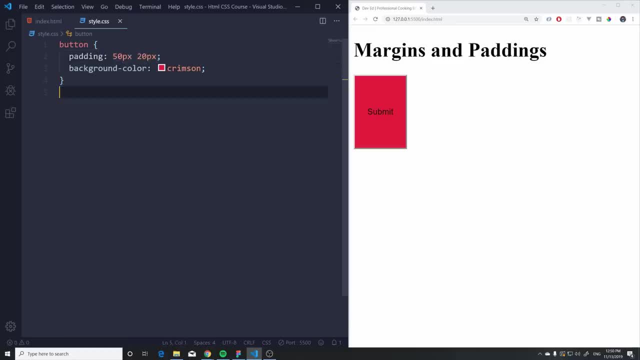 then what's going to happen is, as soon as you have two values, the first value is going to be applied to top and bottom and the second value is going to be applied to left and right. So here we have 50 on top, 50 on bottom, and here we're going to have 50 on top, 50 on bottom. 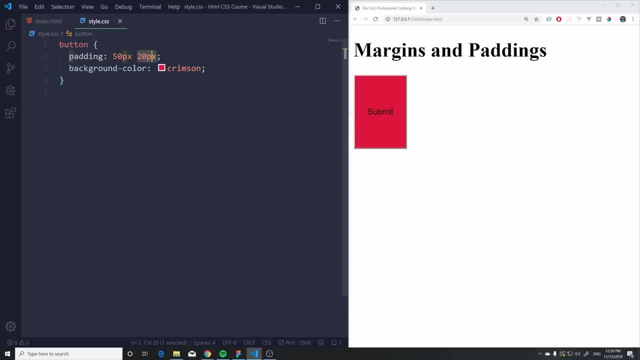 And here we have 20 on left and 20 on right. If I want to add a custom on all four, then I can add two more values. I can say 10 pixels and 5 pixels. So what happens here is we count clockwise from up here all the way around. 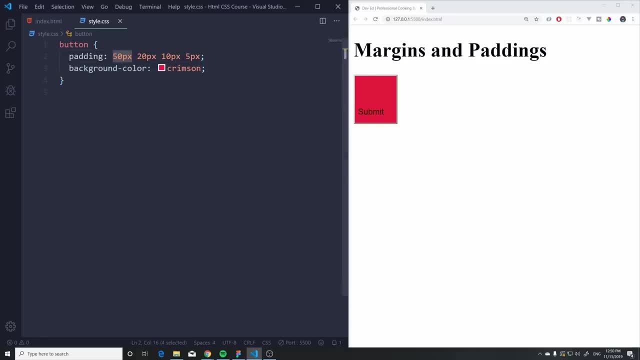 So the first one, 50 pixels, is going to be top. The second one, 20 pixels, is going to be right. So there's 20 pixels space here. The third one is going to be 10 pixels, here on the bottom. 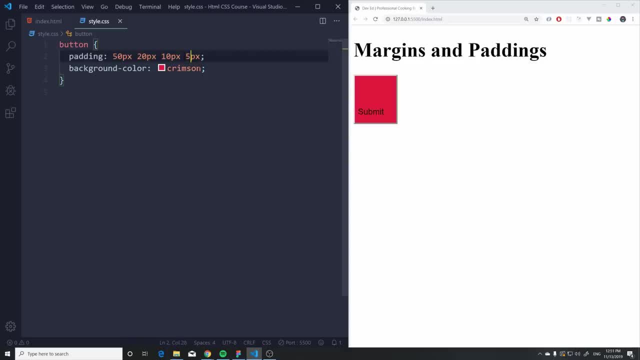 And 5 pixels here on the left. So if I say 0 pixels here, there's not going to be any additional space. As you can see, the button hits the corner perfectly there, So you just count from top all the way around. 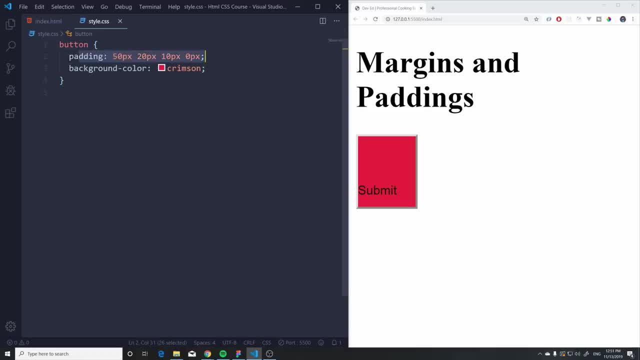 And that's how you can add it. So this is actually a very simple way of doing it. You need to wrap your head around it a bit. You need to drink your coffee first in the morning, And then it's going to click with you more. 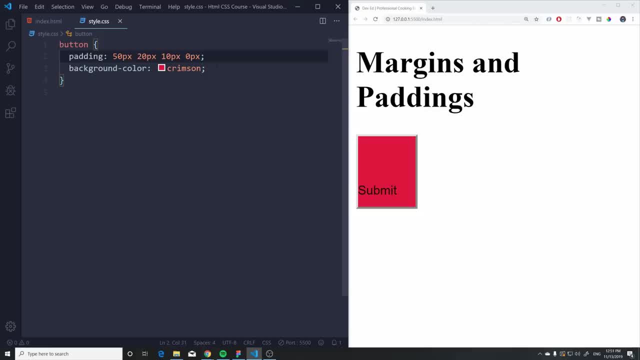 But there's another way you can do this Is by actually typing it out like this: Padding top, And then you can add 20 pixels, Or padding left And right and bottom and all the other ones. You can type them out like this individually too. 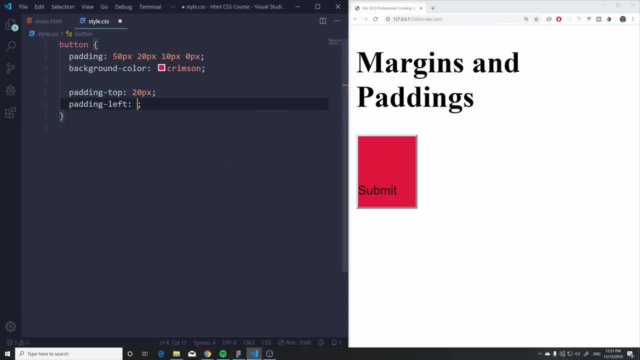 But this is a bit more. Let me change this so it kind of matches the one: up here, 50.. And then down here left, Let's do right, It's 20.. And then we have on the Bottom, we have 10, and then padding left is going to be zero. 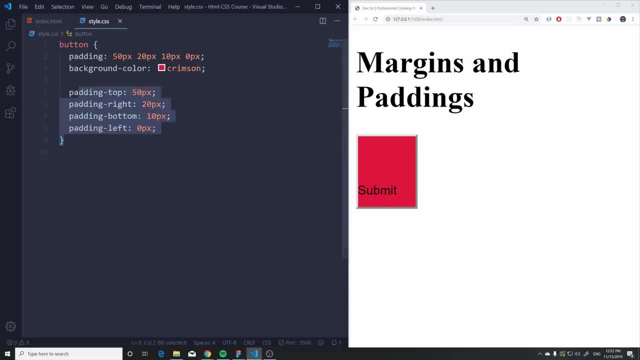 Okay, so take a look. This should technically override this up here. So if I remove this, it's going to be the same thing, as you can see. Okay, if I change this to 100, now this is going to change. 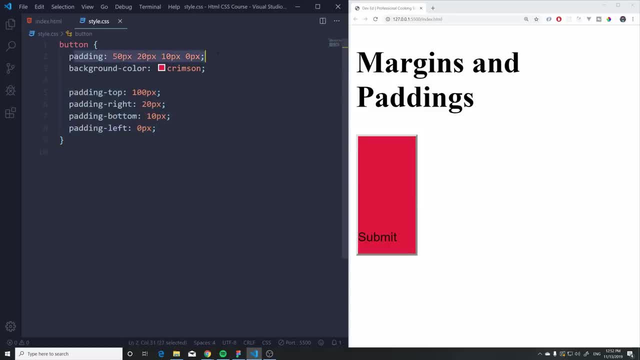 But take a look at how much code we write here and how much code we write here. So I highly recommend you to practice with this. And in case you don't need a property, maybe I just want to add 50.. Maybe I just want to add 50 top right. 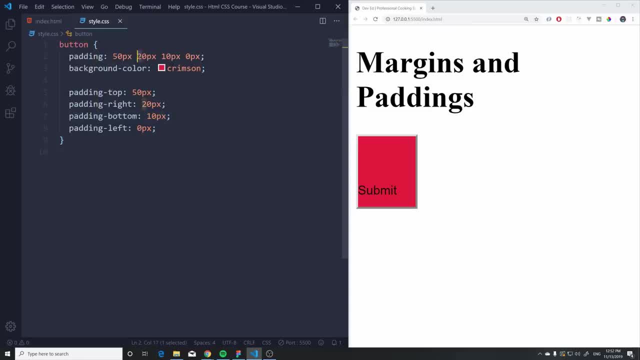 I want zero and bottom I want zero. I can just change these to zero, like this, And it's still going to work the same way, as you can see. Oh, never mind, I messed something up, So let's take a look again. 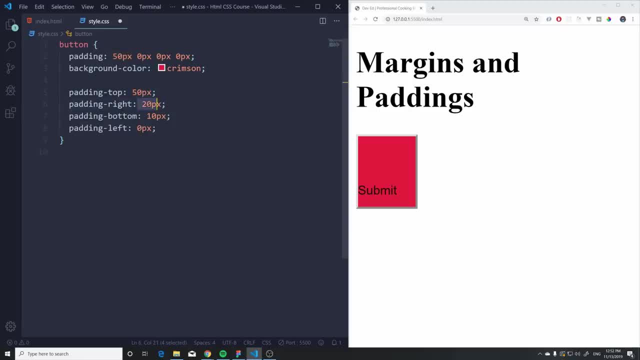 50 top. Okay, that's good, All right, So here it would be zero, because we have zero here and here is zero, And that should work fine. But in this case, if we only have one, then it's fine to just use padding top. 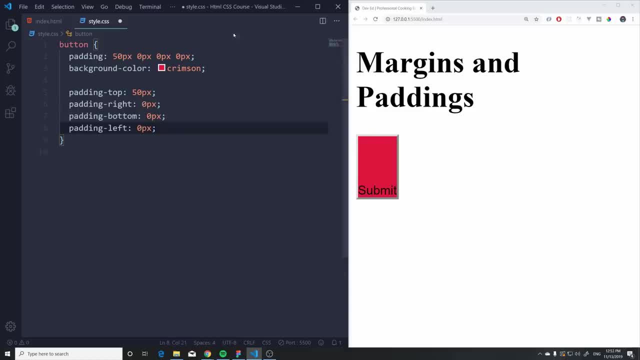 If you just only want to add it to one side. But generally you're going to see that you're going to use a lot of either one value or with two values, So either adding it everywhere or adding top, bottom and left and right. 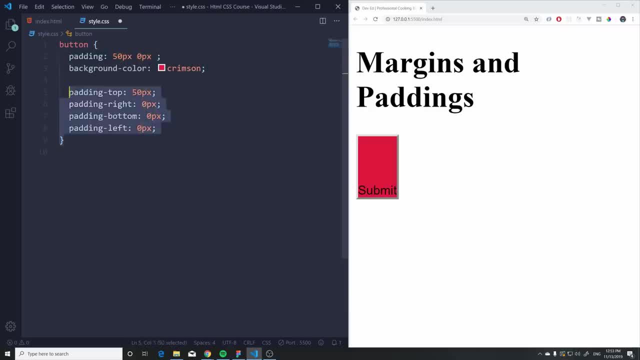 So this is top, bottom, and now it's left and right. Okay, So it's going to take a bit of practice, but it's okay because we're going to get a ton of it with these paddings and these margins. So, as you can see again, 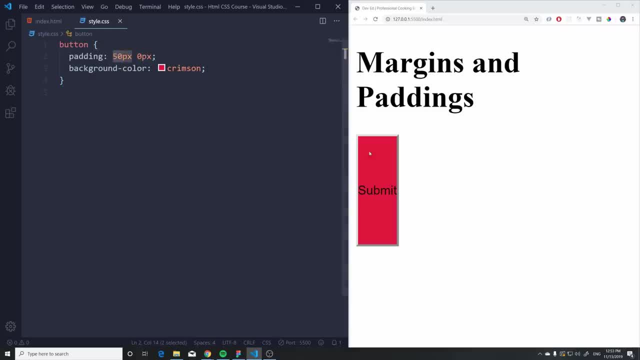 now, if I just add, have two values. the first one is going to be top and bottom 50, and on the left and right it's going to be zero. Okay, So it's not that complicated, It's quite simple. 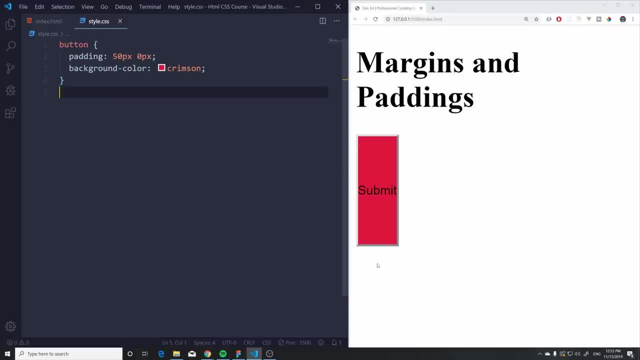 All you have to remember is that margins are going to be on the outside of the element, are going to add spacing on the outside and paddings are going to be added on the inside of the element. Okay, perfect. Next up, we are going to use the. we're going to explain the box model. 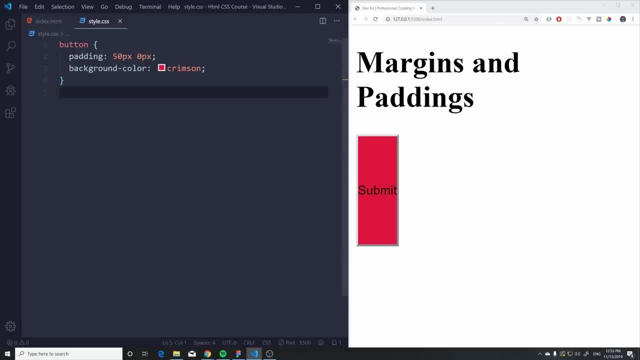 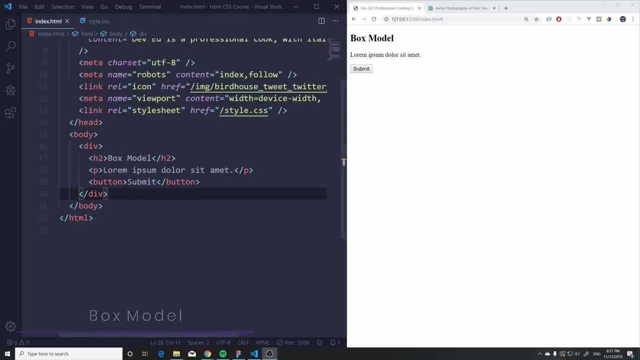 Tom, Tom, Tom. What's? Okay Box model? Well, you will find out in the next episode, so stay tuned. Okay, Let's cover the box model. Sounds so fancy, but it's not. this is something that you might not use per se, but it's it's very important to know about. 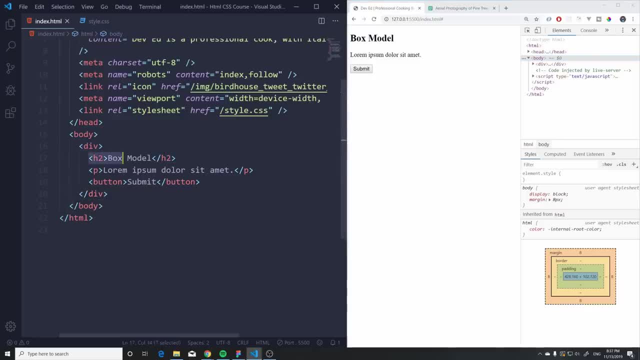 So all a box model is again. I just have a div here with a H2 AP and a button. All a box model is if we hover, if we grab this tool and we hover over all of these elements, you're going to see that you're inside. 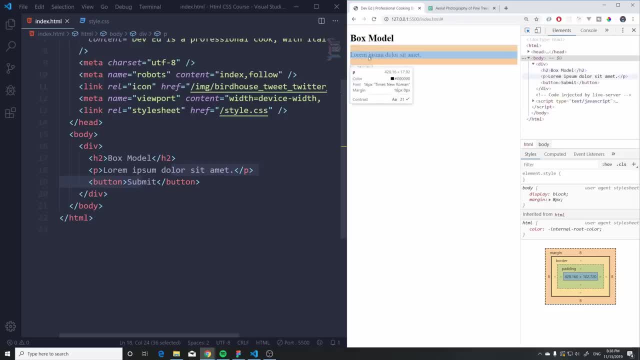 A rectangle or some sort of box. even this, even the P tag, even the button, has some sort of outline, uh, with like orange and different colors. Sometimes, as you can see on this button, if I zoom in, it has even green and everything. 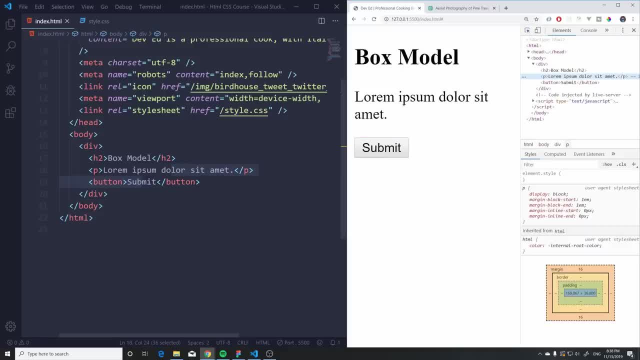 So what is that? Well, if we take a look, let's say, on this text, here is the box model. the blue part of the box model is the element itself. So the text in this case, right, Uh, padding, it doesn't have any padding. 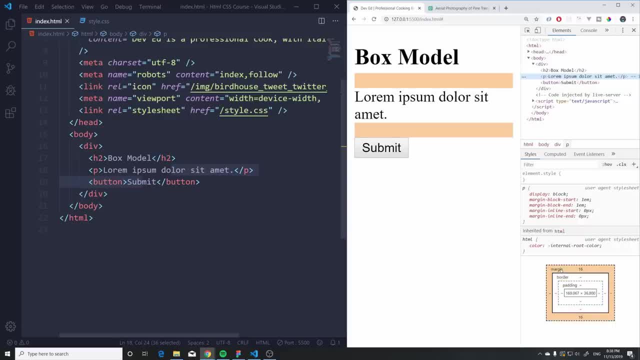 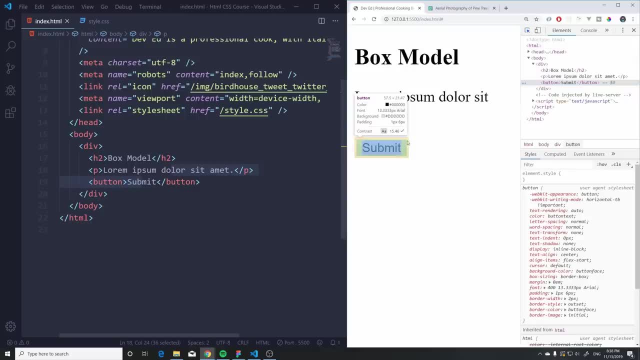 And neither does it have a border. However, it does have a margin, So take a look. Okay, Let's take a look at the button. The button has the border, which is that yellow. It has the green, which is the padding, and the blue, which is the text. 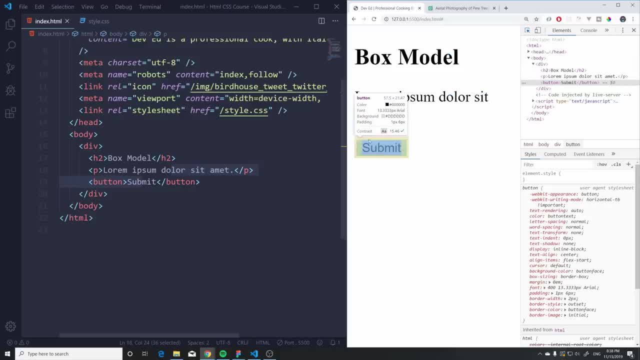 So that's basically the mob box model. All of these different properties bunched up together makes the box model: the paddings, the margins, the borders and the element itself. Okay Now, How is this useful? or why is this useful? 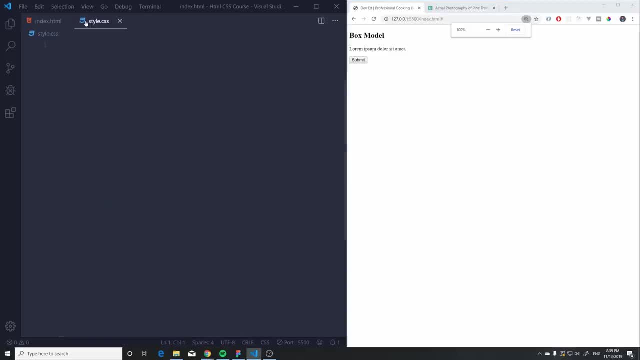 Well, it's just good to know about, because let me show you if I go to CSS and I just grab a diff here and maybe I just want to add a background color, or maybe I have multiple cards here, So let me kind of duplicate these a few times like this: 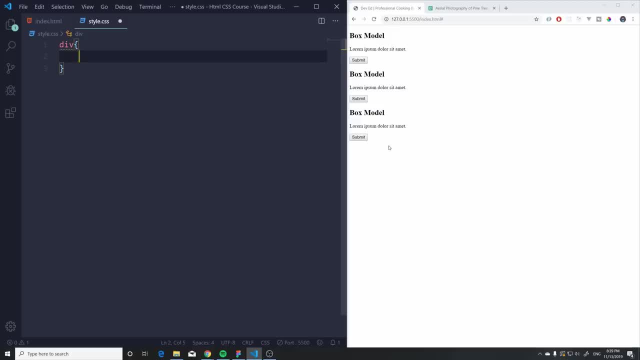 All right, I'm going to hit save and imagine like we have some sort of card system. Now we haven't talked about how we can position these elements kind of the way we want, but we're going to cover that in just a bit. 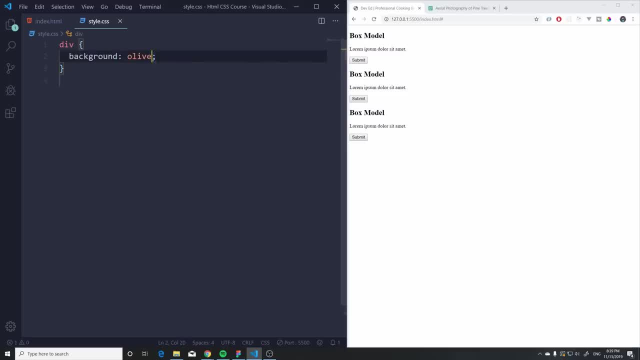 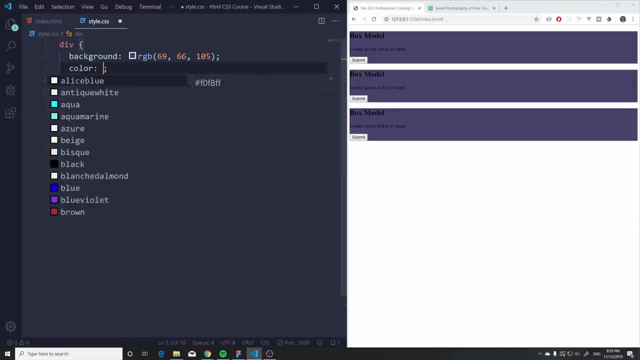 So let's just add a background Color to this. Let's go Nice, I wanted something beautiful. This is not gorgeous. Uh he, bluish, I love the bluish colors. and let's also add a color of white so we can kind of see the text inside there. 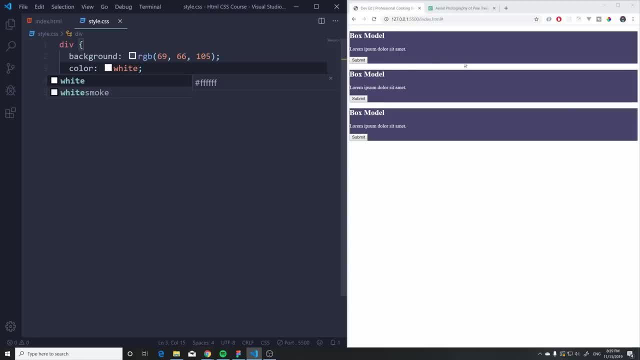 Okay, Perfect. So we have this. Okay, Now, what if I add and change the width of this? So maybe I just add a width of around- let's do 300 pixels, Okay, So it's this size, Perfect. 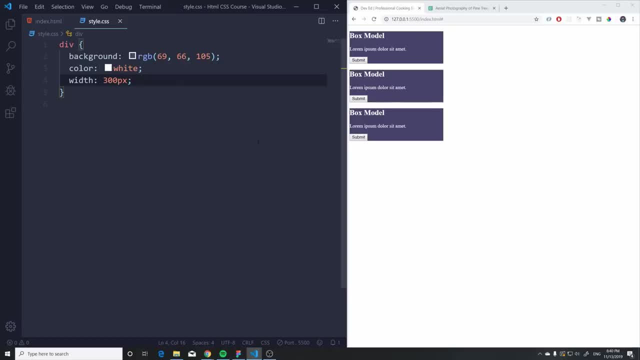 Um, okay, What happens if I add a padding to this? So I want to add the padding of 20 pixels to this. Well, Oh, okay, Hold on, The thing grew. the thing grew a lot, and sometimes this can be problematic because we might add paddings and margins in different places. 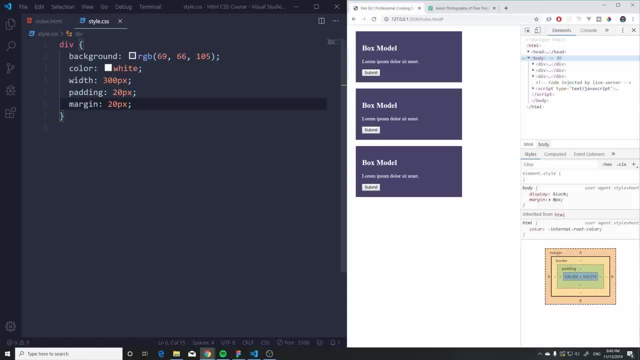 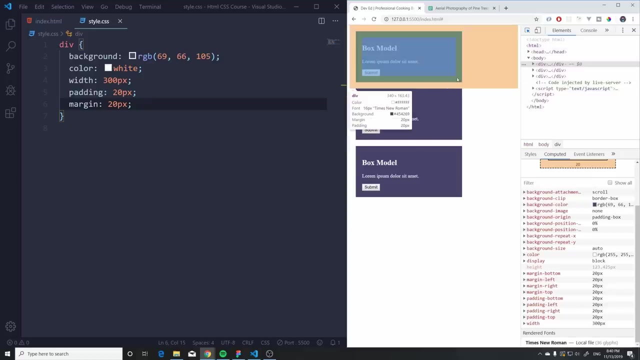 Uh, sometimes it might look good, but the problem is that the amount of pixels that are original box hat has changed. So if we take a look on the dev now, um, if we go over to the computed section here, you're going to see that. all right, let's see where. where can we see, um, the size? basically, what I'm trying to tell you is that, look at this, the size of the div grew. 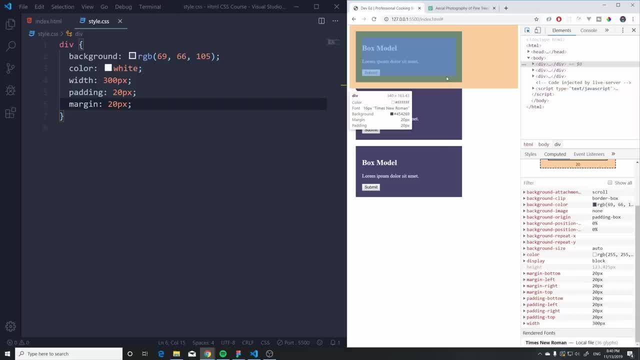 So, as you can see, it's 340 by 163 pixels, So that means that the padding that was added actually grew the element itself. So now Our whole box is way bigger than we intended, And sometimes we might want to have some fixed amount of sizes for these things. 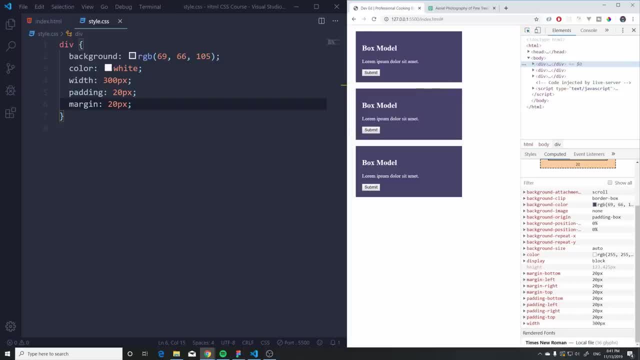 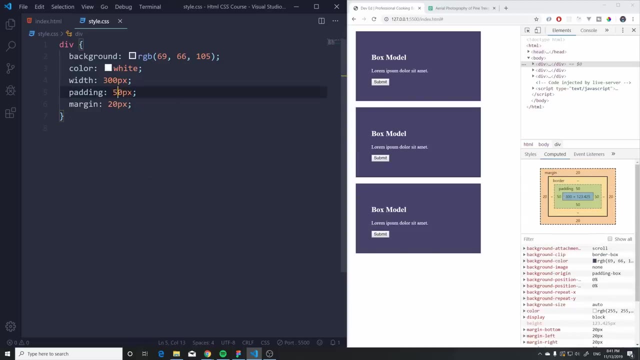 And this might cause a lot of problem because I might calculate something that should be around 300 pixels, But if I add some padding to it, it's going to grow. So, as you can see, if I'll make it something more dramatic for you, if I add something like 50 here, you're going to see that it grows a lot. 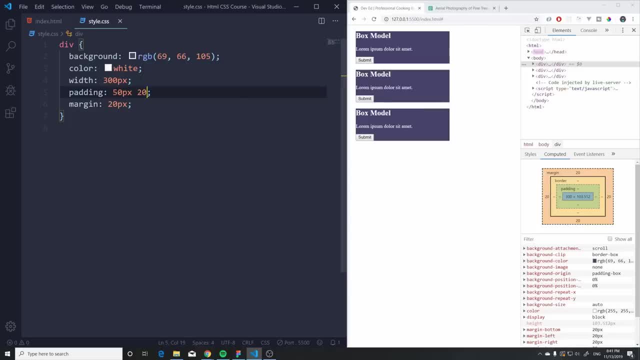 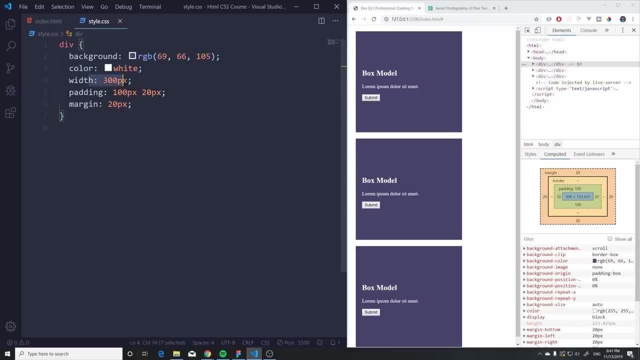 And let me just add the top bottom, actually like this: Um, let me add pixels here. So, as you can see, if I increase the size it keeps growing a ton and I don't want that. I just want to have this width precise here. 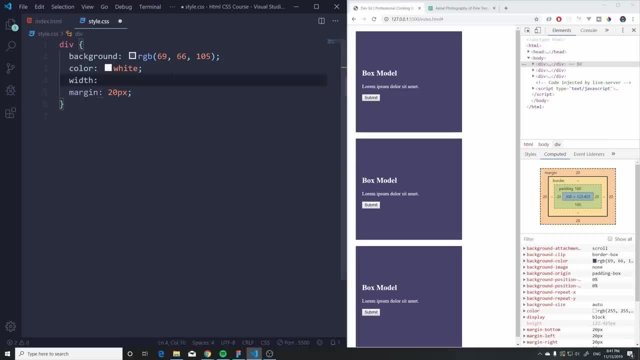 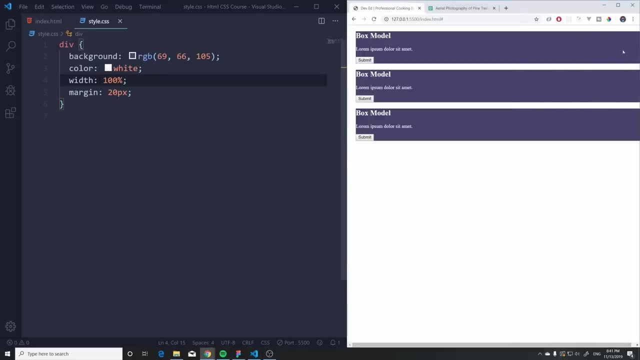 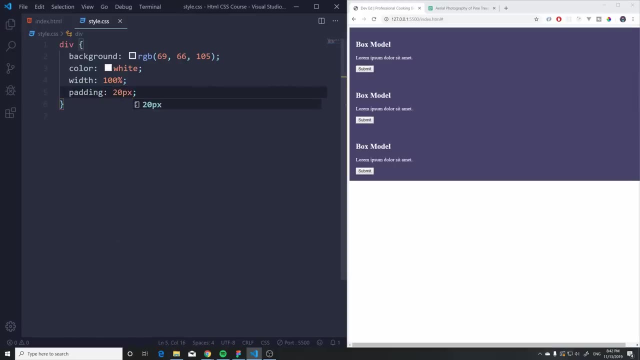 Okay, And we can also do this by: take a look, I'll give you another example. Maybe I add a a width of 100%, like this. Okay, perfect, Let me close this up. but take a look, If I add a padding of 20 pixels, or actually, we also have the margin, look my, my. 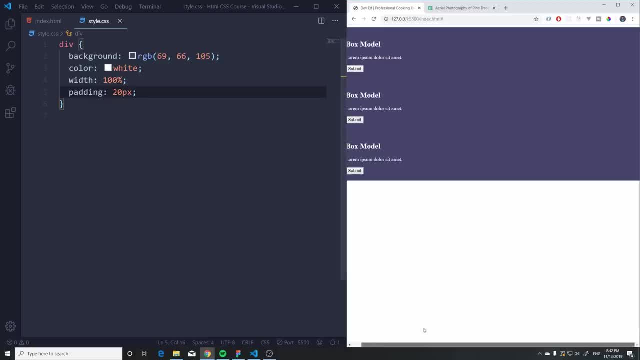 My scroll bar appeared. I don't want this to happen. I might just want to add some padding, So the text is not stuck there like this. as you can see, it's stuck there, So I want to just have some padding. but now the element grew. 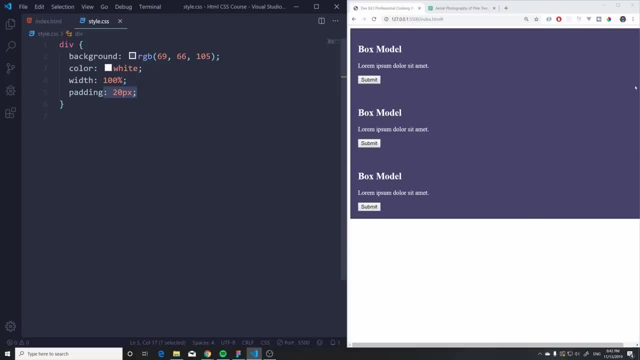 So of course, it's like a hundred percent plus 20 padding, All right. So that's why we can scroll this way. So there is a good fix for this, And I highly recommend you to do this. What we're going to do is we're going to grab all elements and we're going to remove all the basic stylings. 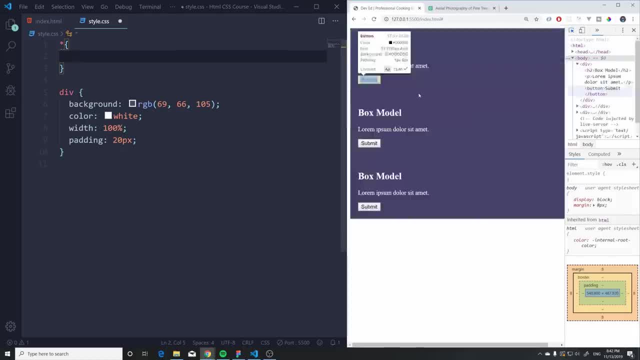 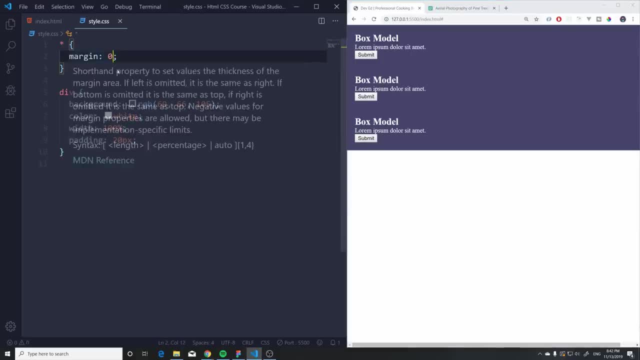 So the body has some styling on it with margins, as you can see, and the H one as well. So first of all, I want to get rid of those issues by adding margin zero. as you can see, now we don't have those empty, weird lines. 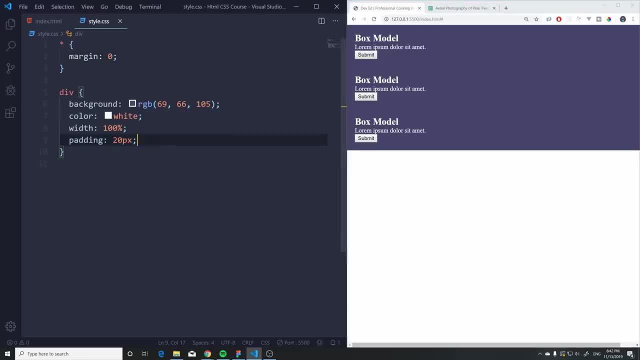 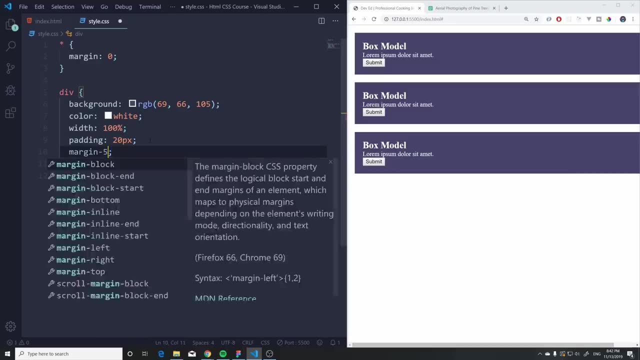 Okay. So that's step number one. Okay, Let's also add a margin- 20- to this, just so it's a bit more spacey. Uh, let's just do top margin, top. I'm going to do 20 pixels, Okay. 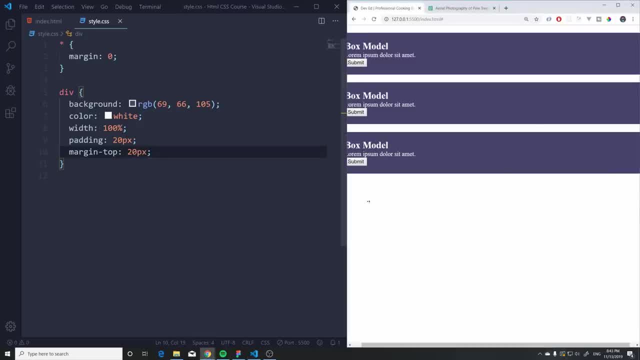 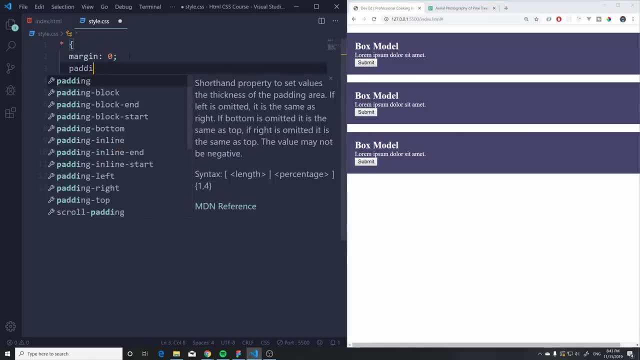 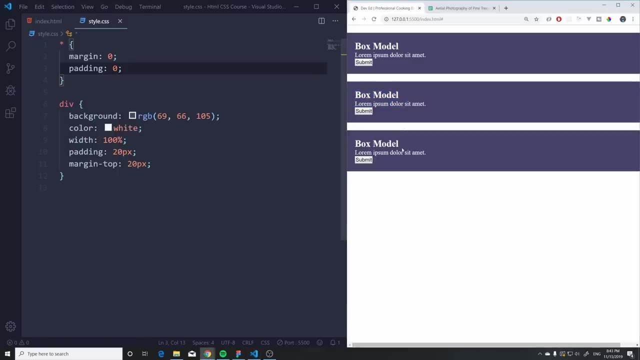 All right, there we go. That's what I want to have. Okay, We can still scroll, because the padding affects it. And now what I want to do is also remove additional paddings from all the elements, Just because the reason why I'm doing this is because I don't want the box model and the elements itself to control how I design my things. 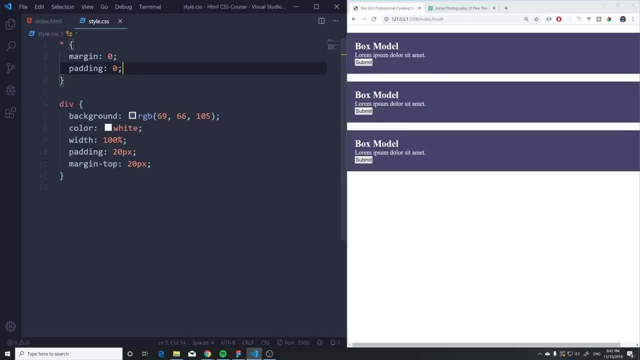 I want to start from scratch and I want to add it myself, but here's the property that's going to change everything. We're going to say box sizing, border, box, And, as you can see, now we cannot scroll anymore because everything that we add- all the paddings, all the borders that we add to our, our elements now- are going to be contained within. 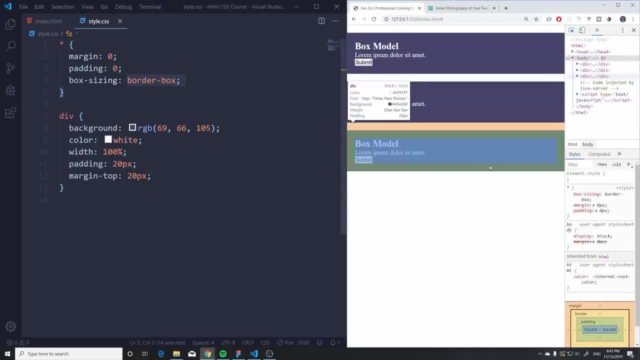 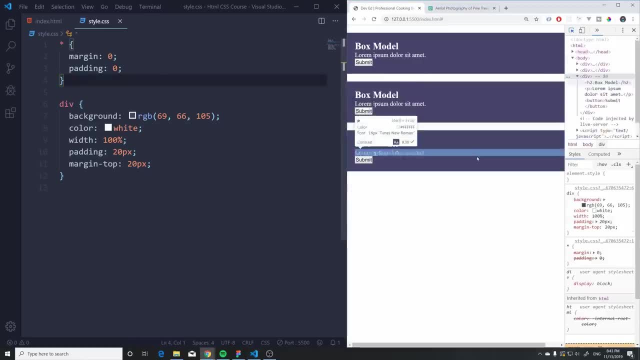 So if we check right now, as you can see, the padding is going to be on the inside, just like that. If I remove this, take a look, If I remove this, then we can scroll again, and that's not what we want. 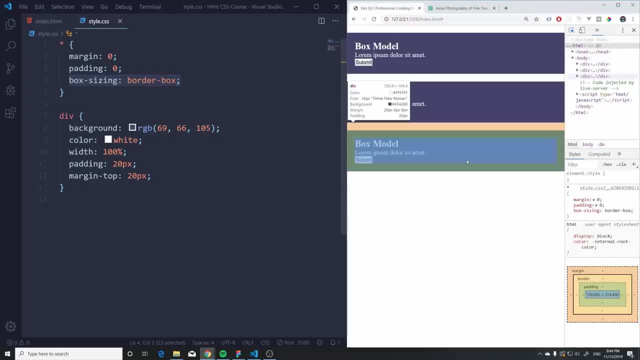 Okay, If we add this back now, we cannot, because, take a look, the element size, uh uh, stays the same. So another way I can illustrate this is if I add a width of something very large. So let's do a width of 300 pixels. 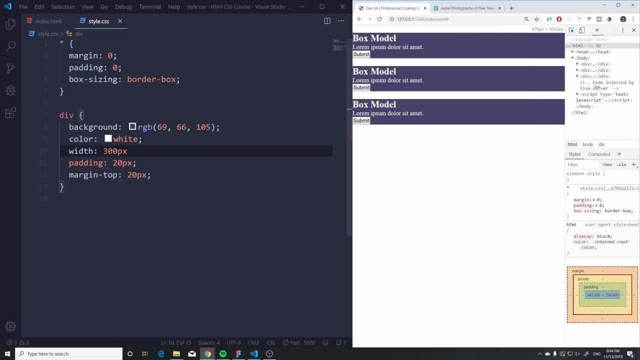 All right, 300 pixels, There we go. Uh, I cannot see this, but it's okay. So Let's take a look at these. What size of this if I close this up? oh, nevermind, I messed it up. 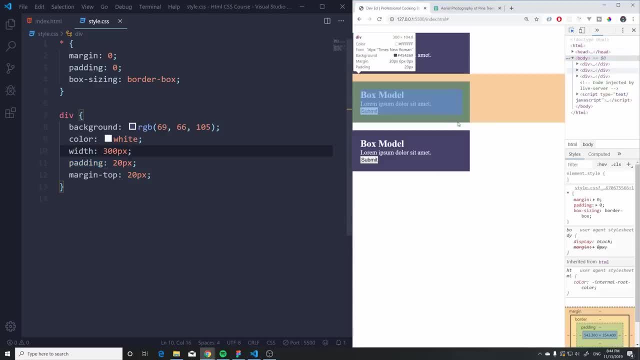 I didn't close this. There we go. Uh, now our element is 300 pixels long, Exactly how I want. even with the padding, it's not going to be a problem. But when I, when I start removing this box size, as you can see, it grew a bit and now it's 340. 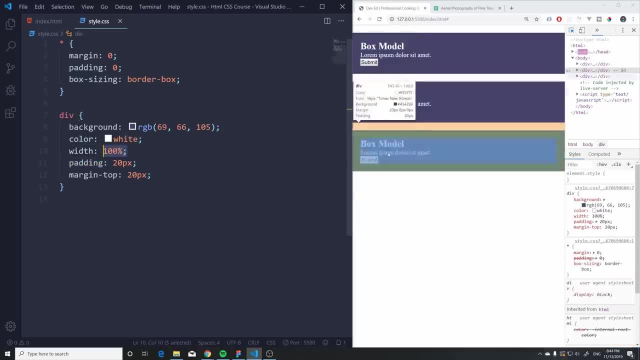 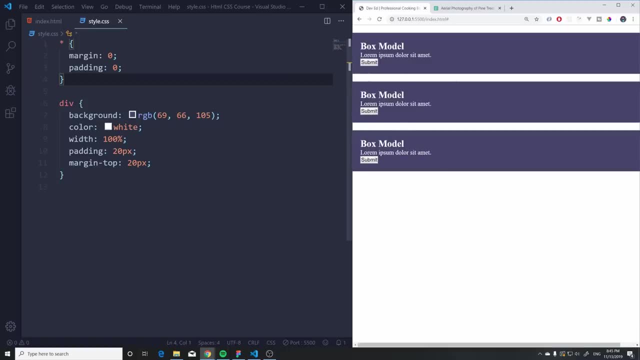 So that's a simple example that I wanted to show you. that can mess it up, Like the scroll thing where you might add some paddings, and then you're like: eh, why can I scroll on my website? Or why is My CSS behaving the way it is? is because the box sizing is, uh, set by default on content. content box. 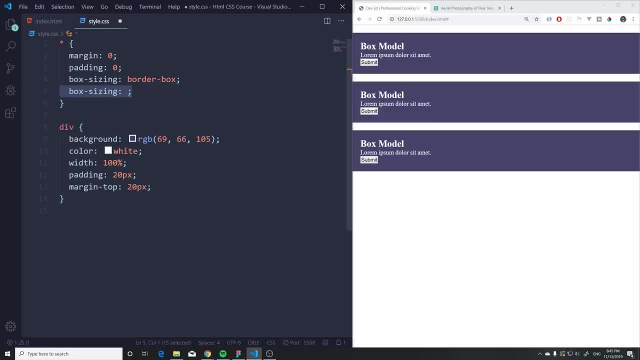 All right, And this can give us trouble because it's going to set the padding and everything and the borders on the outside. So I'll show you again. I'll show you another property with border. We can add a border of three pixels. 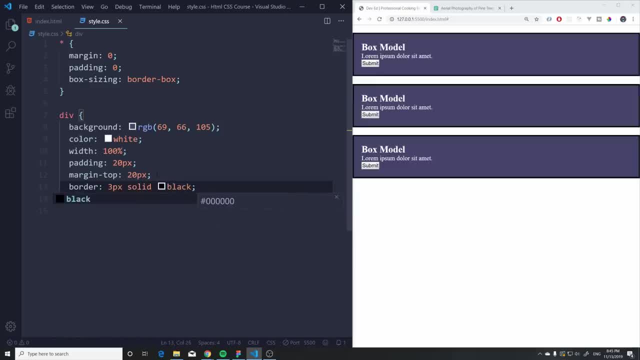 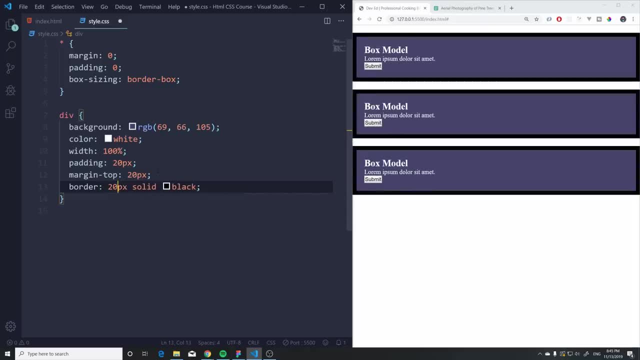 Uh, the second property is going to be solid and we're going to say black. Okay, So there we go. And now let's increase the size by 10.. So, as you can see, it keeps getting added on the inside. There we go. 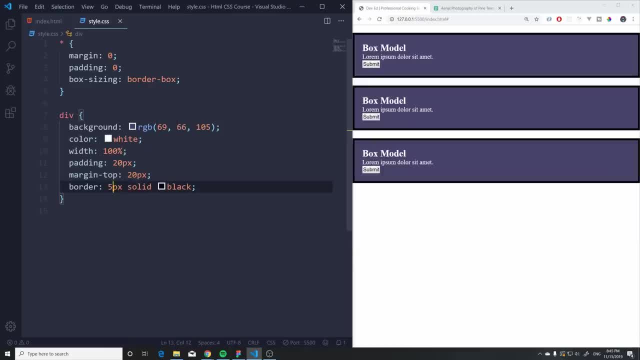 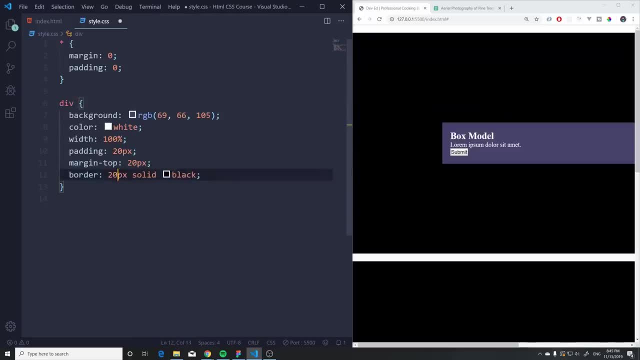 But if we go back to five pixels and we start removing this border box, it's safe. Let's start increasing this. Oh no. Okay, That's too large, Let's do 50.. Oh, look at that. Oh no. 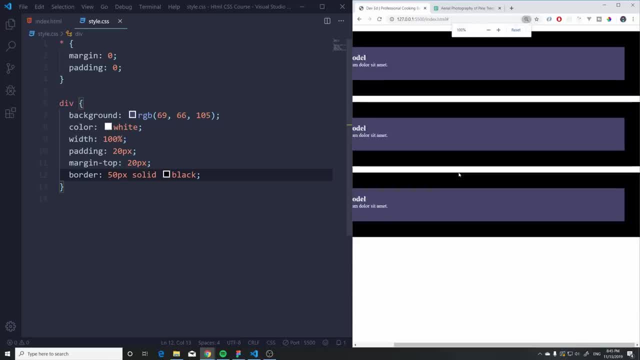 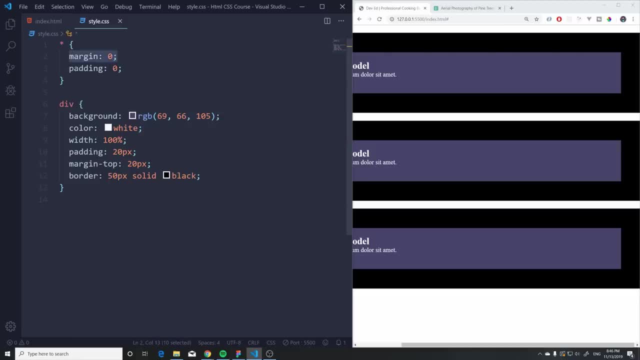 We are overflowing and everything is growing, So that's basically border box. Just make sure, whenever you are Starting out With your website or anything, just had margin zero, padding zero and add that box, sizing, border box- because it's going to save you a ton of issues. 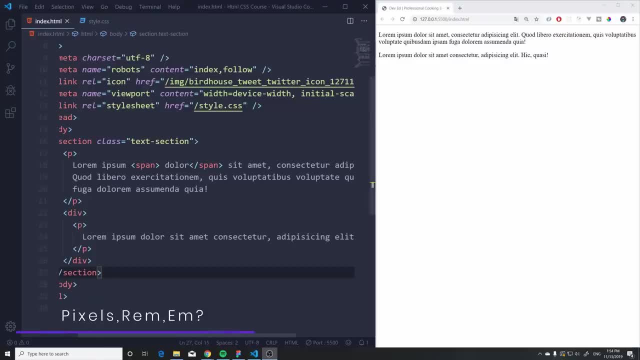 Okay, I promise you we are almost done with the boring stuff And in just a bit we are going to experiment with some more fun things you can do in CSS, such as adding images and backgrounds and creating some cool styles with some cool properties. 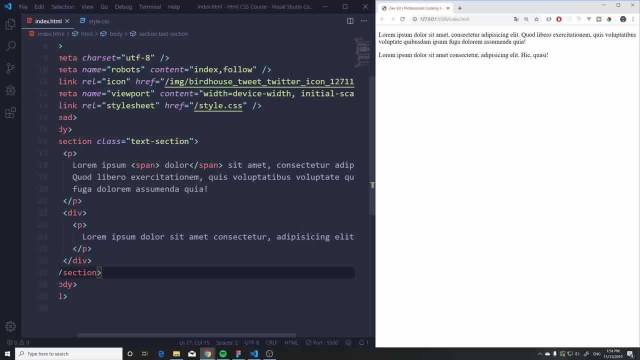 But there are a few essential things that we still Have to get through, unfortunately, but it's going to gratefully help you and make you understand what's really going on, because you're going to have some certain cases where you're going to be confused and you're not sure why your CSS is behaving the way it is. 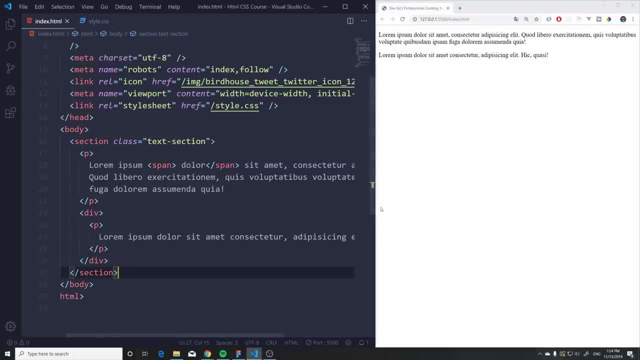 And these are some things that, again, we just have to go through, And one of them is the sizes of pixels and Ms and rems. So these units, what are these units and how are they behaving? So let me Quickly show you an example here. 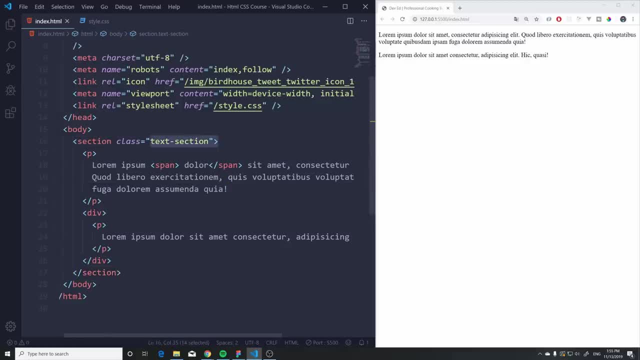 We have a section here. I just gave it a class of text section because it has only a paragraph, but I also created a diff here with another paragraph. Okay, So typically we've seen pixels and that's like most common pixels are everywhere. 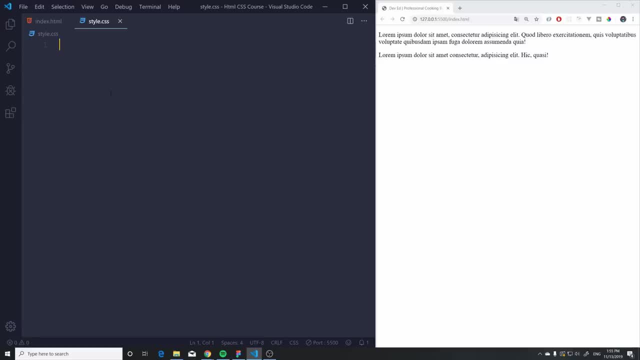 When they get the new iPhone gets announced, they tell you how many pixels, little pixels per inch, they have. So everybody knows pixels. So let's take that class And Let me kind of show you something. Let's put the class here. 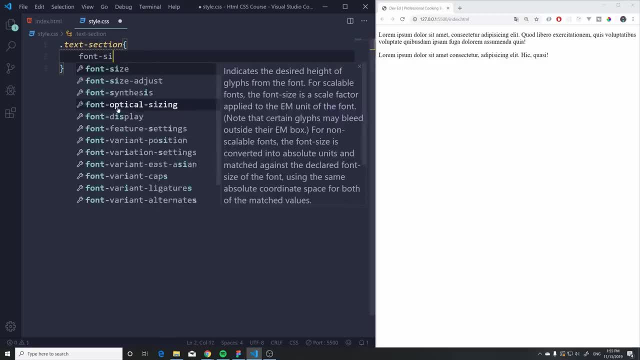 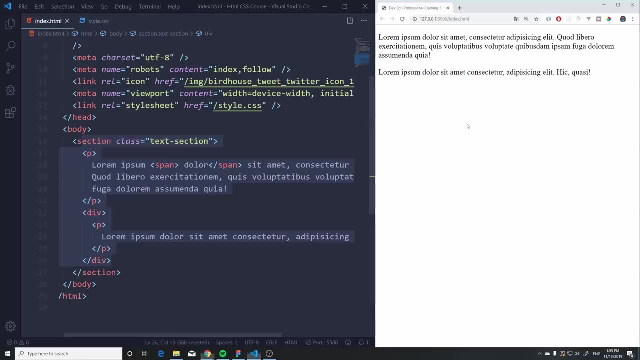 Oops, there we go. Okay, So if I set the size- a font size- of this to 20 pixels, well, everything is going to be 20 pixels, So all the paragraphs are going to have 20 pixels, and we can take a look at that. 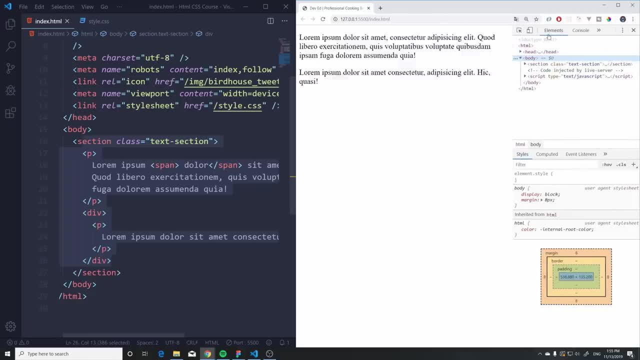 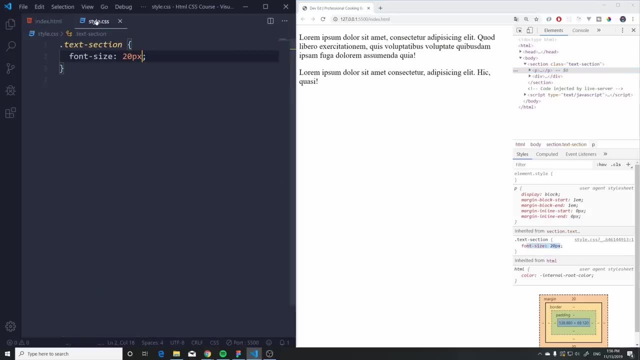 If we open up with F 12, this developer tools, and we click on one of these paragraphs, as you can see here, it says font size is 20 pixels. Okay, Very cool. Now The interesting thing is, I can go, maybe, inside this div and set this paragraph as well. 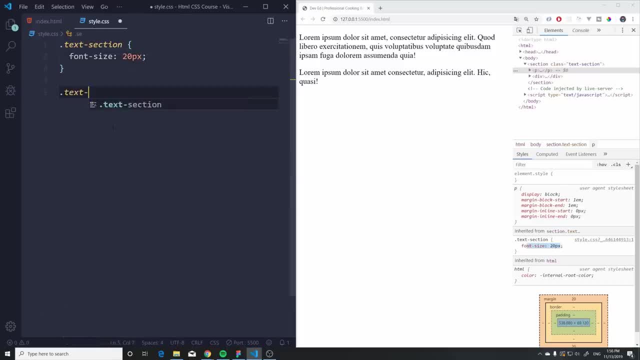 Okay, So we can say text section, div, so we can get this div and I can say font size of 30 pixels in here, So that grows this to 30 pixels, Okay, Well, cool, As you can see, Okay. 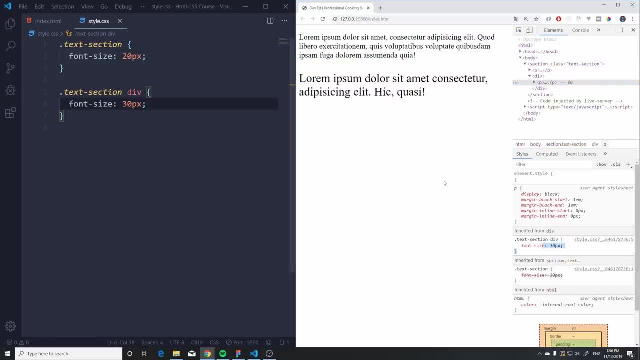 Well, we have 30 now here, Okay. So what's the problem with this? Well, there are a few problems with this, even though this might seem super simple. the problem is that, accessibility wise, this is not Might be that ideal. 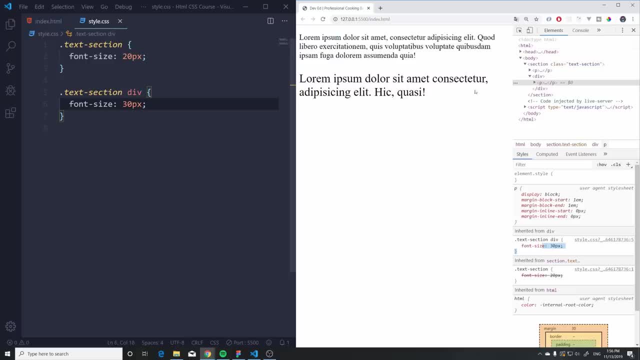 And I want to quickly show you this here, even though I have an accessibility section coming up later in the course. Um, this pixel that is set here is fixed, Can it? it cannot be modified, It's set in stone. So maybe if a user wants to change the size of their font in the browser because they might not see your text very well, maybe this text they cannot see it very well. 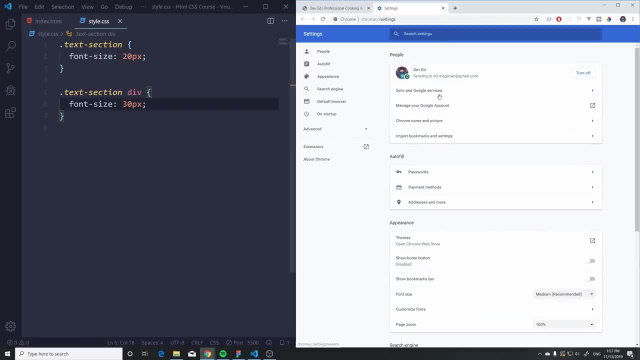 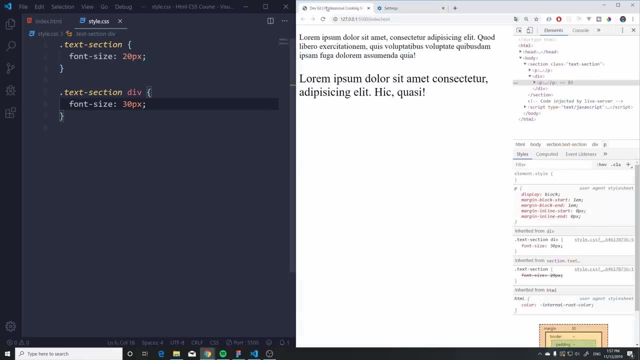 Well, if they go to Settings here and they want to change the font size, which I'm not sure where it is- Uh, it's here font size. If I change this to small, maybe? well, nothing changes Very small hopes. 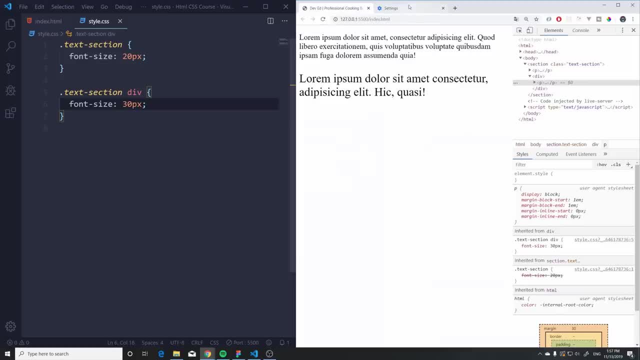 Very big. as you can see, nothing gets affected and that can be a problem And especially for people who use different font sizes and they might want to have some. they might want to have the text very easily, Be Easy to read. 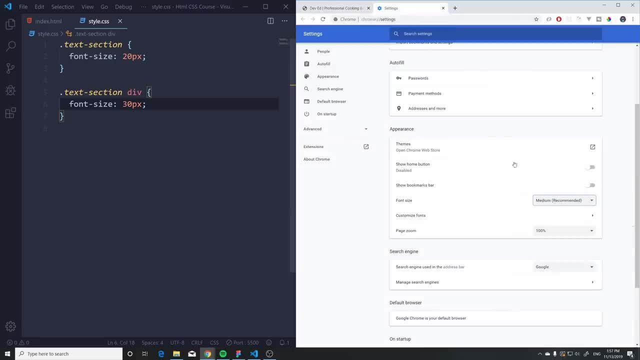 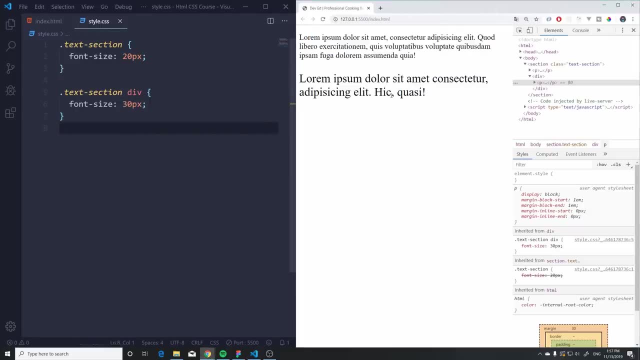 I need one for speaking too, because I cannot speak. So accessibility, wise pixels- is not that great of an idea. Also, it's not a great idea for responsive design, because you have a fixed set of value. here You have 20 and 30.. 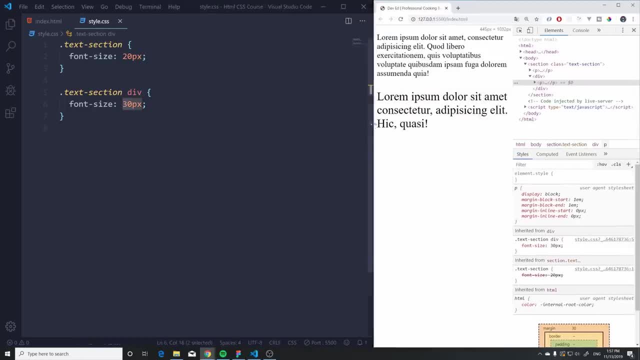 So maybe if we go on mobile, so if we go smaller like this, we have to do some tricks to change each and every value to match a mobile screen font. So you might have Modify this section and this section to get the results we want. 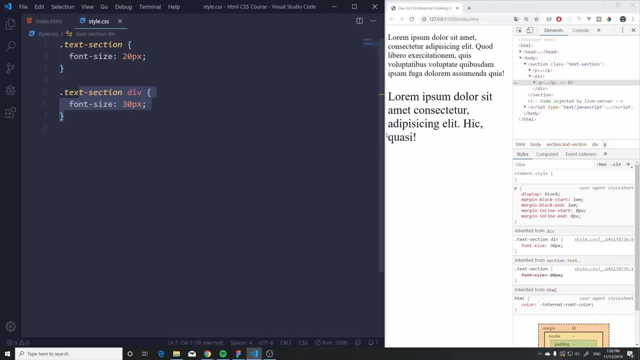 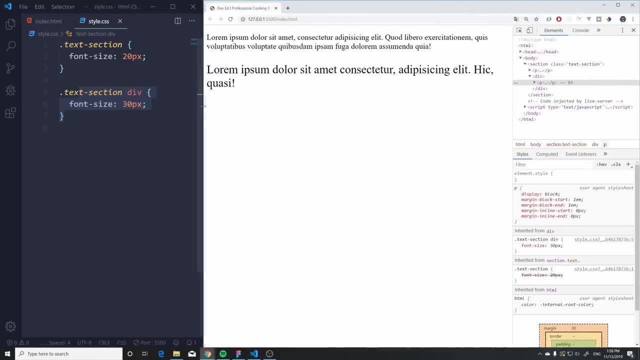 Again, we're going to get into that and later a bit uh, when we cover media queries, which basically just allows you to change all your elements based on the size of the screen. So basically, when you go to mobile, you can change the font sizes. 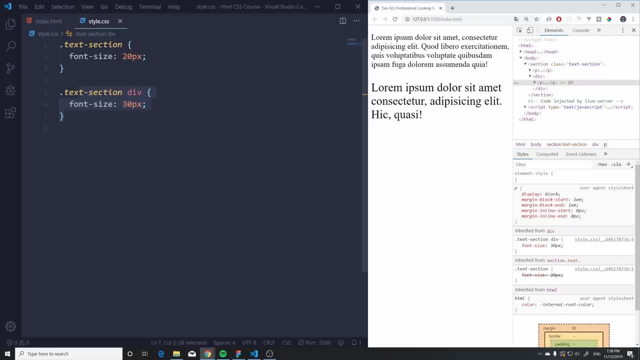 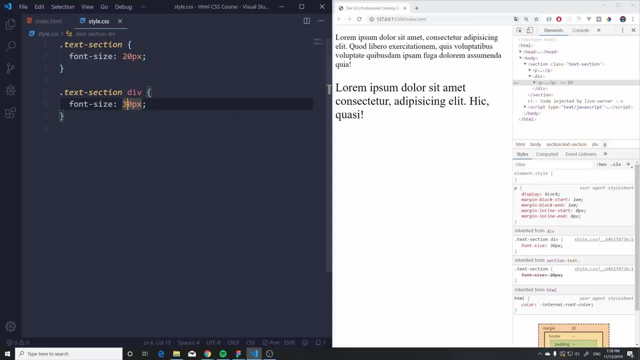 You can change the styles, the colors and everything else. So pixels make it a bit tricky because you have to keep changing them, because they're fixed. So another alternative That we have is Ms. So Ms units are written like this: Let me quickly show you, let me, let's get rid of everything. 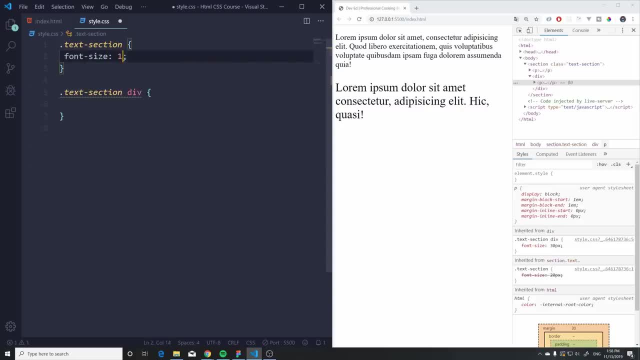 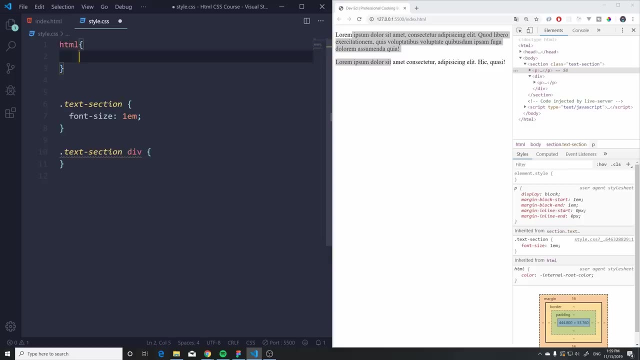 I'm going to say font size, one M all. right, Hit save And by default that's going to be 16 pixels. And- and there is actually a secret little bastard here that we don't know- but HTML sets the pixel size and HTML, by the way, is the root element. 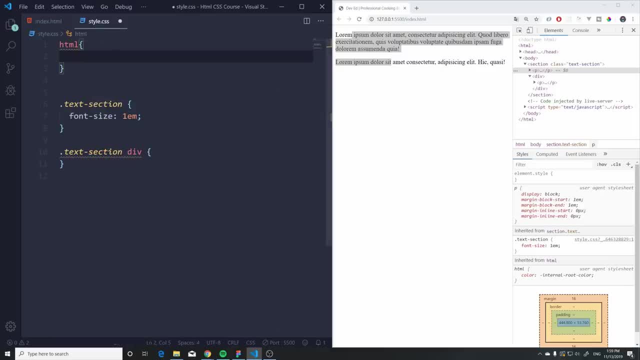 Of our website here, So this one. it gets set by default to a font size of 16 pixels. Okay, We cannot see this, but this is happening kind of behind the scenes And, as you can see, if I save it, nothing really changes. 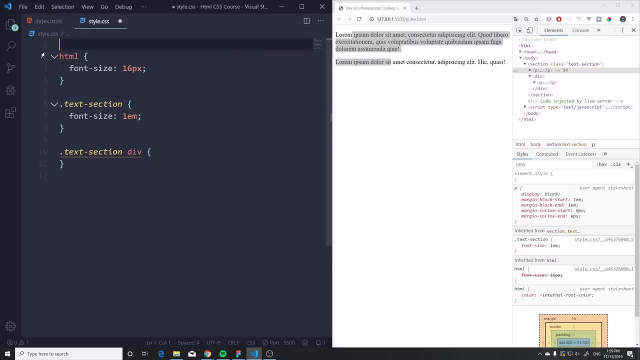 Uh, so I'm going to comment this out, and I didn't show you how you can comment things out in CSS, So let me show you now. you just basically add a slash and a a star sign and everything you wrap inside This. 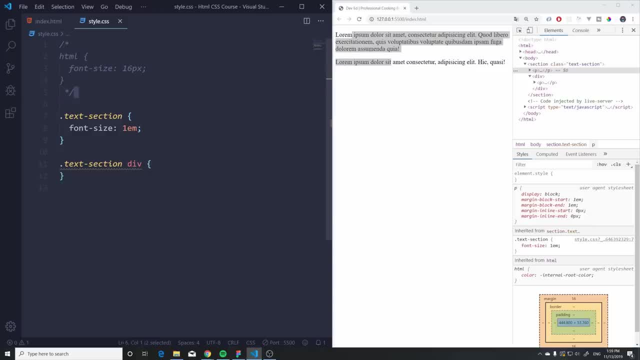 Slash, star sign and then star sign. slash basically doesn't get executed in your code, Okay, So if I want to wrap this, uh, the code is not going to work anymore. Take a look. Okay, But this is actually the default. 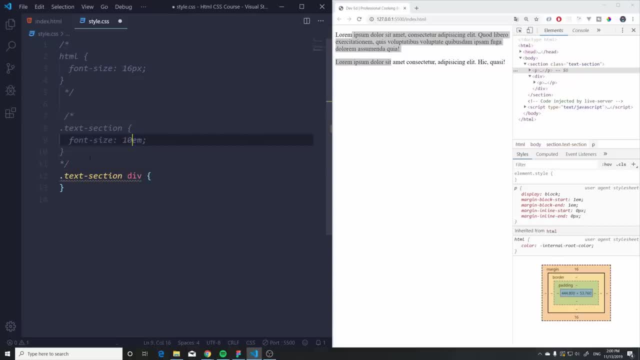 So if I change this to something like 10, nothing happens, Okay, So let's go back, Let's get rid of this, All right. So it's 16 pixels, Very cool. So if I want something like 24, uh, I can set it. 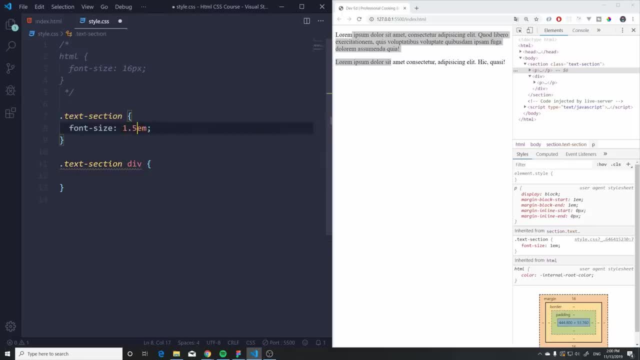 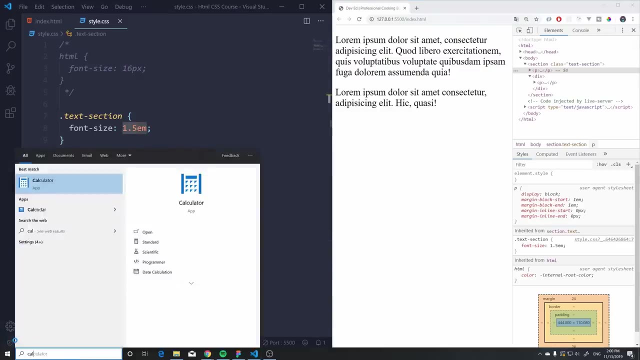 To 1.5, right, And then we get 25 pixels. There we go. Okay. Now the cool thing is, if I did that calculation correct, uh, you do 16 times 1.5, and then you get excuse myself, excuse me. 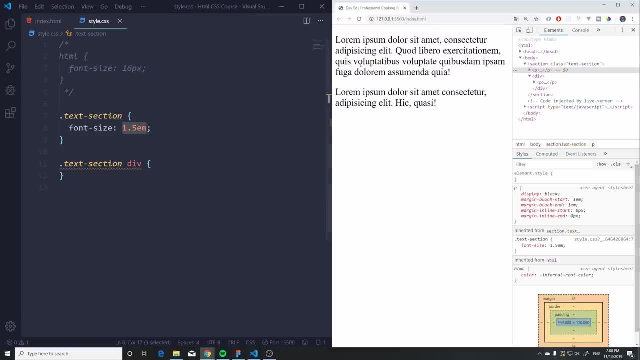 All right, Okay, We good, We good. It's 24, 24.. Okay, So, basically, you multiply everything by the element. Okay, That you have, So the the parent element. So, Ms, basically take a look at the parent element. but I want to show you where it gets a bit tricky. 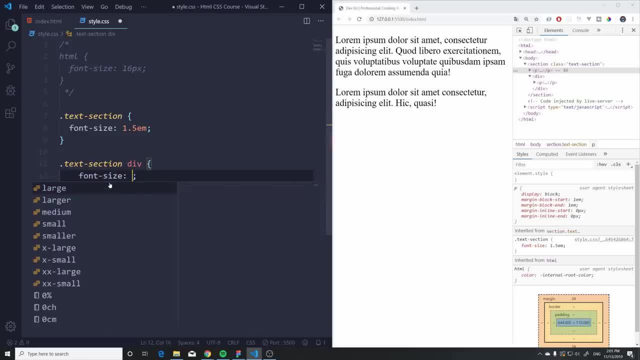 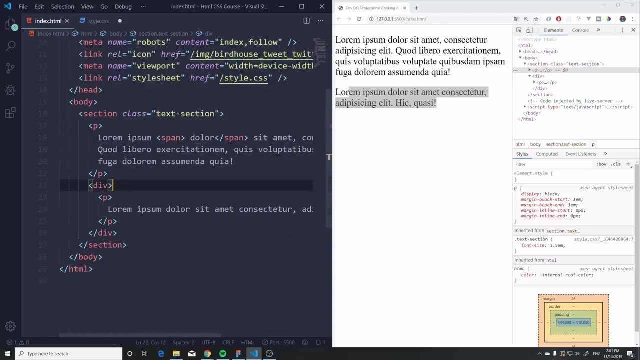 If I go here and I want to say, maybe I want to have a font size and I'm going to say 1.5.. Okay, It's going to be the same font size, this one which is kind of uh, useless to add, to be honest, because we already defined it up here. but I just want to show you the difference. 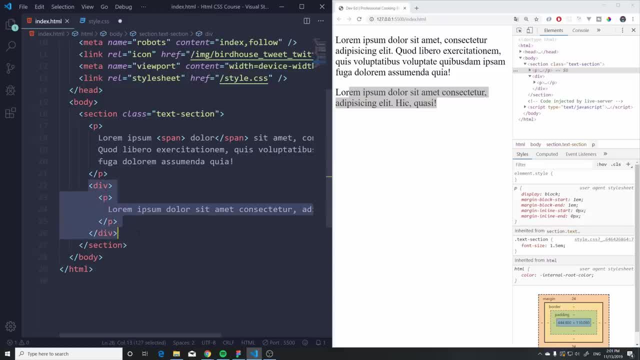 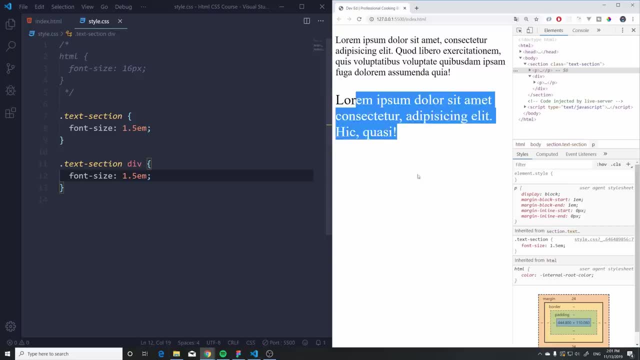 Okay, So basically, I'm going to add it to this P tag. So then the div and this P tag. if I add a 1.5 M, well, why is this bigger? now, What M does is it- takes a look at the parent element. 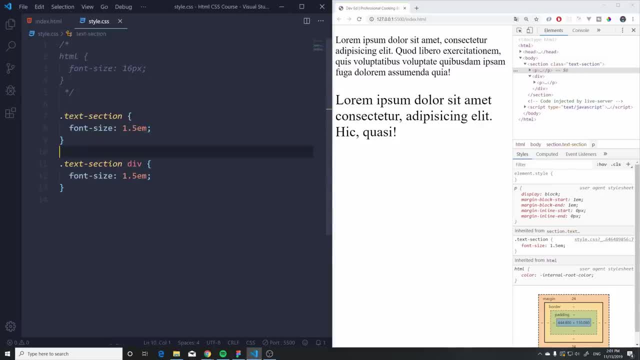 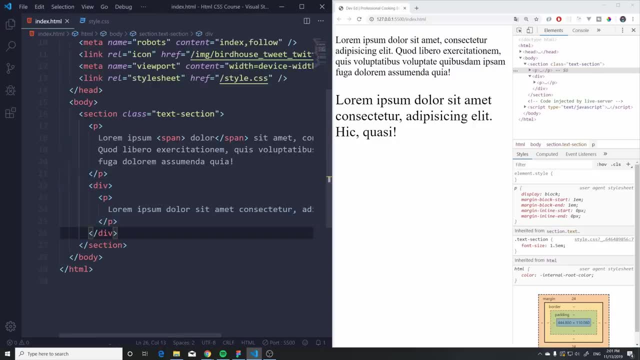 So it takes a look at the parent element and it multiplies it. And then this parent element takes a look at its parent element and then multiplies it. So take a look What happens. We added 1.5 M M to this and it's going to be like: okay, I'm going to multiply it by my parent elements. font size. 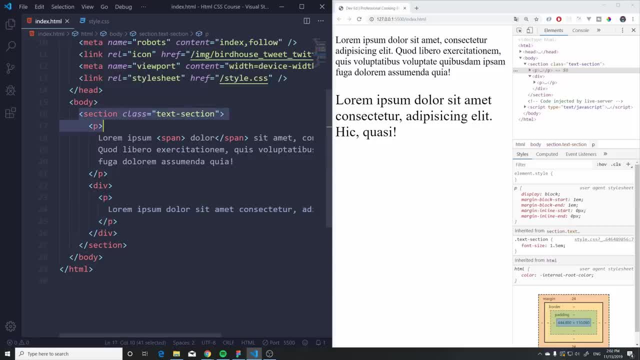 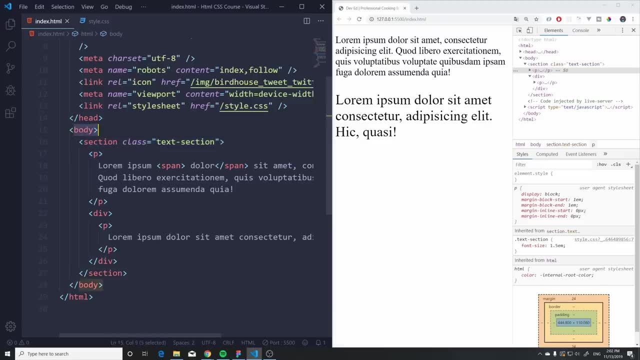 So it's going to take a look at the section and it's going to be like: oh, you're 1.5.. Okay, 1.5 times, 1.5 times. what's the parent of this element is the body, and what's the body's parent? it's HTML, which has the default size of 16.. 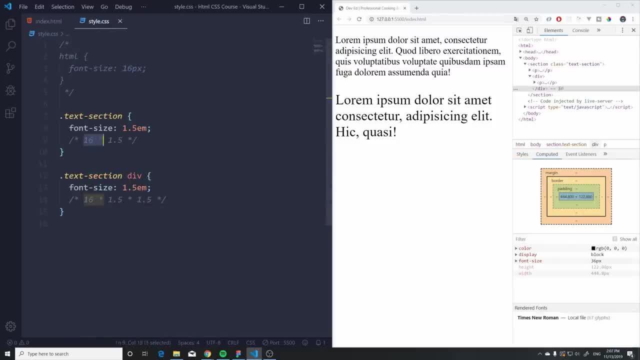 So this is what is basically happening: You add 16 times 1.5, because it looks at the root element and then down here It adds 16 times 1.5.. So the parent and then this element that we gave it here. 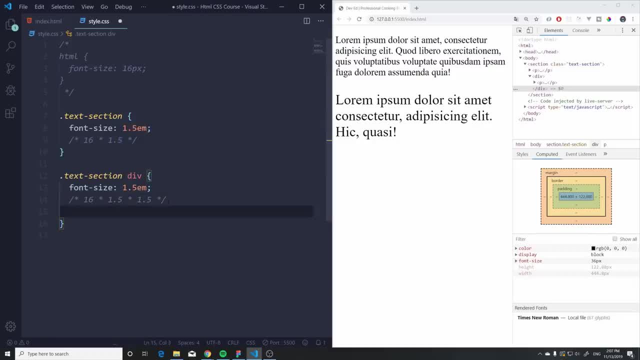 Okay, Now check this out. This is kind of interesting. What if we add a margin top to this div? let's have one M, all right? How is that calculated? Well, let's look at the div. As you can see, the font size is 36 pixels and the margin top is 36 pixels. 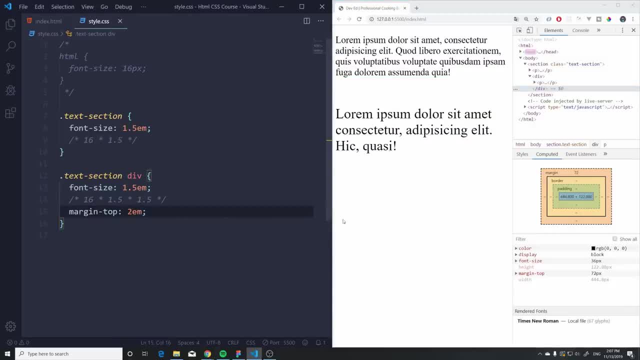 But what happens if I change this again to something like two M? well then it's, it's 72. So now you have to say 16 times 1.5 times 1.5 times two. All right, So hopefully this is getting clear. 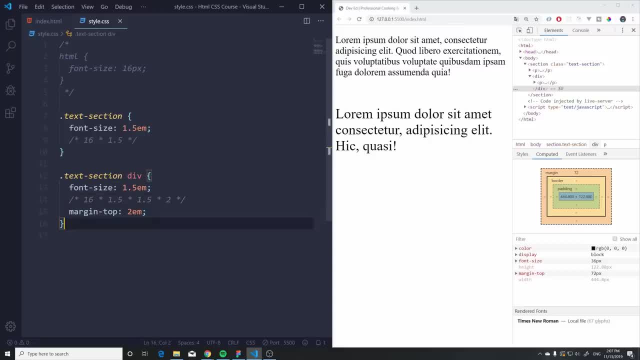 You just keep adding more and more and you're duplicating more. So now it takes into consideration this, this and this times, this, All right. So wherever you have defined a font size, you're going to have to keep multiplying, and this is going to get quite crazy. 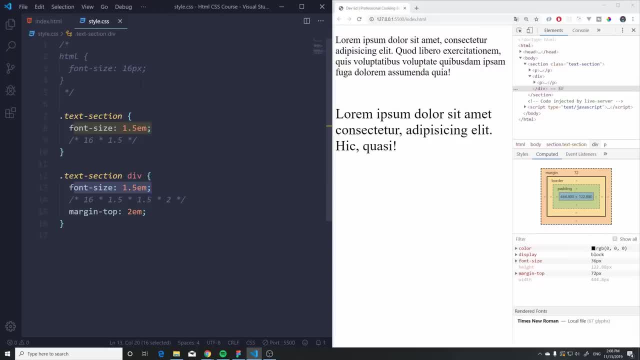 And, as you can see, it's it, it it makes things not fun. Okay, I never used this, by the way, So you can catch a breath right now. You can sit back, you can watch this, enjoy it. 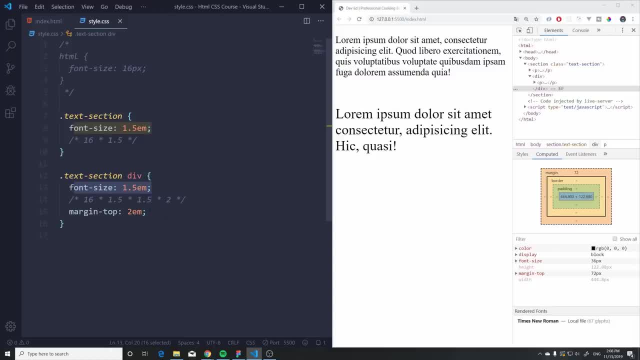 And knowing that you're almost never going to use this. but I want to make make it even weirder for you. If you want to break this, you can just add a font size. If you set a pixel font size, then it doesn't inherit it anymore. 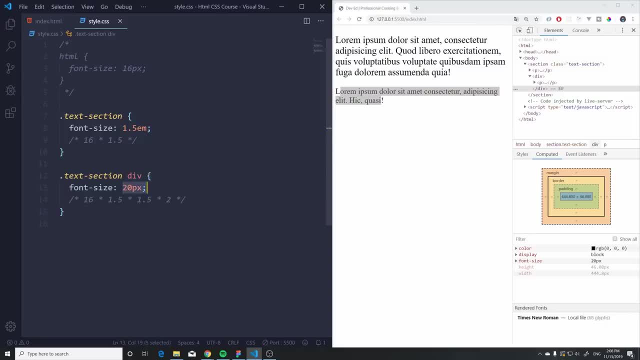 Okay, But if we change this to equal A font size like this and then we add an M unit, So margin top, let's do two Ms again, Now it's going to inherit only this one. We're not going to be doing the multiplications anymore, because if we set a pixel here, it's going to destroy that inheritance. 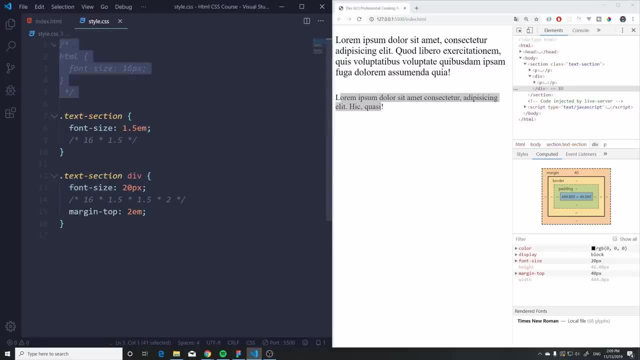 It's not going to take a look anymore at the parent if and the parent of the parents div. So now it just looks at: okay, it's 20 pixel times two, Okay, Oh, my goodness, This is so confusing, Okay. 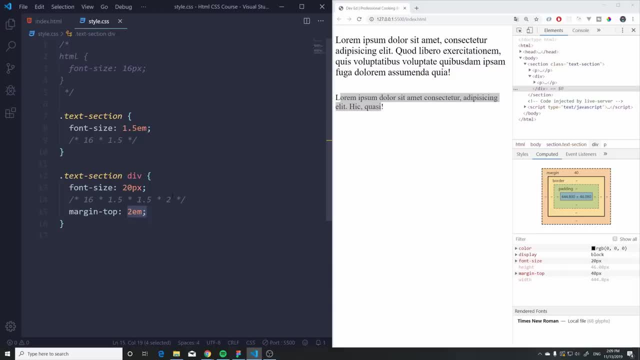 Don't worry, because we have a new unit here to the rescue. We have something called REM, and the only difference between the REM and the M is that we are not going to inherit from parent to parent to parent. We are only going to inherit from one single one, which is the root parent, which is this HTML element. 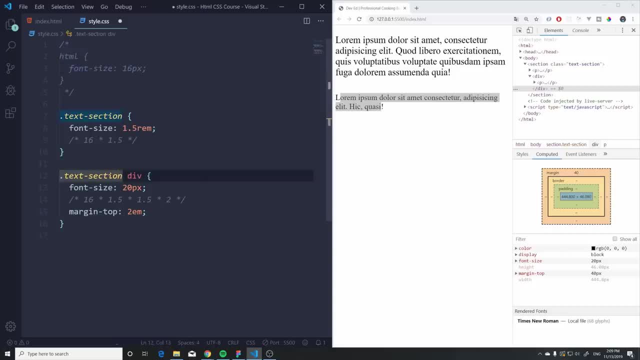 So when we set a REM, It's only going to take A look at this HTML font size. Okay, So let me show you how this clears everything up. So simply, we can go to the text section and maybe I want this to have 16 pixels. 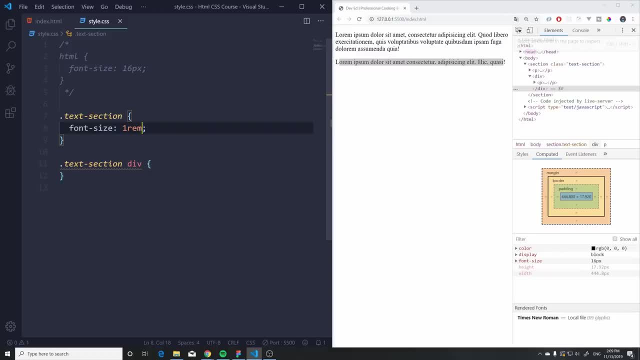 So I can set the font size of one REM. If I hit enter, we can take a look. This has, this has 16.. So if I want 24, I put 1.5.. Okay, So now it's 24.. 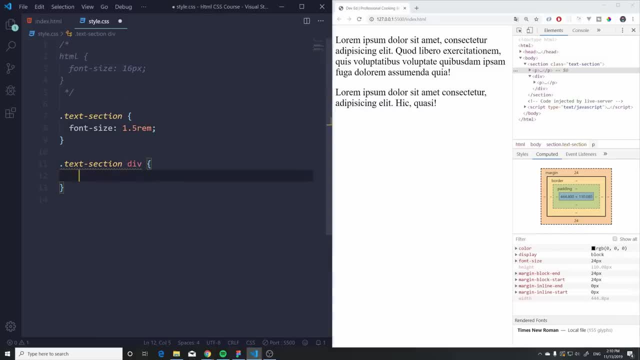 Okay, But maybe on this one I want to change it to something bigger. Or maybe accidentally I put it the same size: 1.5 REM. It doesn't matter, because this one exclusively looks at the HTML and this one still exclusively looks at the HTML. 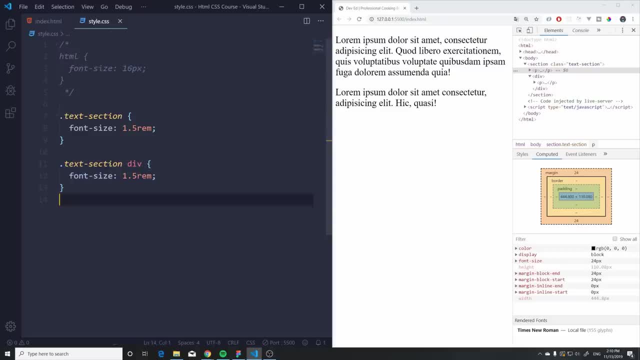 So only at the root, we don't have to worry about taking the look where this thing is nest nested. Where is it here, Is it there? It doesn't matter. You always going to know that whatever REM you put here is always going to be relative to the font size of the HTML. 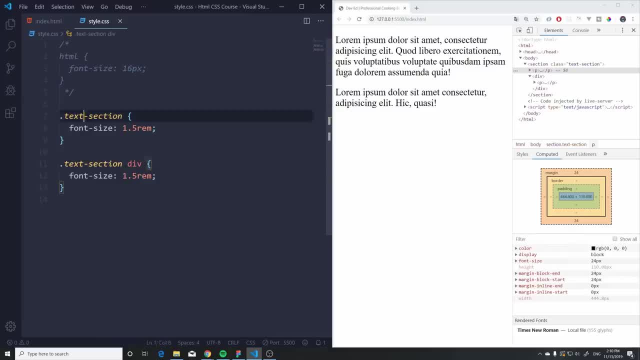 Which makes it actually super easy. You know why? Because we can modify this HTML. So if I remove this HTML I can set a font, a specific font size here, so that this REM calculation is going to be easier, because right now 1.5 REM is kind of tricky to calculate, right? 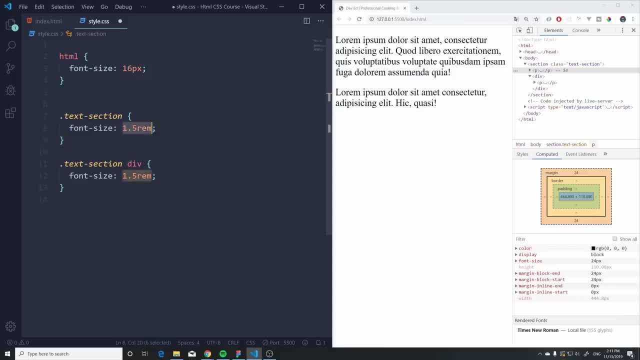 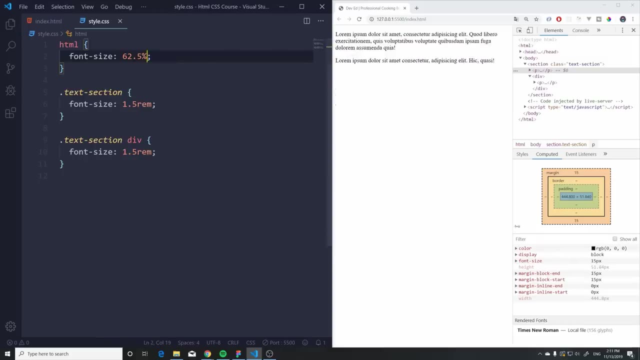 You have to say: okay, so what's 16 times 1.5?? So that can get a bit annoying. So what we can do is set a percentage here, Okay, Okay, So 62.5, I believe 5% like this, which is going to give us exactly one REM is going to be exactly 10 pixels. 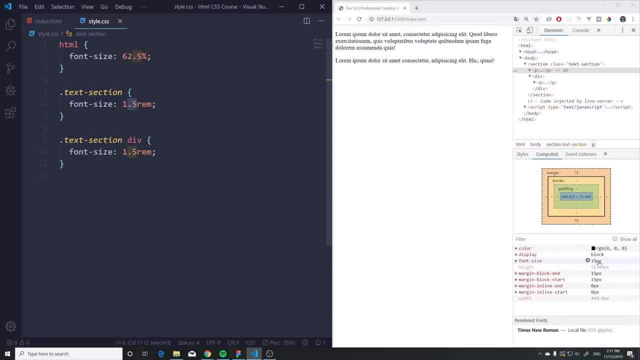 As you can see here, 1.5 is exactly. we're going to be six, 15 pixels. So this way we can style everything the way we want. I can come here If I want this to be 16 pixels, I can just say 1.6, REM boom. 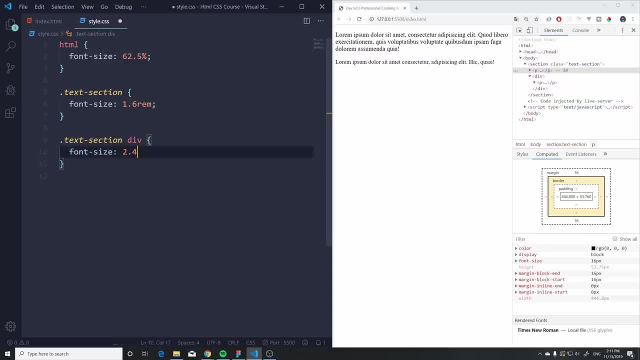 We have 16, maybe on this dip I want 24.. I can say 2.4.. I can say 3.4.. I can say four: 5, 6,, 7,, 8,, 9,, 10,, 11,, 12,, 13,, 14,, 15,, 16,, 17,, 18,, 19,, 20,, 21,, 22,, 23,, 23,, 24,, 24,, 25,, 26,, 27,, 28,, 29,, 30,, 30,, 31,, 32,, 33,, 35,, 36,, 37,, 38,, 38,, 40,, 39,, 40,, 41,, 42,, 43,, 43, 44, 45,, 45,, 46,, 47,, 49,, 49,, 50,, 51,, 52,, 51,, 52,, 53,, 52,, 53,, 54,, 45,, 46,, 57,, 52,, 55,, 56, 56, 57, 58,, 58,, 51,, 52,, 52,, 52,, 53,, 53,, 52,, 53,, 53, 58. 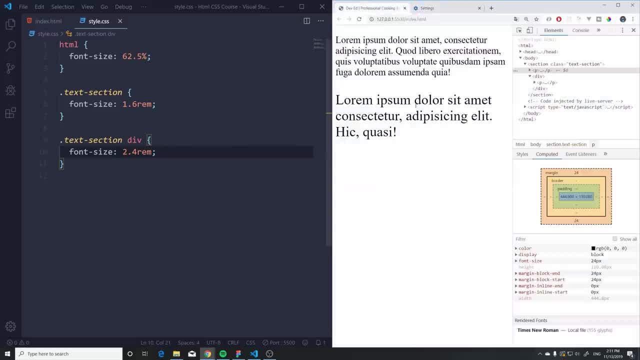 If I want to change the font size of this to something bigger, like large, it's going to affect it. It's going to work perfectly fine. Very small, as you can see, things work perfectly and this is going to be extremely easy to also make the text. 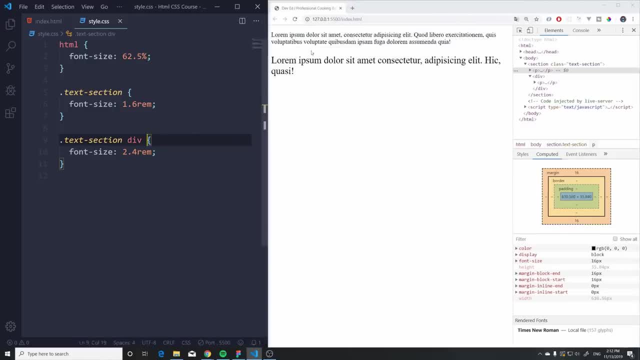 responsive. so when we resize the screen we don't even have to add those media queries that we're going to see later on. we can just mess around with these in a specific way again when we're going to get to the media responsive websites, and we can make this responsive very easily. 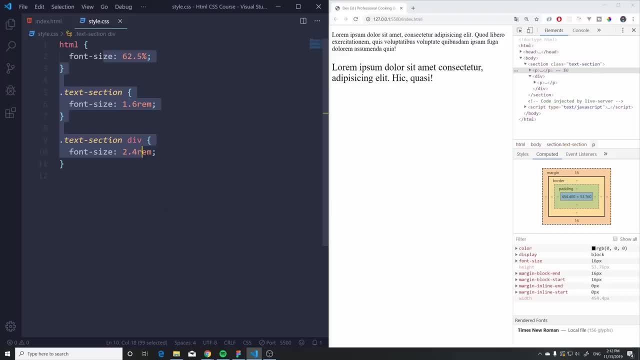 okay. so highly recommend you, highly recommend you to use rem, highly recommend you to avoid pixels and m's. m's might come into play and even pixels, but very rarely. i really want you to put a heavy focus on using rems. so just set your html font size to 16- 62.5 and that way it's very. 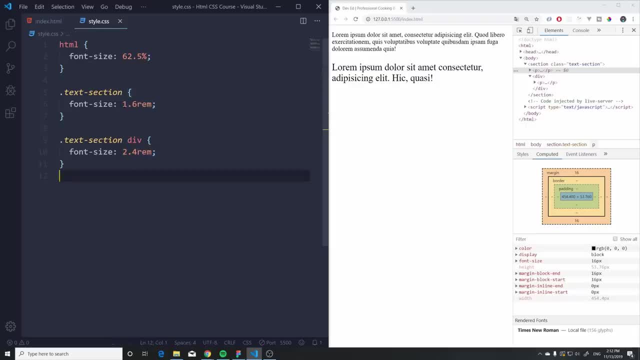 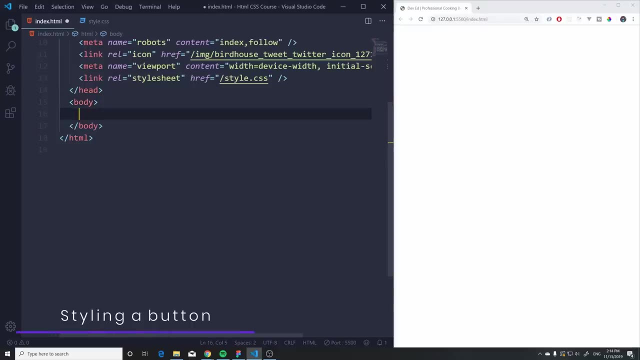 easy to add the numbers here, because one is going to be 10, so 1.5 is going to be 16, 2.4 is going to be 24. okay, so those are rems, m's and pixels. wow, awesome, can we? can we do some fun stuff now? i think the time has finally come for us to actually build out. 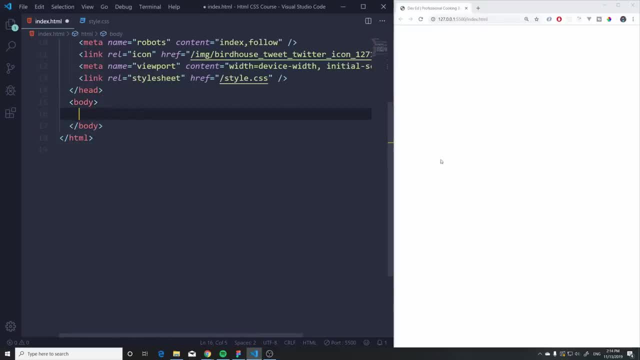 something nice for once. so let's look at borders and we're going to create a nice looking button for once. okay, so by default, if you're going to put a button on the screen, let's say sign up, it's going to look so ugly. take a look at that. what is that? get it off my screen please. that looks. 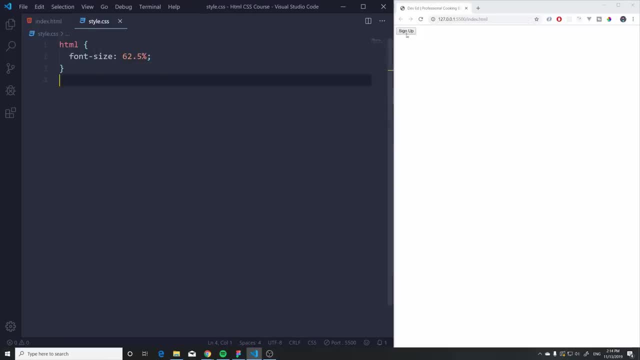 terrible, okay, so we're going to take a look at a few properties that we can add to this to make it look cool. so we can get the button here like this, and, first of all, what i want to do is make this a bit larger. all right, because right now it it doesn't look that good. okay, so what we can do, 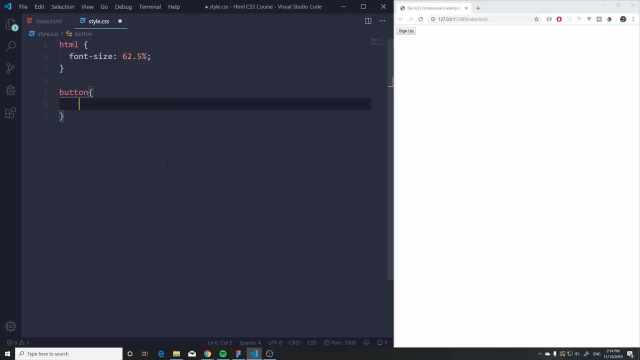 is, we can add maybe some padding and some margin to this. so first of all i want to just add some margin so it's not stuck up there in the corner. so let's do something like let's do 10 rems, okay, and hit save, all right, so it's a bit kind of there 20.. 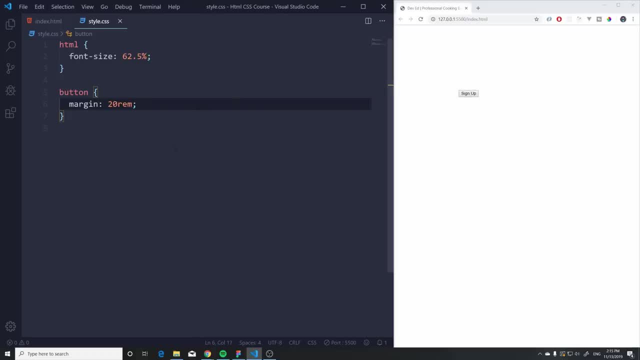 okay, there we go. so we have the button position there, perfect. so next, what i want to do is add some padding to this, because the button right now is kind of small. so the way we can do that is we can say padding and we can add a padding of: let's experiment. 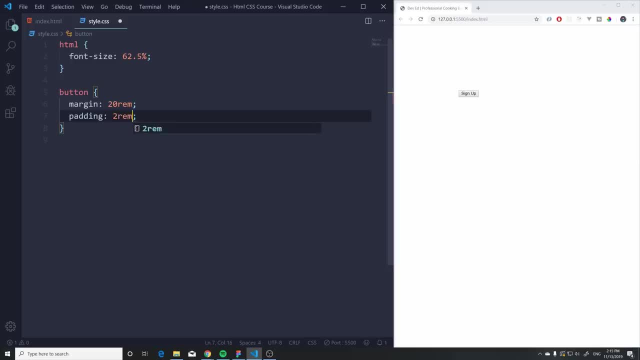 top and bottom. i don't want it to be that high, so i want to say 2 rem, and on the left and right let's try 4 rem. okay, that looks, that looks way better. perfect, let me zoom in actually a bit, okay, actually. no, that's fine, okay, so there we go. we have that now. what i want to do is get rid of. 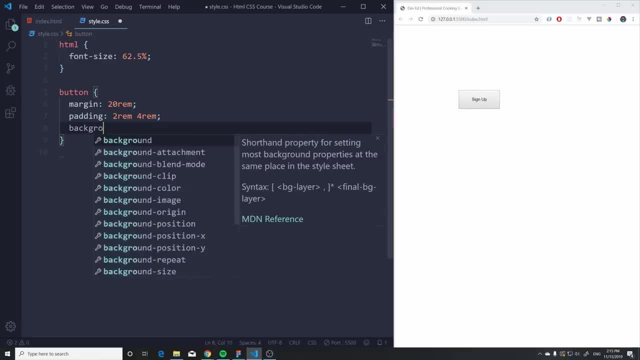 that background color because, oh my goodness, it's ugly. so the way we can get rid of it is: we can see background color and we can see none and, as you can see, that doesn't work. so the one we actually need to use here is background, and when we hit save, it's going to get rid of it. perfect, but we 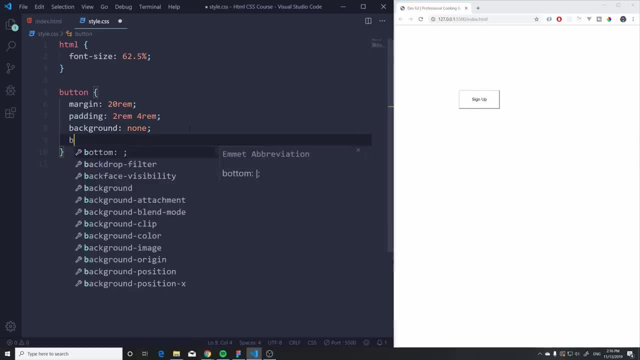 still have this ugly border on top, so to remove that, we can just say a little bit more alleg pics and it's making their way up here. so let's take a moment to bedroom. this time is talking to build. we need to make. our equipment is built different, right, so we need a little bit more wusky and we're. 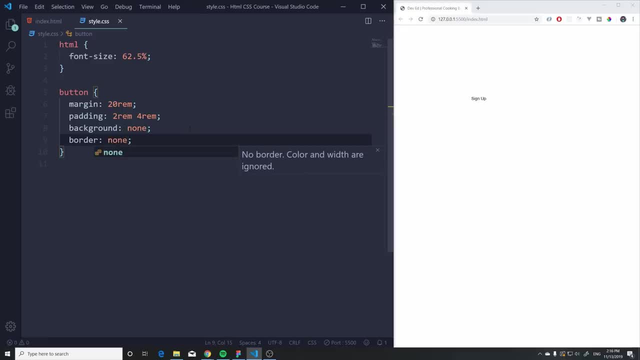 doing all the modern things right now. okay, we're going to add some padding here and add some edges. if we border and we can say none, and that's going to remove the border as well. however, if we want to have the border and we want to change it here, what we 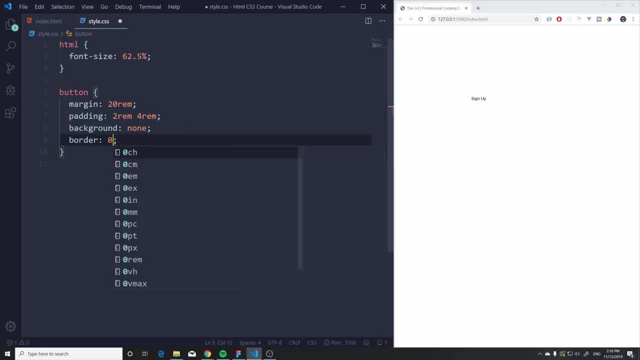 can do is we can add a size to it, so I can say one 0.1 rem, and I can say so. this is the first property, the size. the second is going to be solid, which we're going to take a look at it in a bit, and the third one is going to be the color. 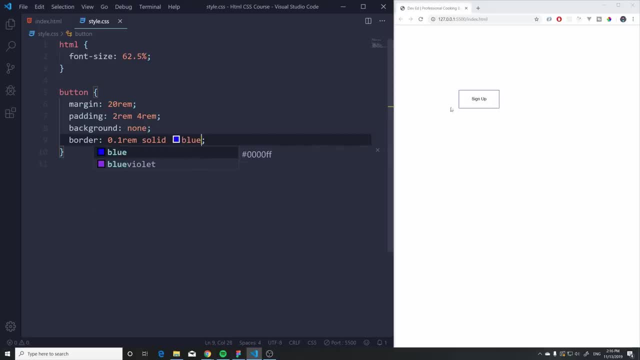 so I can say blue and hit save and, as you can see, we have it right there. now let's change this blue color to something. let's also increase this a bit, like that, and let's change this color. we hover over it sometimes. it doesn't want. 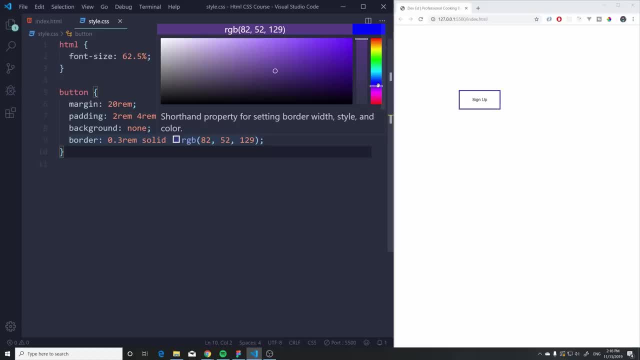 to work. let's get a nicer blue color- I like a purplish, something like that, a bit more vibrant. let's add some color to this. okay, perfect, so there we go. okay, so this is the size. this is the color, but what is this? well, so this is the size. this is the color, but what is this? well, so this is. 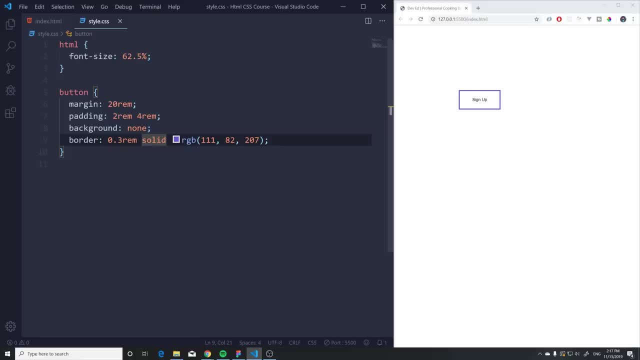 the size. this is the color. but what is this? well, so, this is the color. but what is this? well, so, this is the color. but what is this? well, so, this is the color. but what is this? solid makes the whole border full. solid makes the whole border full. 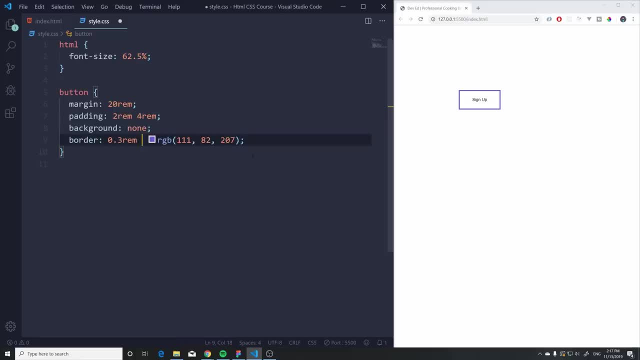 solid makes the whole border full. there are a few other ones here that we. there are a few other ones here that we. there are a few other ones here that we can experiment, can experiment, can experiment which is going to be, and the cool thing which is going to be, and the cool thing. 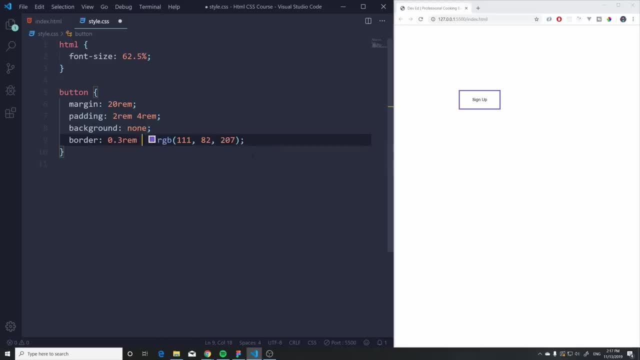 which is going to be, and the cool thing that you can do is sometimes just type that you can do, is sometimes just type that you can do is sometimes just type like this, and sometimes it can give you like this, and sometimes it can give you like this and sometimes it can give you, sometimes it cannot. I believe, when you 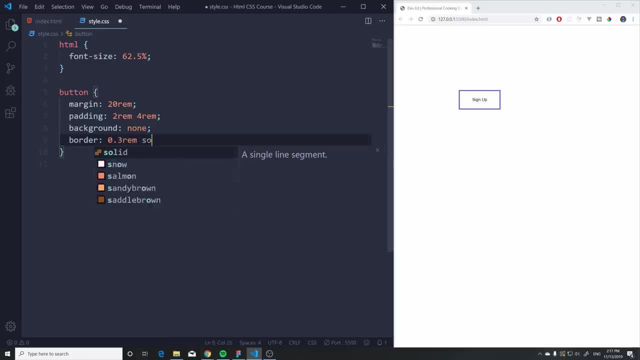 sometimes it cannot. I believe, when you sometimes it cannot, I believe when you first start typing like this solid, let's first start typing like this solid. let's first start typing like this solid, let's see all right, and then we have, I believe. see all right, and then we have, I believe. 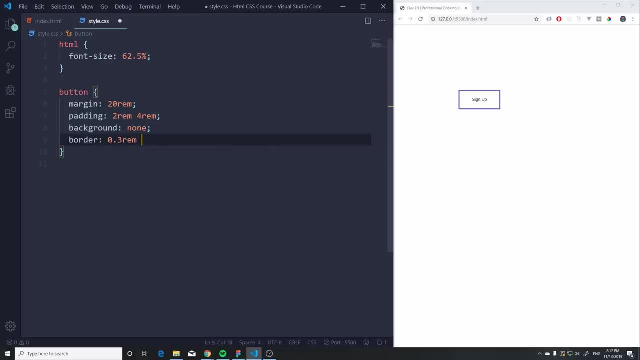 see. all right, and then we have, I believe, it only gives you the colors. it only gives you the colors. it only gives you the colors, unfortunately, but there's one called unfortunately, but there's one called unfortunately, but there's one called dotted like this and as you can see, 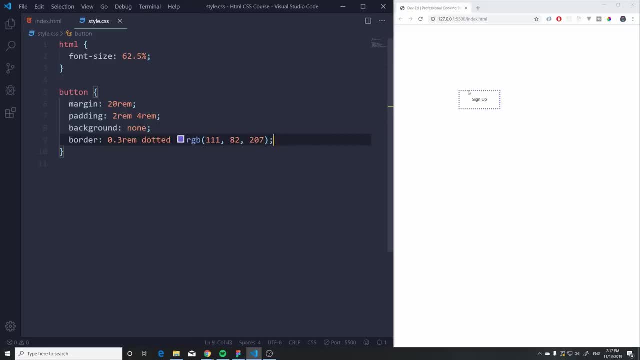 dotted like this and, as you can see, dotted like this and, as you can see, that just adds thoughts to it. there's that just adds thoughts to it. there's that just adds thoughts to it. there's also ones that add lines to it, but also ones that add lines to it, but 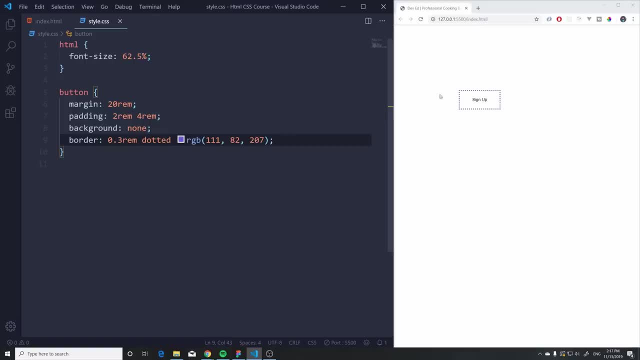 also ones that add lines to it. but generally to be honest, you're rarely generally to be honest. you're rarely generally to be honest, you're rarely gonna use these. I mean if you find some gonna use these. I mean if you find some gonna use these. I mean if you find some edge cases where you are you want to add. 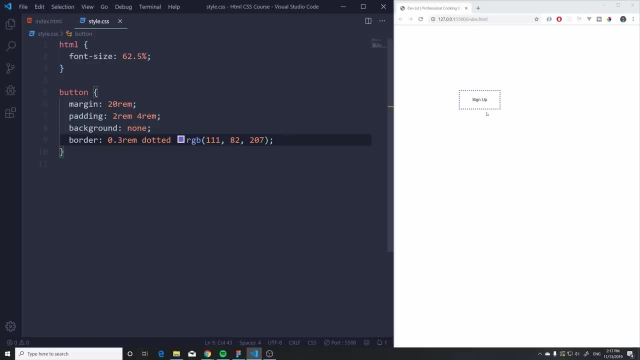 edge cases where you are. you want to add edge cases where you are. you want to add dots to your buttons, or just border dots to your buttons, or just border dots to your buttons, or just border dots, for some reason. but it looks like dots for some reason. but it looks like. 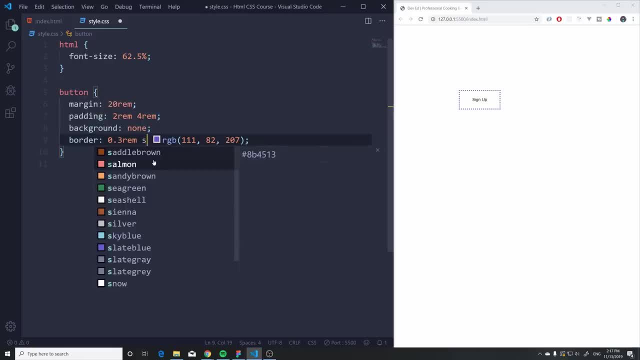 dots for some reason, but it looks like something from the 90s, so I'm just gonna something from the 90s. so I'm just gonna something from the 90s. so I'm just gonna keep it solid here and mostly you're. keep it solid here and mostly you're. 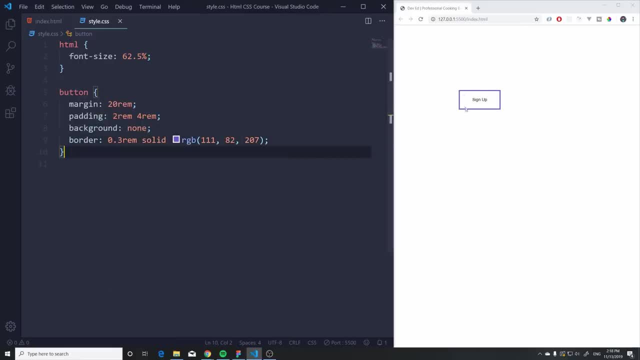 keep it solid here and mostly you're probably gonna have solid borders, probably gonna have solid borders, probably gonna have solid borders anyways. okay, so we added a border of anyways. okay, so we added a border of anyways. okay, so we added a border of solid here. okay. next up, what I want to do: 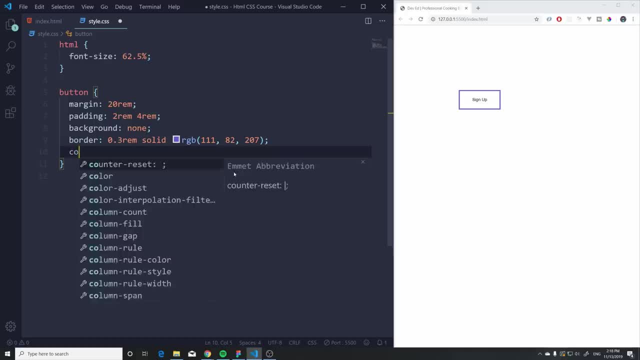 solid here: okay, next up. what I want to do: solid here, okay, next up. what I want to do is: I want to change the color of this is. I want to change the color of this is. I want to change the color of this text as well, so we can see color and we. 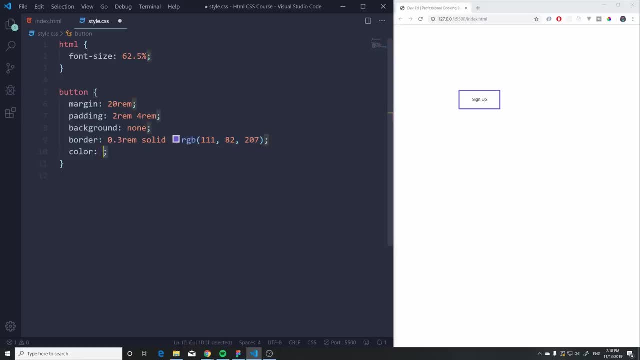 text as well, so we can see color and we text as well, so we can see color and we can say we can actually just copy paste, can say we can actually just copy paste, can say we can actually just copy paste this color from up here, save and there. 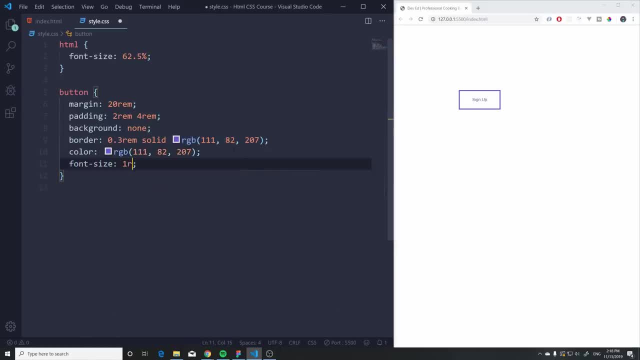 this color from up here, save. and there. this color from up here, save. and there we go. we can also adjust the font size, we go. we can also adjust the font size, we go. we can also adjust the font size of it. font size: one rim, there we go. oh. 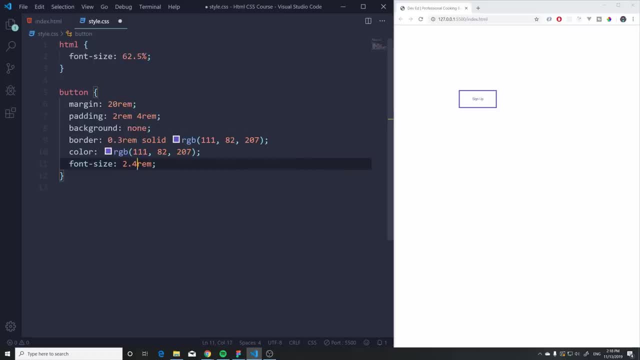 of it- font size, one rim, there we go. oh of it- font size, one rim, there we go. oh, that's gonna be 10. so let's do maybe 2.4. that's gonna be 10. so let's do maybe 2.4. that's gonna be 10. so let's do maybe 2.4. is that gonna be too learned, that's? 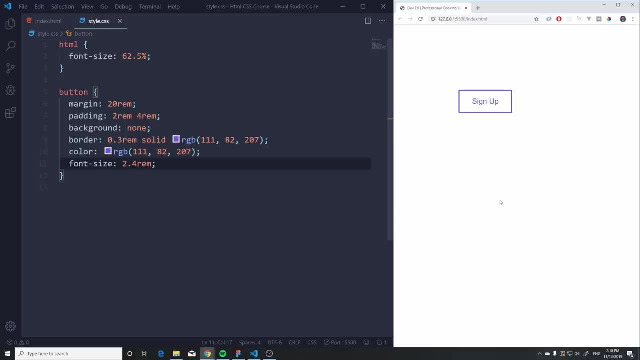 is that gonna be too learned? that's. is that gonna be too learned? that's gonna be fine. so there we go. we have a gonna be fine. so there we go. we have a gonna be fine. so there we go. we have a nice-looking button going on here. 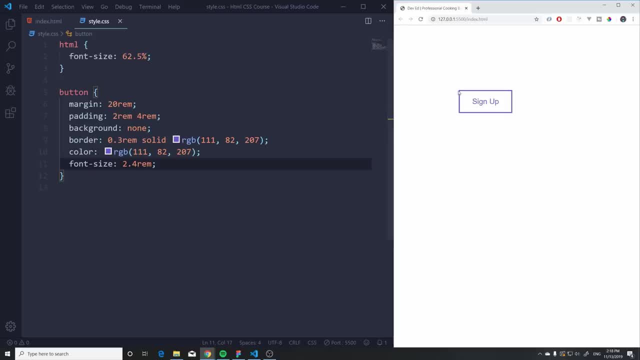 nice-looking button going on here. nice-looking button going on here. there's another property that I want to. there's another property that I want to. there's another property that I want to cover. maybe you want to make these edges cover. maybe you want to make these edges. 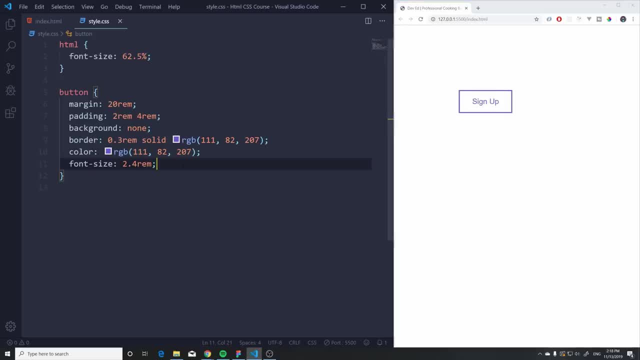 cover. maybe you want to make these edges round a bit. you don't want this to be so round a bit. you don't want this to be so round a bit. you don't want this to be so boxy. so what we can do is add a border. 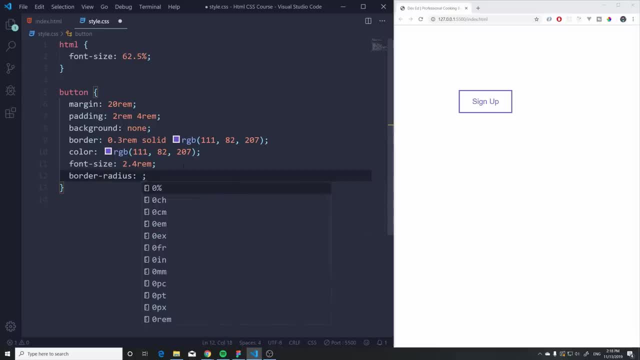 boxy, so what we can do is add a border boxy. so what we can do is add a border radius to this, and by adding a border radius to this, and by adding a border radius to this and by adding a border radius, we can smooth this out and we can. 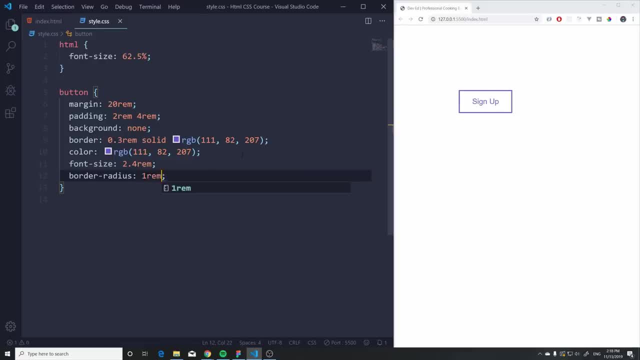 radius. we can smooth this out and we can radius. we can smooth this out and we can make it rounder. so if I add something, make it rounder. so if I add something, make it rounder. so if I add something like one rem, that's gonna add 16 pixels. 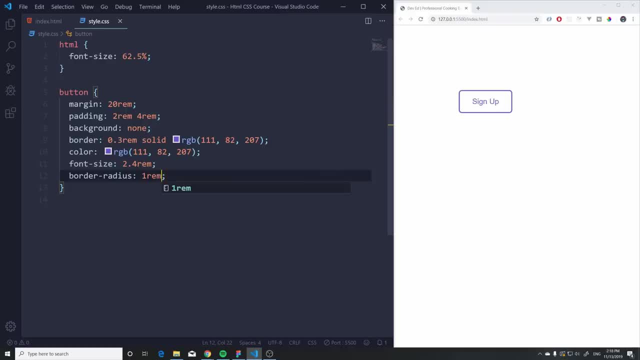 like one rem that's gonna add 16 pixels. like one rem that's gonna add 16 pixels of border radius to this 10 pixels. I of border radius to this 10 pixels. I of border radius to this 10 pixels. I apologize, we have this HTML thing here. 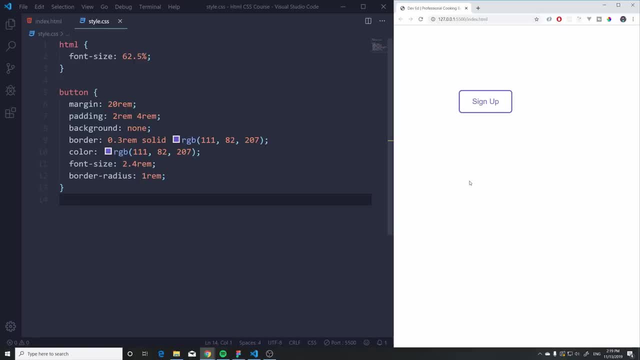 apologize, we have this HTML thing here, apologize. we have this HTML thing here and that makes one rem 10 pixels. okay, so, and that makes one rem 10 pixels, okay, so, and that makes one rem 10 pixels, okay. so, there we go. that makes it look way way. 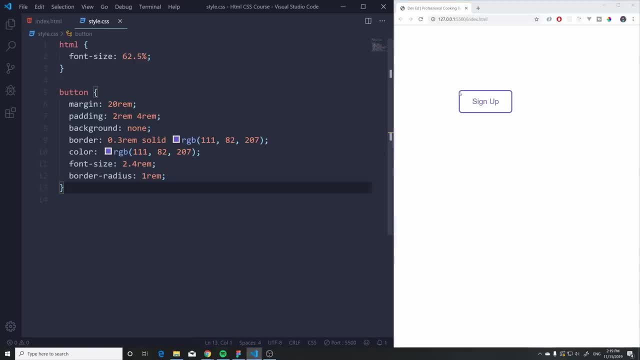 there we go. that makes it look way, way. there we go. that makes it look way, way nicer. if you want to add specifically nicer, if you want to add specifically nicer. if you want to add specifically, maybe to the top left or bottom left a, maybe to the top left or bottom left a. 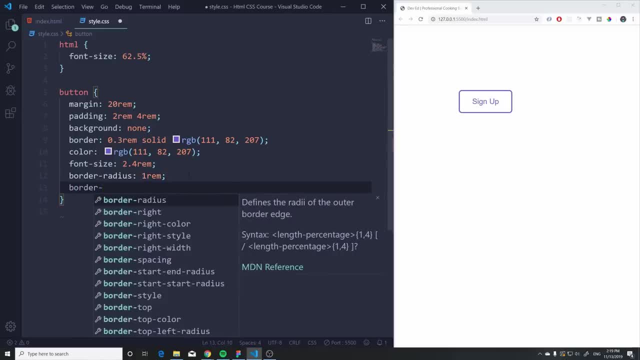 maybe to the top left or bottom left, a border radius, you can also do border border radius, you can also do border border radius, you can also do border. let's do you left top left radius, all. let's do you left top left radius. all. let's do you left top left radius, all right, so this is gonna be this one top. 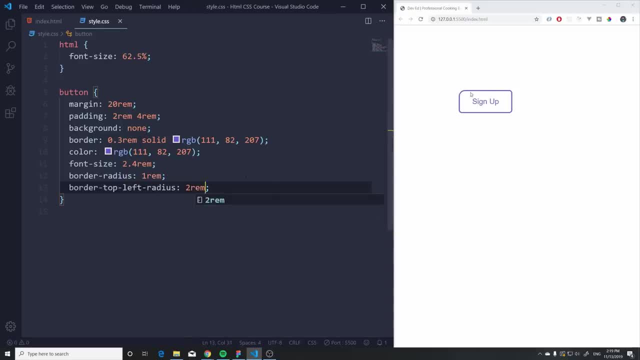 right. so this is gonna be this one top right. so this is gonna be this one top left, and you can add to Ram here, so as left, and you can add to Ram here, so as left, and you can add to Ram here, so, as you can see, that's gonna make it even. 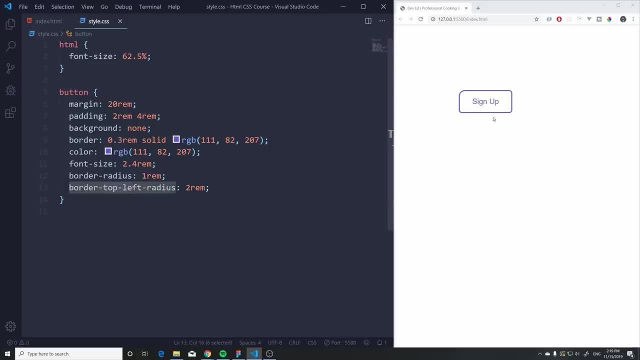 you can see that's gonna make it even. you can see that's gonna make it even rounder for you. there we go, so you can rounder for you. there we go, so you can rounder for you. there we go. so you can do top left, you can do top right, bottom. 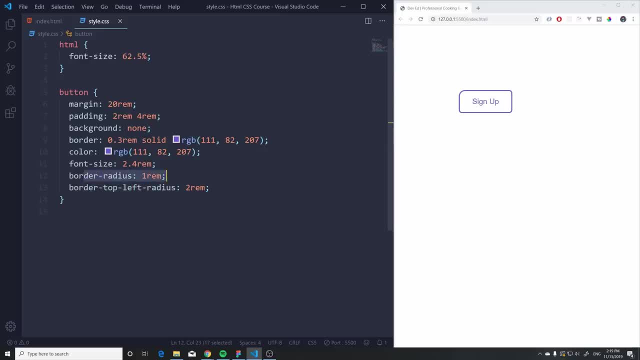 do top left, you can do top right, bottom do top left, you can do top right, bottom left, bottom right. but this kind of adds left, bottom right, but this kind of adds left, bottom right, but this kind of adds it to all of it, which mostly this is: 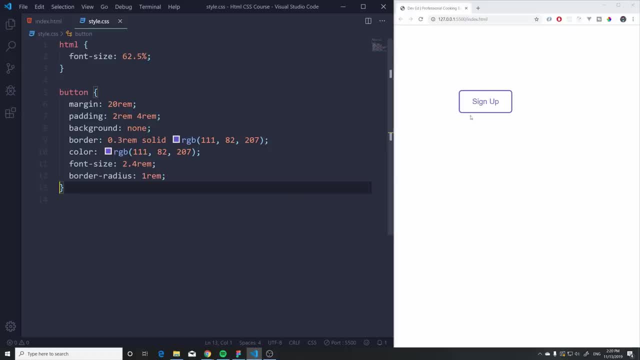 it to all of it, which mostly this is it to all of it, which mostly this is what you're gonna use anyway. if you want what you're gonna use anyway, if you want what you're gonna use anyway, if you want to make this perfectly round what you. 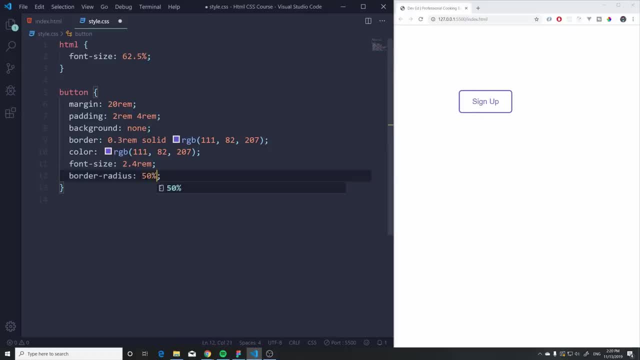 to make this perfectly round. what you to make this perfectly round, what you can do is add 50%, so 50% is gonna make. can do is add 50%, so 50% is gonna make. can do is add 50%, so 50% is gonna make it round. now it's not round here because 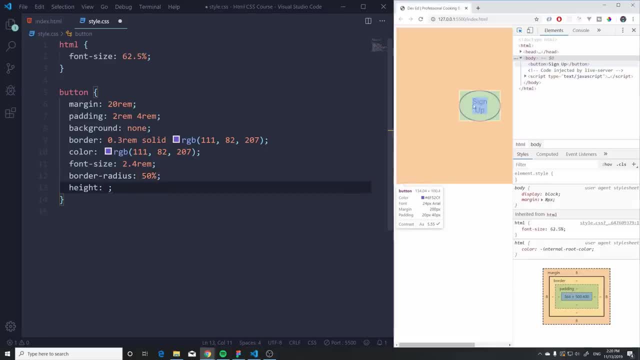 it round now, it's not round here. because it round now it's not round here, because the element size also needs to be round. the element size also needs to be round. the element size also needs to be round. so this kind of looks rectangular, right. so this kind of looks rectangular right. 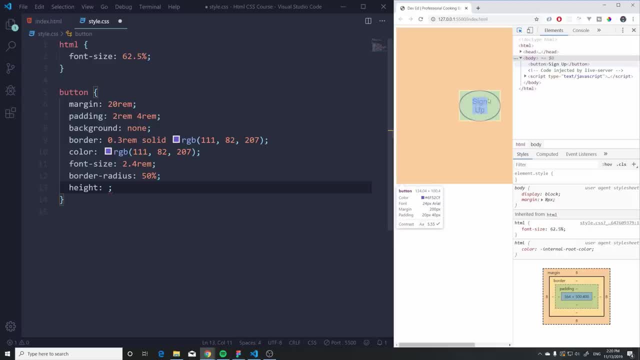 so this kind of looks rectangular right now, but what we need here is to have a now. but what we need here is to have a now, but what we need here is to have a perfect square for this to be round, so perfect square for this to be round, so 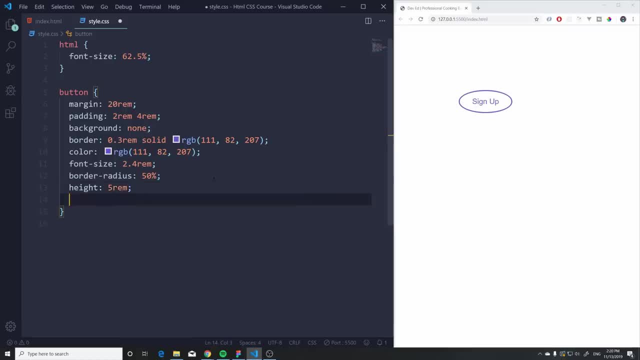 perfect square for this to be round. so if I just set a height of 5 rem here, and if I just set a height of 5 rem here, and if I just set a height of 5 rem here and a width of 5 rem, I think we need a bit. 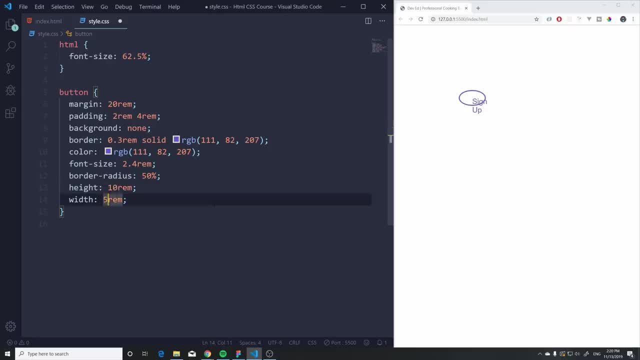 a width of 5 rem. I think we need a bit a width of 5 rem. I think we need a bit more. that's too small, so let's do 10 and more. that's too small, so let's do 10 and more. that's too small, so let's do 10 and 10. is that too small? 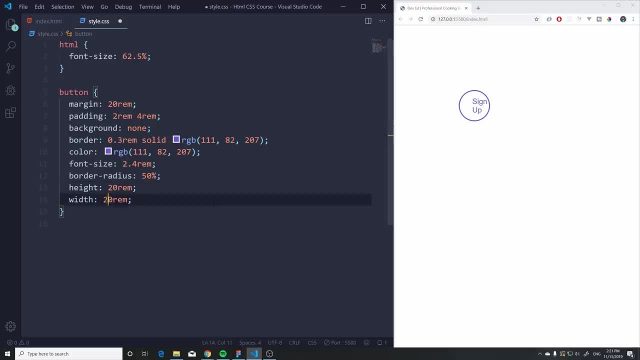 10 is that too small? 10 is that too small? 20 and 20 all right, so there we go. so if 20 and 20, all right, so there we go. so if 20 and 20 all right, so there we go. so if the element is way larger here and if we 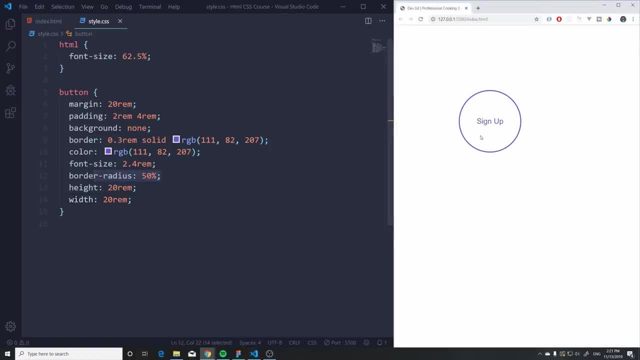 the element is way larger here. and if we- the element is way larger here- and if we set the border radius to 50, then we are set the border radius to 50, then we are set the border radius to 50, then we are gonna get a perfect circle, awesome. so 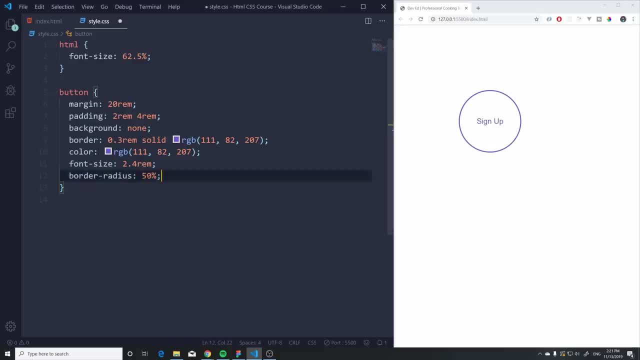 gonna get a perfect circle- awesome. so gonna get a perfect circle- awesome. so let's remove these for now, and what I let's remove these for now and what I let's remove these for now, and what I want to do is also show you something. want to do is also show you something. 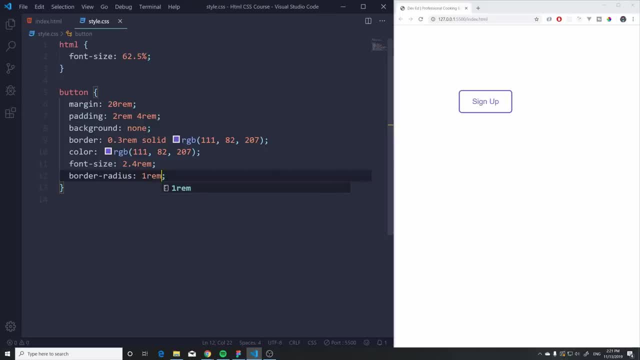 want to do is also show you something else. so let's change this back. I believe else, so let's change this back. I believe else, so let's change this back. I believe we had one rem. we can also change this. we had one rem, we can also change this. 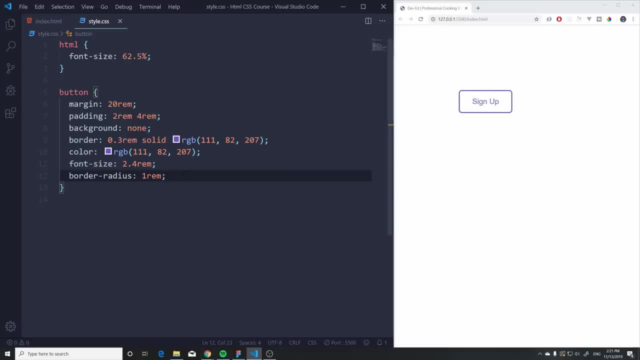 we had one rem. we can also change this button. if we want to make it full, we button. if we want to make it full, we button. if we want to make it full, we can add a background of the this color can add a background of the this color. 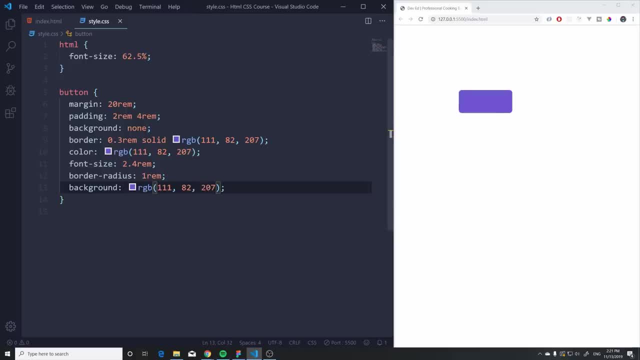 can add a background of the this color that we had up here. so let's add this that we had up here. so let's add this that we had up here. so let's add this color up here. but now the problem is: color up here, but now the problem is. 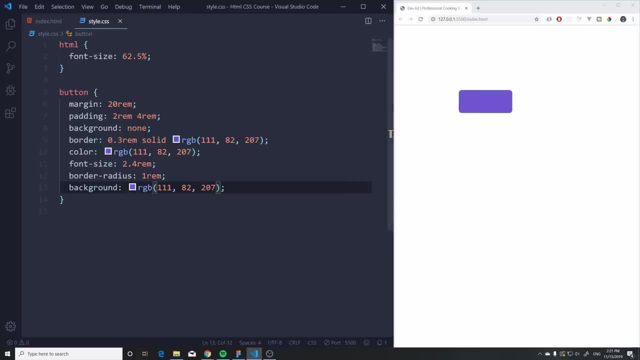 color up here. but now the problem is that the text is okay. we cannot see the. that the text is okay. we cannot see the. that the text is okay. we cannot see the text. so we need to change this to white text. so we need to change this to white. 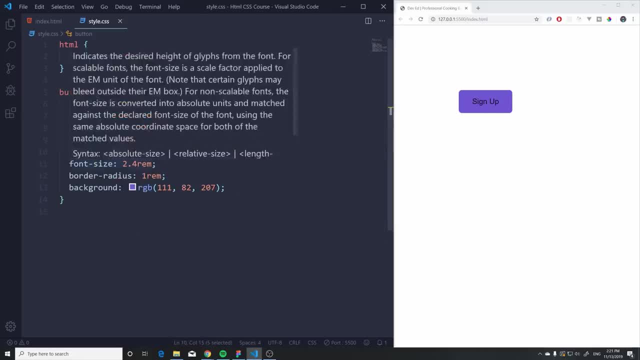 text. so we need to change this. to white. so there are two. all right not to color. so there are two. all right not to color. so there are two. all right not to color. to white: all right, so there's two. to white. all right, so there's two. 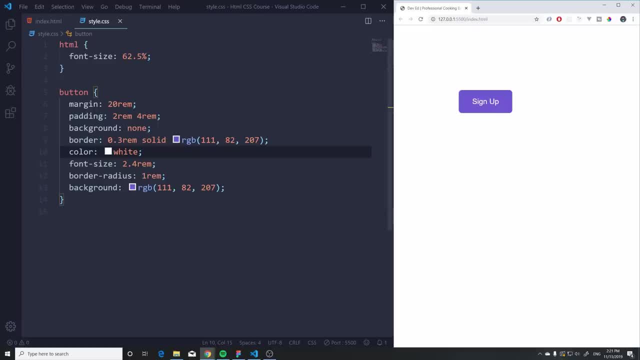 to white. all right, so there's two different styles of buttons there for you, different styles of buttons there for you, different styles of buttons there for you. if you want to experiment, but yeah. if you want to experiment, but yeah, if you want to experiment, but yeah, that's how you can create a simple nice. 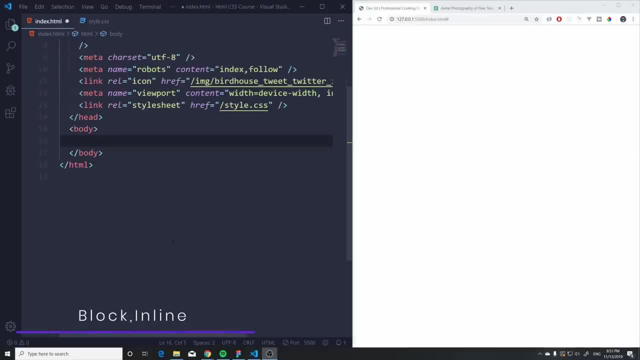 that's how you can create a simple nice. that's how you can create a simple nice looking button. let's take a look at looking button. let's take a look at looking button. let's take a look at display block, inline and inline block. so display block, inline and inline block. so 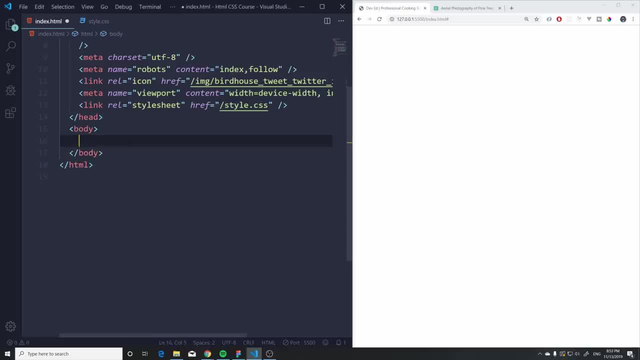 display block, inline and inline block. so many of them, all right. what are these? many of them, all right. what are these? many of them all right. what are these things? so we have noticed that whenever things. so we have noticed that whenever things. so we have noticed that whenever we start adding like a header for: 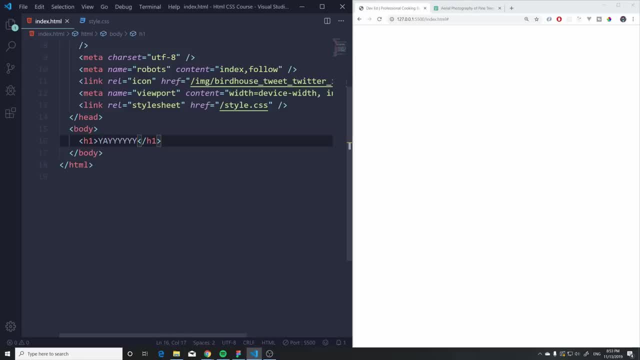 we start adding like a header, for we start adding like a header, for example, so we can say that yeah and hit example. so we can say that yeah and hit example. so we can say that yeah and hit. of our page here interesting and the. of our page here interesting and the. 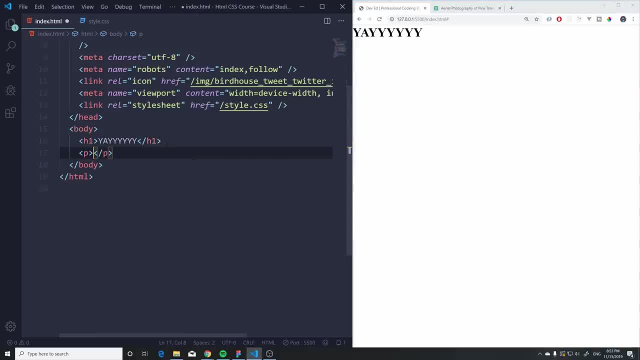 of our page here interesting, and the more interesting part is if we add. more interesting part is if we add. more interesting part is if we add another one and we're gonna say no, then another one and we're gonna say no, then another one and we're gonna say no, then this is gonna be dropped underneath. so 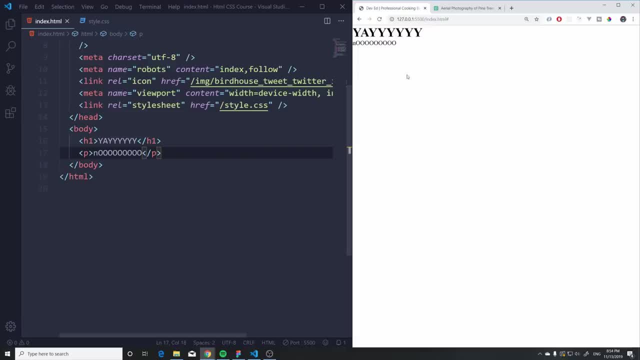 this is gonna be dropped underneath. so this is gonna be dropped underneath. so some elements have a display type of. some elements have a display type of. some elements have a display type of block, which basically means that they're block, which basically means that they're block, which basically means that they're gonna take up the whole space here. the 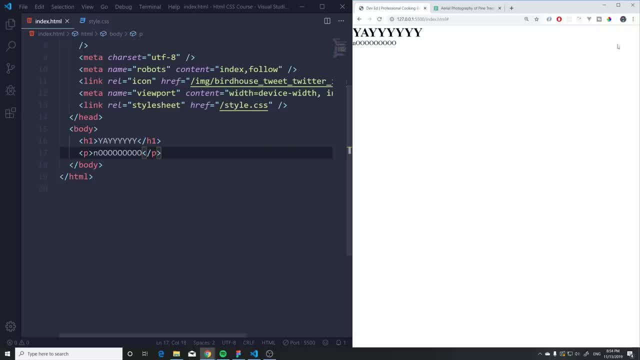 gonna take up the whole space here. the gonna take up the whole space here, the full width here, and they're gonna have a full width here and they're gonna have a full width here and they're gonna have a line break, so they're gonna drop the. 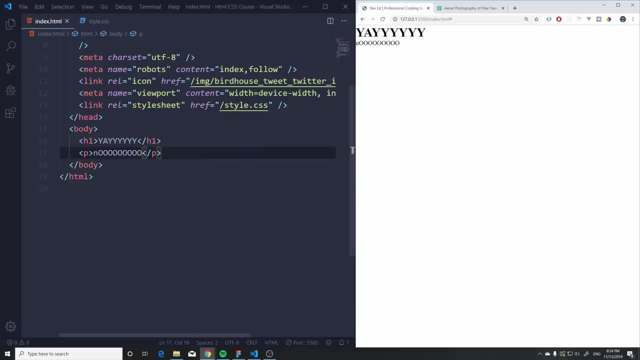 line break. so they're gonna drop the line break. so they're gonna drop the next element down below. okay now if we next element down below. okay now if we next element down below. okay now, if we get this h1 that we did, we can still get this h1 that we did, we can still. 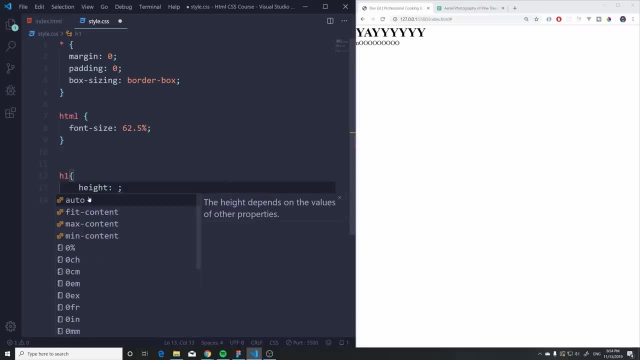 get this h1. that we did. we can still add a height to it. if we want, we can do add a height to it. if we want, we can do add a height to it if we want, we can do, for example, like two rems to it and 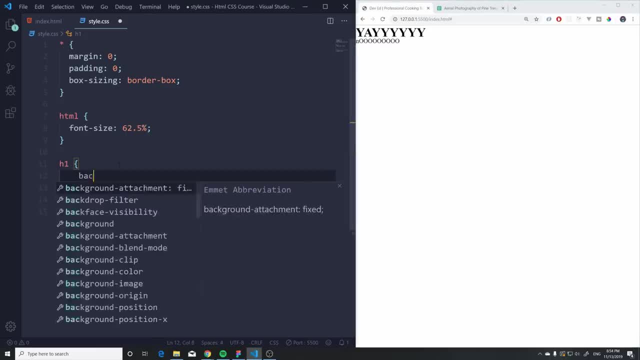 for example, like two rems to it and, for example, like two rems to it. and let's take a look really quickly. let's, let's take a look really quickly. let's, let's take a look really quickly. let's also add the background color to this. 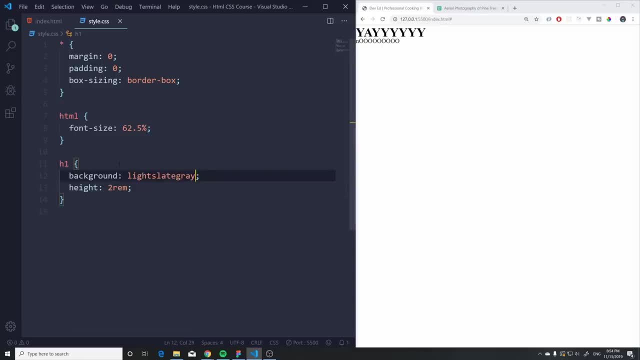 also add the background color to this, also add the background color to this. background light- light- gray, there we go. background light- light, gray, there we go. background light- light gray, there we go. perfect. so let's increase the size of perfect. so let's increase the size of. 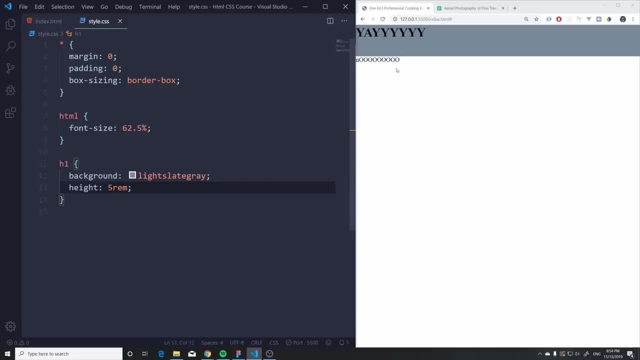 perfect, so let's increase the size of this, because it was too small: 50. all this because it was too small: 50. all this because it was too small: 50, all right, so we can add some height to it. right, so we can add some height to it. 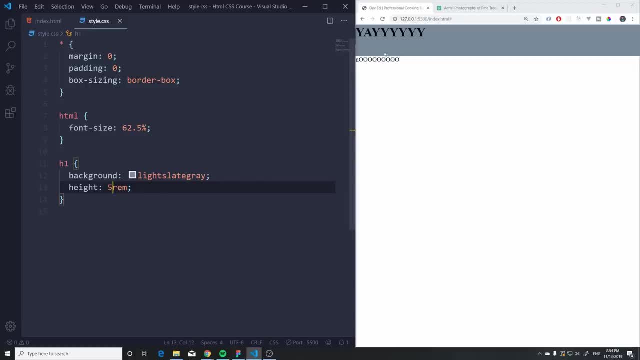 right, so we can add some height to it. if we want, that's perfectly fine. but if we want, that's perfectly fine. but if we want, that's perfectly fine. but there are a few elements that act a bit. there are a few elements that act a bit. 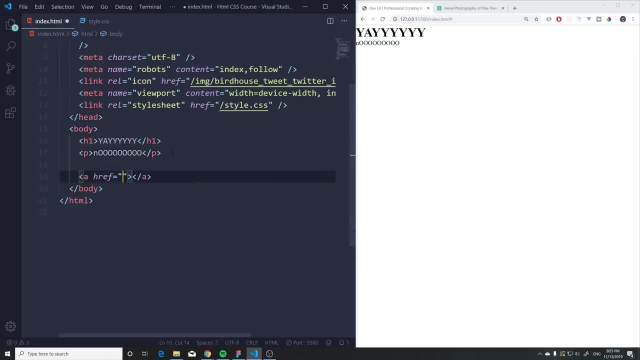 there are a few elements that act a bit differently, so let me show you one. if I differently, so let me show you one. if I differently, so let me show you one. if I add an anchor tag down here below, and add an anchor tag down here below, and 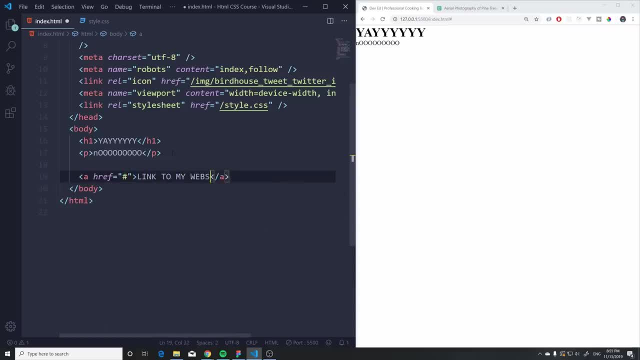 add an anchor tag down here below, and, and I'm gonna say link to my website and I'm gonna say link to my website and I'm gonna say link to my website. alright, it's safe. so there we have let's. alright, it's safe. so there we have let's. 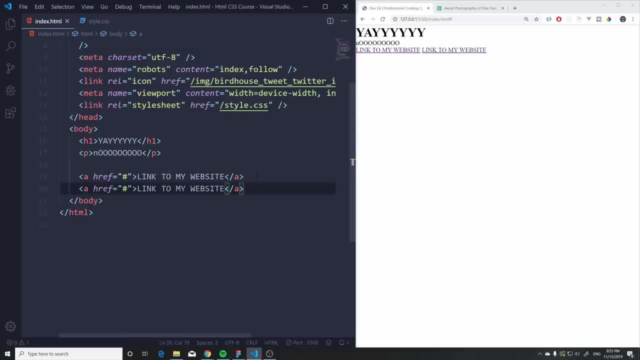 alright, it's safe. so there we have. let's copy this and add it again. let's see, copy this and add it again. let's see, copy this and add it again. let's see what happens then. hmm, that's strange the. what happens then. hmm, that's strange the. 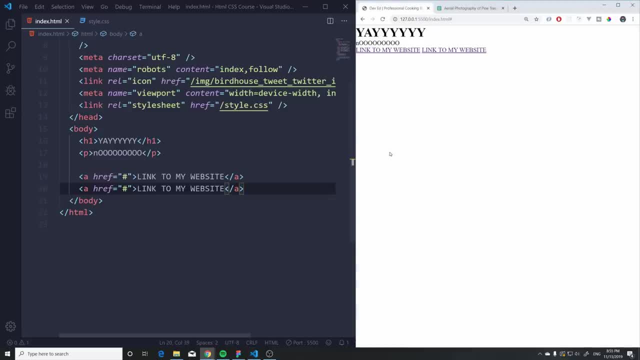 what happens then? hmm, that's strange. the link is on the right. why is this not on? link is on the right. why is this not on? link is on the right. why is this not on the bottom? so there are a few elements. the bottom, so there are a few elements. 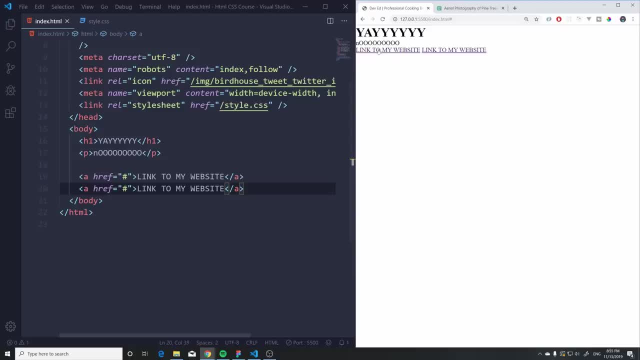 the bottom. so there are a few elements that are displayed differently. this is that are displayed differently. this is that are displayed differently. this is called displayed in line and what it called displayed in line and what it called displayed in line, and what it means is that it doesn't do a line break. 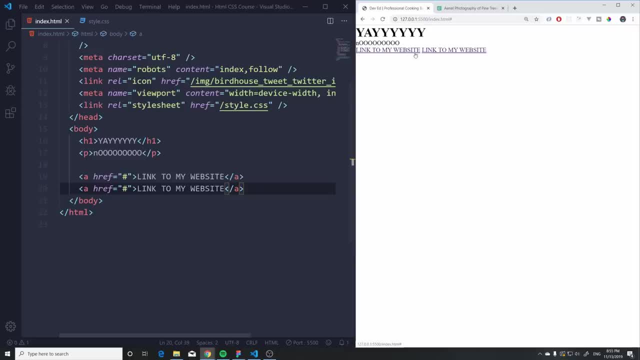 means is that it doesn't do a line break. means is that it doesn't do a line break and it doesn't take up more space than and it doesn't take up more space than and it doesn't take up more space than the element itself. so, if we add 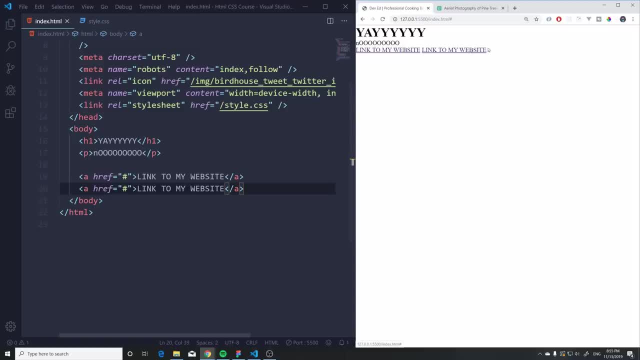 the element itself. so if we add the element itself, so if we add something else- another inline element, something else, another inline element, something else, another inline element- it's gonna be here right next to it and it's gonna be here right next to it and it's gonna be here right next to it. and I can show you another one. we can do it. 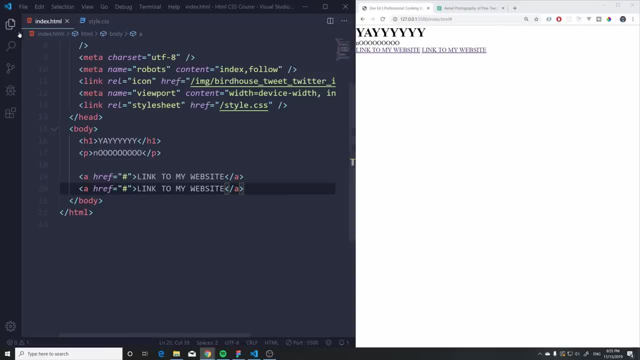 I can show you another one. we can do it. I can show you another one. we can do it with an image as well. that is an inline with an image as well. that is an inline with an image as well. that is an inline. so if we go back here, I'll just drop in. 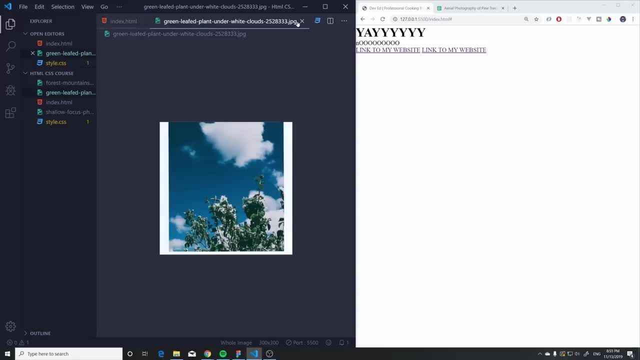 so if we go back here, I'll just drop in. so if we go back here, I'll just drop in an image of this green leaf, I'm not sure. an image of this green leaf, I'm not sure. an image of this green leaf, I'm not sure. if we go down here and I'm gonna add an. 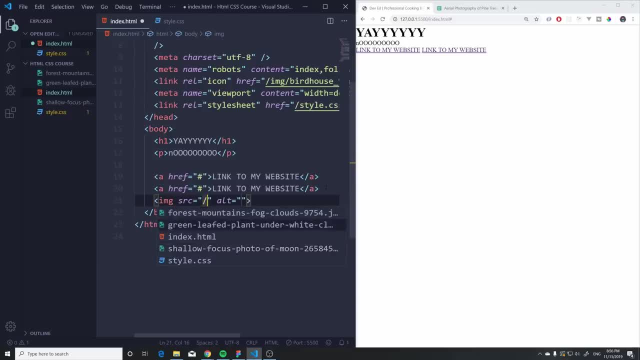 if we go down here and I'm gonna add an, if we go down here and I'm gonna add an image, let's add the source of green image, let's add the source of green image, let's add the source of green leaf. so, okay, this is here and you know what? 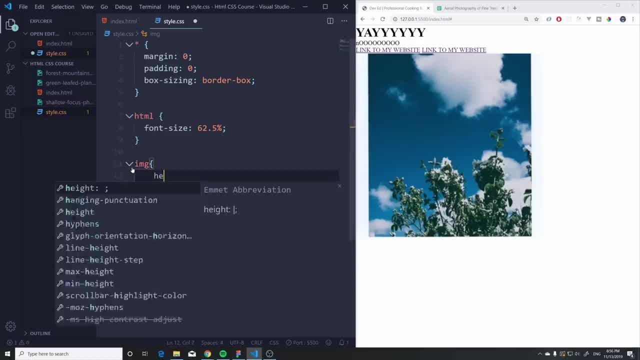 leaf. so okay, this is here, and you know what leaf. so okay, this is here. and you know what? this is a bit still too large, so I'm this is a bit still too large. so I'm, this is a bit still too large, so I'm gonna change the size of it to height. 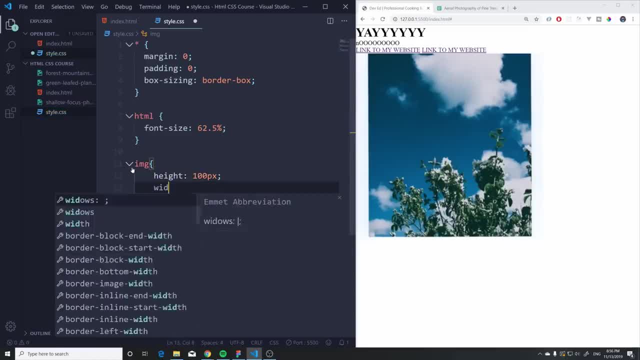 gonna change the size of it to height. gonna change the size of it to height. 100 pixels and width. why am i doing 100 pixels and width? why am i doing 100 pixels and width? why am i doing pixels? let's do rems. let's do 10 rems. 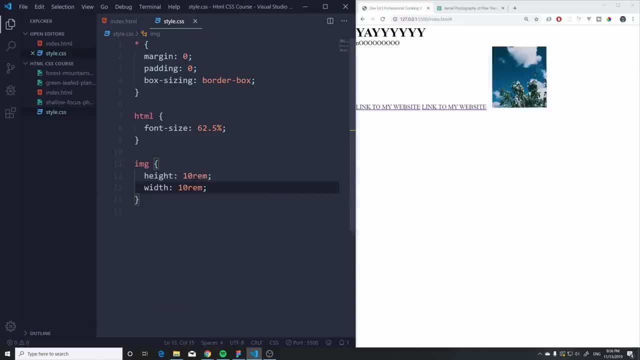 pixels- let's do rems, let's do 10 rems. pixels- let's do rems, let's do 10 rems. and width of 10 rems- it's safe, all. and width of 10 rems- it's safe, all. and width of 10 rems- it's safe, all right, so it's way smaller now. okay, take. 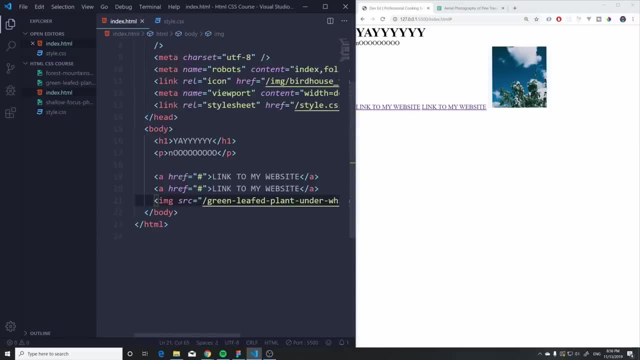 right, so it's way smaller now. okay, take right, so it's way smaller now. okay, take a look, this one is here as well. and if I a look, this one is here as well. and if I a look, this one is here as well. and if I duplicate this again, as you can see this, 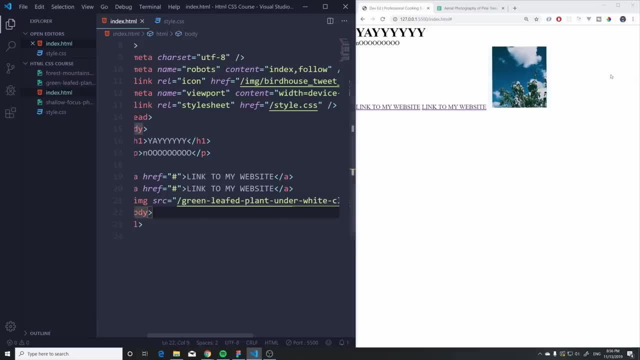 duplicate this again, as you can see this. duplicate this again, as you can see. this is still coming next to it now. if it is still coming next to it now, if it is still coming next to it now, if it doesn't have any space anymore, here it's. 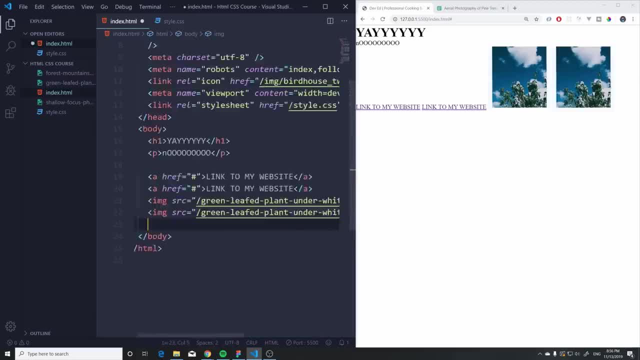 doesn't have any space anymore here. it's doesn't have any space anymore here. it's probably gonna jump down. so let's do it. probably gonna jump down. so let's do it. probably gonna jump down. so let's do it. and let's add another one. as you can see, 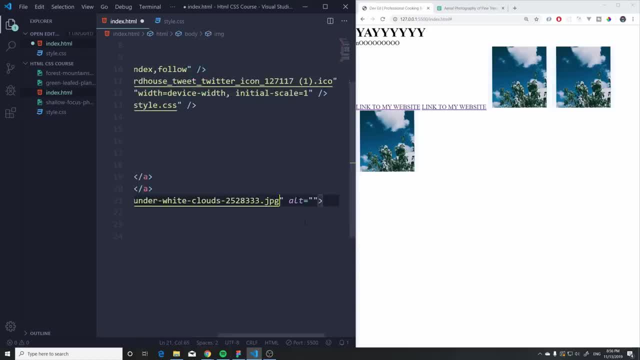 and let's add another one. as you can see, and let's add another one. as you can see, it jumps down because it just doesn't, it jumps down because it just doesn't, it jumps down because it just doesn't have any space. okay, let's remove it. 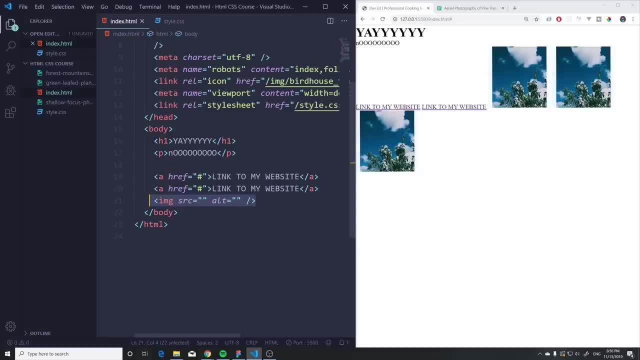 have any space? okay, let's remove it. have any space? okay, let's remove it, because I want to show you something else, because I want to show you something else, because I want to show you something else. so that's the first thing, the other. so that's the first thing, the other. 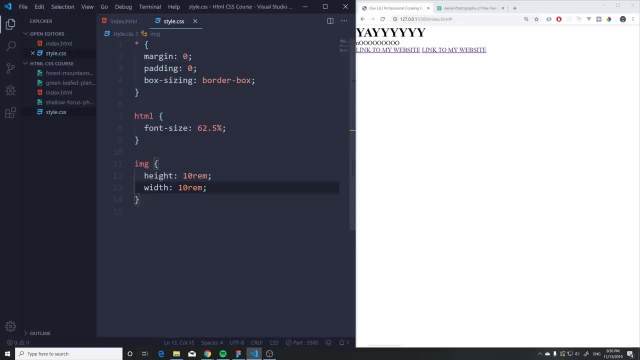 so that's the first thing. the other interesting thing about these in lines, interesting thing about these in lines, interesting thing about these in lines is: let's take a look, let's remove the is. let's take a look, let's remove the is. let's take a look, let's remove the image and add the anchor tag. so I want. 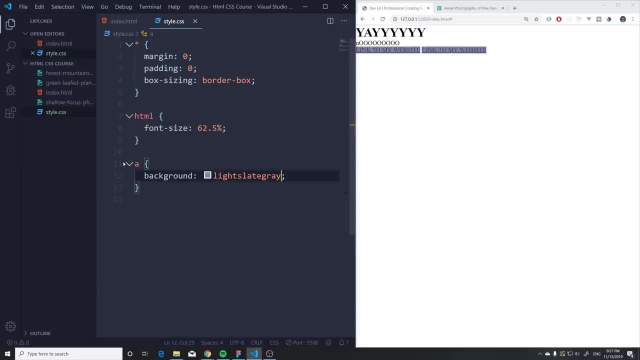 image and add the anchor tag. so I want image and add the anchor tag. so I want to add a background to this of light. to add a background to this of light, to add a background to this of light gray. okay, what if I want to add some? 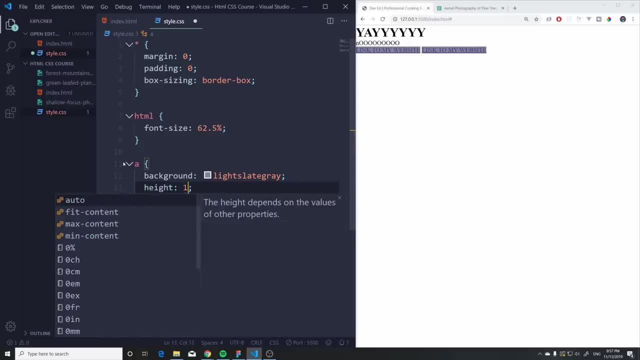 gray. okay, what if I want to add some gray? okay, what if I want to add some height to this? let's add a height of 10 height to this. let's add a height of 10 height to this. let's add a height of 10. rem, hit, save and oh, nothing happens. 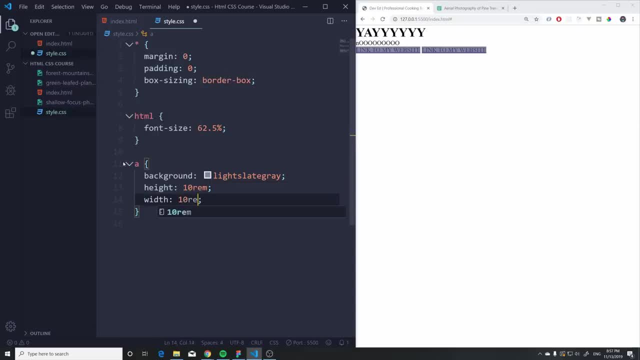 rem hit save and oh, nothing happens. rem hit save and oh, nothing happens. all right, let me try to add a width to. all right, let me try to add a width to. all right, let me try to add a width to. this pen around- still nothing happens. this pen around- still nothing happens. 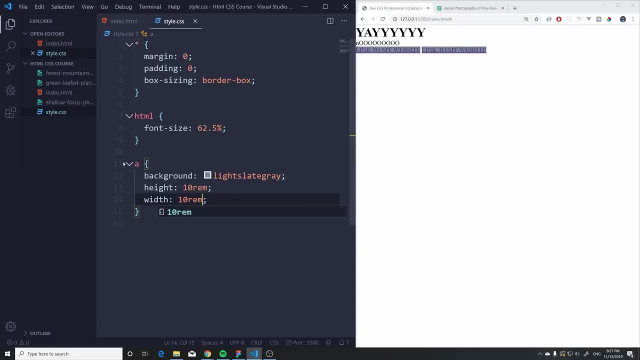 this pen around, still nothing happens. turn to turn. what is this sorcery? oh, my turn to turn. what is this sorcery? oh, my turn to turn. what is this sorcery? oh my goodness well, basically in line elements. goodness well, basically in line elements. goodness well, basically in line elements. you, you cannot add the height or width. 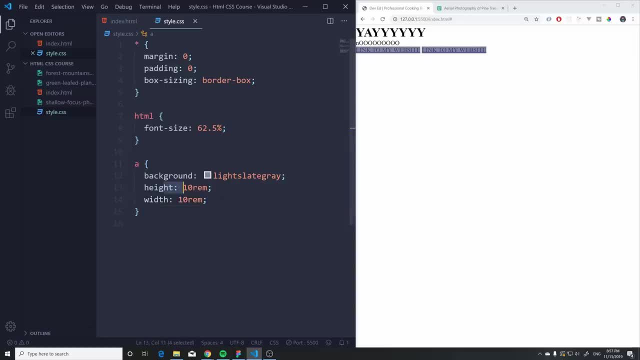 you, you cannot add the height or width. you, you cannot add the height or width to them. it just doesn't work. it doesn't to them. it just doesn't work. it doesn't to them. it just doesn't work. it doesn't like it. it doesn't like it. okay. what if? 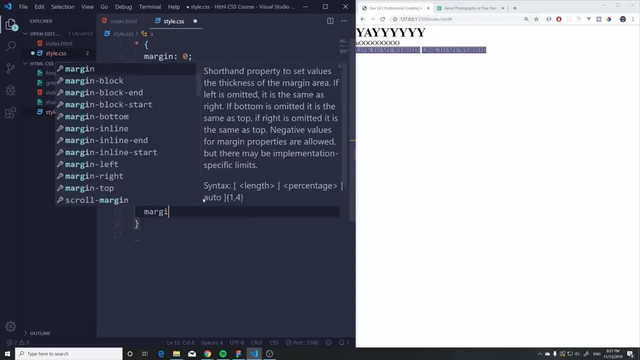 like it, it it doesn't like it, okay. what if like it, it it doesn't like it? okay. what if we try to add some padding to them? or we try to add some padding to them? or we try to add some padding to them, or some margin. let's try margin 3, rem. okay. 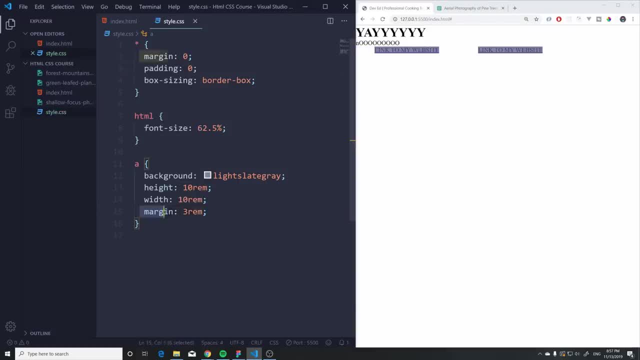 some margin. let's try margin 3 rem. okay, some margin. let's try margin 3 rem. okay, margin works kind of in a weary way. so margin works kind of in a weary way. so margin works kind of in a weary way. so when you add margins to inline elements, 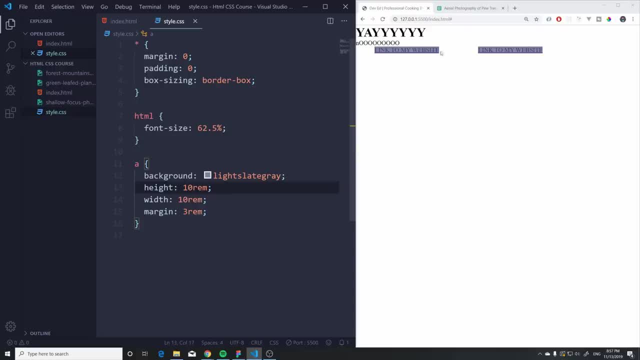 when you add margins to inline elements. when you add margins to inline elements, only the left and the right property is only the left and the right property is only the left and the right property is gonna work. it's not gonna add on top or gonna work. it's not gonna add on top, or 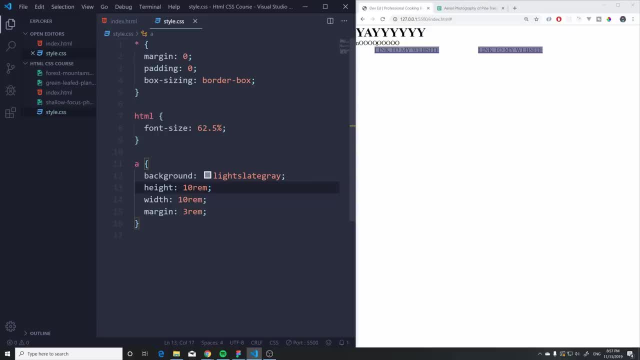 gonna work. it's not gonna add: on top or on bottom: okay, so only left and right. so on bottom: okay, so only left and right. so on bottom: okay, so only left and right. so basically, all you need to remember is basically all you need to remember is: 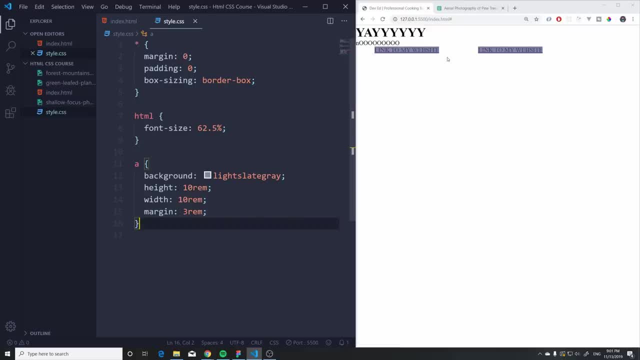 basically, all you need to remember is that inline respects left and right, that inline respects left and right, that inline respects left and right, margins and paddings, but not top, and margins and paddings, but not top and margins and paddings, but not top and bottom. all right, we cannot have a height. 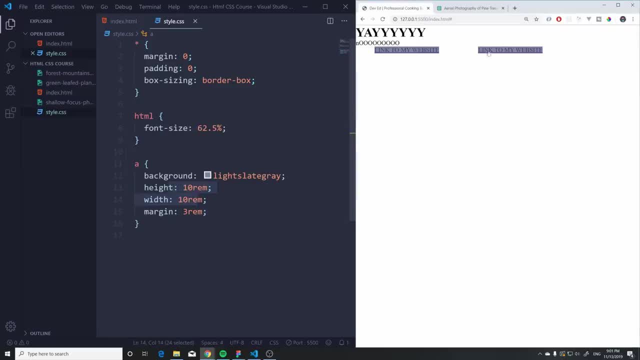 bottom- all right. we cannot have a height bottom- all right. we cannot have a height or what that doesn't work. it allows you, or what that doesn't work. it allows you, or what that doesn't work, it allows you, to add other elements next to it, and 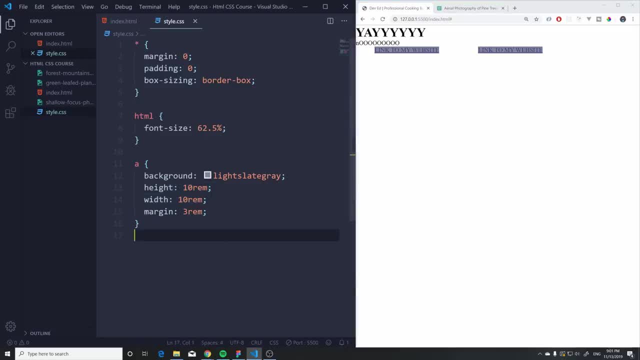 to add other elements next to it and to add other elements next to it, and and that's kind of it okay, now there is, and that's kind of it okay. now there is, and that's kind of it okay. now there is one last one, a special one we can add. 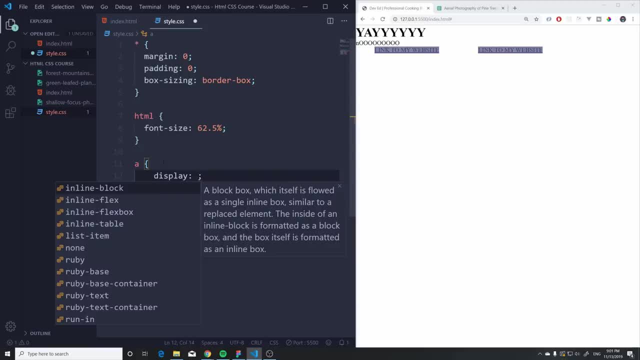 one last one, a special one. we can add one last one, a special one. we can add display and, by the way, we can change display and, by the way, we can change display and, by the way, we can change these if we want. take a look, let me. 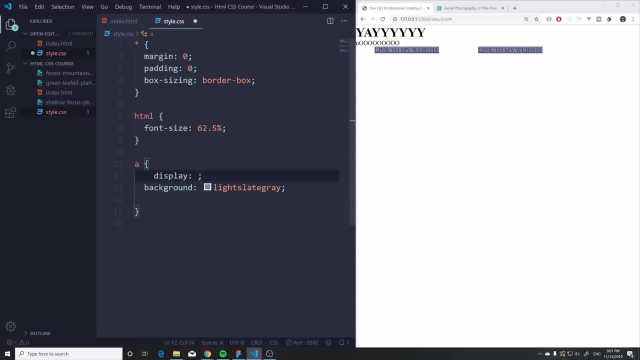 these. if we want take a look, let me these. if we want take a look, let me remove everything here like this, and what remove everything here like this? and what remove everything here like this? and what I'm gonna do is add display block to. I'm gonna do is add display block to. 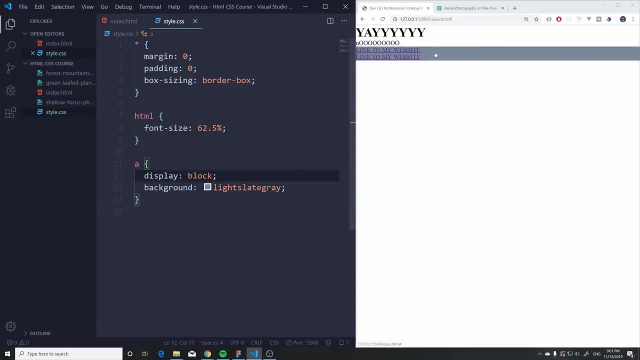 I'm gonna do is add display block to the a text. look, we just transform them to the a text. look, we just transform them to the a text. look, we just transform them to display block. they take up the full display block. they take up the full display block, they take up the full width and they drop to a new line. so 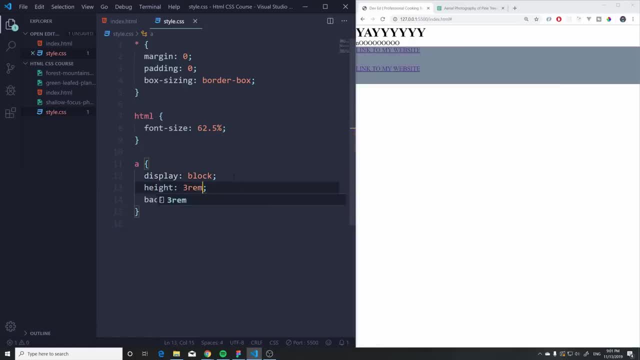 width and they drop to a new line. so width and they drop to a new line. so there we go now I can add the height to there. we go now. I can add the height to there. we go now. I can add the height to it. I can see three rim, and now take a. 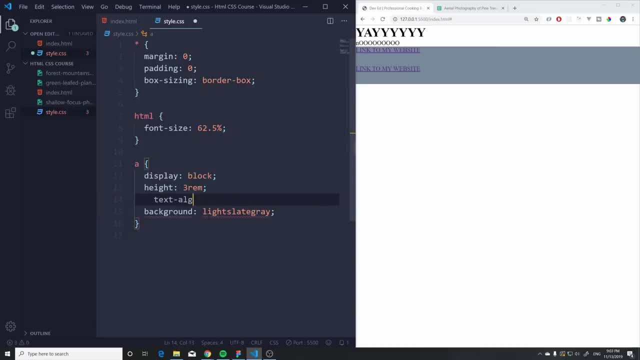 it. I can see three rim. and now take a it. I can see three rim. and now take a look. if you wonder how you can align, look. if you wonder how you can align, look. if you wonder how you can align that to the center, you can add a text. 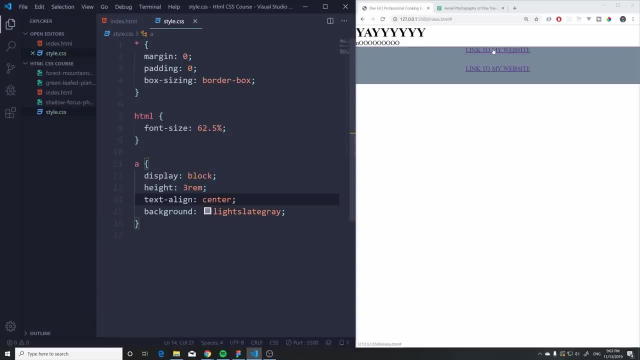 that to the center. you can add a text. that to the center. you can add a text: align Center and it's gonna move it. align Center. and it's gonna move it. align Center and it's gonna move it straight there. nice perfect if you straight there. nice perfect if you. 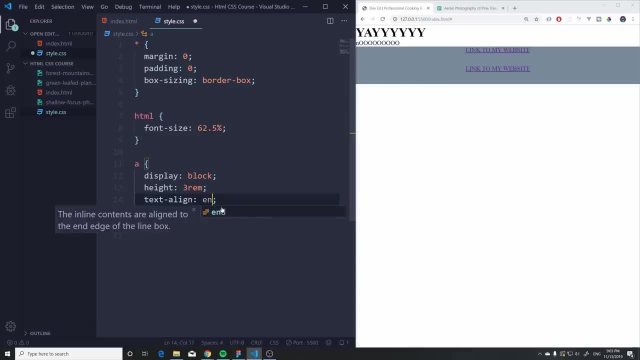 straight there. nice, perfect. if you wonder what else you can do, you can do wonder what else you can do, you can do wonder what else you can do. you can do text the line and you can move it to the text the line and you can move it to the. 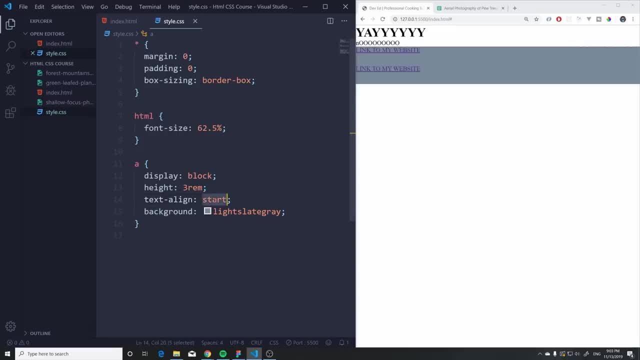 text the line and you can move it to the end and start. obviously it's gonna move end and start. obviously it's gonna move end and start. obviously it's gonna move to the start. there are a few other ones to the start. there are a few other ones. 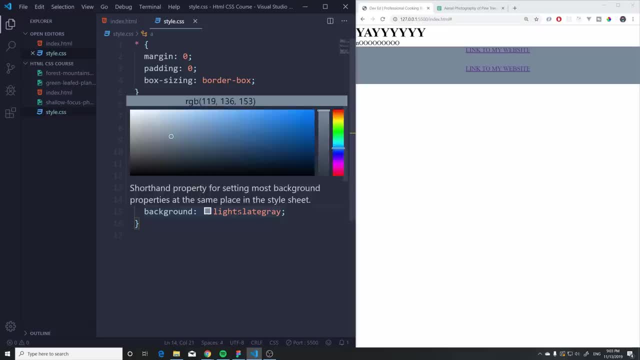 to the start. there are a few other ones, but these are kind of the basic ones. but these are kind of the basic ones, but these are kind of the basic ones that we might use okay perfect, so we that we might use okay perfect, so we that we might use okay perfect, so we moved it there. we can also move this. 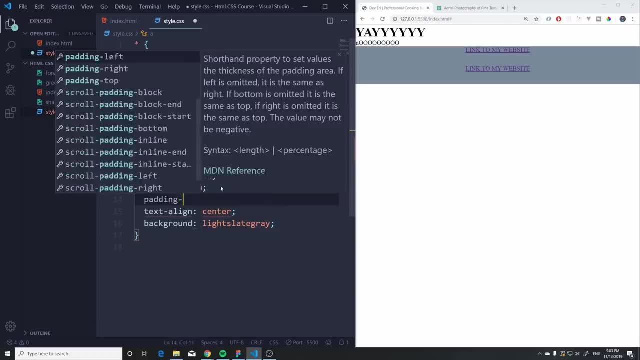 moved it there. we can also move this. moved it there. we can also move this down a bit if we want. we can add a bit down a bit if we want. we can add a bit down a bit if we want. we can add a bit of a padding top if we want. I don't know. 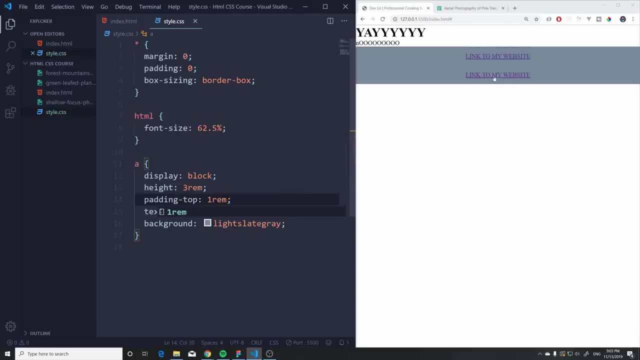 of a padding top if we want. I don't know of a padding top if we want, I don't know. let's do like one REM, that should be. let's do like one REM, that should be. let's do like one REM, that should be fine. that looks okay. okay, so this is. 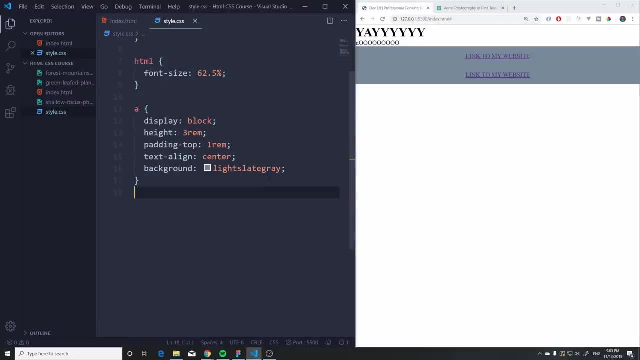 fine, that looks okay, okay. so this is fine, that looks okay, okay. so this is what we have: we can modify it. and lastly, what we have: we can modify it. and lastly, what we have: we can modify it. and lastly, what I want to show you is- maybe I do- 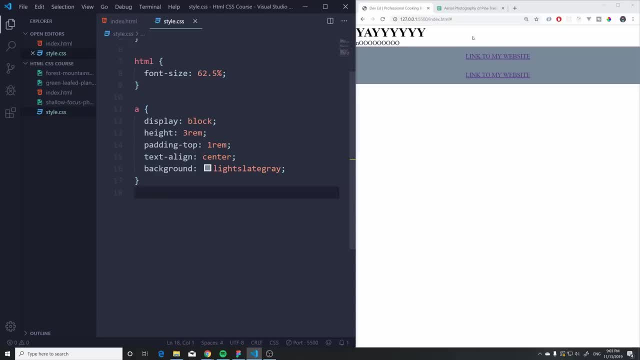 what I want to show you is maybe I do. what I want to show you is maybe I do. you want to have these links, one next to you, want to have these links, one next to you, want to have these links, one next to each other. and I do want to add some. 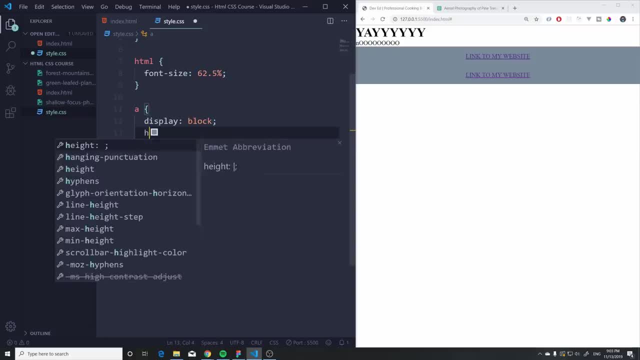 each other and I do want to add some each other and I do want to add some height and padding to them. so how can I height and padding to them? so how can I height and padding to them? so how can I do that? let me remove everything again. 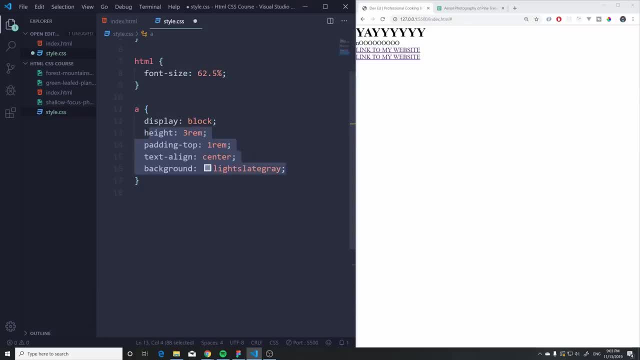 do that, let me remove everything again. do that, let me remove everything again, so we start from scratch. actually I want so we start from scratch. actually I want, so we start from scratch. actually I want that sexy background color, there we go. that sexy background color, there we go. 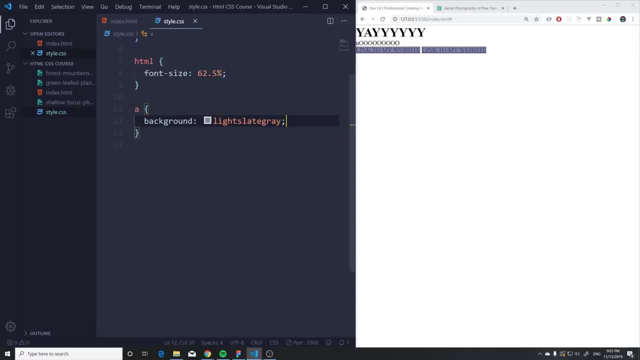 that sexy background color. there we go and this: I'm gonna remove this, so it's. and this: I'm gonna remove this, so it's. and this: I'm gonna remove this, so it's in line. we can change it to something. in line, we can change it to something. 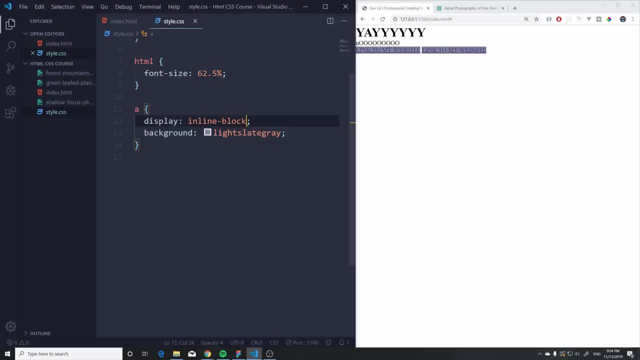 in line. we can change it to something called display inline block and this is called display inline block and this is called display inline block, and this is kind of like a, a combination of the two, kind of like a, a combination of the two, kind of like a, a combination of the two. but the difference is here, with the. 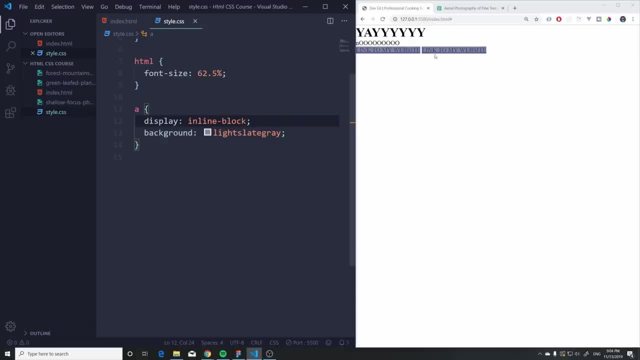 but the difference is here with the, but the difference is here with the inline block is that it respects the top inline block, is that it respects the top inline block, is that it respects the top and bottom margins and padding and it and bottom margins and padding and it. 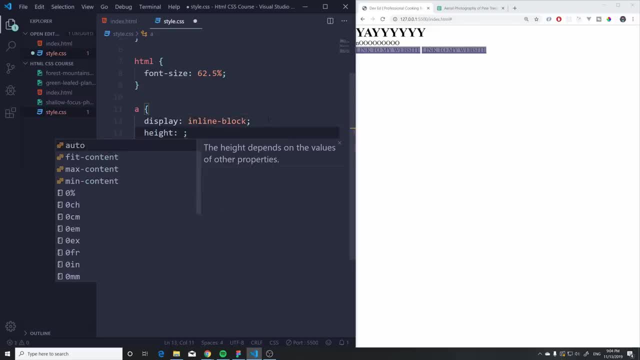 and bottom margins and padding, and it also respects height and width. so if I also respects height and width, so if I also respects height and width, so if I try to add a height of 20 ram to this, I try to add a height of 20 ram to this, I 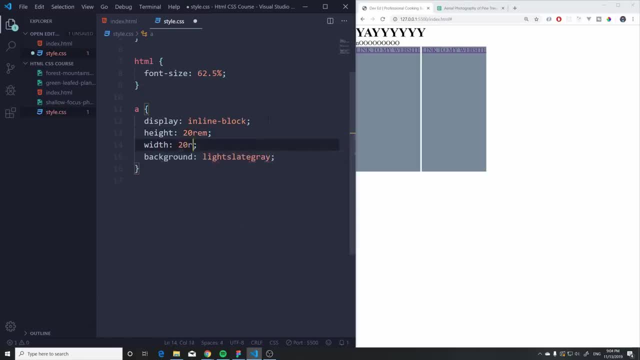 try to add a height of 20 ram to this. I can do it. if I want to add the width of, can do it. if I want to add the width of, can do it. if I want to add the width of 20 ram, I can do that as well. look at. 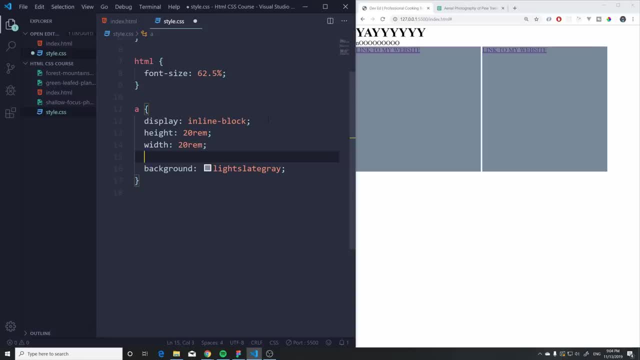 20 ram. I can do that as well. look at 20 ram. I can do that as well. look at that. we have two boxes now and I can that. we have two boxes now and I can that. we have two boxes now, and I can also mess around with margin if I add a. 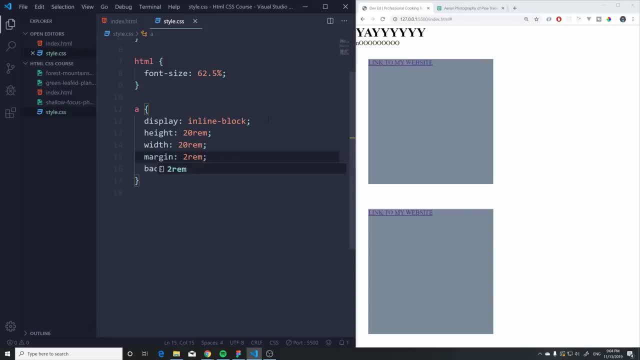 also mess around with margin. if I add a also mess around with margin. if I add a margin of two ram here, that's gonna jump. margin of two ram here, that's gonna jump. margin of two ram here, that's gonna jump it over because it doesn't have any. 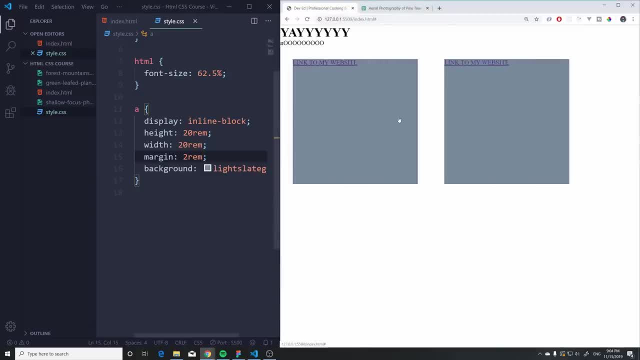 it over because it doesn't have any it over because it doesn't have any space anymore. but, as you can see, it does space anymore. but, as you can see, it does space anymore. but, as you can see, it does add it to the top and it does add it to. 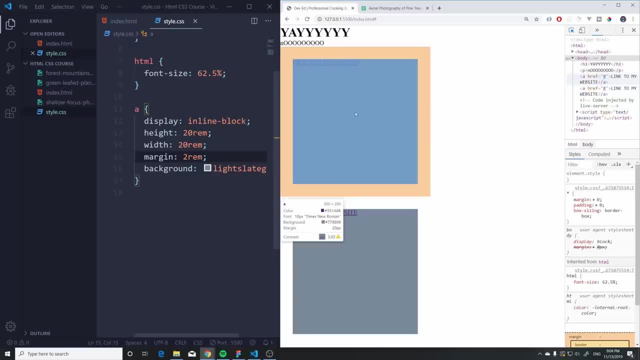 add it to the top, and it does add it to add it to the top, and it does add it to the bottom as well. take a look: the the bottom as well. take a look the the bottom as well. take a look. the anchor tag has top and bottom, same goes. 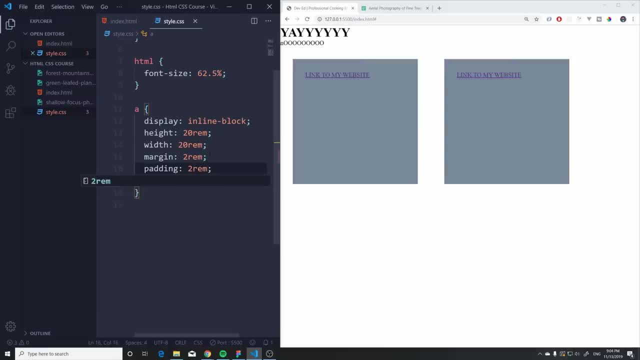 anchor tag has top and bottom. same goes. anchor tag has top and bottom. same goes with padding. so if I drop a padding up with padding, so if I drop a padding up with padding, so if I drop a padding up to rem, that's gonna work just fine as. 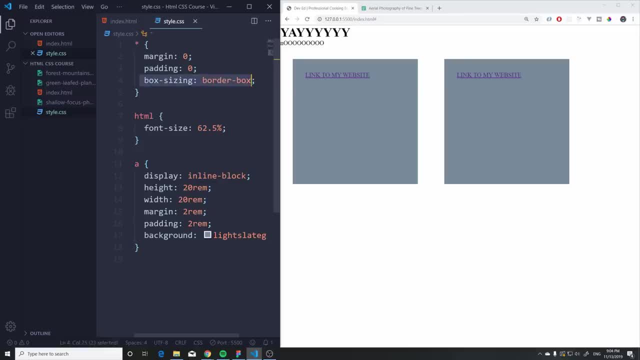 to rem, that's gonna work just fine. as to rem, that's gonna work just fine, as you can see the text moved here. just you can see the text moved here, just you can see the text moved here. just because we have this box sizing border, because we have this box sizing border. 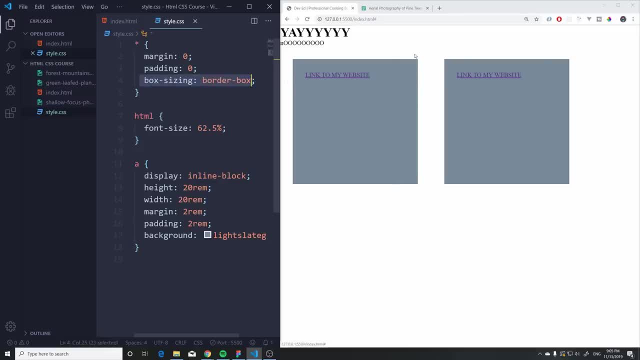 because we have this box sizing border box, so it adds that padding on the box. so it adds that padding on the box. so it adds that padding on the inside, so the element doesn't grow. we inside, so the element doesn't grow. we inside, so the element doesn't grow. we covered this in the last video because 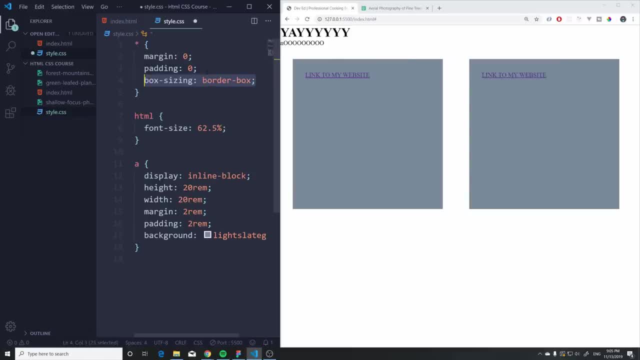 covered this in the last video. because covered this in the last video? because if you remove this, oh no, that's not what. if you remove this, oh no, that's not what. if you remove this, oh no, that's not what we want. so let's add that back, okay. 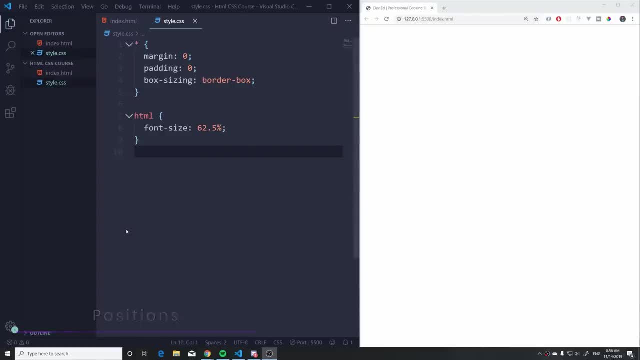 we want, so let's add that back. okay, we want, so let's add that back. okay, there is two more things that I want to. there is two more things that I want to. there is two more things that I want to cover before we start building out. 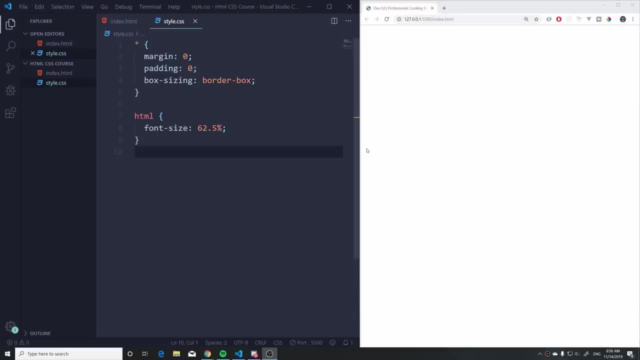 cover before we start building out cover, before we start building out something: a super simple project here. something a super simple project here, something a super simple project here, before we move on to the media queries. before we move on to the media queries, before we move on to the media queries and making mobile friendly things, and 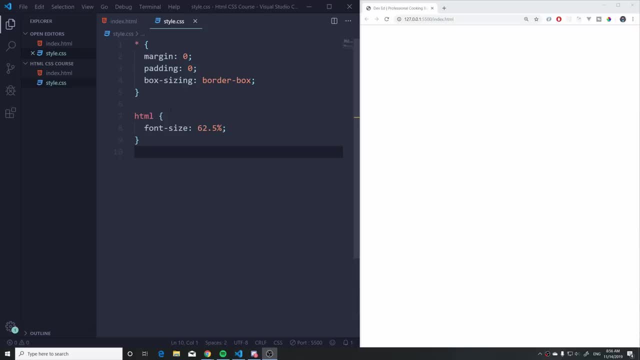 and making mobile friendly things, and and making mobile friendly things, and then building out those three nice, then building out those three nice, then building out those three nice projects. so what I want to cover is projects. so what I want to cover is projects. so what I want to cover is positioning things and let's go into our 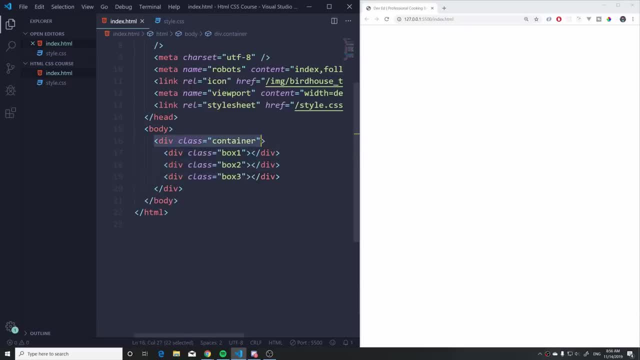 positioning things and let's go into our positioning things and let's go into our HTML here. what I did, I would just add HTML here. what I did, I would just add HTML here. what I did, I would just add it: a div with a class on container and 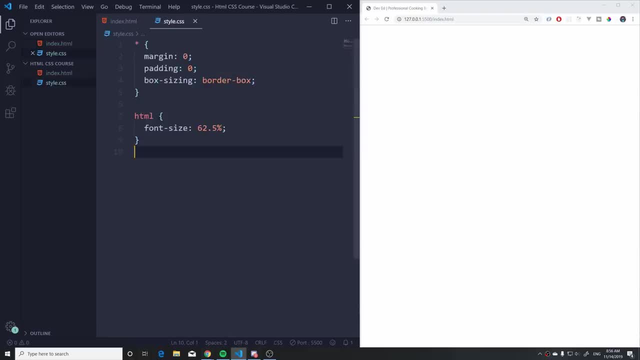 it a div with a class on container, and it a div with a class on container and three boxes inside. so what I want to do, three boxes inside. so what I want to do, three boxes inside. so what I want to do is tile them a bit. so what we're gonna? 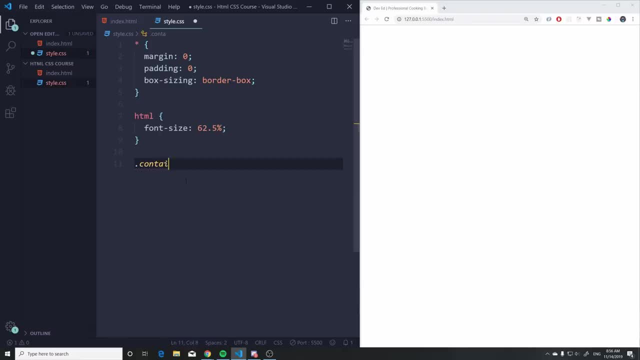 is tile them a bit. so what we're gonna is tile them a bit. so what we're gonna do here is: we're gonna get that container. do here is: we're gonna get that container do here is: we're gonna get that container. like this container, perfect and 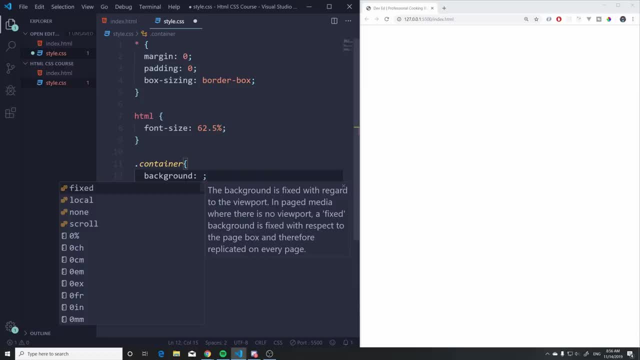 like this container perfect, and like this container, perfect, and I'm just gonna add a dark background color. I'm just gonna add a dark background color. I'm just gonna add a dark background color so we can see this and I want to. so we can see this and I want to. 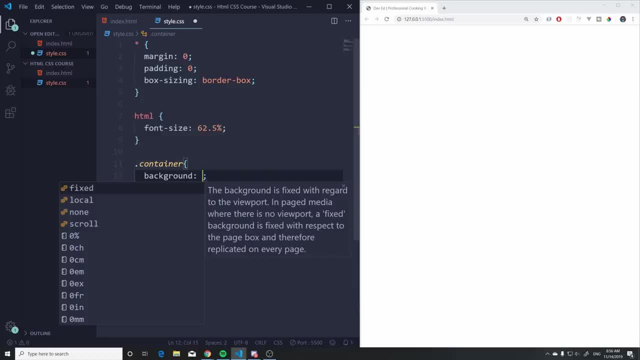 so we can see this and I want to show you a few cool new tricks and CSS. show you a few cool new tricks and CSS. show you a few cool new tricks and CSS that we can do so background, I'll just that we can do so. background, I'll just. 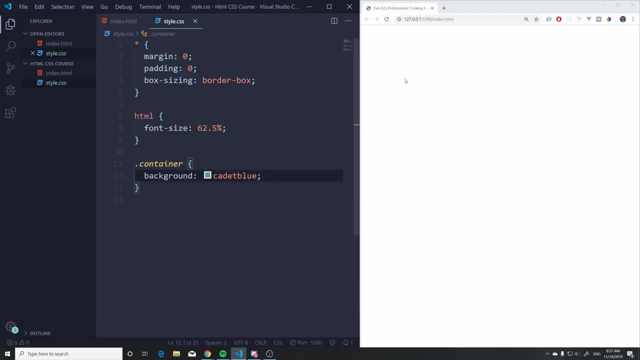 that we can do so. background: I'll just add a color like this and I'll change it. add a color like this and I'll change it. add a color like this and I'll change it afterwards so as you can see right now, afterwards, so as you can see right now. 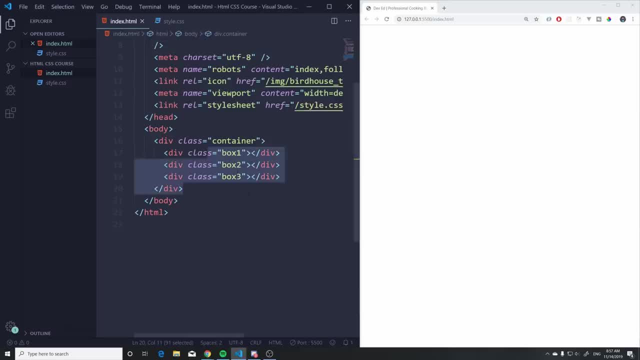 afterwards. so, as you can see, right now we cannot see anything, and the reason we cannot see anything and the reason we cannot see anything, and the reason why we cannot see anything is because we. why we cannot see anything is because we. why we cannot see anything is because we don't have any content in our body. so if 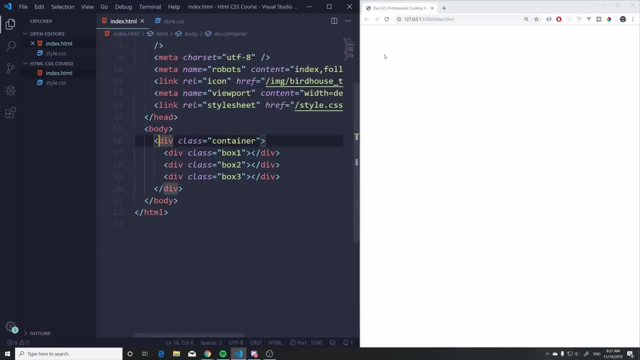 don't have any content in our body. so if don't have any content in our body, so if your content is empty, then you're not. your content is empty, then you're not. your content is empty, then you're not going to see any background color as. 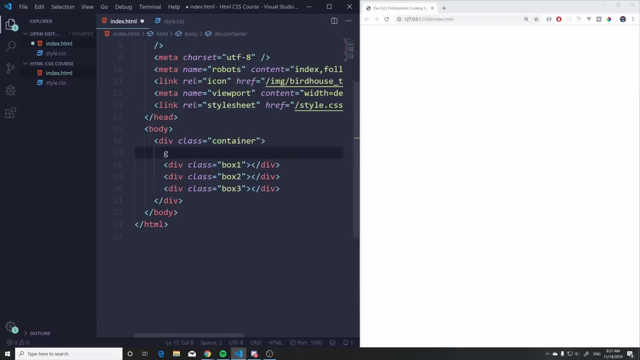 going to see any background color as going to see any background color as soon as we start adding something to it, soon as we start adding something to it, soon as we start adding something to it. so maybe a drop in a h1, here you're. so maybe a drop in a h1, here you're. 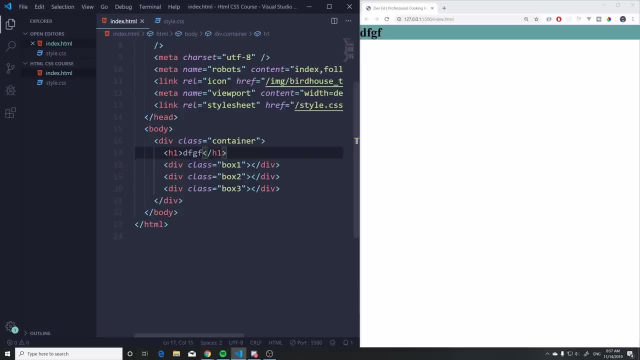 so maybe a drop in a h1 here: you're gonna see that that that background is gonna see that, that that background is gonna see that, that that background is gonna appear. and the reason why this gonna appear and the reason why this gonna appear and the reason why this happens is because by default, we cannot. 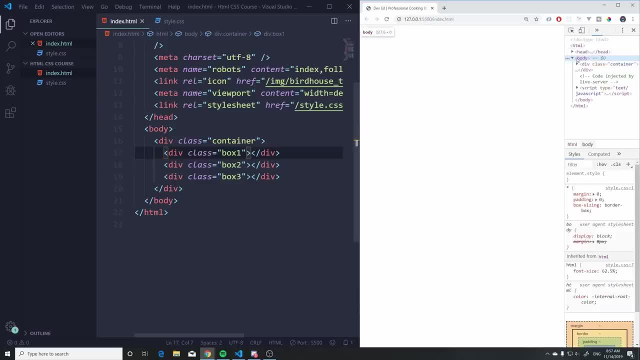 happens is because by default we cannot happens is because by default we cannot see the HTML or the body. because as see the HTML or the body? because as see the HTML or the body? because as long as there's no content in it, the long as there's no content in it, the 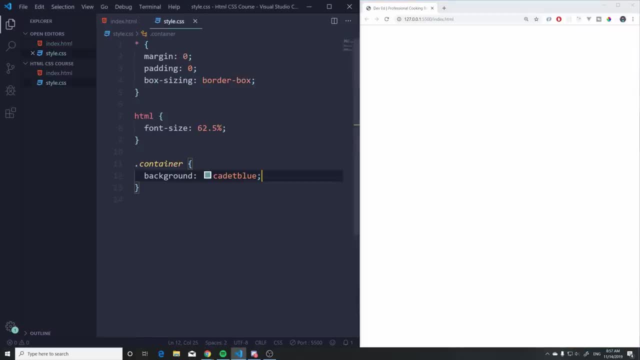 long as there's no content in it, the height is not gonna be set, so we can. height is not gonna be set, so we can. height is not gonna be set, so we can change that. that's okay. so if we want to change that, that's okay. so if we want to. 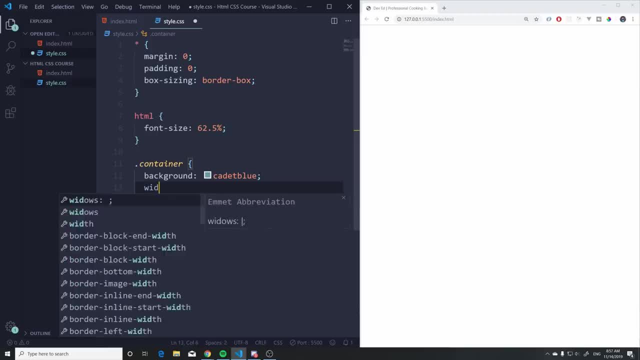 change that. that's okay. so if we want to see something here, what we can do is we see something here. what we can do is we see something here. what we can do is we can add a width that we can see. so if I can add a width that we can see, so if I 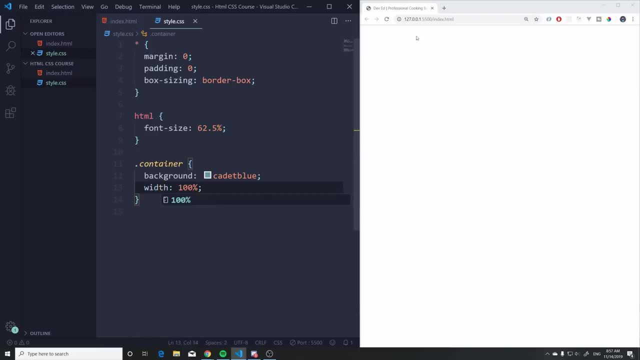 can add a width that we can see. so if I had a hundred percent here, well, we still had a hundred percent here, well, we still had a hundred percent here, well, we still cannot see because we don't have any, cannot see because we don't have any. 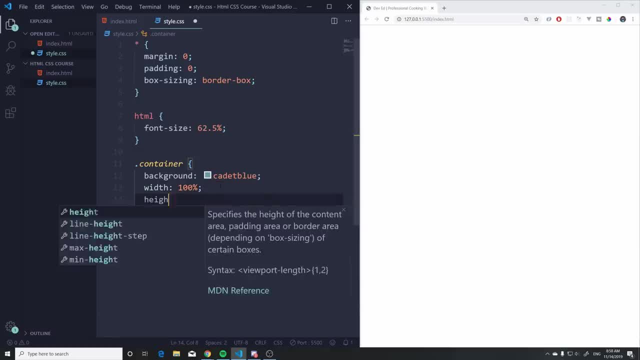 cannot see because we don't have any height. so the interesting thing is if I height. so the interesting thing is if I height. so the interesting thing is if I try to set a height to this of 100%, to try to set a height to this of 100%, to. 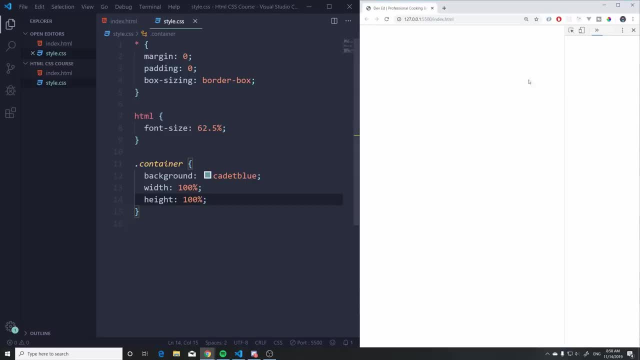 try to set a height to this of 100% to take up the full screen. we cannot see. take up the full screen. we cannot see. take up the full screen. we cannot see anything. and again, that's the reason why. anything. and again that's the reason why. 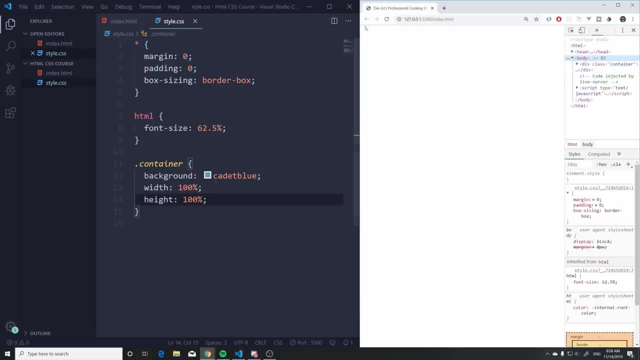 anything. and again, that's the reason why: because we have no content here and the because we have no content here and the because we have no content here and the body is set to, it doesn't have a height. body is set to, it doesn't have a height. 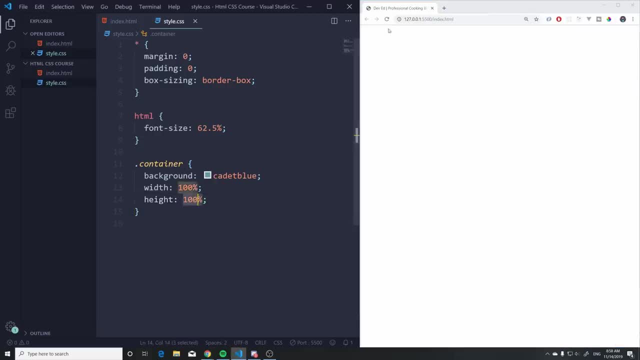 body is set to, it doesn't have a height. so when you try to set the height of so, when you try to set the height of so, when you try to set the height of 100% of nothing, then nothing's gonna. 100% of nothing, then nothing's gonna. 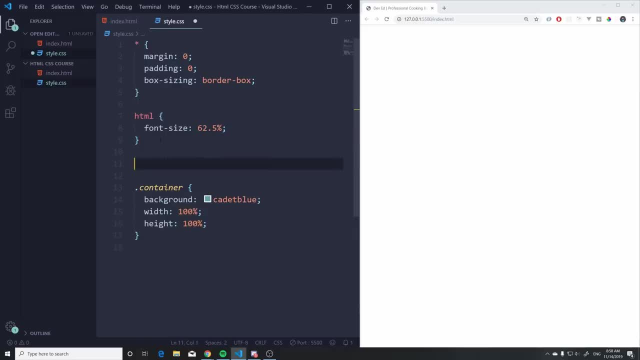 100% of nothing, then nothing's gonna happen. so a quick fix for this is gonna happen. so a quick fix for this is gonna happen. so a quick fix for this is gonna be to take the HTML and the body and be to take the HTML and the body and 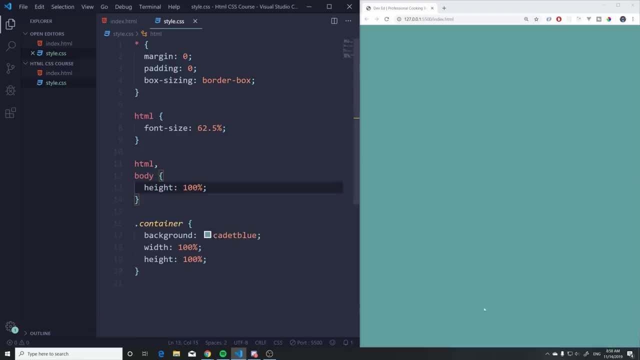 be to take the HTML and the body and just add a height of 100% to it, and just add a height of 100% to it, and just add a height of 100% to it, and that's gonna stretch all the way down. that's gonna stretch all the way down. 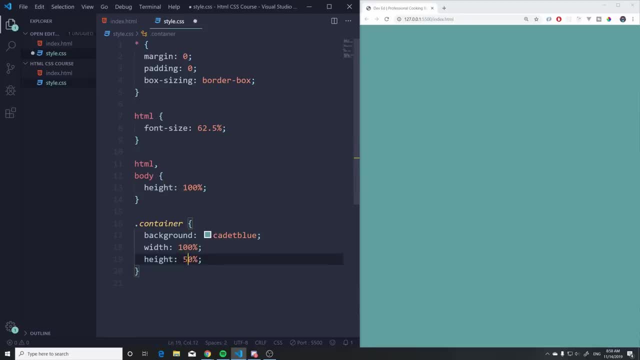 that's gonna stretch all the way down here, okay. and now if I change the height here? okay. and now if I change the height here, okay. and now if I change the height of the container to something like 50% of the container, to something like 50%. 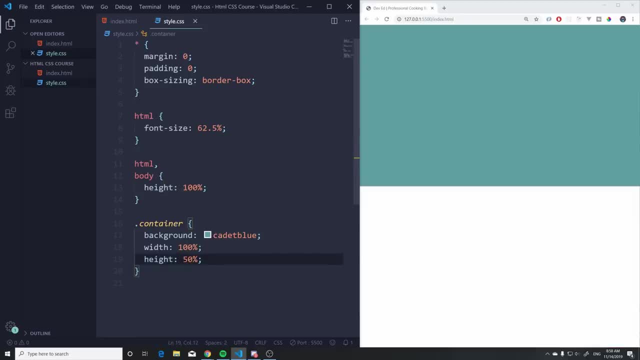 of the container to something like 50%, then it's gonna take 50% of the height. then it's gonna take 50% of the height. then it's gonna take 50% of the height of the body. now we're gonna look at a. 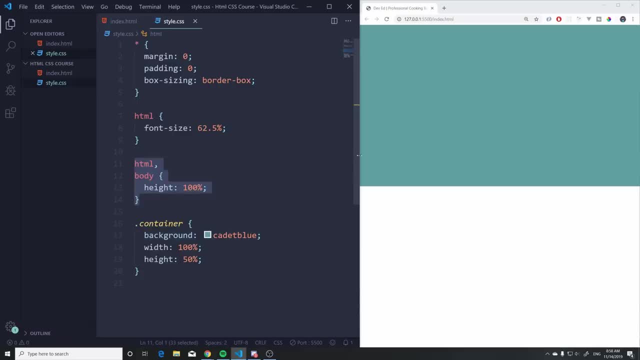 of the body. now we're gonna look at a of the body. now we're gonna look at a better solution than this. when we get to better solution than this, when we get to better solution than this, when we get to responsive media with VH and VW, you're. 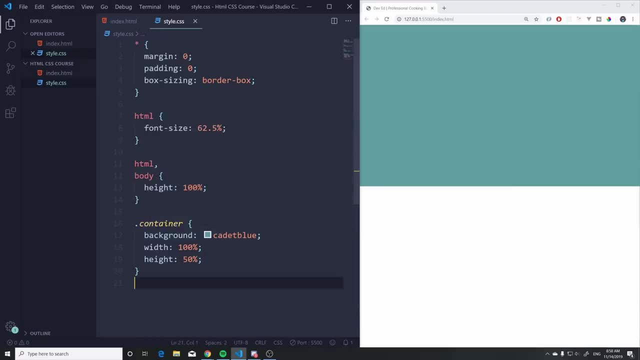 responsive media with VH and VW. you're responsive media with VH and VW. you're gonna see that it's gonna be more fun. gonna see that it's gonna be more fun. gonna see that it's gonna be more fun. okay, but for now we're gonna set it like: 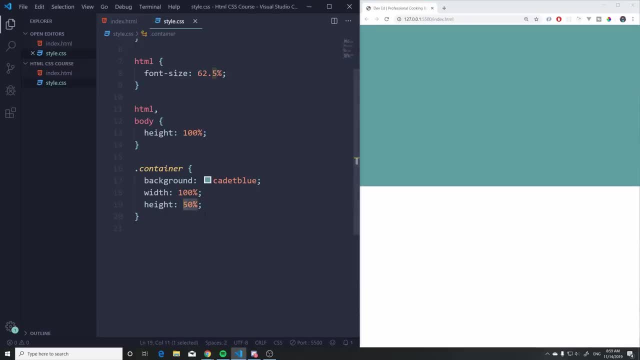 okay, but for now we're gonna set it like okay, but for now we're gonna set it like this, which is completely fine. so I this, which is completely fine, so I this, which is completely fine, so I actually want this to be around. let's actually want this to be around. let's do 80%. and the width, let's also do 80%. 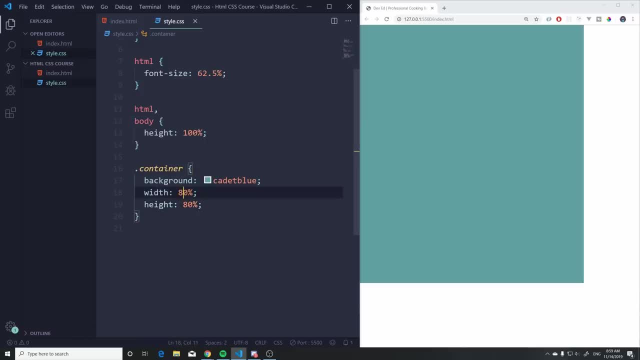 do 80% and the width, let's also do 80%. do 80% and the width. let's also do 80% on the width. okay, so something like that on the width. okay, so something like that on the width. okay, so something like that. and what, if I want to Center this in the 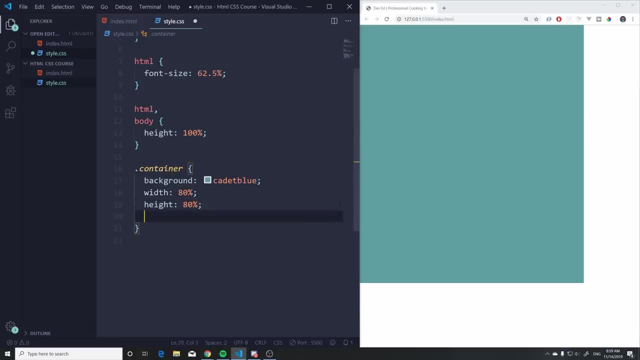 and what if I want to Center this in the? and what if I want to Center this in the middle? there's a cool trick that you can middle. there's a cool trick that you can middle. there's a cool trick that you can do with margin. if we set margin to auto. 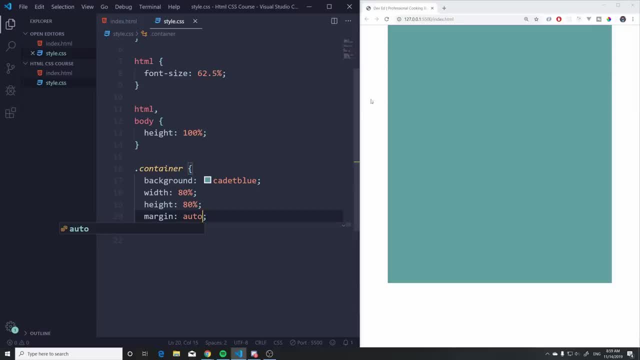 do with margin. if we set margin to auto. do with margin. if we set margin to auto, it's automatically gonna allocate the. it's automatically gonna allocate the. it's automatically gonna allocate the space on the left side and on the right, space on the left side and on the right. 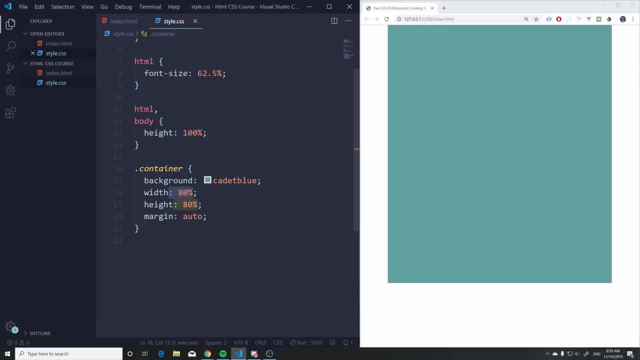 space on the left side and on the right side. it's gonna split up the remaining side. it's gonna split up the remaining side. it's gonna split up the remaining width here, so 10% and 10%, and it's gonna. width here, so 10% and 10%, and it's gonna. 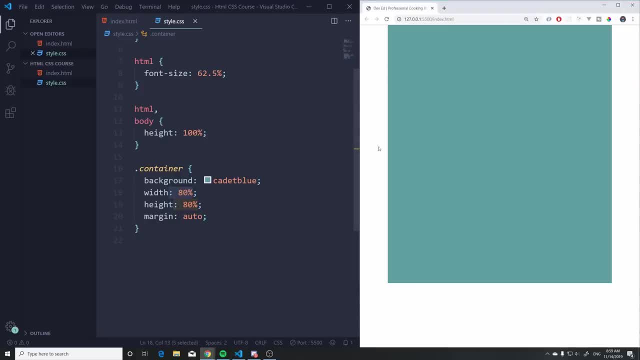 width here. so 10% and 10% and it's gonna drop it on the left and on the right. so drop it on the left and on the right. so drop it on the left and on the right. so whenever you want to take a div or a. 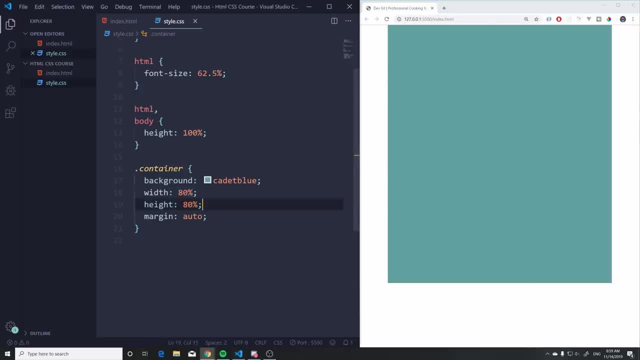 whenever you want to take a div or a, whenever you want to take a div or a container or some sort and you want to container or some sort and you want to container or some sort and you want to position it in the middle, you can do a. 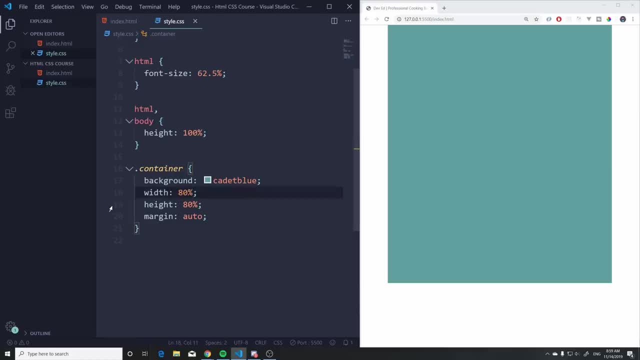 position it in the middle, you can do a. position it in the middle, you can do a margin auto as long as your width is margin auto, as long as your width is margin auto, as long as your width is smaller than 100%, because if it's one, 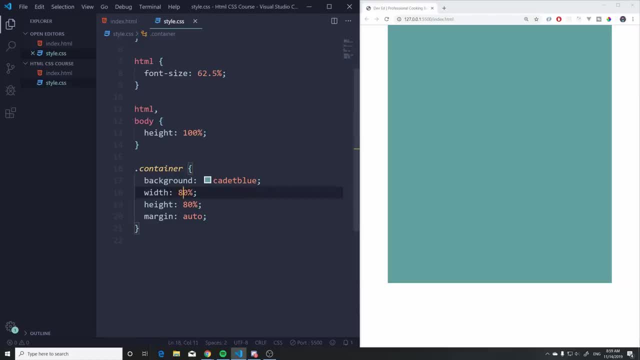 smaller than 100%, because if it's one smaller than 100%, because if it's one hundred percent, then it's gonna take up hundred percent, then it's gonna take up hundred percent, then it's gonna take up the whole screen. okay, so let's do. 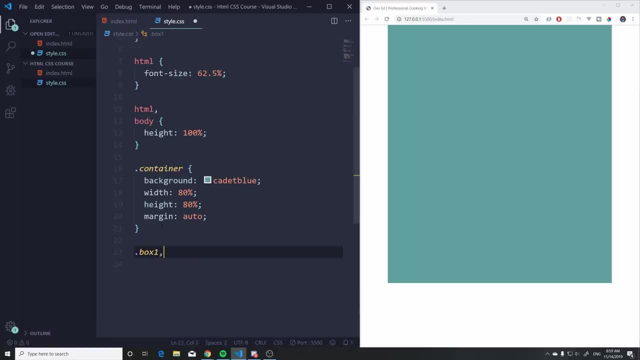 the whole screen. okay, so let's do the whole screen. okay. so let's do something here with the boxes. I'm gonna something here with the boxes. I'm gonna something here with the boxes. I'm gonna take box one, box two and comma box three. take box one, box two and comma box three. 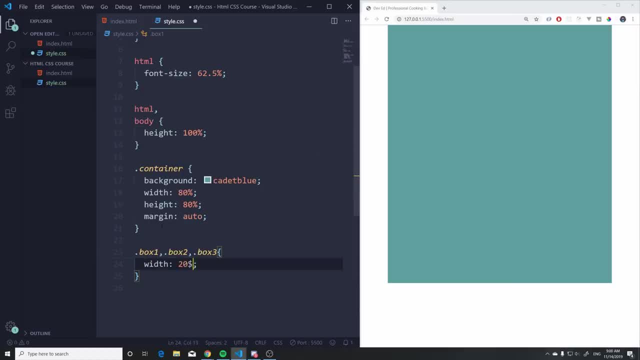 take box one, box two and comma box three, so I can select all of them and add the. so I can select all of them and add the. so I can select all of them and add the width to them. so I can do 20% and the. 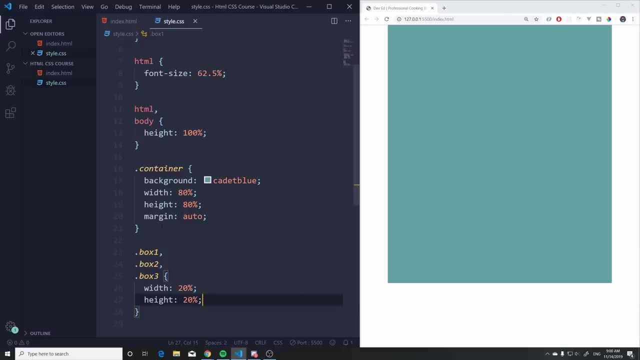 width to them, so I can do 20%. and the width to them, so I can do 20%. and the height of 20%, like this, and hit save: height of 20%. like this, and hit save. height of 20%. like this, and hit save. okay, now, if I go down here, I can add a. 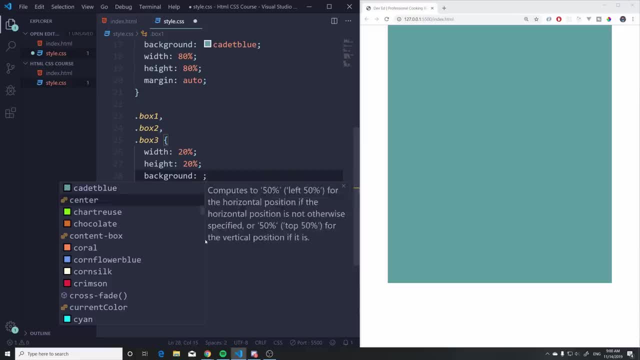 okay, now, if I go down here, I can add a. okay, now, if I go down here, I can add a background color to all of them. I can do background color to all of them. I can do background color to all of them. I can do background. let's do something intense. 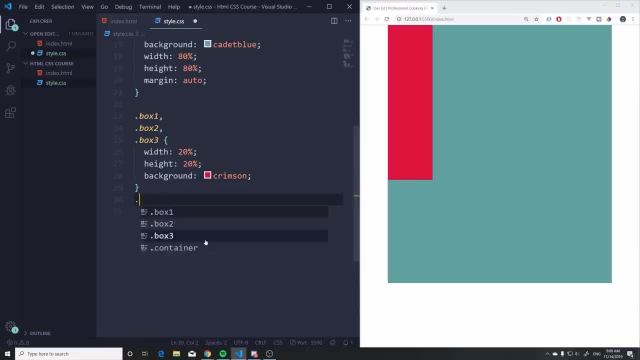 background. let's do something intense background. let's do something intense like this amazing. and what I can do now like this amazing, and what I can do now, like this amazing and what I can do now is just like box two and just change the is just like box two and just change the. 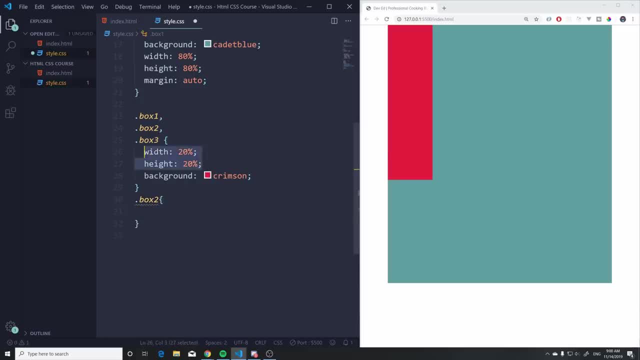 is just like box two and just change the background color. so the reason why I background color, so the reason why I background color, so the reason why I did this was so I'm not, so I don't did this was so I'm not, so I don't. 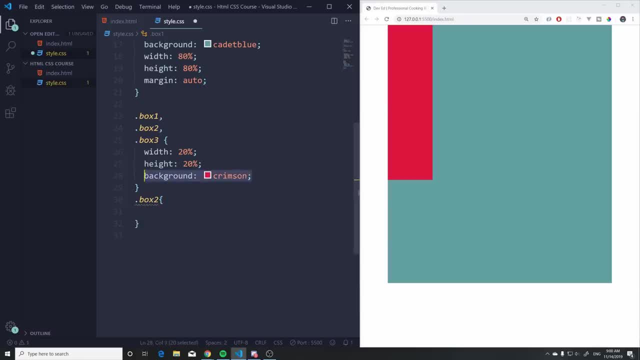 did this was so. I'm not, so I don't. duplicate these settings over and over. duplicate these settings over and over. duplicate these settings over and over again. so we change the background color again. so we change the background color again. so we change the background color there. let's change it here as well. so. 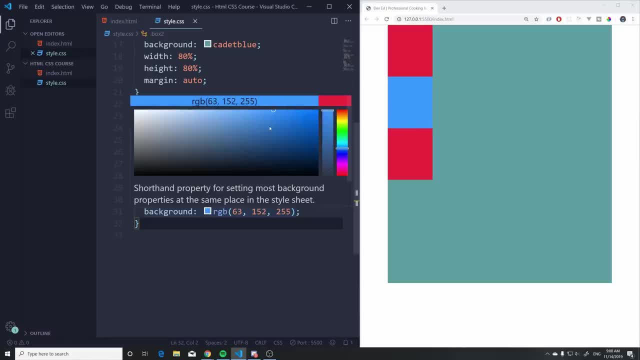 there, let's change it here as well. so there, let's change it here as well. so, let's do something like an intense blue. let's do something like an intense blue. let's do something like an intense blue. all right, these colors make me sad I. all right, these colors make me sad I. 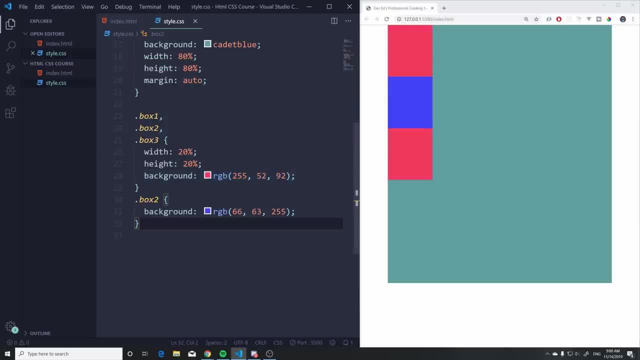 all right. these colors make me sad. I don't like the way they look. I want to don't like the way they look. I want to don't like the way they look. I want to make them obvious, but I don't want them. make them obvious, but I don't want them. 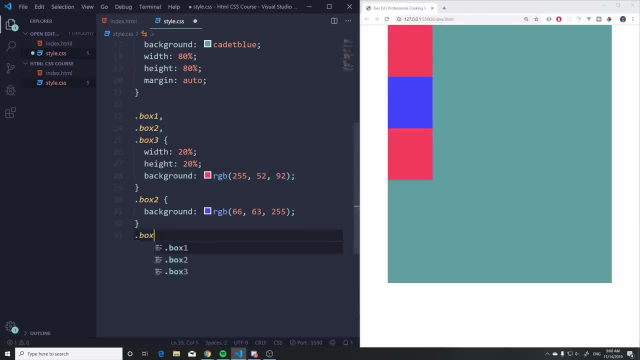 make them obvious, but I don't want them to make your eyes hurt, so let's also to make your eyes hurt. so let's also to make your eyes hurt. so let's also take box 3 here and add a back. let's take box 3 here and add a back. let's. 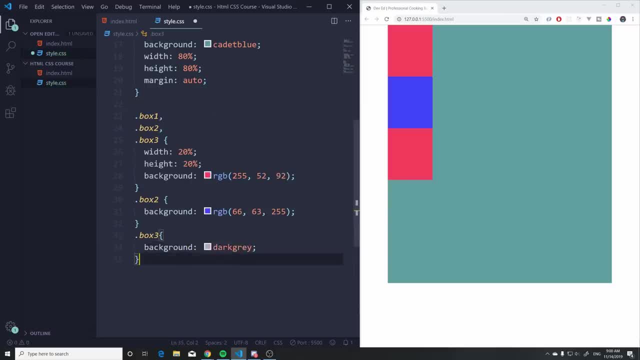 take box 3 here and add a back. let's try a green color, not dark gray. try a green color, not dark gray. try a green color, not dark gray. let's show we do a dark one. let's do a. let's show we do a dark one. let's do a. 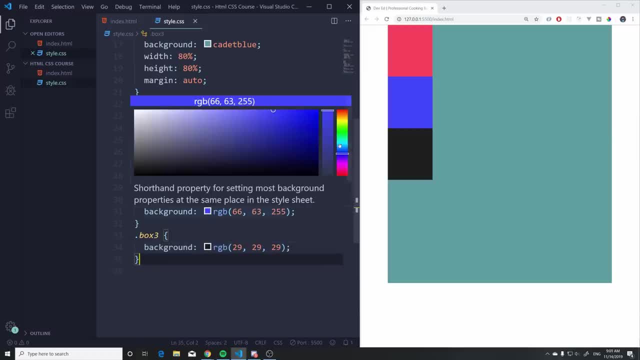 let's show we do a dark one. let's do a dark one, there we go. dark one, there we go. dark one, there we go. that's too green, poor green has there we. that's too green, poor green has there we. that's too green, poor green has there. we are like an ocean, ocean color and the 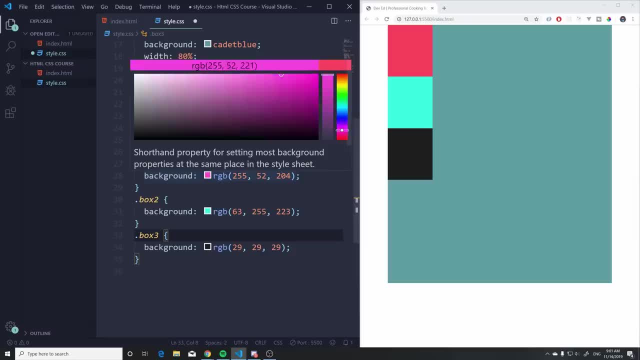 are like an ocean ocean color. and the are like an ocean ocean color. and the red can leave as well with a nice pink red, can leave as well with a nice pink red, can leave as well with a nice pink purple. okay, there we go, some new colors. 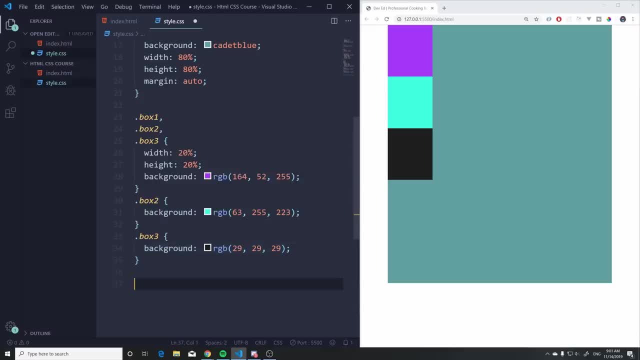 purple- okay, there we go some new colors. purple- okay, there we go some new colors there for you. so let's take a look at there for you. so let's take a look at there for you. so let's take a look at these positions. what our positions? how do? 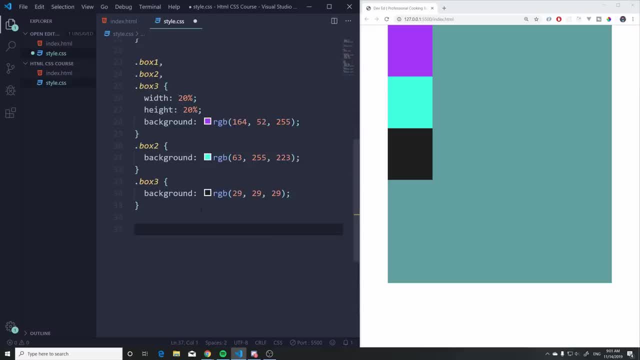 these positions, what our positions? how do these positions? what our positions? how do we apply them? what do they do? let's we apply them. what do they do? let's we apply them. what do they do? let's try it with the box. let's let's try it. 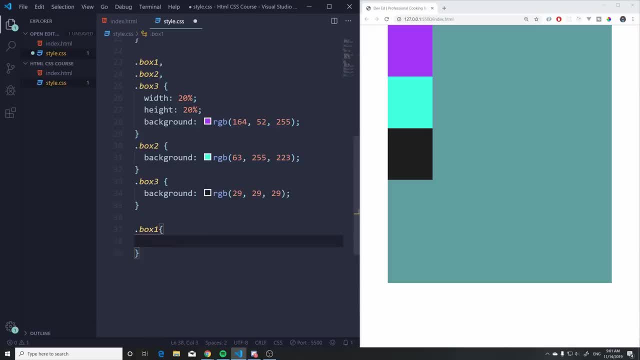 try it with the box. let's, let's try it. try it with the box. let's try it with the box one. okay, the first one, the with the box one. okay, the first one, the with the box one. okay, the first one, the purple lovely box. so what happens if I? 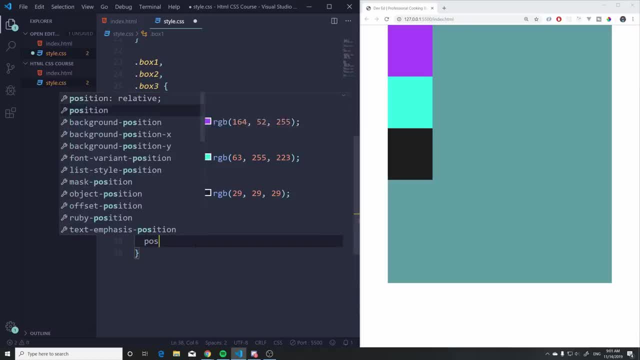 purple lovely box. so what happens if I purple lovely box? so what happens if I add by default: all elements are add by default. all elements are add by default. all elements are positioned static like this and as you positioned, static like this and as you positioned, static like this and as you can see, it says: the box is a normal box. 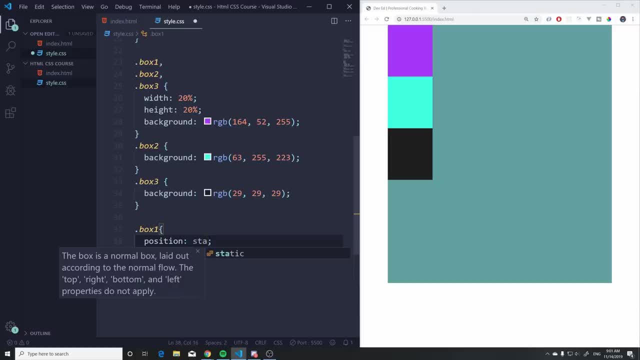 can see it says the box is a normal box. can see it says the box is a normal box, laid according to the normal flow, all laid according to the normal flow, all laid according to the normal flow, all right. so the way we basically added the right, so the way we basically added the, 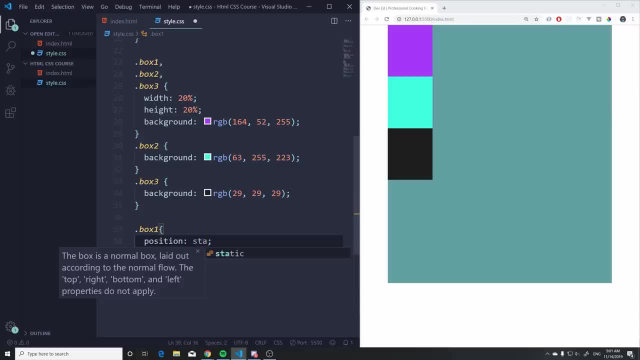 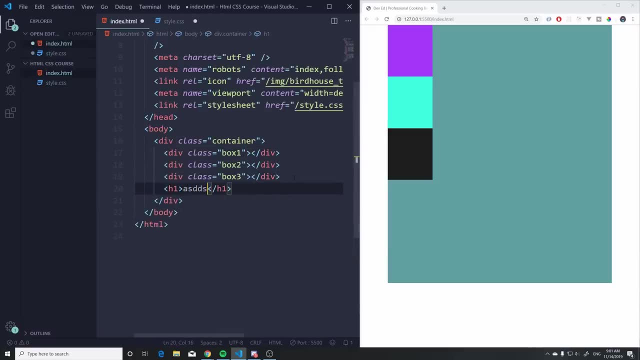 right. so the way we basically added the elements in our HTML, that's the way. elements in our HTML. that's the way. elements in our HTML. that's the way here. if I had a h1- blah, blah, blah, hit here. if I had a h1- blah, blah, blah, hit. 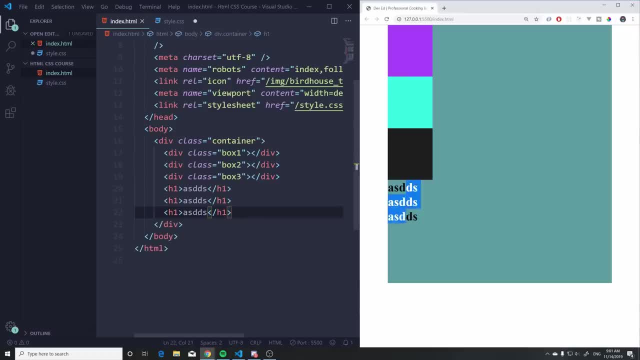 here if I had a h1 blah, blah blah, hit save. so they're just going with the save. so they're just going with the save. so they're just going with the normal flow of the HTML. okay, so nothing. normal flow of the HTML. okay, so nothing. 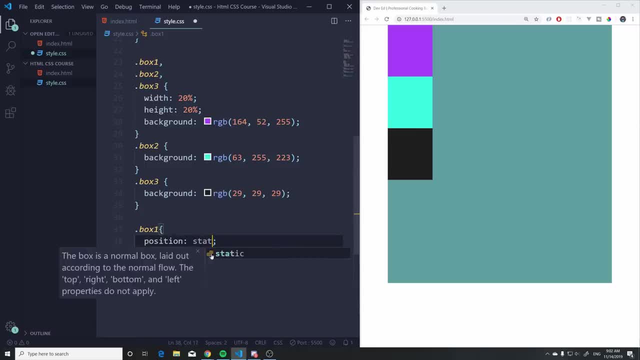 normal flow of the HTML. okay, so nothing really special. however, if I change the really special, however, if I change the really special, however, if I change the position static as you can see nothing. position static as you can see nothing. position static as you can see nothing happens to position absolute. let's say: 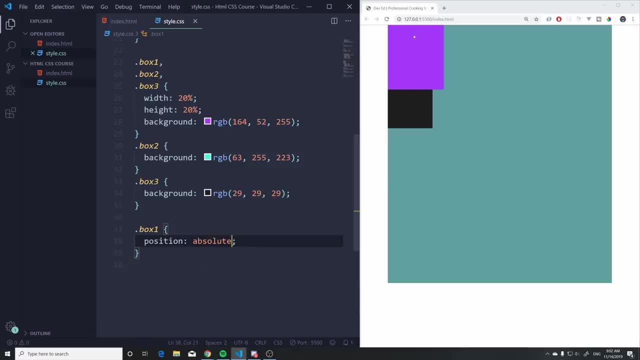 happens to position absolute, let's say: happens to position absolute, let's say absolute. what's gonna happen? is that absolute? what's gonna happen, is that absolute. what's gonna happen is that this element is gonna be ripped out of. this element is gonna be ripped out of. 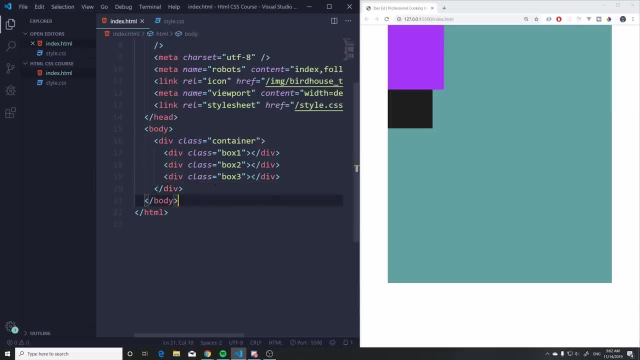 this element is gonna be ripped out of the normal document flow. you can think the normal document flow, you can think the normal document flow. you can think of it as we literally just take out the of it, as we literally just take out the of it, as we literally just take out the element and it doesn't care about where. 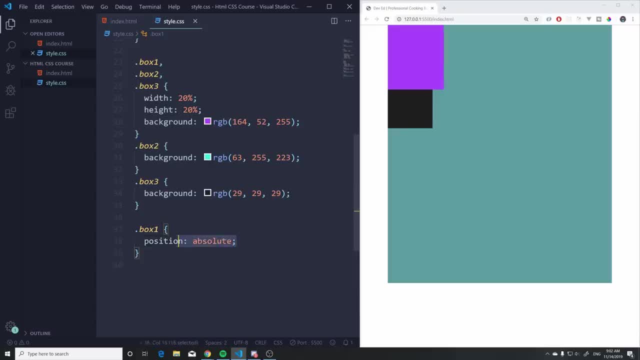 element and it doesn't care about where element and it doesn't care about where it is in the position anymore. so what it is in the position anymore, so what it is in the position anymore. so what happened- and it's a bit hard to see, but happened and it's a bit hard to see, but 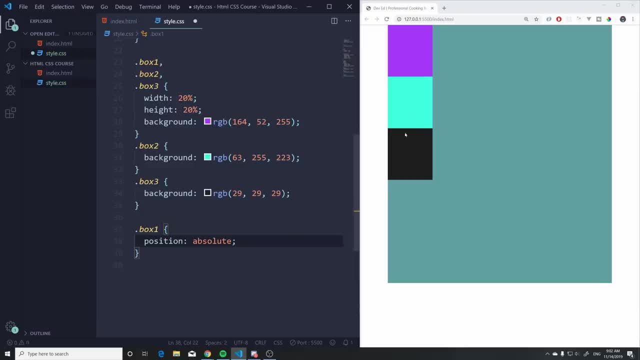 happened and it's a bit hard to see, but as soon as we add this, these two get. as soon as we add this, these two get. as soon as we add this, these two get pushed up all right. so it's kind of like: pushed up, all right. so it's kind of like. 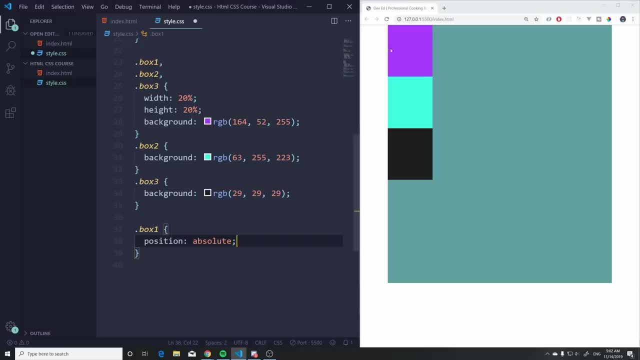 pushed up, all right. so it's kind of like this doesn't exist anymore. so it's kind this doesn't exist anymore. so it's kind this doesn't exist anymore. so it's kind of like we grab this out of here and of like we grab this out of here and 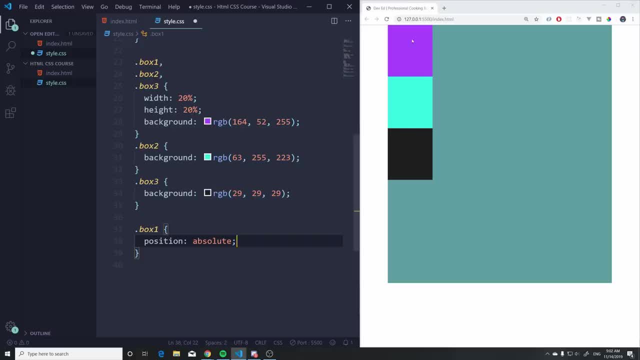 of like: we grab this out of here and these other boxes just get pushed up, these other boxes just get pushed up. these other boxes just get pushed up because it's like, oh, I have empty space. because it's like, oh, I have empty space. because it's like, oh, I have empty space, I shouldn't be down here, so they get. 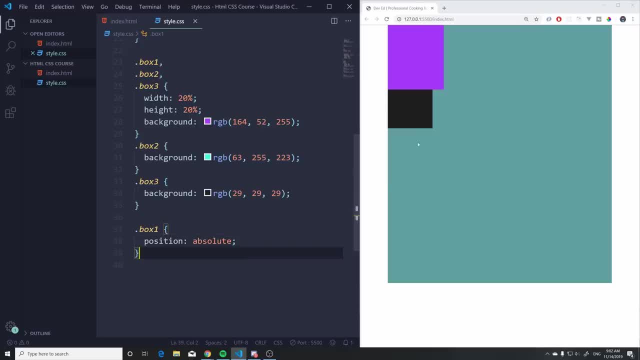 I shouldn't be down here so they get. I shouldn't be down here so they get pushed up. so if I had saved, this gets pushed up. so if I had saved, this gets pushed up. so if I had saved, this gets taken out and those elements get pushed. 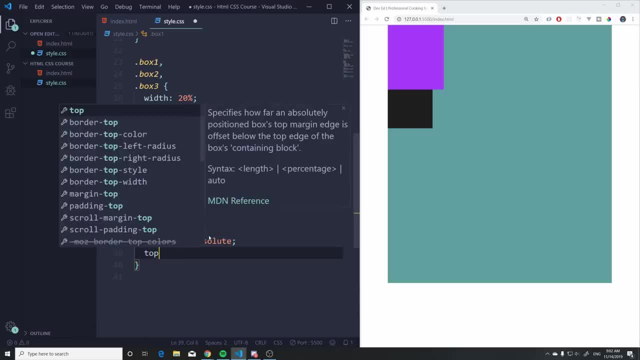 taken out and those elements get pushed taken out and those elements get pushed up, and now we have access to four new up, and now we have access to four new up, and now we have access to four new properties called top, left, bottom and properties called top, left, bottom and. 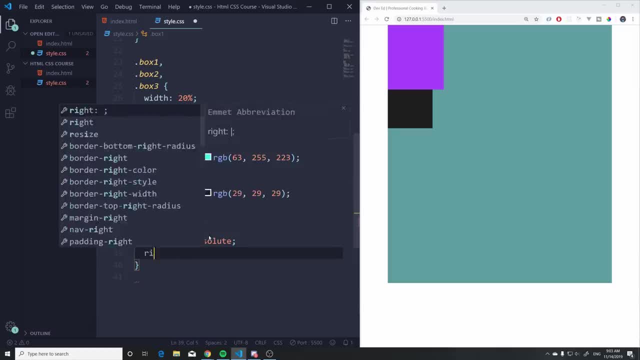 properties called top, left, bottom and right. and what happens if we add so right? and what happens if we add so right? and what happens if we add so? let's try what if I do bottom zero REM? let's try what if I do bottom zero REM? let's try what if I do bottom zero REM. it's safe. as you can see, it gets stuck. 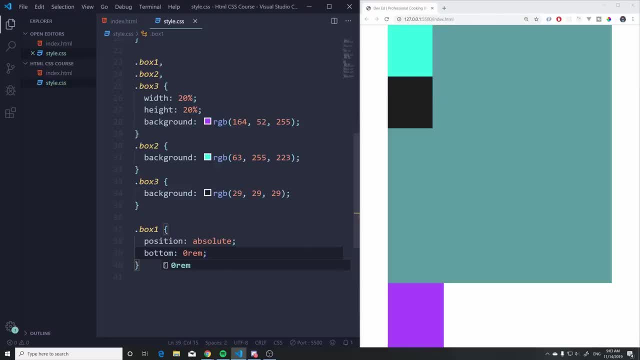 it's safe, as you can see, it gets stuck. it's safe, as you can see. it gets stuck at the bottom of the page here, okay, at the bottom of the page here, okay, at the bottom of the page here, okay. what happens if I add left, left, zero, we? 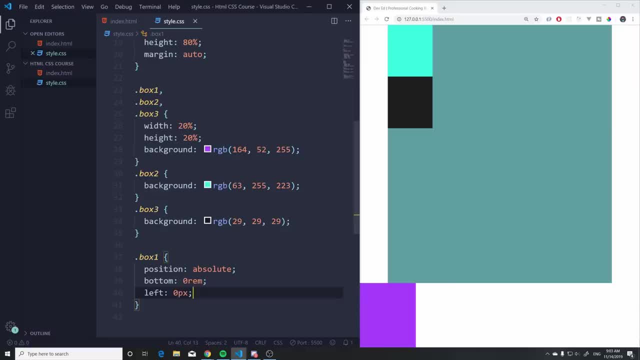 what happens if I add left, left zero? we what happens if I add left, left, zero? we can even see zero pixels, that's fine. it can even see zero pixels, that's fine. it can even see zero pixels, that's fine. it gets stuck to the left here. now, as you. 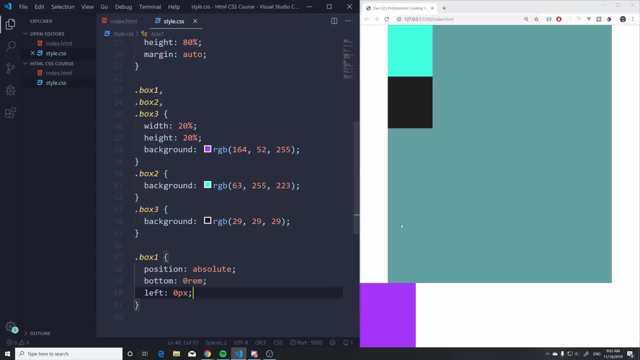 gets stuck to the left here now as you gets stuck to the left here now, as you can see these got pushed up here and it can see these got pushed up here and it can see these got pushed up here and it doesn't care about this box, that it was. 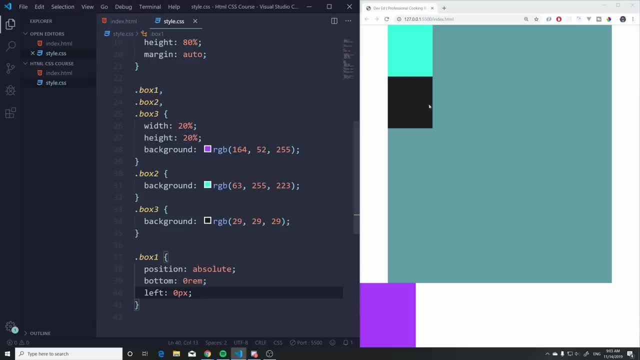 doesn't care about this box that it was. doesn't care about this box that it was in. you can imagine like it doesn't care in. you can imagine like it doesn't care in. you can imagine like it doesn't care about anything. it gets ripped out of the. 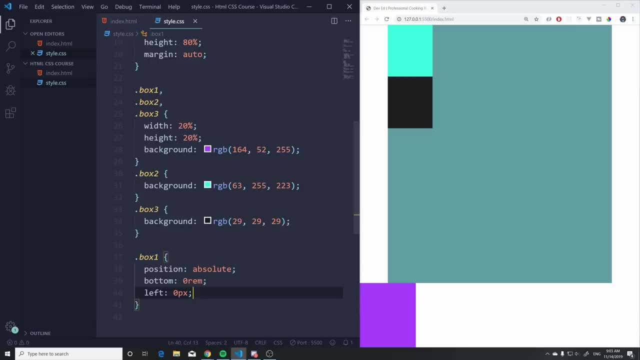 about anything. it gets ripped out of the about anything. it gets ripped out of the page and it just sits where you want it page and it just sits where you want it page and it just sits where you want it to sit. so zero basically means here left. 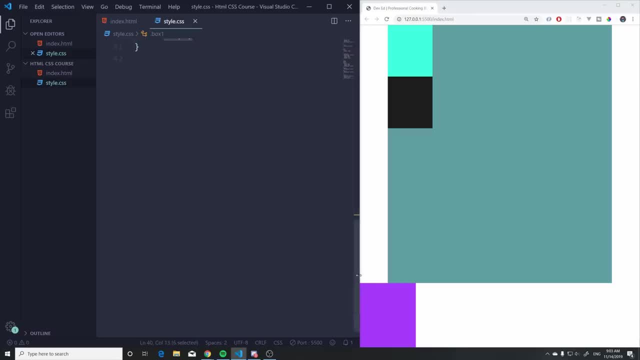 to sit, so zero basically means here left to sit, so zero basically means here left. zero, basically zero pixels away from the zero, basically zero pixels away from the zero, basically zero pixels away from the left side of the screen here. so if I left side of the screen here, so if I 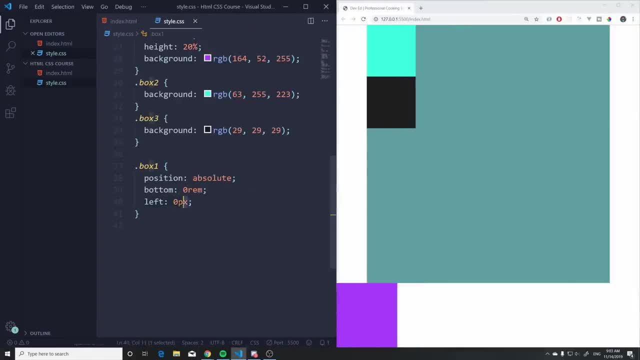 left side of the screen here. so if I move this around as you can see zero, if move this around as you can see zero, if move this around as you can see zero, if I add some pixels here, or let's do REM. I add some pixels here, or let's do REM. 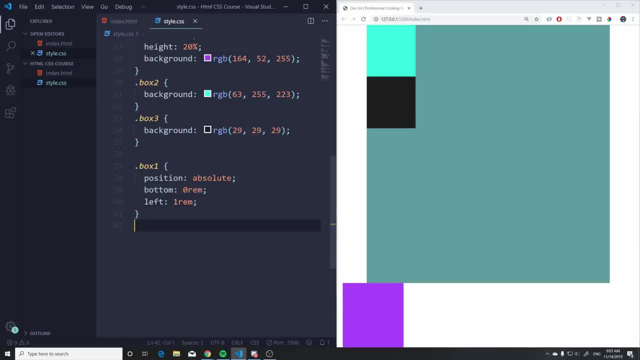 I add some pixels here, or let's do REM one rim. it's gonna have 10 pixels from one rim. it's gonna have 10 pixels from one rim. it's gonna have 10 pixels from the left, if I want to push it up a bit. 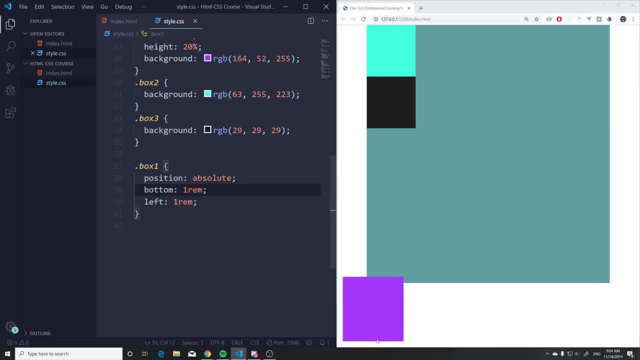 the left if I want to push it up a bit, the left, if I want to push it up a bit, I can do one rim from the bottom. so I can do one rim from the bottom, so I can do one rim from the bottom. so there we go. so it's very easy to. 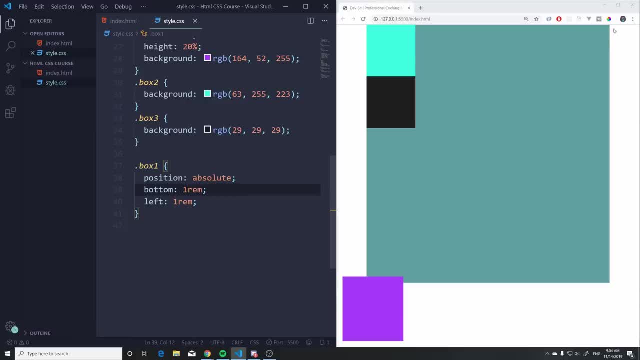 there we go, so it's very easy to there we go, so it's very easy to position this kind of the way you want, position this kind of the way you want, position this kind of the way you want. maybe I want it top and and a down here. 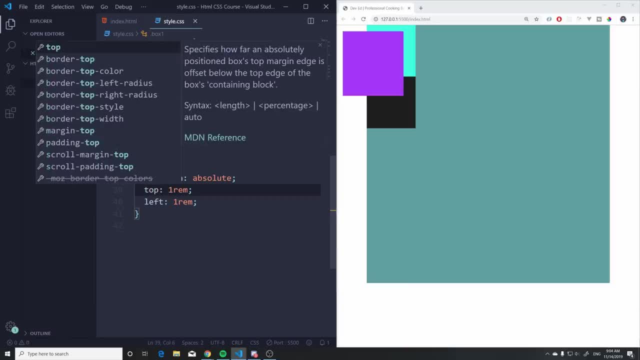 maybe I want it top and and a down here. maybe I want it top and and a down here so I can do top and right- it's safe, and so I can do top and right- it's safe, and so I can do top and right- it's safe. and now it's here, maybe I want to push it. 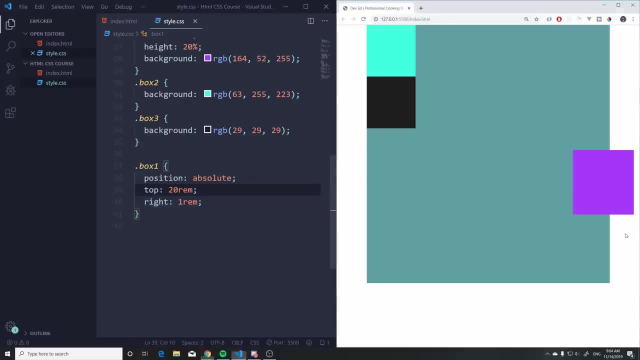 now it's here, maybe I want to push it. now it's here, maybe I want to push it down. it's 220, there we go, so I can move down. it's 220, there we go, so I can move down. it's 220, there we go, so I can move this anywhere I want. what, if I want to? 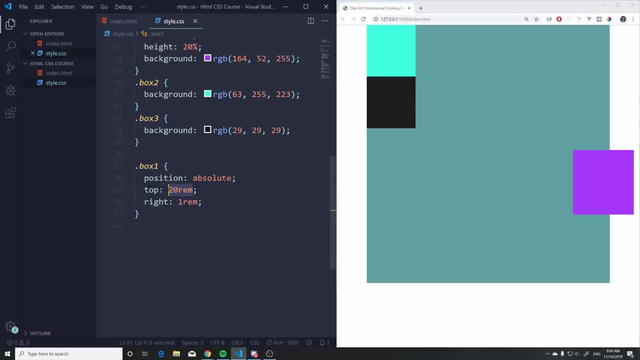 this anywhere. I want what if I want to this anywhere. I want what if I want to Center this here? well, we can also use Center this here. well, we can also use Center this here. well, we can also use percentages. now. something's weird is percentages now. something's weird is: 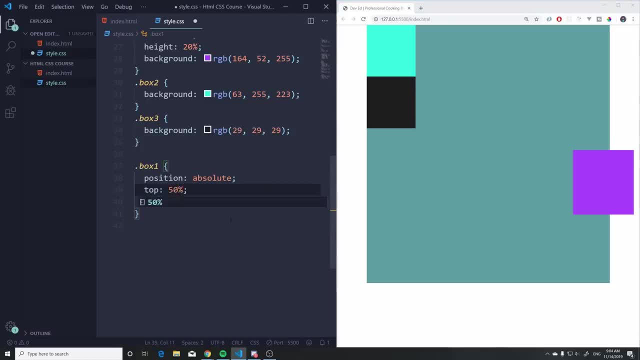 percentages. now something's weird is gonna happen. so I'm gonna add 50% and gonna happen. so I'm gonna add 50% and gonna happen. so I'm gonna add 50% and hit save and, as you can see, this doesn't hit save and, as you can see, this doesn't. 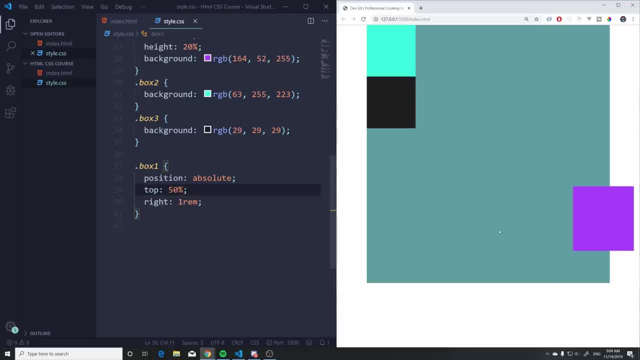 hit save and, as you can see, this doesn't look in the middle for some reason and look in the middle for some reason. and look in the middle for some reason and it actually is in the middle, but I want. it actually is in the middle, but I want. 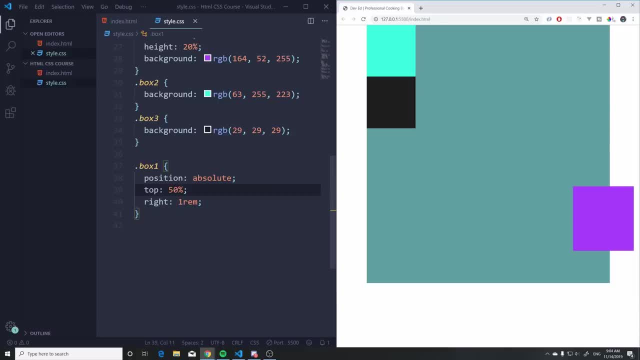 it actually is in the middle, but I want to explain this kind of how this works, to explain this kind of how this works. to explain this kind of how this works. so if we look from up here all the way, so if we look from up here all the way, 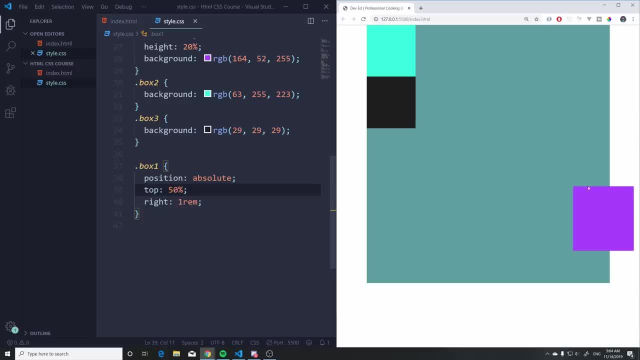 so, if we look from up here all the way down in the center here, what this is the down in the center here, what this is the down in the center here, what this is the center, this is where the element starts. center, this is where the element starts. 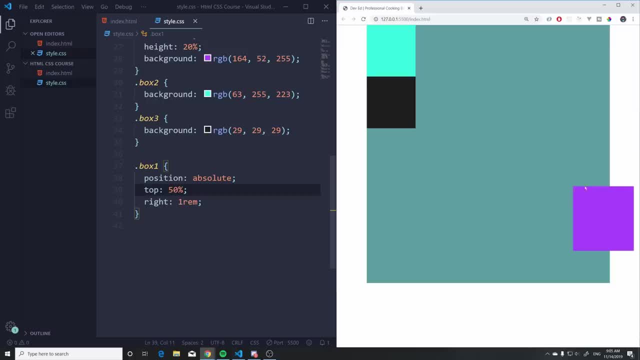 center. this is where the element starts, so this is where it puts it. but right, so this is where it puts it. but right, so this is where it puts it, but right now the content. so the box actually has now the content. so the box actually has now the content. so the box actually has some height to it and width to it, right. 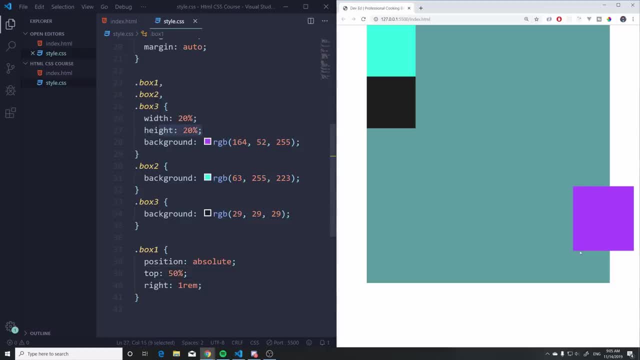 some height to it and width to it right, some height to it and width to it right, so 20%. so obviously it's gonna go a bit so 20%. so obviously it's gonna go a bit. so 20%. so obviously it's gonna go a bit down right and it doesn't look centered. 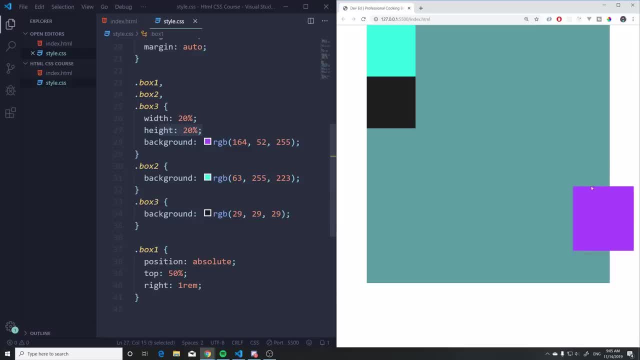 down right and it doesn't look centered down right and it doesn't look centered. so what we want to do, it would be really so what we want to do. it would be really so what we want to do. it would be really cool if we would have a property that. 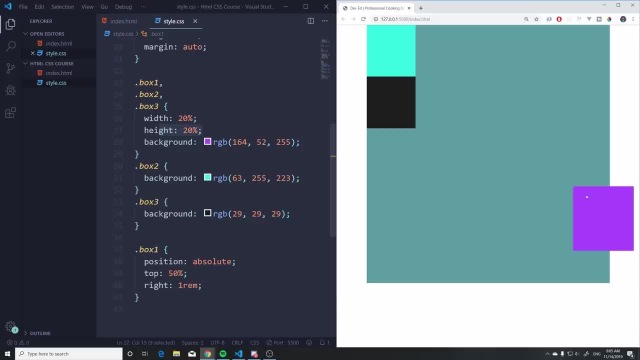 cool if we would have a property. that cool if we would have a property that would take just this element, just this would take just this element. just this would take just this element, just this purple thing: take this and just move it. purple thing, take this and just move it. 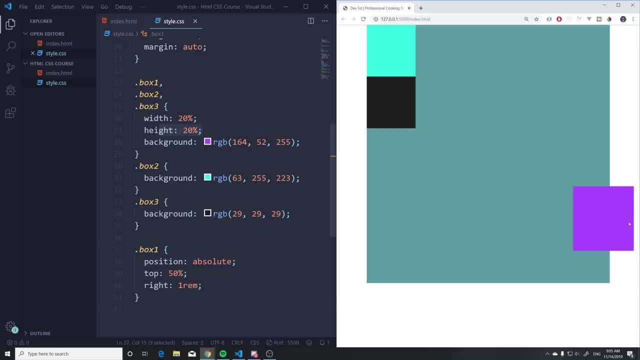 purple thing. take this and just move it up by half, so just the size of this, and up by half, so just the size of this, and up by half, so just the size of this, and take half of it and push it up and there. take half of it and push it up and there. 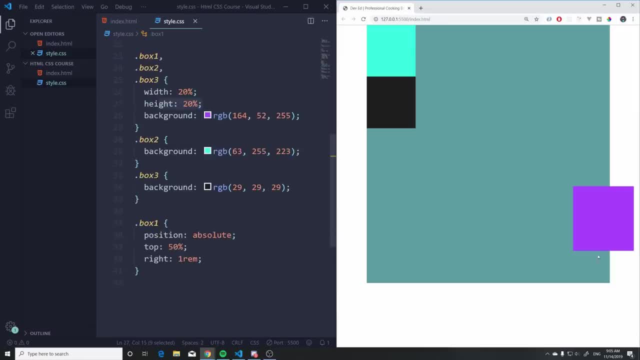 take half of it and push it up, and there is actually a property that can do. that is actually a property that can do. that is actually a property that can do that which is called translate transform, which is called translate transform, which is called translate transform, translate. okay, so let's do that, but 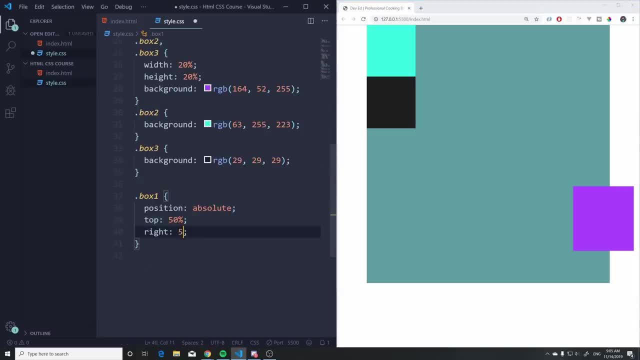 translate okay, so let's do that. but translate okay, so let's do that. but before we do that, let's move the right. before we do that, let's move the right. before we do that, let's move the right one to 50% as well, 50% as we can use. 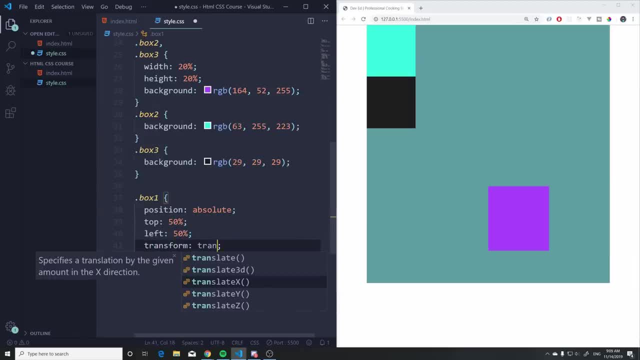 one to 50% as well 50% as we can use one to 50% as well 50% as we can use. something called transform translate, something called transform translate, something called transform translate. alright, and you can move the X and the. alright, and you can move the X and the. 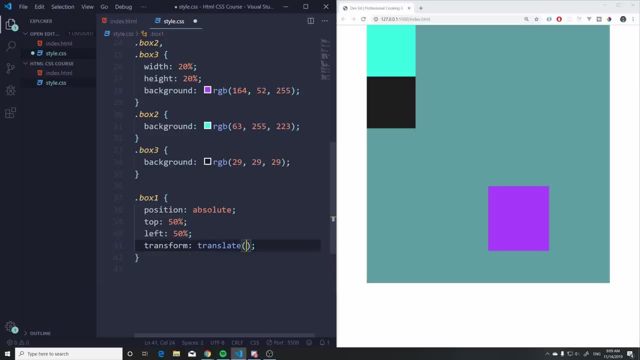 alright, and you can move the X and the Y, or optionally you can do translate like Y, or optionally you can do translate like Y, or optionally you can do translate like this and you can add two values with this. and you can add two values with this and you can add two values with translate X. you would add one value here. 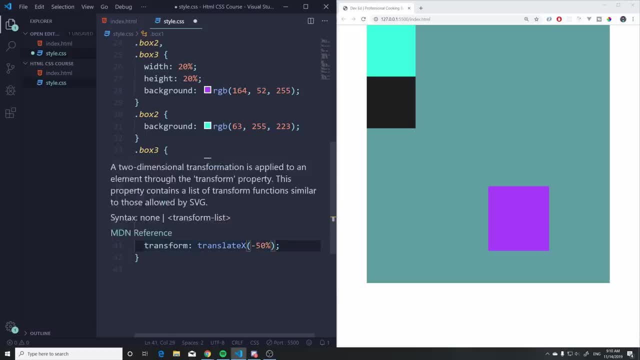 translate X, you would add one value here. translate X, you would add one value here. so like minus 50% and with no value. so like minus 50% and with no value. so like minus 50% and with no value. here you can add to X and the Y, so we: 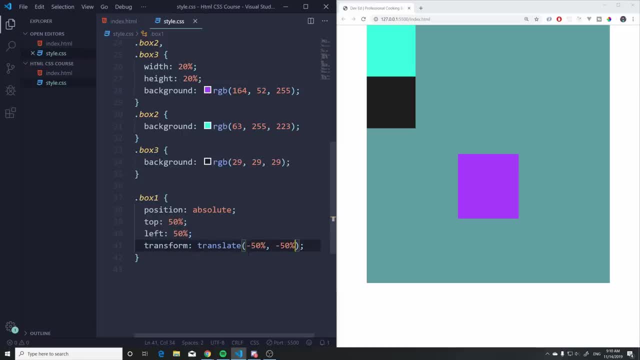 here you can add to X and the Y, so we, here you can add to X and the Y, so we can say X and Y minus 50 minus 50, and as can say X and Y minus 50 minus 50, and as can say X and Y minus 50 minus 50, and, as you can see, that's gonna move it. 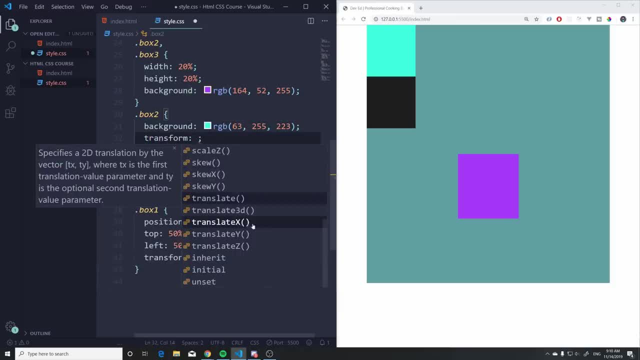 you can see that's gonna move it if I add to the box to a transform and if I add to the box to a transform and if I add to the box to a transform. and let's just translate X if I move this by. let's just translate X if I move this by. 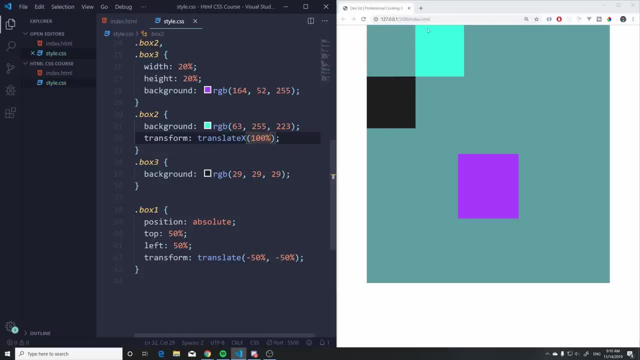 let's just translate X. if I move this by a hundred percent, then it's gonna a hundred percent, then it's gonna a hundred percent, then it's gonna perfectly move it the size of the box to perfectly move it the size of the box to perfectly move it. the size of the box to the right. okay, if I want to do the. 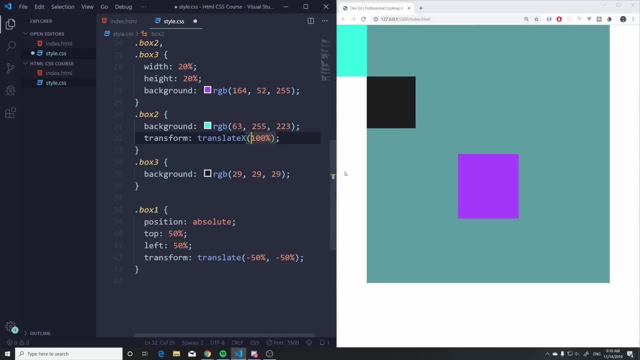 the right. okay. if I want to do the, the right okay. if I want to do the opposite way, I can say minus, and there opposite way, I can say minus, and there opposite way, I can say minus. and there we go also. what we did here was just do. 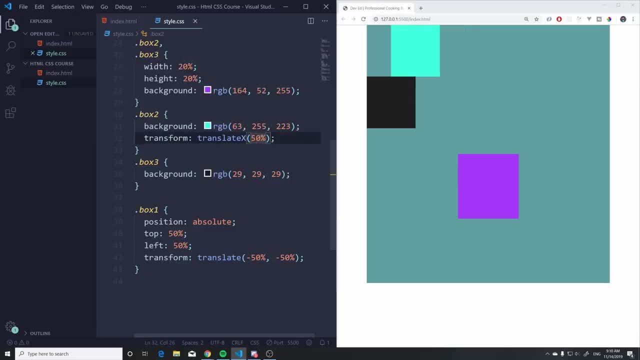 we go also. what we did here was: just do we go also. what we did here was just do 50%, because I wanted the element to be 50%, because I wanted the element to be 50%, because I wanted the element to be centered, so like this, as you can see, 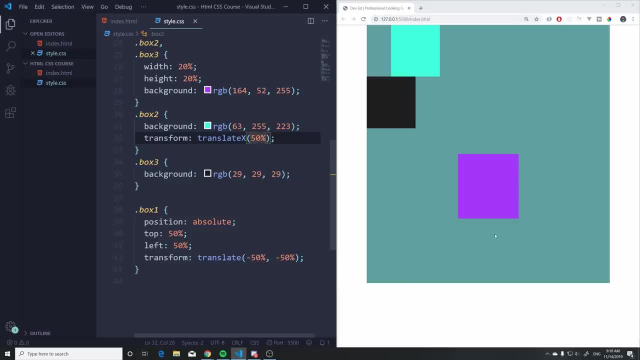 centered. so like this, as you can see, centered. so like this, as you can see: perfectly moved 50% to the left and perfectly moved 50% to the left and perfectly moved 50% to the left and upwards. so it's centered. okay, let's get. 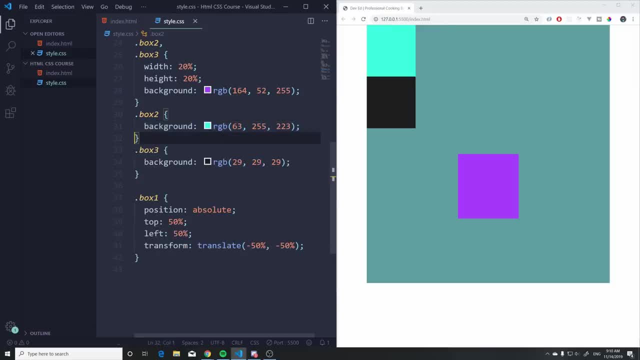 upwards, so it's centered. okay, let's get upwards, so it's centered. okay, let's get rid of this, and I want to show you rid of this, and I want to show you rid of this, and I want to show you something else. so this is how you can. 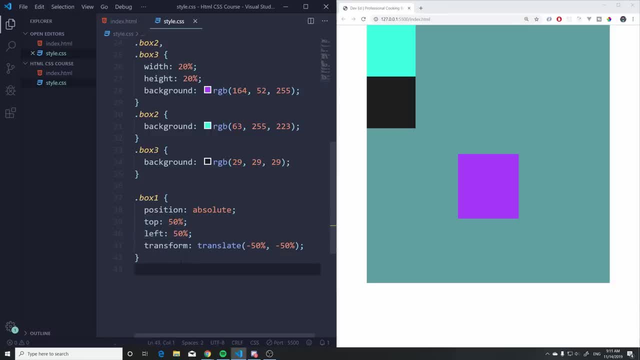 something else. so this is how you can something else. so this is how you can position it perfectly in the middle. you position it perfectly in the middle. you position it perfectly in the middle. you add top 50 left 50 and the transform. add top 50 left 50 and the transform. 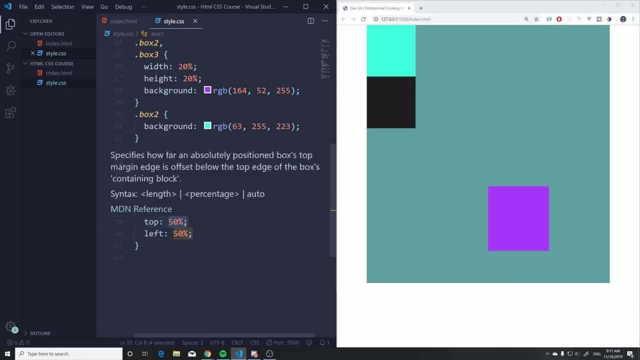 add top 50, left 50 and the transform. get rid of this. let's just move this top. get rid of this. let's just move this top. get rid of this. let's just move this top to 0%. there we go, and let's move it to. 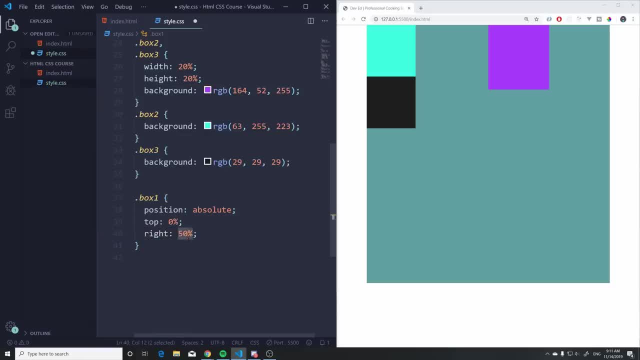 to 0%. there we go, and let's move it to to 0%. there we go and let's move it to the right 0%. what if I want this to be the right 0%? what if I want this to be the right 0%? what if I want this to be relative to the box? okay, I don't want. 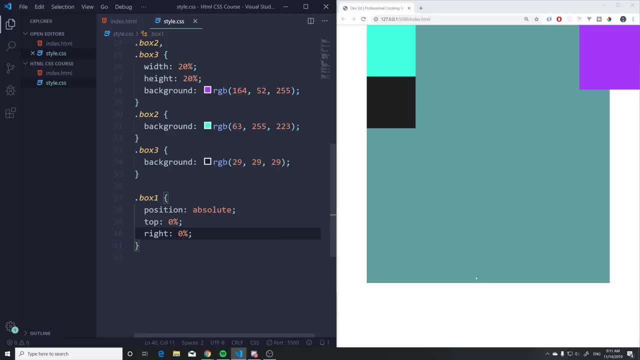 relative to the box. okay, I don't want relative to the box. okay, I don't want this to be out here. I want it to stick this to be out here. I want it to stick this to be out here. I want it to stick basically, to this box. so to do that all. 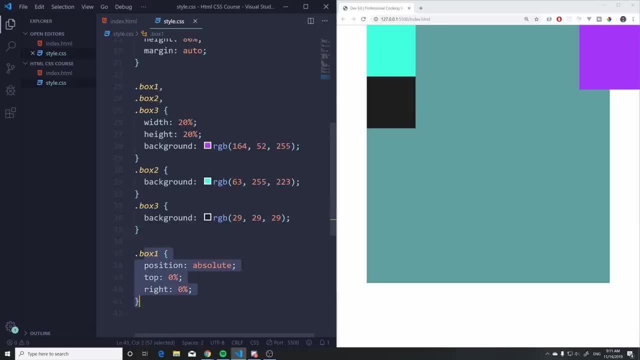 basically to this box. so to do that, all basically to this box. so to do that, all you have to do is, if you have a box one, you have to do is: if you have a box one, you have to do is, if you have a box one here, if you add position relative to the 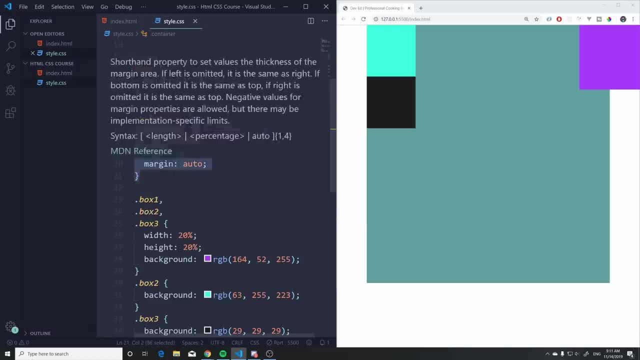 here, if you add position relative to the here, if you add position relative to the parent element or any parent you want to parent element or any parent you want to parent element or any parent you want to add, this is gonna basically detect the add. this is gonna basically detect the. 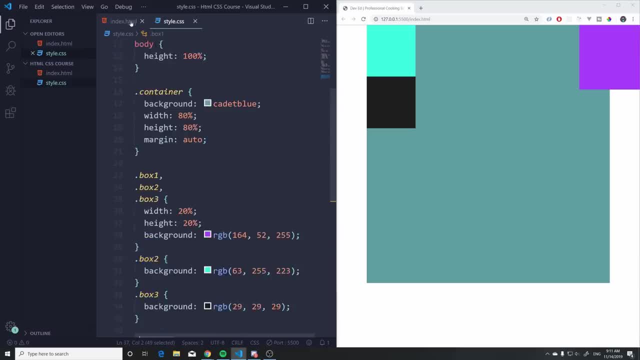 add. this is gonna basically detect the first position relative. you're gonna add first position relative. you're gonna add first position relative. you're gonna add to a parent, so it can be either this one to a parent, so it can be either this one to a parent, so it can be either this one or this one. it's gonna detect it. the. 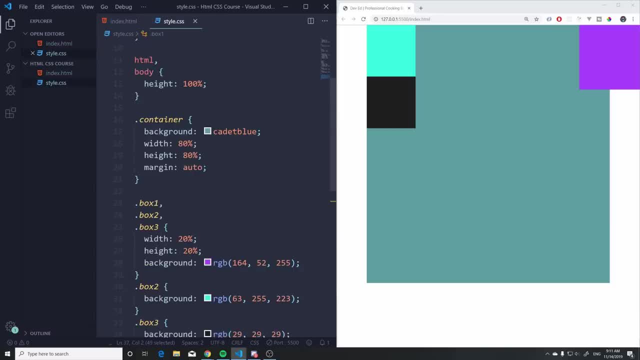 or this one, it's gonna detect it, the. or this one, it's gonna detect it the first time it hits position relative on first time it hits position relative on first time it hits position relative on an element. that's what it's. it is gonna an element. that's what it's, it is gonna. 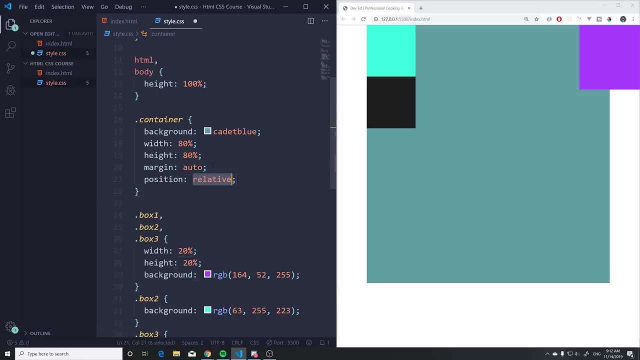 an element. that's what it's. it is gonna stick to. so if I go here and add a stick to so, if I go here and add a stick to so, if I go here and add a position relative and hit save as you can, position relative and hit save as you can. 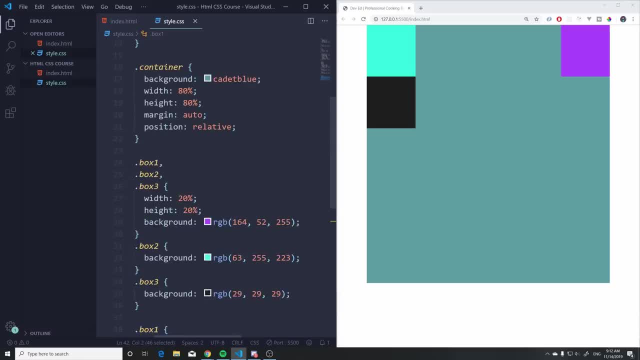 position relative and hit save. as you can see, now it constrains itself to the see. now it constrains itself to the see. now it constrains itself to the thing that we added relative. so you can thing that we added relative. so you can thing that we added relative. so you can imagine it as: okay, I have position. 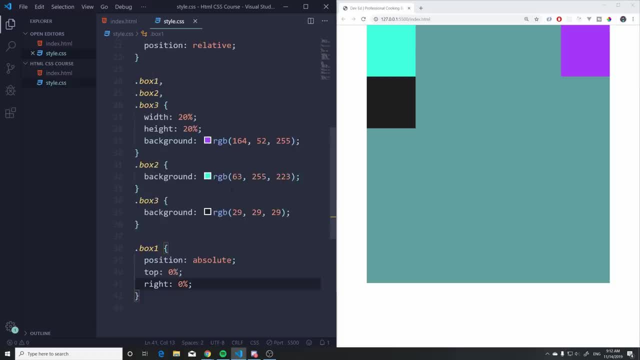 imagine it as okay, I have position. imagine it as okay, I have position, absolute. but what am i relative to my absolute? but what am I relative to my absolute? but what am I relative to my relative to to this, and if it is, then relative to to this, and if it is then? 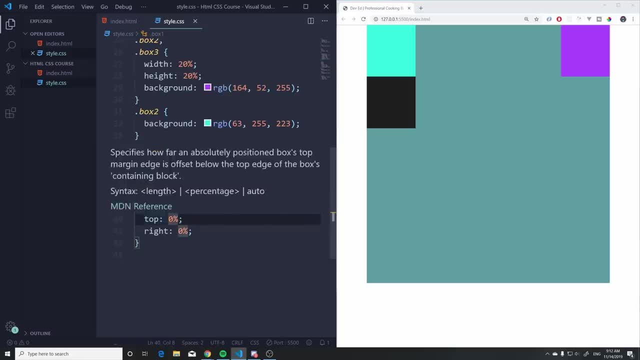 relative to to this, and if it is, then you just add position relative. so now, if you just add position relative, so now, if you just add position relative, so now, if I change this to top 0, as you can see, I change this to top 0, as you can see. 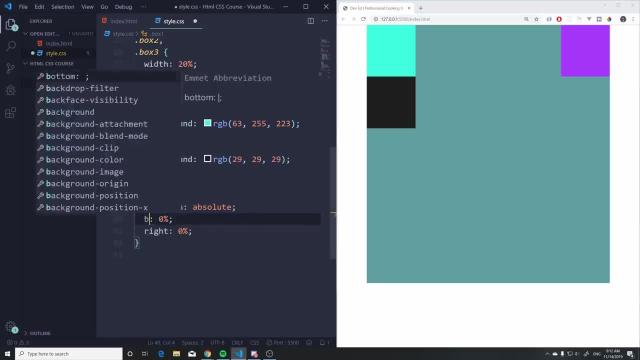 I change this to top 0, as you can see. it's there. I can modify this to bottom. it's there. I can modify this to bottom. it's there. I can modify this to bottom 0 and you're gonna see that it's gonna be 0 and you're gonna see that it's gonna be. 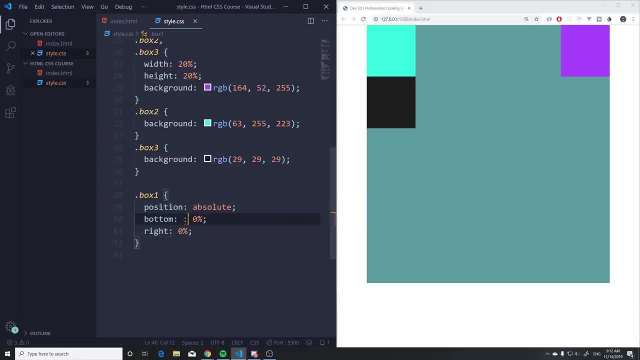 0, and you're gonna see that it's gonna be stuck there, perfectly fine. so now stuck there, perfectly fine. so now stuck there, perfectly fine. so now everything works the same way. it's just everything works the same way. it's just everything works the same way. it's just that everything is stuck in here, okay. 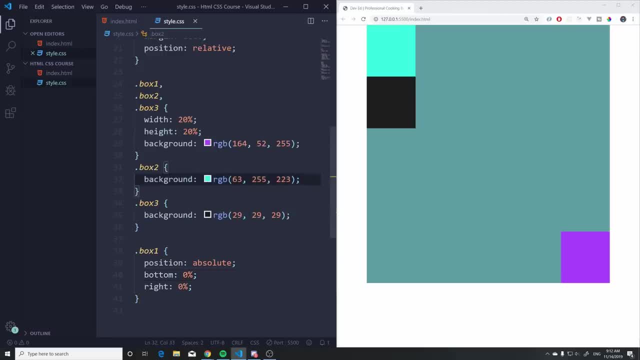 that everything is stuck in here. okay, that everything is stuck in here, okay. now what position relative also does is now what position relative also does. is now what position relative also does is if we go to box 2 here and add a, if we go to box 2 here and add a. 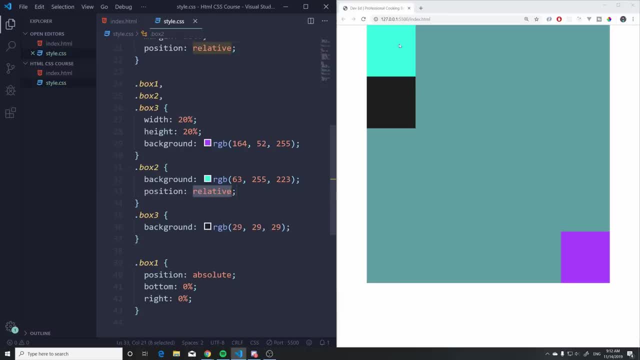 if we go to box 2 here and add a position relative: all right now, this is position relative. all right now. this is position relative. all right now. this is not gonna jump in there, because it's not not gonna jump in there, because it's not not gonna jump in there because it's not its parent, right, it's just gonna look. 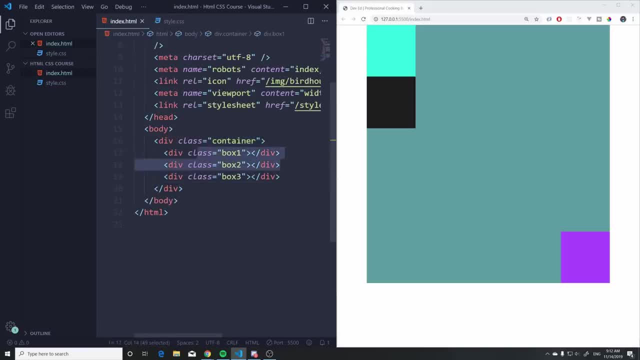 its parent, right, it's just gonna look its parent, right, it's just gonna look at parents. these are kind of siblings in at parents. these are kind of siblings in at parents. these are kind of siblings in here. so it's just gonna look up there here, so it's just gonna look up there. 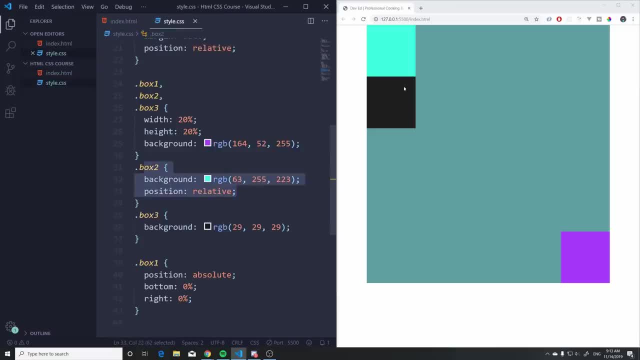 here. so it's just gonna look up there. when you add the position absolute, but when you add the position absolute, but when you add the position absolute, but if you just add position relative to an, if you just add position relative to an, if you just add position relative to an element, all it's gonna mean is that if 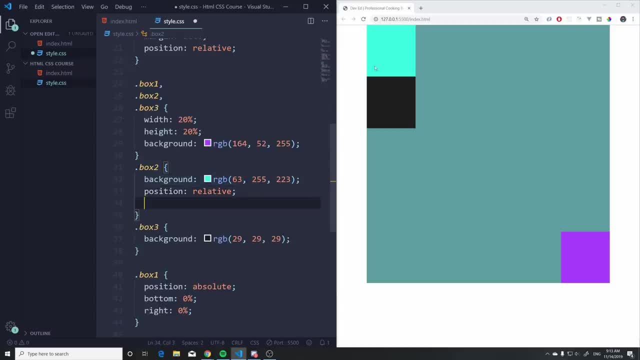 element. all it's gonna mean is that, if element. all it's gonna mean is that if we move this with top left, right and we move this with top left right and we move this with top, left, right and bottom, it's gonna move away from this bottom, it's gonna move away from this. 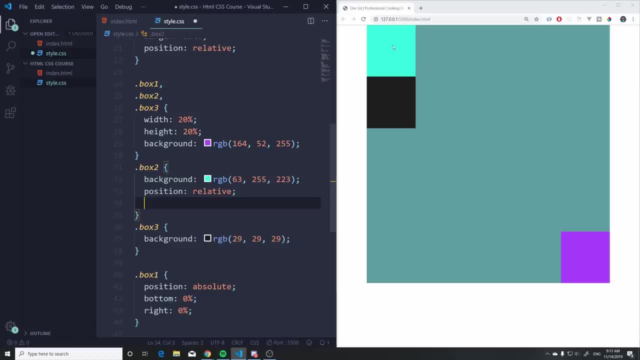 bottom. it's gonna move away from this exact position. so it's gonna keep count exact position. so it's gonna keep count exact position. so it's gonna keep count of where its initial position is and of where its initial position is and of where its initial position is. and then, if we just add something like left: 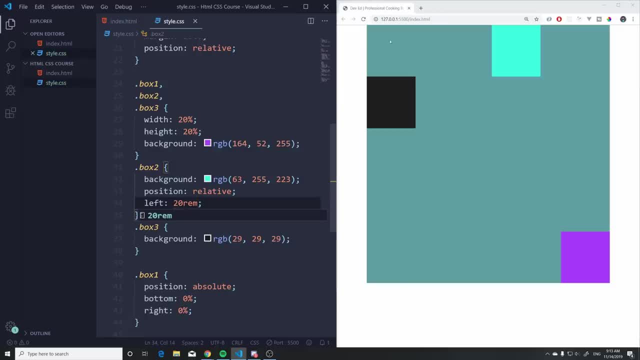 then if we just add something like left, then if we just add something like left- 20 REM, all right, it's gonna move 20 REM, 20 REM. all right, it's gonna move 20 REM, 20 REM. all right, it's gonna move 20 REM from its original position. okay, so let. 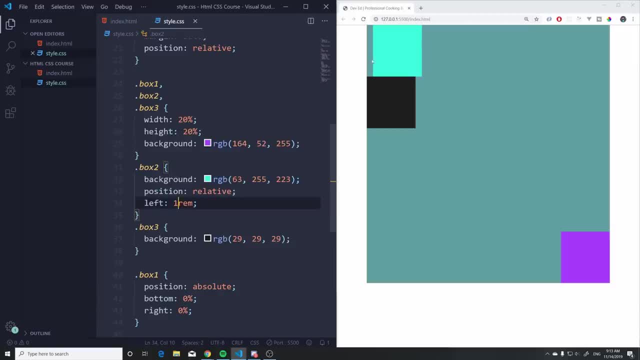 from its original position. okay, so let from its original position. okay, so let me show you one room, so it's gonna move me. show you one room, so it's gonna move me. show you one room, so it's gonna move left one REM from its original position. 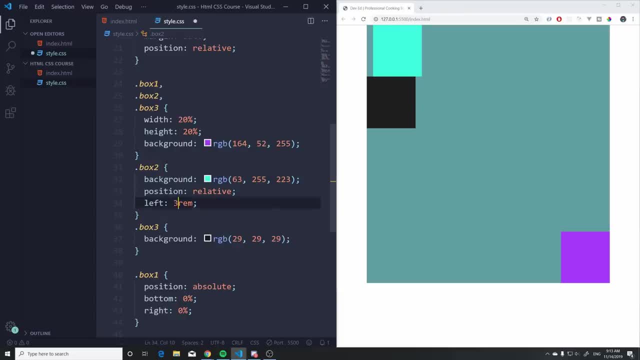 left one REM from its original position. left one REM from its original position. okay, so that it that's very simple. okay, so that it that's very simple. okay, so that it that's very simple. actually, a relative just moves from its. actually, a relative just moves from its. 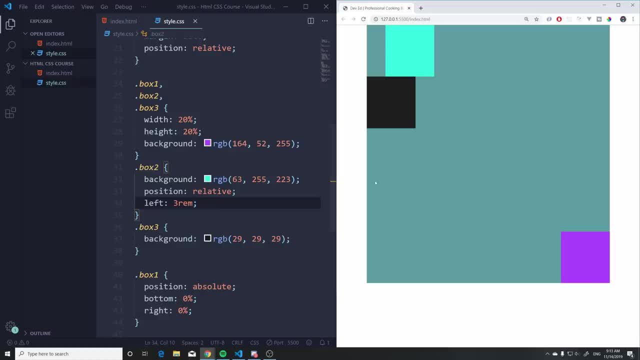 actually a relative just moves from its original position okay, and the next one original position okay, and the next one original position okay. and the next one I want to show you is position static. I want to show you is position static. I want to show you is position static. let's go to the dark box. here we're. 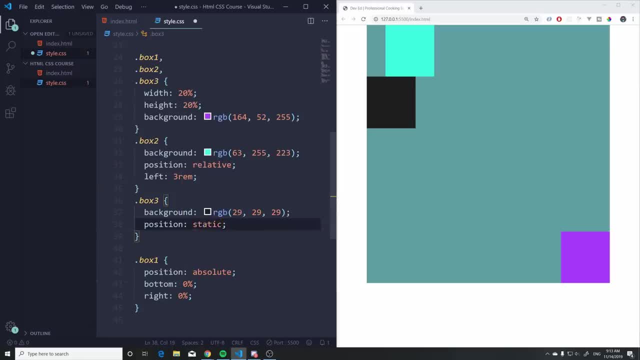 let's go to the dark box here we're. let's go to the dark box here we're gonna add position static. yeah, my gonna add position static. yeah, my gonna add position static. yeah, my apologies. position fixed because static, apologies. position fixed because static. apologies. position fixed because static is the one that has. and what happens? 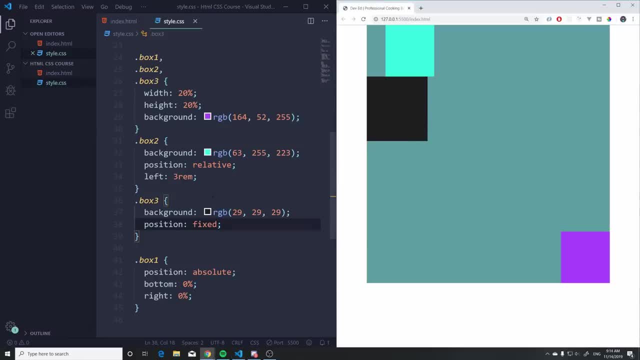 is the one that has, and what happens is the one that has. and what happens right now is: we cannot really see right now, is we cannot really see right now is we cannot really see anything. but if I go up here and I just anything, but if I go up here and I just 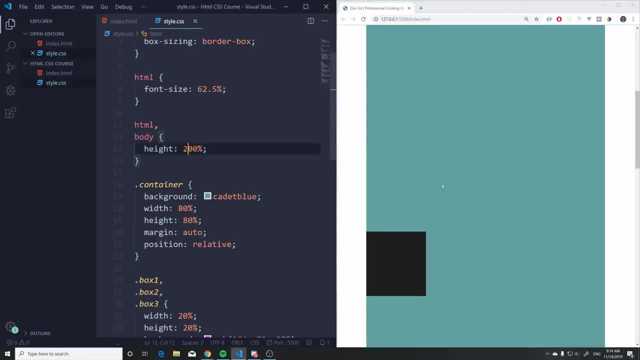 anything. but if I go up here and I just change the body and the height to like, change the body and the height to like, change the body and the height to like 200, just so we can scroll a bit as you. 200, just so we can scroll a bit as you. 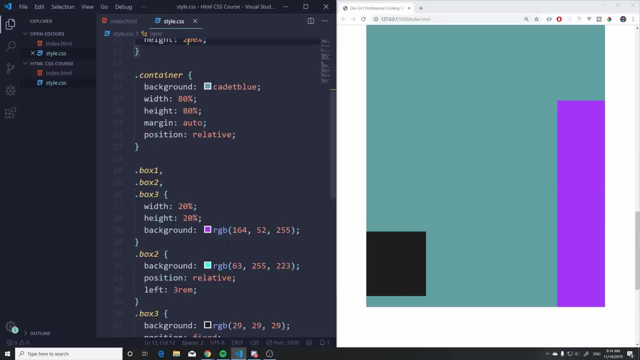 200, just so we can scroll a bit as you can see. what happens is that this element can see what happens, is that this element can see what happens is that this element stays fixed, all right, and I can scroll. stays fixed, all right and I can scroll. 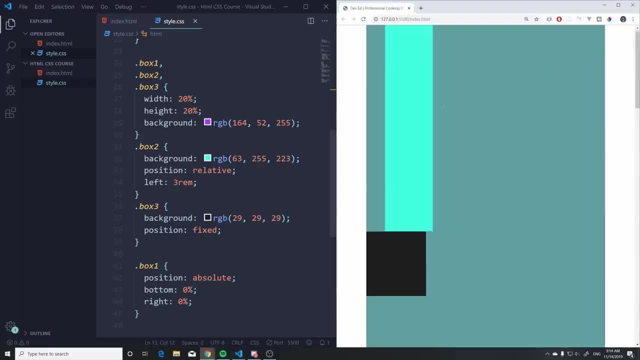 stays fixed, all right, and I can scroll as much as I want and I can position it as much as I want. and I can position it as much as I want, and I can position it wherever I want, it's always gonna be. wherever I want, it's always gonna be. 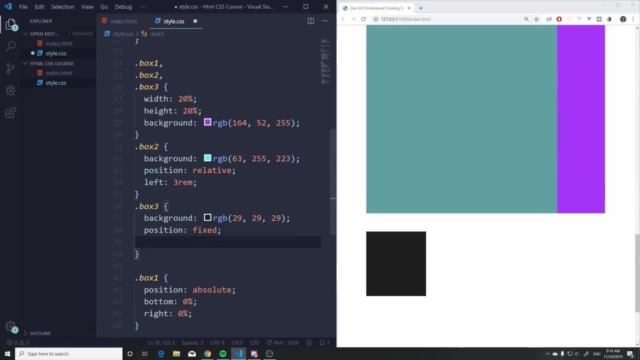 wherever I want, it's always gonna be fixed there. now I can modify its. fixed there. now I can modify its fixed there. now I can modify its position. it's fixed position, so I can position it's fixed position. so I can position it's fixed position so I can say: pop, let's do two REM and see what. 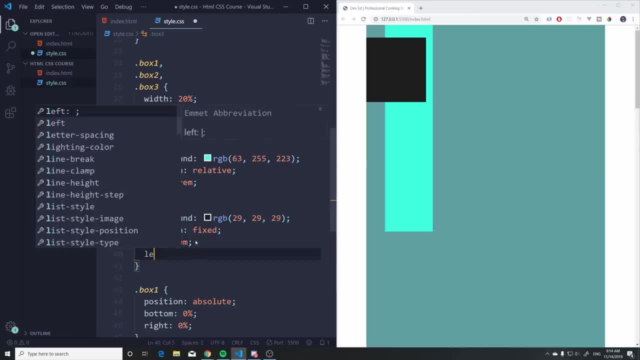 say pop, let's do two REM and see what say pop. let's do two REM and see what happens there. so it's here. maybe I want happens there, so it's here. maybe I want happens there, so it's here. maybe I want to move it left 10 REM and again I can. 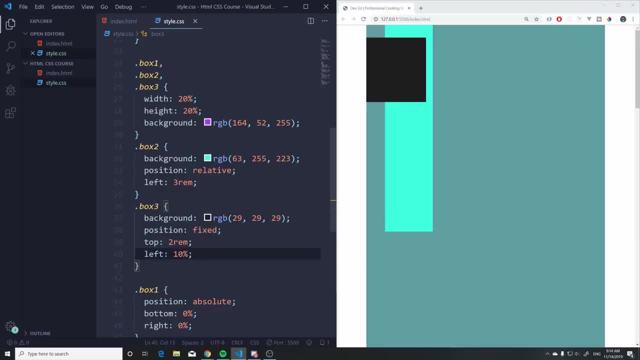 to move it left: 10 REM, and again I can. to move it left: 10 REM, and again I can. add percentages very just like the other. add percentages very just like the other. add percentages very just like the other ones. let's do, let's do five REM more 10. 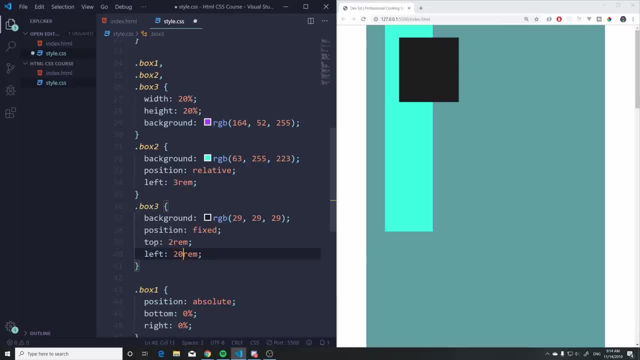 ones, let's do. let's do five REM more 10 ones, let's do. let's do five REM more 10 REM. you want, Oh, even more. this is not REM. you want, Oh, even more. this is not REM. you want, Oh, even more. this is not enough. 20 REM, okay, so I can position it. 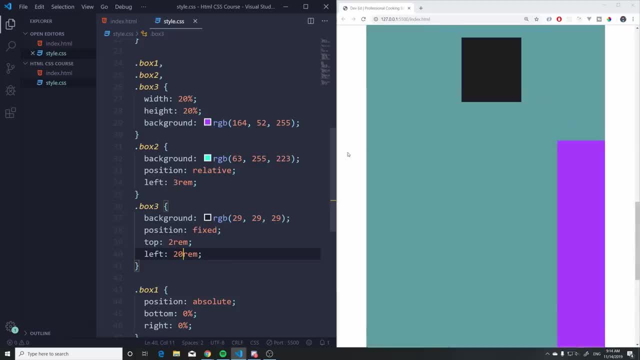 enough 20 REM okay, so I can position it. enough 20 REM okay, so I can position it there, okay. and even if I go outside it there okay. and even if I go outside it there okay. and even if I go outside, it doesn't matter where I go, it's always. 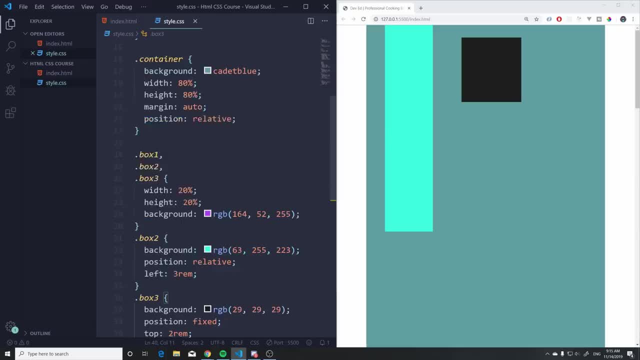 doesn't matter where I go. it's always doesn't matter where I go. it's always gonna be fixed. okay, so that is fixed. you gonna be fixed. okay, so that is fixed. you gonna be fixed. okay, so that is fixed. you might be using this, if you have maybe. 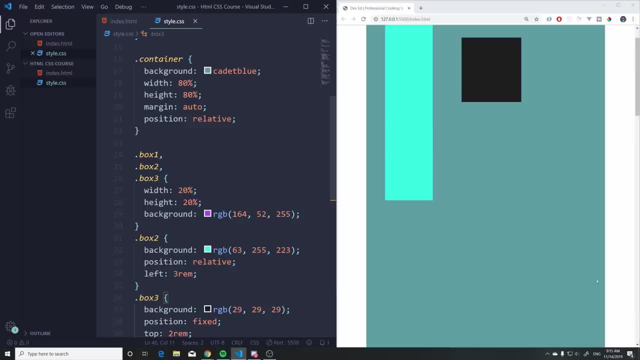 might be using this if you have. maybe might be using this if you have maybe some kind of chat or something, or maybe some kind of chat or something, or maybe some kind of chat or something, or maybe a footer or a nav that's always stuck up- a footer or a nav that's always stuck up. 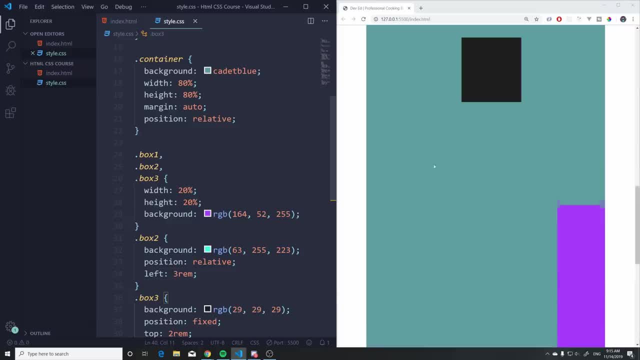 a footer or a nav that's always stuck up there and that's where you can use this there, and that's where you can use this there and that's where you can use this. so maybe you have your content, but you. so maybe you have your content, but you. 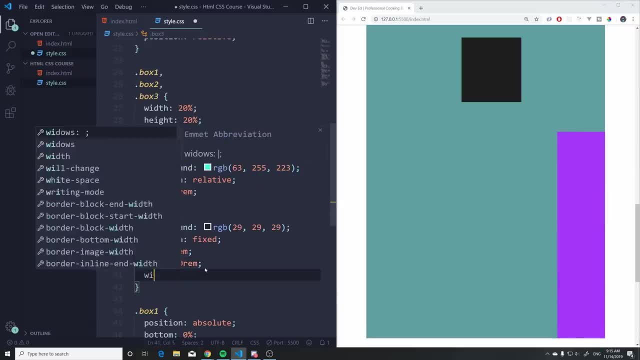 so maybe you have your content but you have a nav, so we can even add height and have a nav. so we can even add height and have a nav. so we can even add height and width to this, so I can stretch this out. width to this, so I can stretch this out. 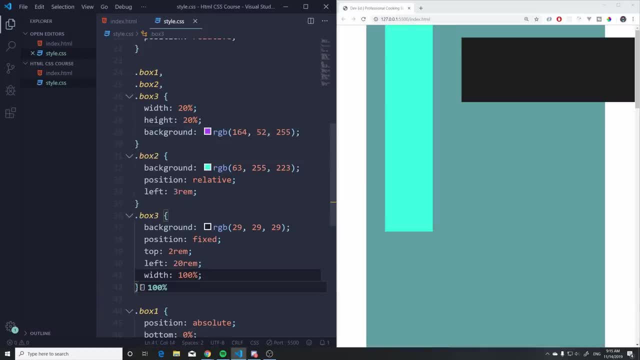 width to this, so I can stretch this out with 100%. if I want hit, save, all right with 100%. if I want hit, save, all right with 100%. if I want hit, save, all right. and then let's move left to 0. so I'm 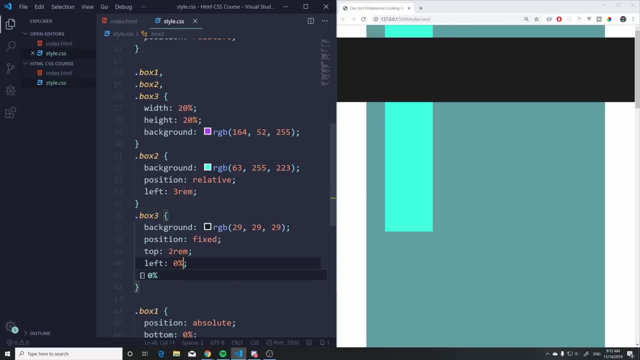 and then let's move left to 0, so I'm. and then let's move left to 0, so I'm gonna say 0%, like that, and top it's gonna say 0%, like that, and top it's gonna say 0%, like that, and top it's gonna be 0% and close this up and there. 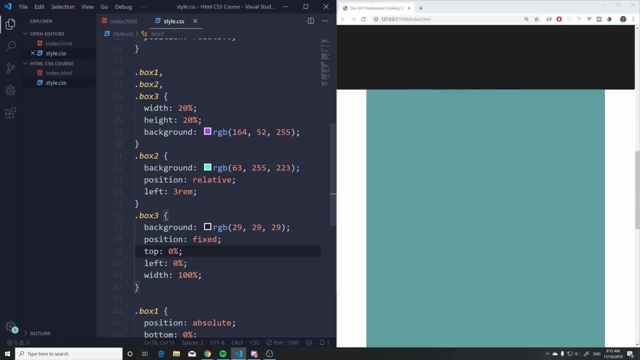 gonna be 0% and close this up, and there gonna be 0% and close this up, and there we go. you can imagine this as being your we go. you can imagine this as being your we go. you can imagine this as being your navigation, and it's always there, well, it. 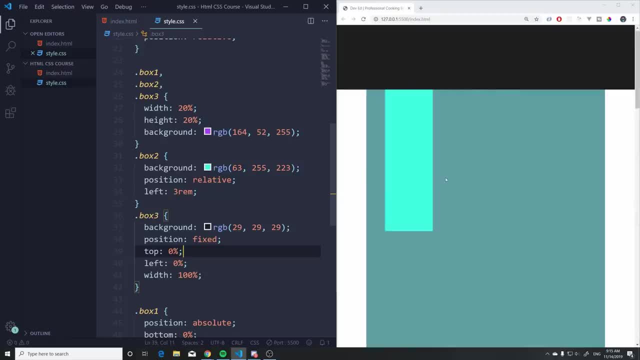 navigation, and it's always there. well, it navigation, and it's always there. well, it wouldn't be so thick, but you get the wouldn't be so thick, but you get the wouldn't be so thick, but you get the general idea. okay, so that's the one now. 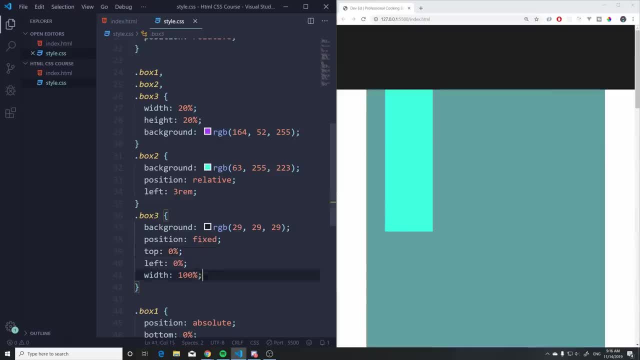 general idea: okay, so that's the one now. general idea, okay, so that's the one. now there's another one I want to show you. there's another one I want to show you. there's another one I want to show you, which is called positions sticky. so 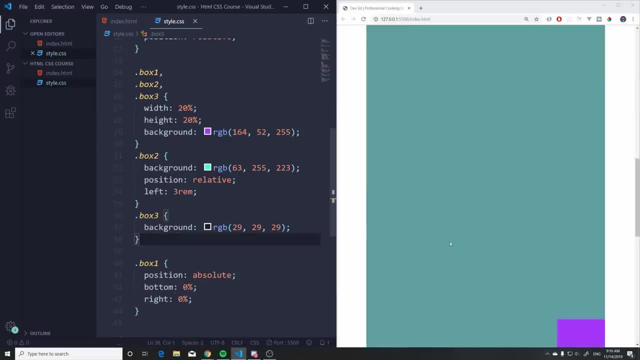 which is called positions sticky. so which is called positions sticky. so let's remove everything from here, and we let's remove everything from here, and we let's remove everything from here, and we are back to this now. let's change back. are back to this now. let's change back. 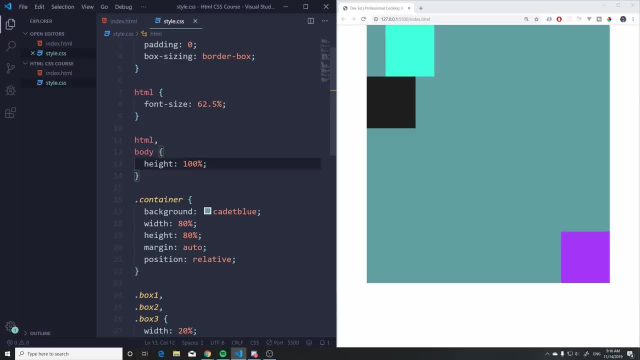 are back to this. now let's change back the size to 100. all right, actually, I the size to 100. all right, actually, I the size to 100. all right, actually, I need a bit more height here. so I'm gonna need a bit more height here. so I'm gonna. 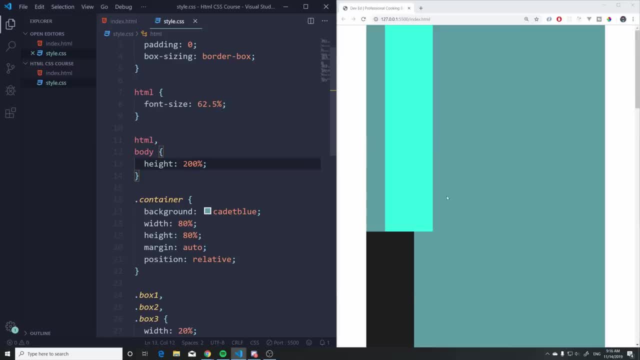 need a bit more height here. so I'm gonna add 200, even though these are kind of add 200, even though these are kind of add 200, even though these are kind of stretched. we can kind of fix this if we stretched. we can kind of fix this if we. 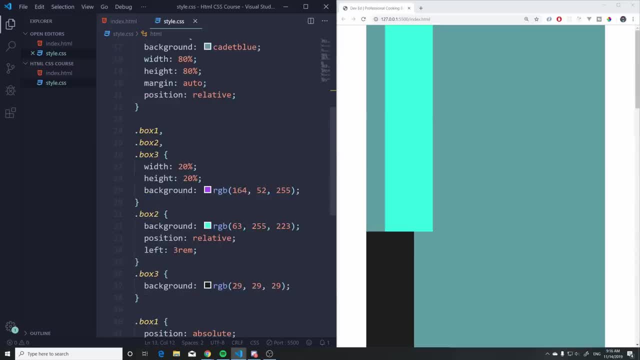 stretched. we can kind of fix this if we want. if we go to the boxes and change want. if we go to the boxes and change want. if we go to the boxes and change the height to 10, okay, just make them a. the height to 10, okay, just make them a. 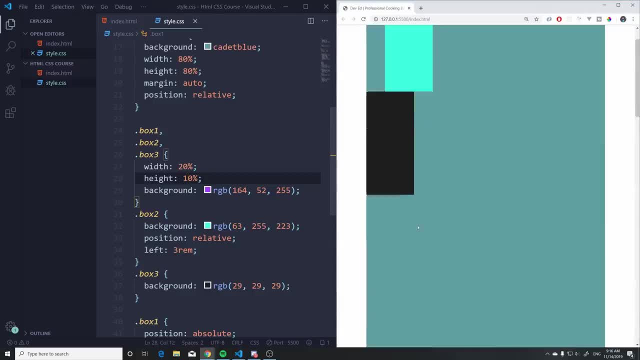 the height to 10. okay, just make them a bit shorter, but I want to have some bit shorter, but I want to have some bit shorter. but I want to have some scrollable space here. so if I go to the scrollable space here, so if I go to the 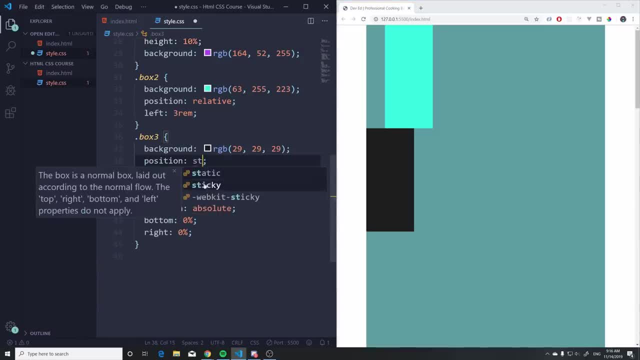 scrollable space here. so if I go to the box 3 and add a position sticky, hit box 3 and add a position sticky, hit box 3 and add a position sticky, hit save. nothing's gonna happen. but as soon save, nothing's gonna happen, but as soon. 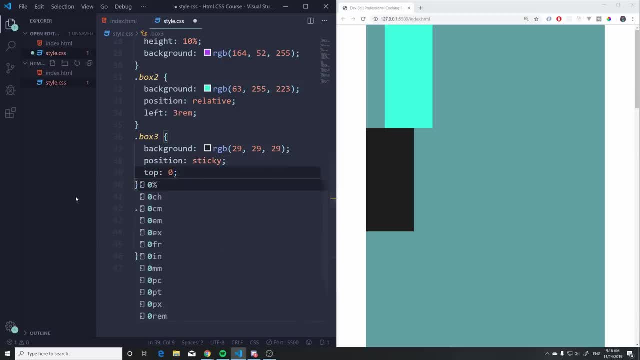 save, nothing's gonna happen. but as soon as I add top 0% and hit save, as soon as as I add top 0% and hit save, as soon as as I add top 0% and hit save as soon as I start scrolling, as you can see that. 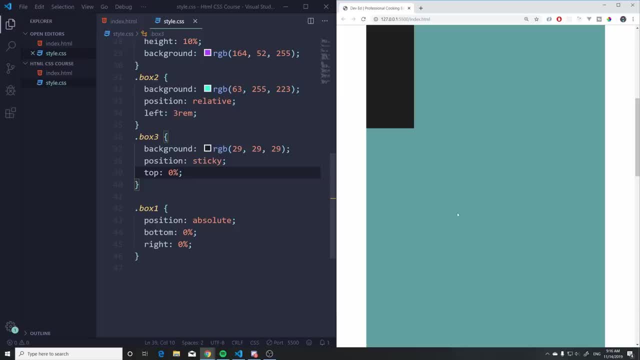 I start scrolling, as you can see that I start scrolling, as you can see that black thing sticks there. but as soon as black thing sticks there, but as soon as black thing sticks there, but as soon as I move up it it kind of stops, so it gets. 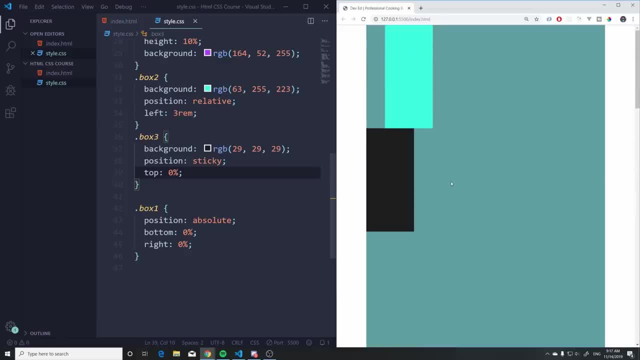 I move up it, it kind of stops, so it gets. I move up it, it kind of stops, so it gets sticky. and as soon as I move up, it's sticky. and as soon as I move up, it's sticky. and as soon as I move up, it's back to normal. so what this does it? 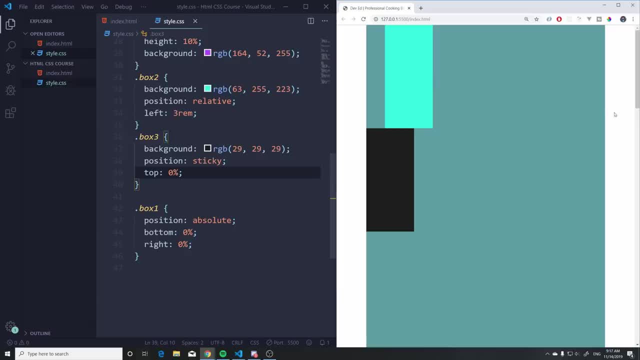 back to normal. so what this does? it back to normal. so what this does? it switches from position relative to switches from position relative to switches, from position relative to position fixed. so when we scroll down position fixed, so when we scroll down position fixed, so when we scroll down and it hits that top zero, so as soon as 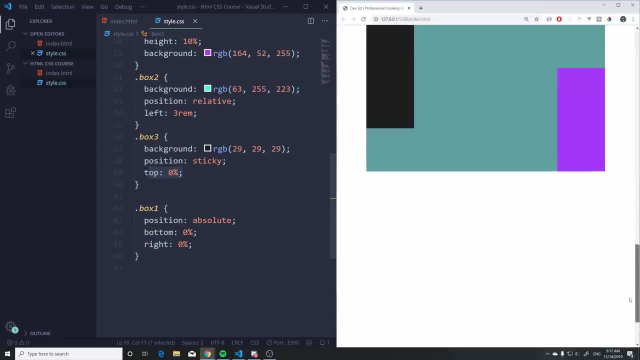 and it hits that top zero. so as soon as- and it hits that top zero, so as soon as it hits that top zero, it's gonna stick. it hits that top zero, it's gonna stick. it hits that top zero, it's gonna stick there. all right, you can come up with. 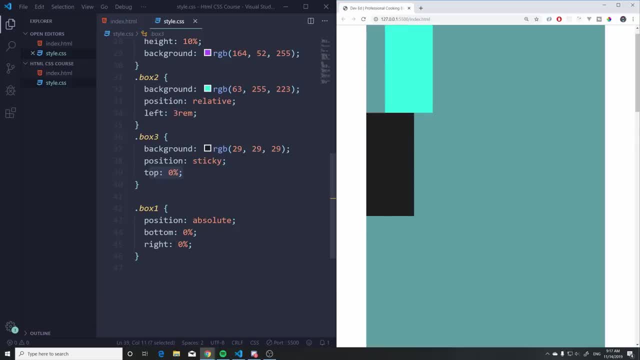 there. all right, you can come up with there. all right, you can come up with some cool things here as well with this, some cool things here as well with this, some cool things here as well with this. and you can do the same thing with, and you can do the same thing with. 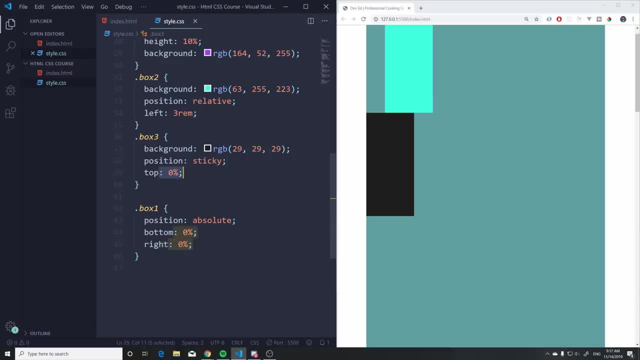 and you can do the same thing with whenever it hits the bottom or or the. whenever it hits the bottom or or the. whenever it hits the bottom or or the right or the left. okay, so this works on right or the left. okay so this works on right or the left. okay so, this works on all of those properties. so these are the. 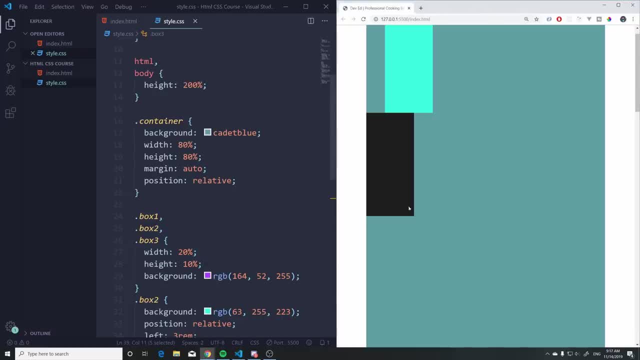 all of those properties. so these are the all of those properties. so these are the positions now. we're not going to be positions now. we're not going to be positions now. we're not going to be using this to exclusively align, using this to exclusively align, using this to exclusively align, sometimes for very specific purposes. 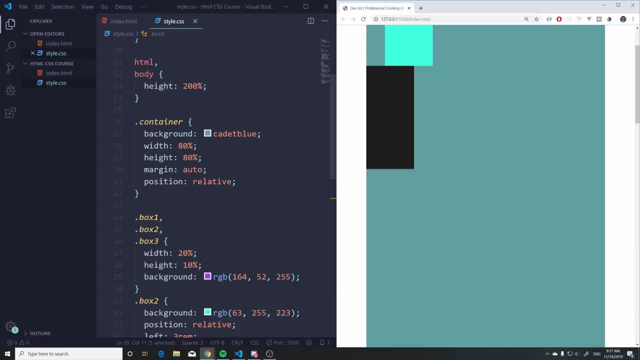 sometimes for very specific purposes, sometimes for very specific purposes. then we're gonna cover when we are gonna. then we're gonna cover when we are gonna. then we're gonna cover when we are gonna get into building out the project that's get into building out the project that's. 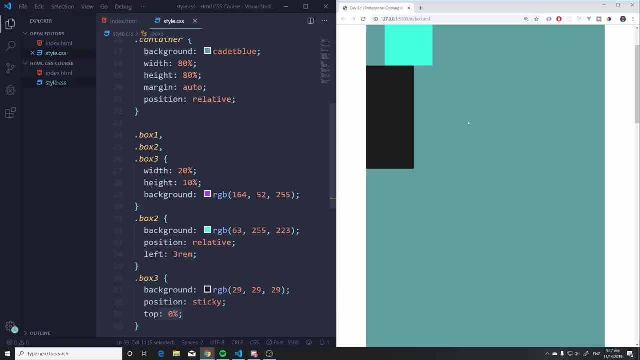 get into building out the project. that's where you're gonna see exactly when and where you're gonna see exactly when and where you're gonna see exactly when and how we're gonna use these. but these are how we're gonna use these. but these are how we're gonna use these. but these are very helpful and they're gonna help us a. 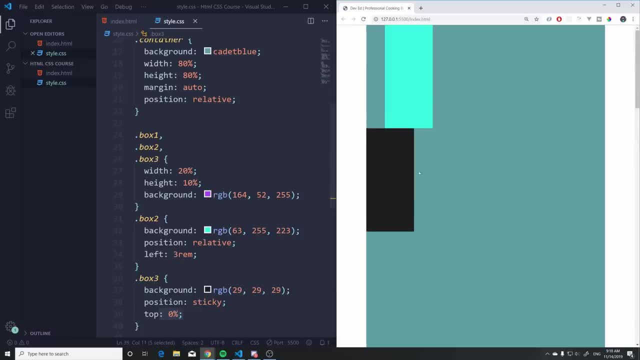 very helpful and they're gonna help us a very helpful and they're gonna help us a ton. so now let's get into aligning and ton. so now let's get into aligning and ton. so now let's get into aligning and floats. and that was a super old way of. 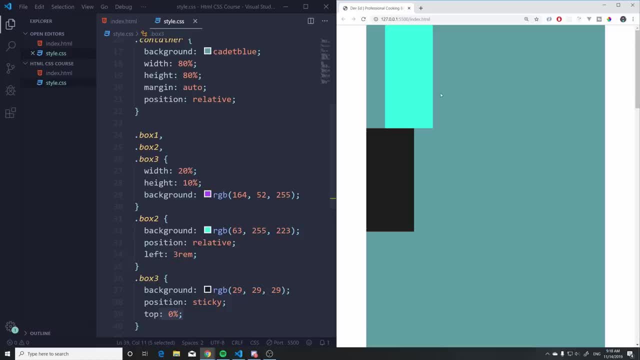 floats and that was a super old way of floats and that was a super old way of aligning content and positioning content. aligning content and positioning content, aligning content and positioning content. that we're not gonna use, but I'm gonna. that we're not gonna use, but I'm gonna. 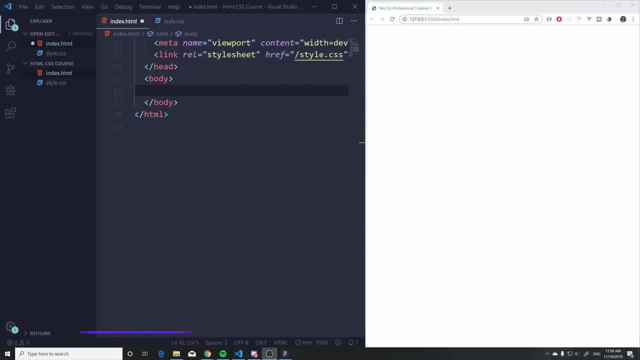 that we're not gonna use, but I'm gonna show it to you just for fun. okay, after show it to you just for fun. okay, after show it to you just for fun. okay, after this episode, we are finally gonna build this episode. we are finally gonna build. 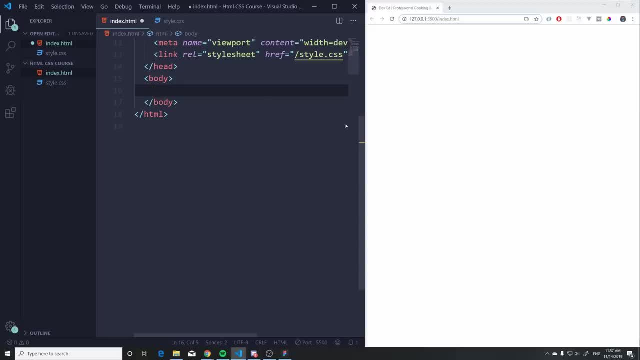 this episode, we are finally gonna build something out. is it gonna be good? no, something out. is it gonna be good? no, something out. is it gonna be good? no, it's not gonna be good because we're it's not gonna be good, because we're it's not gonna be good because we're gonna use a super old method of aligning. 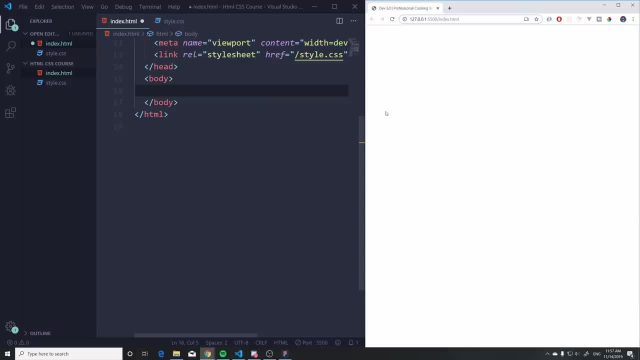 gonna use a super old method of aligning. gonna use a super old method of aligning and positioning our elements so, and positioning our elements so and positioning our elements so basically creating our structure for our, basically creating our structure for our, basically creating our structure for our website. we're gonna be using something. 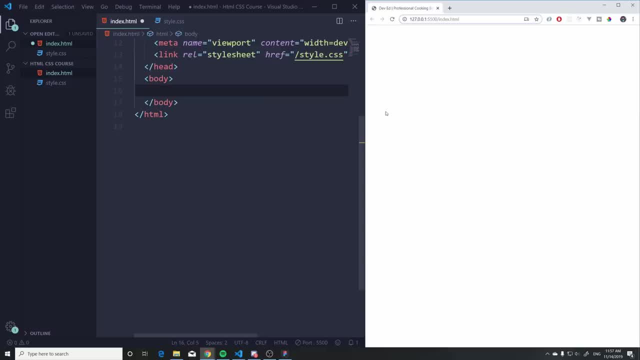 website. we're gonna be using something website. we're gonna be using something called floats, and I don't recommend this called floats and I don't recommend this called floats and I don't recommend this at all. but we're gonna do it just so, we at all, but we're gonna do it just so we. 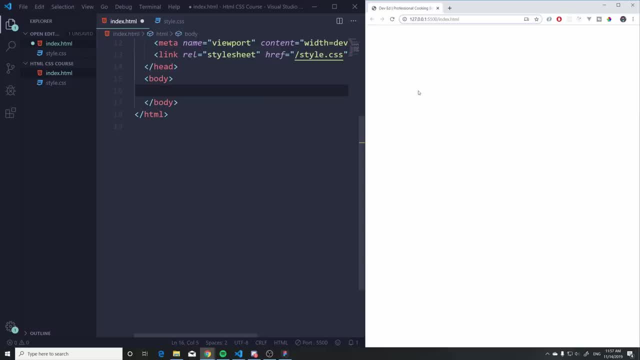 at all, but we're gonna do it just so we can create a super basic website after can create a super basic website after can create a super basic website. after that we're gonna jump into flexbox, which that we're gonna jump into flexbox, which that we're gonna jump into flexbox, which enables us to do some, some designs. very 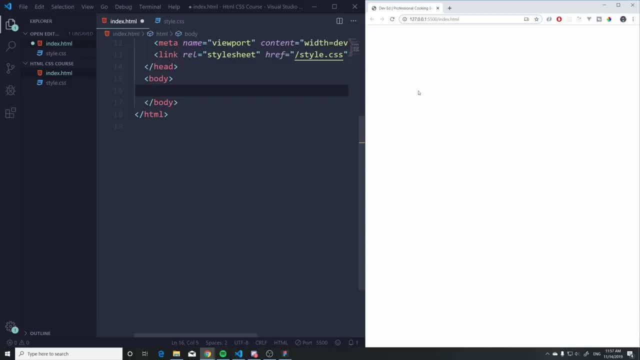 enables us to do some some designs, very enables us to do some some designs very simply: some layouts, responsive layouts- simply some layouts, responsive layouts, simply some layouts, responsive layouts, and all of those wonderful stuff. so, and all of those wonderful stuff, so, and all of those wonderful stuff, so, bear with me, we're gonna do two more. 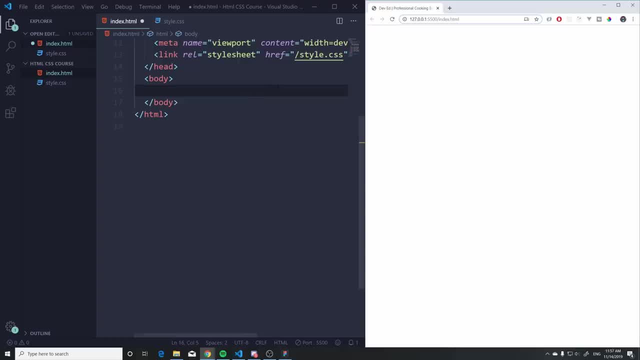 bear with me, we're gonna do two more. bear with me, we're gonna do two more quick episodes and later on, if we're quick episodes, and later on if we're quick episodes, and later on if we're also in the projects, we're also gonna. also in the projects, we're also gonna. 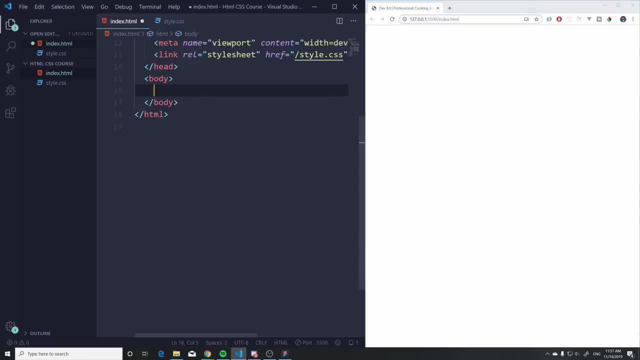 also in the projects, we're also gonna cover other CSS properties and some cover other CSS properties and some cover other CSS properties and some other tips and tricks. okay, so I'm not other tips and tricks. okay, so I'm not other tips and tricks. okay, so I'm not gonna cover all everything that you can. 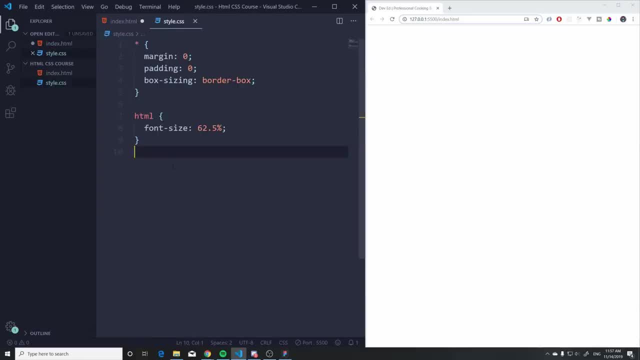 gonna cover all everything that you can. gonna cover all everything that you can do in CSS because, frankly, that's do in CSS, because, frankly, that's do in CSS, because, frankly, that's honestly just a waste of time. we want to. honestly just a waste of time. we want to. 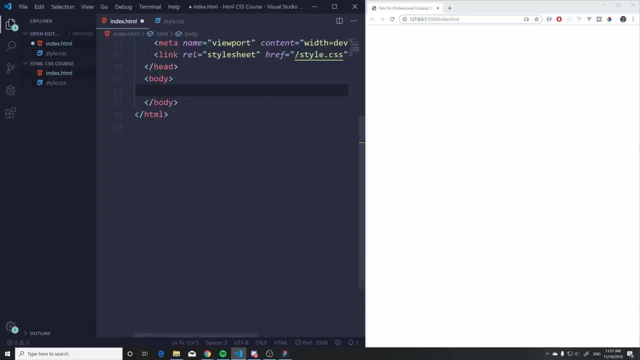 honestly just a waste of time. we want to know all the important stuff and when know all the important stuff and when know all the important stuff and when we're actually building projects. it's, we're actually building projects, it's we're actually building projects. it's gonna be more valuable to see there that. 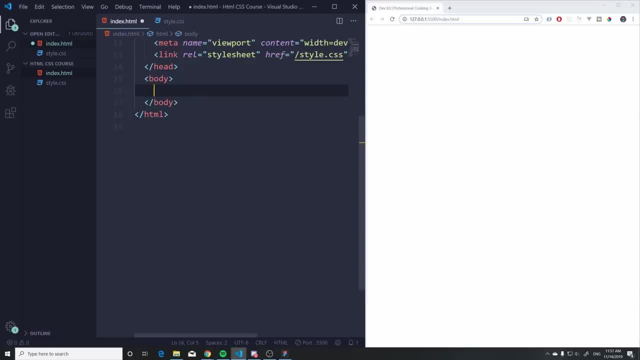 gonna be more valuable to see there. that gonna be more valuable to see there. that just means building it out here for zero. just means building it out here for zero. just means building it out here for zero reason. so one I want to cover which I reason. so one I want to cover which I. 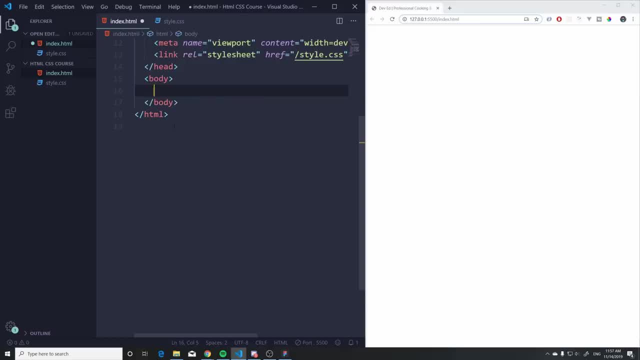 reason. so one I want to cover which I think is fairly important, that you're think is fairly important, that you're think is fairly important that you're gonna use it. a lot is something called gonna use it. a lot is something called gonna use it. a lot is something called pseudo classes. alright, so I'm gonna add: 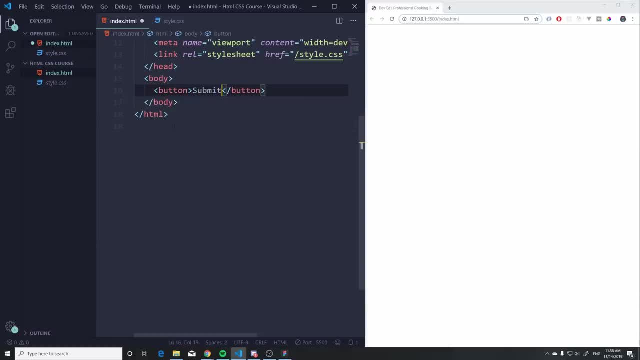 pseudo classes. alright, so I'm gonna add pseudo classes. alright, so I'm gonna add a button here. I'm just gonna keep it a button here. I'm just gonna keep it a button here. I'm just gonna keep it very simple and I'm gonna add a submit. 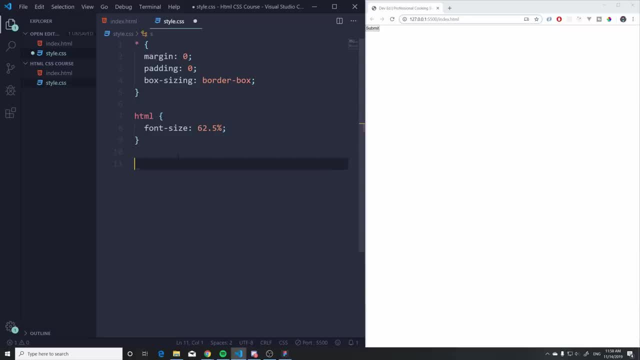 very simple and I'm gonna add a submit. very simple and I'm gonna add a submit. okay, so there we go, so we can get that. okay, so there we go, so we can get that. okay, so there we go, so we can get that button here. I'm gonna say button, that's. 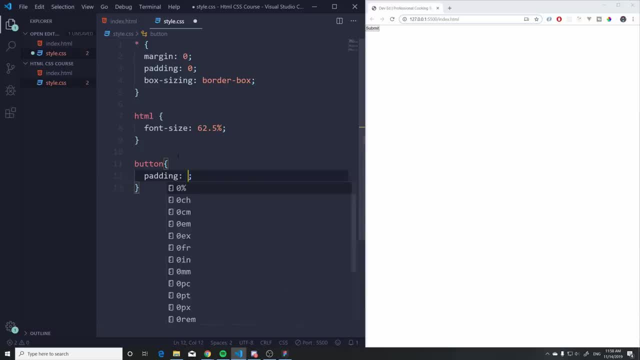 button. here I'm gonna say: button, that's button. here I'm gonna say: button, that's not a class, just a simple button and not a class, just a simple button and not a class, just a simple button. and I'm gonna say: padding, we're gonna do 2. 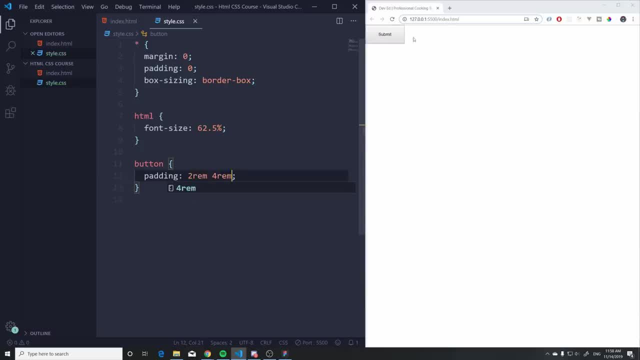 I'm gonna say padding, we're gonna do 2. I'm gonna say padding, we're gonna do 2 rem and 4. rem for the width and the, the rem and 4 rem for the width and the, the rem and 4 rem for the width and the, the for the width. yeah, that's, that's what I. 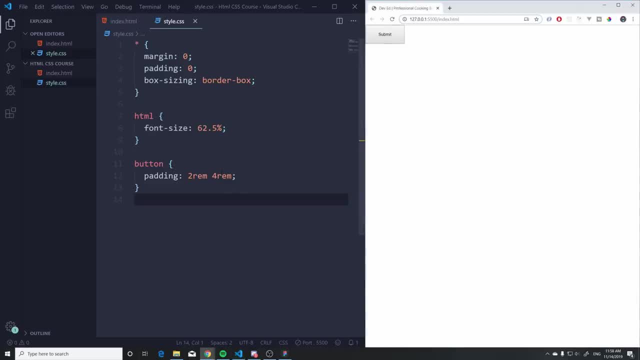 for the width: yeah, that's that's what I. for the width: yeah, that's that's what I tried to say. so, take a look at this. we tried to say so: take a look at this. we tried to say so: take a look at this. we can style this the way we want, but let 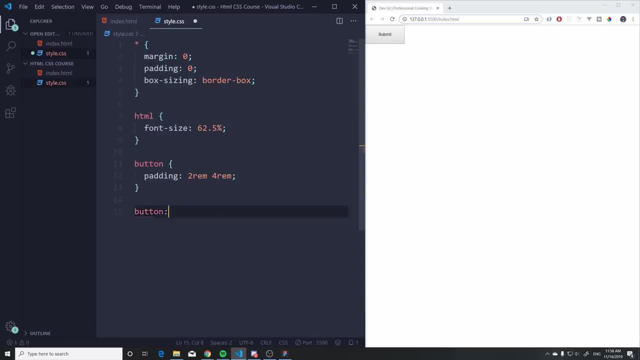 can style this the way we want. but let can style this the way we want. but let me kind of show you what these pseudo me kind of show you, what these pseudo me kind of show you what these pseudo classes are. you can select the button. classes are, you can select the button. 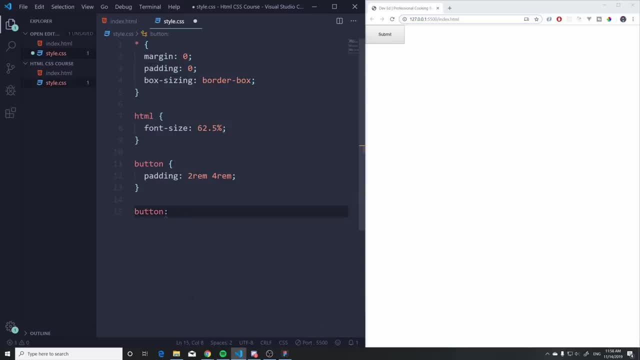 classes are. you can select the button and you can add this colon here and what, and you can add this colon here and what, and you can add this colon here, and what you do is. let me show you a few pseudo. you do is. let me show you a few pseudo. 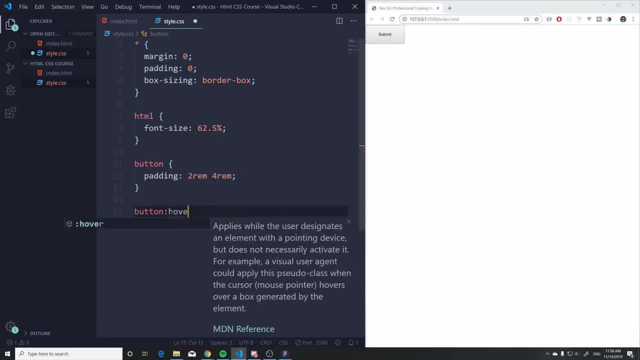 you do is let me show you a few pseudo classes. one is called hover, and when we classes, one is called hover, and when we classes, one is called hover and when we add it like this, what happens is if we add it like this. what happens is if we 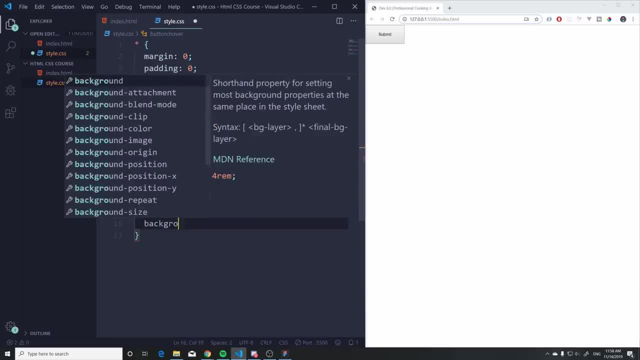 add it like this: what happens is if we change, if we add another property like change, if we add another property like change, if we add another property like background lights blue or light gray. background lights blue or light gray. background lights blue or light gray. when we hover over it, as you can see, 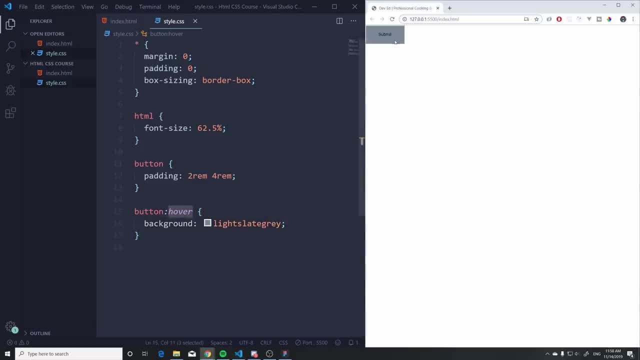 when we hover over it, as you can see. when we hover over it, as you can see, that background changes its color. so only that background changes its color. so only that background changes its color. so only when your mouse gets hovered over that. when your mouse gets hovered over that. 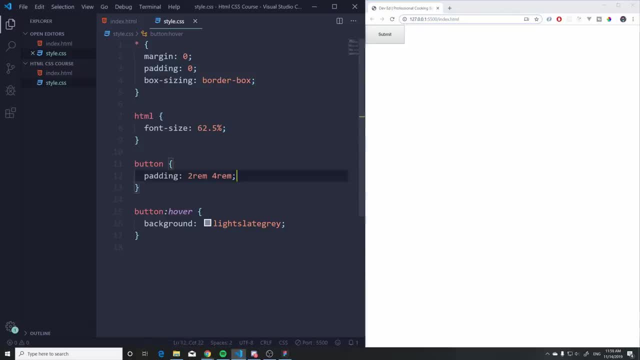 when your mouse gets hovered over that lane, that button, the properties change. lane that button: the properties change. lane that button: the properties change. now we can do this on almost everything. now we can do this on almost everything. now we can do this on almost everything. so I can take the padding here and maybe 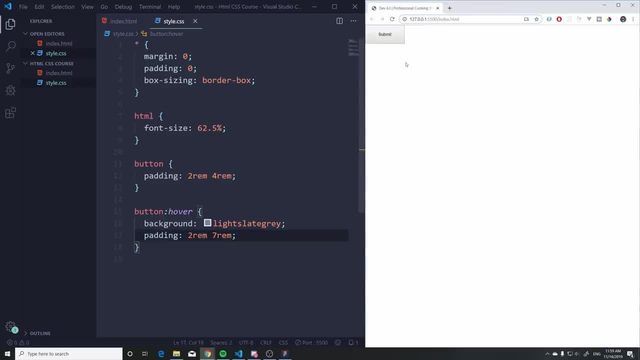 so I can take the padding here and maybe, so I can take the padding here and maybe I can make this longer, so that works as I can make this longer, so that works. as I can make this longer, so that works as well. take a look, so this is one that 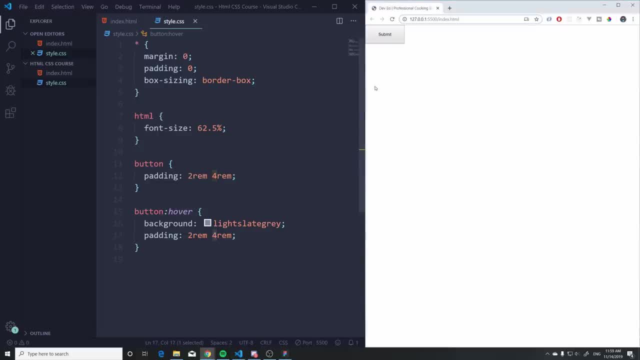 well, take a look. so this is one that- well, take a look. so this is one that we're gonna use a lot when we want to. we're gonna use a lot when we want to. we're gonna use a lot when we want to hover over something, to give like an. 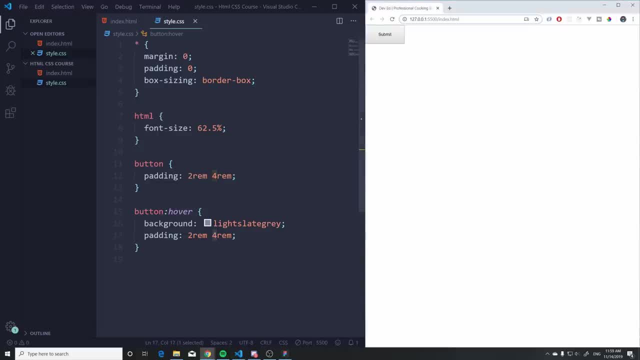 hover over something. to give like an hover over something, to give like an indication that it, when we hover over it, indication that it, when we hover over it, indication that it, when we hover over it, it's gonna have some kind of effect. let it's gonna have some kind of effect. let 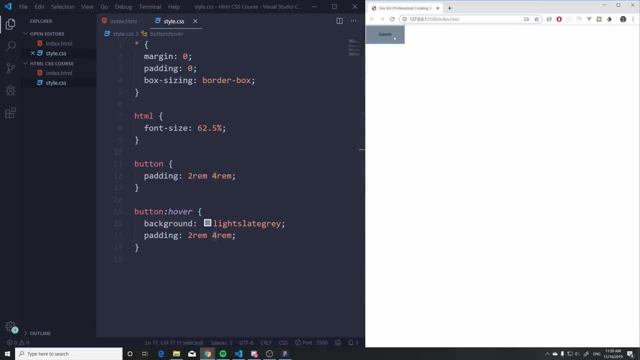 it's gonna have some kind of effect. let me also show you when we hover over this. me also show you when we hover over this. me also show you when we hover over this. as you can see, it's just a normal mouse. as you can see, it's just a normal mouse. 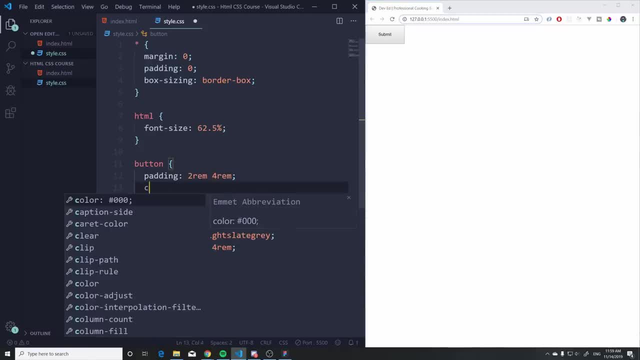 as you can see, it's just a normal mouse. we can also change the cursor, so I can. we can also change the cursor, so I can. we can also change the cursor so I can go to the button and add a cursor. go to the button and add a cursor. 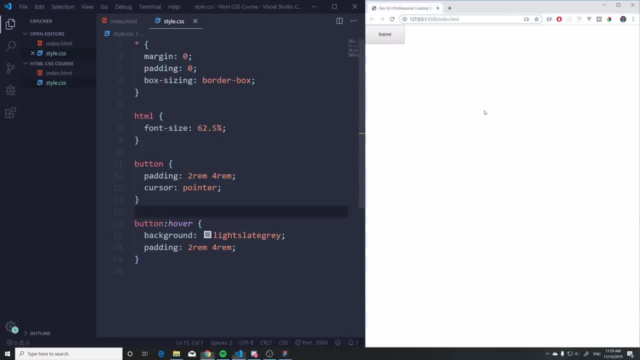 go to the button and add a cursor pointer to this and when we hit save pointer to this, and when we hit save pointer to this, and when we hit save, you're gonna see that it changes the. you're gonna see that it changes the. you're gonna see that it changes the cursor. so now it's like a clickable. 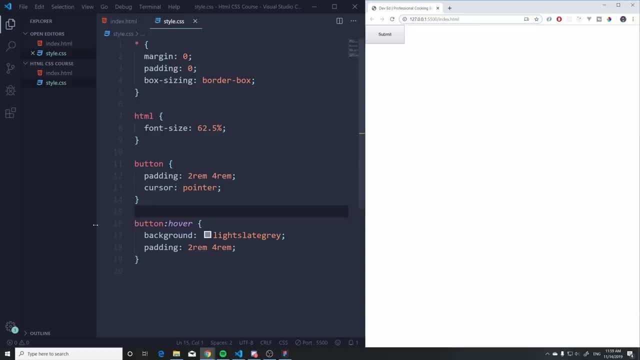 cursor, so now it's like a clickable cursor. so now it's like a clickable pointer cursor and that's what I tried, pointer cursor, and that's what I tried, pointer cursor, and that's what I tried to say: okay, so another one, I want to, to say: okay, so another one, I want to. 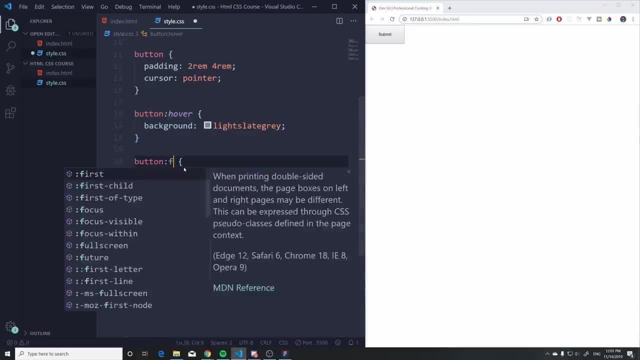 to say okay. so another one I want to show you is called focus, so let me copy: show you is called focus, so let me copy: show you is called focus, so let me copy this over here: I'm gonna change this, this over here. I'm gonna change this. 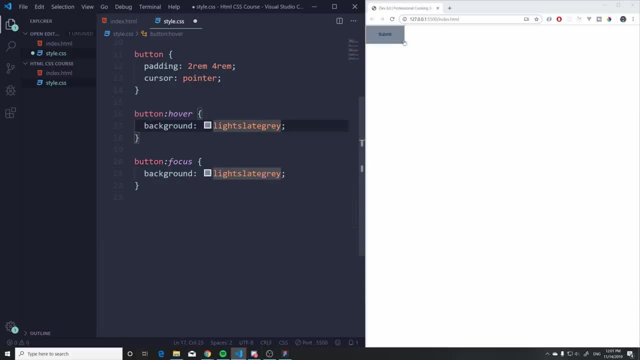 this over here. I'm gonna change this focus, which all means that when the focus, which all means that when the focus, which all means that when the turn green and when we unclick from it, it's turn green and when we unclick from it, it's. 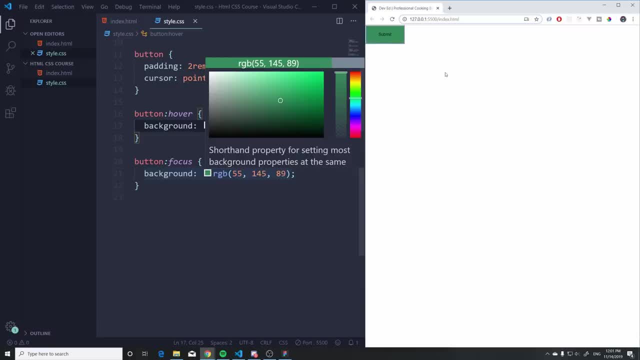 turn green and when we unclick from it it's gonna turn back to normal. so hover gonna turn back to normal. so hover gonna turn back to normal. so hover, focus on hover. I can show you a better focus on hover. I can show you a better focus on hover. I can show you a better example with the input like this. so we 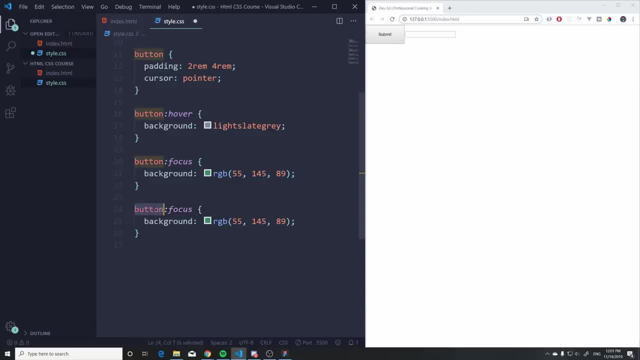 example with the input like this: so we example with the input like this: so we add an input text and then I'm gonna add an input text and then I'm gonna add an input text and then I'm gonna copy this over and just change it to: 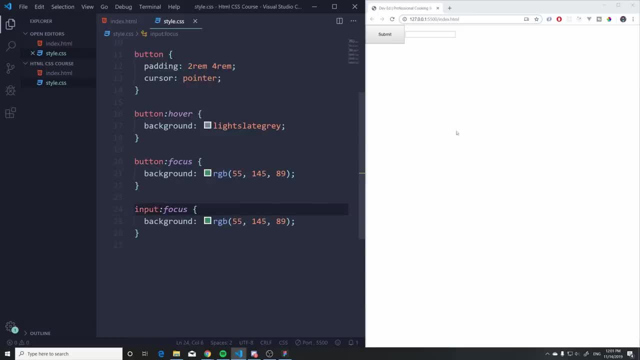 copy this over and just change it. to copy this over and just change it to input. so when we hit tab, you're gonna input. so when we hit tab, you're gonna input. so when we hit tab, you're gonna see if we hit tab here. now, that's focused. 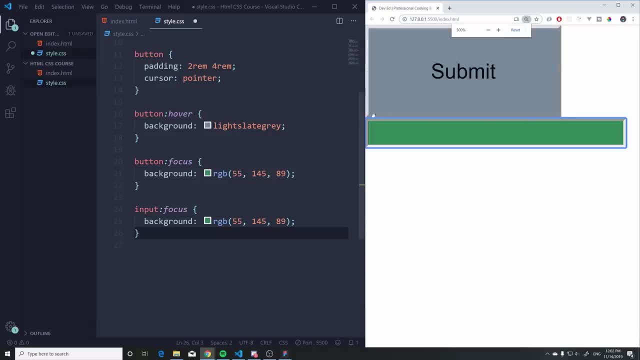 see if we hit tab here now, that's focused. see if we hit tab here now, that's focused. if I hit tab again, that's gonna be. if I hit tab again, that's gonna be. if I hit tab again, that's gonna be focused. you can tell by the blue outline. 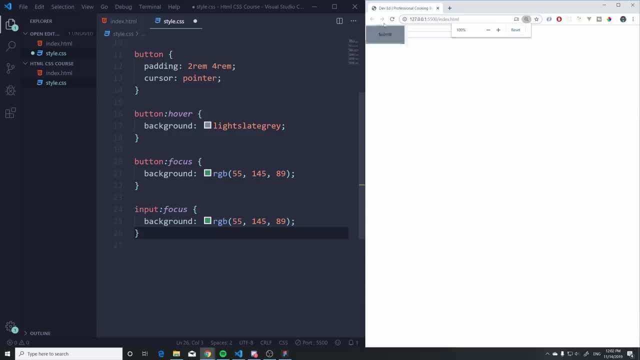 focused. you can tell by the blue outline focused. you can tell by the blue outline on top of it. so that is focused, that's on top of it. so that is focused, that's on top of it, so that is focused. that's something that we are also gonna use. a. 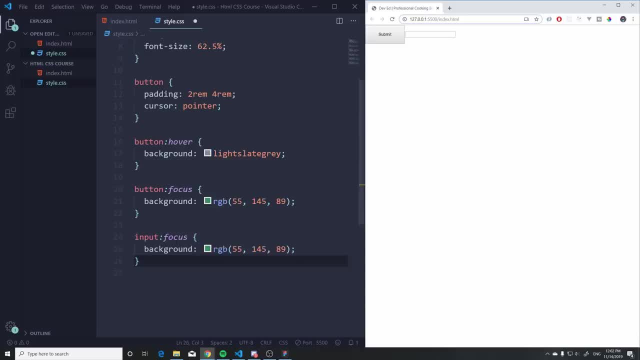 something that we are also gonna use, a something that we are also gonna use a lot all right, and you've seen a few lot all right, and you've seen a few lot all right, and you've seen a few already. you've seen that we had that. 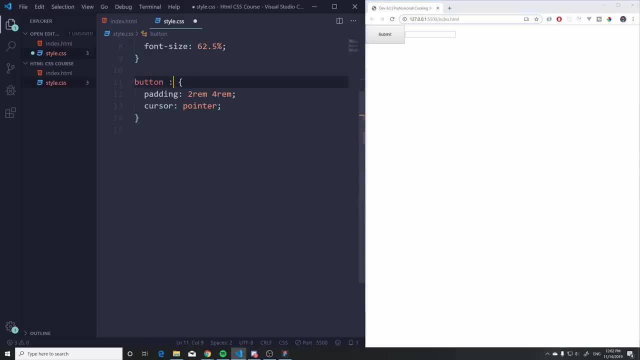 already. you've seen that we had that already. you've seen that we had that- and child so and child like this right and child so and child like this right and child so and child like this right, and we can add a one and that's gonna, and we can add a one and that's gonna. 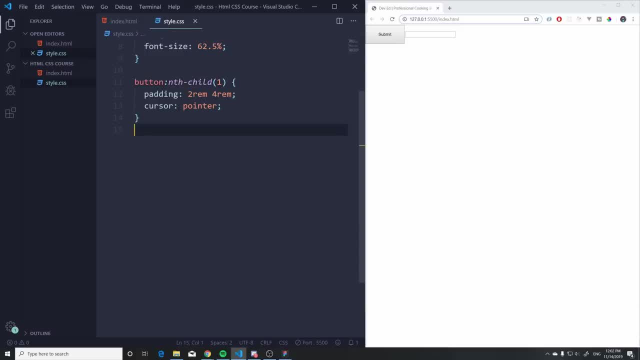 and we can add a one, and that's gonna select this one. let me get rid of that. select this one. let me get rid of that. select this one. let me get rid of that. really quickly, there we go, so that's really quickly. there we go, so that's. 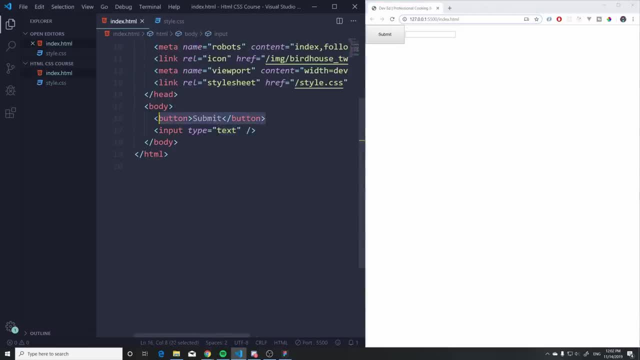 really quickly. there we go. so that's gonna select only this button, the first gonna select only this button, the first gonna select only this button, the first button that it detects. so if I duplicate button that it detects, so if I duplicate button that it detects, so if I duplicate this a few more times, as you can see, 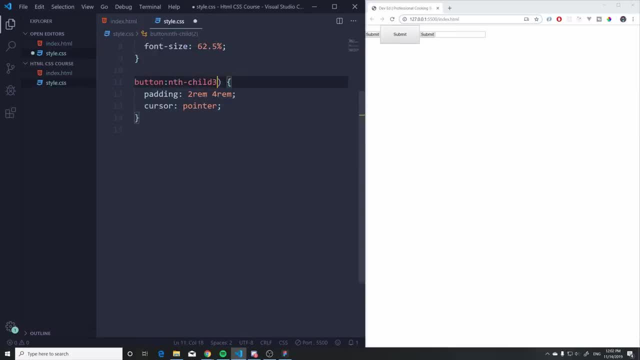 this a few more times, as you can see this a few more times. as you can see, that's the one that gets selected. add 2: that's the one that gets selected. add 2: that's the one that gets selected. add 2 and 3, and that is a pseudo class as well. 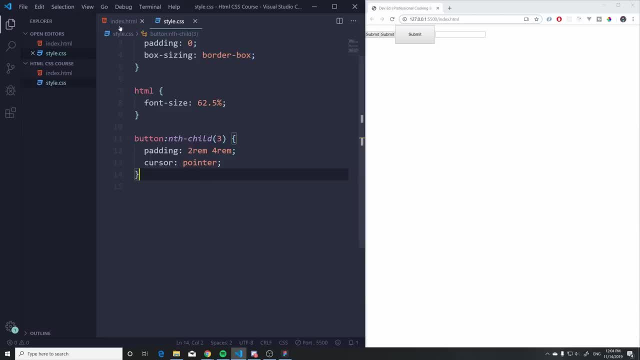 and 3, and that is a pseudo class as well. and 3, and that is a pseudo class as well. now there's another thing called pseudo. now there's another thing called pseudo. now there's another thing called pseudo elements. let me show you that, really elements. let me show you that really. 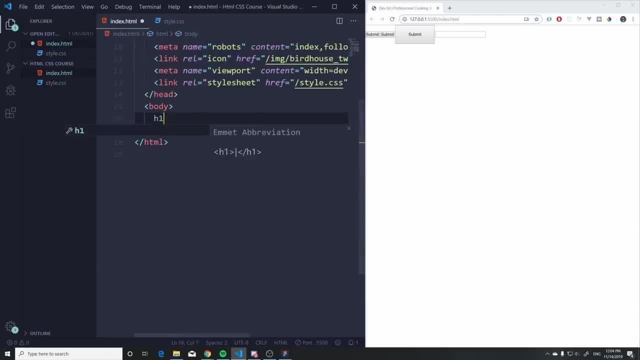 elements. let me show you that, really quickly, let's get rid of everything, and quickly let's get rid of everything, and quickly let's get rid of everything. and I'll just add a h1. that's gonna say: I'll just add a h1. that's gonna say: 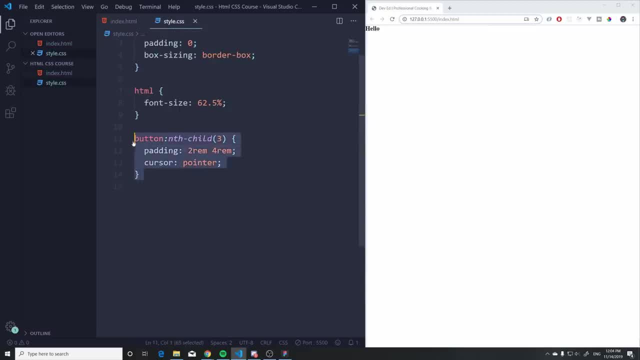 I'll just add a h1. that's gonna say hello, all right, a pseudo element is used. hello, all right. a pseudo element is used. hello, all right. a pseudo element is used to add additional content from within. to add additional content from within. to add additional content from within your CSS. I know it's crazy, so let me. 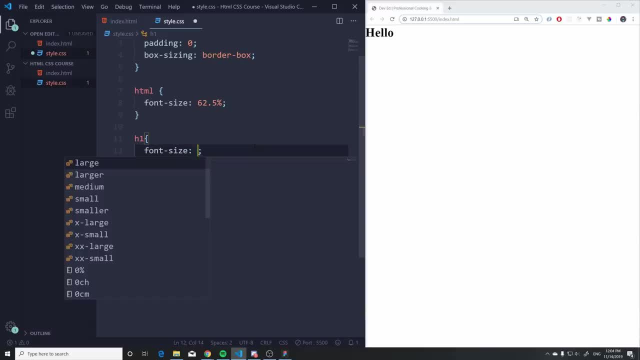 your CSS. I know it's crazy, so let me your CSS. I know it's crazy, so let me show you we can get the h1 at a font. show you we can get the h1 at a font. show you we can get the h1 at a font size of, let's say, for REM. all right, 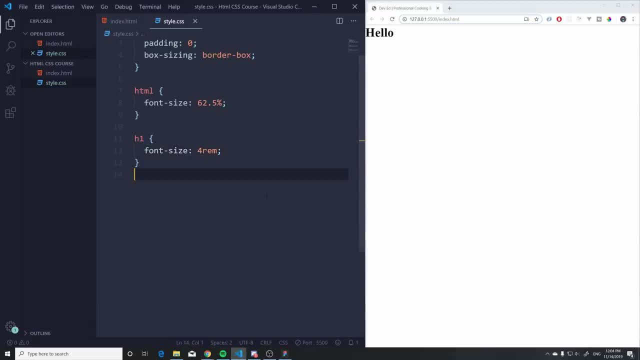 size of, let's say for REM: all right. size of, let's say for REM: all right, let's make the smaller, okay. so what you? let's make the smaller okay. so what you? let's make the smaller, okay. so what you can do is you can say h1 and add two. 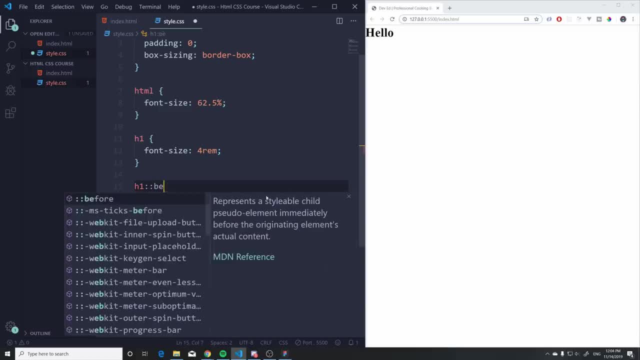 can do is you can say h1 and add two can do, is you can say h1 and add two colons and say after or before all colons. and say after or before all colons and say after, all, right, and basically what after is gonna do, is you? 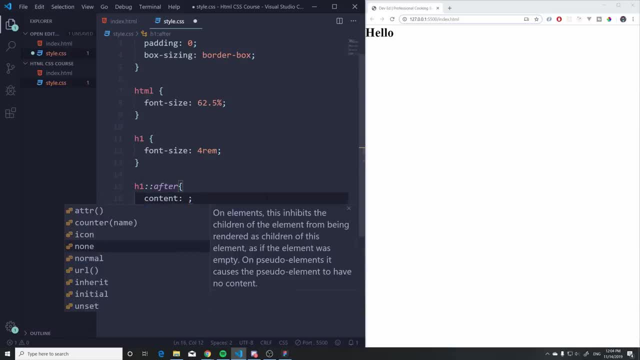 right and basically what after is gonna do. is you right and basically what after is gonna do is you can add content within your HTML. can add content within your HTML. can add content within your HTML: here so content and you add two quotes and here so content and you add two quotes and. 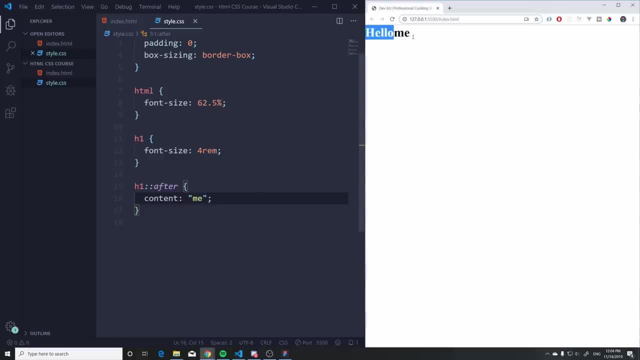 here so content, and you add two quotes and you can say hello me and, as you can, you can say hello me and, as you can, you can say hello me and, as you can see, it's gonna add additional content here. see, it's gonna add additional content here. 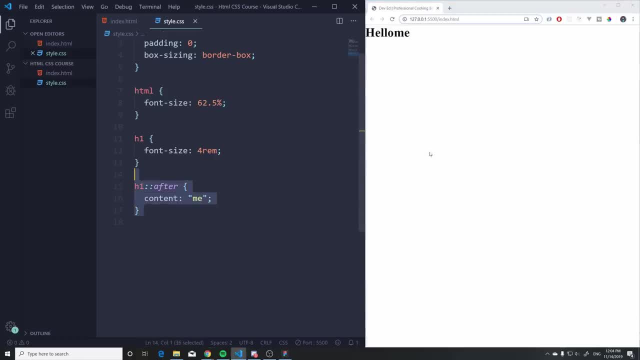 see it's gonna add additional content here. now we cannot select this. because now we cannot select this? because now we cannot select this? because this is done within your CSS and in your. this is done within your CSS and in your. this is done within your CSS and in your HTML markup. if we check here: h1, it only 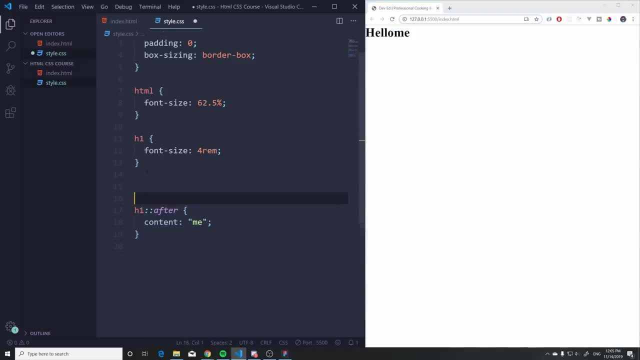 HTML markup. if we check here h1, it only HTML markup. if we check here h1, it only says hello, and this can be done as well. says hello, and this can be done as well. says hello, and this can be done as well with before. so we can say: before all. 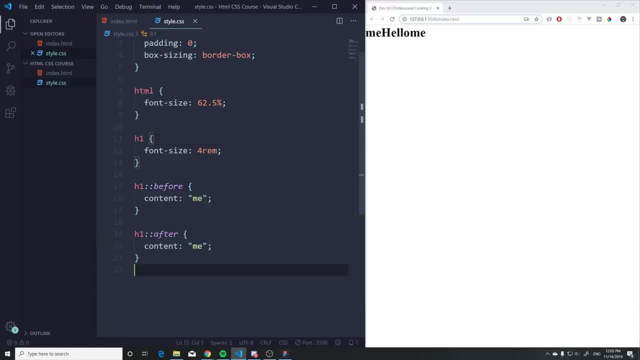 with before. so we can say before, all with before. so we can say before: all right, and there we go, we can add some right, and there we go. we can add some right and there we go. we can add some content before it. now, honestly, this is content before it. now, honestly, this is. 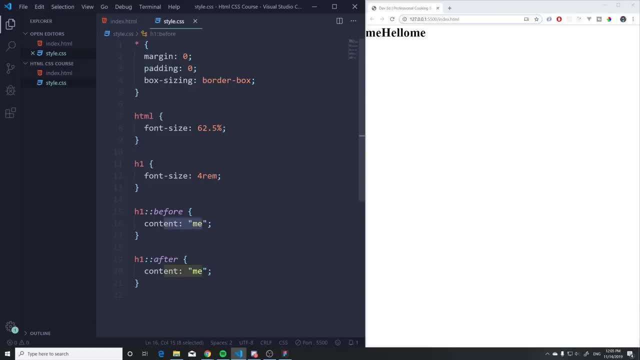 content before it. now, honestly, this is mostly used not to actually add content. mostly used not to actually add content, mostly used not to actually add content but to style an element in a few, but to style an element in a few, but to style an element in a few different ways, and we're gonna see in. 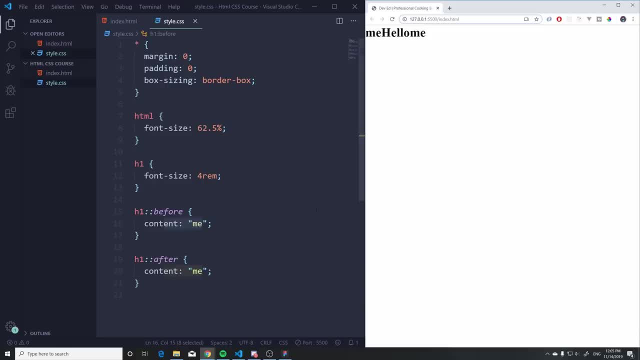 different ways and we're gonna see in different ways and we're gonna see in the last part of the series, right after the last part of the series, right after the last part of the series, right after this video, how we can use this in a more, this video, how we can use this in a more. 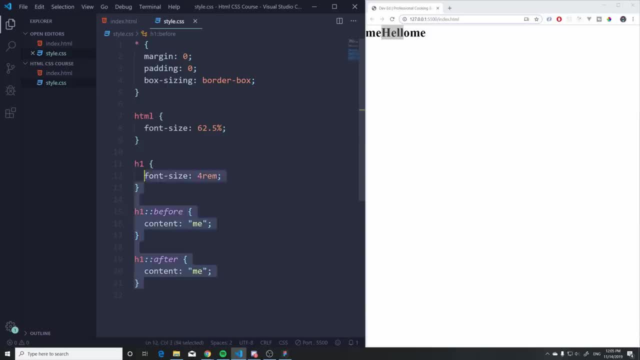 this video, how we can use this in a more practical way. I should say so. but I practical way, I should say so, but I practical way, I should say so. but I wanted to show you these who you know, wanted to show you these who you know, wanted to show you these who you know. and then you have pseudo classes and 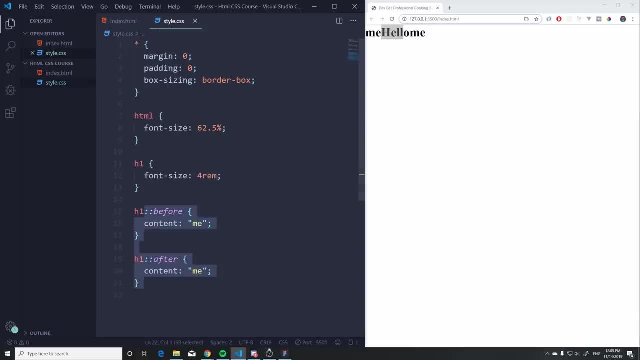 and then you have pseudo classes, and and then you have pseudo classes and also pseudo elements. okay, so, let's take also pseudo elements. okay, so let's take also pseudo elements. okay, so let's take a look at the old ways of how we used. a look at the old ways of how we used. 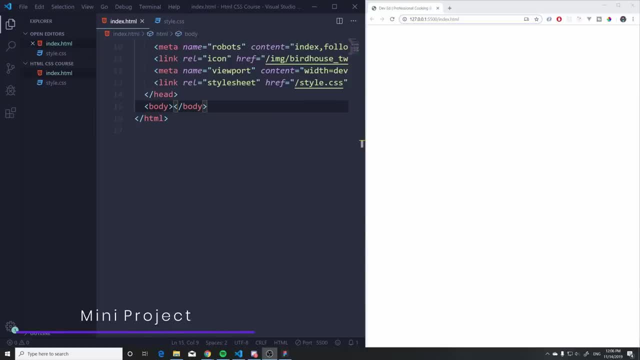 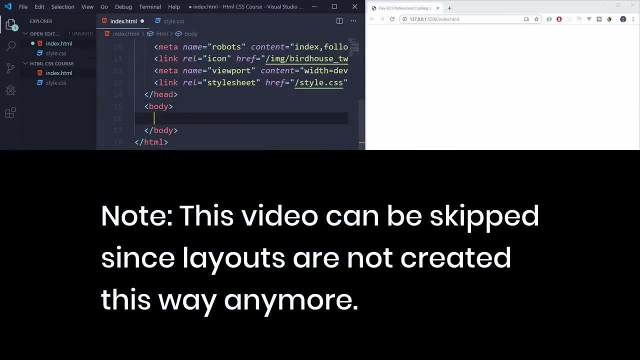 a look at the old ways of how we used to create layouts. okay, let's throw to create layouts. okay, let's throw to create layouts. okay, let's throw. so let's cover floats. let's start off with. so let's cover floats. let's start off with. 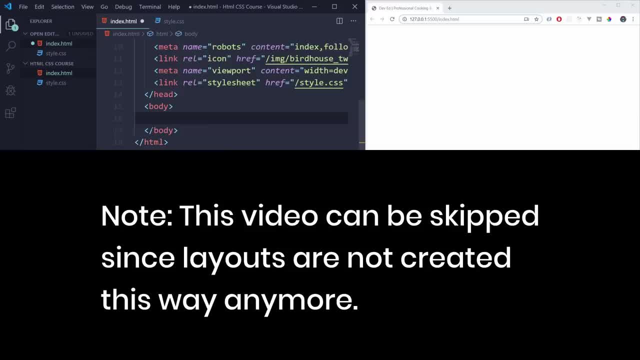 so let's cover floats. let's start off with just a few boxes, and then we're just a few boxes, and then we're just a few boxes, and then we're gonna implement a website. so let's do a box. gonna implement a website, so let's do a box. 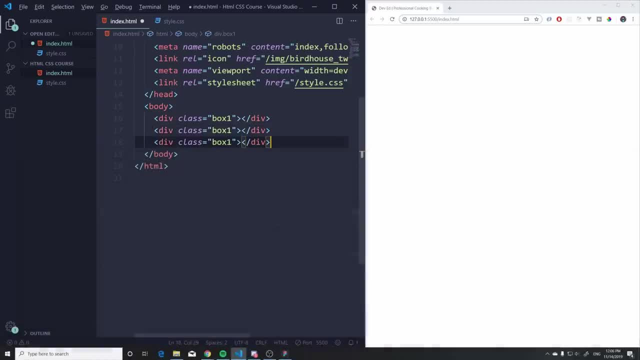 gonna implement a website, so let's do a box one, a box two and a box three. all one, a box two and a box three. all one, a box two and a box three. all right, I'm gonna change the names of this so. right, I'm gonna change the names of this so. 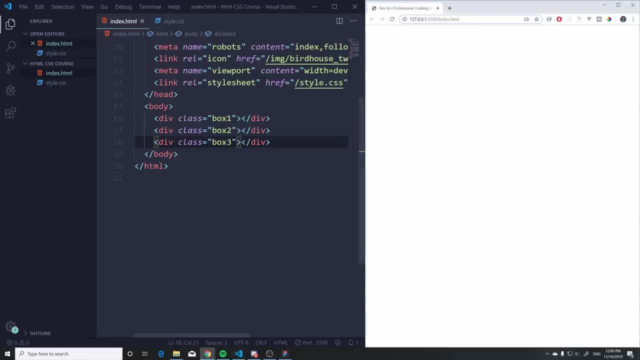 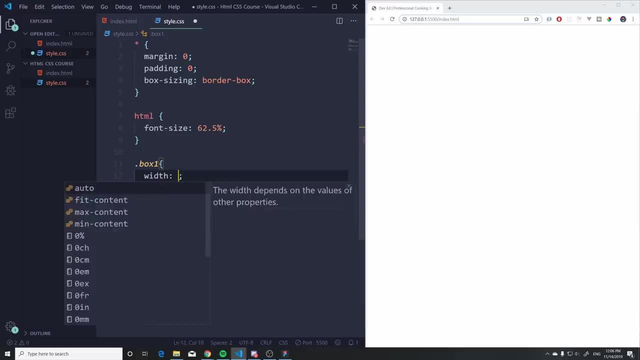 right, I'm gonna change the names of this so you can imagine these as beings. just you can imagine these as beings. just you can imagine these as beings- just some kind of content on your website. so some kind of content on your website, so some kind of content on your website. so I'm gonna set something like 30 Ren and 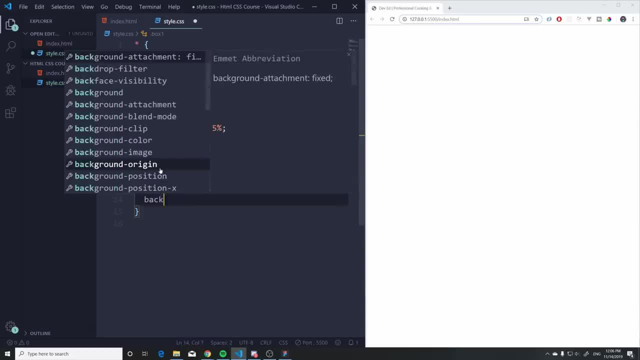 I'm gonna set something like 30 Ren. and I'm gonna set something like 30 Ren and hit save- all right, let's also add a hit save. all right, let's also add a hit save. all right, let's also add a background color to this background. 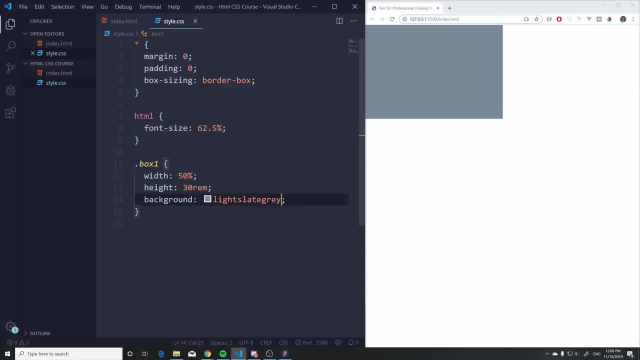 background color to this background background color to this background: light gray. so there it is. we can also light gray, so there it is. we can also light gray. so there it is. we can also change this so it looks more like a box. change this so it looks more like a box. 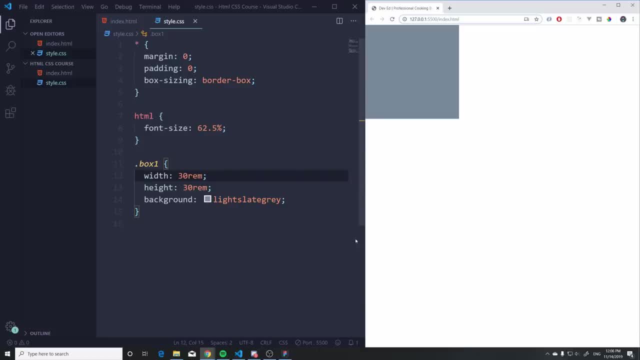 change this so it looks more like a box. we can do a 30 rem, there we go, so that's, we can do a 30 rem, there we go. so that's, we can do a 30 rem, there we go. so that's one, and then let's copy this over, or? 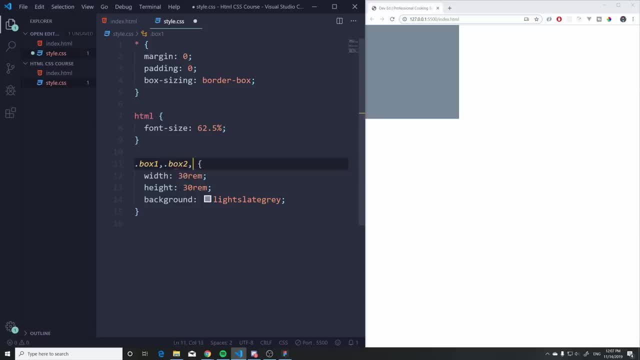 one and then let's copy this over, or one and then let's copy this over, or actually, what we can do is we can just actually what we can do is we can just actually what we can do is we can just duplicate this like so, all right, just so. 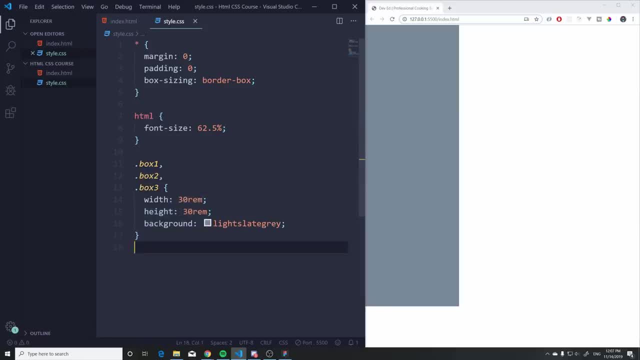 duplicate this like so. all right, just so. duplicate this like so. all right, just so. we also have the turkey ramps on top of, we also have the turkey ramps on top of, we also have the turkey ramps on top of it, and then we can change the background. 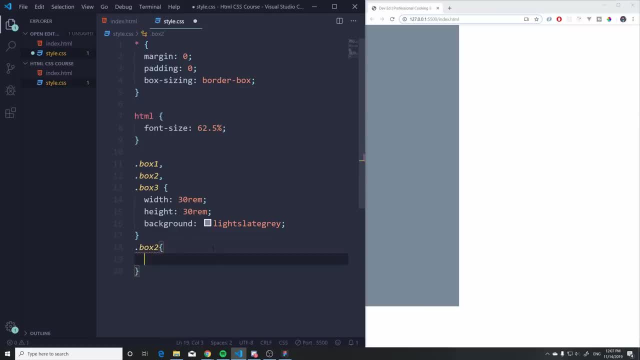 it and then we can change the background it, and then we can change the background. colors box 2 is gonna be background of colors. box 2 is gonna be background of colors. box 2 is gonna be background of. you know what we can do, actually, just 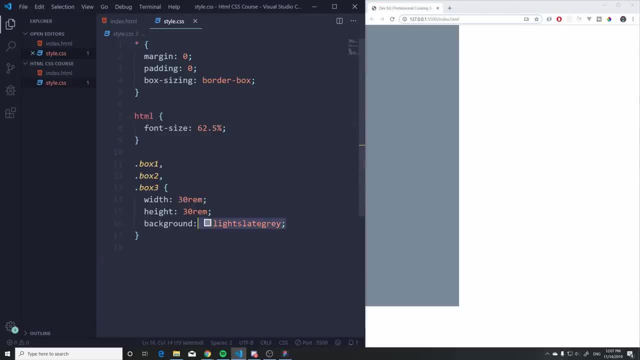 you know what we can do, actually, just you know what we can do, actually. just add a border to this and not a add a border to this and not a background. so let's remove this and just add a border of two pixels. all right, so these are. 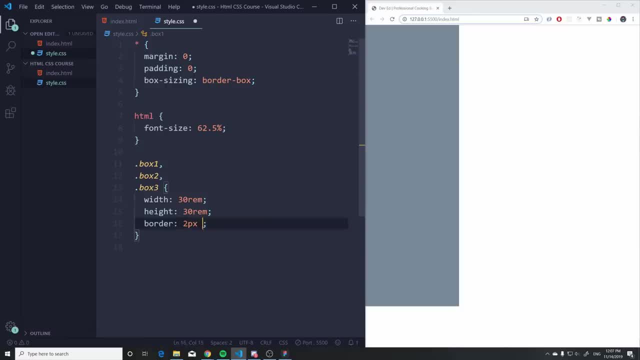 this is going to be the size of the border, solid is going to be the type of the border and finally, the color. we can just do black for now, okay, and basically we can change these to other ones, but they're not that nice. i can say dotted, but oh, no, that's, that looks terrible, so let's change back. 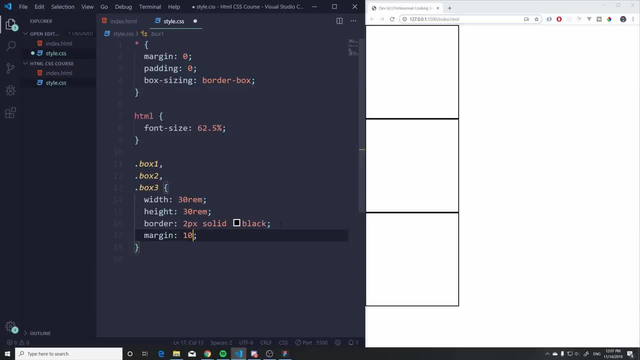 to solid, okay, let's also add a bit of margin between these 10. let's do one rem- okay, perfect. so i have these boxes. let's also add some content to it. let's make these larger a bit. let's do 50- okay, very nice. larger 80- very good, okay. and i also want to show you another cool property. 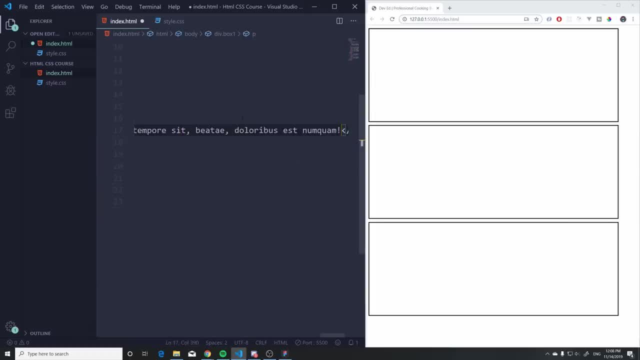 and here i'll just add a p tag: lorem 50. it's safe. all right, just some text. and i can calculate the size of the border, so let's do that. okay, so let's do that. okay, so let's do that. and i can calculate the size of the border, so let's do that. okay, so let's do that. okay, so let's do that. 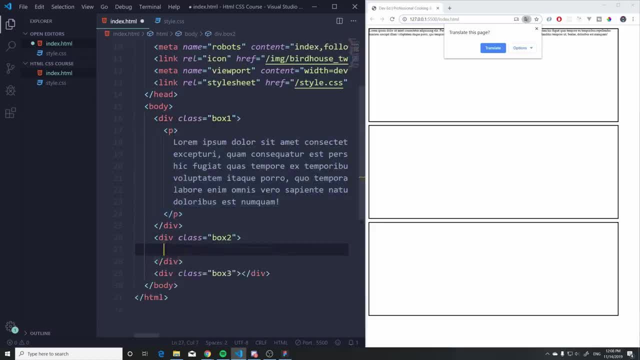 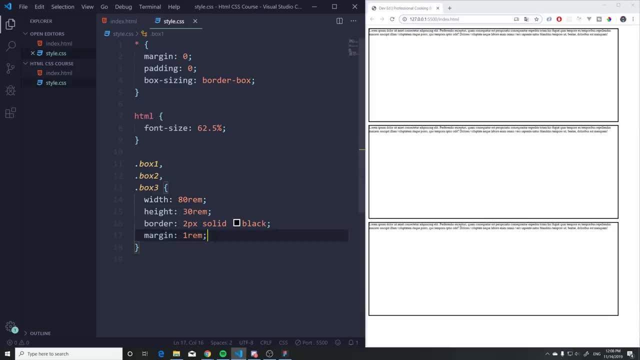 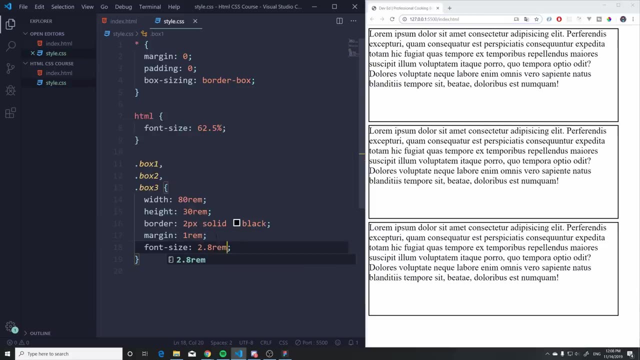 copy this over to box two and box three as well. okay, just so we have some text. okay, let's also add a font size here. so let's do font size and we're gonna do 2.8 rem. okay, perfect, so we have our content. as you can see, if i just change this to smaller, we're gonna have an issue. 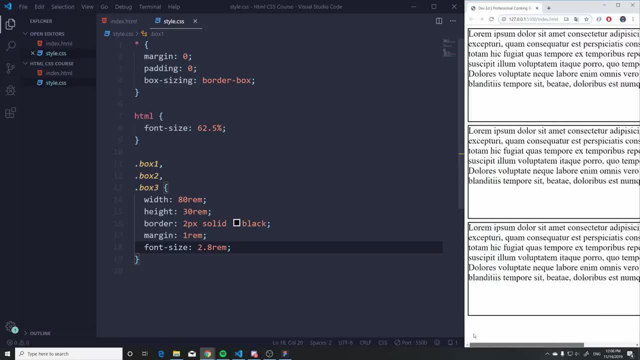 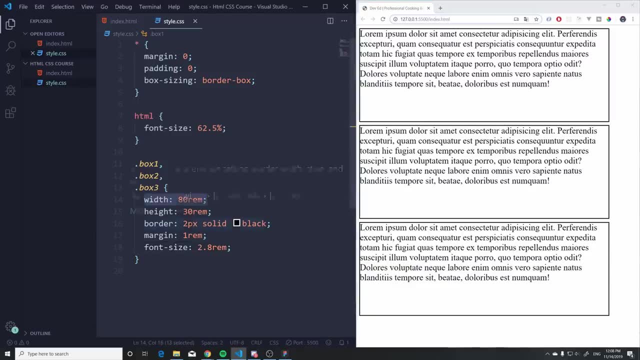 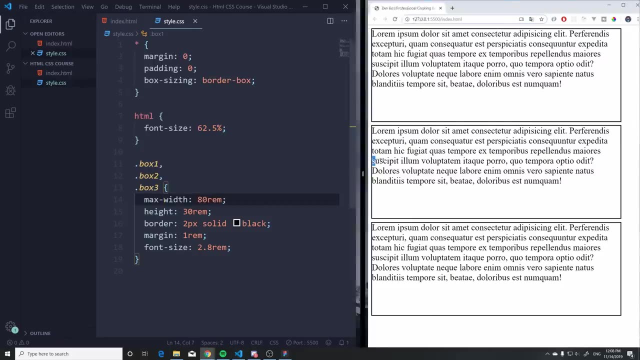 we can scroll, and that's something that you probably might not want to do. so what you can do is you can also limit this, and i'm going to introduce you something called max width. so if i change this to max width, let's see if that has any effect. if we make the smaller as you can. 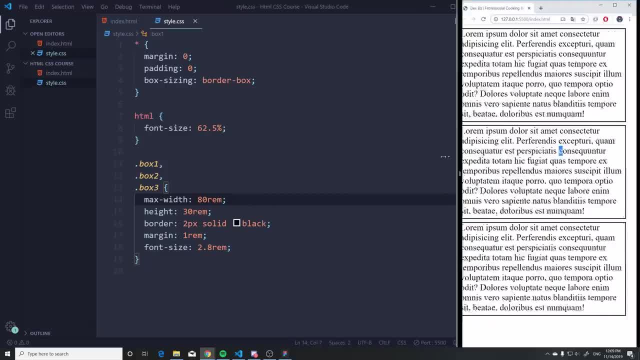 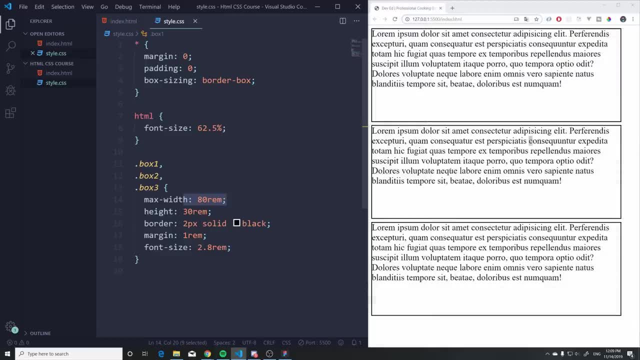 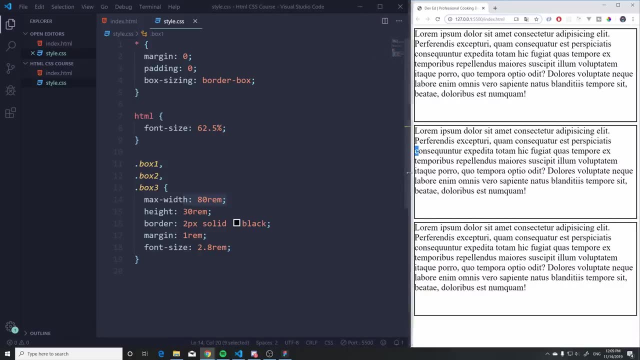 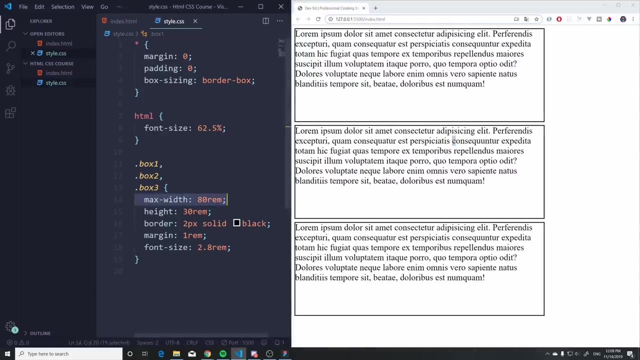 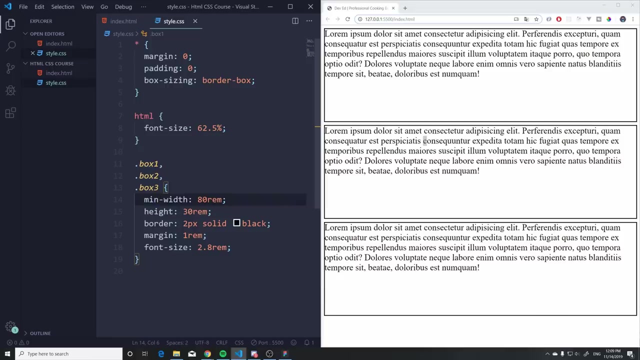 see, the maximum has to be 80, but it cannot go above that. it cannot go above that size of the. it actually wraps the text around it, all right. so we're basically putting a limit over our width, okay, and this can be used also as minimum. so the text basically should have a minimum. 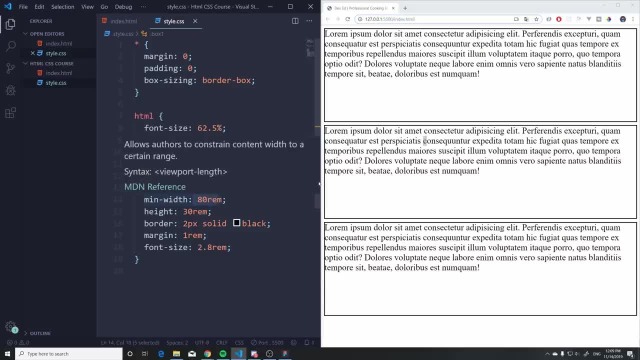 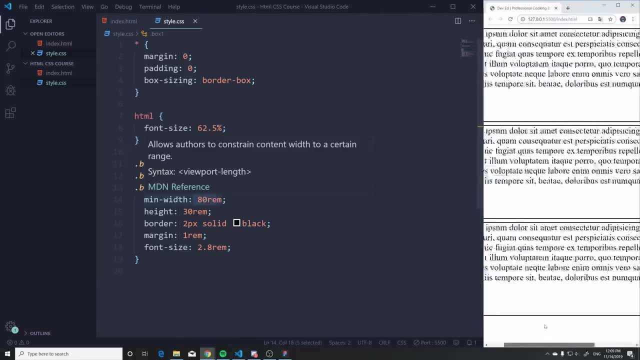 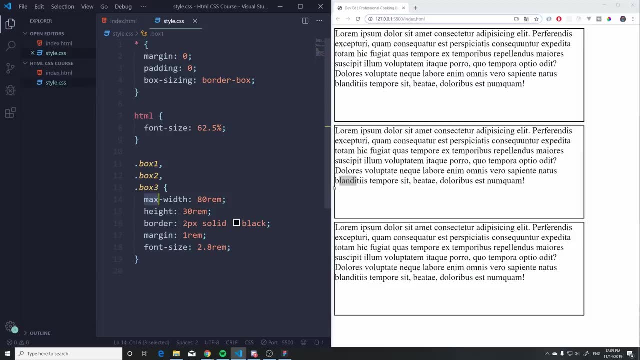 width of 80. it cannot be any smaller than this. that's what it says. so if i go smaller than that, it doesn't let it go smaller. so that's the maximum of the minimum. i i should say okay, and we're gonna see this with height and everything, but for now let's just leave it at max. 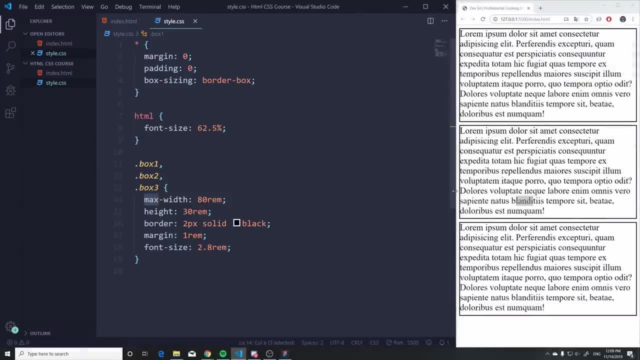 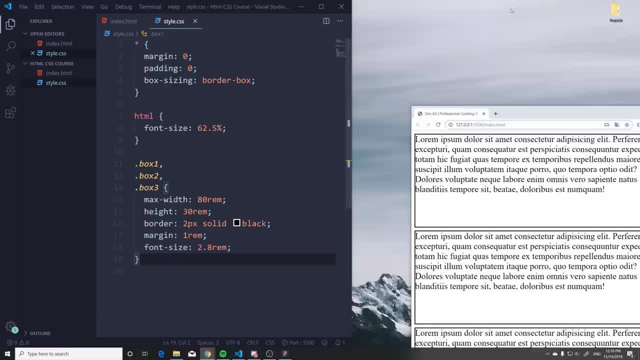 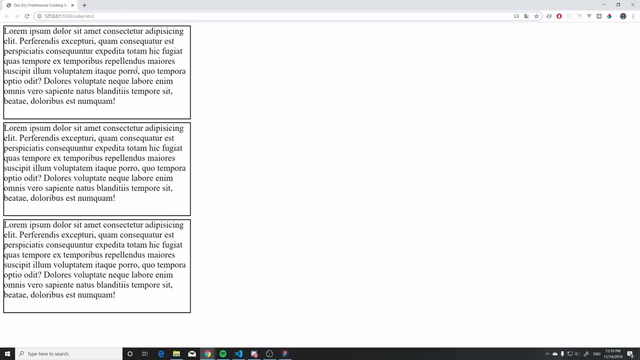 so the text actually wraps around it, perfect, okay, very good. so that's step one, and now let's take a look on how we can position these. i'm actually going to make this full screen like this, and i'm going to make it a bit smaller. let's do 60.. okay, what if i want to have this? 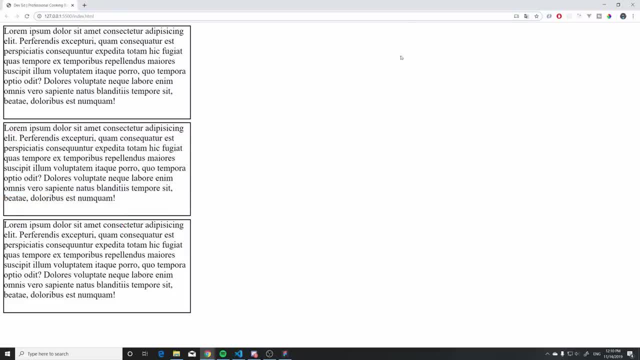 content. so the second part here: go up here. how can i do that? what can we do? well, there is a property called float, and this was used to actually create layouts, so you can imagine like you can do these on divs as well, and on elements as well, on anything that. 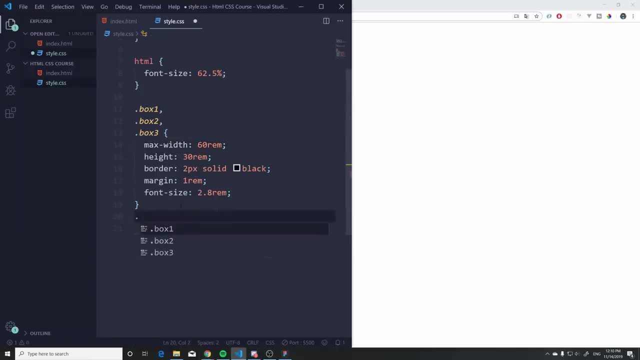 you want. so what you can do is i can grab the box too and i can say: float, let's try. what happens, what? What happens if I float it on the left side? All right, that's some weird things happening here. This kind of breaks. 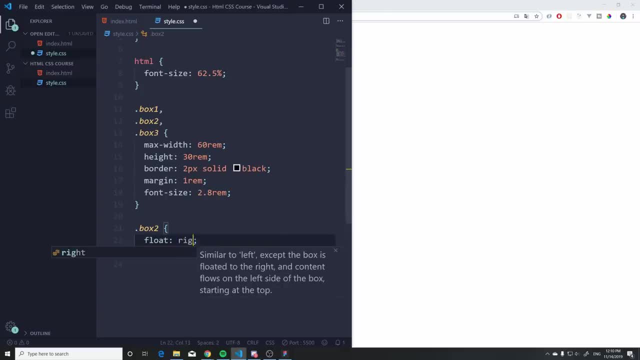 As you can see, the border goes up. What happens if I do on the right? All right, the content kind of flows over on this side. And if you don't know which box is which, let's kind of add some background colors to them. 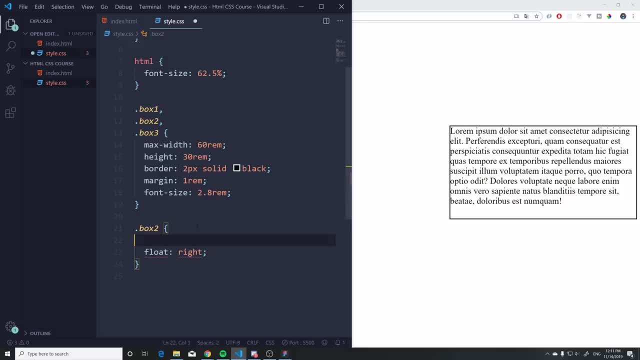 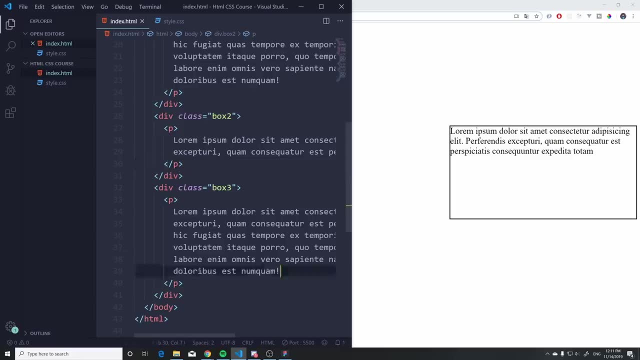 So box two is gonna have a background, or we can actually just add a title for in now to make this a bit more clear. So let's remove some text from here. Let's remove some text from here And let's remove some text from here. 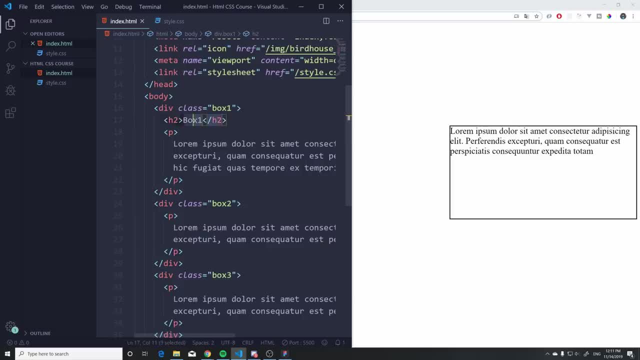 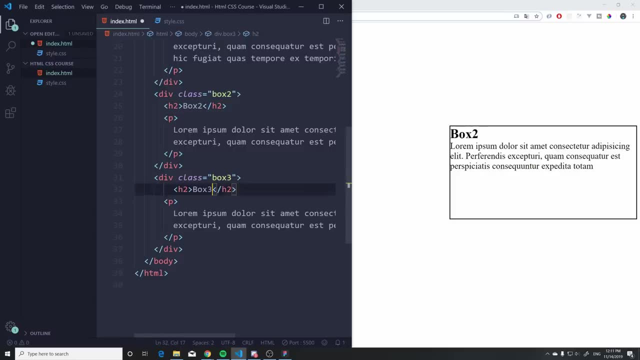 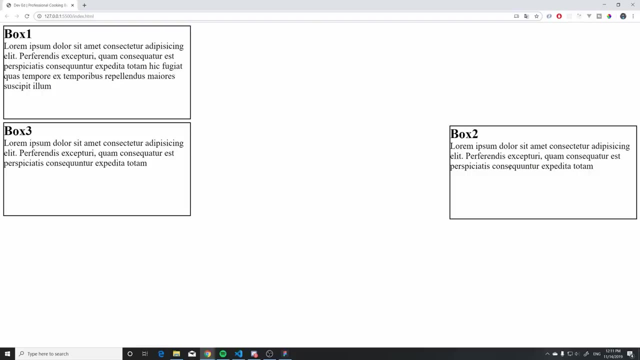 And we'll just add a H2 box, one like that, and box two and box three. Okay, perfect. So when we add on the box two a float to the right, it goes on the right side, Okay. so that's what I kind of want. 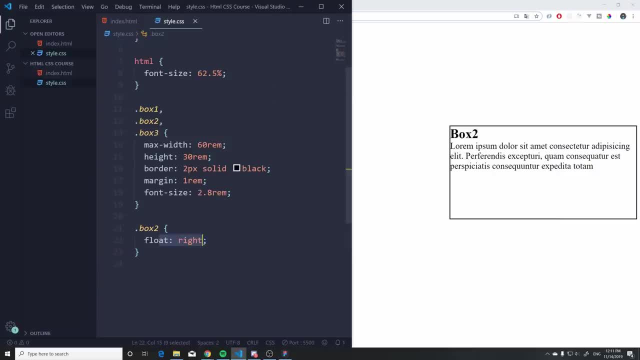 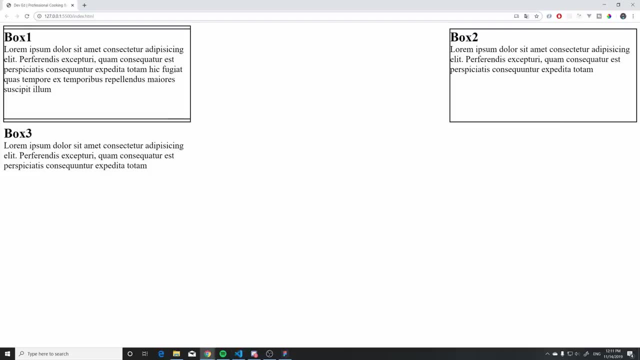 I want this to go up here, And the way you can do that is you can get the box one and float that on the left. So when you do that you have the box one here and the box one there. So basically you can kind of imagine. 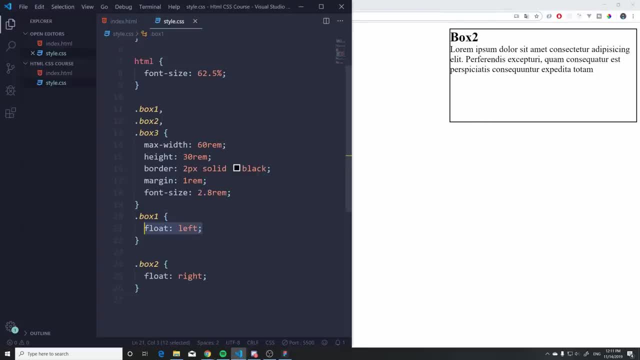 where you want your content to be. If I wanna, if I switch this over right and left and hit save, now the box floated to the right side and the box two floated to the left side. So this is how you can kind of position things. 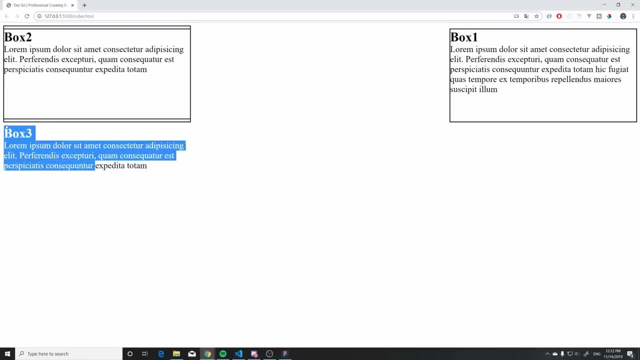 the way you want. However, there's one problem. This one breaks, as you can see- And this was a big issue and this is why I don't recommend it- just because it's very hard to style things this way- and you also have this issue where the height collapses. 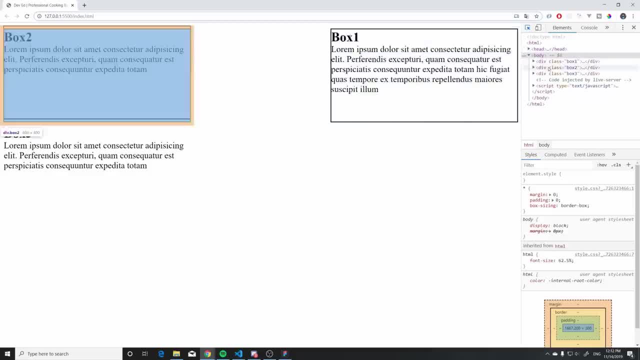 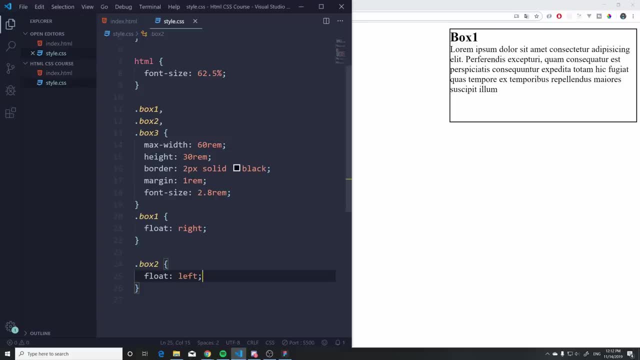 and things just don't go the way you want. As you can see, we have a box one, box two and that's it. this box three gets cut off. So the way you need to fix this is to add a clear. 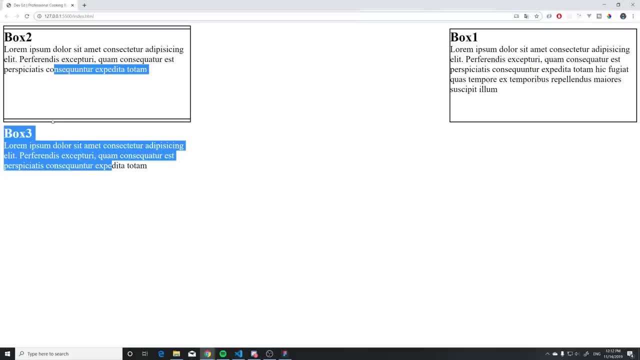 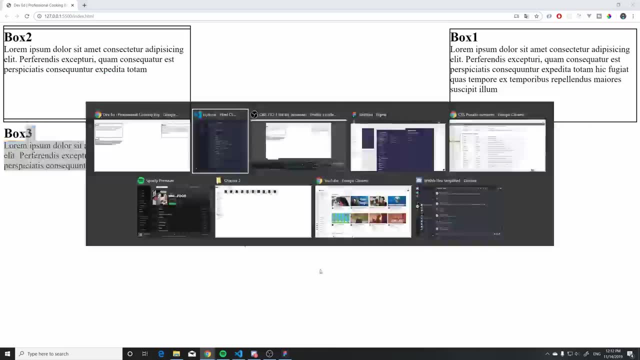 all right, because what happens now is all of the clear in this text. here you have to change this text, So what I'm gonna do is I'm gonna go to X bar short the content down below. So box three tries to be put up here next to the box one. So let's change. 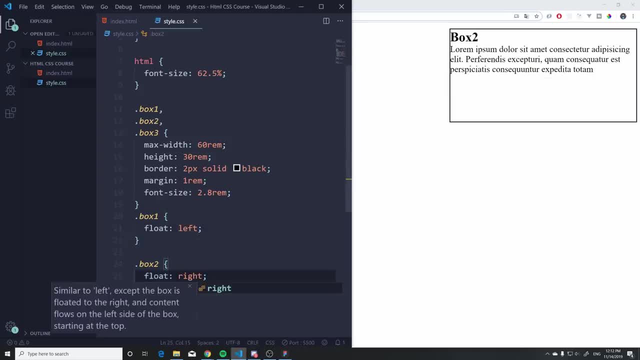 this back. Let me say left and right and hit save, And let's try to make this a bit smaller to see if we can see the results. So, as you can see, you have these weird things going on here. So to fix this, all you have to do is go below the boxes that you added the float on, and then you need. 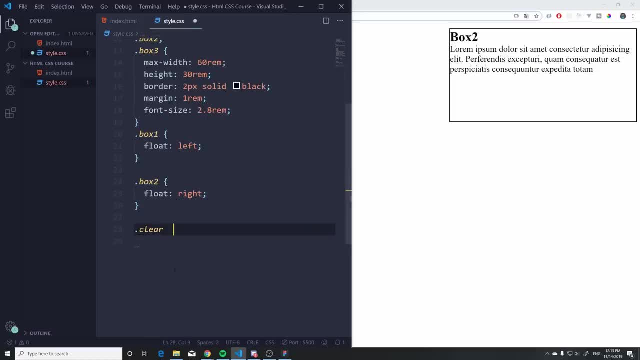 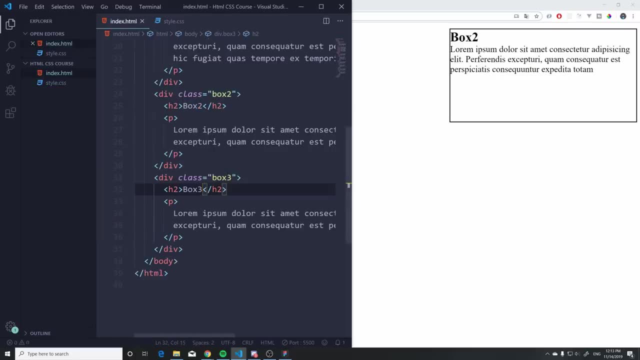 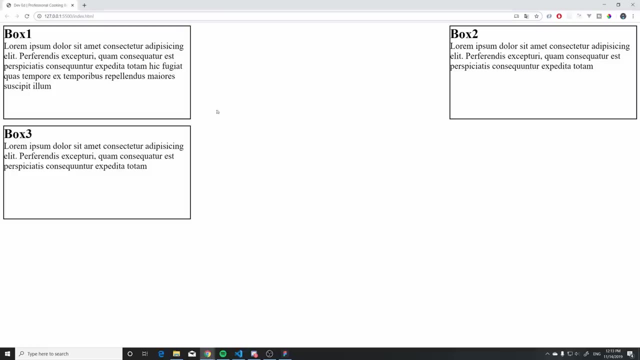 to clear it. So what we can do is create a class called clear, like this, and just add clear both and hit save. So now, if I introduce this down below, so after the box two I'll just add a clear- This is going to fix all of our issues. Okay, so there we go. It's a bit weird, So what you need? 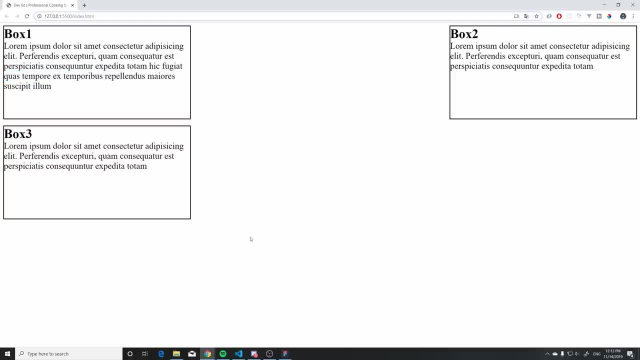 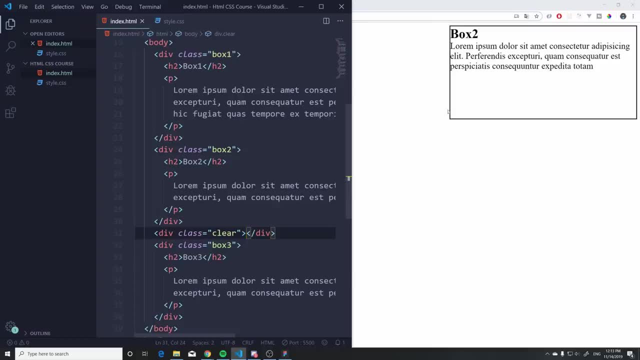 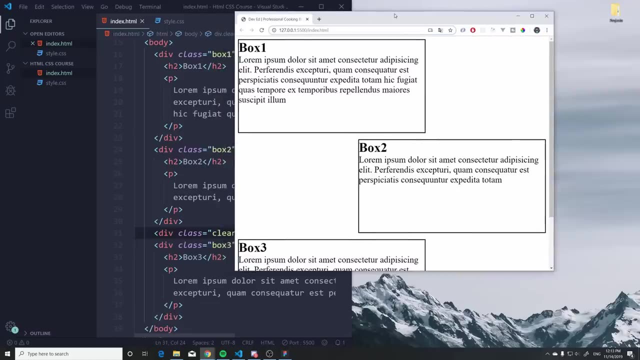 to do is just add, float left and float right to the elements and then clear, So the other content that you have does not break. Okay, but this is so weird And if we have something more complex, this can get tricky, And also making this responsive and nice can also be tricky, As you can see. as long as it. 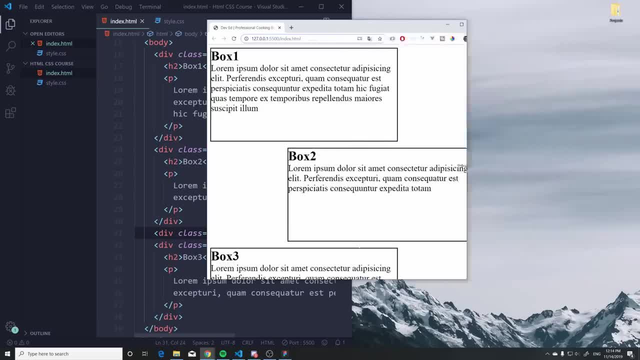 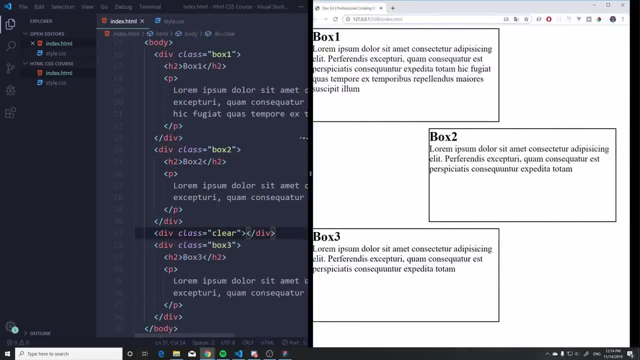 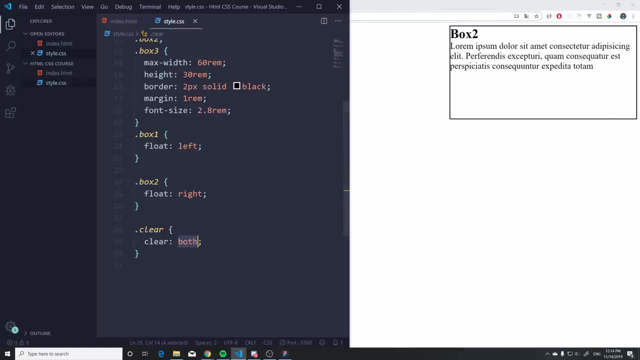 doesn't have space. it does jump down there, which is pretty good, But it's still not that great. All right, there we go, Super awesome. So now what I would want to do is maybe, maybe, change this and add- don't add this max width. maybe we can do 50%, 50%, width, 50%. Let's see what happens. 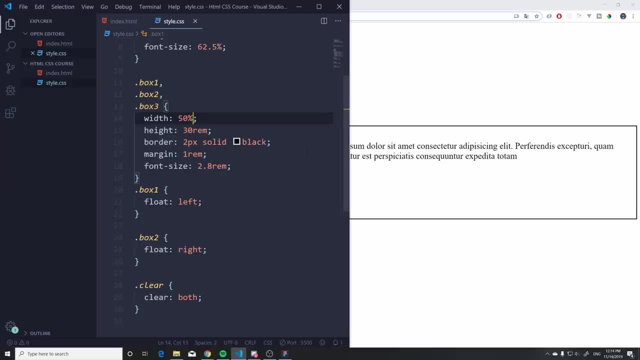 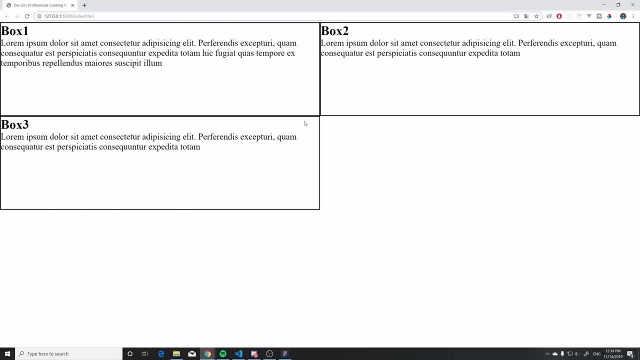 Okay, the content jumps down here, Because we also added- let's see, we also added some margins. So if we remove the margins now, it's perfectly stuck up there. So if you want to exactly split this up, then now you have to take into consideration, like how much space you want in here. So maybe I want 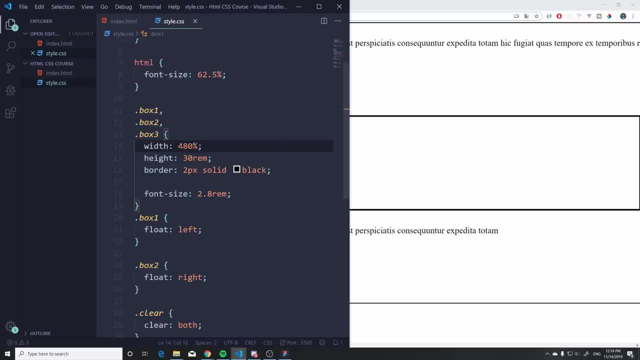 to do 48%, just to leave a bit of space hanging there like that, And then maybe we can add a bit of margin, So I can say margin of like 0.5%. All right, there we go. So we also have a bit of. 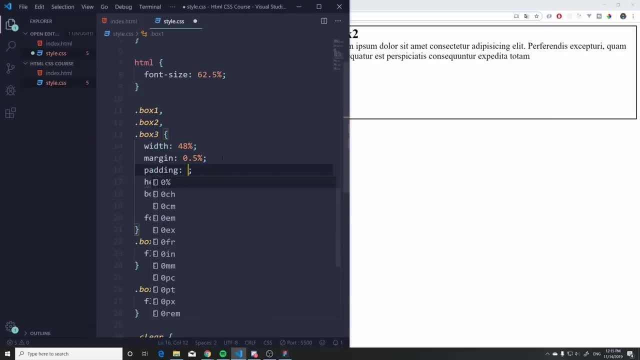 spacing And also in the boxes. maybe we can add a bit of a padding. Padding. let's do one rem, All right, so the are not stuck all the way up there, And then we can continue on with the box three. So maybe on 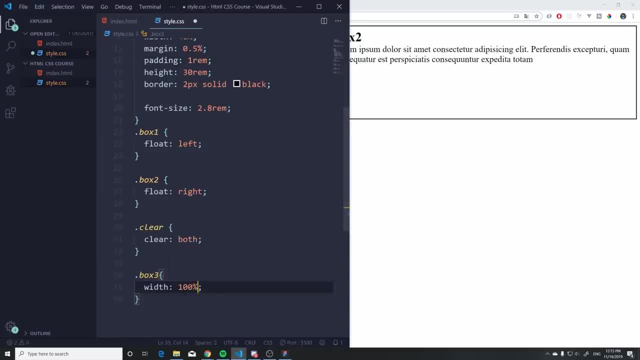 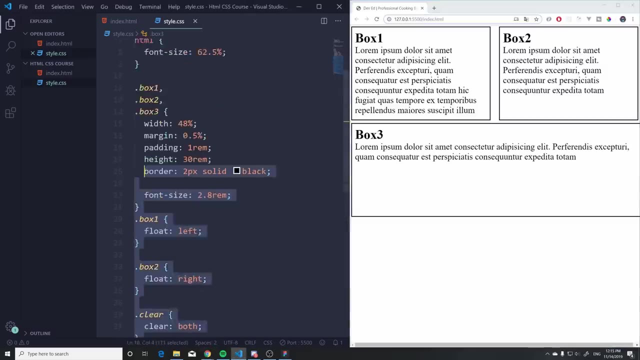 the box three. I want this to stretch all the way, So I can say width 100%, And now it stretches all the way. Okay, so now this is a way that you can create some layout. So let's throw together a simple page here just to experiment with this and and kind of mess around with this. So let's. 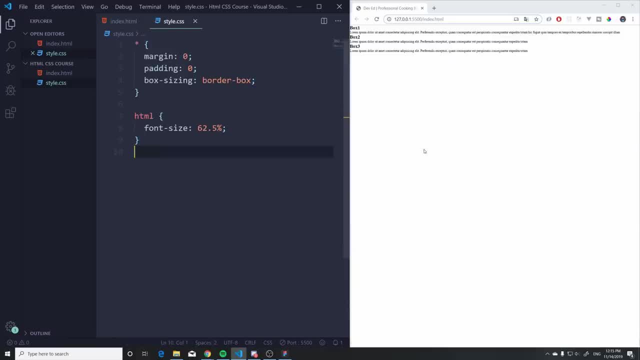 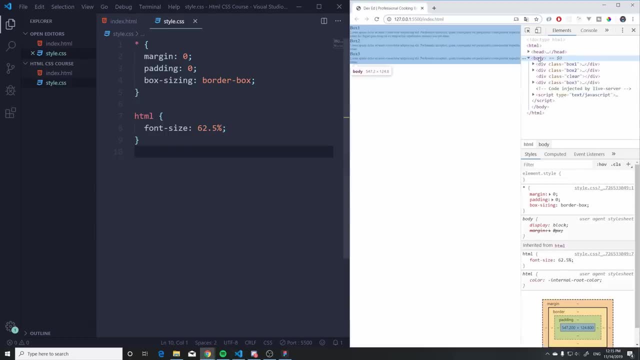 get rid of everything here. And another thing I want to show you is something with the height. So, by default, the HTML and the body tag are going to take the height of the content that you have. So, as you can see, it takes the height of the content that you have. So if you try to, 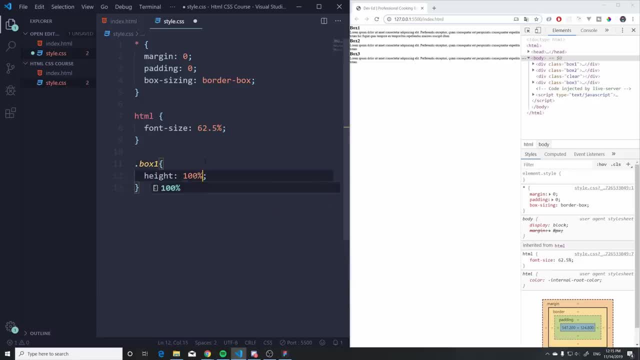 add, maybe on a box one. if you try to add a height of 100%, you're going to see that nothing happens. And the reason why nothing happens is because, well, it tries to take the height of the body, which already is the height of the content. So 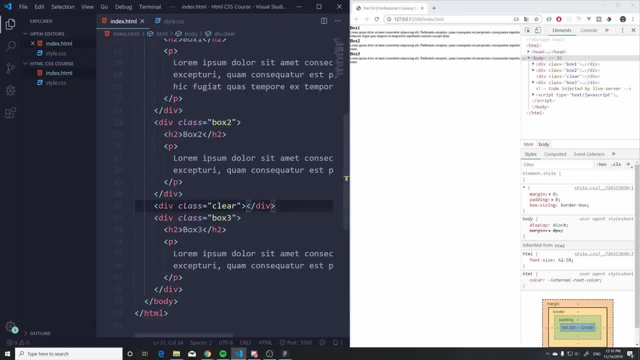 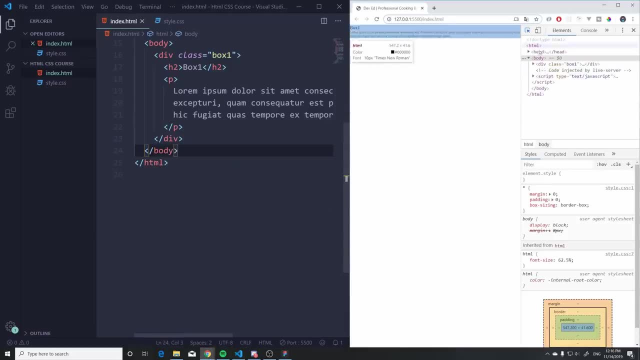 there is no height. There's no. what about height of content? nothing to stretch, right? so maybe we just have this. maybe let me just illustrate this a bit more clearly. maybe we just have this box one, right? so so if we take a look at the box one, height is just the height of the content. and if we 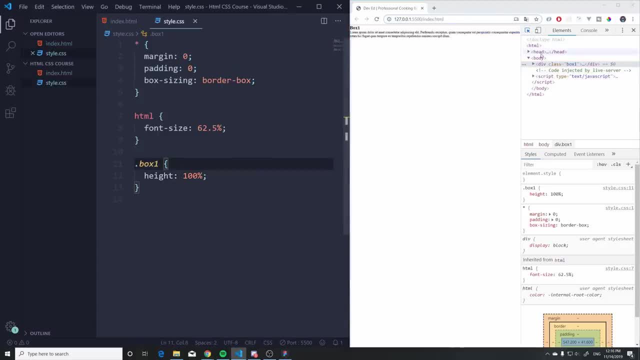 try to add height 100%, well that's not gonna do anything because the body site is already the size of the content, so it's like useless. so a way you can fix this is you can extend the HTML and the body's height so you can say HTML: body. 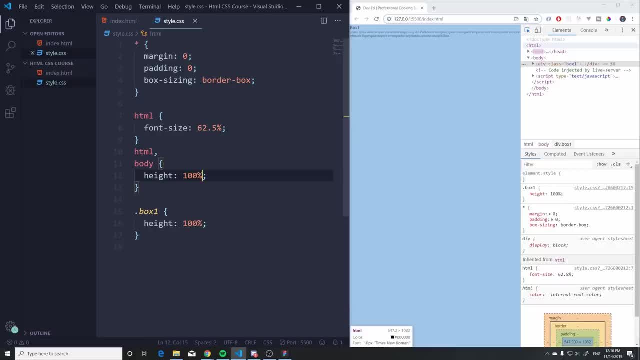 and you can set that, the height, 100%. and now, as you can see, the bodies and the HTML site extends all the way down right. so now on the box we also have a hundred percent, because we defined it here. so if I add 50 now it's gonna be 50% of the. 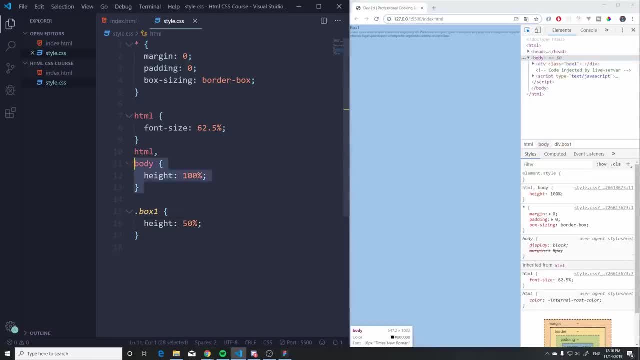 body's height. okay, so this is a quick hack that you can do, but we're gonna introduce some better methods that we can do this rather than adding HTML body 100%. but I want to clarify this as well, just for you to know. so let's remove everything. 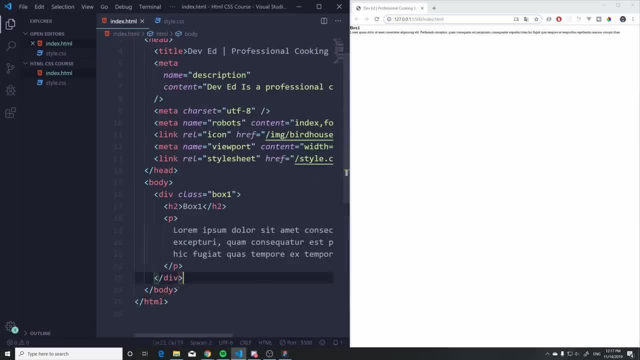 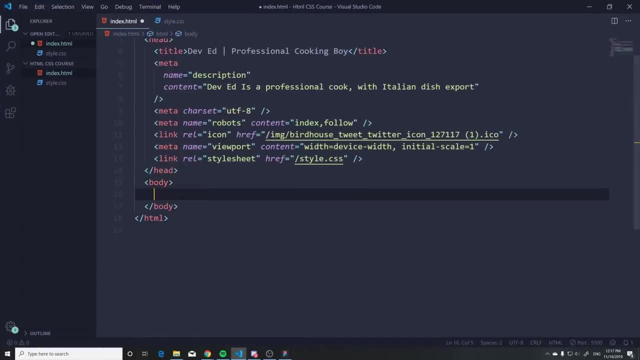 and let's start off building out something simple. so let's just throw together like a navigation that we might have. so I'm gonna full screen this, let's go down here and what I'm gonna do is just start off with a header, all right, and in this header we're gonna have a navigation. so we're gonna. 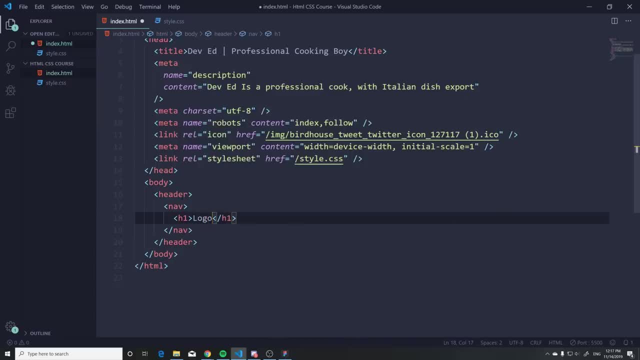 throw in a logo here, which is gonna be a H1 logo. now I'm also gonna give it an ID of logo. perfect. underneath we're gonna throw an unordered list and here we have our anchor tags. so, LIA, all right, just to keep the semantics correct. I'm gonna duplicate this two more times. I'm gonna. 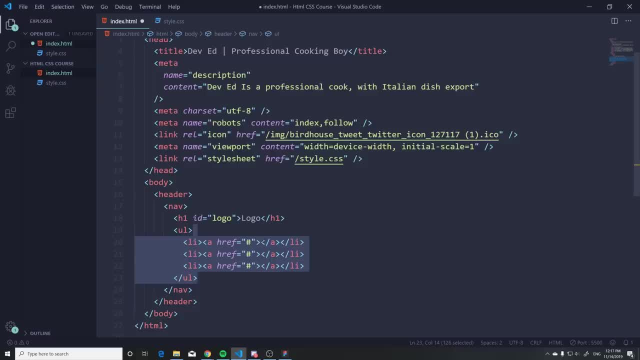 add the hashtag here and just so it doesn't actually bring us anywhere. okay, here we're gonna have home, this is gonna be about and this is gonna bemot about, and this is gonna be correct, dif vezes, And I need to use the image header. so, vize wise, it doesn't include the. So when you're basically doing that, authorities, can you change things? 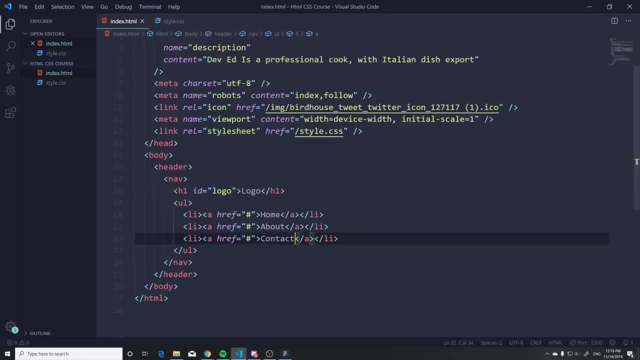 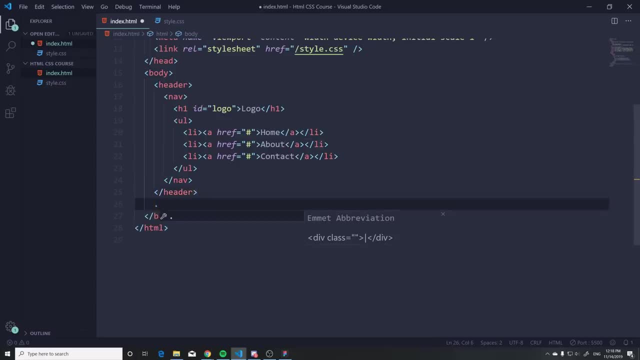 h, stri k in Bigeren, probably always knowing how to do it when you're not going to� contact Perfect. Okay, Underneath, let's do maybe a big image underneath, All right, Some sort of hero image. So we can create a section like this, And in this section we can also have a header. 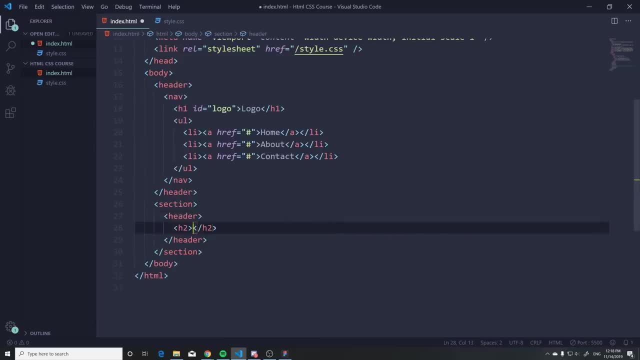 So we can say header, And here we can have a H2 that's going to say let's make it about some kind of cooking thing, Cooking, the cooking, the cooking master. All right, And underneath here let's throw a H3 that's going to say cooking. I don't know what I want to say. Buy our homemade. 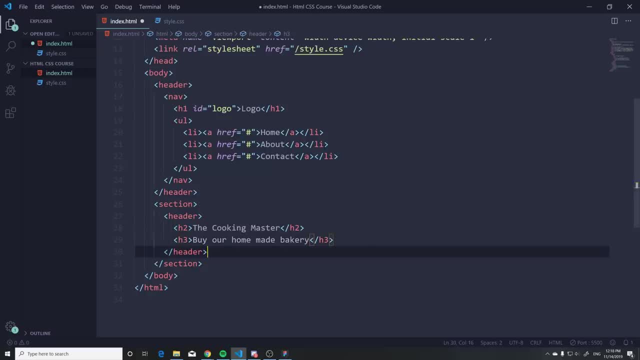 bakery. All right, And let's also. all right, that's going to be good. I'm happy with that, And we're going to keep this simple, like this, Perfect, And you know what? Let's actually get rid of the header And we're also going to throw a button underneath just to keep this a bit more. 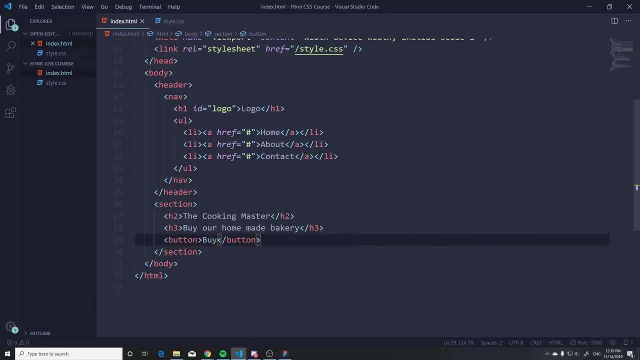 simple Button. We're going to say buy and hit save. I'm also going to add a class of hero to this, our hero section, And underneath let's do maybe a form, So we can do a section, And this is going to be called. 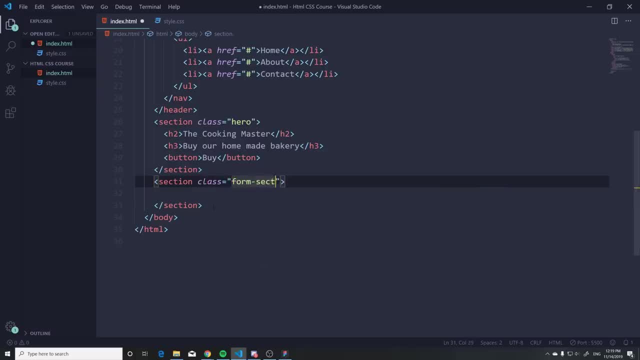 class. I'm going to add a class of form section to this. We can also do a hero section, just to keep everything consistent. and hit save, Okay. And this: I'm going to have a header that has a H2 and it's going to say contact us, Hit save, And underneath the header we are going to throw in 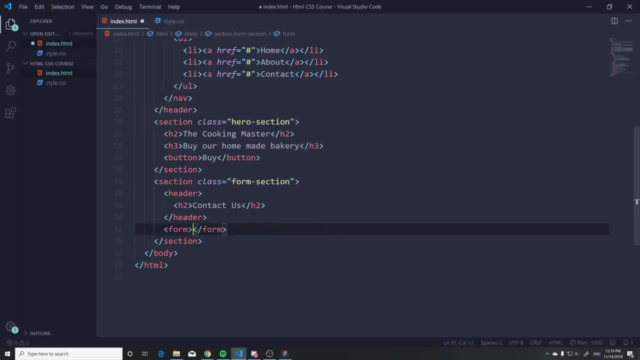 a form. I'm going to remove the action for now, because this is not really going to do anything, And here I'm just going to drop a label for name And after this let's write name in here. After this, we're going to also drop in an input with a type text. Perfect, So we can now duplicate this. 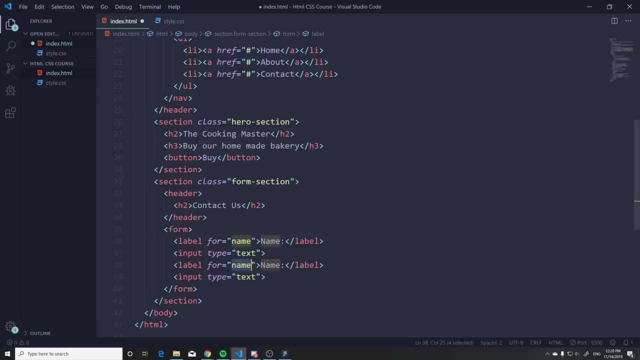 two more times like this. We can change this for email And we can say email And here we can input type email. That's good, And we can also add on these inputs. I forgot to add a name. that's going to say name On this one. 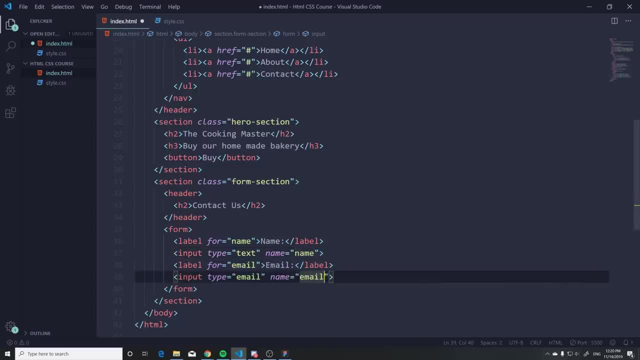 name is going to be email And let's also add an ID of name input, And here we can add an ID of email input. Perfect, Let's hit save on that. Everything is clear. And finally, maybe we have a label for email And here we can add an ID of email input, And here we can add an ID of email. 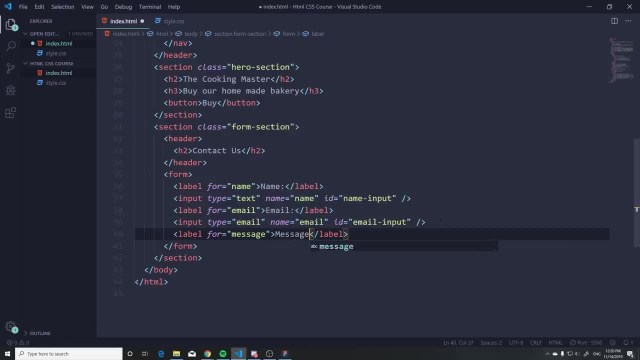 For a message Message, And this is going to be just a text area, Text area with a name of message, An ID of message. There we go, And actually we need to change these. here We're going to say for name input and for email input. Where is it For email input? All right, And we 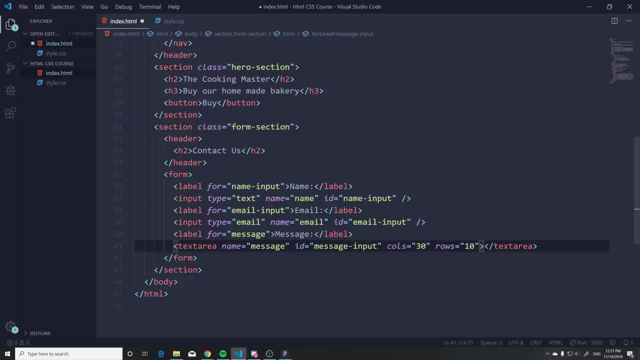 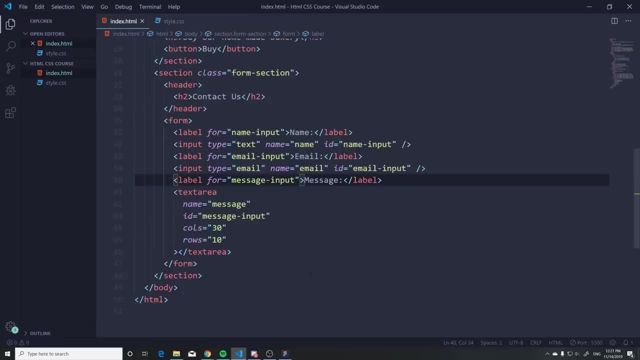 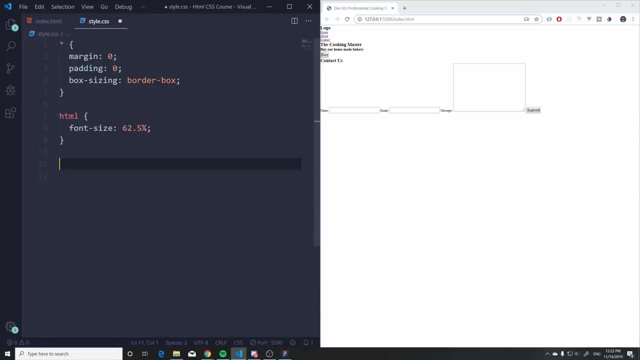 can do message input Here as well. Okay, Let's copy and paste. Lovely, Hit save. Okay, We have everything that we need. Okay, So take a look. This is what we have. Looks lovely. Let's go to our CSS. Let's remove the. 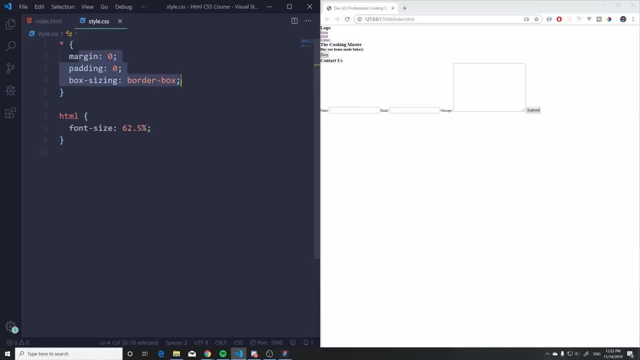 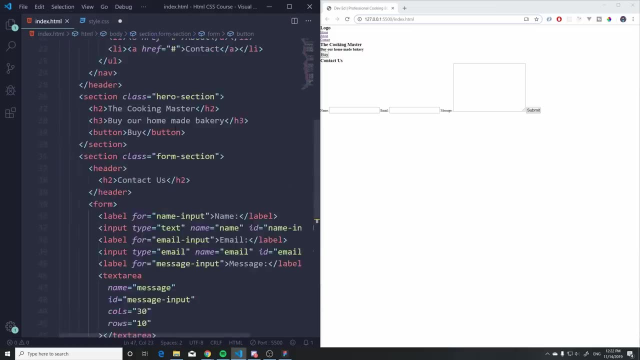 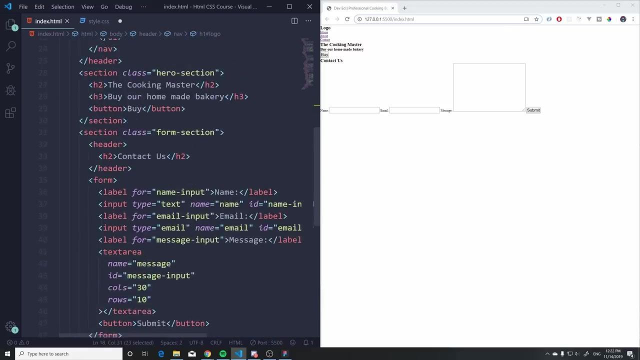 additional code And all I have here is just the margin padding and the box sizing and the font size on the HTML. Lovely, Okay. So let's start off, maybe, with doing some simple things, Maybe some global things That we can adjust, Such as the size of our H1, of our H2s, of our headings, And maybe anchor. 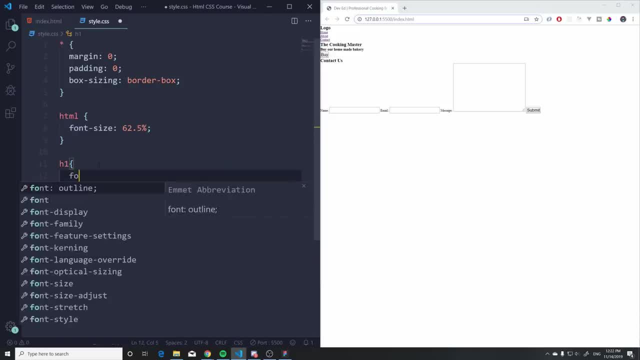 tags. So what we can do is take the H1,, add a font size of 2.8 rem, Hit save All. right, That's fine. Let's also get the H2 and the- just the H2.. This is going to be a font size of 4.5 rem All. 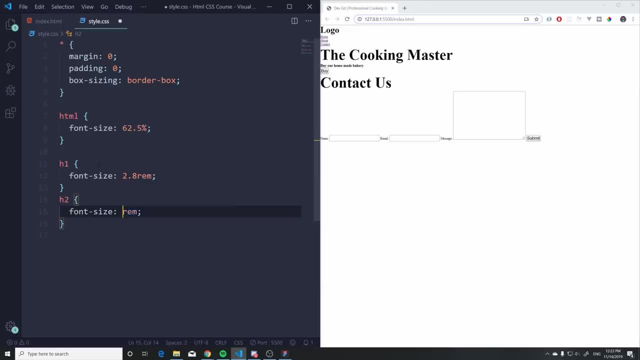 right, These are going to be the big sections on our page. Maybe smaller, 3.6 is going to be fine. Okay, There we go. I also want to add a bit of a padding to these. Let's do 5 rem top and bottom, Maybe 3. And 0 rem left and right. Okay, Just to space them. 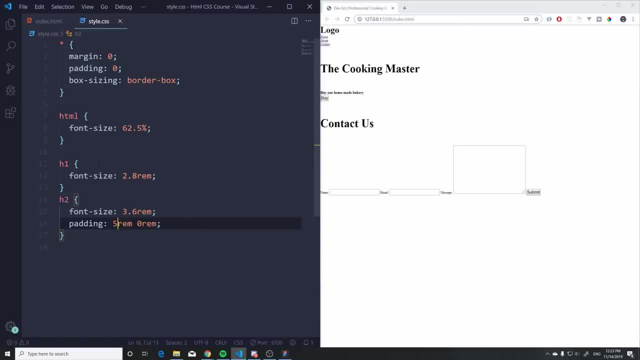 out now, Let's do 5. Save, Okay, Perfect, So let's kind of focus on this one first. On the upper corner, Let's also add an li here, So we remove some basic stylings. Actually we. 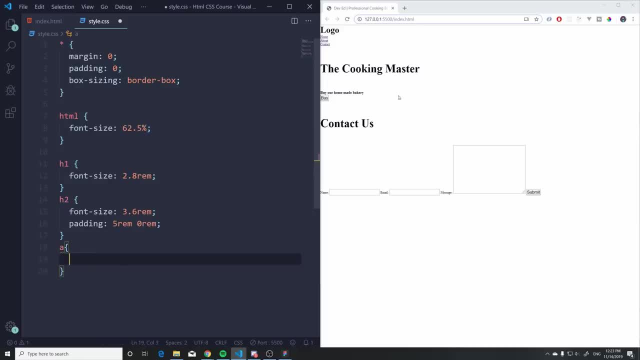 we can grab the A tag here, because if you try to change the color of this, it's not gonna work. If I say LI and add the color of red, nothing's gonna happen. So we specifically need to change the anchor tag, because that's what gives the color to these, not the LI. 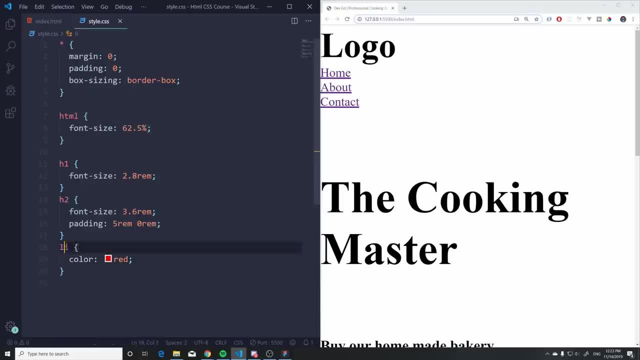 So these are laid inside the A tag, but to change them we specifically need to select that. So let's add a color of black to this and we might change this if we want, And let's remove the text decoration and we say none. 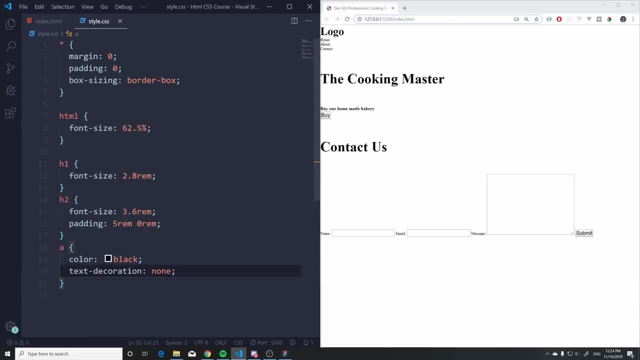 and that's gonna remove the underline there. Okay, let's also change the font size. Let's do 2.4 rem. let's see That's good. all right, I'm happy with that. Let's zoom out, Okay, and I also wanna. okay. so that's kind of it for now. 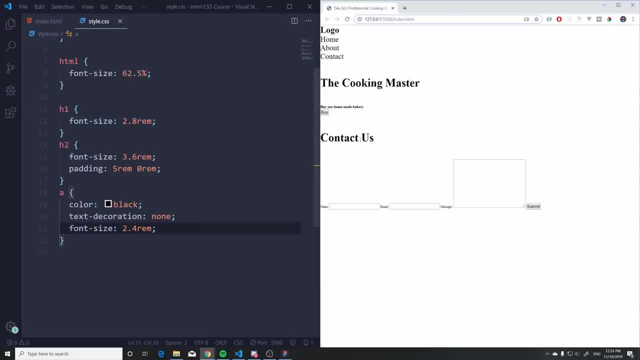 And is there something else? The H3,. we can change that too. So let's do H3,. let's give this a font size of 2.8 rem. That's good. And also the button. we give this a font size of 1.8 rem. 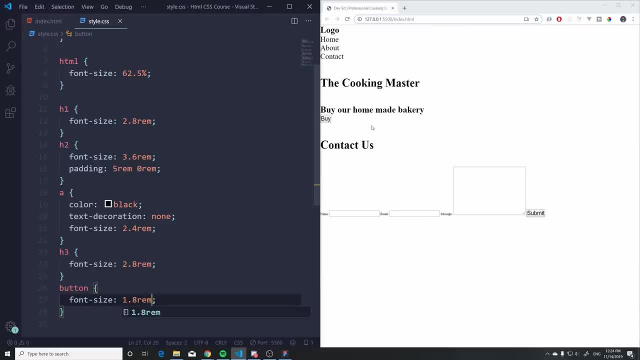 Hit save. Okay, so that's good. Now what I wanna do is start making this nav. So I'm gonna go all the way down here and I'm gonna select my nav. I'm gonna throw a background color on it. Let's do, let's just pick out something here. 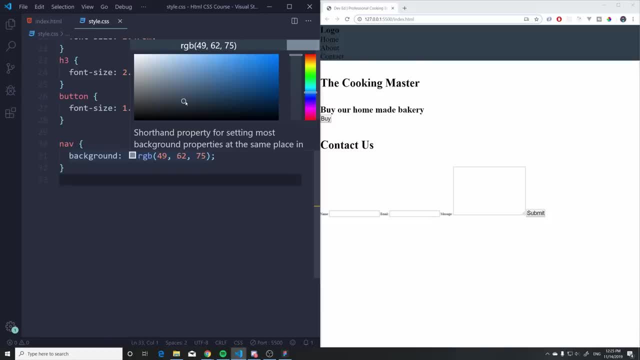 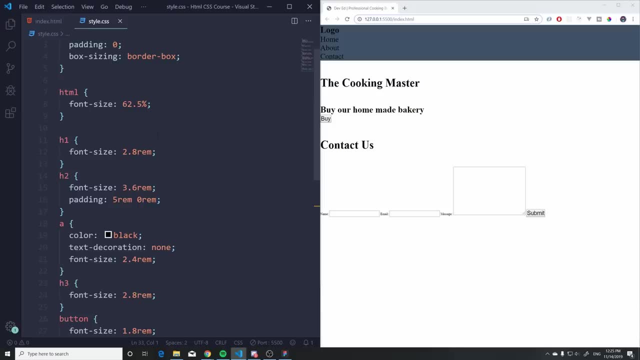 Shall we go dark? Let's go dark, Let's go blueish. dark color here, All right, something like this. Okay, and now what I wanna do is actually change the color of these So I can say color white, because that's kind of hard to see. 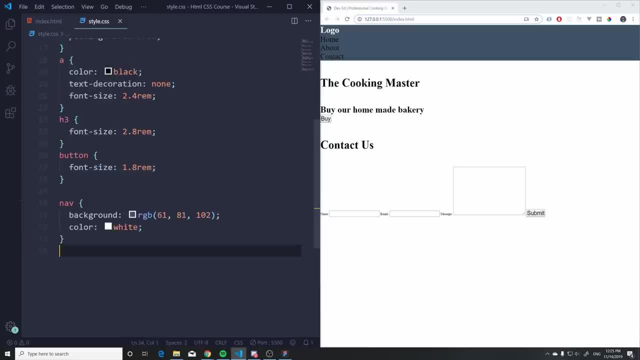 Okay, and, as you can see, we also specifically need to change it on our anchor tags. So I'm gonna actually go up here and change this to white. Now I'm changing everything, so all the anchor tags to white, So if I have any other one, 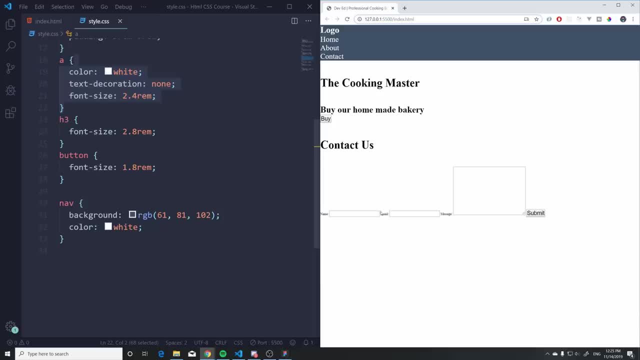 those are gonna be white too, And if I have it on the white background, you cannot see it. So in case you wanna add additional ones and you cannot see it, don't panic, It's because we globally changed it up here, Okay, so if you remember, 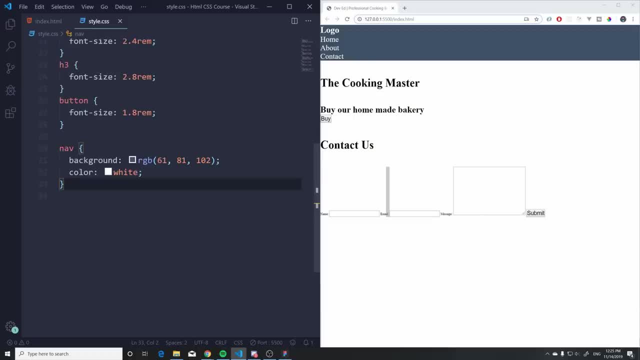 how we can move these is by using floats. So I can go down here, I can select nav H1, and I can say float left, because I want this to be on the left side. Okay, now this kind of moves in a weird way here. 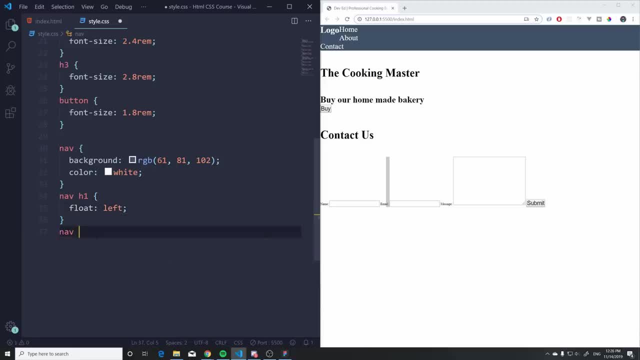 So what I wanna do is say: nav, and I'm gonna select the UL, and I wanna float that right. All right, and now this breaks our height. so everything collapses in a weird way, But, as you can see, it's kind of in the perfect position that we want it to be. 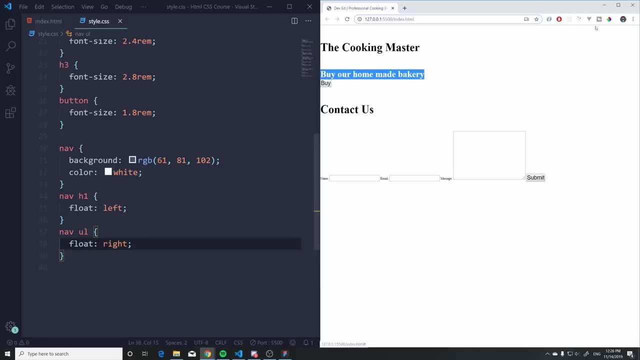 So, if I can drag this over, you're gonna see that we have the home there and we have the logo, So the position is good, but it broke our height. So if you remember, we can go up here and just add a clear. 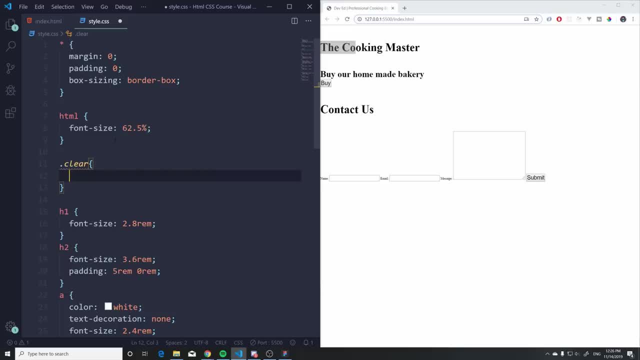 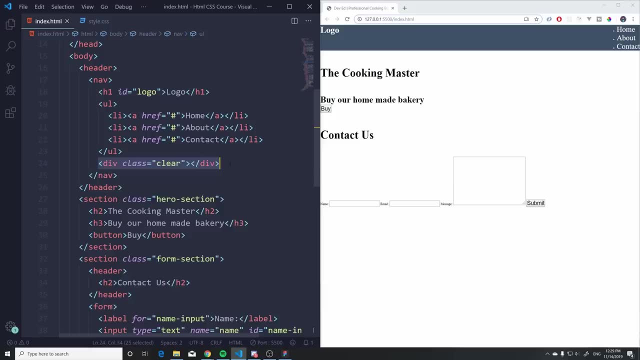 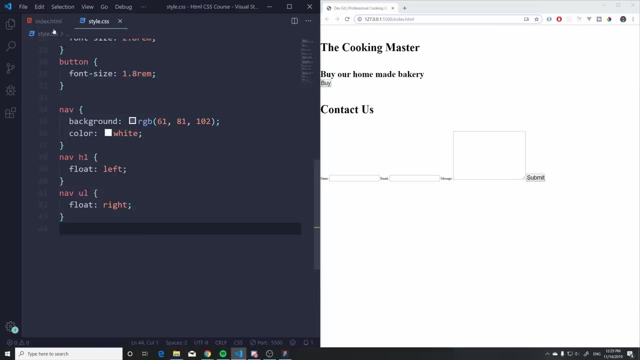 So the class and we can say clear both In our HTML. we can just add this class of clear right underneath here, So right underneath where you are finished with your floats. So I added the H1, the UL and right after that we add the clear. 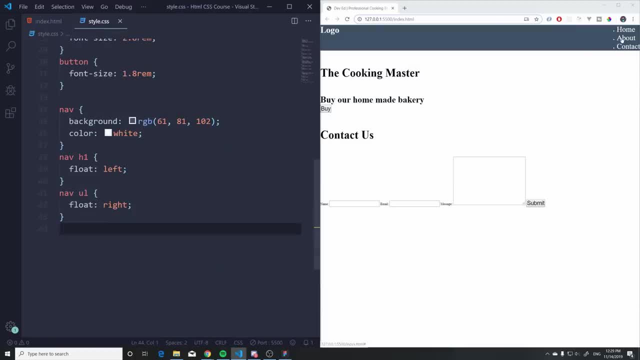 Okay and boom. everything works the same way. Now, as you can see, our LI tags here are also in a block style, and I want them to be. I want them to be in a block style and I want them to be in a block style. 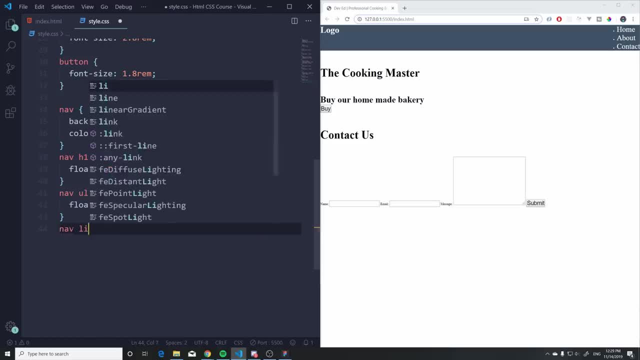 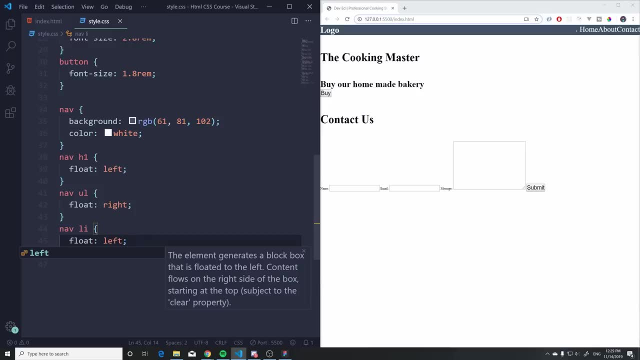 and I want them to be one next to each other, So we can also grab that nav LI and we can float those as well. Let's add a float to the left and boom, there we go, We have one next to each other. 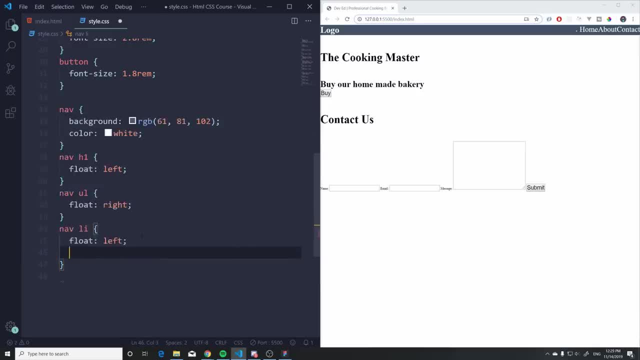 We can add some margins to them, or our paddings. Let's add a little margin here, and we're only gonna do it left and right. So the first one's gonna be zero and the second one is gonna be three, or we can do four. 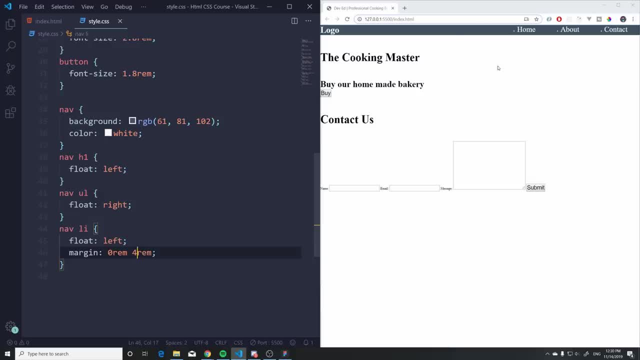 There we go. I also wanna remove those dots underneath. I don't want those. So what we can do is, on the UL we can say list style and we can say none, and that's gonna get rid of it, Perfect. 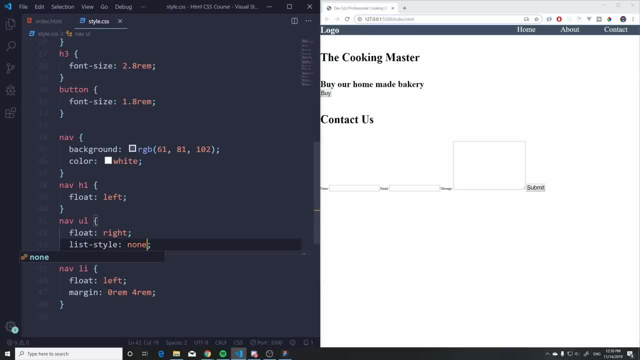 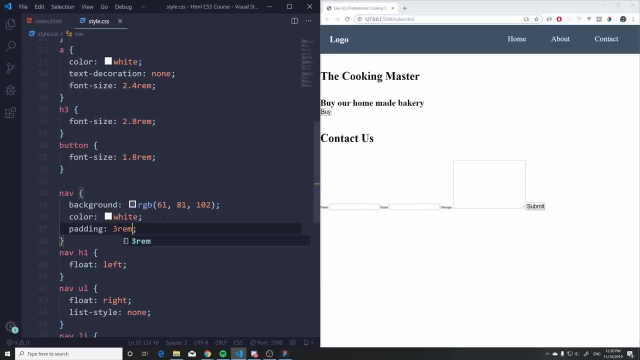 So now I can maybe add a bit of space in between these so I can go up here to the nav and add some padding to this. We can do three rem, all right, So that adds some padding all the way across here. Okay, so there we go. 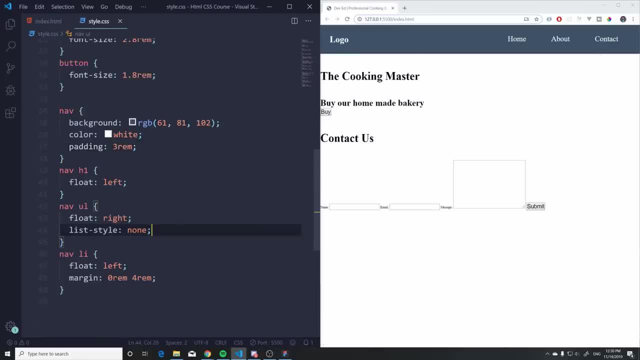 That's a simple way that you can create a nav, and that's a simple way that you can create a nav, and that's a simple way that you can create a nav. is this the right way? I have better methods to show you. 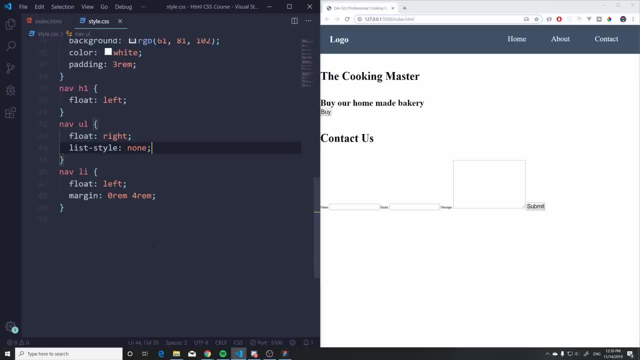 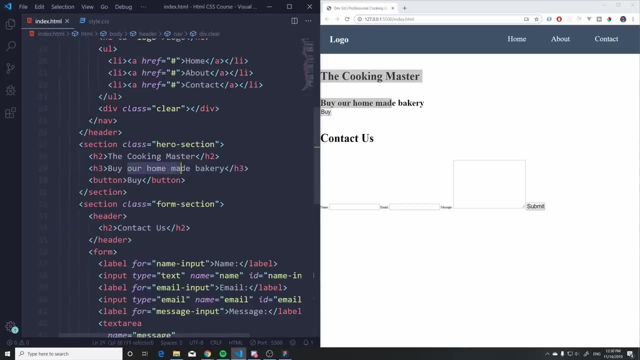 after we finish this section. This is a pain, to be honest, but hey, let's continue, why not? So we have this section here now with the hero, this one. Okay, so what we can do is get that hero section. 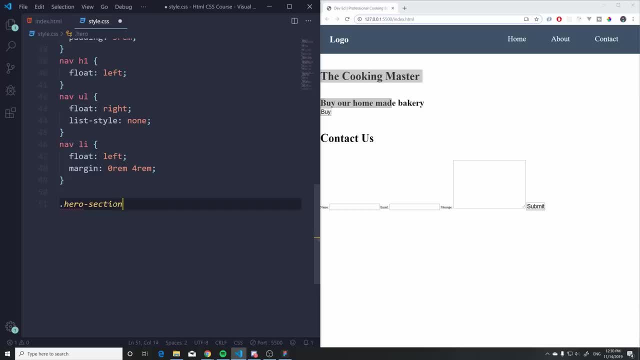 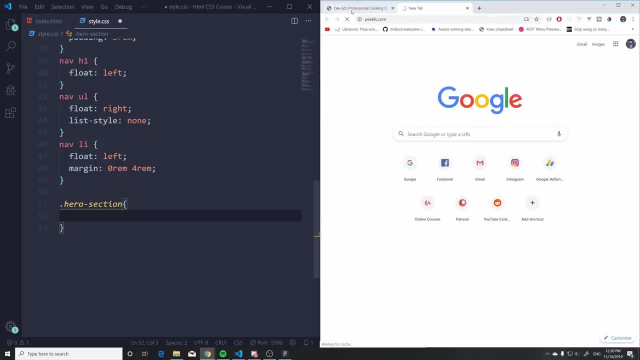 and let's get an image- hero section- and what I wanna do is add a background image to this. How can I add a background image? Well, let's go and explore and find an image. Let's go on Pexels. I'm gonna open the file here. 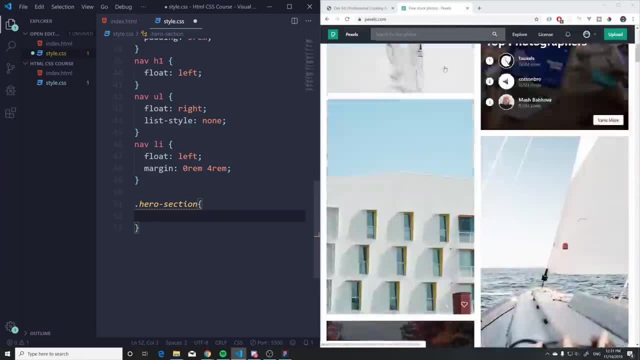 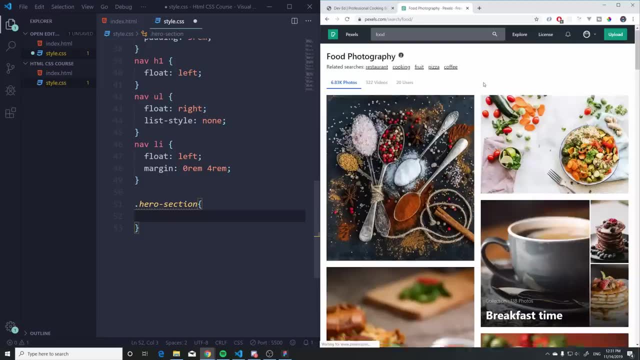 and hopefully the internet works today. Let's do something with food bakery. Let's search. Let's search. Pexels is slow today. There we go. Let's scroll down here. Maybe we can use this one, okay, So let's get this one. 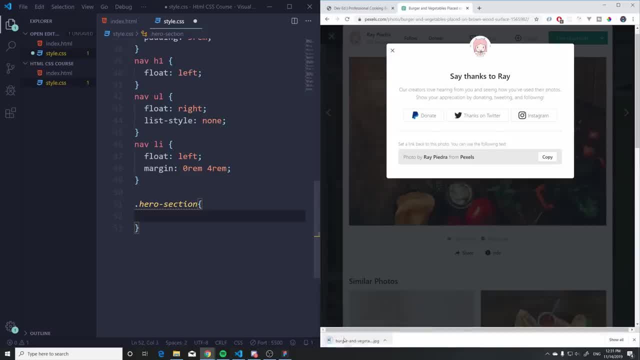 We can do the large. That's fine. Hit download and I'm just gonna drop it in here for now. Now you can create folders to make a background, to make everything nice, but for now it's gonna be fine. 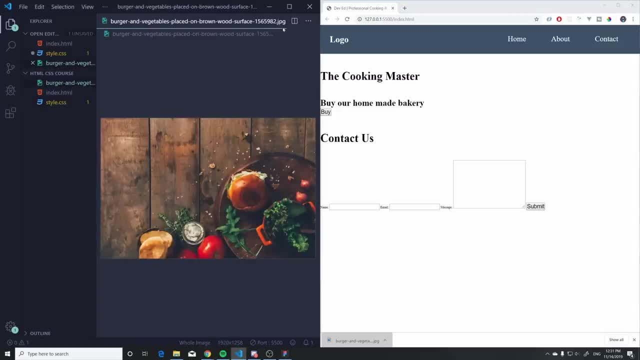 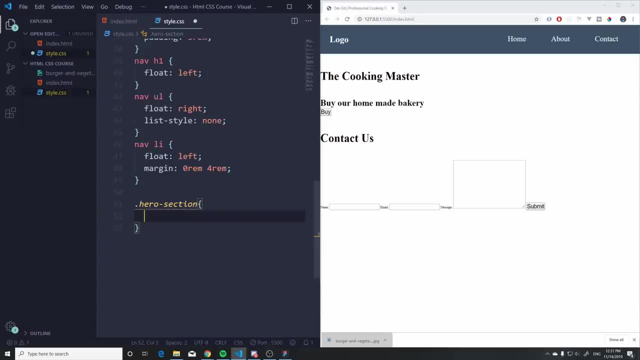 Okay, we can go back to our CSS. Can I close this? Do I have enough space? Okay, nevermind, No, close, There we go. So to add a background image, all we have to do. let me make more space here. 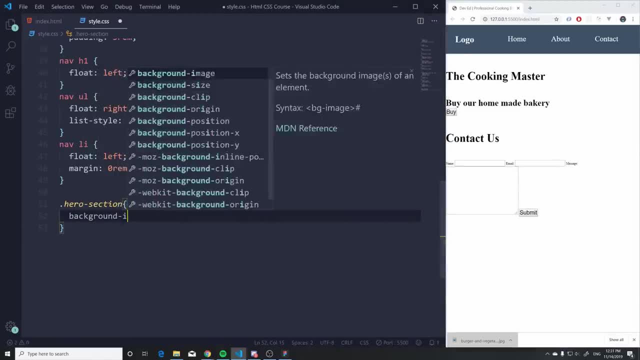 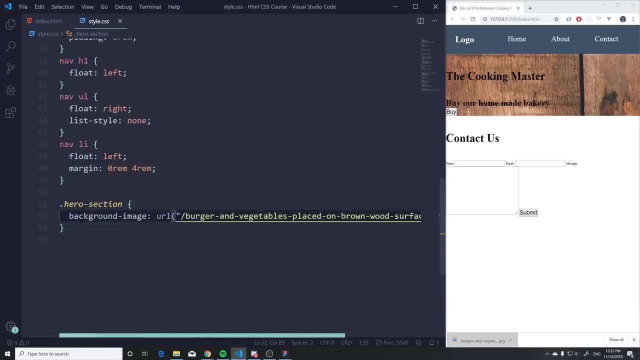 all we have to do is say background-image, and here we can say URL and add some quotes and we can drop in the image Burger vegetables. There we go. Take a look, We have the background image. Perfect. That's exactly what I want. 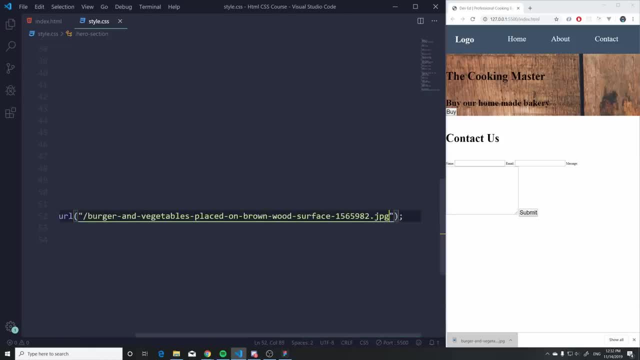 However, this is kind of small, so we can increase the height of this if we want. So let's go here and just add a random height. Let's do 30 rem. Let's see. Okay, that's still too small. 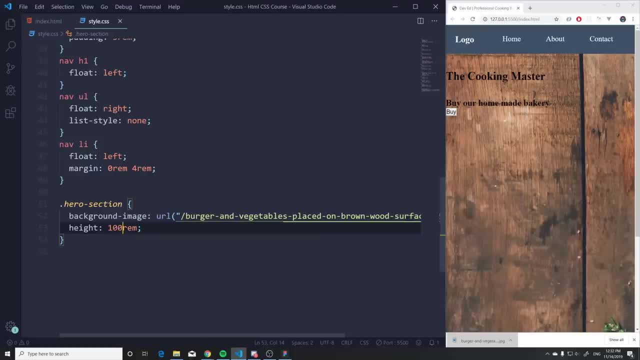 Let's do like 100 rem, Rem, rem. Okay, so something large like this: Eh 80.. There we go. I don't want this to cover everything, So perfect. So we have this, but, as you can see, this doesn't look that great. 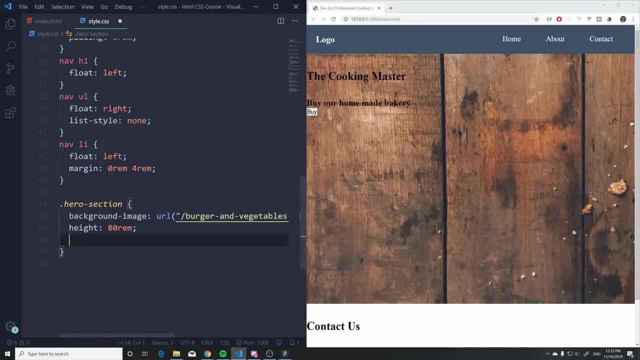 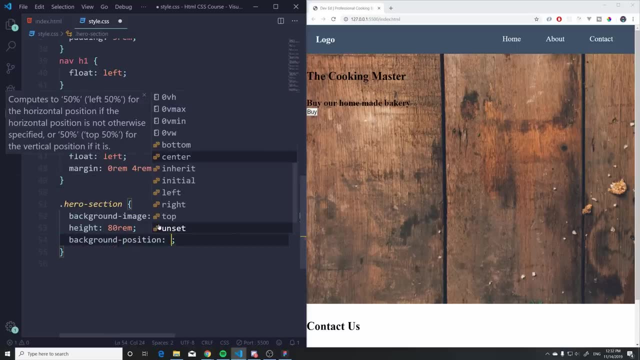 So a way you can change that is by adding a background position. If we change the background position we can move the image up, left, right or bottom. So if I say top, it's gonna move it to the top of the image. 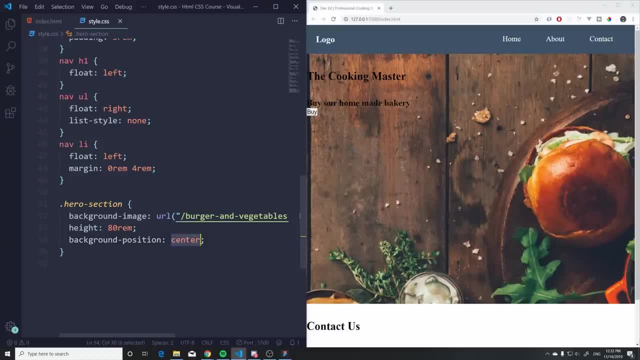 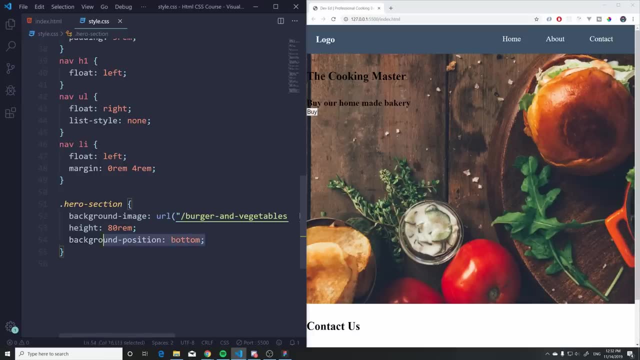 If I say center, it's gonna drop it in the center, and if I say bottom, it's gonna go all the way down. Okay, but this still doesn't look that great. So what we can also do is let me remove this. 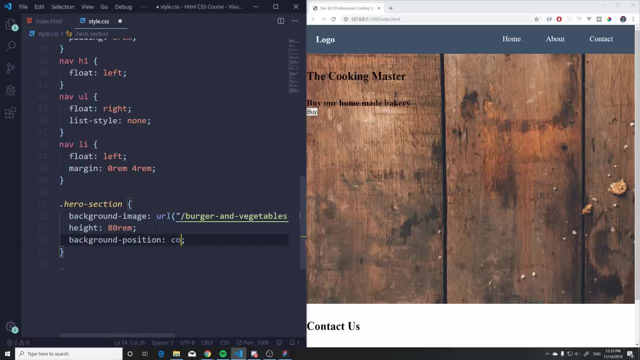 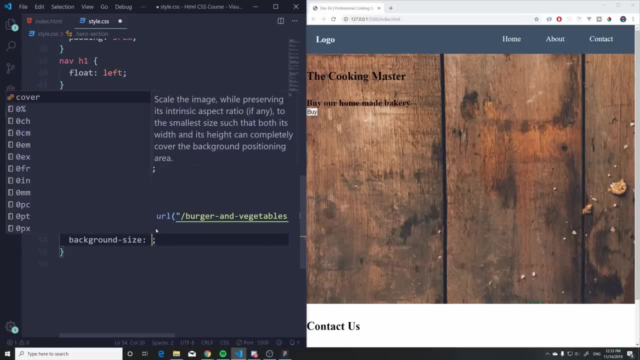 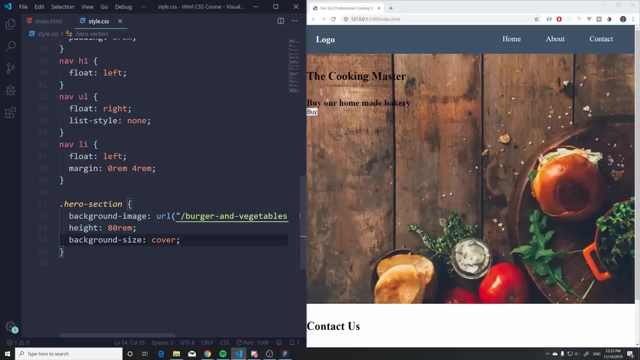 is: add a background position, Not background position- my apologies- Background size and we can modify this as well. If we add cover, you're gonna see that it says scale the image while preserving its intrinsic aspect ratio. So if we add this, as you can see, 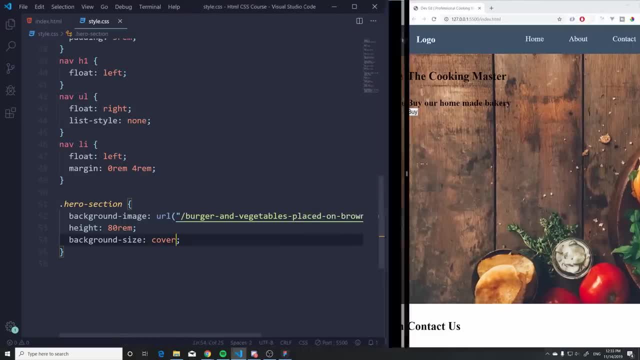 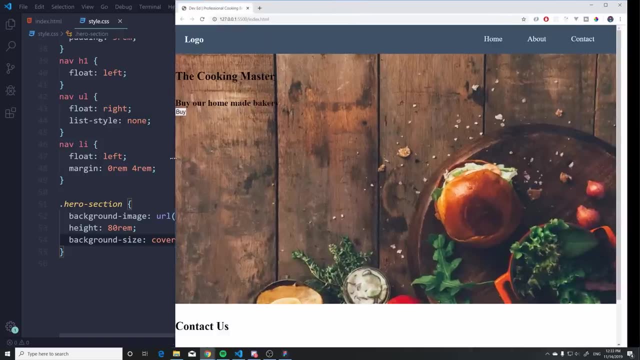 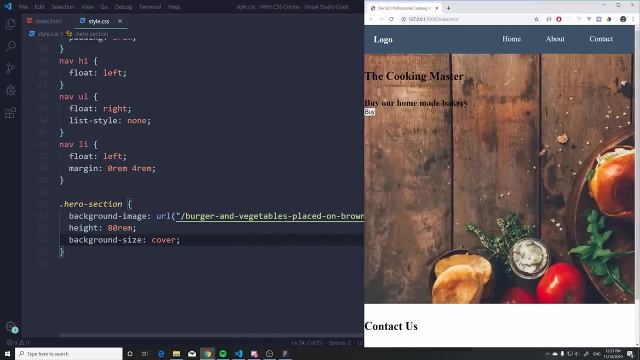 we see most of the image and when we scale it down, you're gonna see that it scales and it keeps the aspect ratio All right. so that's a good step. right there, We can also change the position if we want. 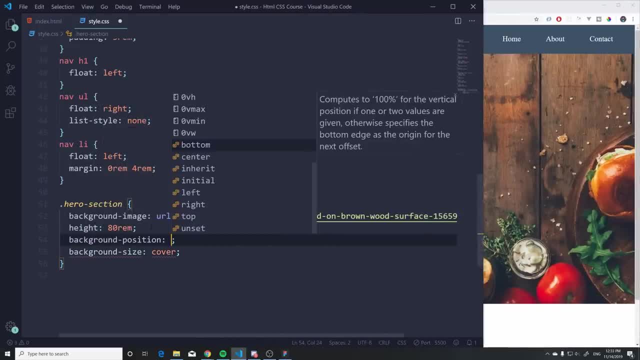 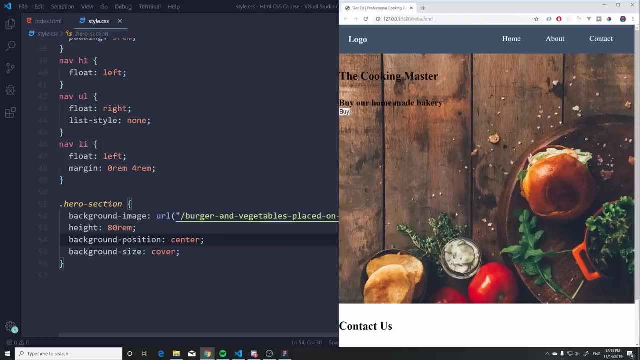 Maybe center background position and say center. Okay, let's see how that looks. Okay, I'm kind of happy with that because I wanna see the burger and these chips, so that's good. Okay, so we have that. 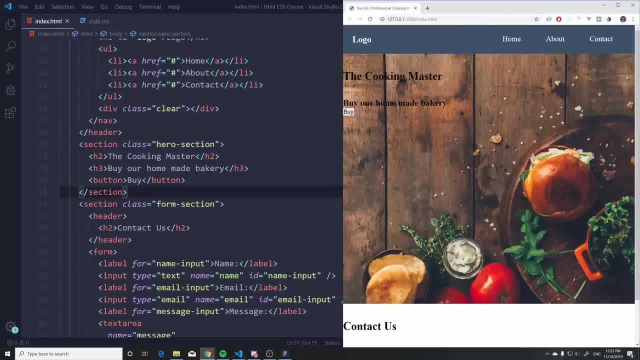 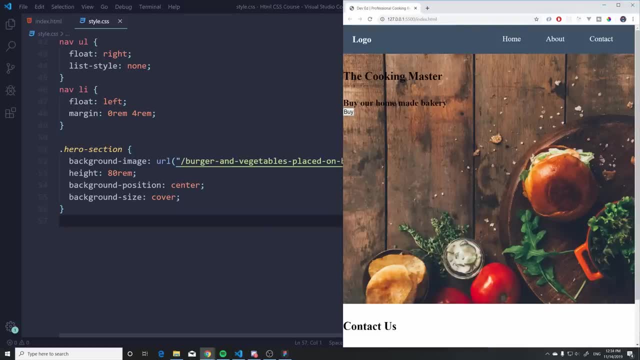 Now what we can do actually is we can just align everything here to the middle. So how can we align everything to the middle? What we can do is go here and just say text align, and we can say center, and, as you can see, 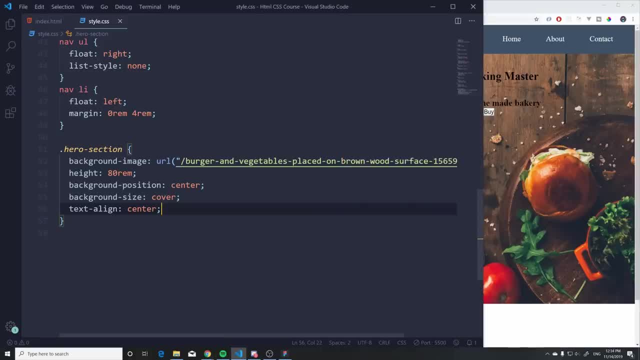 that drops it perfectly in the center. We can push down the content. Let's just change the color to white for now, like that- and let's drop it to the center. So what we can do is add a padding top of text. 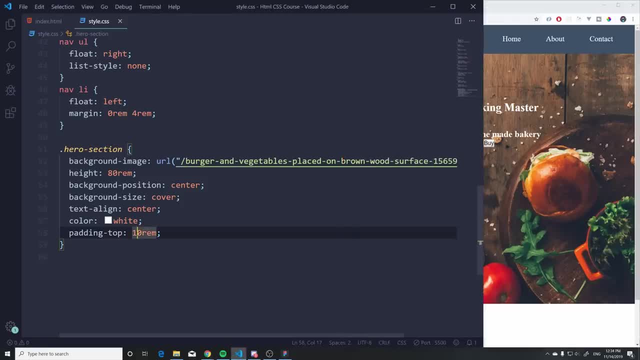 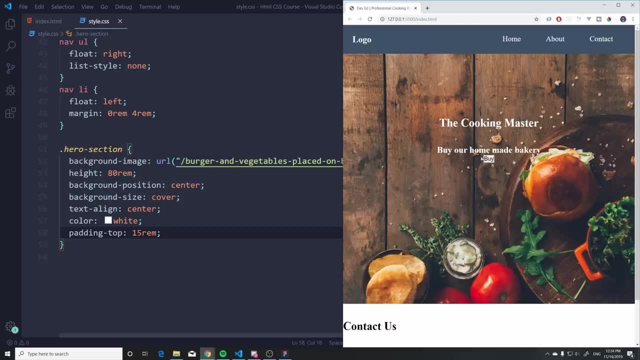 And then hit save, that drops it down. here We can drop it more, Let's say 15, perfect, Okay, so what I can also do is style this a bit nicer, because it doesn't look that good And also, you know, it's kind of hard to see the white. 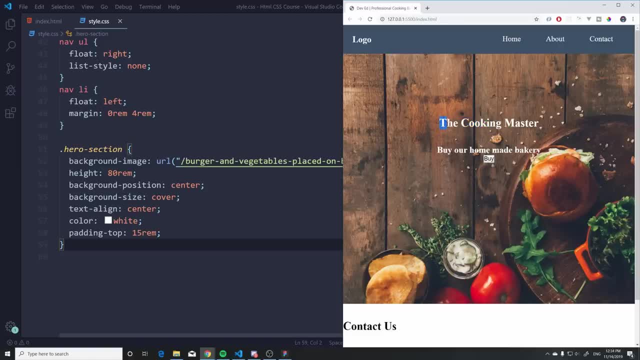 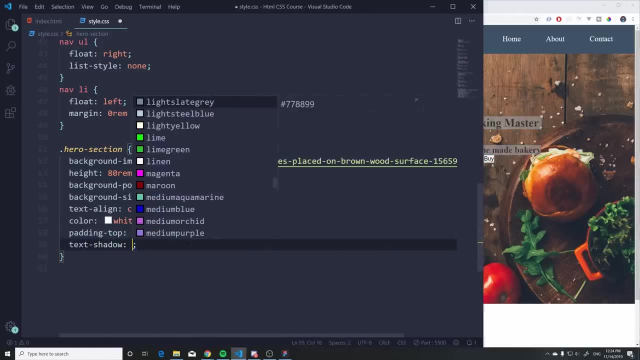 especially if you have something a bit lighter color, It's gonna be way more difficult for you to see this. So one thing that you can do is add a text shadow, and by adding a text shadow, this takes three parameters. It's gonna say three pixels, three pixels, three pixels. 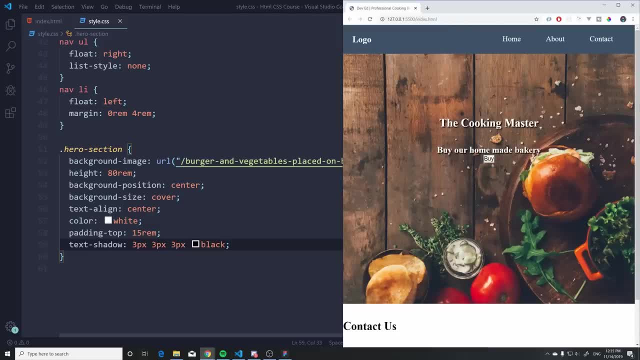 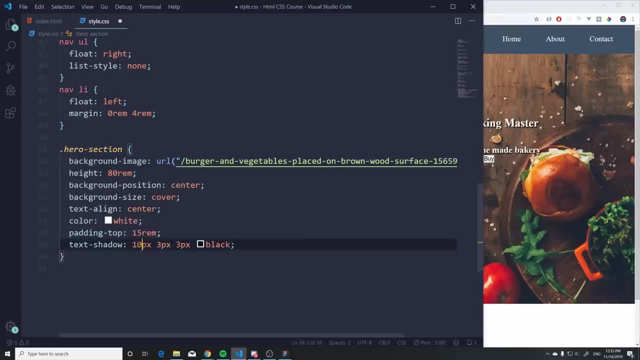 and a color. I'm gonna say black and I'm gonna explain everything. So the first one, and the second one is gonna be the position of it. So if I change this to 10,, as you can see, it moves it 10 pixels to the right. 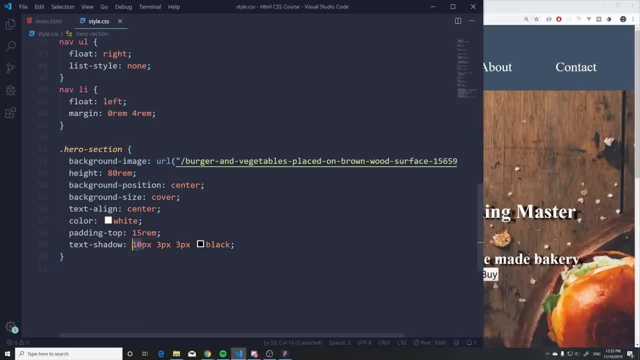 So the shadow now is to the right. Now I don't want this to be as large, so I'm gonna keep it three. so it's quite close to the white one, so it gives that nice contrast. This works in y-axis, so if I add 10 here, 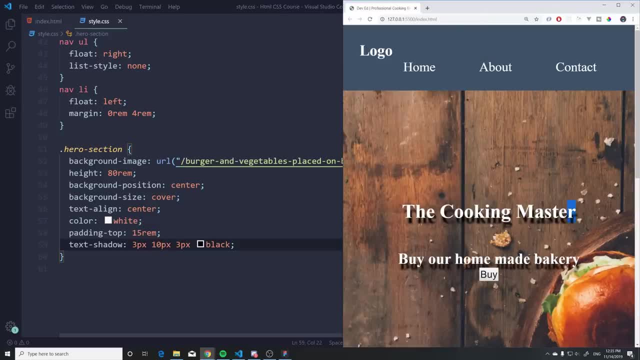 it's gonna move it down this way and minus is gonna move it up that way, okay, So I'm gonna keep it fairly close with three pixels and this property is gonna increase basically the radius of the blur, So if I add something big like 10,. 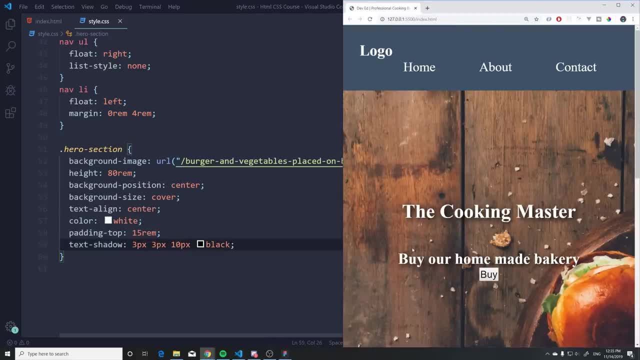 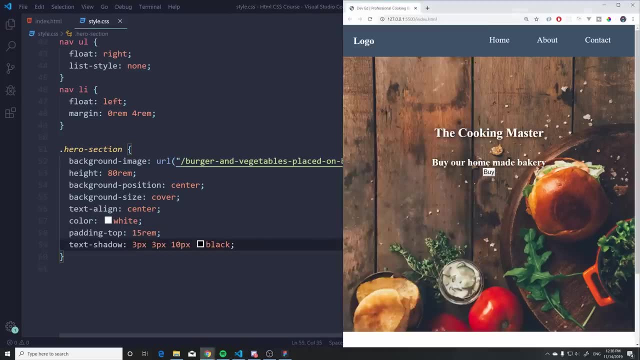 it's gonna get more and more blurry, so it's not that sharp looking. This is fine. I think it's pretty good. compared to this, This is a bit harder to read. next to this, This kinda comes out a bit more, so that's good. 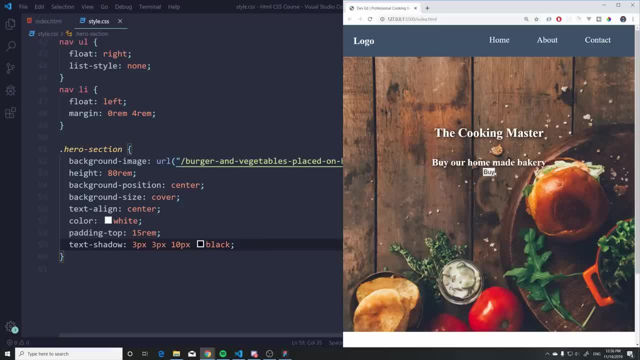 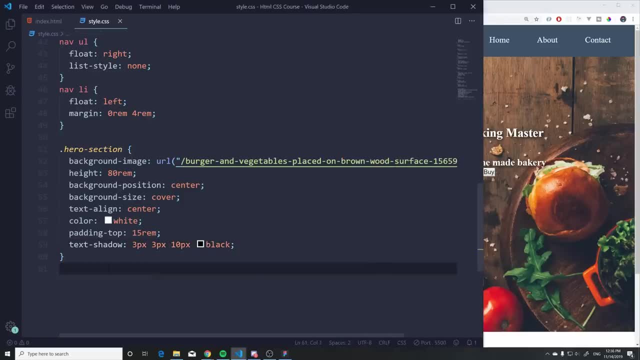 Next up. what I wanna do is I wanna maybe push this button down a bit and style it a bit nicer. So what I'm gonna do is go to hero section and I'm gonna say: button okay. And this one is gonna have a padding of: let's do. 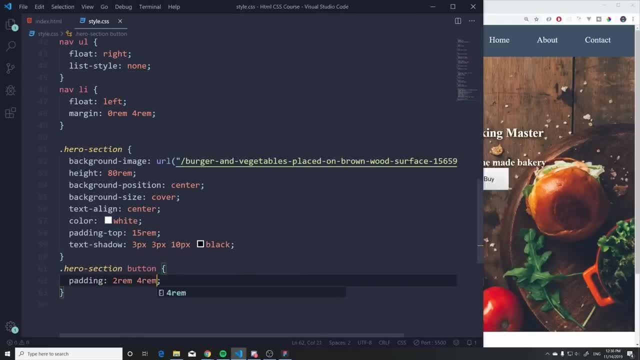 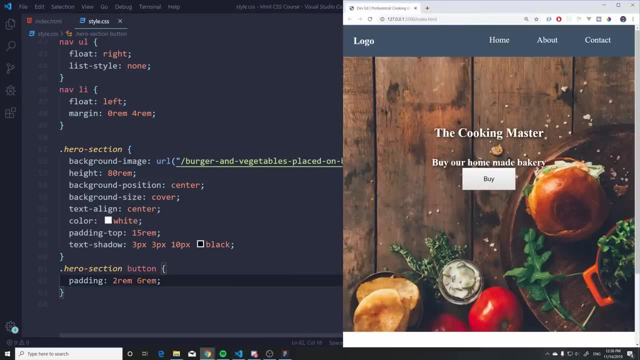 two rem and four rem. Hit, save. there we go. that's what we have. Maybe we can make this larger, like six. so it's a bit wider. Let's do four, or maybe four and one. All right, I don't want it extremely large. 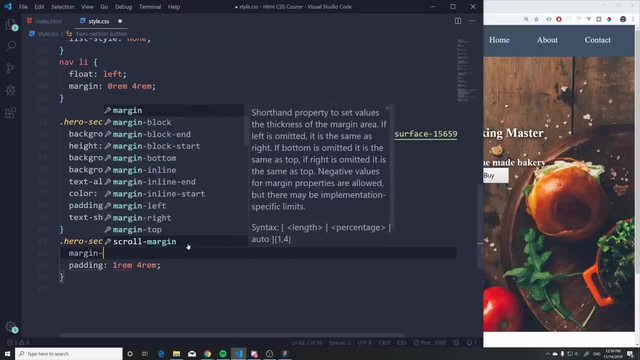 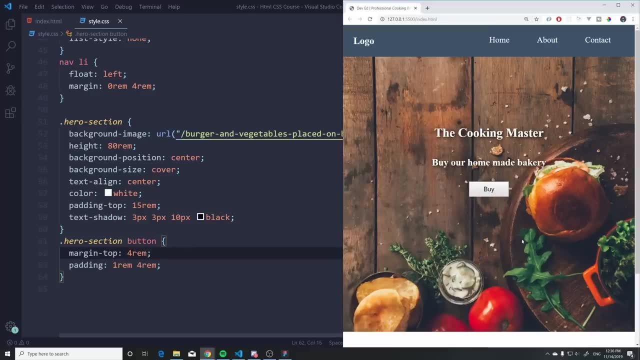 And that's good. And we can also add a margin top here of one rem. All right, maybe more three or four. There we go, Just to give it a bit more depth, More space. Let's remove the background. We can add this background that we had up here. 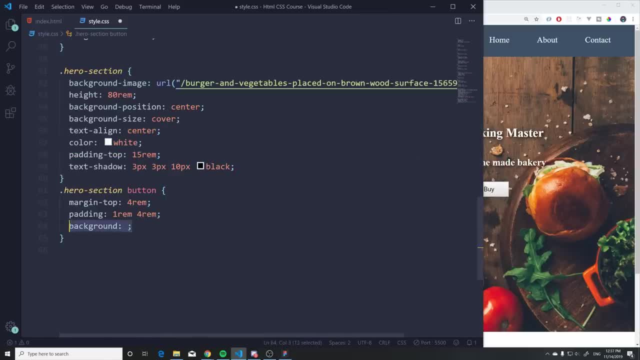 just to kind of match the design. So I'm gonna copy it from up there to here And we're gonna remove the border. We're gonna say border none. to get rid of the ugly border, We're gonna change the color of it to white. 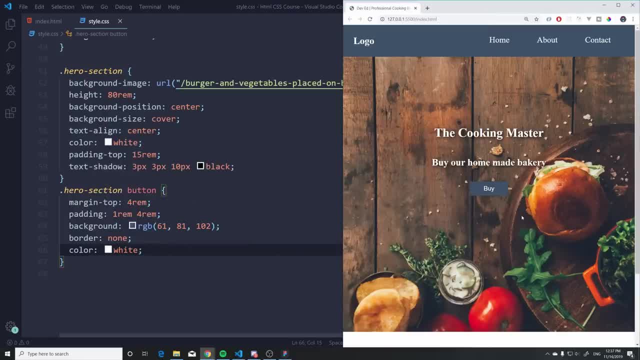 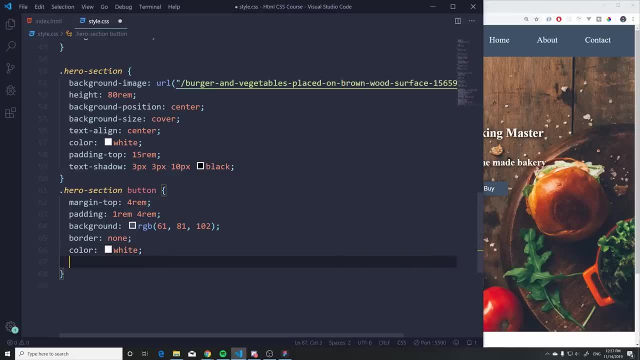 so we can see the text Perfect. And lastly, what I wanna do now, as you can see, this kinda blends with the background, So that's not that great. Let's change the cursor to pointer. So what you wanna do is have a pretty nice contrast. 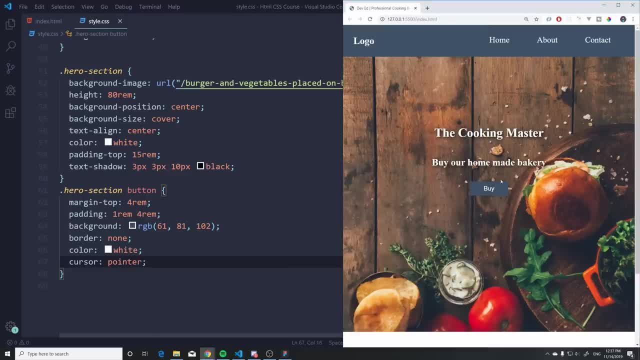 in between these- the image and the button here. So one thing you can do is either change the color of this or maybe add an image that's not so dark, Cause if I change this to something more like this now, it's more visible. 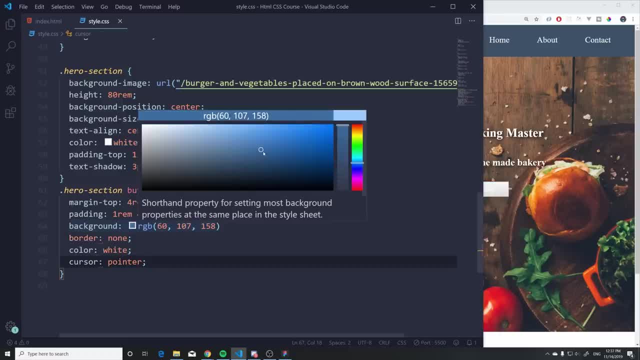 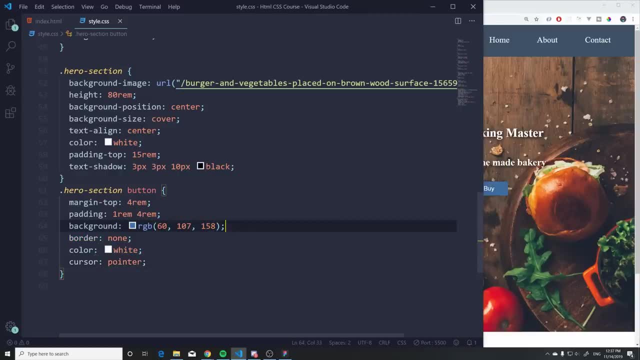 And you know what. We can actually add a custom one here. What am I changing? All right, let me go back here. I forgot the semi-colon, So it broke all my code. Maybe we can do something more visible like this: 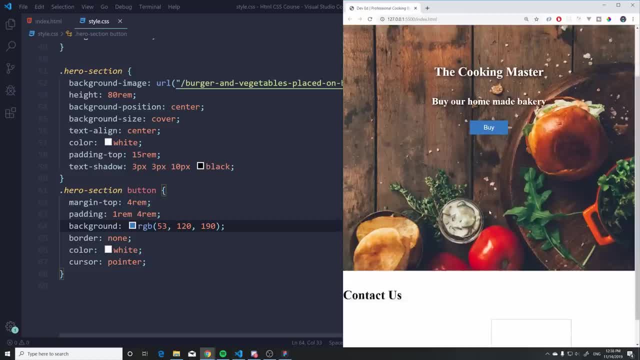 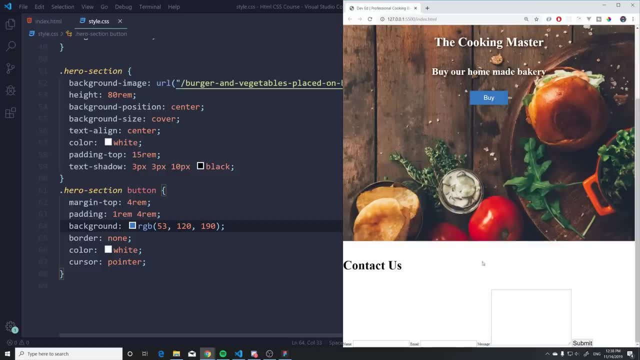 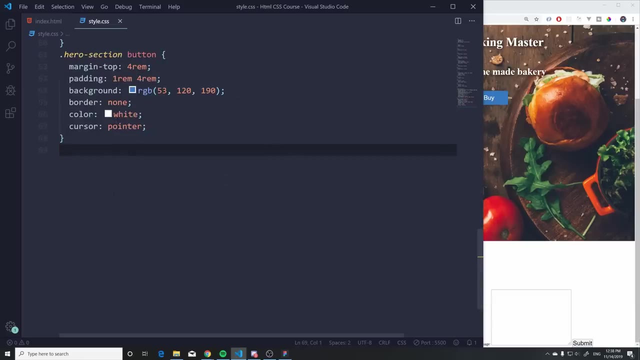 Okay, so that's way better. All right, so that's what we have. That's the section, And on the contact one, let's move down there. What we can do is also text align this to the center so we can get the form section. 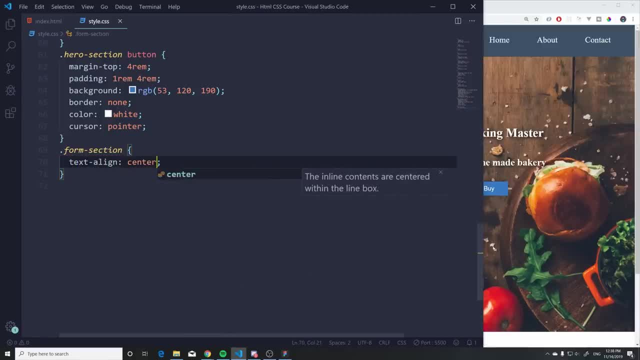 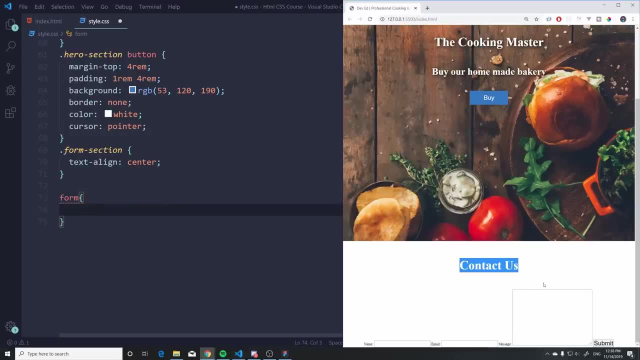 We can say: text align center. Let's take a look what that does. All right, so it aligns this to the center. Now we can get the form like this And, as you can see, these are kind of displayed in line, and this is not something we wanna do. 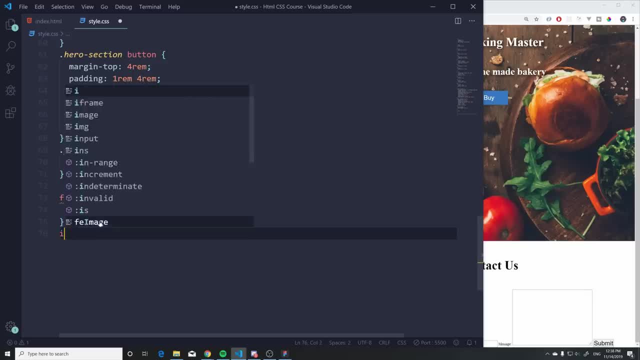 So what we can do is come down here and we can get the form input and the labels and the text areas. So I'm basically selecting all of them And make sure to add form to all of them. So form input, the form label and the form text area. 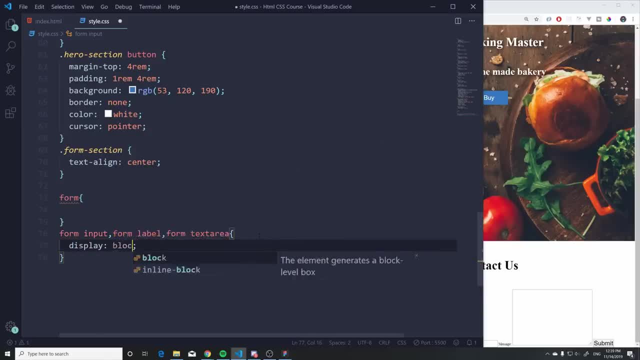 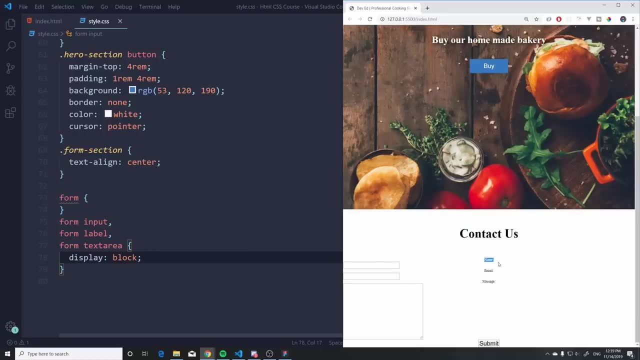 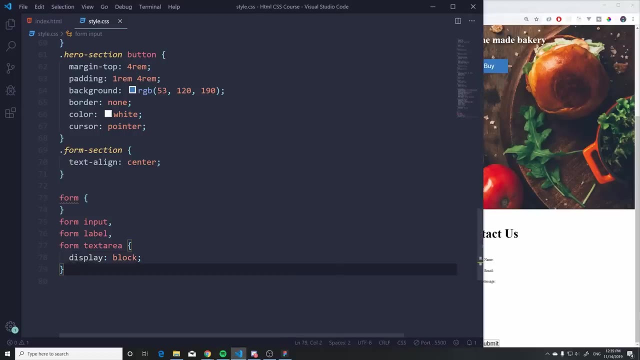 And we can grab all of these and add a display of block. All right, and now they're gonna be one underneath each other. Okay, so, as you can see, the text gets aligned here, but the inputs don't. So the way you can align that as well is: 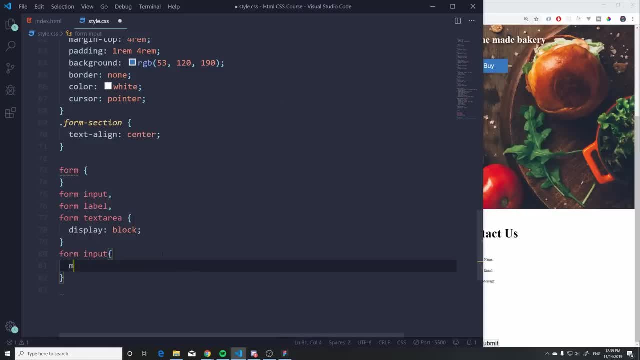 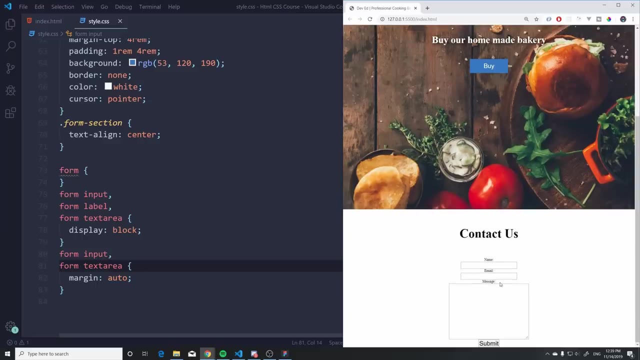 let's get the form input and we can add a margin of auto to this. Let's see, does that work? Okay, so that works. We can also do that to the form text area Like that. hit save, Let's go down here, and that aligns everything as well. 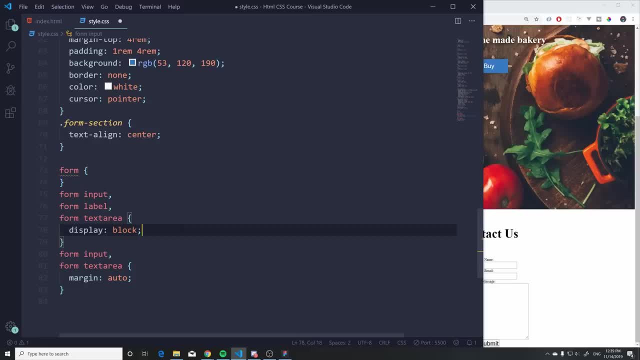 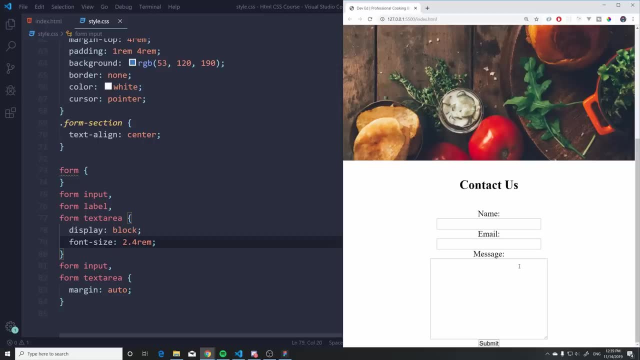 Let's also just get the. we can add the font size here. Font size 2.4, rem hit save. There we go. that's way better, way larger. Let's also add some space in between these. So let's go here. 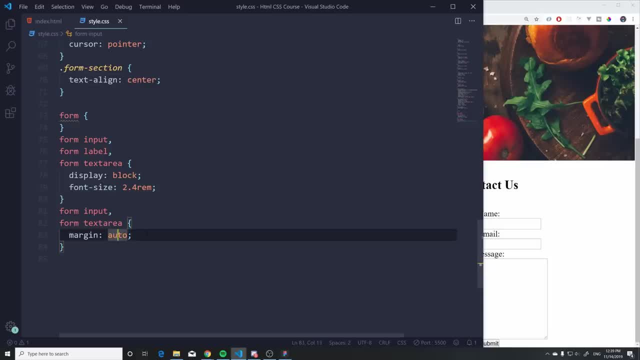 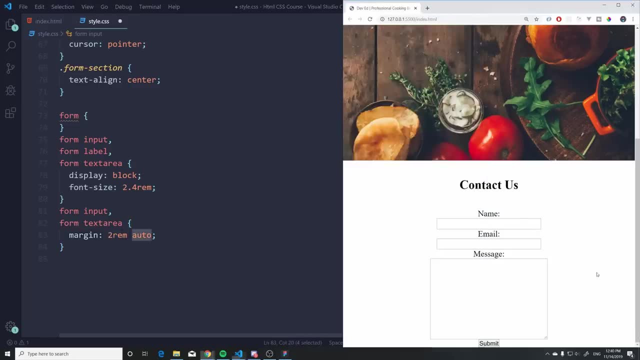 And add a. I mean we need margin on top So we can add another one here, 2 rem. So this is only gonna apply to top and bottom, but this is gonna take care of aligning it in the center. So if we hit save now, we have more space. 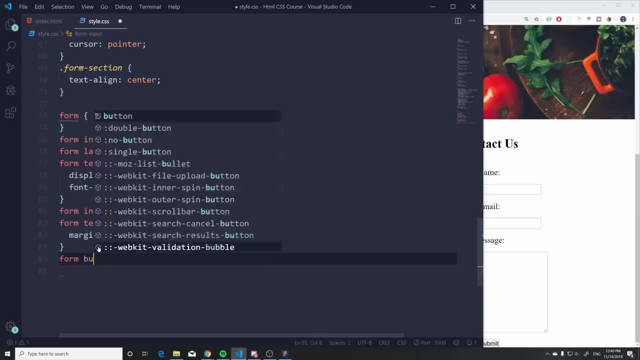 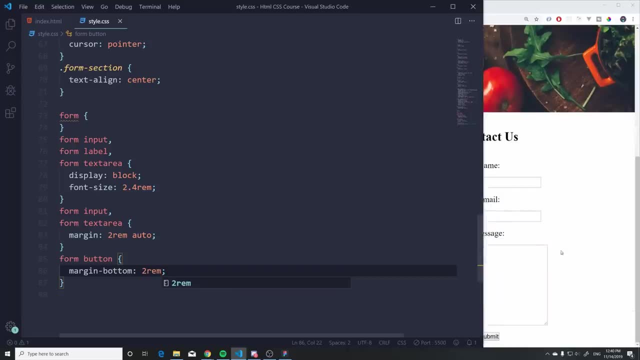 And finally, we can maybe add it to the button as well, Form button, and we can add a margin bottom of 2, rem, Hit save and there we go, we have more space Or something big like five. All right way, better 10.. 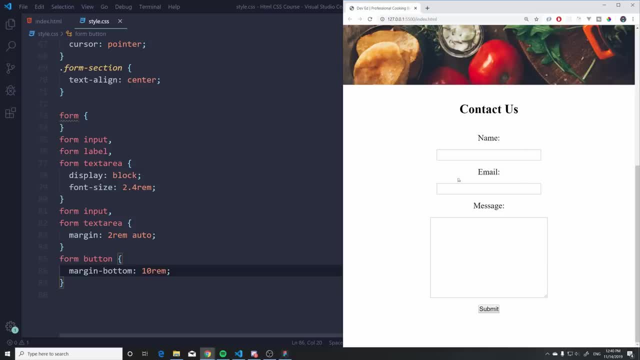 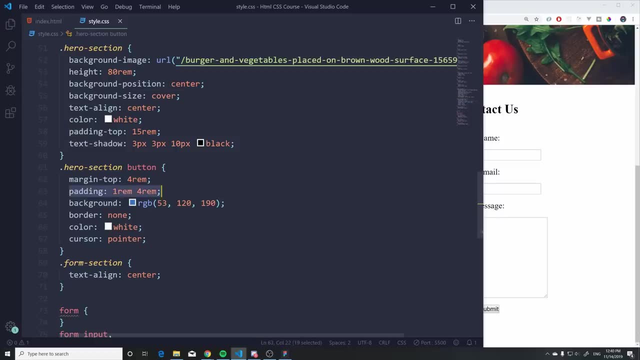 We are ambitious. Okay, perfect, that's what we want. So now we can style this the way we want For the button. we can also copy everything from here, So let's copy the padding, background, border and color and cursor. 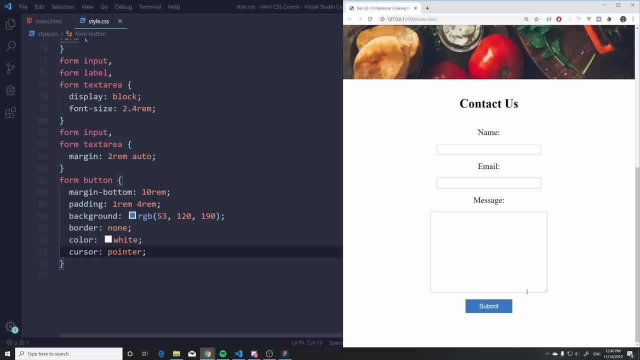 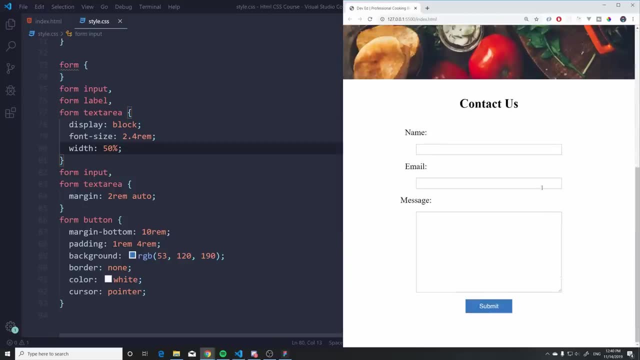 Okay, and bring it down here, Hit save and now we have that. Lastly, what I wanna do is come here and add the width to all of them, something like 50%, So they match the same size. As you can see, it takes up half of the size of the screen. 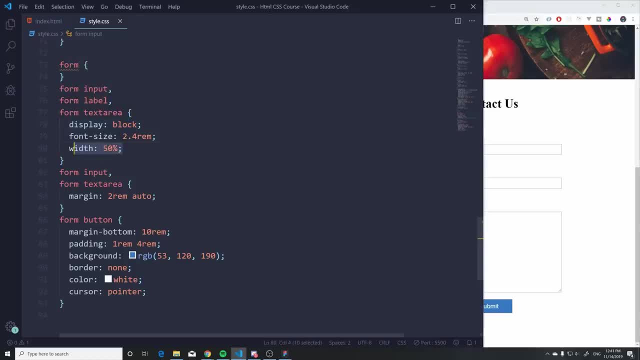 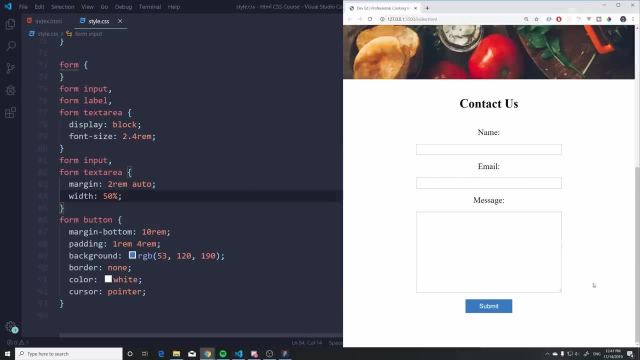 So that's good, but we added it. Let's just add this to the input and the text area. actually, Let's bring it down here. let's see how that looks. Okay, so that looks good. We can also add it to the button. 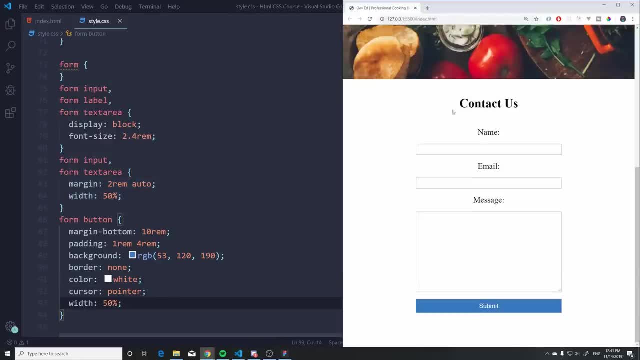 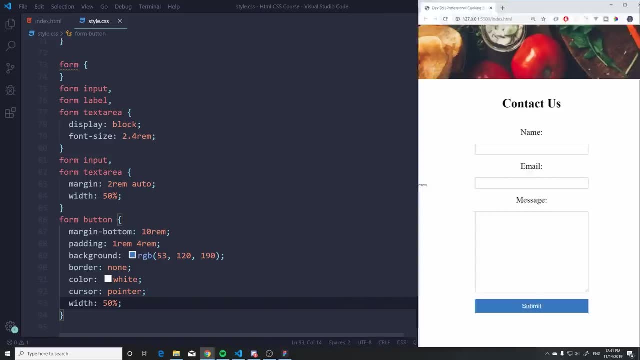 So let's add a width of 50% to the button, So it kinda matches the whole flow here. So there we go. that's how we can kinda throw together a website. Now is this responsive? Uh, kind of, but not really. 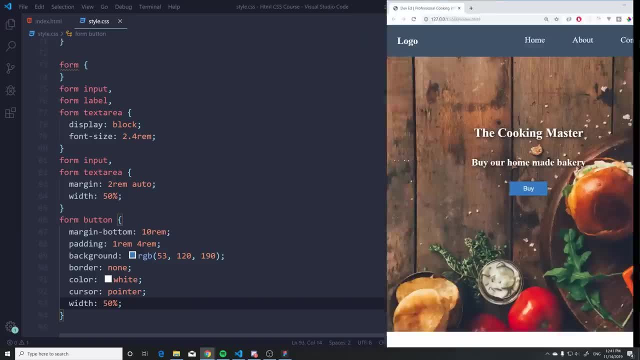 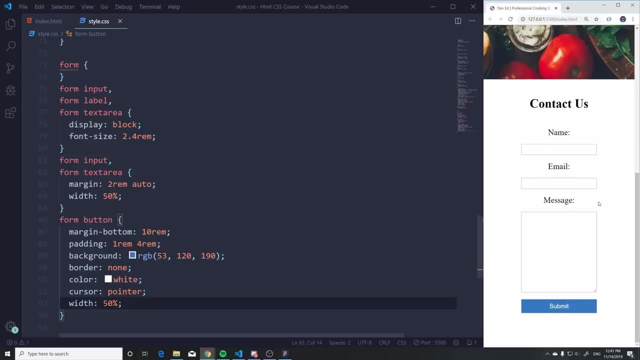 As you can see, when we go down here, that kinda drops there. it doesn't look that nice. And yeah, if this would be smaller, this would be super squished together here. So there are still a few issues here And also just making this layout is a bit. 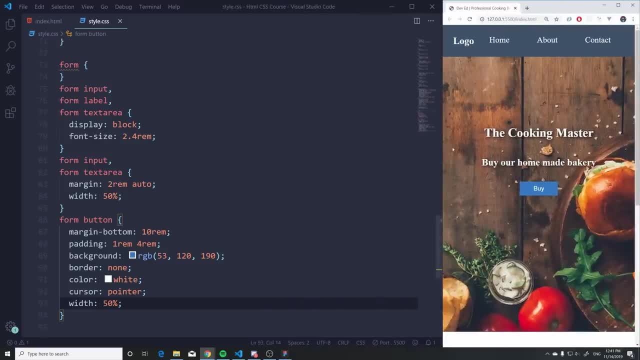 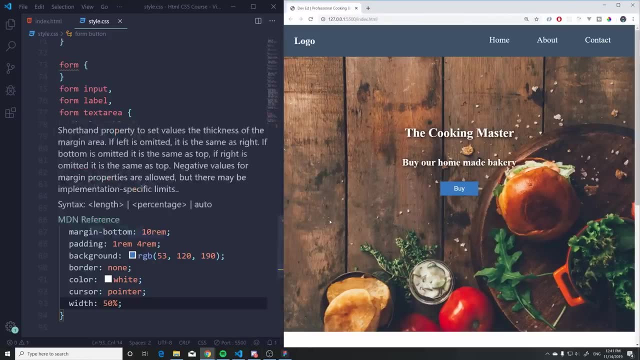 it's just not that fun using these floats and then clearing things, So next up we are gonna take a look at some better ways of doing things. So I apologize if this video is a bit long, but hopefully you learned a few things here. 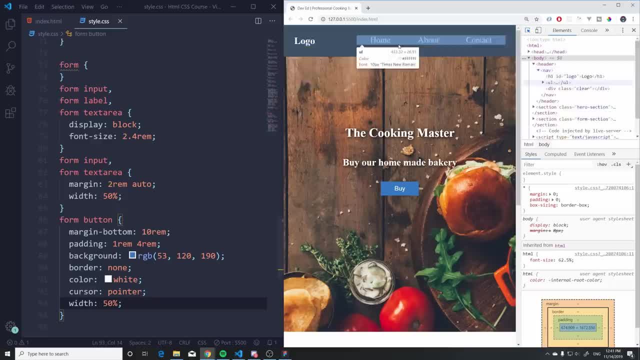 And also, as you can see here- I forgot to point this out- These anchor tags here are not perfectly aligned with the logo. here, As you can see, they're a bit more up there. So what you need to do now with this style? 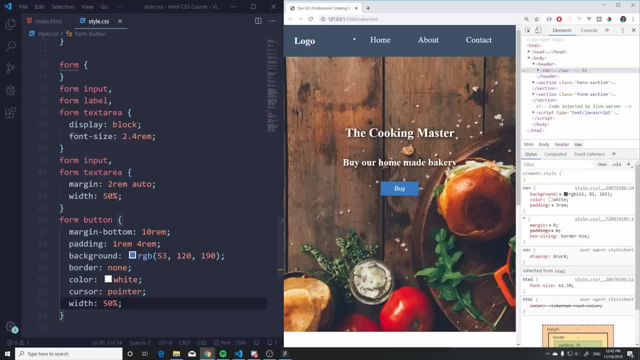 is to kinda match the padding. So add the same amount of paddings and the same amount of margins or paddings, So they're perfectly centered here. Okay, But again, this is kind of hard, So it would be nice if you would have an actual 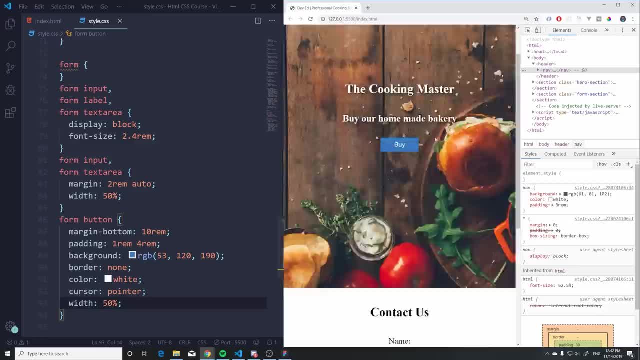 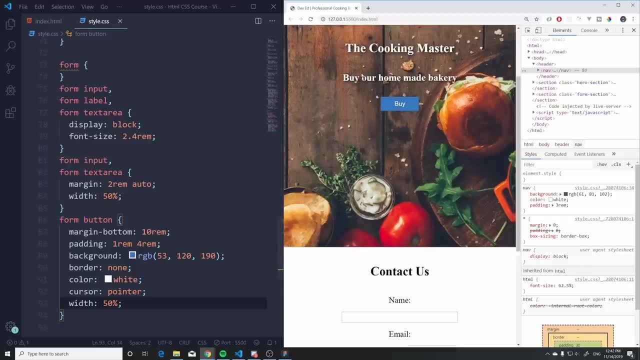 a better tool to make these layouts. And this is actually a very simple layout. It's a one column layout. We don't have multiple sections here. that's coming in one to the left and one to the right. It's just kind of everything dropping beneath each other. 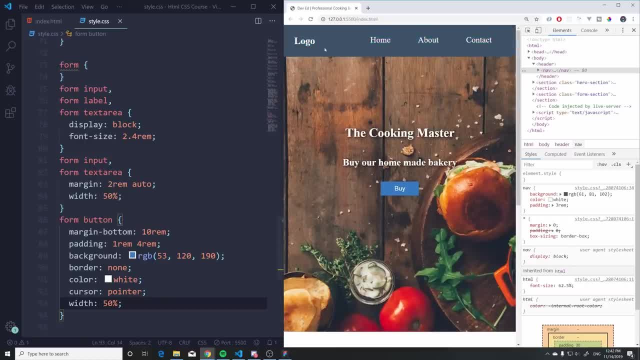 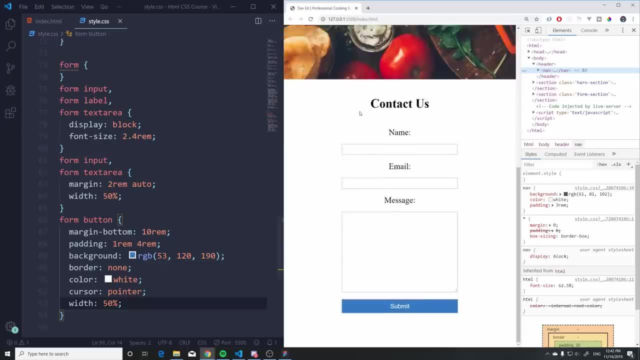 This is kind of the only two column layout we did with the logo and the UL here, So we had to float this. Other than that, we didn't really have to float anything else. Okay, stop talking, Ed. Show us the good stuff.